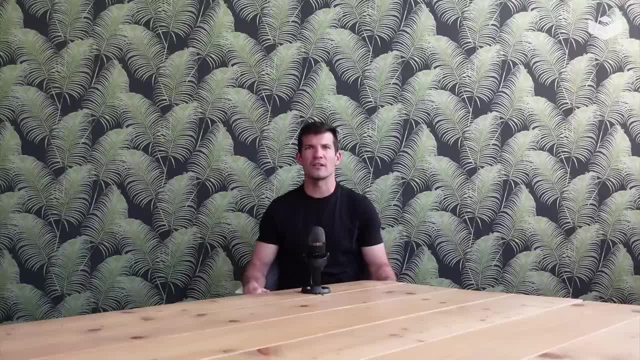 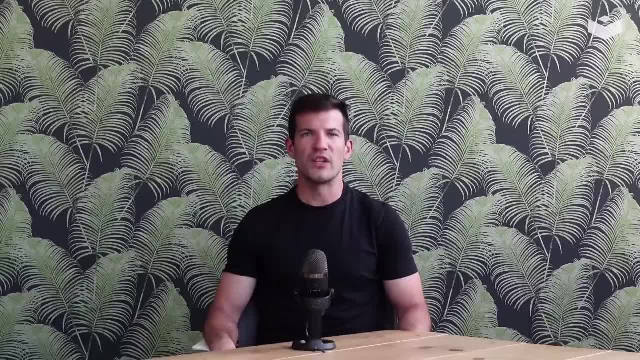 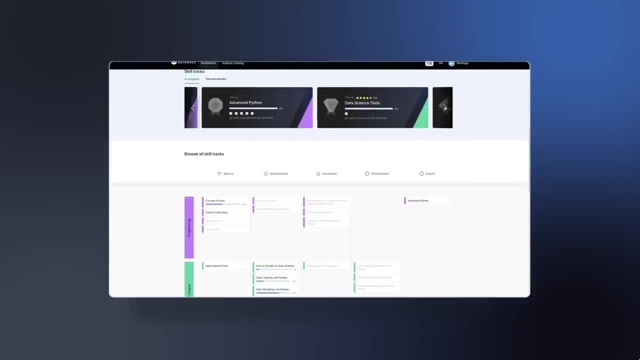 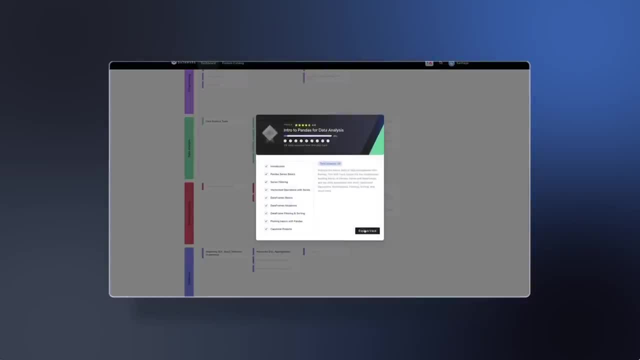 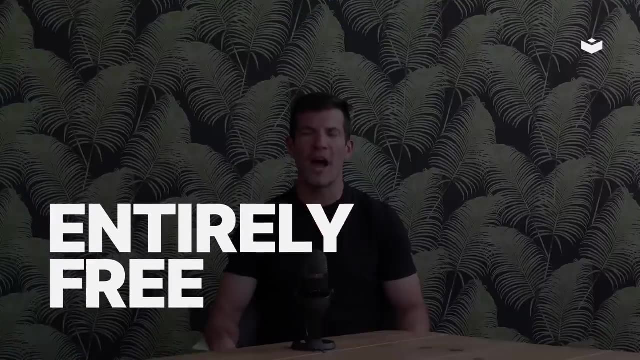 There are no videos, just projects to resolve with bite-sized activities that you can check at each stage of the process. The best part is that it's entirely free and we'll explain you how to sign up in just a bit- And this is also the reasoning behind this- by example series. 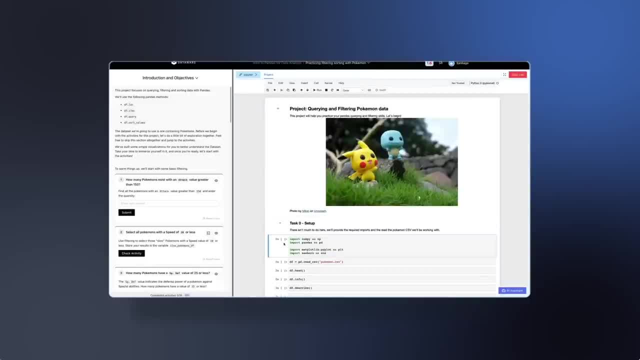 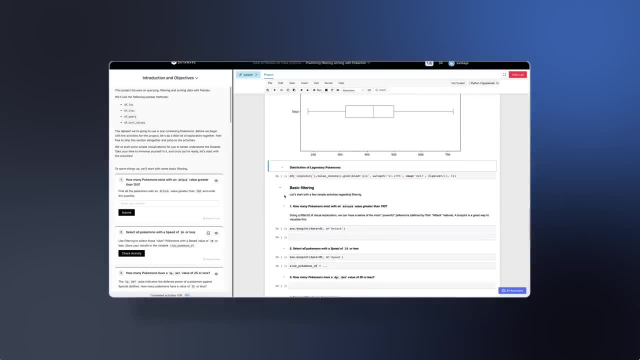 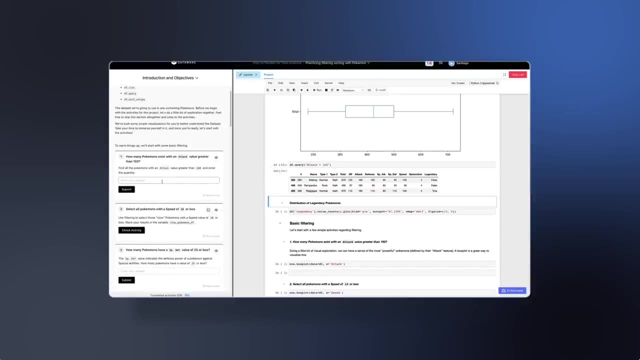 This video focuses on resolving real projects, brainstorming and discussing the solutions and the pitfalls along the process. We'll encourage you to try to solve the projects by yourself first. even pause the video before we reveal the solutions. We want you to put your skills to a test and challenge yourself. 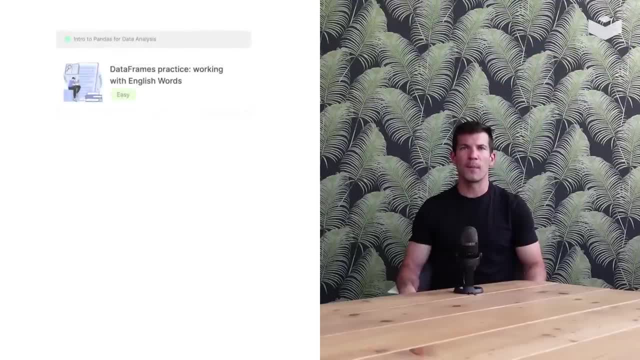 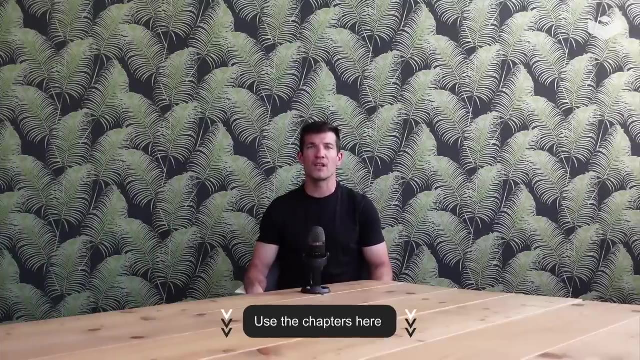 This video covers all the most important aspects of data management with pandas, including data analysis, data cleaning and data wrangling. Each project focuses on a different topic and the complexity grows from start to finish. We have separated all each project as a chapter and you can jump back and forth. As we've mentioned before, 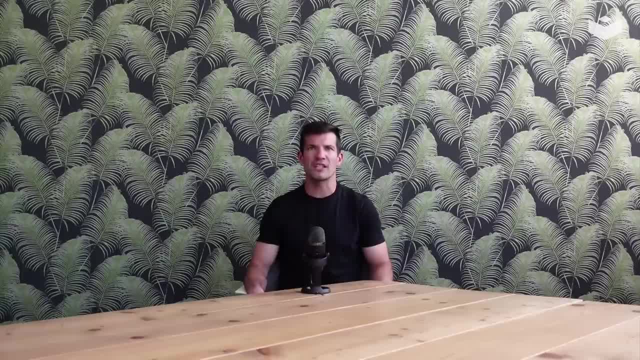 we encourage you to pause the video and try to resolve each activity by yourself first. You can find a list of all the projects we are resolving and the instructions to sign up at datawarsio slash freecodecamp. With all that said, let's just get started solving projects right now. 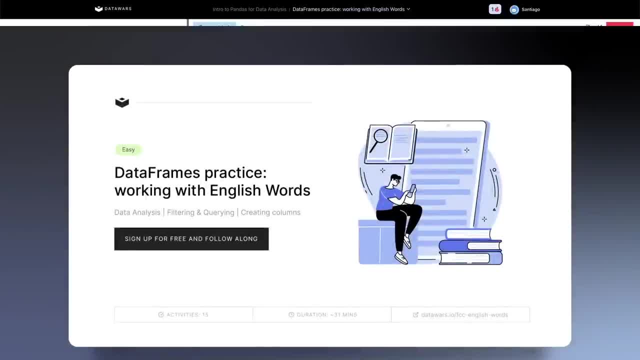 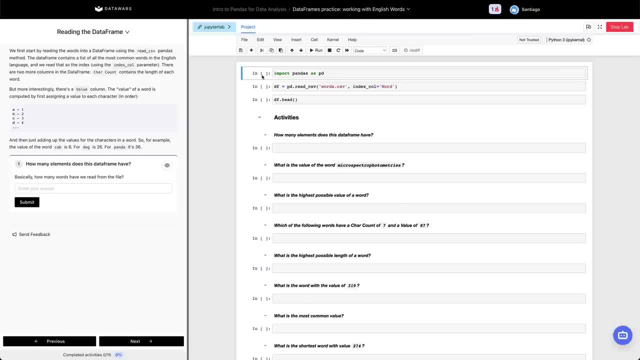 In this project, we're going to be practicing our skills dealing with pandas, data frames, We're going to be doing some selection understanding index selection, we're going to be creating a new column and we're going to do some statistical summarization methods And, finally, 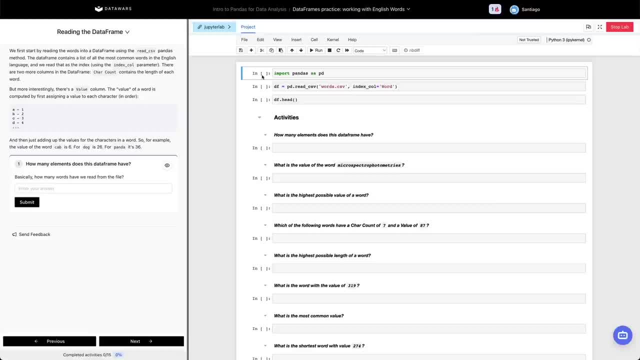 we're going to do some question answering by creating conditionals, Okay, so like selection based on different conditions or queries we want to write. So this is kind of on the simpler side for this series. we're just getting started with data frames again. 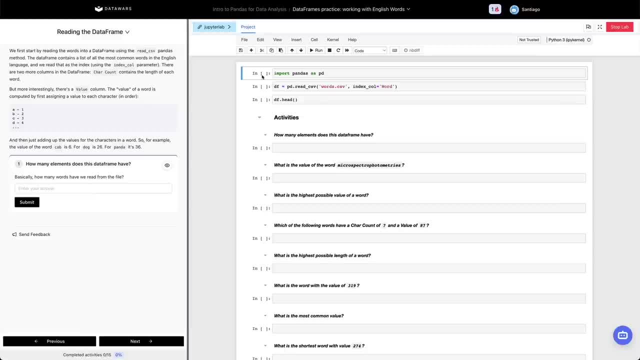 doing statistical methods, some selection by the index, creating a column, doing some conditionals and that's it. If you feel comfortable with these topics, just move ahead to other sections of the videos. you we get a little bit more, gets a little bit more challenging. As usual, I'm going to encourage. 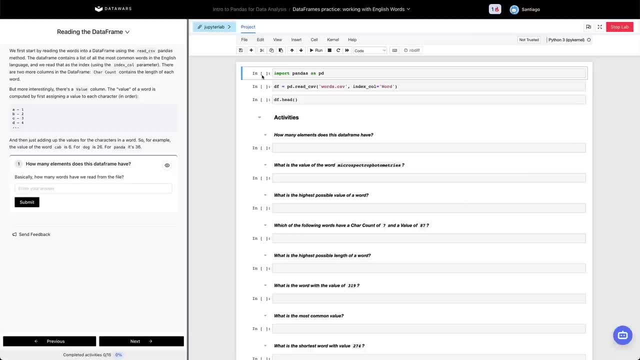 you to just pause the video before each activity and try to resolve it by yourself, So you can gain some of that application of the skills right. Worst case scenario: you can just resume the video and take a look at the way I resolve it And, by the way, there are going to be different ways of. 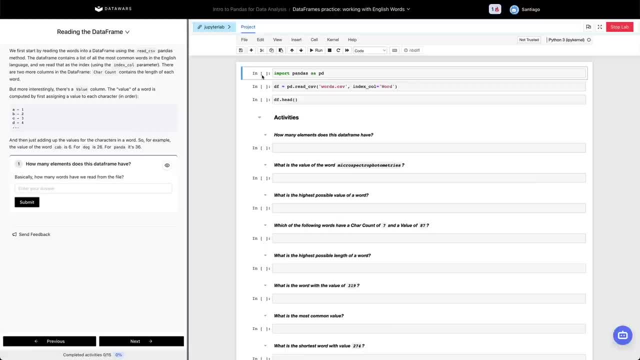 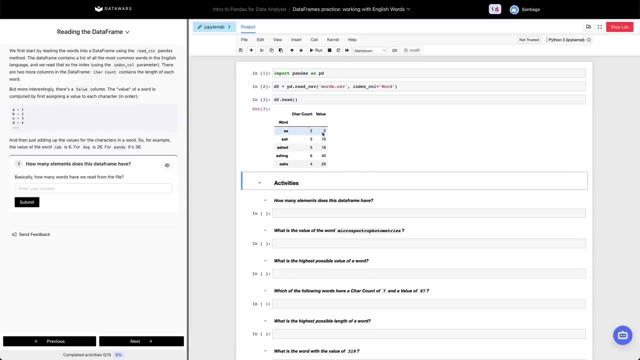 resolving these things, these activities, So you might even stumble upon something new that you do by yourself and I do something different, And that can be a very rich experience. So let's get started. This data frame, the data set we're using, is a data set containing a big 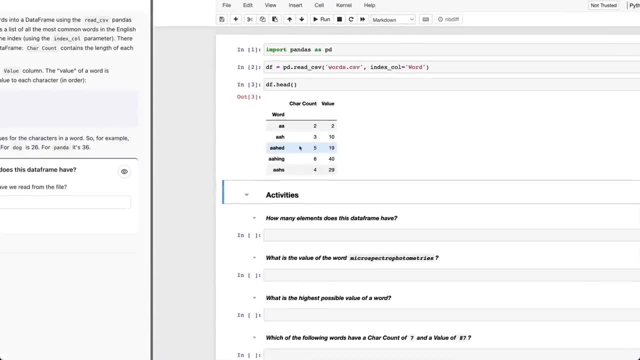 list of English words, And the index is going to be the word itself And we're going to talk about the index in a second. And then we have two columns: chart counts or character counts, and the value of the word. the character count, that's easy, it's just the length of the word. 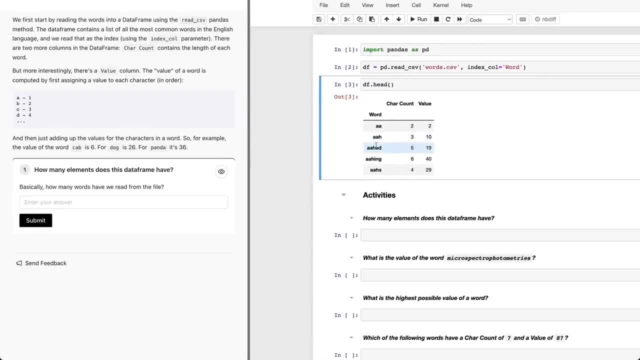 that's it, And the value is computed by adding up all the individual values of each character, And the individual values are just defined in this way. So A is one, B is two, C is three, etc. So in this case is one plus one, one plus one plus the value of H, which I don't know. 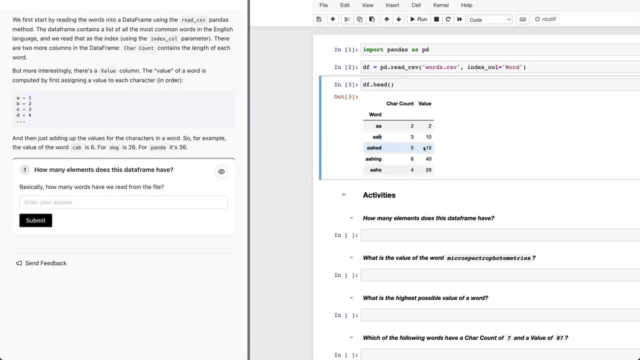 where is H 1011.. Whatever, Actually, we know it is eight, because this one with plus one is two and the value is 10.. So H is probably the word, the a, the criteria number eight, And that's it. this is already given. So we have already read the data frame. 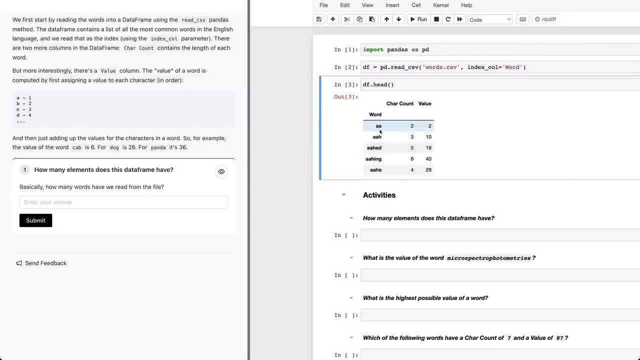 and we're going to get started with some activities. The important piece about this data frame is that the index is the word, like the words themselves make the index. So whenever we want to call it, we're going to do this and then call it an index. 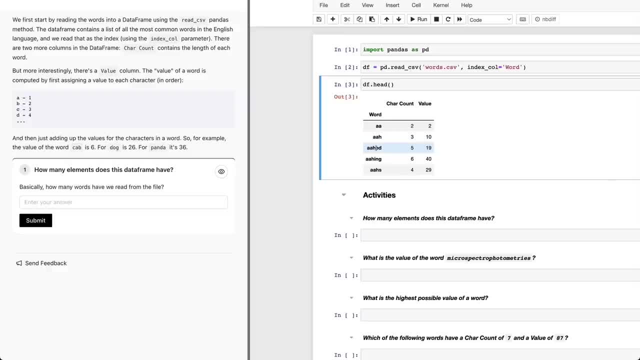 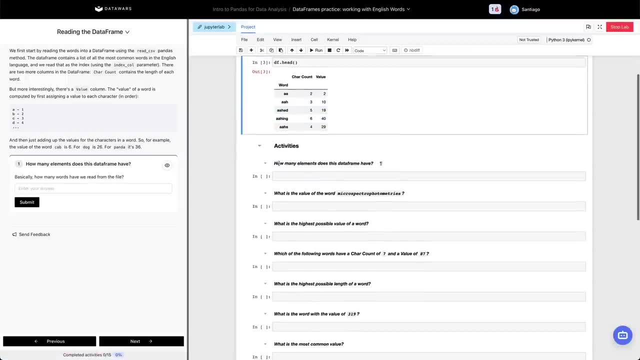 to access a given word. we can just do it by the index, And this is why it's so important to understand how indices work in pandas. So let's get started right off the bat with the first activity, which is: how many elements does this data frame have? there are multiple. 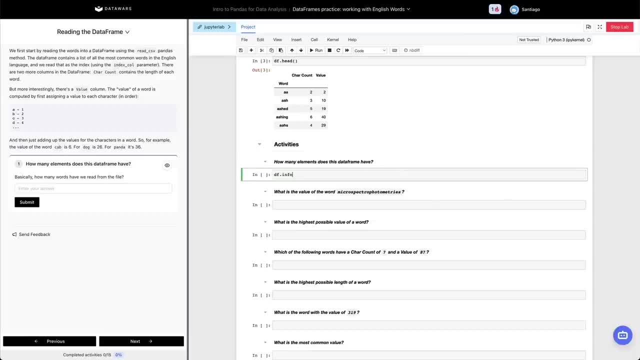 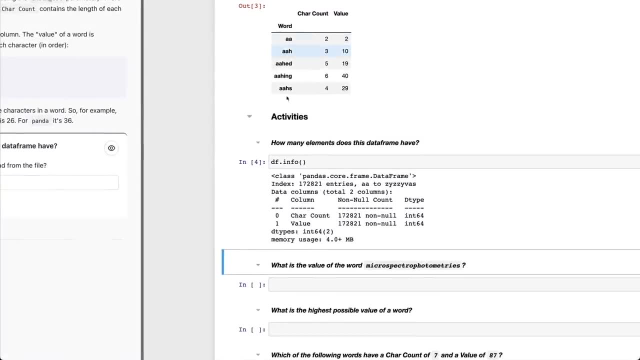 ways of answering that. the first one is with the info method, which is one of the most common ones. pretty quickly we go with info and it gives us an understanding of the index. it tells us that the index, just an index, with entries that go from AI, and that's it to. 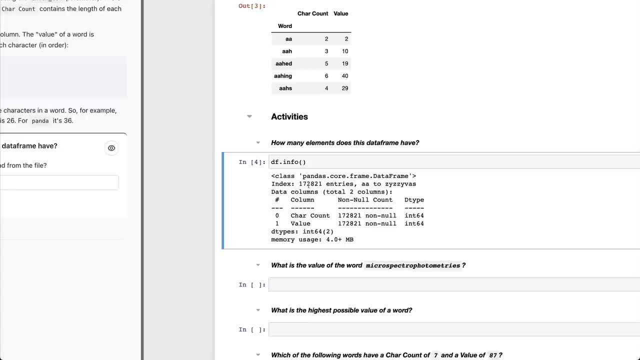 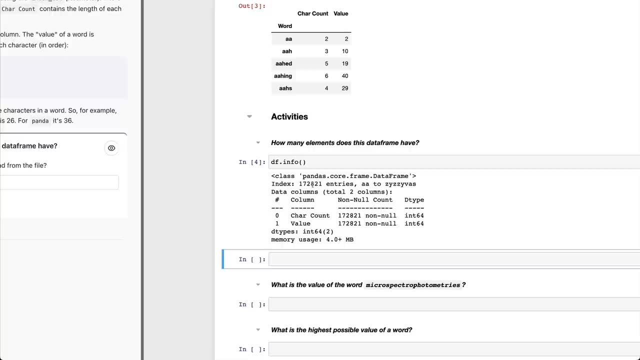 these word, which I don't know what it means, And we have a total of 1171, 172821 words. we can also use the shape method. This gives us kind of the shape of the of the matrix, if you want, in the data frame, and of course the values are the same. So we're going to 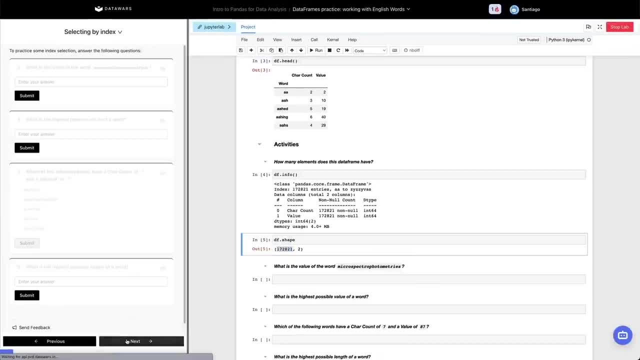 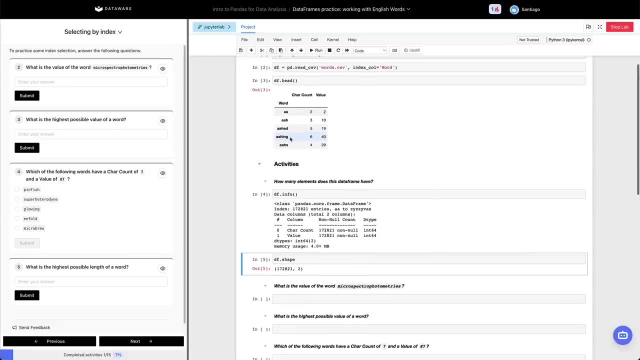 plug this one in and see how it works. Thank you, goes, there you go, it works, Okay. moving forward, what is the value of the word? this thing that I'm not going to even pronounce, And this is a very interesting activity Because 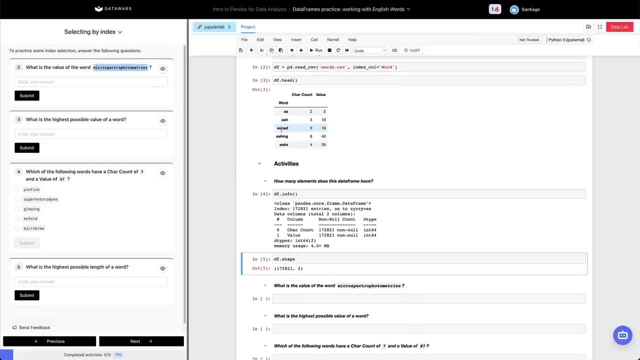 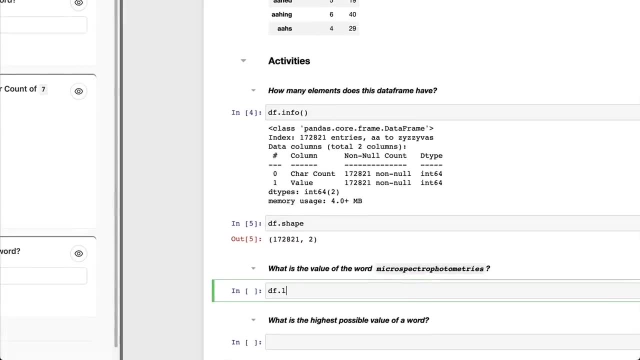 remember we're going to be doing selection by index. So, as the index is the word itself, I can just use the dot lock method- And this should be familiar dot lock- that does index selection. So we can just pass whatever value I want for an index using the dot lock method. 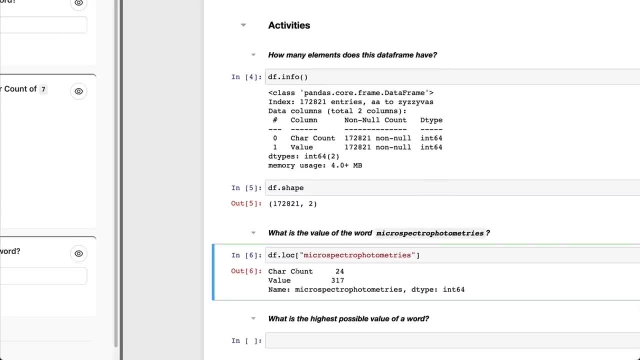 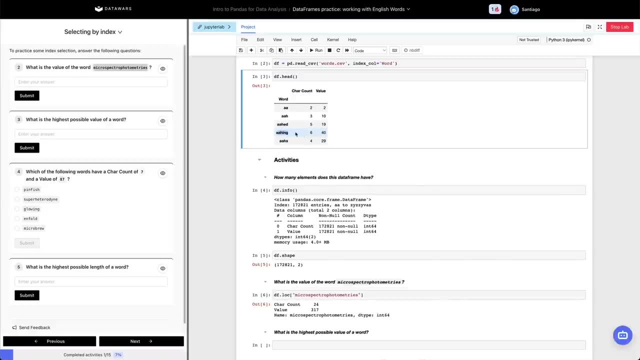 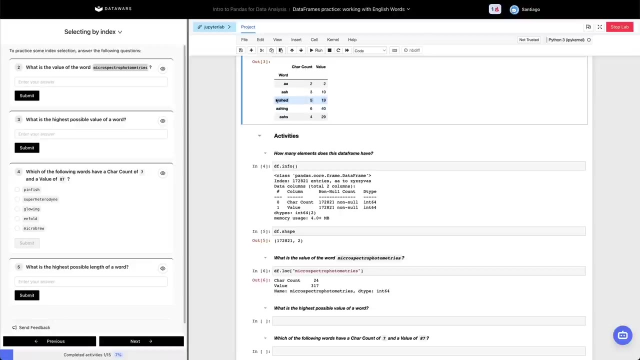 And that's going to give me the results. In this case it gives me the, the row itself, the entire row. So we did like this row selection, but the result is in a series. So the projection, to put in a way the result of row selection, which is kind of horizontal structure, is going: 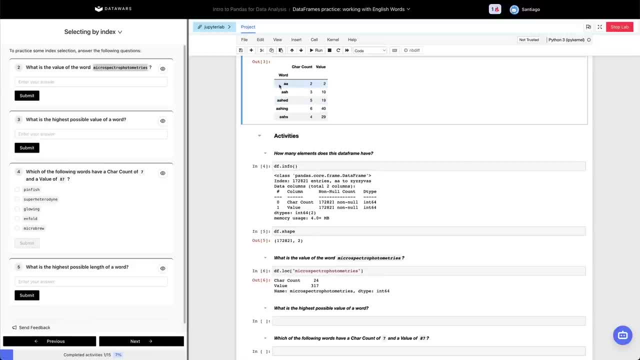 to be a vertical structure which is a series. Right, you see the shaping, right the, the transposing operations. like we go from something that is a row to something that is a series and it's not pretty special. don't pay too. 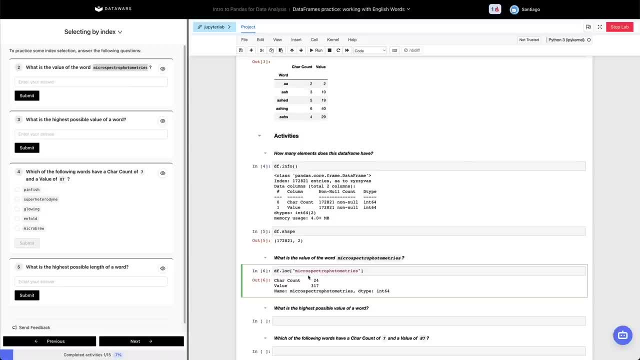 much attention to. it's just to refer to the fact that the row is represented as a series, And here we can see that the value of these word is 317.. Something also very convenient if you're doing selection is that the left dot lock method- and we're going to increase here the size- the f dot lock accepts to. 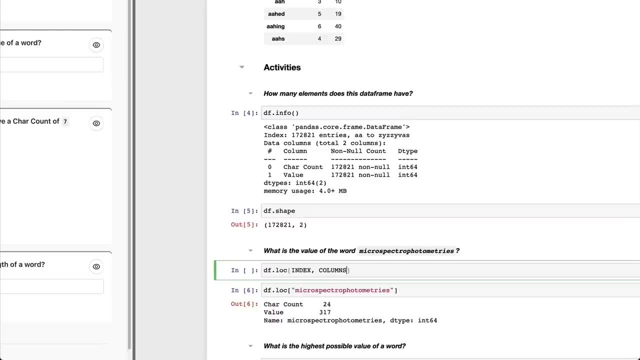 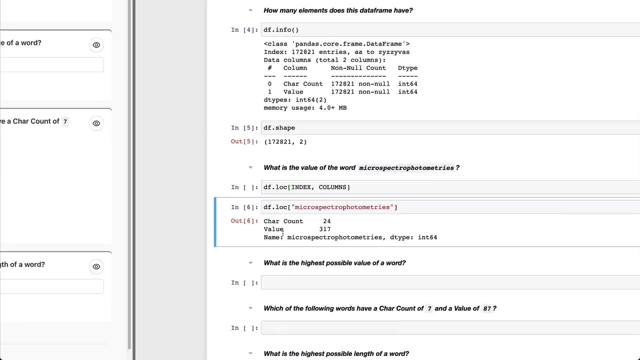 parameter, the index selection, and then the columns. right, Why is that? Imagine that we have 100 columns. it's going to be very hard to just, you know, browse, scroll to the value we're looking for. you can just pause here what the column we want to use. 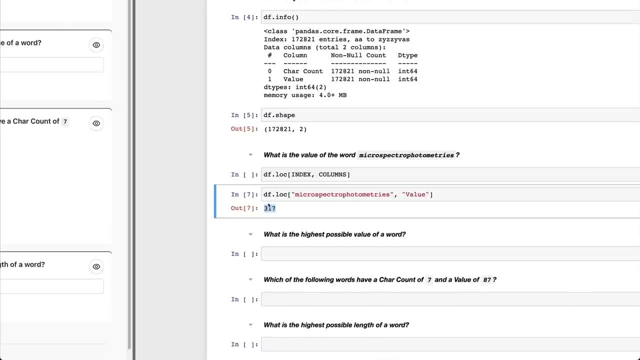 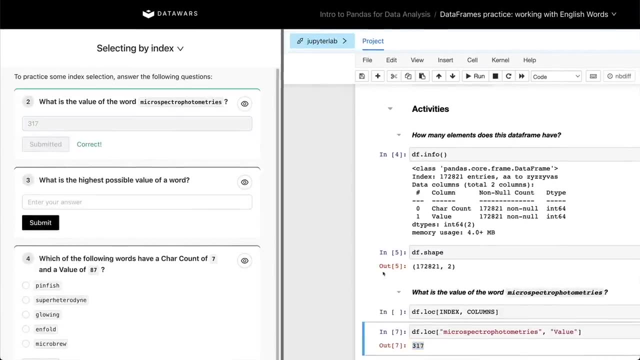 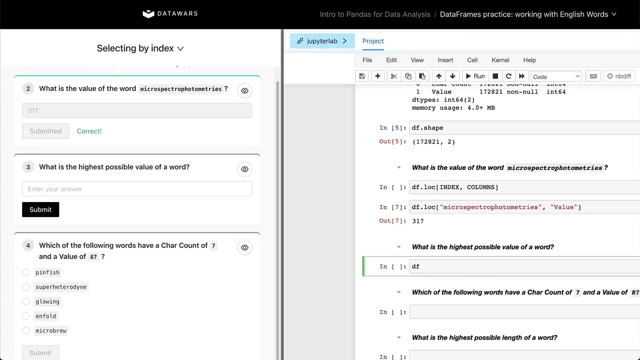 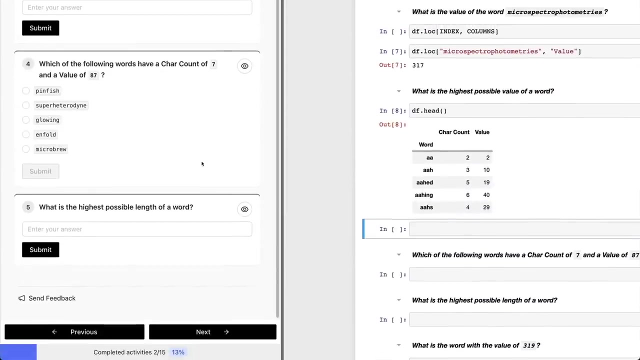 In this case, we're going to use value right there And the value is 317.. So let's go ahead and try it, And it worked as expected. What is the highest possible value of a word? DF at that? we're going to use two methods. let me show you once again: data frame- what 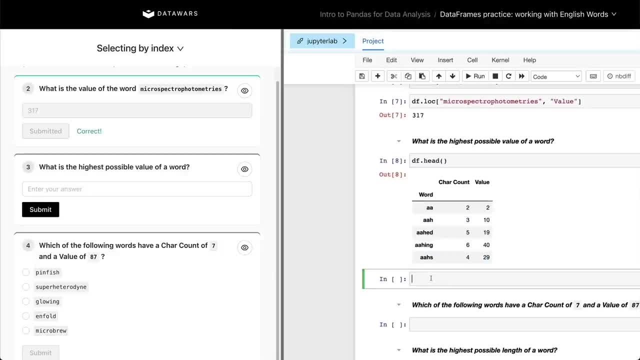 is the highest possible value. we can do DF at the value and do a max method. right, that's going to give us the maximum value there. Or we can just do the F dot max. You can just to have the max statistical method computed for the whole data frame, right In this case. 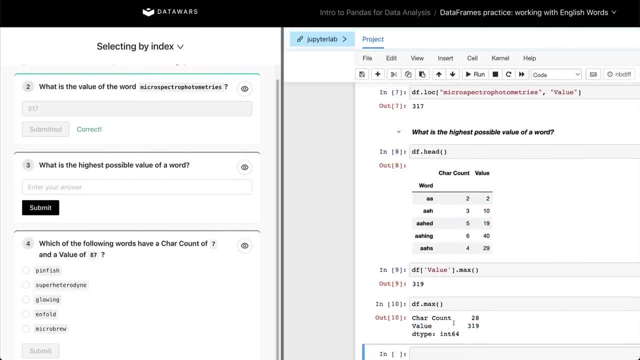 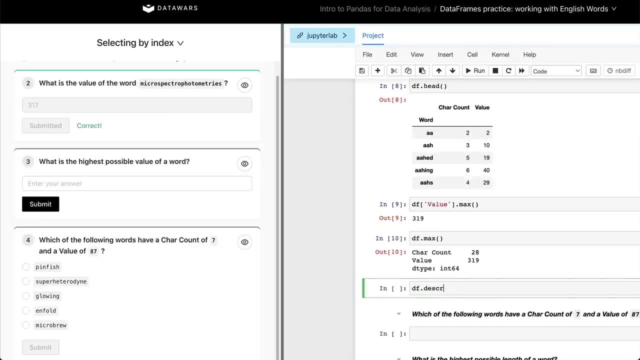 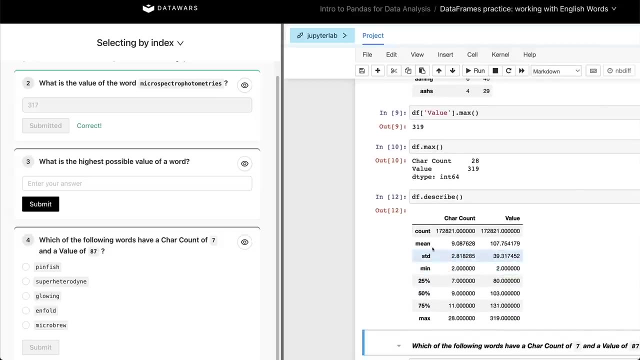 we see again the value 319, or something that is pretty common is: do the f dot describe. And this method is just going to give you this tribe. There we go. Oh, auto completed. It's going to give you some more statistics of all your numeric columns, In this case, 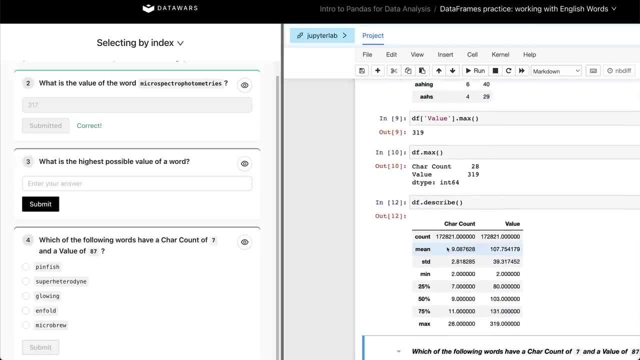 we only have two columns and both are numeric, So we're good, And it gives you some more statistics of all the values right there. So, for example, the average value, the average chart count, you know the, the minimum value, the maximum value for character, count the. 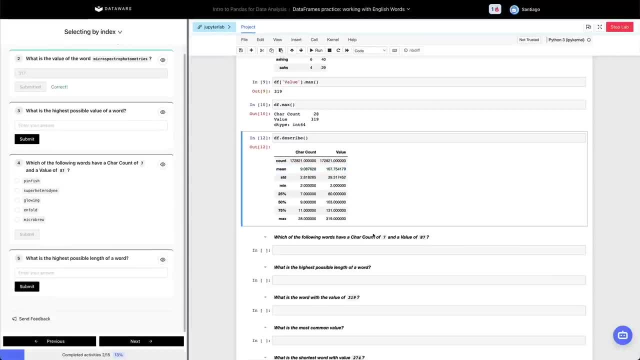 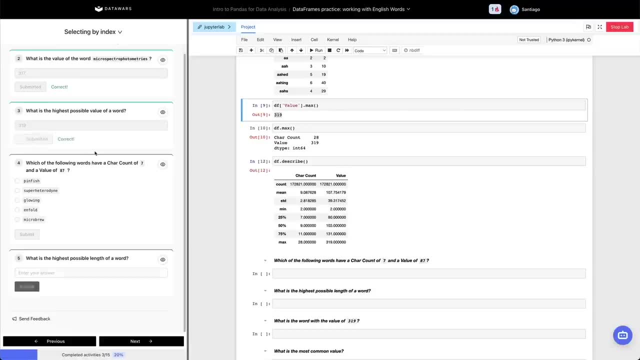 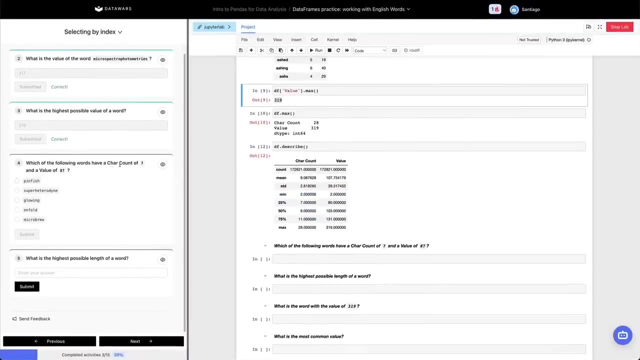 maximum value for value, etc. it's gonna give us some summary statistics. So I think we have multiple methods. we're gonna go here with 319 and submit the activity, And that worked. Now the next one, which, of the following words, have a chart count of seven and a value. 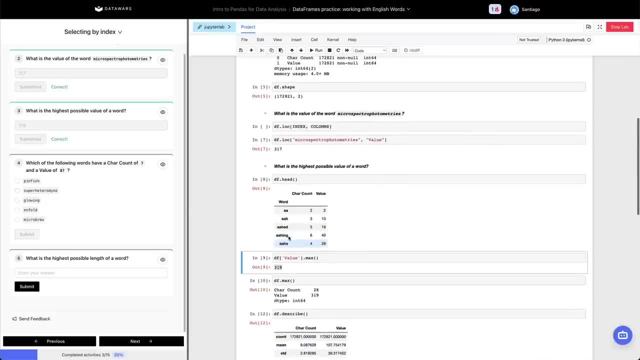 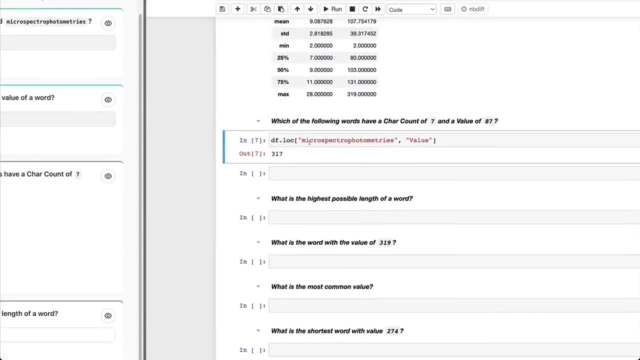 of 87. And this is pretty interesting because in the way we did selection before- I'm gonna copy this thing right here- we, the way we did it before, was just by passing one value of the index. we were, we worked with just one word, But selection in pandas, the f dot. 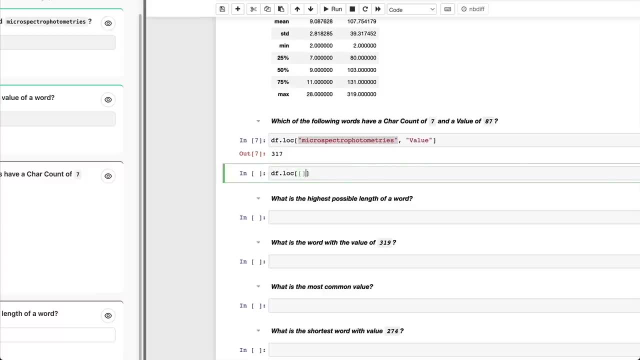 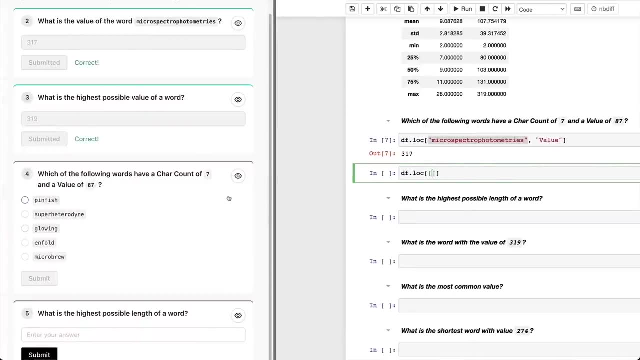 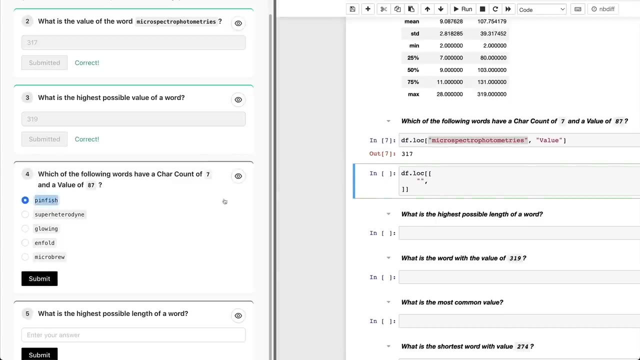 lock here takes potentially a list of index values to retrieve. So here, instead of passing just one value, I can pass each one of them, And there's going to be a little bit of an annoying procedure. I'm going to just copy and paste all the words here. you feel free to fast forward, I will not copy. 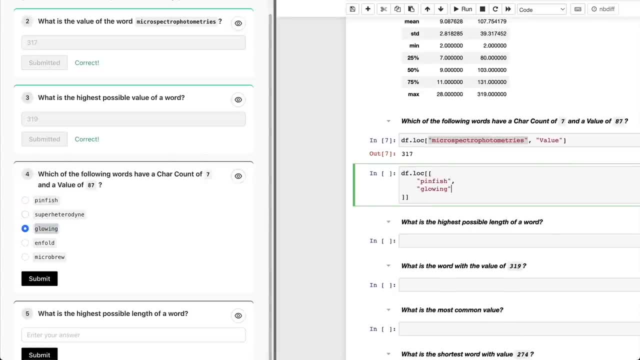 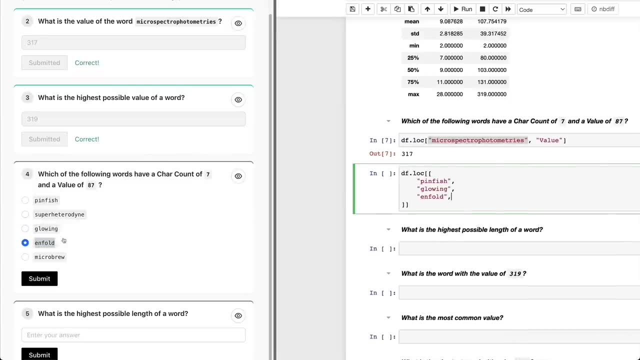 this one because it definitely has more than seven characters. just gonna you know quickly and see which ones have seven characters. I think this one has more than seven characters, but doesn't matter, So let's add it anyways. And now you can see that with the f? dot lock you can actually 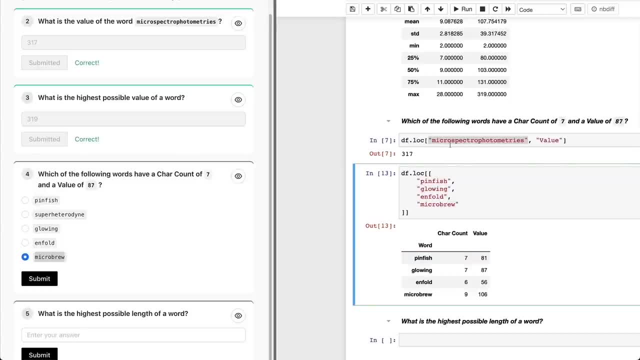 pass multiple indices if you want to get multi selection or just one, you're going to select just one individual row And to answer the activity, which of the following words, have a chart kind of seven and a value of 87. It's glowing right here. we can just. 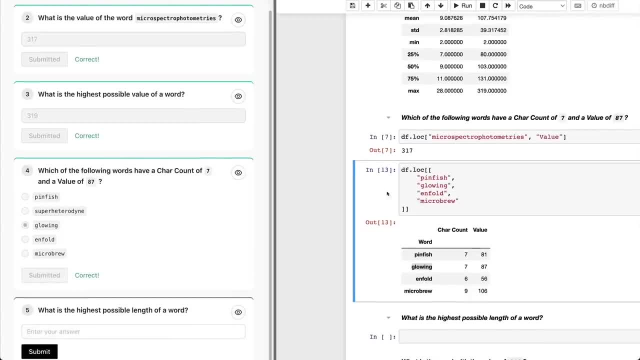 put here glowing and submits And that worked. Just a comment: As we were saying, we're going to do it before. the first elements, in this case is at list, is the list of indices to select. the second one could potentially be just the column, So here I could say value. 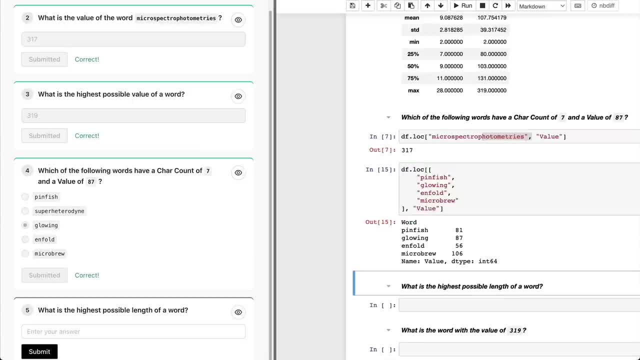 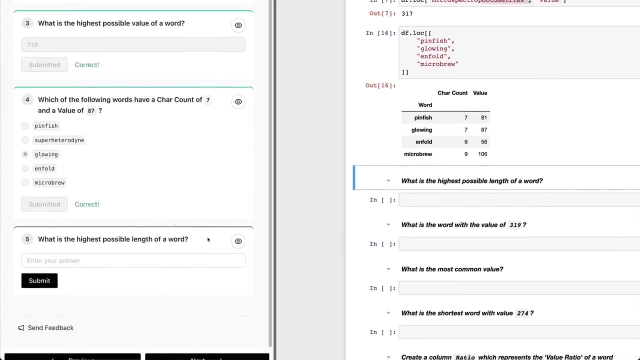 for them. oh, I missed a square bracket And I just get the value for each one of these rows. Of course, in this activity we did both the chart count and the value, So that's why I didn't do it, but just a clarification. So what is the highest possible length of? 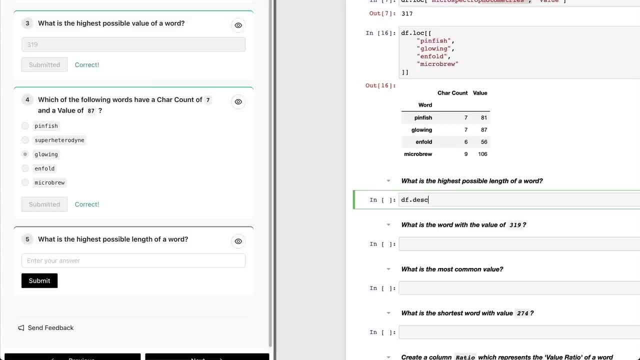 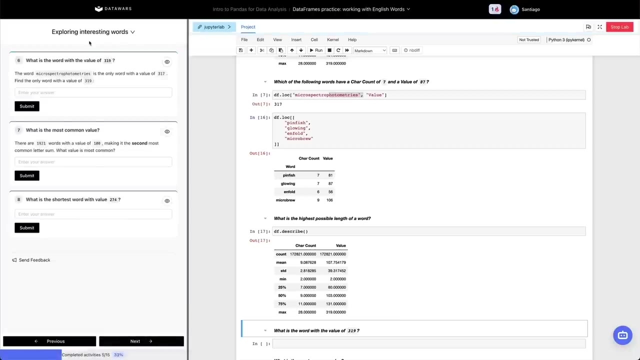 a word. we did it before with describe, we're gonna do it again and chart count. the maximum one seems to be 28.. There we go, Moving on to the next section, which is exploring interesting words. So we did before this activity. there was that, the, this word, and I'm not gonna pronounce. 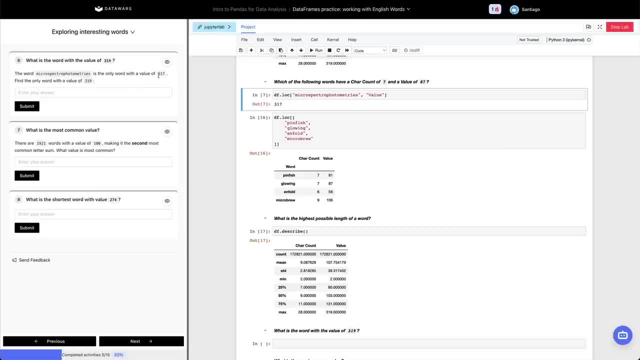 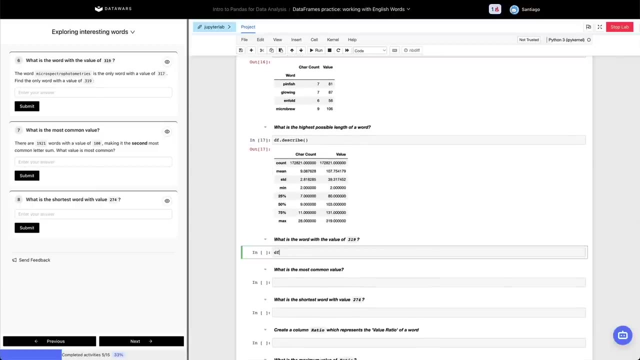 is the only word with a value value of 317.. Find the only word with a value of 319. And there are multiple ways of solving this one we could. let's. let's say we do some sorting first is not going to be the most. 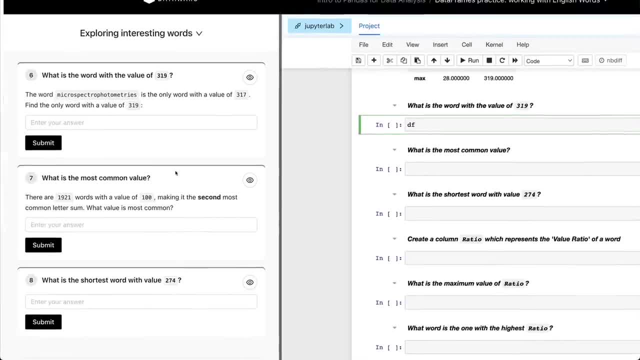 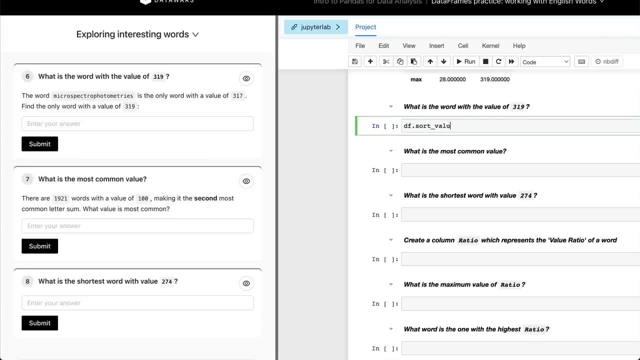 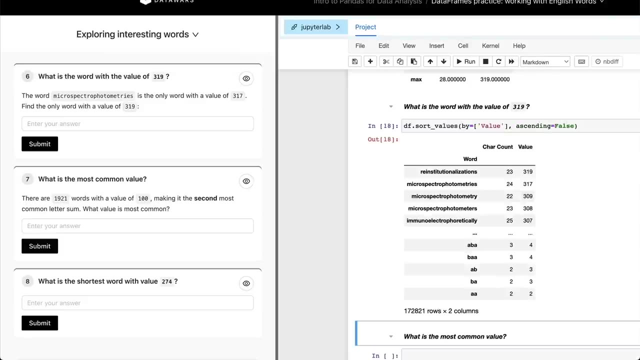 effective way. But let's do some sorting. Let's see if I can put everything. the same frame, df at df, dot. sort values by and value it's gonna be. I'm going to see ascending false In this case, as this word was the one with the highest value. just by sorting we were able to reach that result. 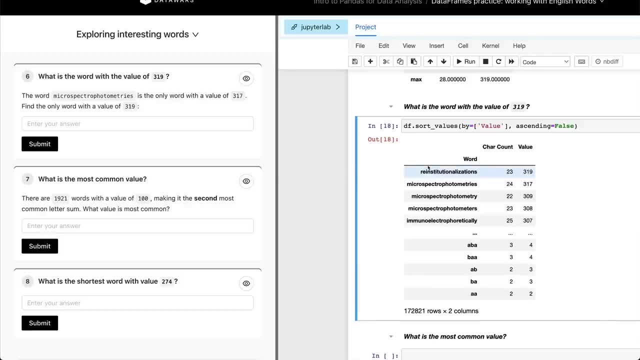 But of course that is not always the case. what happens if here it's asking us for, for I don't know the value of 18. And that is clearly, or Even worse, 50. It's clearly in the middle. I have to just, you know, browse the data. 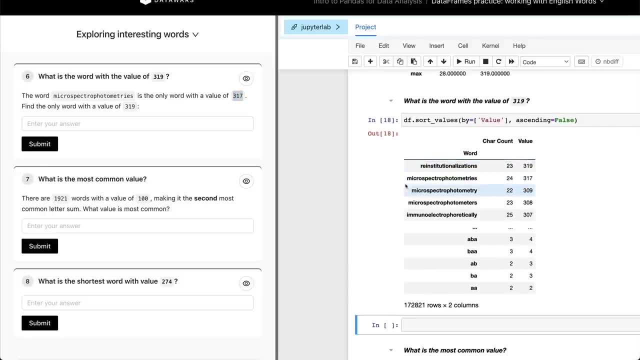 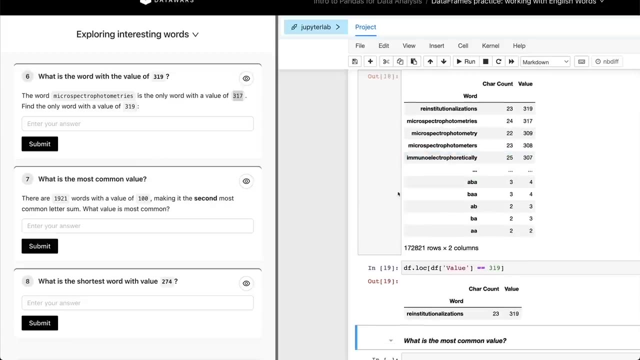 frame to find the correct answer. In this case, what we need to do is some selection when we need to do df at. I'm going to do the whole syntax and we're going to explain it later. dot log, df at value: it's going to be 319.. And this is the first idea of conditional. 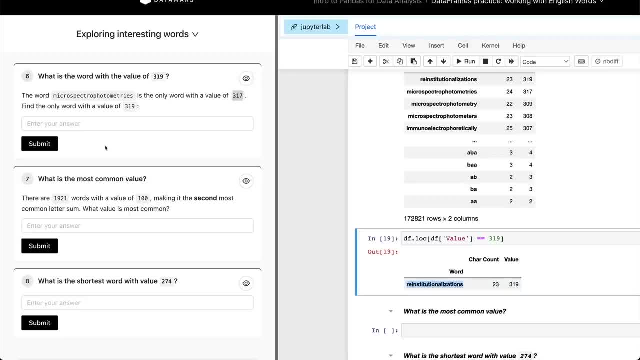 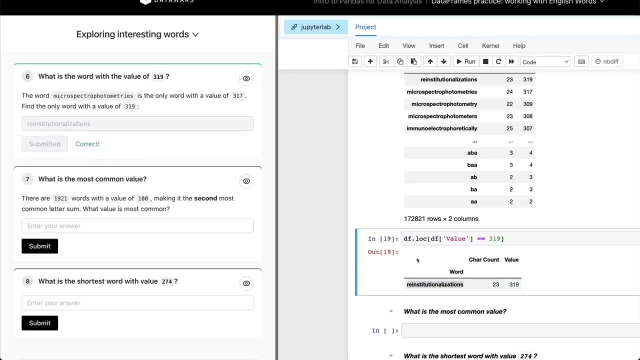 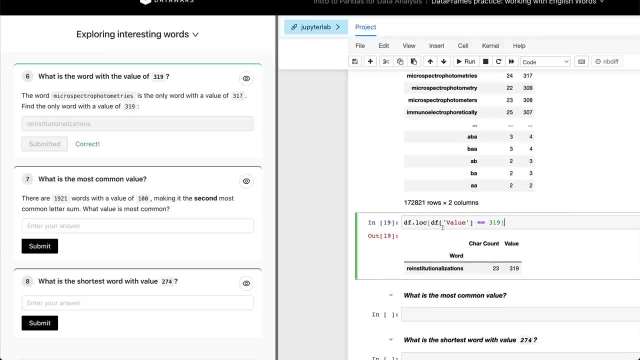 going to plug it in, see if it worked, And if we have a good activity, there you go. It worked. Now, how does this then work? Remember that whenever- I assume you have worked with this before- whenever you have these operations in pandas and if you haven't check out some 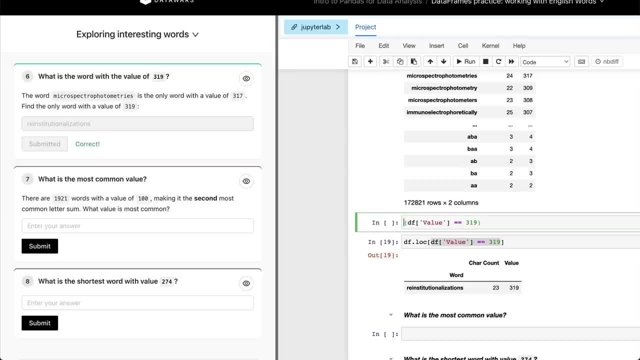 other simpler projects we have in the platform that explain this in more detail. The idea is we are performing this operation that returns a Boolean array, right. So again, refer to the project in the platform. we have, you know, very, very thorough step. 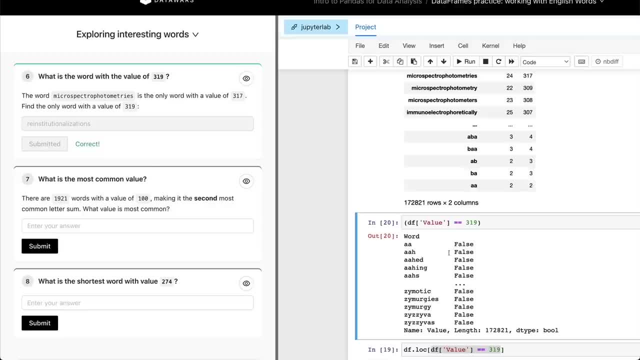 by step process to explain these topics, But basically this: creating a boolean volume as saying select this word, select this word or select this word and indicating if we want to retrieve it or not with a false true value. So in this case we don't want the AA word, we don't want the AA H word, etc. 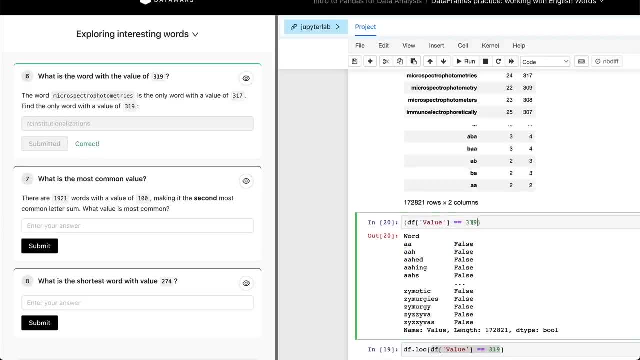 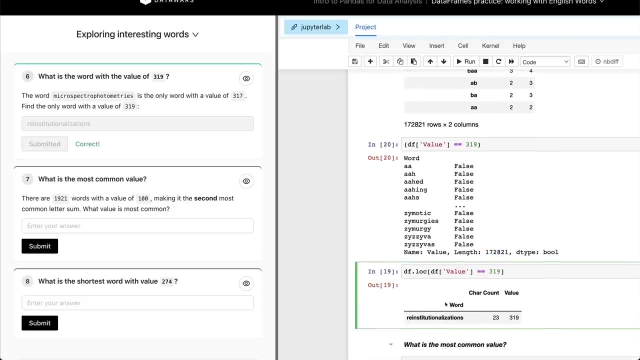 But the ones that fulfill or match this condition will have a true value here. And this case is a long boolean array, is a 172,000 boolean element boolean array, And there's just one true volume, which is the one for this work. 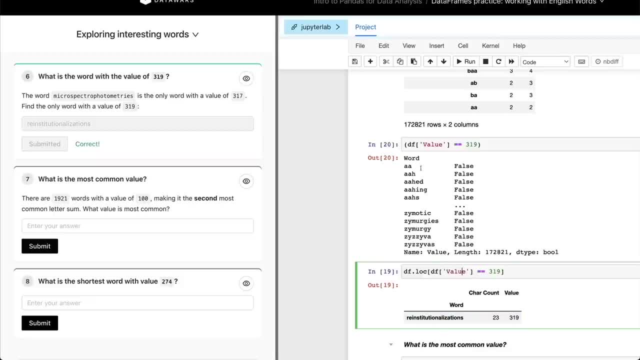 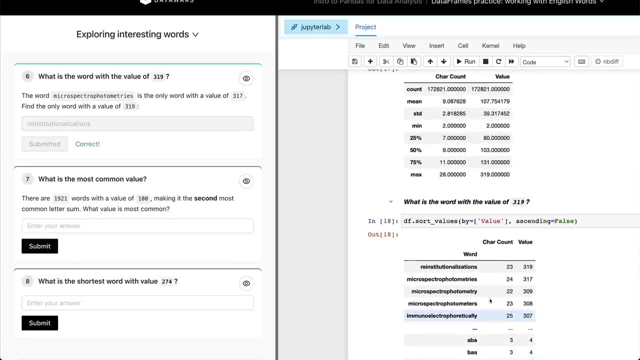 So once these boolean array is resolved to put it away in memory, we pass that boolean array to dot lock method. That's returns Okay, That returns the value. So here is to kind of wrap it up with this idea of dot lock. we have three ways of doing. 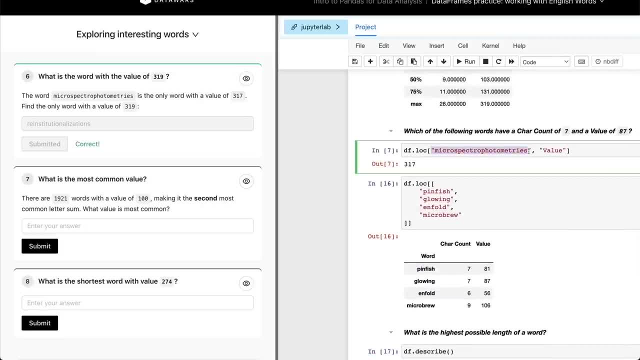 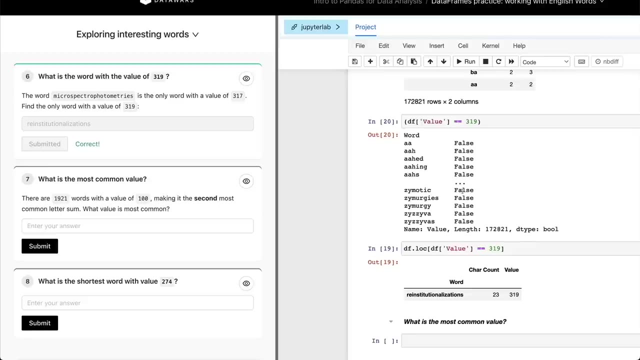 dot lock. we can pass just one value, as we did before For the index, right, we can pass several values for that match the index. or we can pass a full boolean array indicating which elements, which rows, we want to select by just putting a false or a true volume. 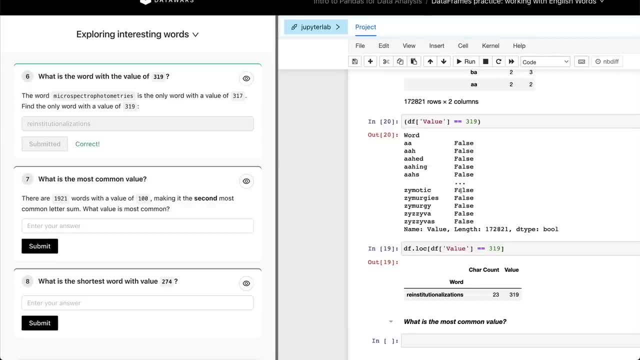 But the one tiny comment that's kind of a question we receive all the time is that: is this efficient? we could have resolved this thing with just iterating on not using any memory to put it away, because at the end of the day we have to create this boolean array. 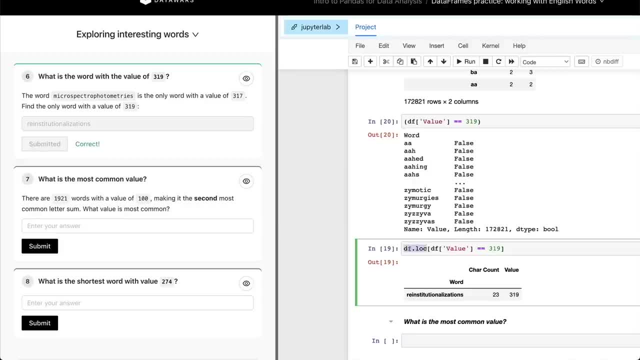 which is going to set in memory, And then we do the selection based on that boolean array. So the question is: why are we going to create this intermediate boolean array if we could? just you know each rate is right. I can do something like for row in the F: if row add value equals 319, print row just. 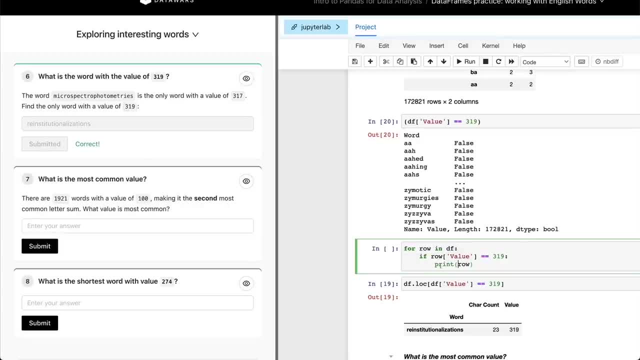 put it away. in reality have to also use the index. But anyway, in this case I'm just doing a more imperative way of resolving this activity And I'm not using any memory, I'm just the data frame is data from this existing memory. 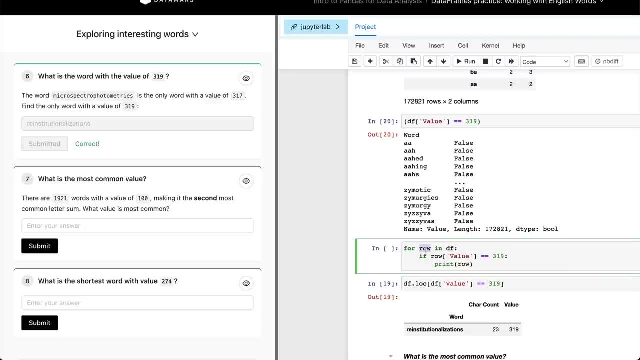 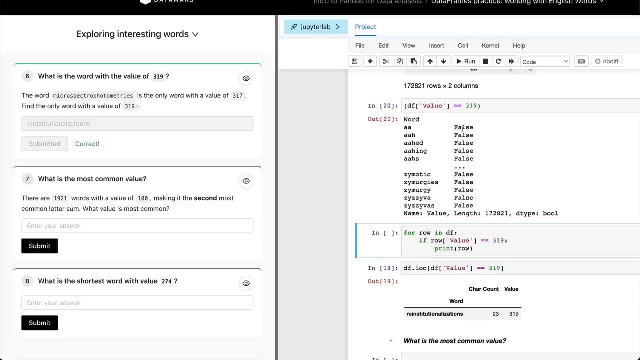 I create an auxiliary. Every slot is for this particular row And this seems to be more efficient, But the reality is that these boolean arrays are actually very, very tiny. they might look like they are this huge, huge, you know series, which all these string values, but in reality, 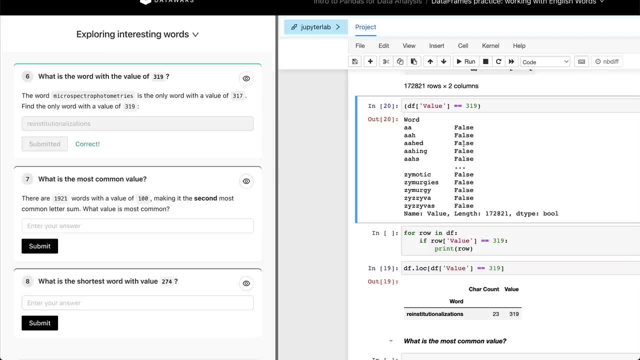 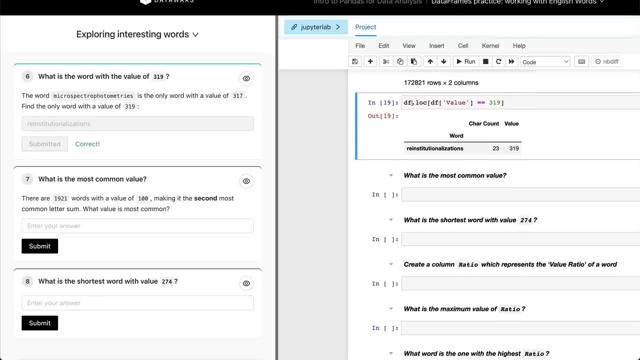 these are just ones and zeros. It's a very small one bit element array right And the index is pretty much same with we have. So just a comment on that On the side. I don't want to get too technical. But again, the beauty of panda selections. this dot lock works by the index. 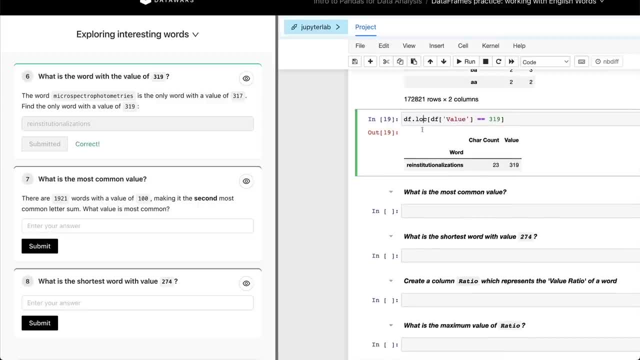 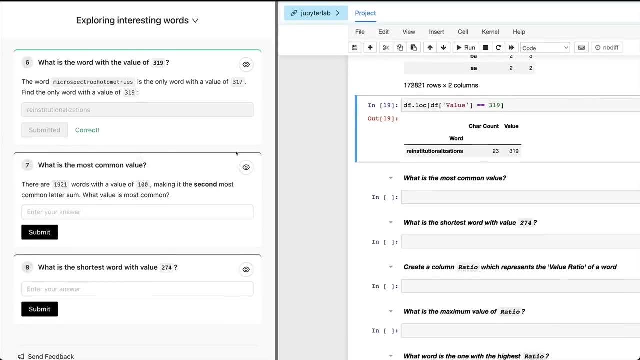 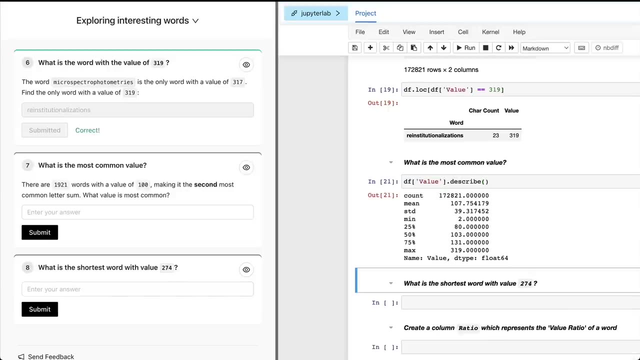 And again we can pass just one value, multiple values or a full boolean array. All right, moving forward, what is the most common value To answer this question we can refer back to? I'm going to do value scribe there, you. 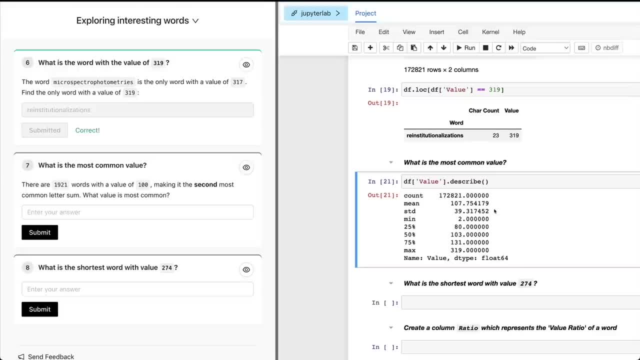 go And we can do different steps, Statistical methods, right. So in this case we have the mean, standard, deviation, minimum, maximum, etc. We also have the median, which is right here, which is the value 103.. And there is one that is not showing up here, which is the mode of the of the given series. 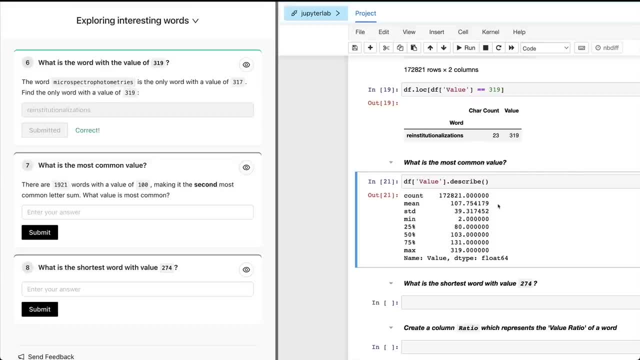 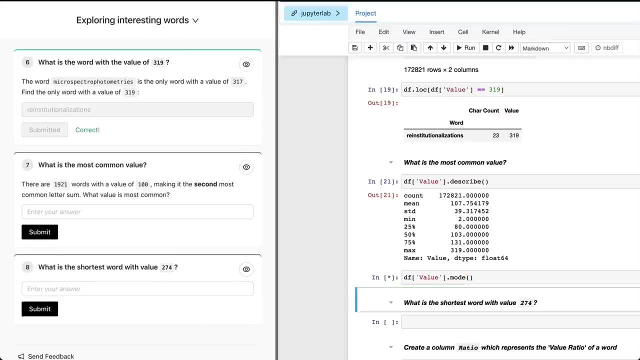 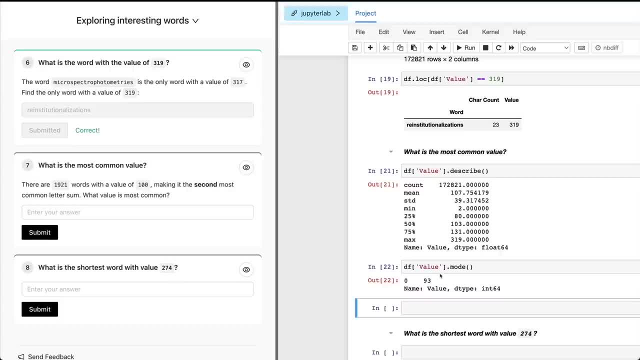 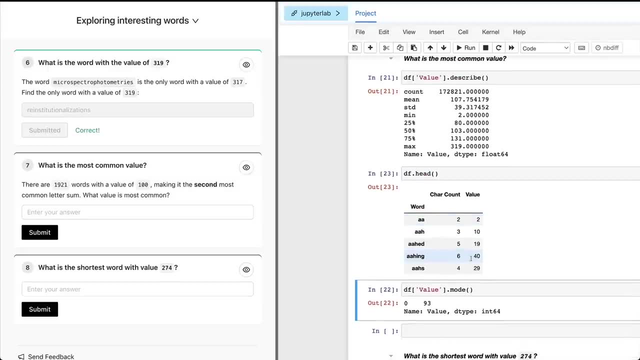 Now this doesn't tell you much, because it just tells you of all the different values we have in our data frame. that's, 93 is not the value that shows up the most times, And we don't know in which situations, because the Carter count may be different. but there, 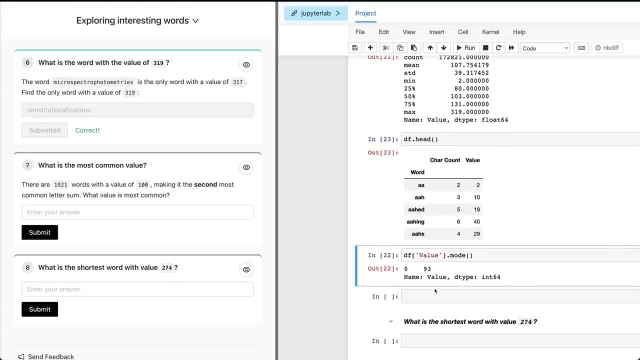 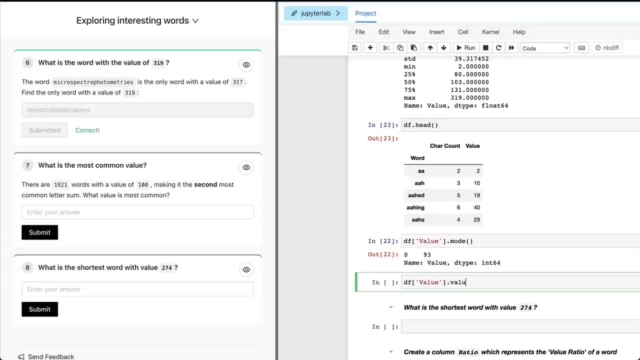 are different characters or the value is different, But a very common method. something that I use all the time is the DF value And we're going to do value counts method. this is a very, very helpful. I get just the first ones. 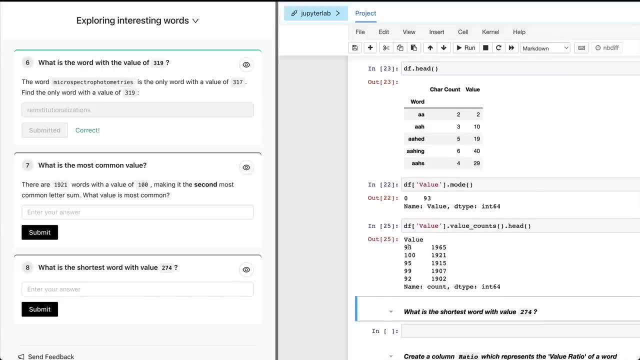 A very helpful method is going to give you this. given value appears 1965 times, So 100,, as activity said, is the second most common value And there are 100. there are 1921 words that match that value. The value 93 is the most common one and there are 1965 words. 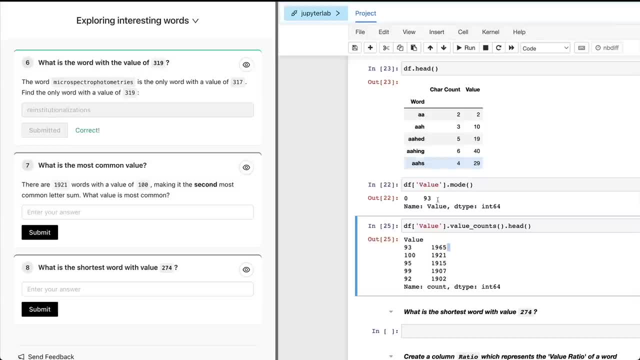 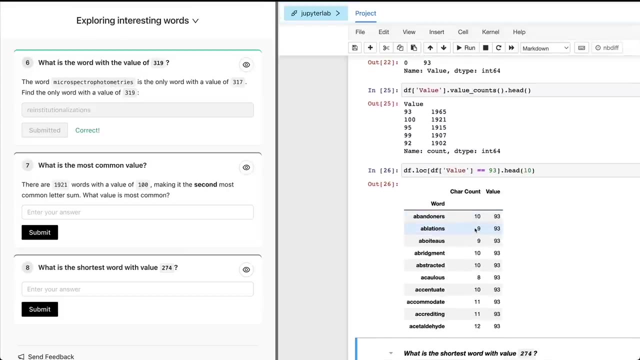 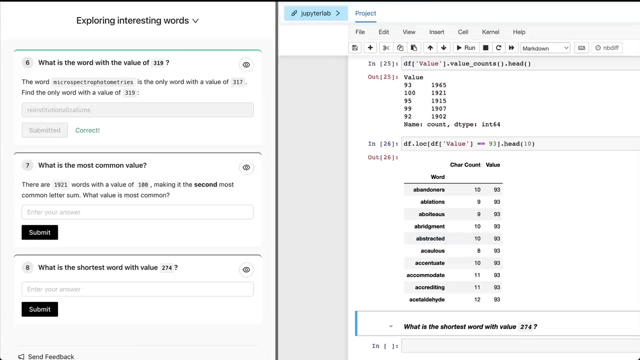 that match that given value. right here we could do something like DF dot lock, DF at value. Value equals 93, we can get here. let's get the first 10. All these words gets our have the same value, even though they have different. 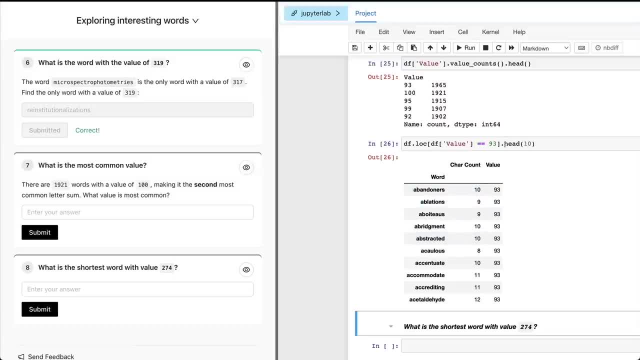 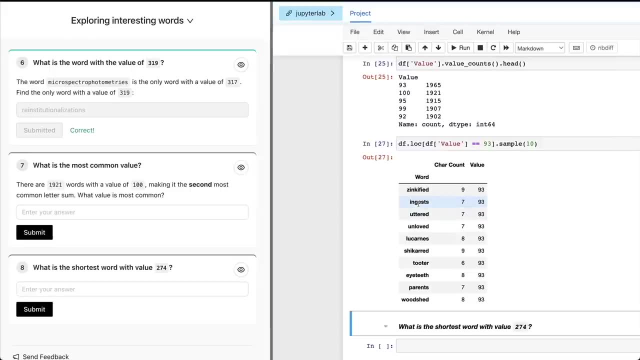 different chart counts, right, because they have different characters. Let me do sample here So we get a random sample of values. who right here we have, for example, ingests have seven characters, and how the vowel is 93. Again, the sum of the characters results in 93. But let's do it again. 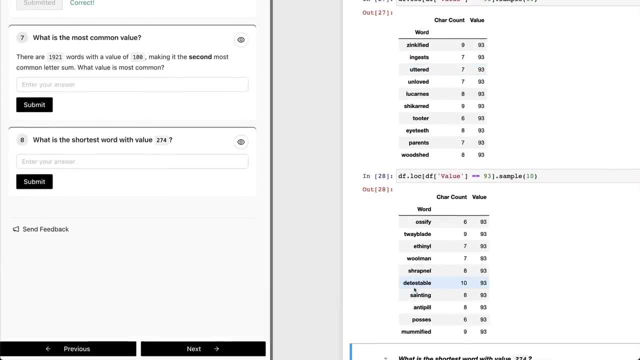 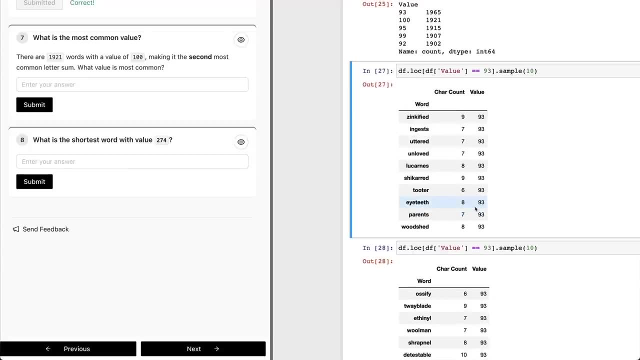 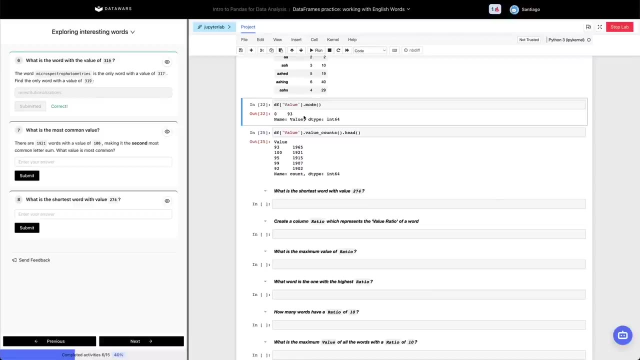 I'm going to keep that one there. The testable has 10 characters and has the same value, right. So again, to compute the mode of a values you can use, to use the mode statistical method or, for me, more common, 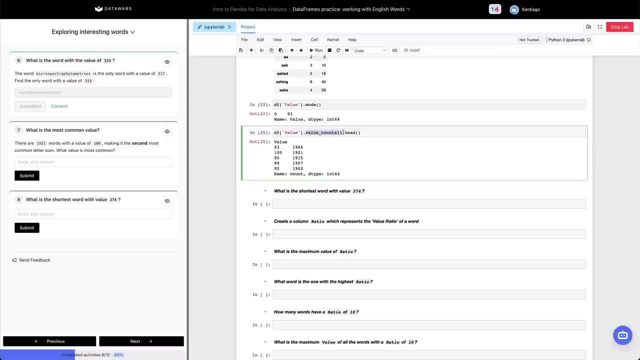 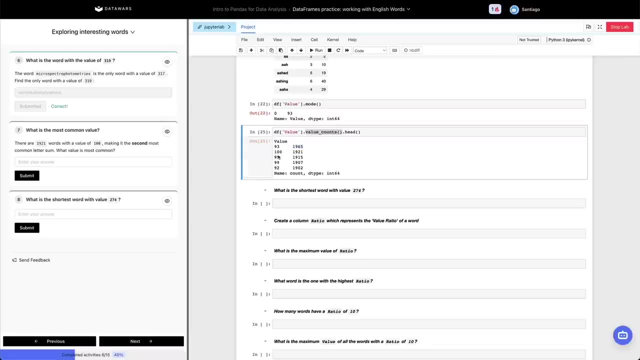 very useful is the value counts method. gives you not just the most common value, gives you kind of a ranking of the most common values in a in a column, and also gives you how many samples you can find of that value. Alright, so we haven't done it, Let's see if it passes. 93 is our most. 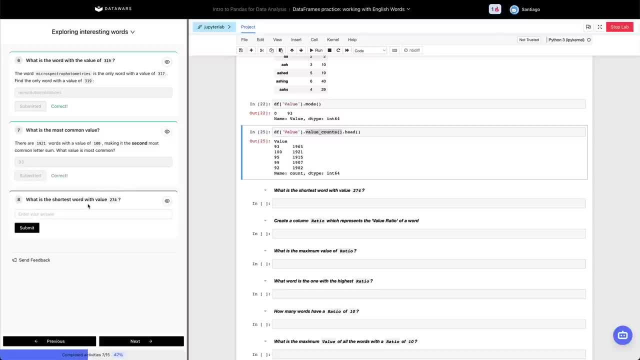 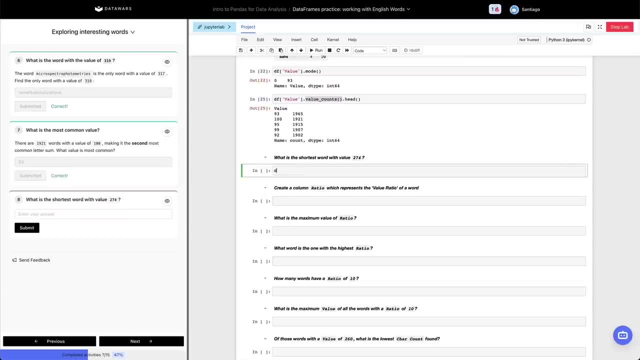 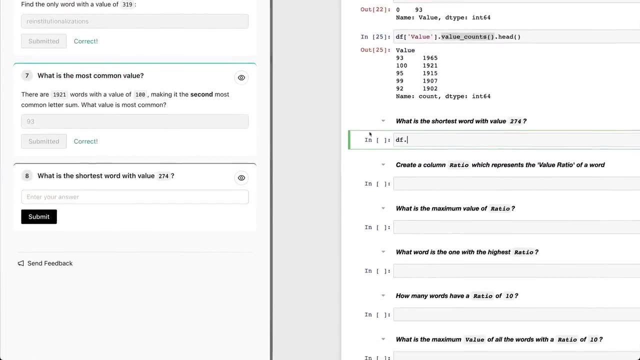 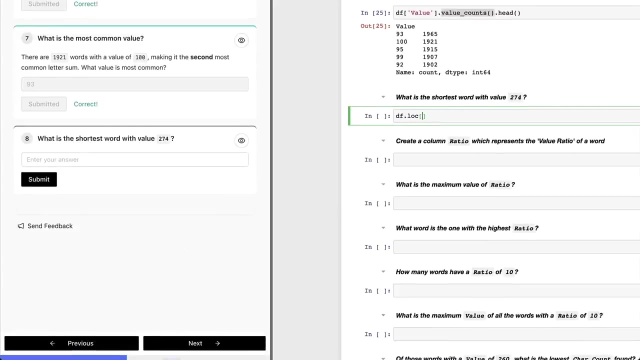 common value. There you go, It worked. What is the shortest word with a value to 74?? Let's resolve that now. DF. we're gonna do a little bit of selection first. So let me align that so we can zoom in: What is the shortest word with the value to 74.. So first we can start by selecting all the 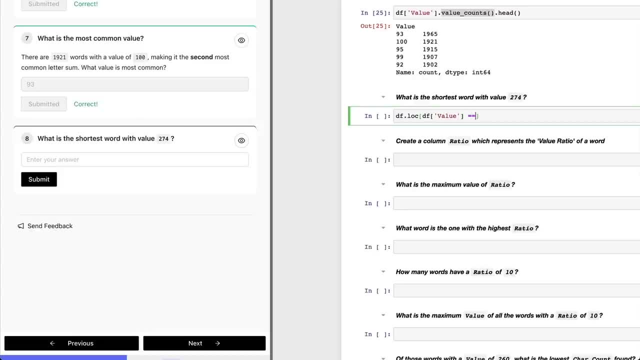 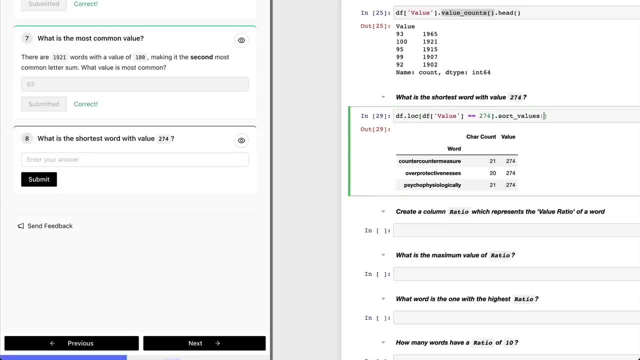 words with a value of 274.. There we go, And then what we could do is either sort of values by char count, And this is going to be the shortest one, Or we could have done a little bit of more selection. I think that 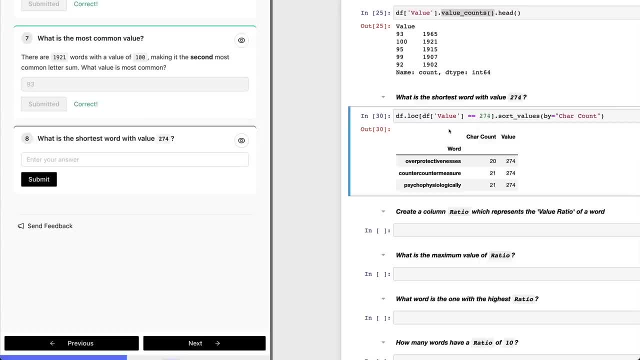 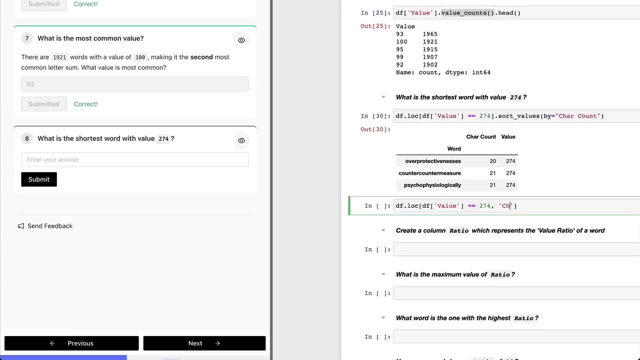 just by doing this method it works. we could have done something like: we get the value, the chart count- sorry here- so we have that, only the given column, and then we get the minimum value right. So what's the minimum value? 20?? With this thing we could have also extended our query. 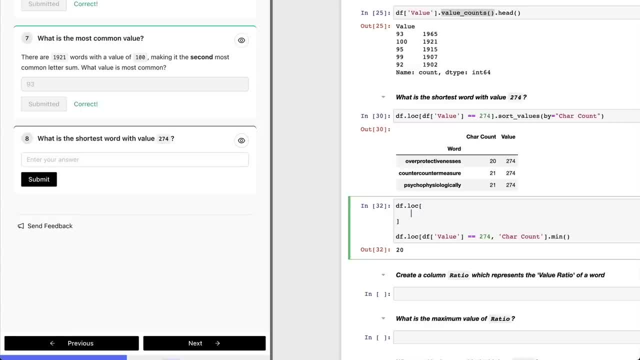 and do df dot log. I'm gonna do that And this and the df dot log. no df at chart count is equals to 20.. That's the one we got before And this is equals to that. And there we go. we can do a. 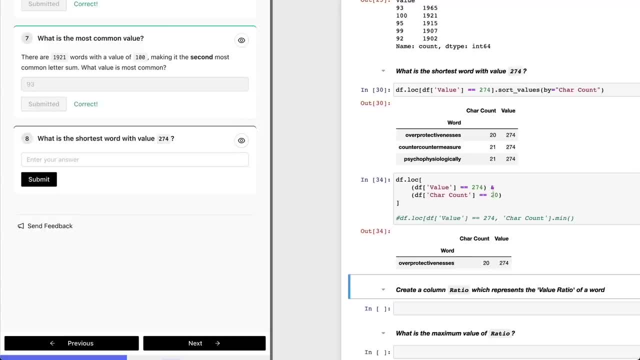 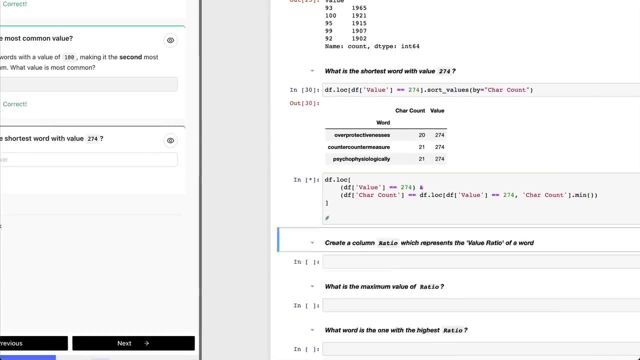 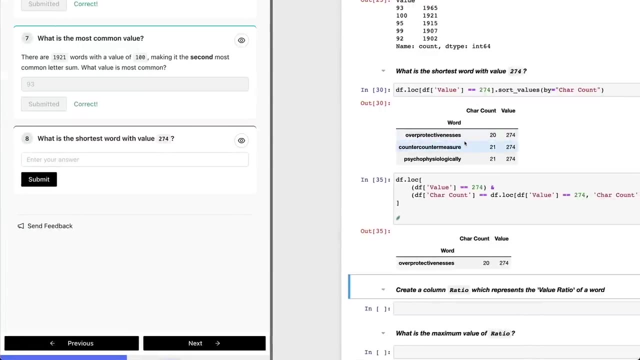 very quick selection. we could have done it also in a way that it's dynamic. So we get plug this value here And this is all the same thing At the end of the day. I think that, just you know, if we don't have too many elements, sorting the values is an easier way to resolve. 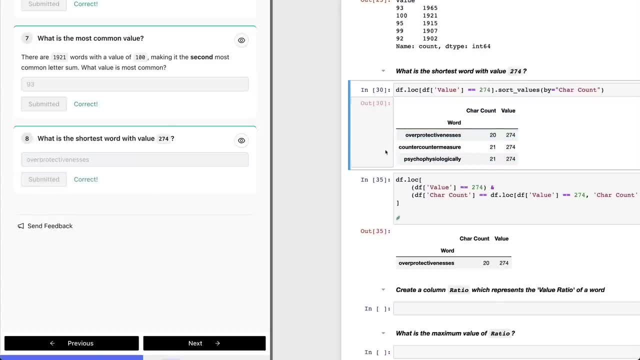 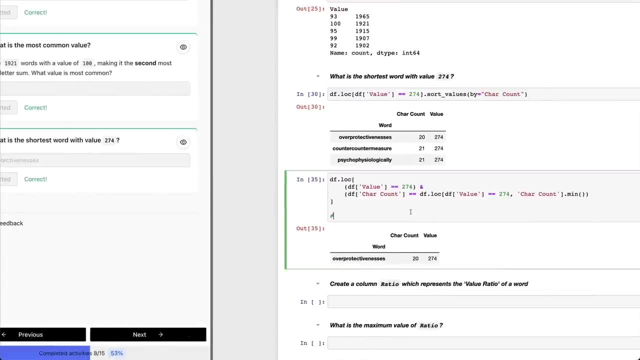 it. So let's go ahead and do it. There we go. By the way, this is something that we do, you know, in production, to put it in a way like in our day to day jobs, all the time. Sometimes you will need to build more dynamic solutions, But sometimes you're just doing some. 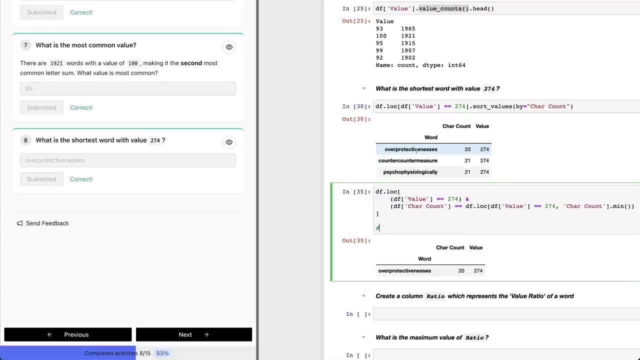 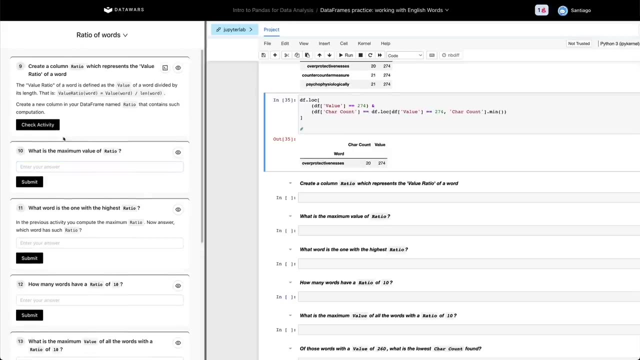 analysis, just exploring data. you know you can keep it easy. just you know, with the different methods you can hear the important pieces, applying the right technique for the right problem. All right, moving forward. Next activity: this is interesting: create a column ratio. 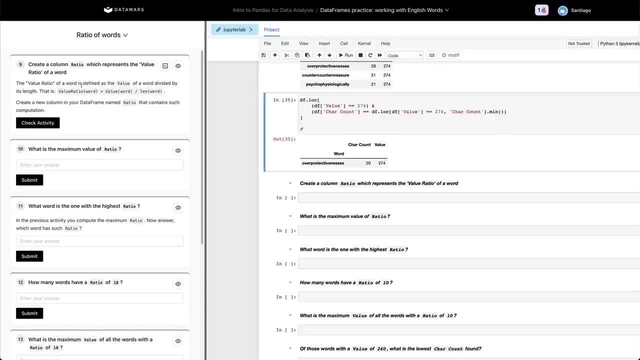 which represents the value ratio of a word, which is defined as the value of the word divided by the character count. So let's do that right now. Stop me if you want to practice this by yourself, But the way to create these ratios is going to be, I mean, 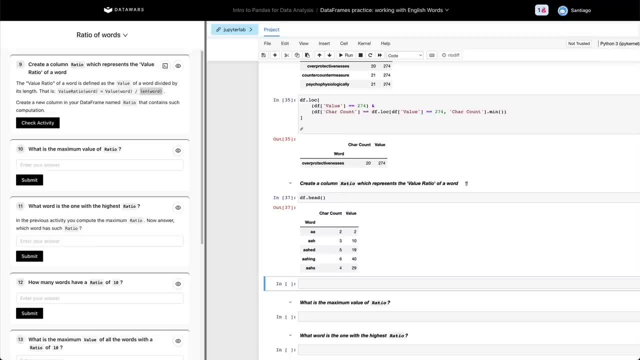 show you. the first head is going to be the F at ratio. that's the name that it's asking us. the column that is asking us is going to be equals to the F at value divided by DF, by chart count. And now we're gonna do this thing again And we have a ratio computed. 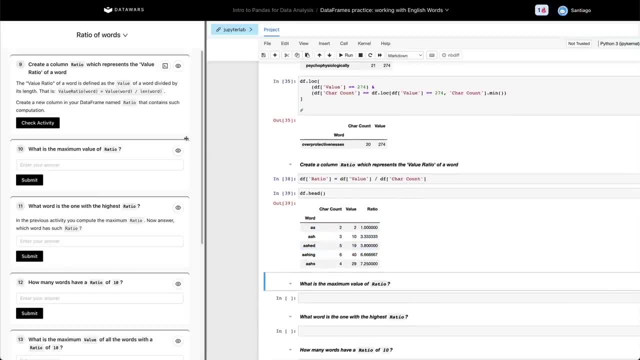 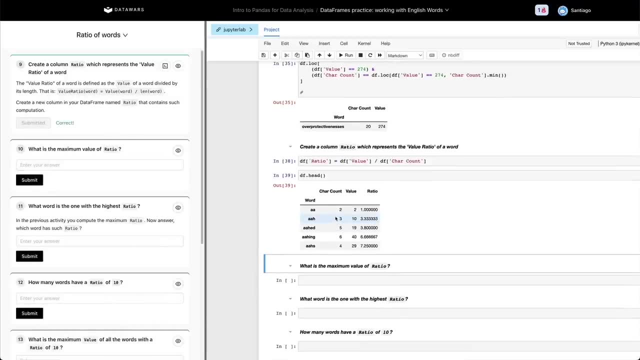 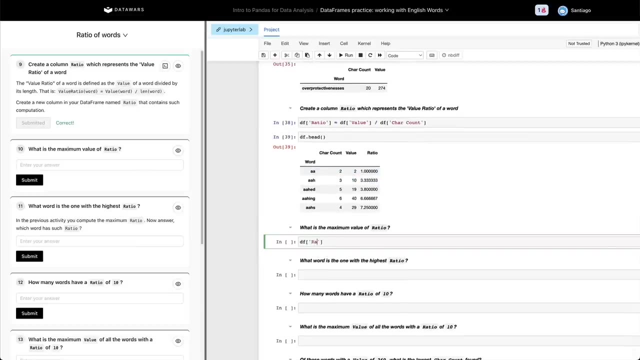 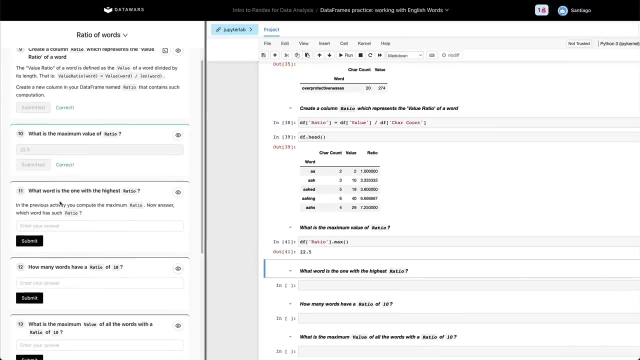 right here. the value divided by the chart counts. Let's check to see if it works. It did work. we are good to keep moving forward. So a few more questions. What is the maximum value of ratio, the F ratio, dot max 22.5?. What word is the one with the highest ratio? And here multiple ways to solve it. 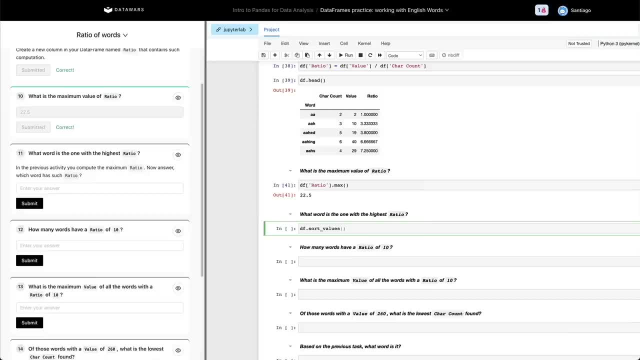 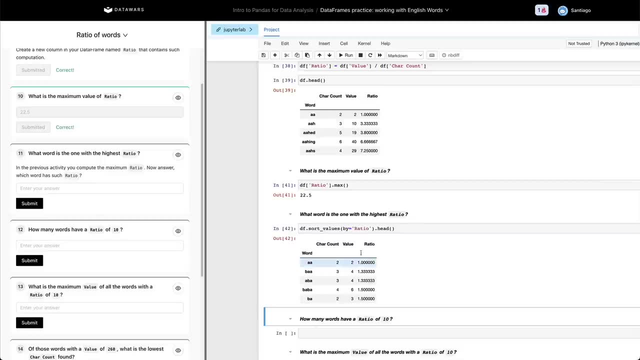 again, sort values- I think is a good alternative- And do by ratio. but here let's do it right here. these in this way: By default our values is sorting in ascending mode. we actually want it flipped. we want to start, you know, with the highest value. we want to start with the highest. 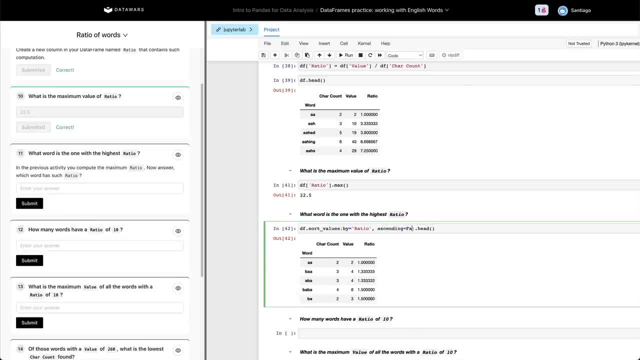 one at the top. we're going to pass. ascending was false. we're going to pass this order And now we have that the highest ratio is 22.5.. What word is the one with the highest ratio? 22.5, the word. 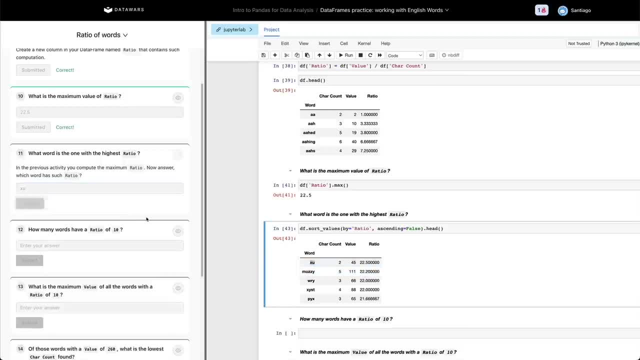 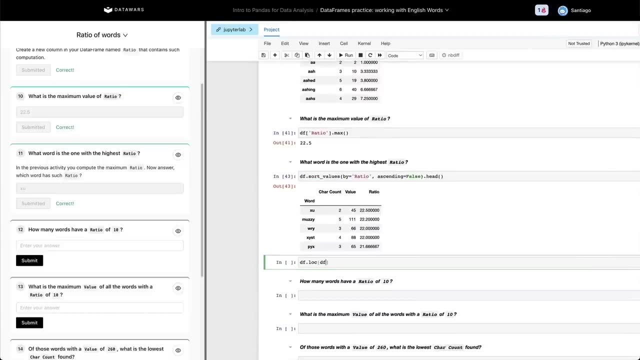 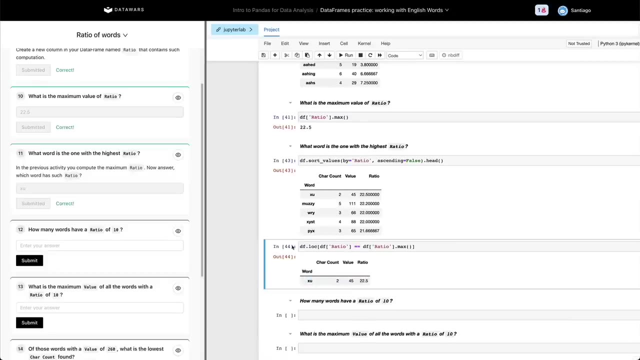 is X- you, As we know, the highest ratio. we could also have written a query, the F dot block, where DF at ratio is equal to the maximum ratio, And that is also X you is the same result. So again, two different ways of resolving the same activity. It's important for you to have all the 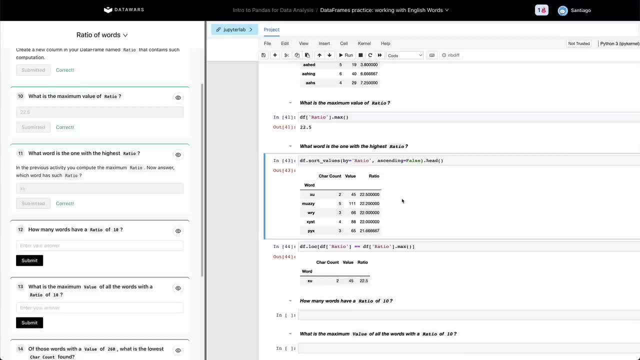 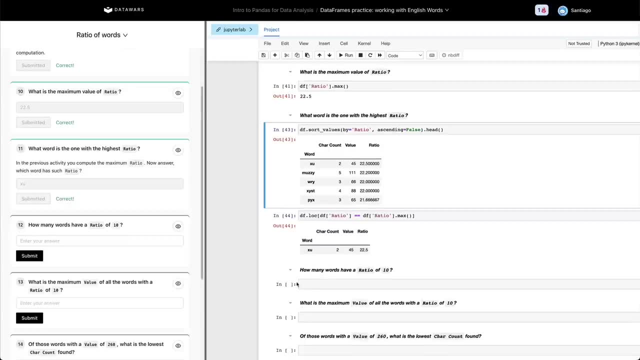 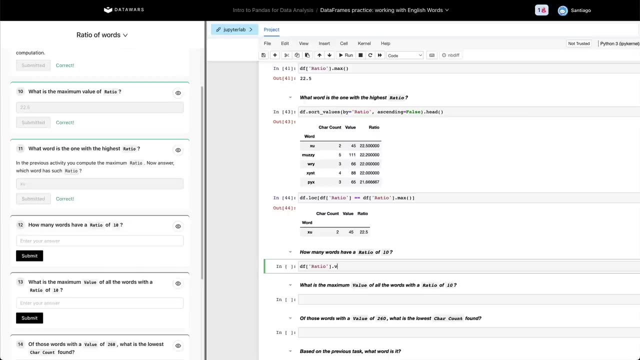 techniques in your tool belt, then which ones you use. it depends on what problem you're solving. How many words have a ratio of 10.. So what we can do here is: we can do DF we could have done. this is not going to work so well. value counts. to get an idea of the values, And here we have just. 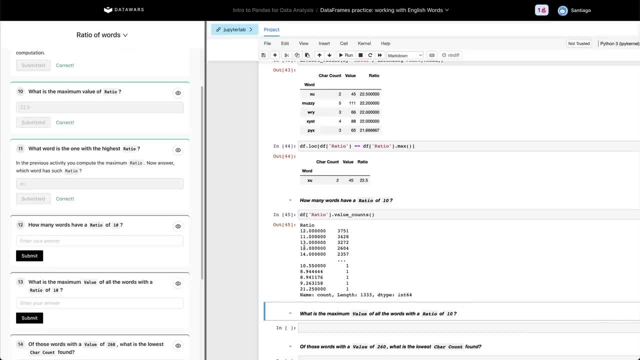 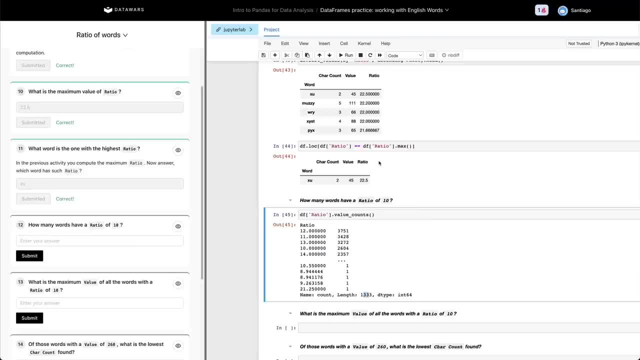 to be able to do this. So we're not going to be able to do this. So we're not going to be able to do this And we're only going to have 333 different ratios. So, as ratio is a continuum variable, 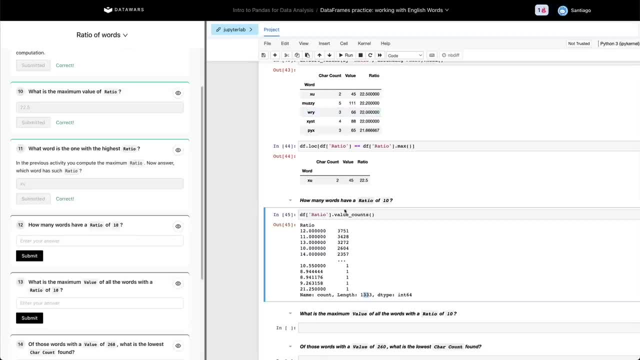 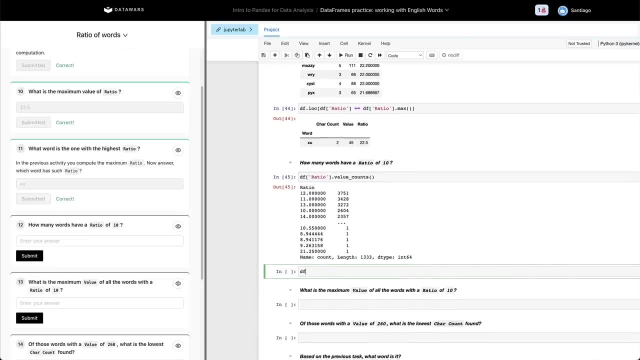 you know, there are multiple individual points. it's usually not convenient to use value counts. Instead, what we want to do is just write a simple query: df dot lock all the rows that have a ratio of 10, right, that's the query. when a belt gives us a bunch of rows, what we can. 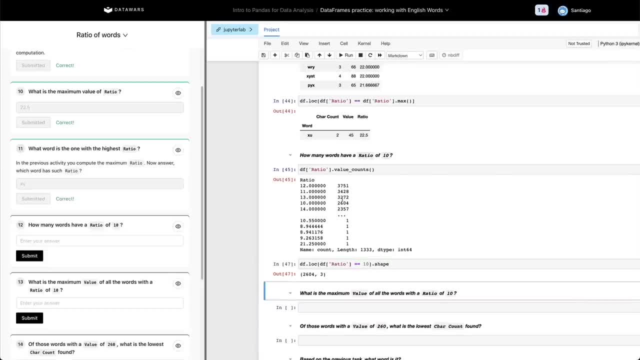 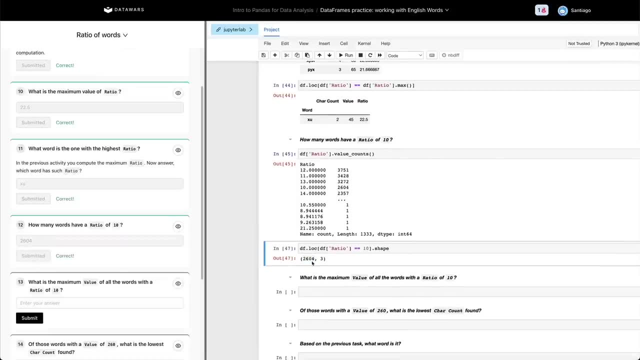 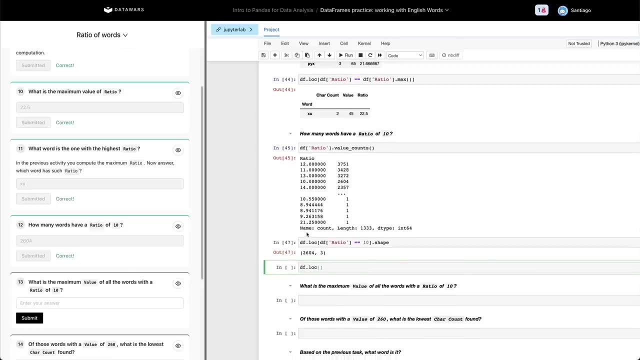 do is just do a shape And that's going to give us the same number we have right here. We're going to plug it in here. Let's do a quick, quick stop here. an asterisk to mention the dot query method. So df, dot log and all the selection is usually 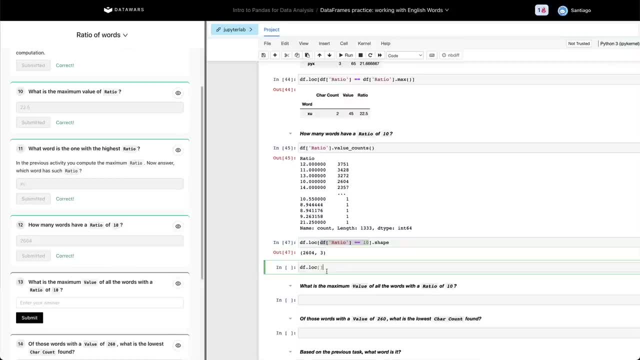 the prefer method because it's the most powerful one, But sometimes you just want to use the query method. that is just kind of a shorthand. you can write it in plain English, is kind of Python based And the query method is just works in this way. we can say: a ratio equals 10. And it's 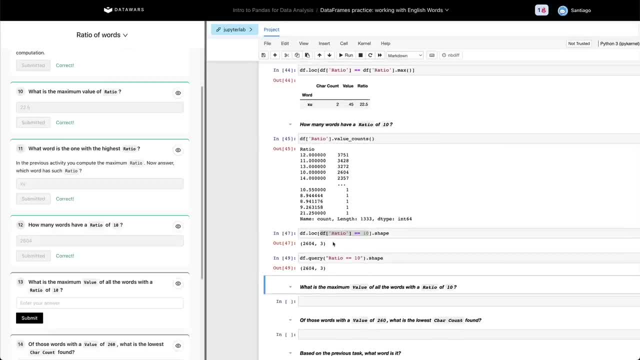 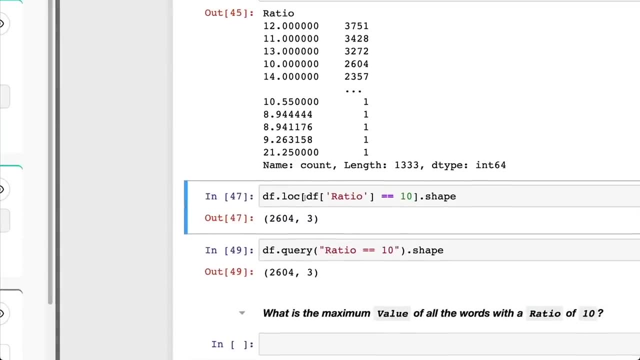 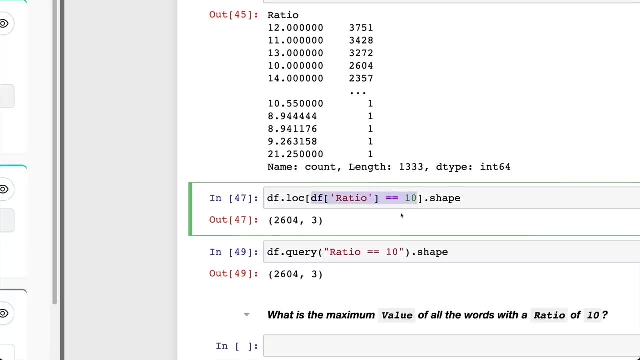 relatively simple. You can use it whenever you have like simple conditions. There you go. here's for you to compare. I personally myself I usually prefer this method, But that's because I'm just very used to it And I like thinking in terms of boolean arrays and complain in combining 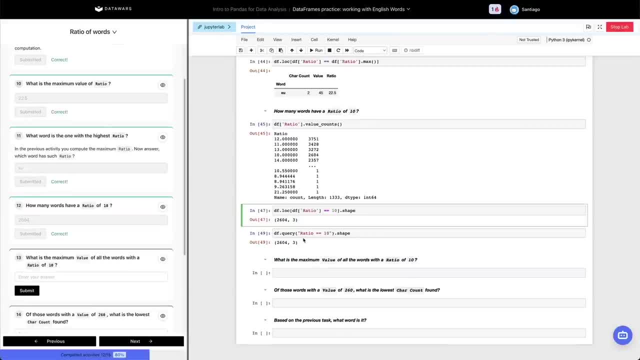 boolean arrays, and all that, up to you. if you want to use query the one that suits you the most, And if you want to use query the one that suits you the most. And if you want to use query the one that suits you the most, And if you want to use query the one that suits you. 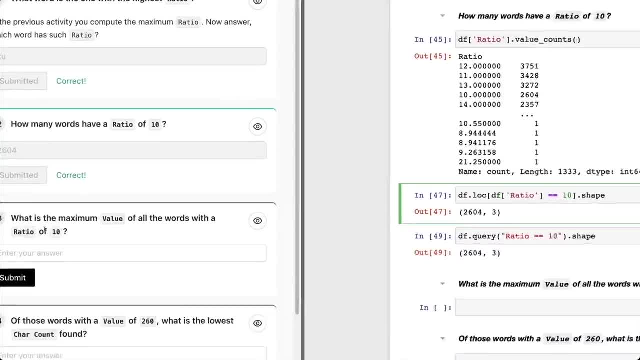 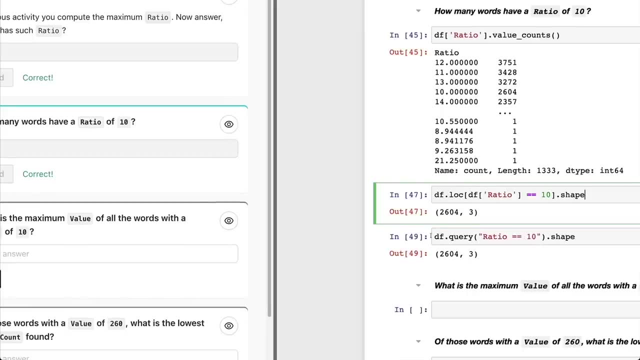 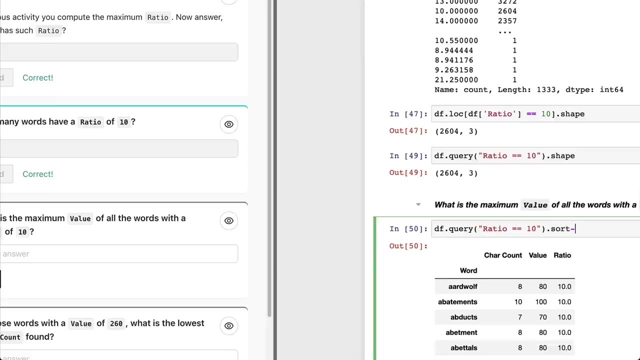 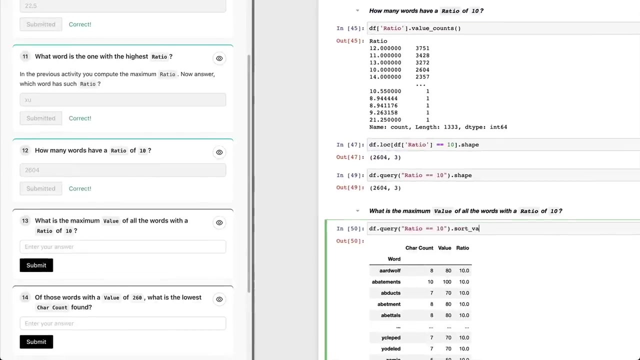 better Moving forward? what is the maximum value of all the words with a ratio of 10.. So we're gonna keep, let's keep query here. This is the results, And what we can do here is we can sort values. let me put in context again: activity. what is the maximum value? sort of values by value. 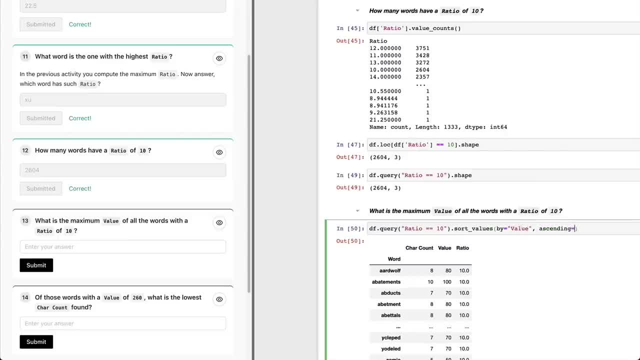 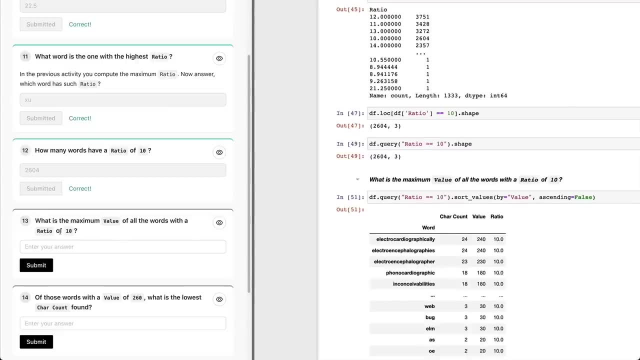 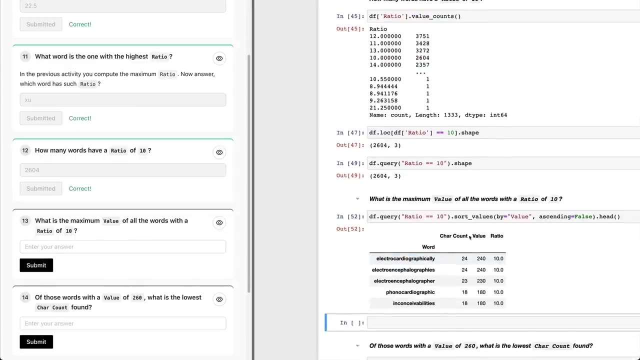 value ascending false. And here we can find what is the maximum value of all the words with a ratio of 10.. Right Head, there you go. we had was the maximum value: 240.. It seems we could have also. 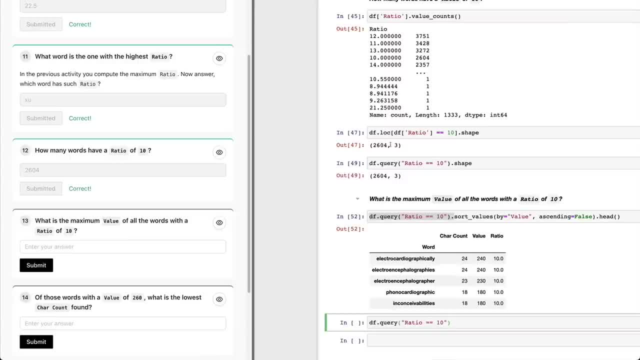 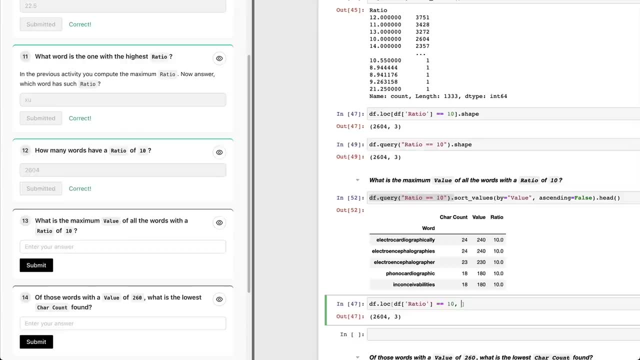 done here. Actually, for this particular solution. I think this method is going to be better. We can do that And we're going to do value. Just get the max. we should get the same result: 240.. And that's the same answer here. The beauty of sort values that sometimes you see. 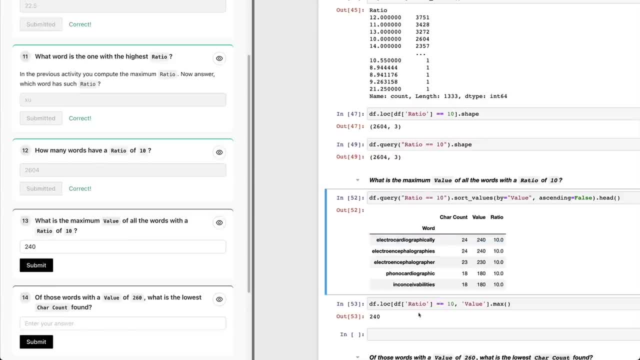 like the data. in this case, you have to trust it, which is fine. we'll have analytical resolution we we can trust it, But it is really like you can trust. it's like the radius 10, char count is 24.. 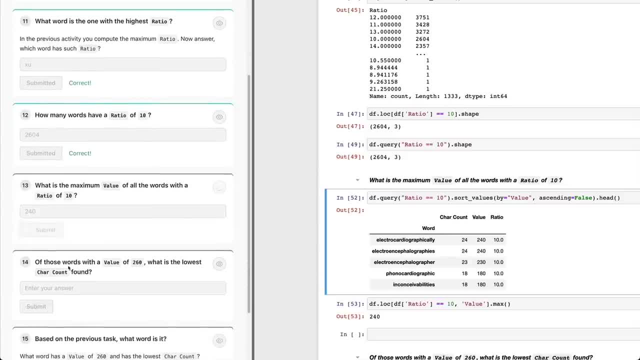 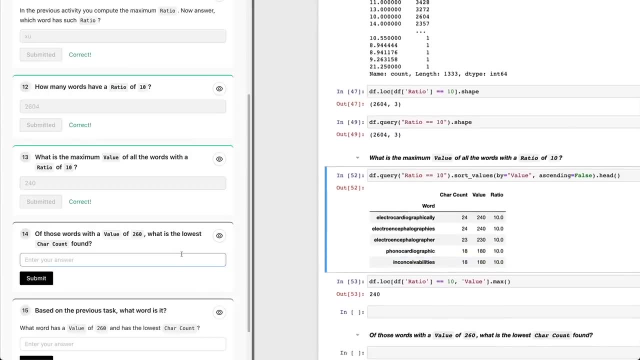 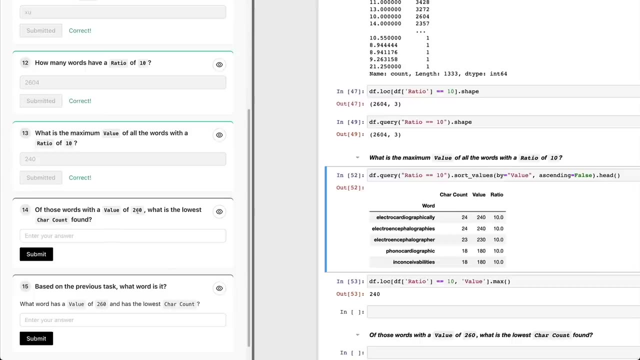 The value is 20 240.. 40,- it's usually a little bit, I don't know. it leaves you at peace to see that the data is okay. Let's keep moving forward. Of those words with a value of 216,, what is the lowest chart count? 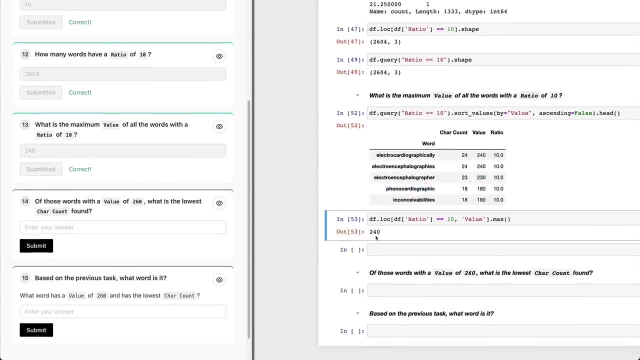 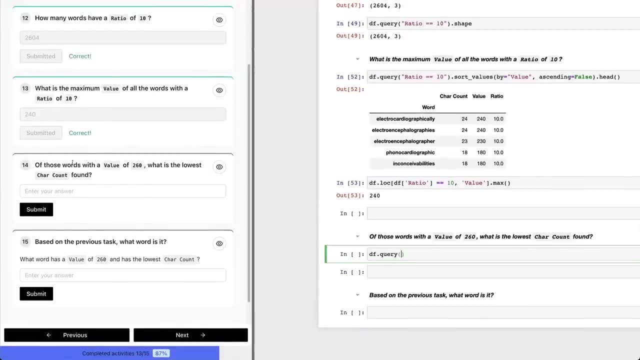 fount. In this case we have pretty much the same thing to here the F. let's do query now. And we're going to do of those words with the values 260.. So value is 260.. What is the lowest chart? 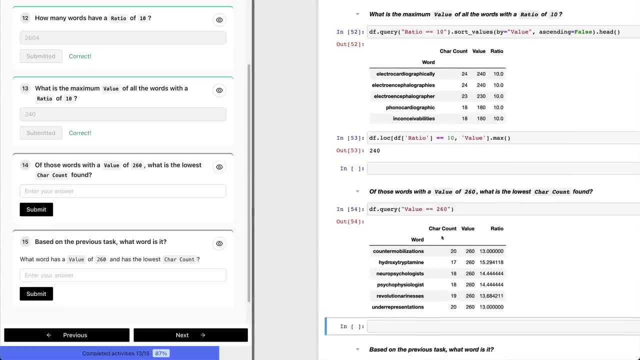 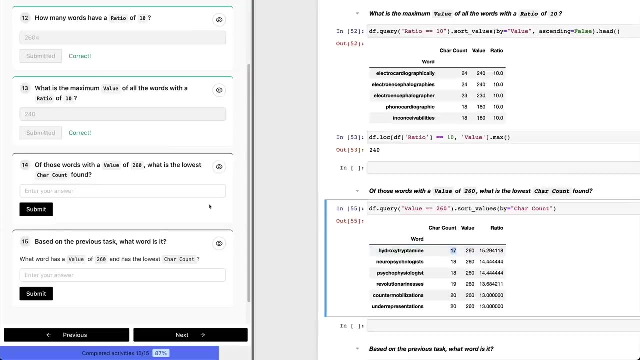 count font. So first, this thing is going to give you all the words with a value 260.. Now we can sort values by chart count And that's going to give us what is the lowest chart count found is 17.. So here we're going to find 17.. There you go, And the last activity. 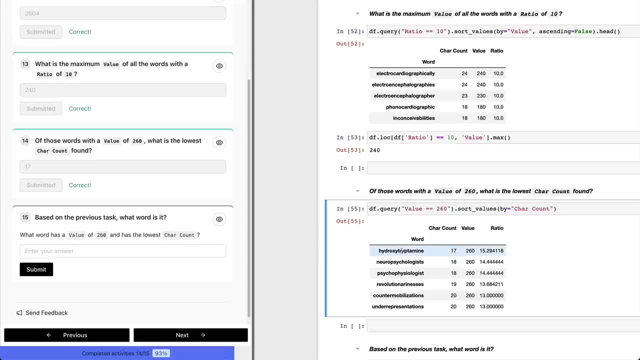 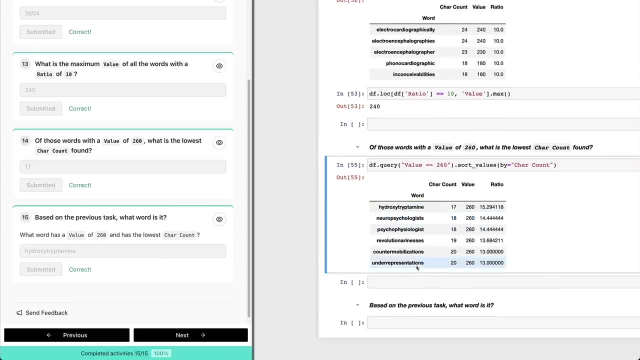 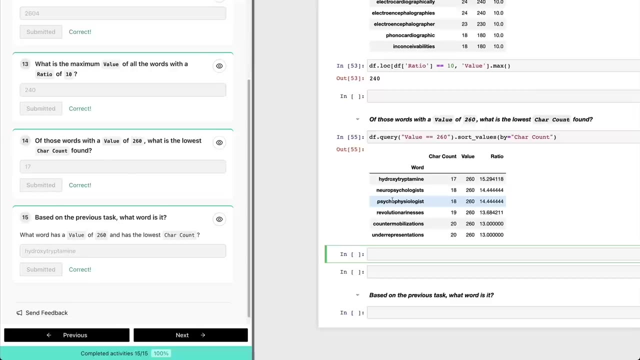 we're going to be done based on the previous task. what word is it? this is the word, And we are good to go. One important one, minimum comments about the query method- And we're just going to wrap it up with this particular project- is that when you're, when you're. 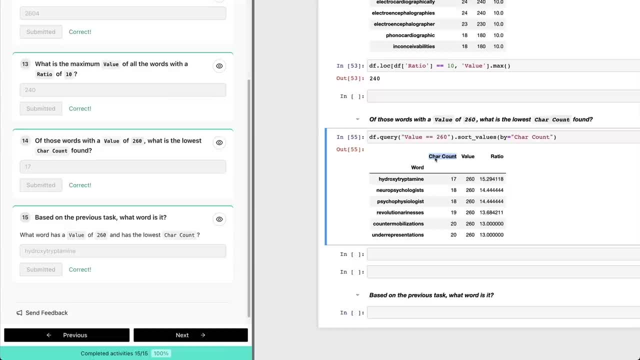 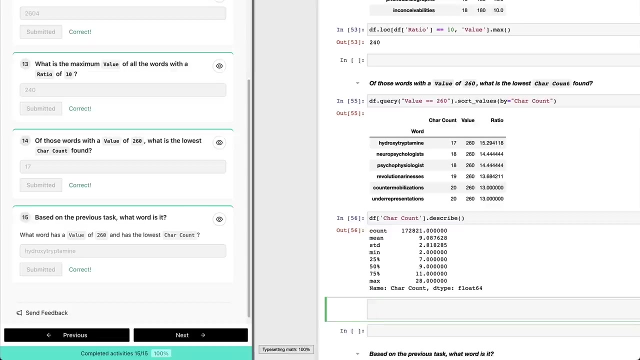 your columns have spaces, you need to surround them in backticks. So let's get, let's invent a new activity just by ourselves here very quickly, And I use this tribe- There you go And say: let's say, I'm just writing this on the fly, I'm fine, all the words with 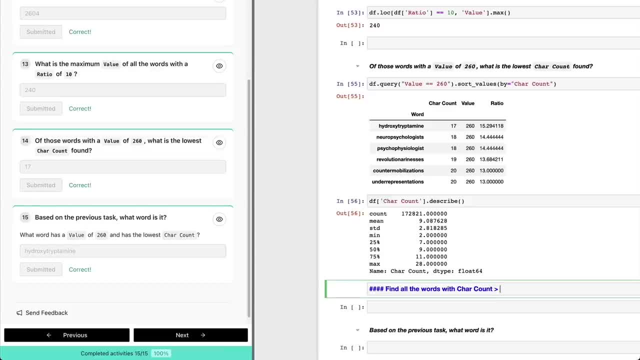 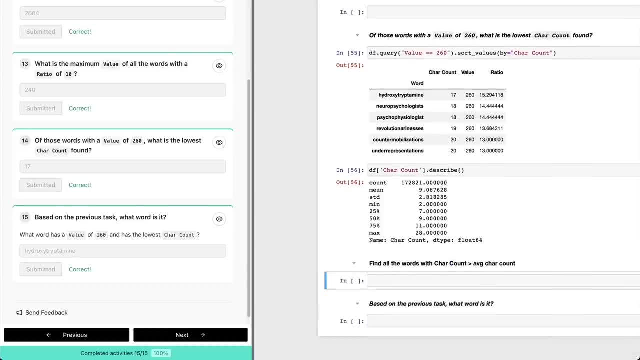 with chart count greater than the mean or the average chart counts. Charlie counts, Yeah, character counts, Right. So this activity we're like just making up on the fly. How can we? first we can compute, then let's say we have. 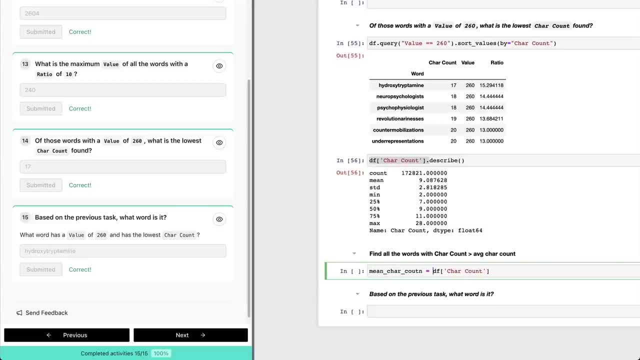 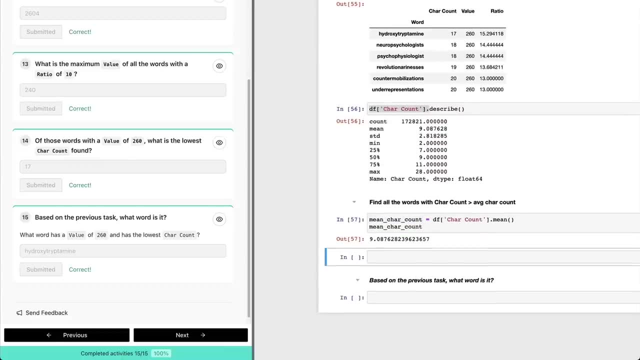 we're gonna mean chart counts, gonna be count, it's gonna be dot mean and we're gonna print it. I'm going to show you how to write the query using this variable. we're going to do the f dot query where chart count- and this is not going to work- is greater. 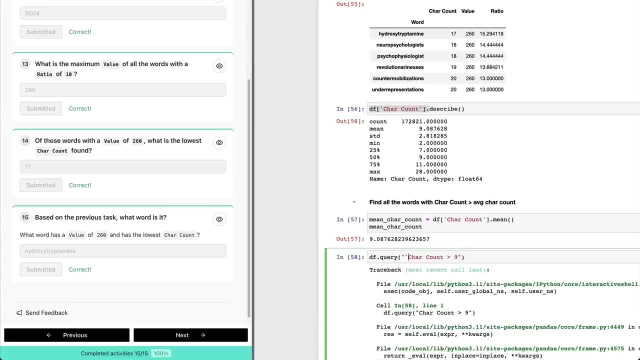 than nine, right? So this is not going to work. because there are spaces, you have to surround them with backticks. That's the first thing you want to work. The second thing is: if you want to reference these variable in here, if I do this, that's not going to work. 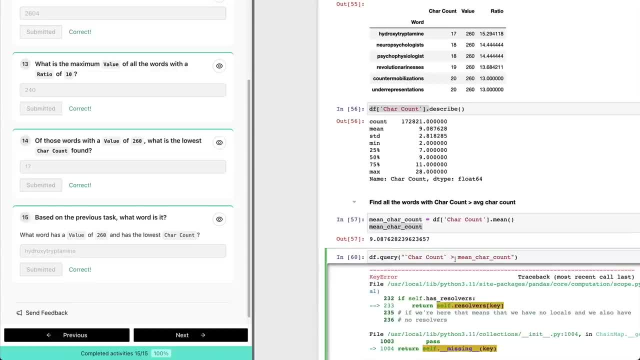 either just going to blow up Because by default, anything that is a name within this query is going to reference a column. So if you want to reference an external variable, what you have to do is pass here the ampersand symbol. in this case gonna say: give me all the values in which this column. 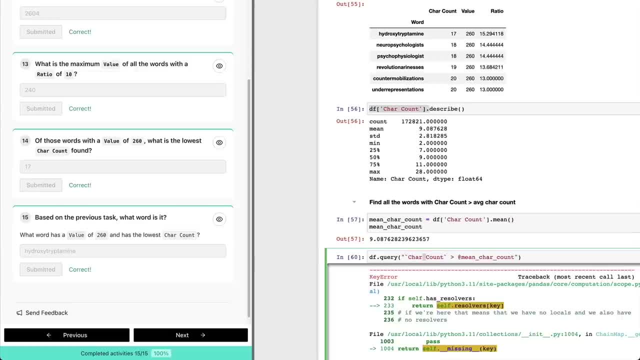 surrounded by backticks. So respect the. the white space is greater than this thing And this thing is referencing an external variable. So go out to put it away To the global scope, or local whatever, and find this value, plug it in and run the query. 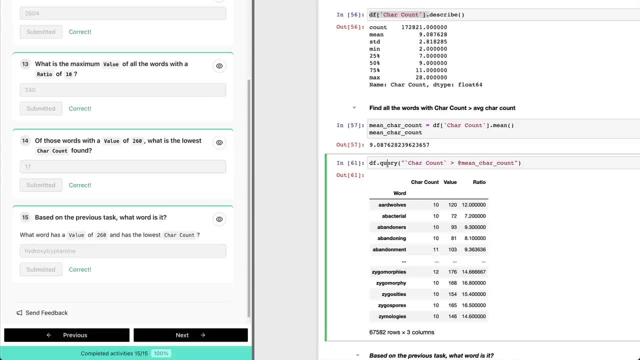 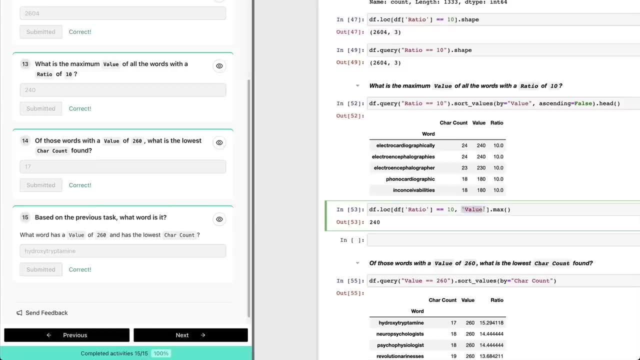 And here is what we can do right there. So again, the query method is convenient. I personally, myself, I prefer to use the dot block method. I like to combine it with column selection. I like to think in terms of Boolean arrays, but it's perfectly fine to use query just. 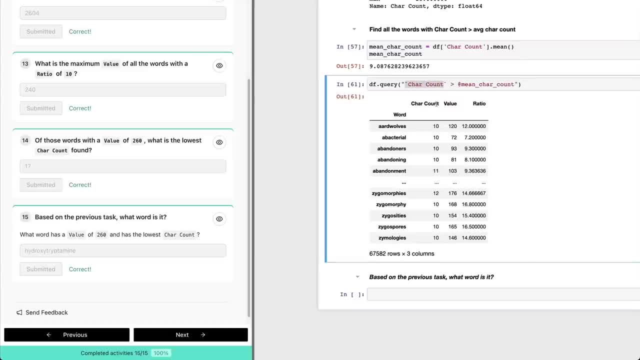 remember this tricks right, That sometimes you're going to need to use backticks, and you're going to need to use backticks For columns with white spaces and you can reference external variables with the symbol. that is it with data frames. let's keep moving forward and solving more projects applying. 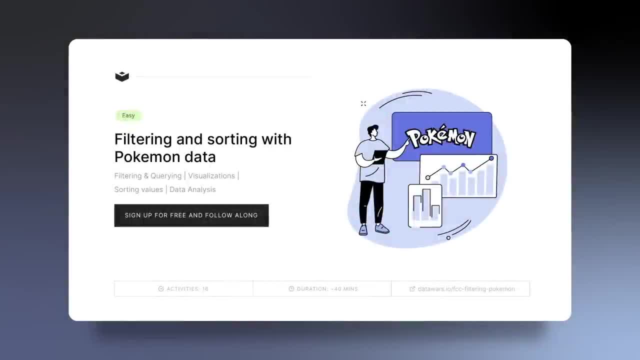 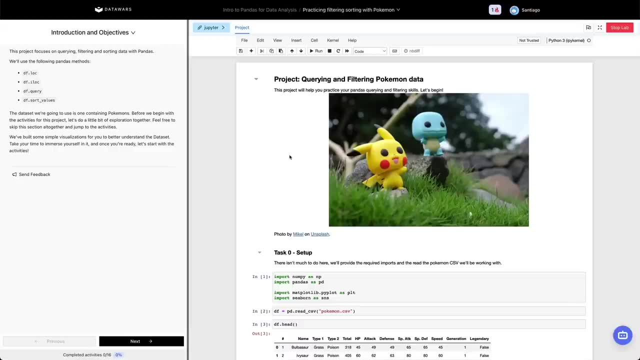 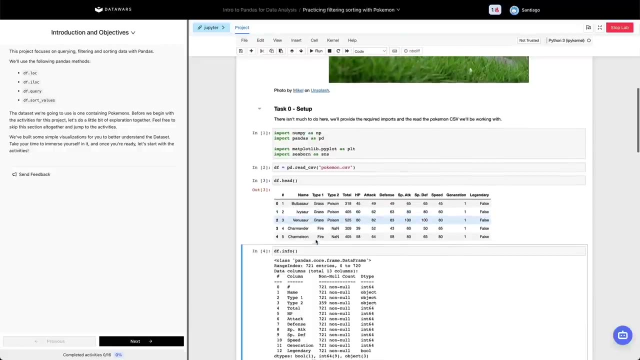 those data science skills. In this project we're going to practice how to filter data sorted, do some selections, some querying- all very useful data analysis techniques. The data that we're going to be working with is a data set containing Pokemon information. 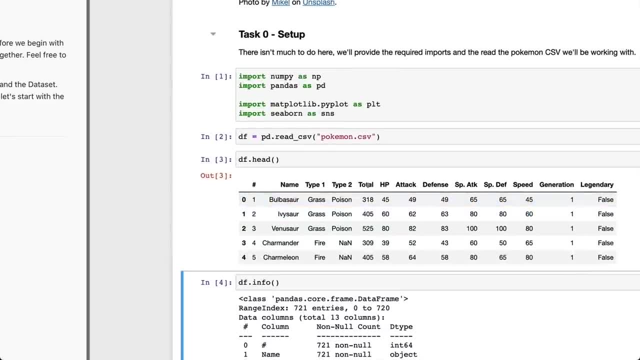 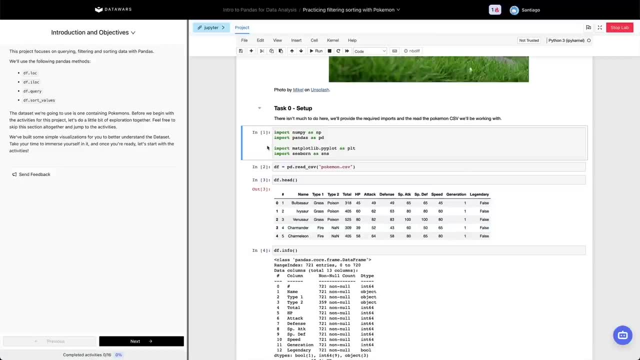 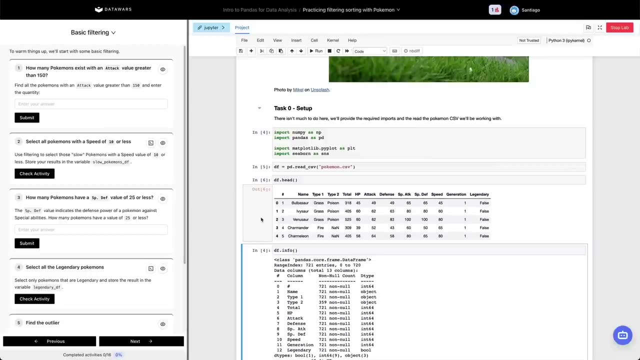 including their type, their stats, some total attack defense and all that, their generation and their legendary status. So let's go ahead and just read the data to get started, And we're going to start working with activities one by one, as usual. just pause if you want. 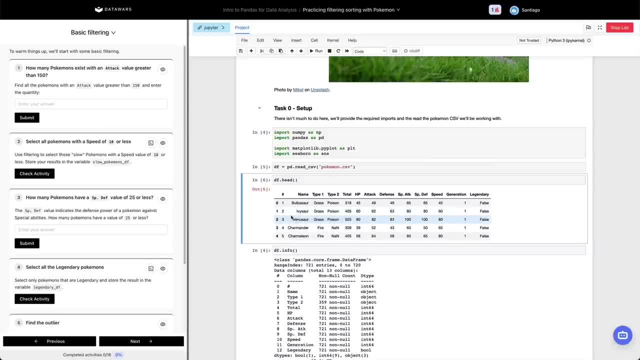 to resolve it by yourself, And then you're going to hear me with the explanation. what I'm going to try doing in this project, or for this project, is giving you all the different possibilities You can think of. so solutions with dot lock, solutions with I lock, if that applies, and 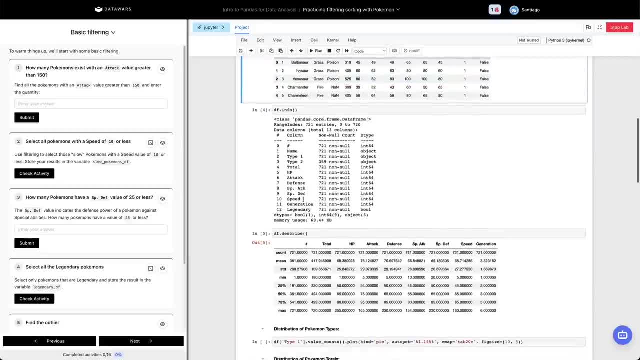 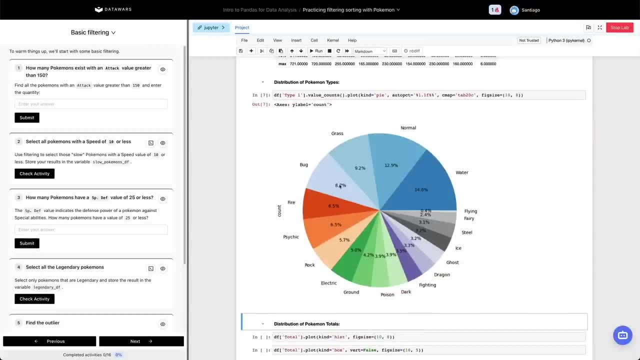 also solutions with the dot query method. The first thing you have in this notebook is a little bit of an information in terms of distribution of the pokemons we have. So, for example, these are all the type one pokemons And you also. we also have some analysis of 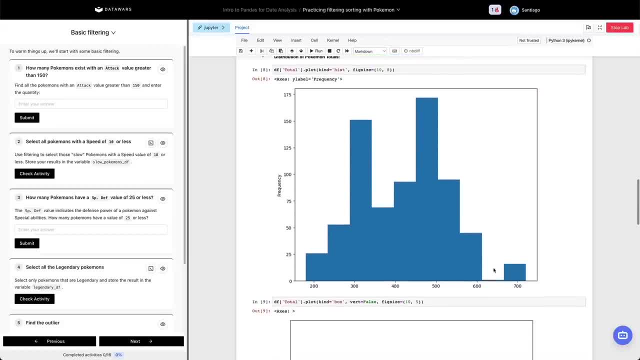 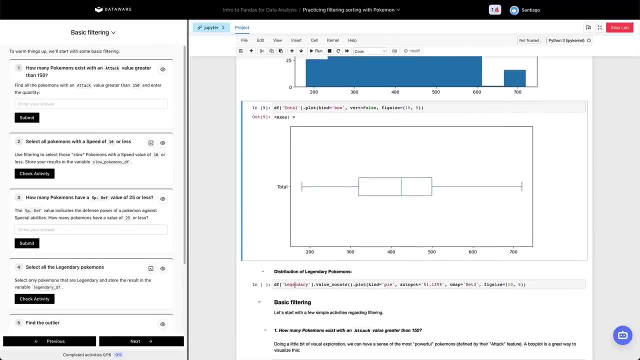 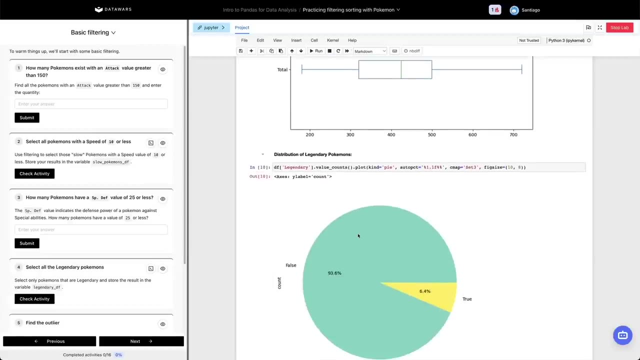 for example, the stats. So, for example, total, we see that there are a few very powerful pokemons, both in terms of histogram and a box spot. So all these visualizations are usually pretty useful. right, When you're sorting your data analysis with a new data set, you just do a quick visualization of 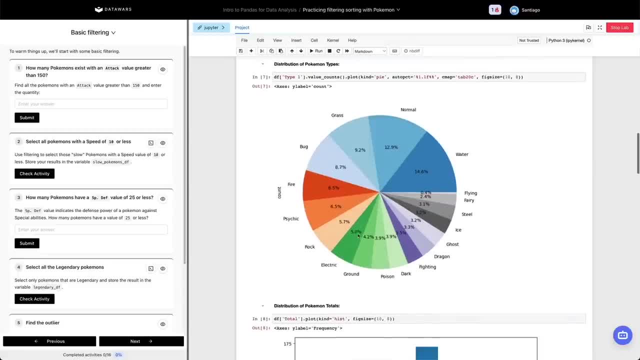 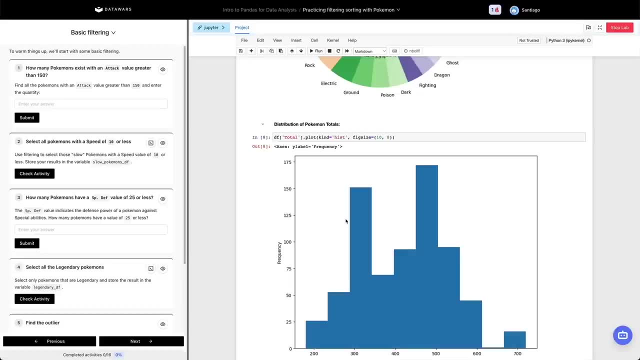 how your data is distributed in terms of, for example, category, categorical fire variables, how they're assigned, or also the ranges distribution of some numeric variables, like, in this case, the total wants to see we we can see the most powerful pokemons. In this case they're. 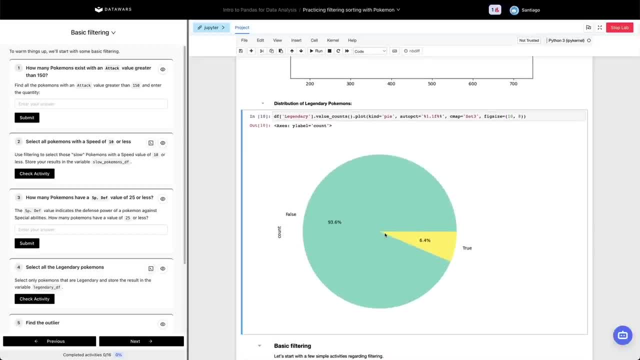 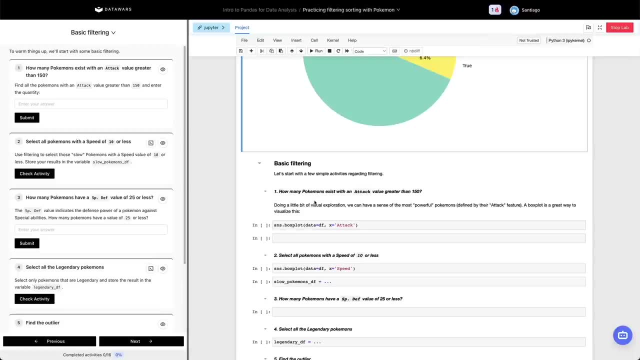 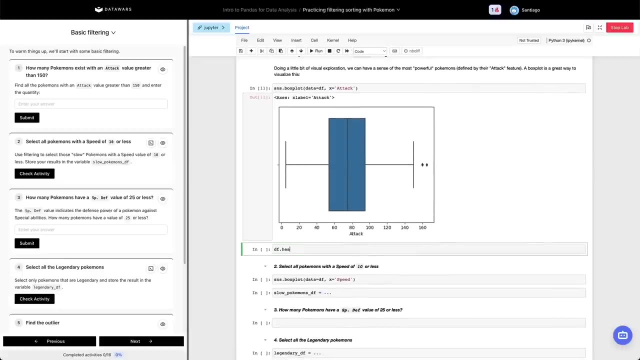 less than a legend. There is status. we can also consider a categorical fire- And on that let's get started with the activities one by one. So how many pokemons exist with an attack value greater than 150? Right, So let's take a look at the data first. That's what. 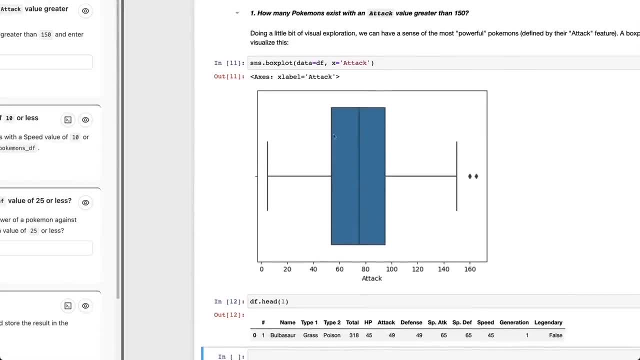 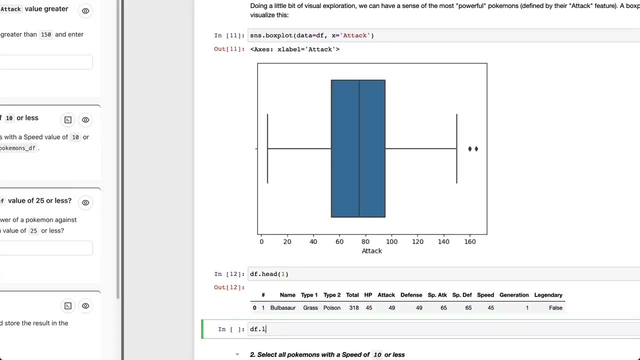 we're dealing with And we're going to focus how many Pokemons exist with an attack, finally, of greater than 150.. So let's get started. pause if you want, And we're going to do DFcom, lock df at attack greater than 150. right, that's going to give us the full list of pokemons with. 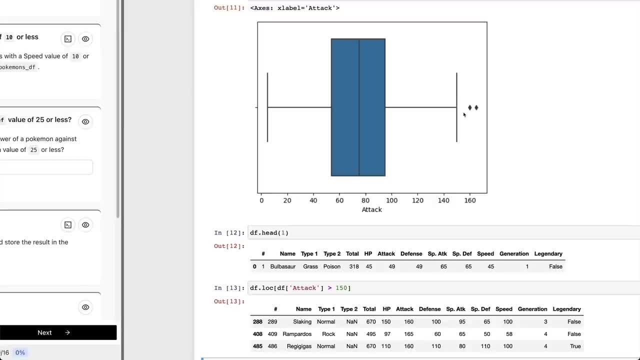 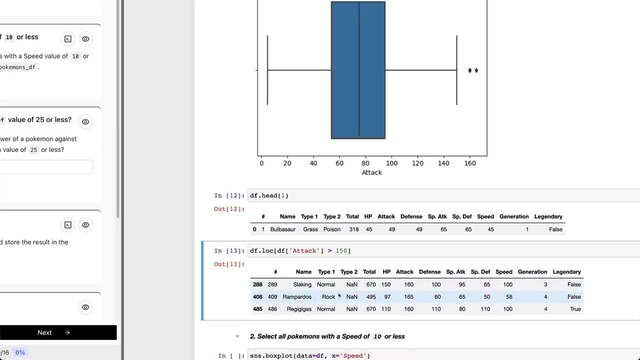 that attack and we can kind of see that there weren't like too many with that value already. with the fox plot, with the query itself, we can get a real sense of how many values we have. in this case we have just three. we could also do something like shape to get it, but again we can. 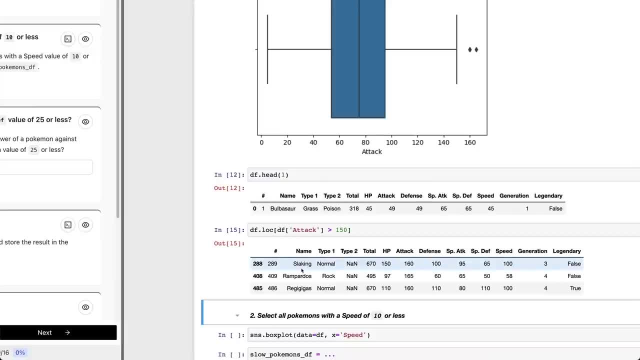 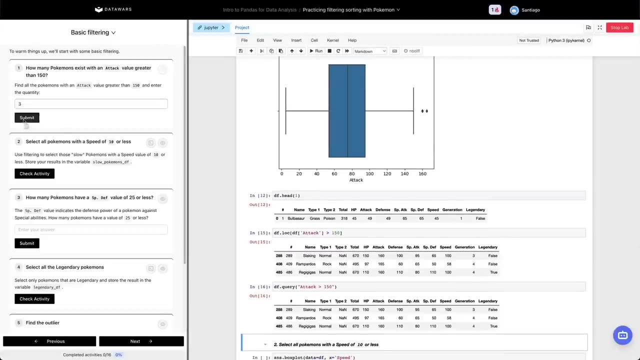 clearly see that there are only three samples that match that. given condition, we can also do the query method. so i can do df dot query where attack is greater than 150, and we get the same results. so let's try it out. see, there you go. it worked correctly. moving forward, select all the 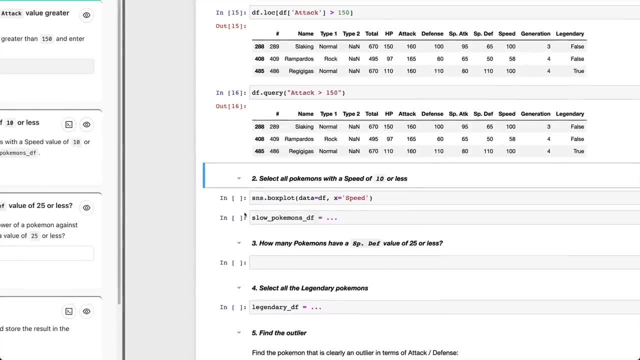 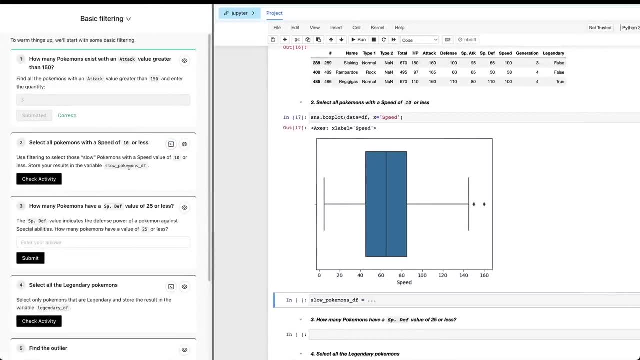 pokemons with the same value and we can see that there are only three samples that match that given condition with a speed of 10 or less. so in this case we need to create a sub data frame. so it says right here: store your results in slow pokemons df. so in this case is a speed of 10 or less, so that's. 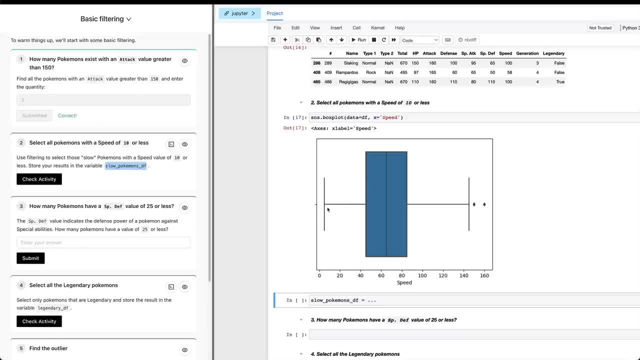 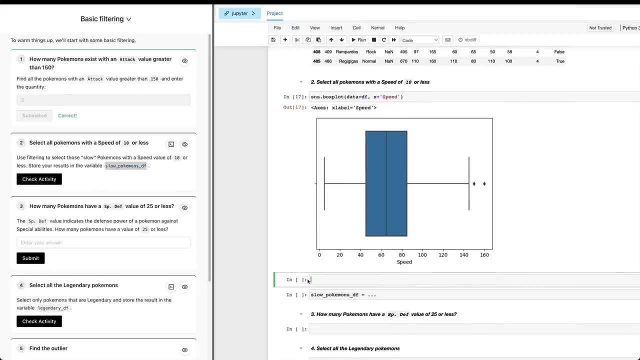 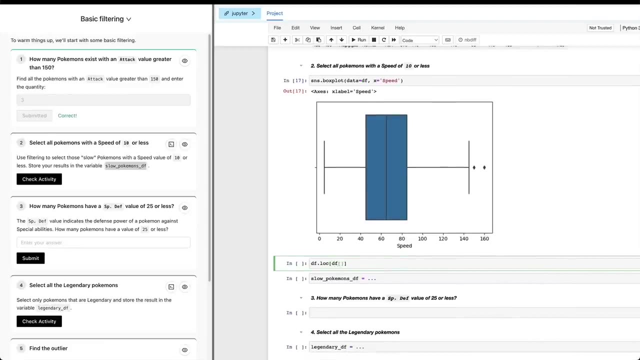 that's gonna be pretty, pretty slow. it's right below. here we have probably 10. it's gonna be a pretty small amount of pokemons, so let's take a look first how many fulfill that condition. speed: df at miss type speed is, uh, 10 or less. so this is less or equals on 10, and we have only a handful. 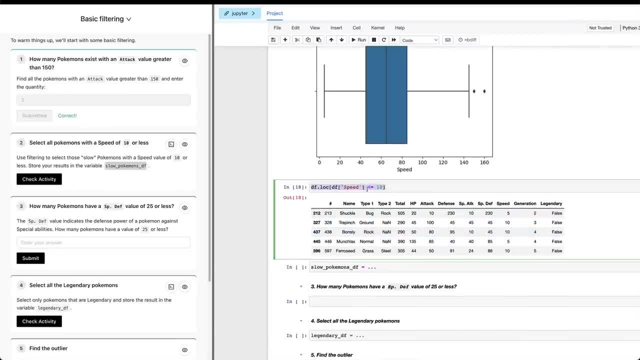 one, two, three, four, five, um, and we can of course assign that to this variable to have a final check with activity. let's do it on the side in parallel. there you go, it worked. and of course, using dot query, it's query speed, df, dot query, and we can of course assign that to this variable to have a final. 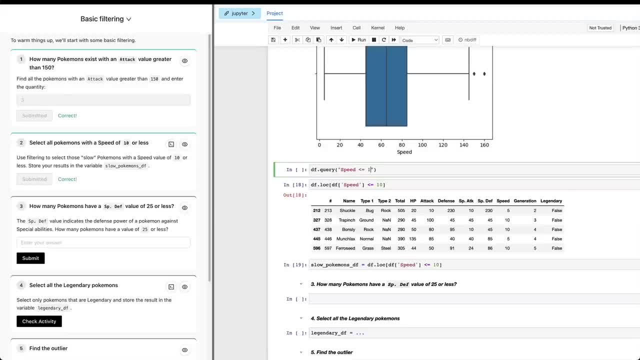 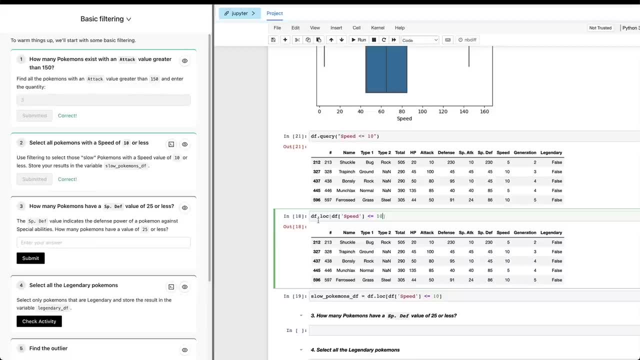 check with activity and we can of course, assign that to this variable to have a final check. speed is less or equals down 10.. from now on i will try to stick to the dot lock method is the one that i prefer, um, instead of using query. but you know you can use either, i prefer. 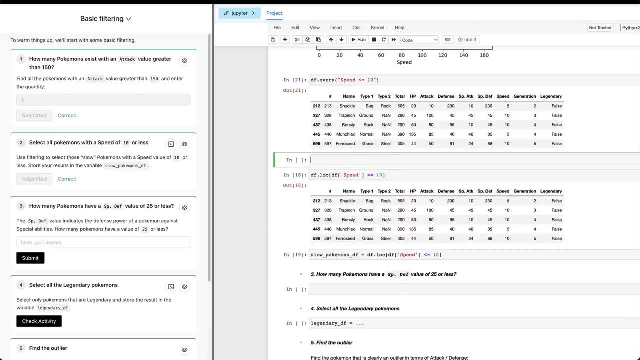 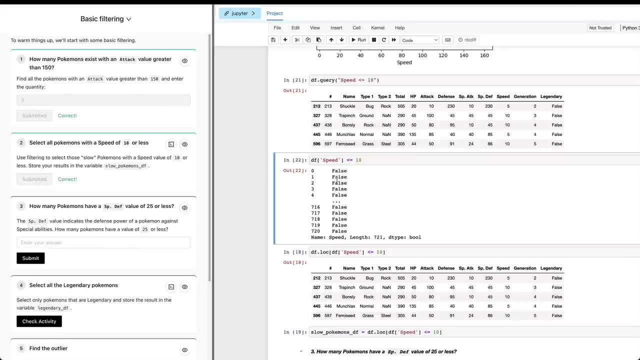 to work with boolean arrays. remember this expression. it's gonna be just a boolean expression, right? so how many of these values are? the values are true are basically that, the values that match the given condition. this is pretty useful if we want to count the values, and this is something. 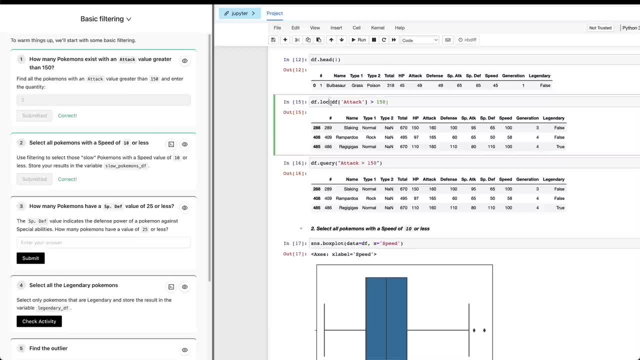 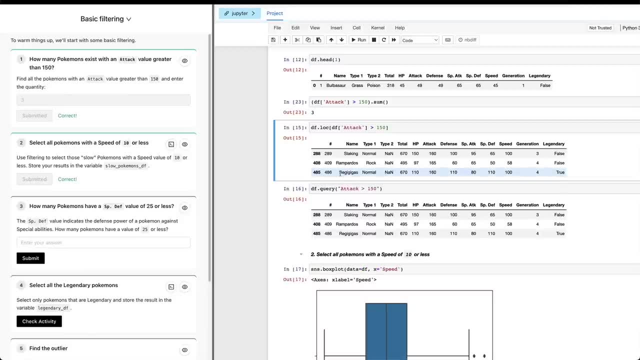 that i could have done in the previous one, which i didn't realize showing before. basically, if i did something like this dot sum, i'm gonna get the same result right: how many values in this full array? so arrays and attack. is an array, let's say a series, a collection that has integers, and then 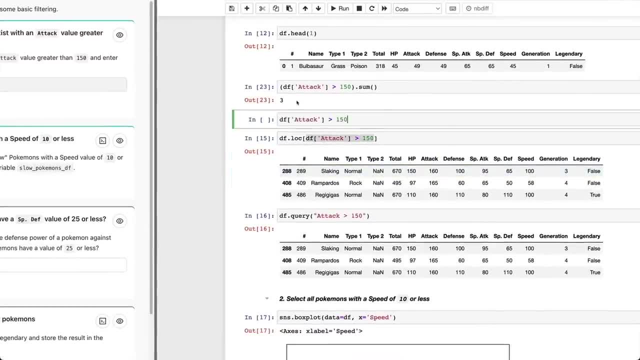 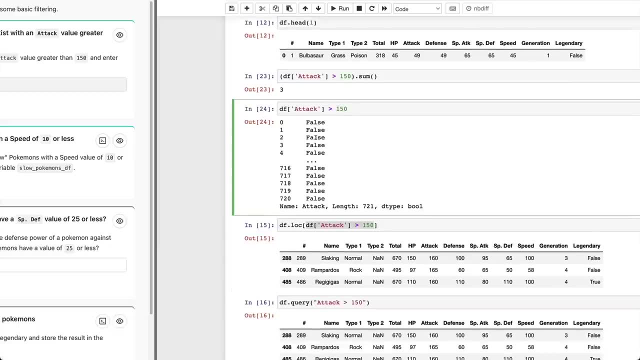 we ask: give me an array, a boolean array, of all the ones that match this condition, in this case greater than 150. so it's going to be false, false, false, false, false, and of course i'm going to have three in this huge array that are true. so in this case, as i told you in the previous project we did with english words- 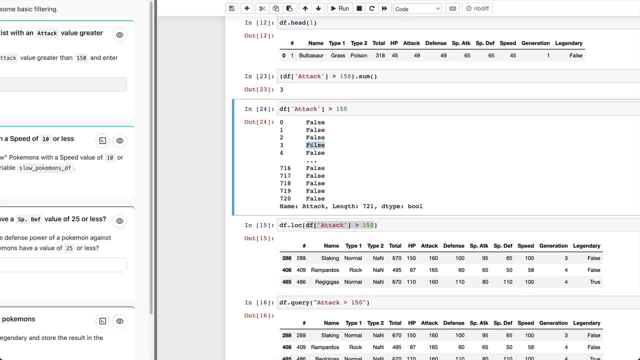 if the array- in this case it seems that they are just, you know, strings saying false and true, in reality this is a boolean array. so in reality these are all ones and zeros. very efficient, very compact array. ones and zeros. we can sum that and we have the final result. in this case, we can count, we can sum right all the ones. 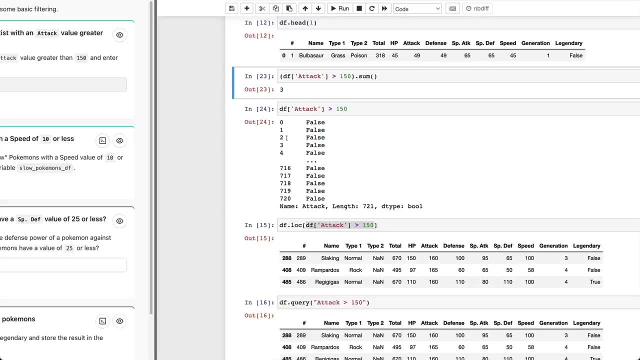 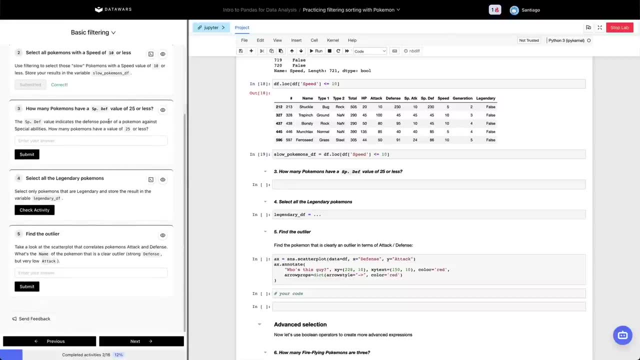 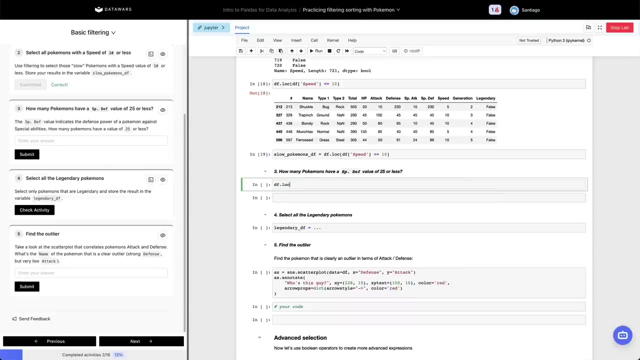 we have just three ones, and that gives us the answer to the previous question as well. all right, moving forward. um how many? let's go here. how many pokemons have a sp death value? special defense value of 25 or less? um, special ability defense. so we're gonna do dflog how many? 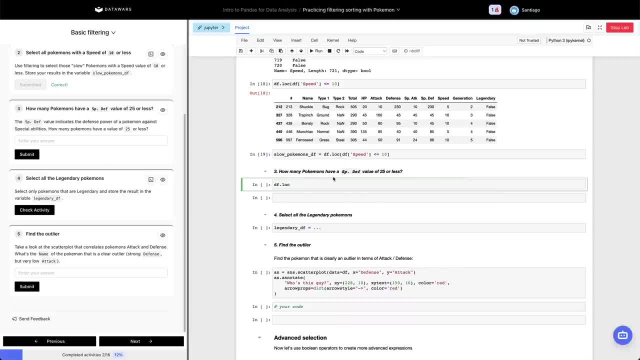 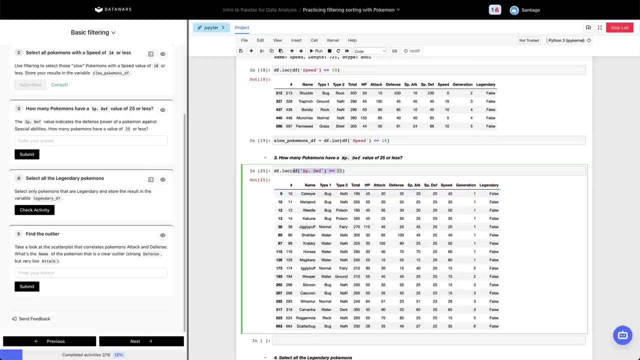 pokemons have a special defense value of 25 or less. we're gonna do df at spdef less or equals than 25, because again it's value of 25 or less, and now we have a bunch. so now we can use the technique that we did before. that is just this. 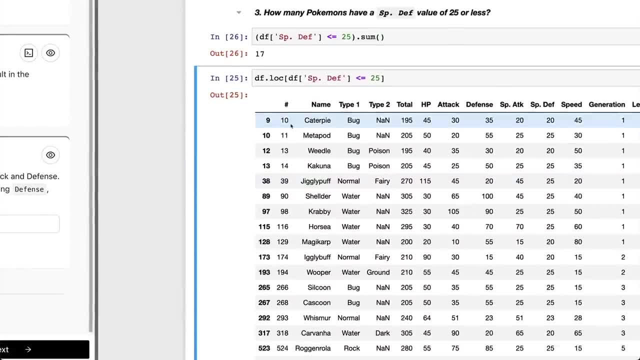 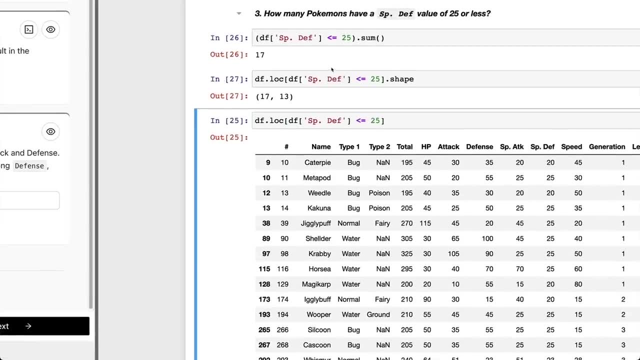 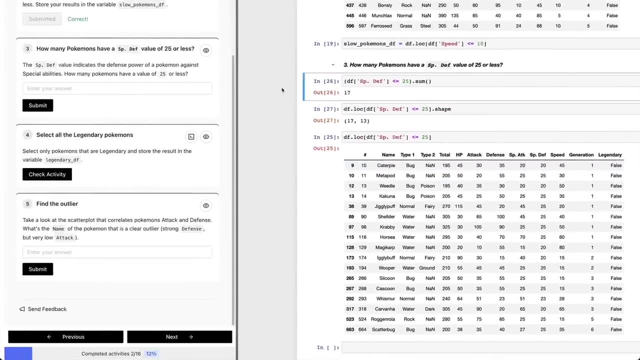 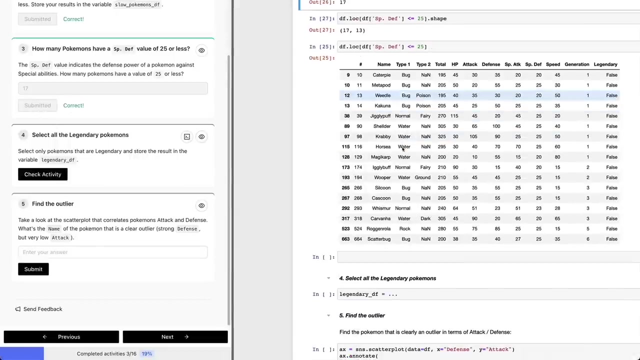 we got some gonna criticize here a bit and we have 17 as a result. i could have done the same thing here: shape and i get pretty much. this table has 17 rows. of course this is a little bit more compact, let's say easier. so let's try it out 17 and see if it works. there you go, they work, we're good to go. 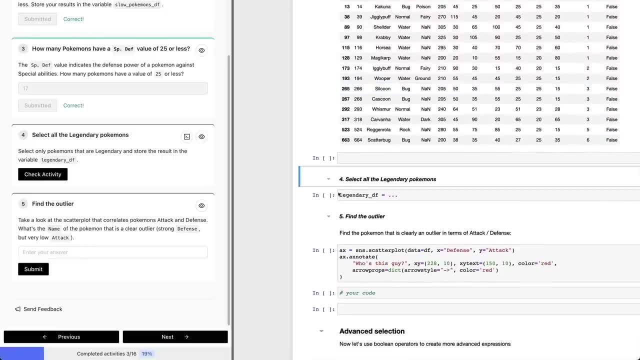 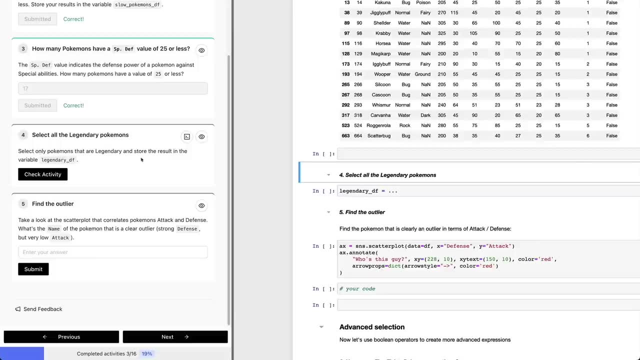 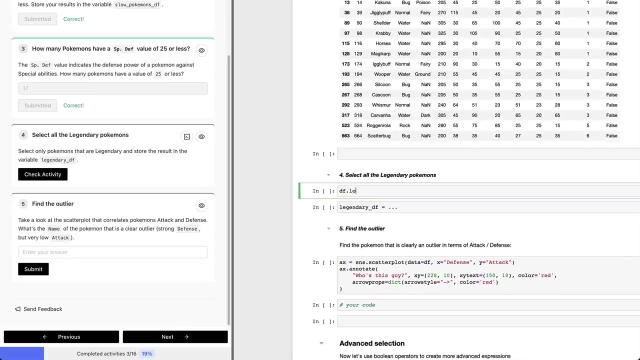 and keep moving progress, making progress. so select all the legendary pokemons. this is pretty interesting one. we have to sort the result. select only pokemons that are legendary and sort the result in the variable legendary dot, legendary df. so that's gonna be dflog df at legendary, but let's 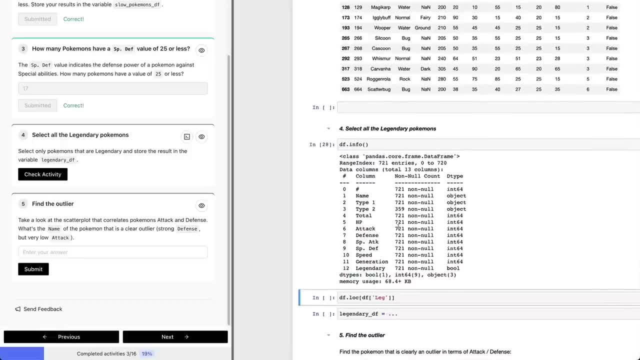 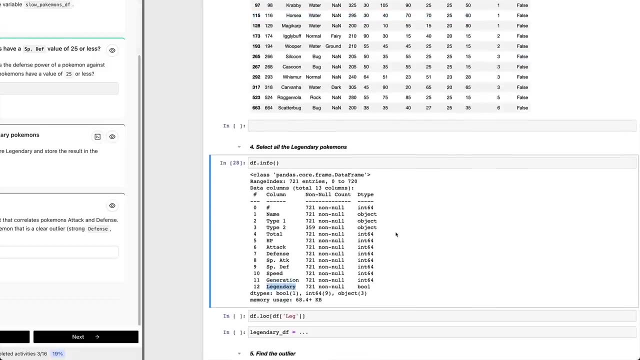 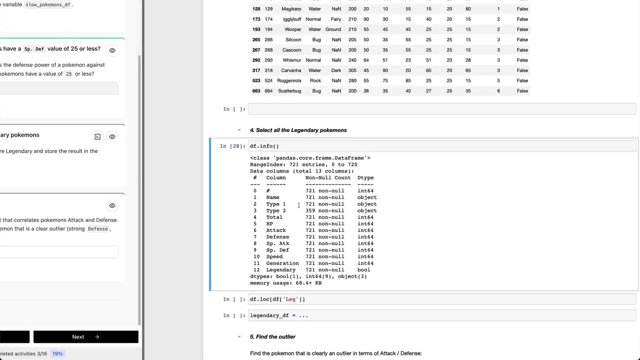 take a look. first, using info method, let's take a look at the legendary column. the legendary column itself is a boolean column, a boolean series given by its type. so that means that it is itself a boolean array with true and false values. we could ask df at legendary how many? 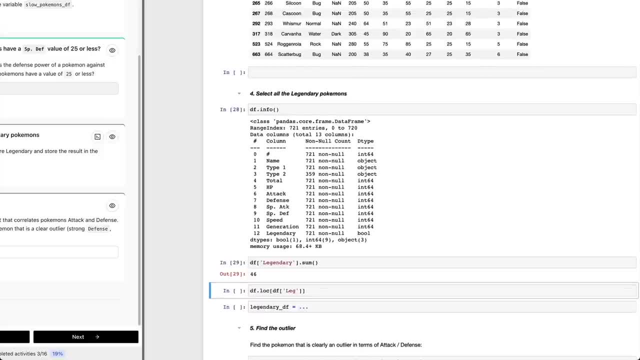 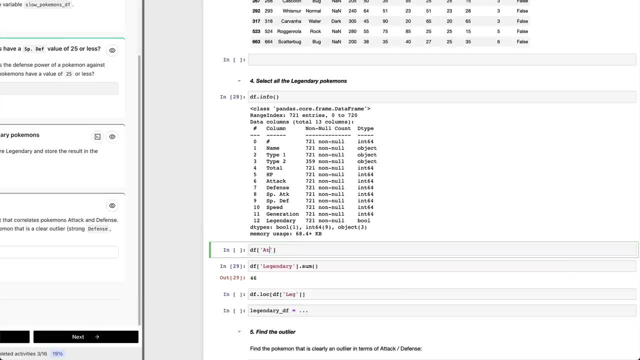 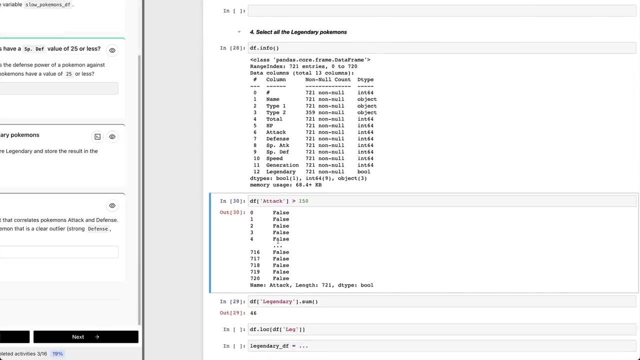 legendaries pokemons we have in this data set and that's just the sum of the legendary status and that's it, because this is a boolean array. so remember, if we did df at attack, for example, greater than 150, and we had this huge boolean array- false, true, false, true. and then we selected: 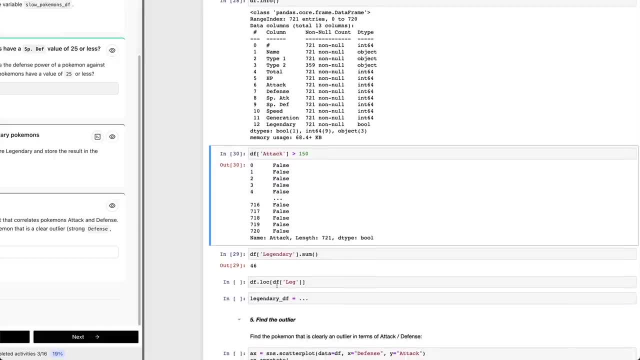 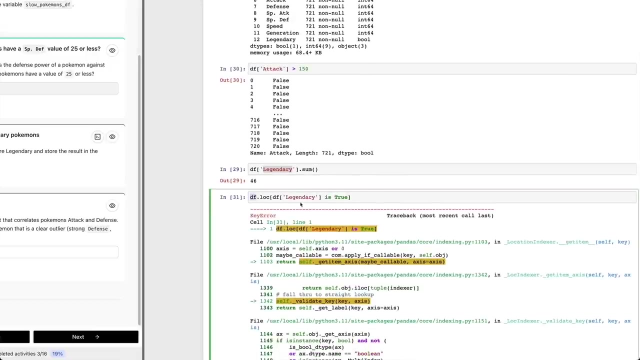 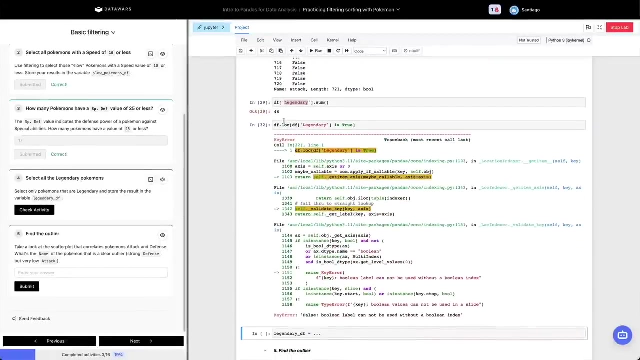 the ones that had a true value. we can pretty much do the same thing here. so we can do the same thing here, and what i'm gonna do is we could say something like this thing is true, right, so give me all the legendary pokemons. uh, what did i do wrong? um, false kind of oh, boolean index df. 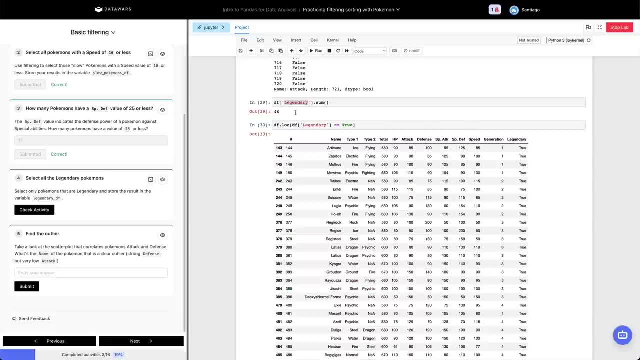 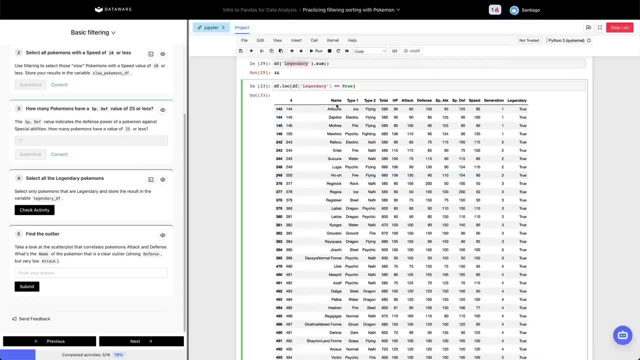 is equals. there you go. my bad is equal to true. but the reality is that the boolean array is true, is that this column itself is a boolean array. so let's just get rid of the true and we say: select all the the pokemons that are legendary, just that. just pass the mask, the boolean mask. 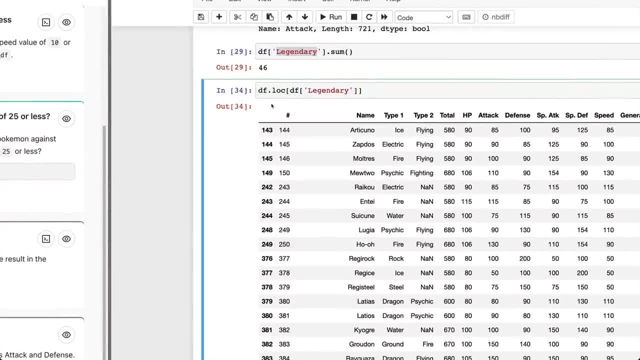 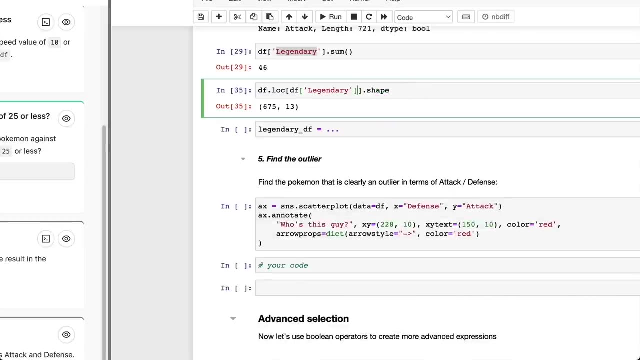 and perform the selection if we want it. let's say we wanted to get all the pokemons that are not legendary, the not the non-legendary pokemons. we can, of course, do something like false we're going to get how many we have, but the reality is we can just invert the array. we had false, false, true, false, right, that was our. 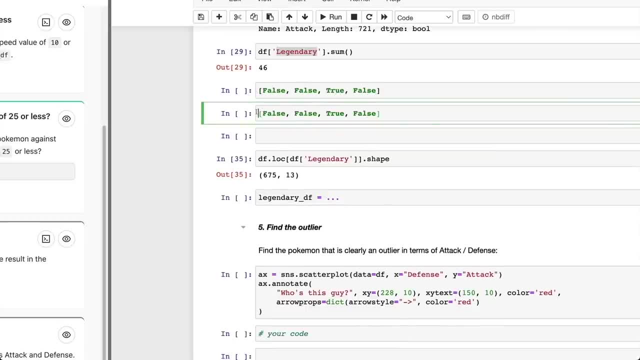 original array. we can do inversion of this thing, negate it with this operator. that's going to give us true, true, false, true. this is false. so what i can do is i can just do the negation here and i get the same result. so sorry, i got a. 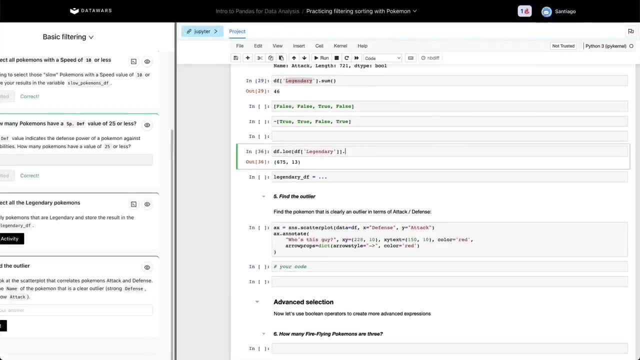 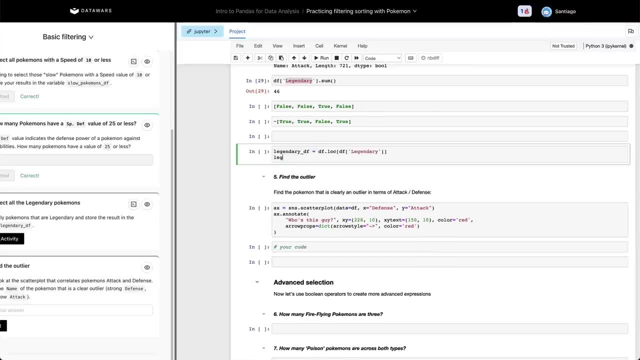 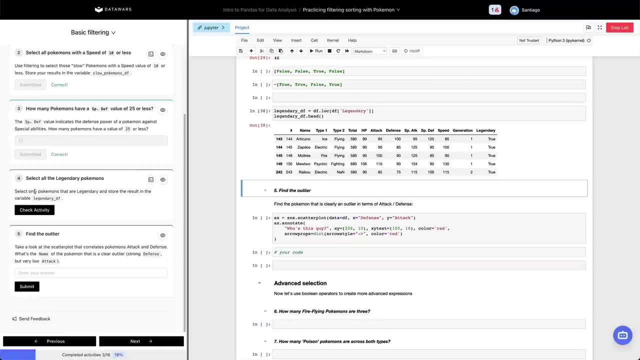 little bit sidetracked. what we want to get is all the pokemons that are of type legendary, and to do that, we're gonna assign that to this variable and we're gonna get the head first five rows. there you go, all legendary, and let's check if the activity passes. this is why it's so important. 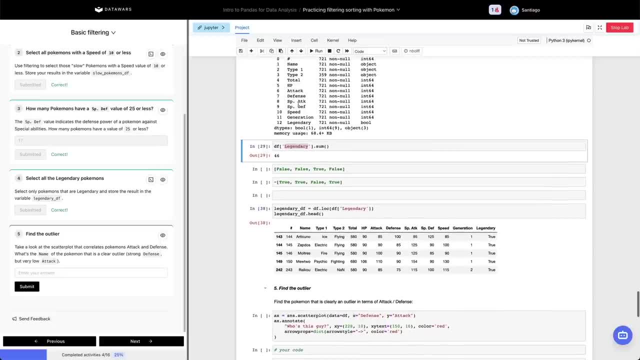 to understand the column types of your data, because sometimes you know the selections or the boolean arrays you're going to be working with are going to be the ones that are going to be working with are not the same depending on the type of the data you want. you have, okay, moving. 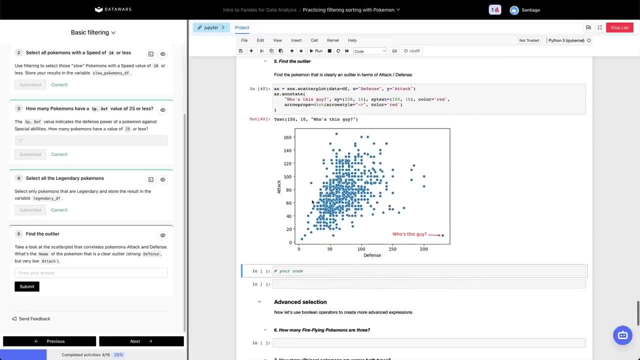 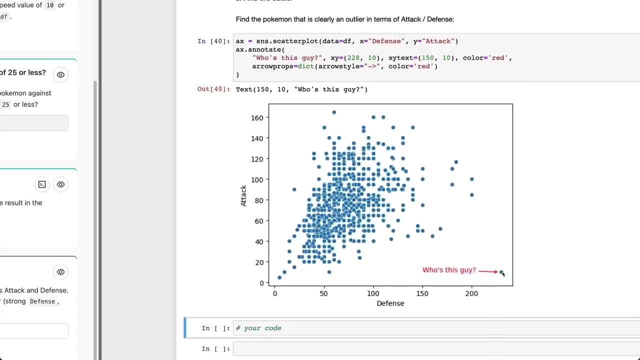 forward, find the outlier. so we have this distribution of pokemons and we have to find this particular one, the one that has a defense value that is pretty big and also an attack value that it's pretty low, right, so this pokemon has a ton of defense but a very low attack. 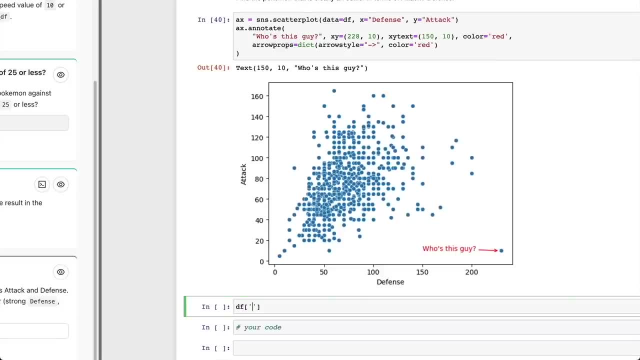 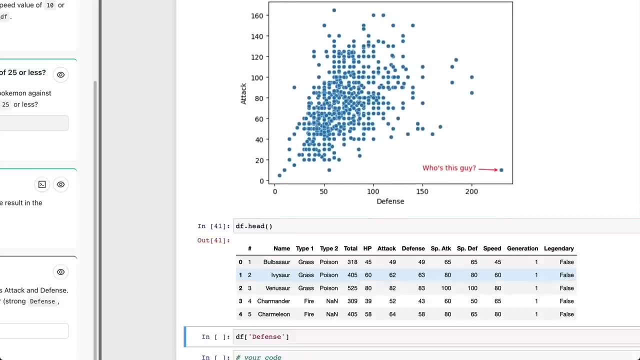 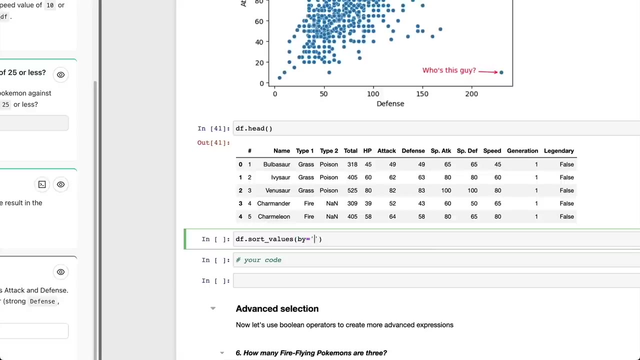 of course we're going to have to find the outlier. and we're going to have to find the outlier, of course we could do something like df at defense: uh, dot, sort, let's, let's, let's do, let's do dfhand, show the whole thing. then we're going to do dfsort values by defense, and 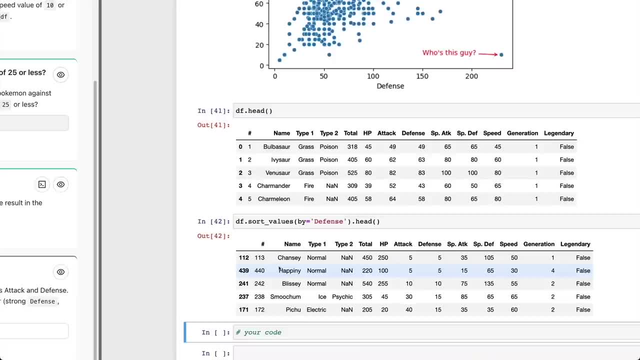 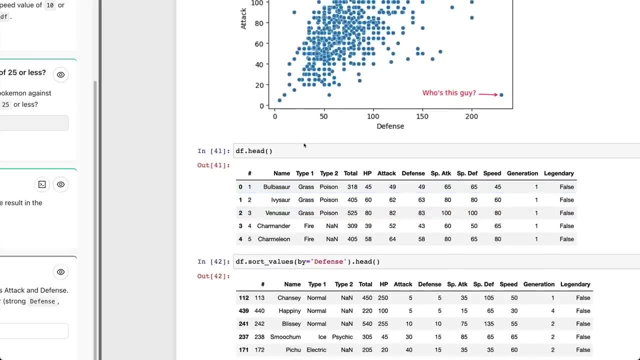 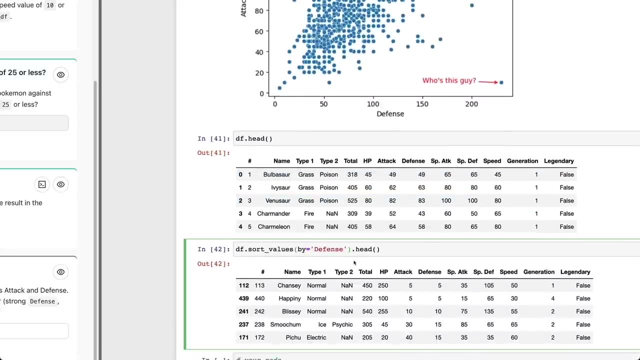 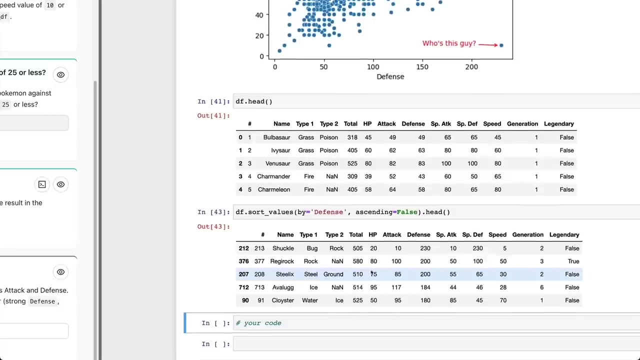 and show the first few. by default, the sorting method is in ascending mode. so we are starting in this way, we're going in this direction, we want to invert that. we're going to do ascending equals false. so now we have the strongest ones here, and here we have the one that has a defense of 230 and an attack right of, in this case, uh. 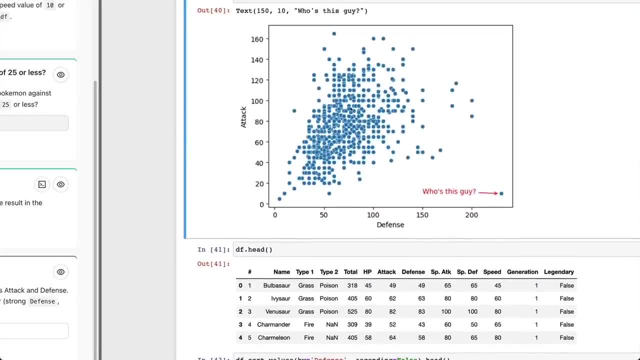 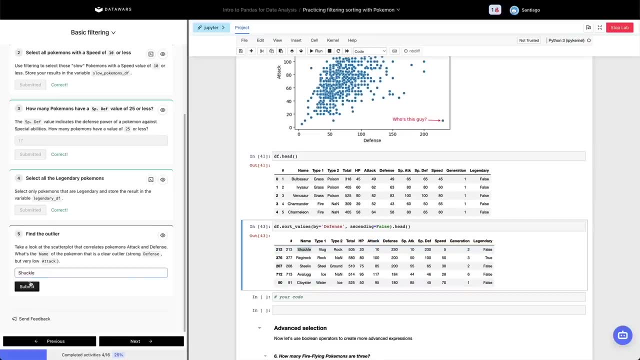 attack here of 10.. this pretty much gives us the the answer right away. let's actually try it out, let's see if this is the one. this is the pokey that activity requests, at least for this particular value. it is that passed, but i want to make it. 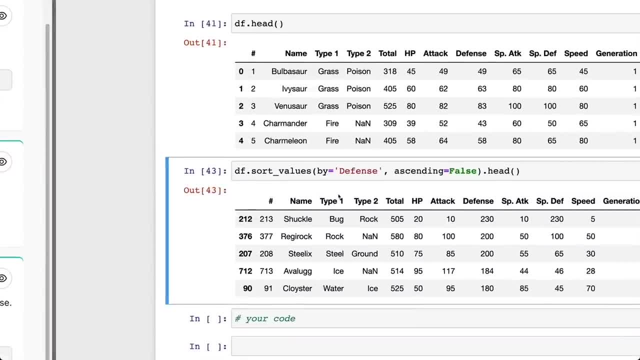 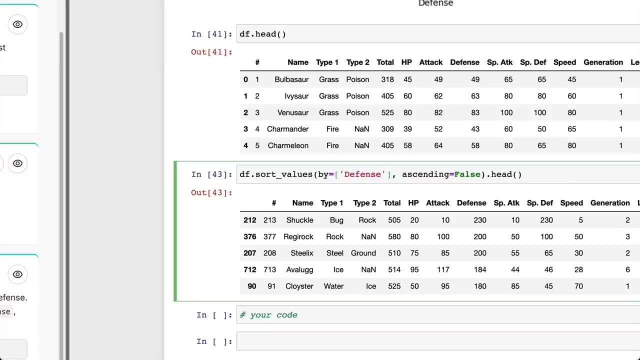 common here is that you can, you can actually sort by multiple um, by multiple criteria. we could also say something that's sort by defense first and then, as a second criteria, sort by attack. there you go, and then for defense we want it to be in descending mode. so ascending is false, but for 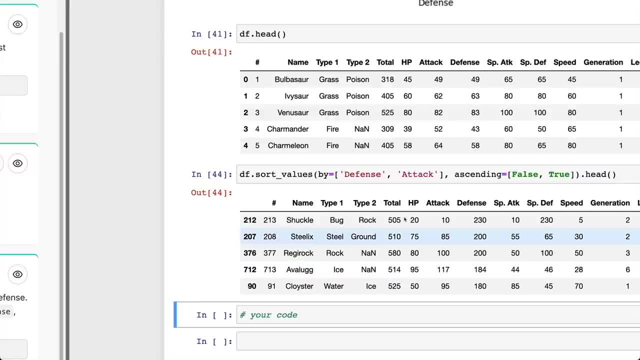 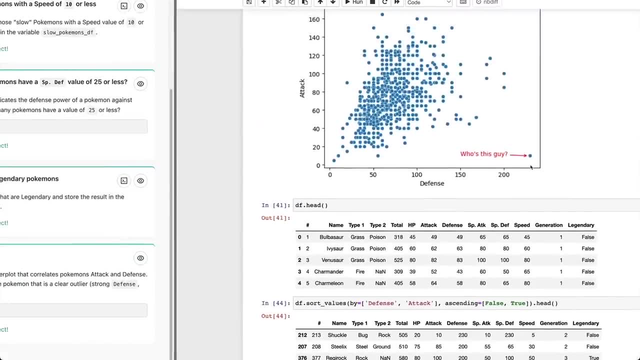 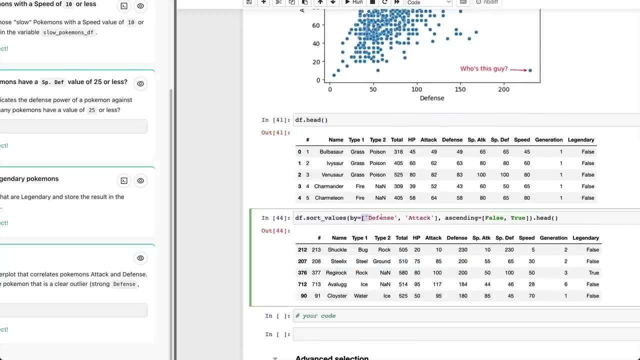 attack. we want it to be in ascending mode again. the result is the same because the data, it's pretty clear. who is this um outlier right here? but again, the understanding is we can sort by multiple criteria. what's going to happen is that the sorting starts here and then we're going to 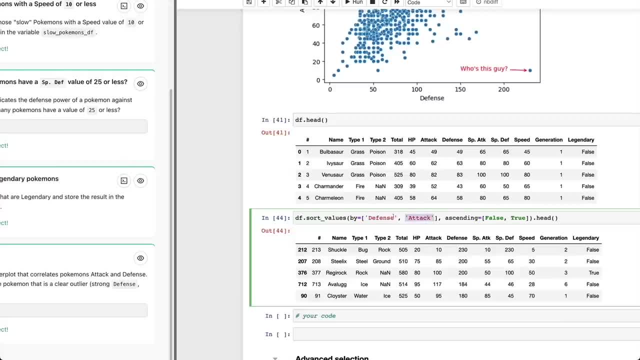 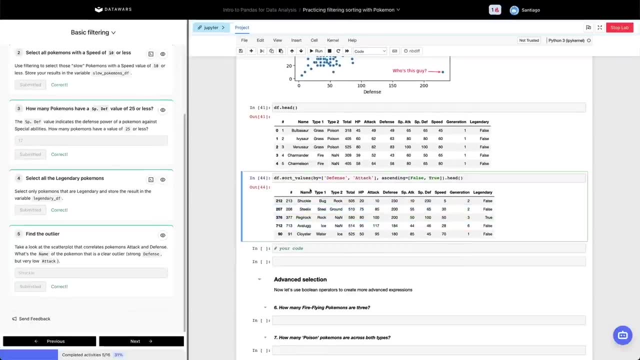 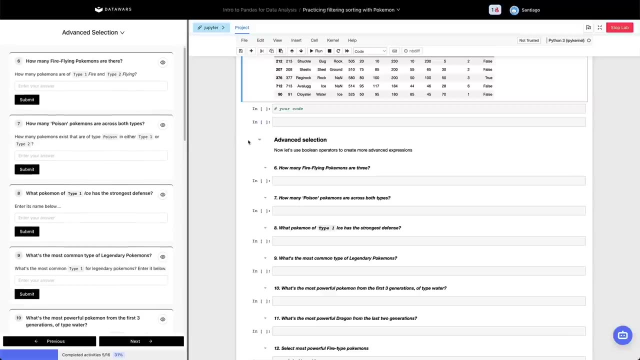 sort by attack in the other direction. we can combine as many as we want of this criteria right here. um, all right, moving forward, more activities. now we're going to get into advanced selection with some boolean conditions. how many far fly pokemons are there? so we want type 1, equals equals fire. 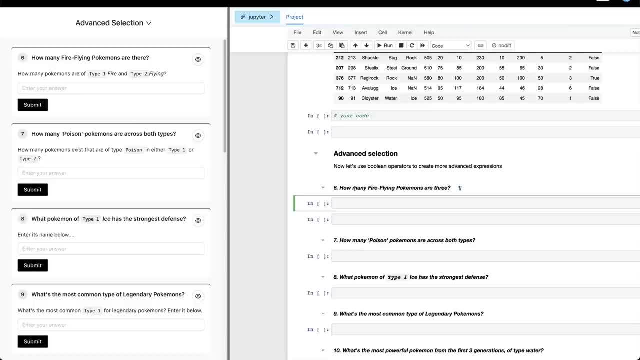 and type 2 equals flying. so what we're going to do is we're going to do dflock and up here again- pause if you want- we're going to do a little bit of boolean operators. the first condition is going to be df at uh. type one is equals to fire right. and the second condition- and how many do we have? 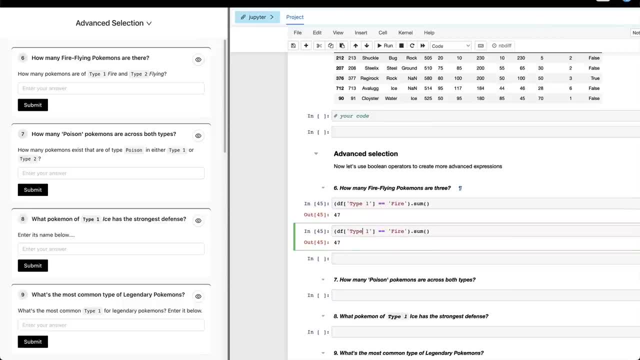 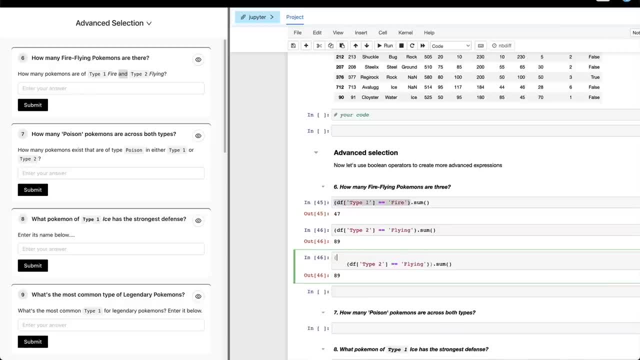 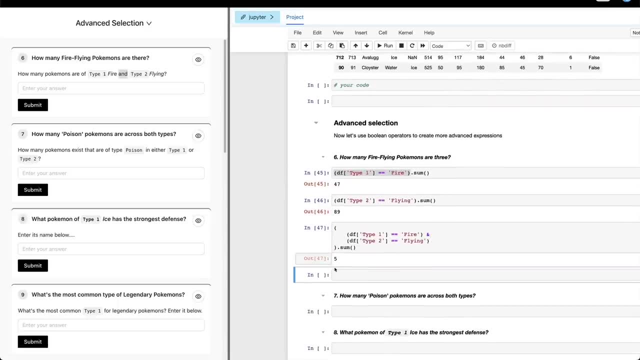 an ampersand operator. So I'm going to break it into different lines here And I'm going to put the operator right here. So you see the conditions. How many far flying Pokemons are there? Seems like we only have five. let's try the result first, And then we're going to explore a little bit more the 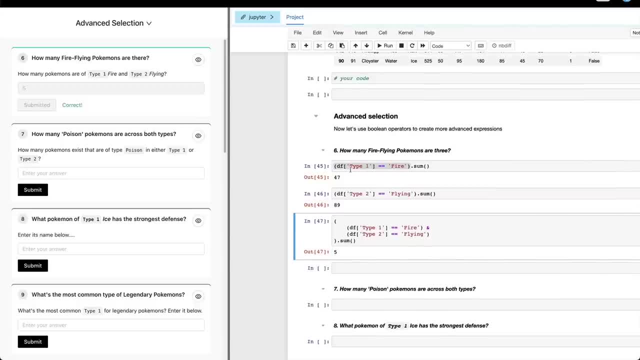 the data frame resulting And, as you can see, I haven't even looked at a single Pokemon. what I'm doing is just combining conditions and summing Boolean arrays. So this is a pretty interesting thing, Because what is happening here is like, let's say, we had only five Pokemons in. 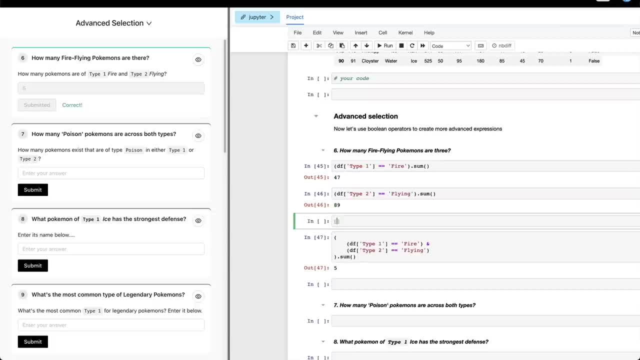 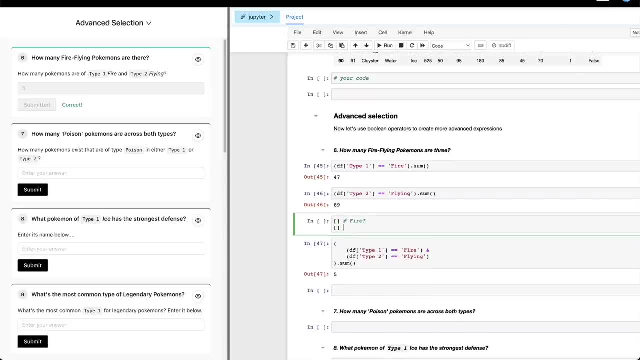 total right we have. and we have the first array here is going to say: type is is fire, and the second array is going to be: is flying right, And we had something like true, true, false, true, false. 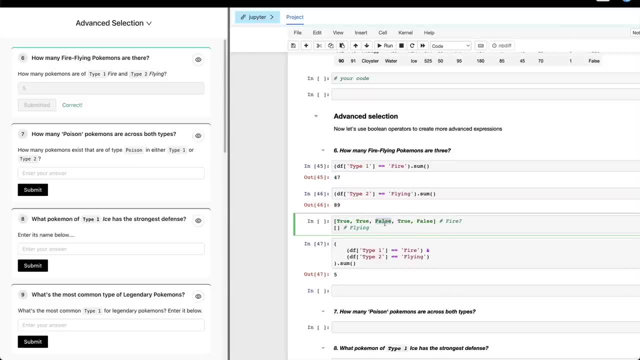 So this is a type fire, type Fire, not type fire. Yes, type fire, not type fire. And then for flying we had false, true, false, false, false. There you go. So in this case, this is the only. 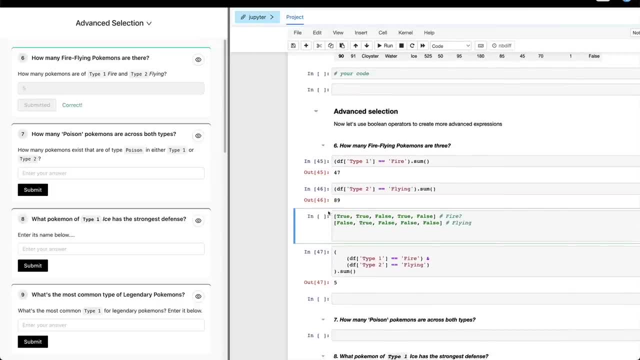 flying Pokemon. What happens? and that's why we have like different results. Of course, we had here a bunch of fire fire Pokemons And here we have a cup of a bunch of flying Pokemons. we have true, valid, false, true, false, false. So we're going to roughly classify them And we are going to 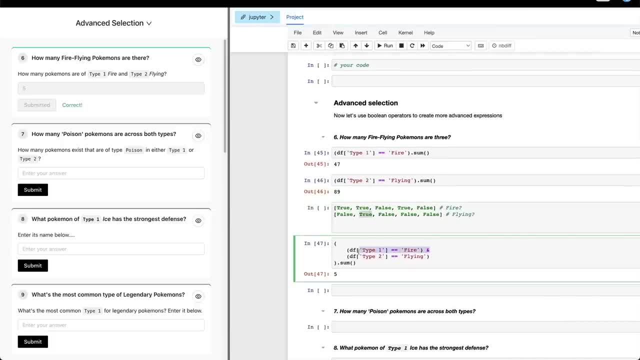 for the condition. but what happens when you we use this ampersand is that we do one by one, bit by bit, boolean value by boolean value, we do the operation, the ampersand operation, which is like the and operation in python. so we do true and false for the first one. so the first one can be: 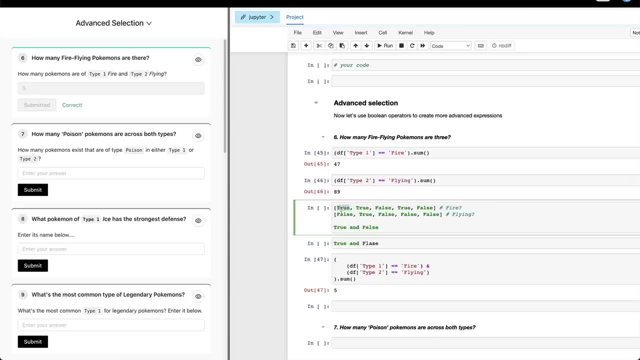 true and false. what is the result of true and false, false, and what then we do? the result of true and true? what is the result of true? and let me show you: true and false is of course false. true and true is true. so we have that. false and false is false. true and false, again, is false. 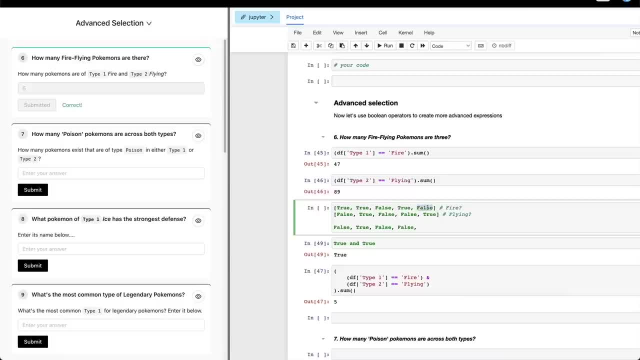 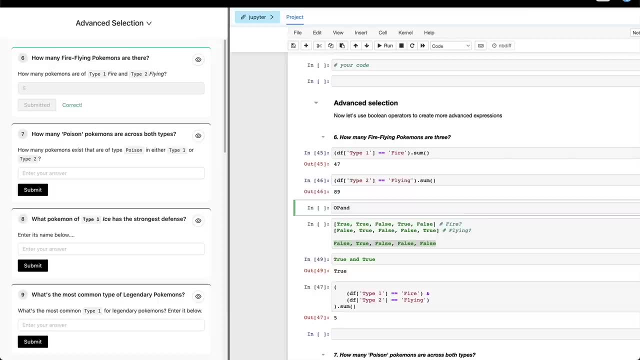 and we could say this one was true, false and true is false. there you go so in an and operation, and we have operate operator one and operator two, or operand operand one and operand two. for this expression, for this whole thing, for this whole expression to be true, 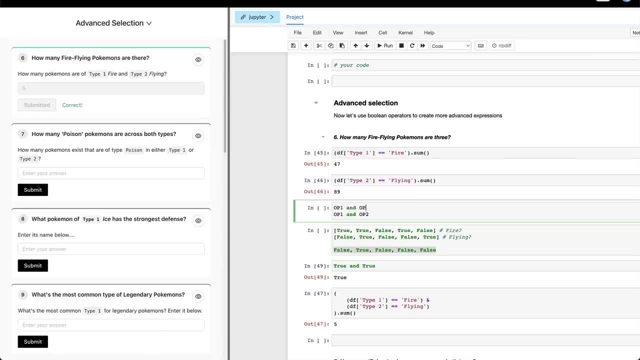 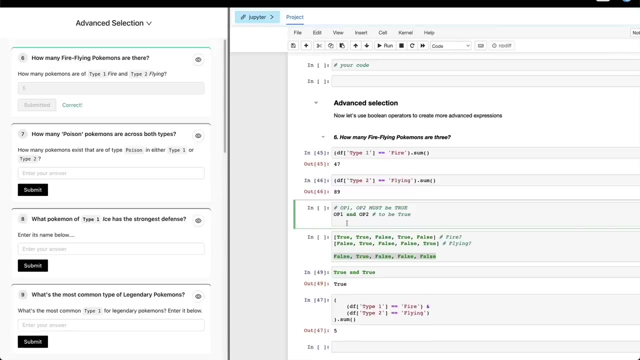 both op1 and op2 must put it this way must be true for this operation to be true. anything else, either op1 is false or op2 is false, or both are false. anything else, anything else, is false. this is just some boolean arithmetic um boolean operation operators, just. 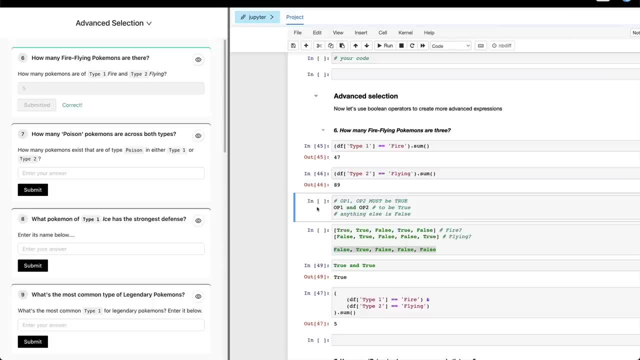 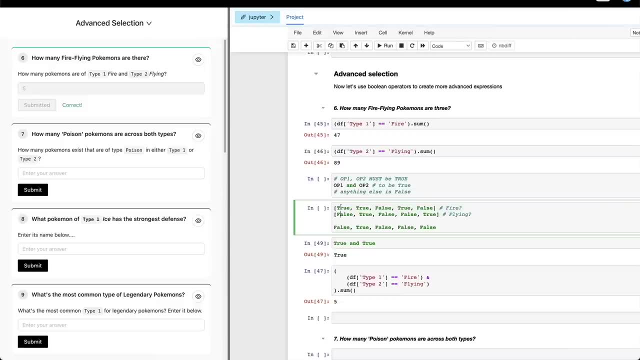 you know a little bit of that applies to python as well. but the interesting thing is that that same operation we're seeing here- a comparison bit by bit, value by value align- is what we're doing right here. so we had 47 pokemon's were of type 1 fire. 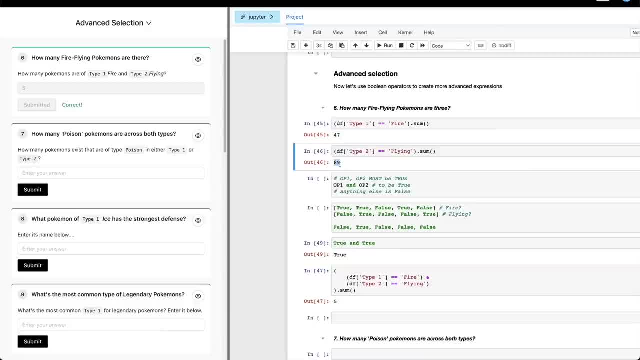 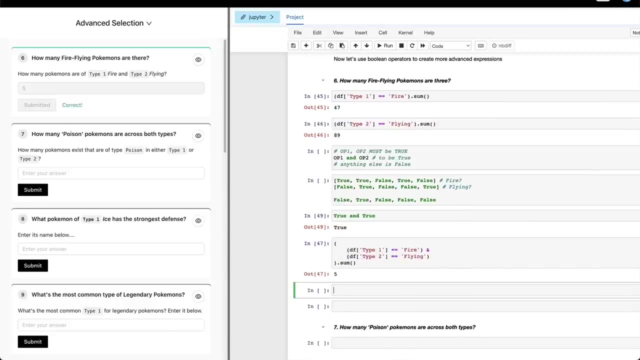 and we had 89 pokemon's were of type 2, flying, and then we combined those things using an ampersand and and operation and the result was only five pokemon's. so we can- we can- actually visualize those sample points. we're gonna do log. 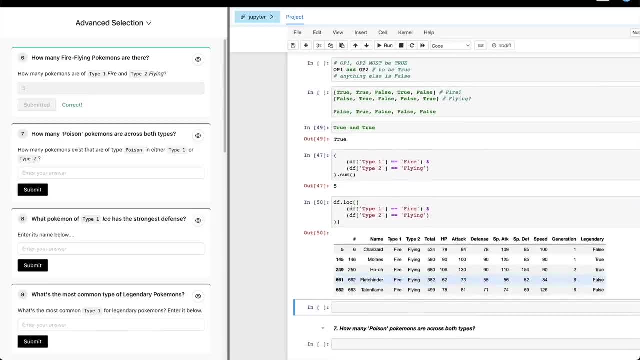 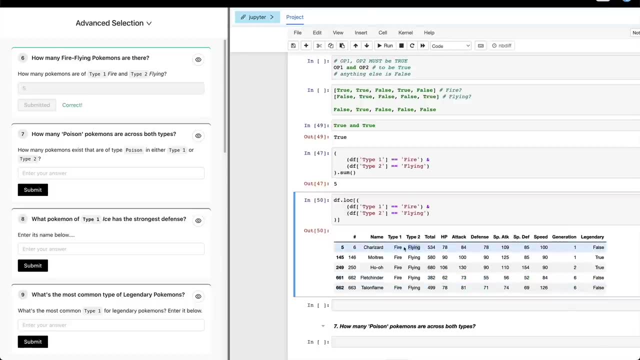 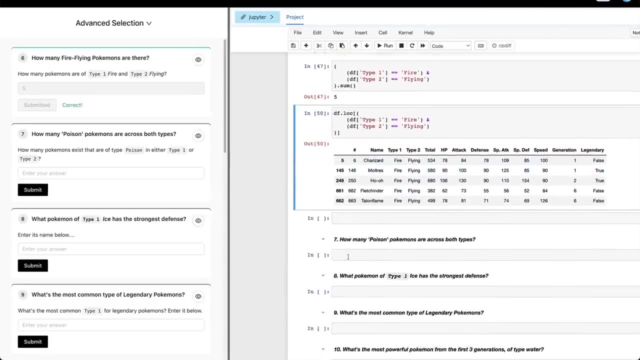 and we're going to pass that condition. and these are the only five pokemons are of type one, fire, and type two, flying. okay, because we are using these boolean operators. okay, moving forward, how many pokemons? oh, no, one thing. one thing. if we wanted to use a query method, we could have. 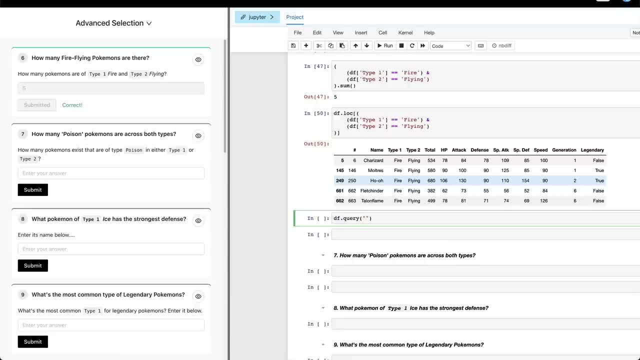 rewritten this thing with query, and we're going to do. remember that if you have white spaces in your column names, you have to surround that with backticks. in this case going to be fire and type two. type two equals flying, and i made a mistake here. flying should be a string. there you go, we. 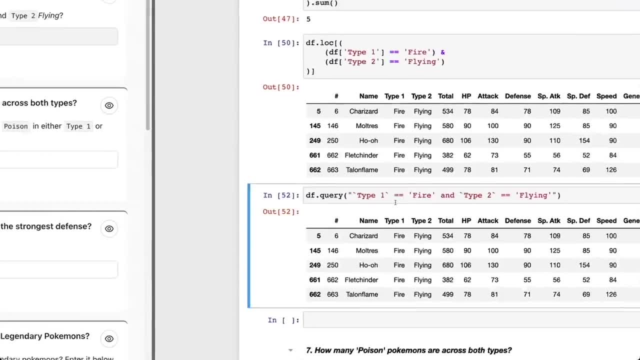 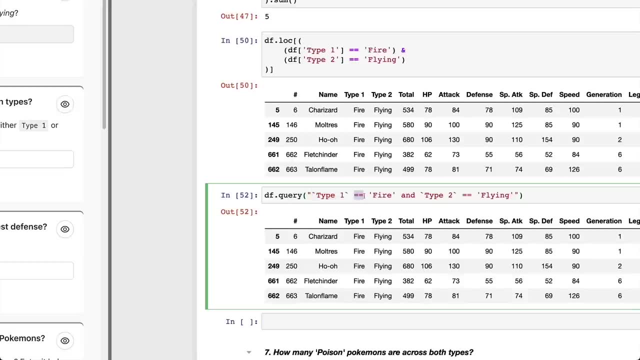 have the final result. so again, this is: this is easier to type. probably we need to put the backticks in the column that has a white space and here we can just use python and we can use a string. you have to make sure you're not you're. 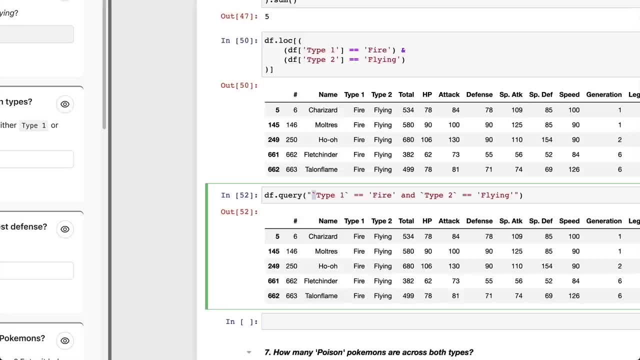 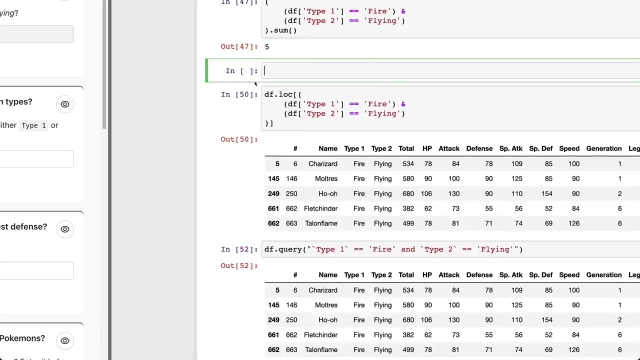 matching or, on the contrary, not matching um, the strings, the string quotes, use you're using to surround the whole expression um. and then we, within the boolean operators, we use the regular python ones. we don't use the and percent, we use just the and. when we are using dot lock form, we must use the boolean operators are and or a, not and, if we're. 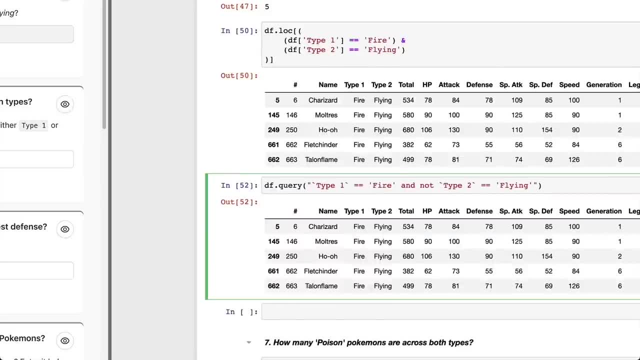 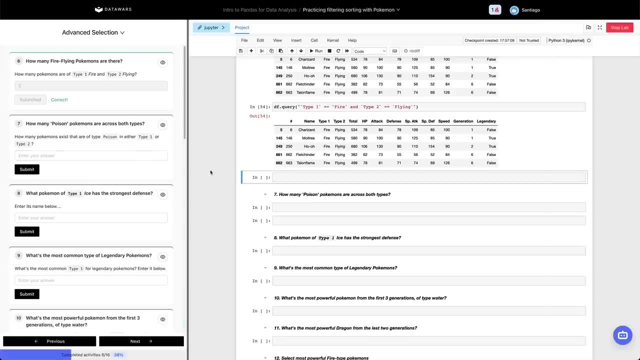 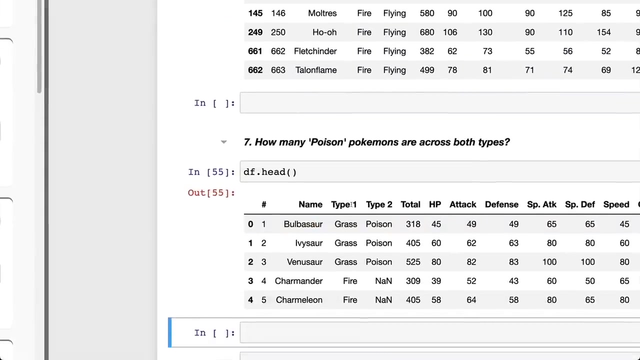 doing something here. uh, let me see if i can do not. yes, we can do a not right here as well. okay, now moving forward um activity number seven. how many poison pokemons are across both types? so, as you can see right here, um, the type of a pokemon is, a pokemon has two types. let's say it has a strong type and 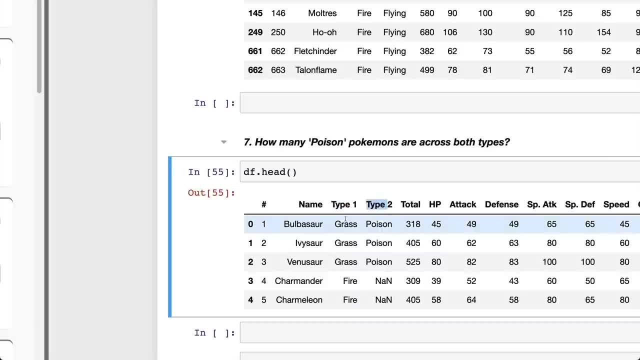 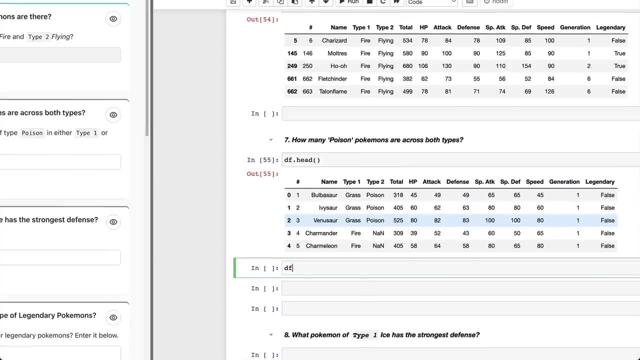 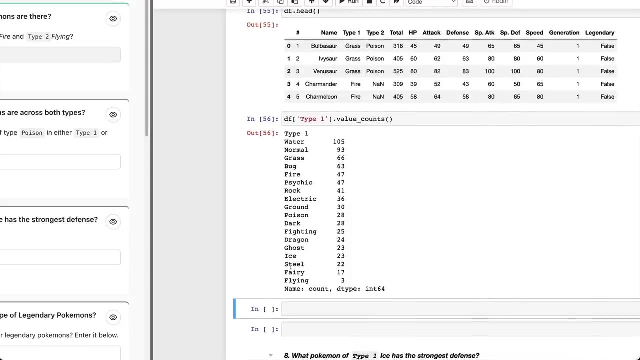 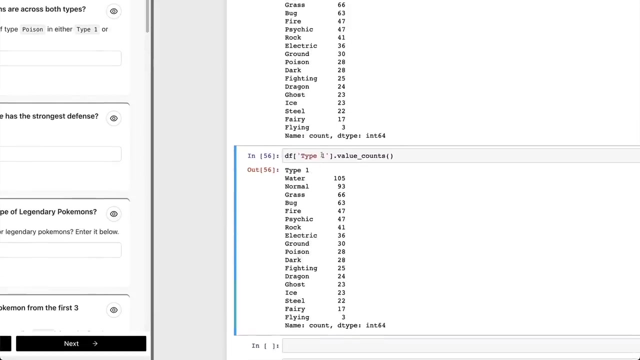 a and a secondary type. the type poison can be applied to either the primary type or the secondary one, because i can actually show you that to you type one counts. we have that. there are poison 28 pokemons that have poison in type one and type two. 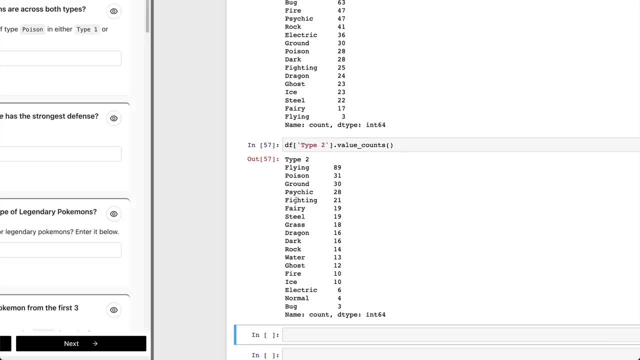 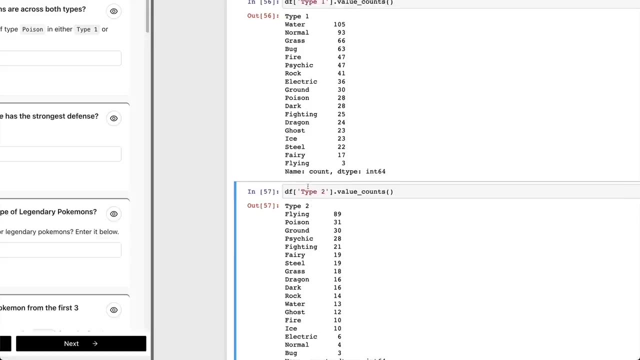 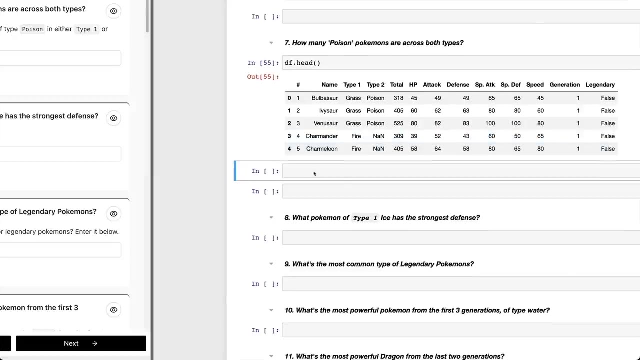 there are- where is it not? 31 pokemons that have poison as secondary type. so we want to basically say: or find how many poisonous pokemons are there in general, right, how many poisonous pokemons we can find in either type. so the expression, and let's start now with the query method. 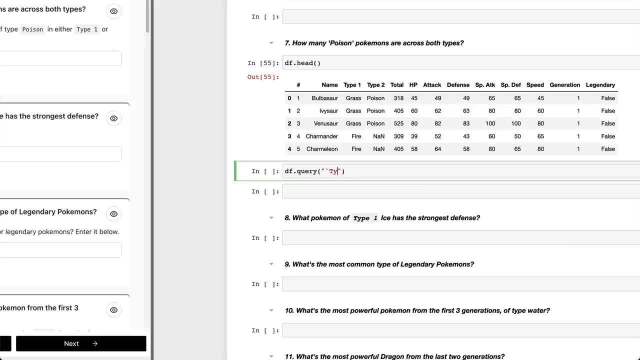 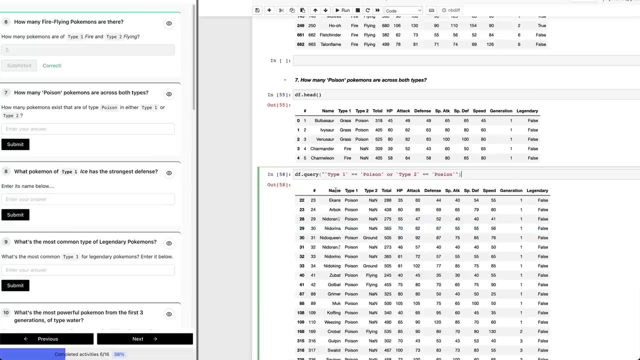 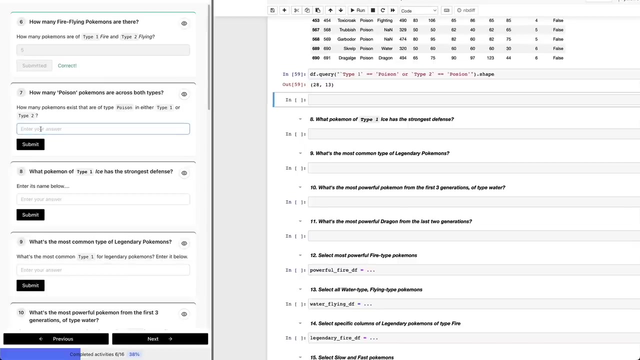 so you can visualize it first. so it's going to be type one equals one, and then we're going to do the query method. so we're going to do the query method in type one, now type two, and then we're gonna do it in a way, but we're going to make it three. 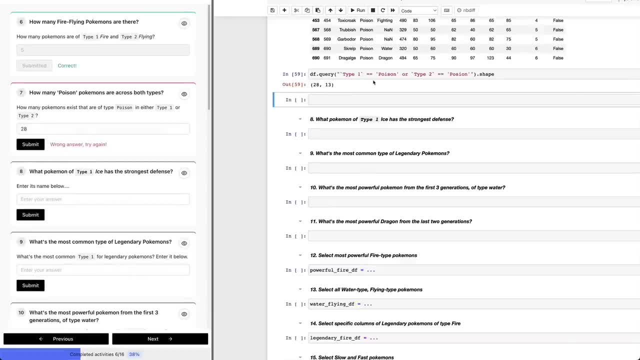 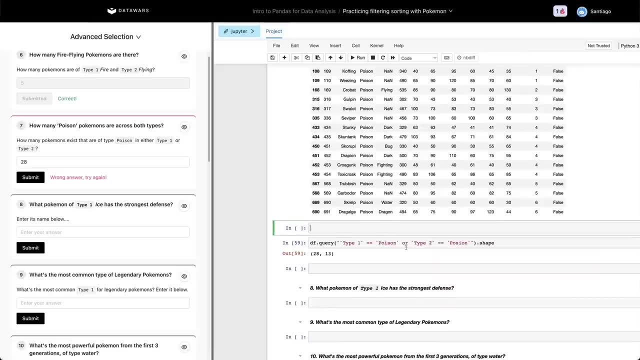 so we're going to break up. aня type two, then type two. now in here over here, type two. type two equals poison dot lock. Oh no, no, no, no, wait, wait, wait, It's just a typo here. 59,, let's try 59. There. 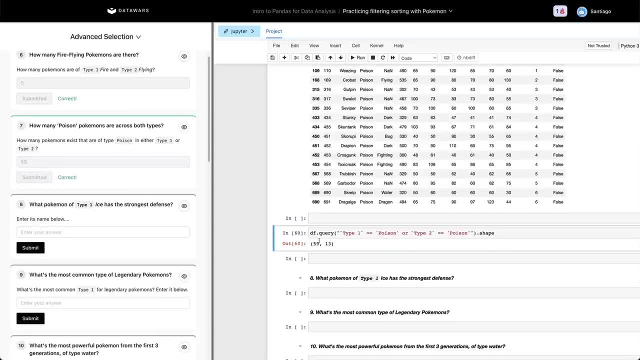 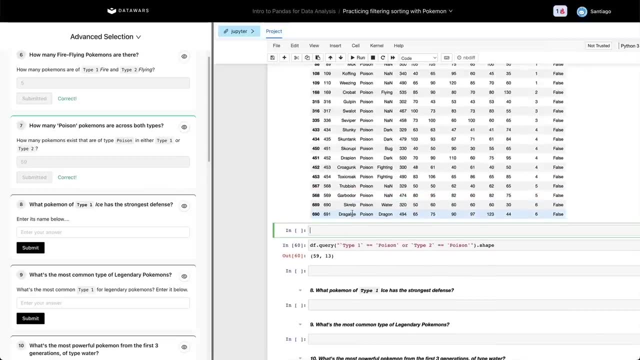 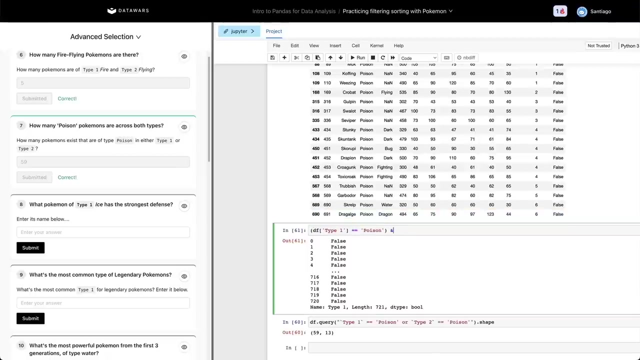 you go, it worked, so it was just a typo. But let's now think about it in terms of the dot lock method. The way it works is pretty much the same thing we did before. df of type 1 equals poison, right? This is going to give us a Boolean array and we can combine that. 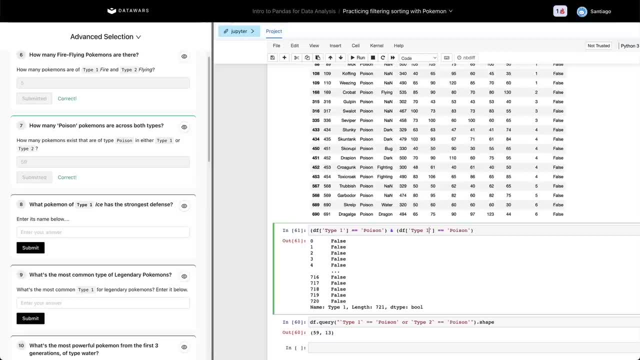 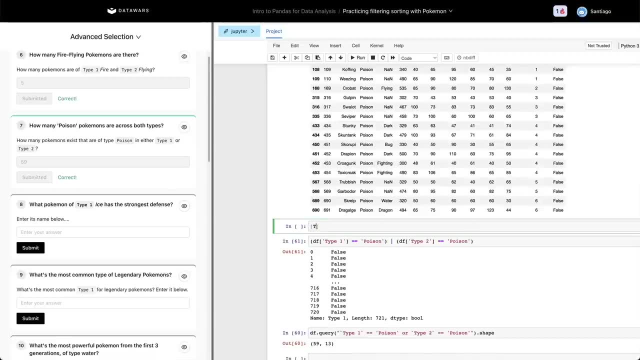 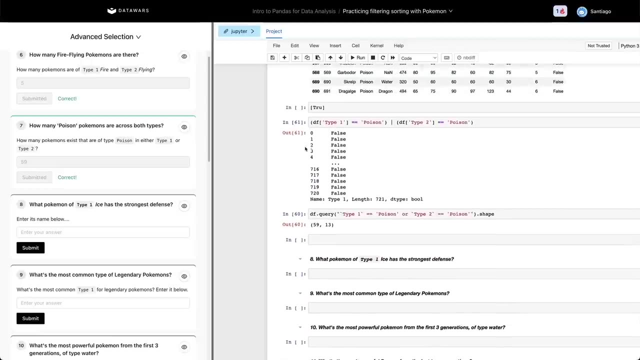 Boolean array, which is pretty much the same expression, which is type 2 points. But here what we want to do is an or operation, and the way it works is: let's say we have- let's see if I didn't delete, there we go- our previous arrays. We're going to use them again. 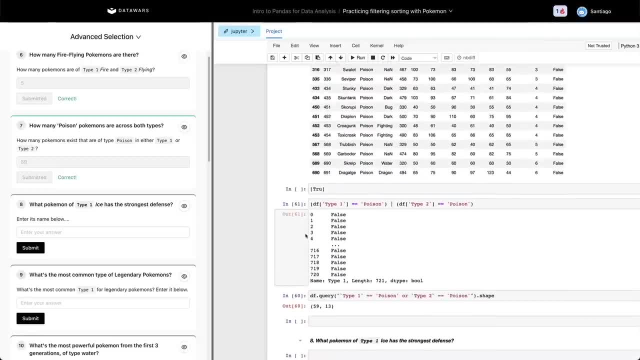 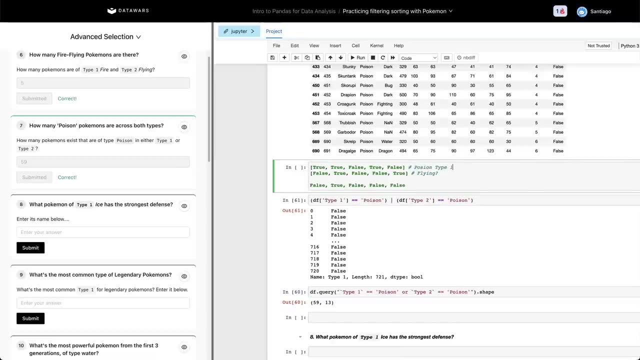 Here, nowhere Here. So let's say we have poison type 1 and type 2.. The way it's going to work now is, as this is an or expression, we care for any of the samples. So if this Pokemon is poisoned here or here, doesn't matter. we want to retain that option. So 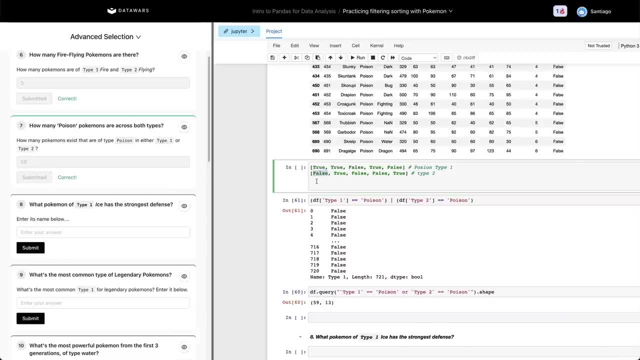 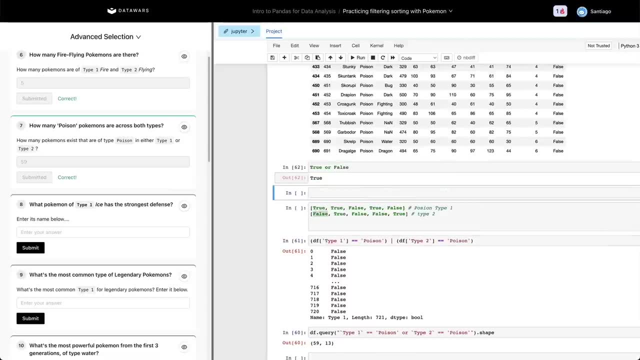 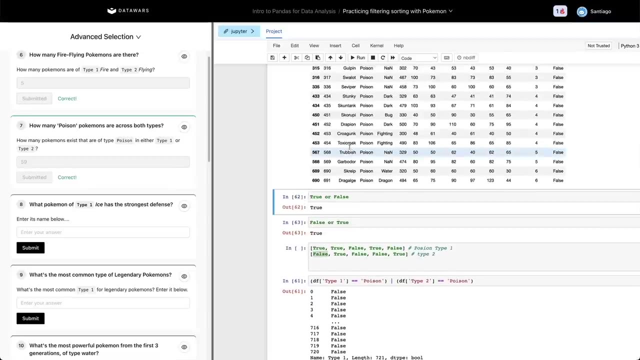 if it's true, here or here, we want to still make the whole thing a true operation. That's the result of doing true or false, for example, or doing false or true right, As we did before- and I can delete this thing and go back to our previous note- we said that if we have 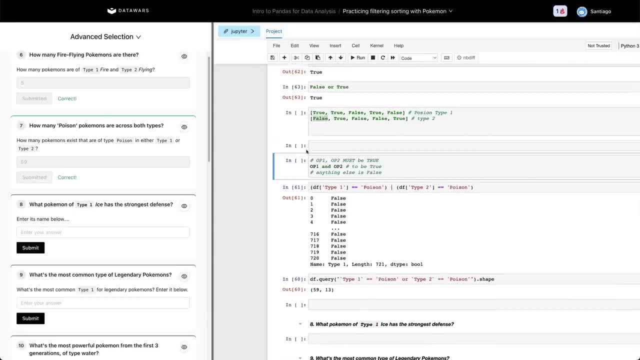 these two operations, that it's op1,, operand1, and op2,, we're going to have a true operation. So if we have op1,, operand2, and I'm still in the- and sorry for the back and forth- 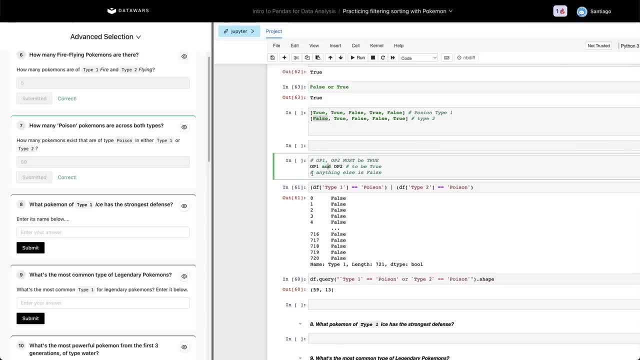 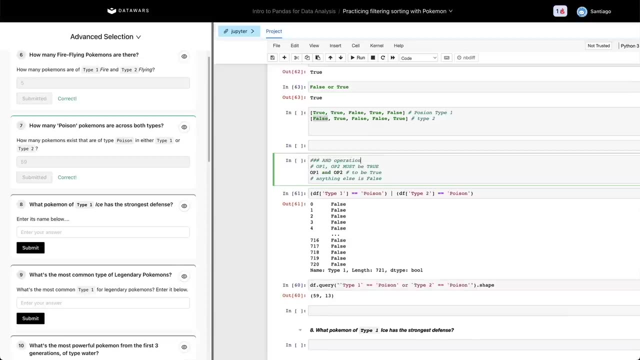 but let's start again. Let's pick up where we were before with the and operator. This thing is going to be true only if both operands are true. So op1 and op2 must be true and this is and operation. op1 and op2 must be true for this whole thing to be true. Any. 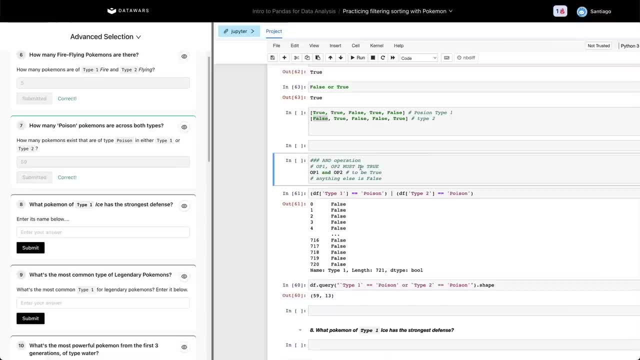 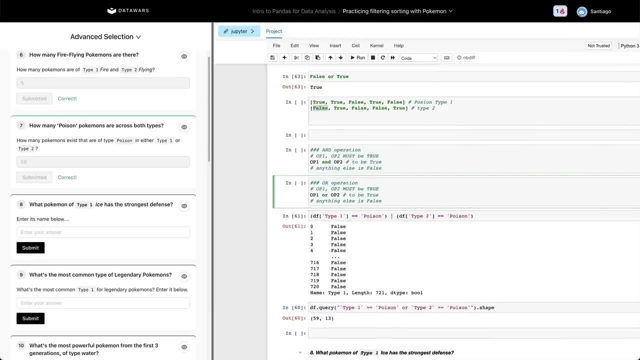 other case, everything is false. We can do a very similar reasoning with the or operation. So op1 or op2 must be false, both of them. for this thing to be false, Anything else is true, And this is you can. 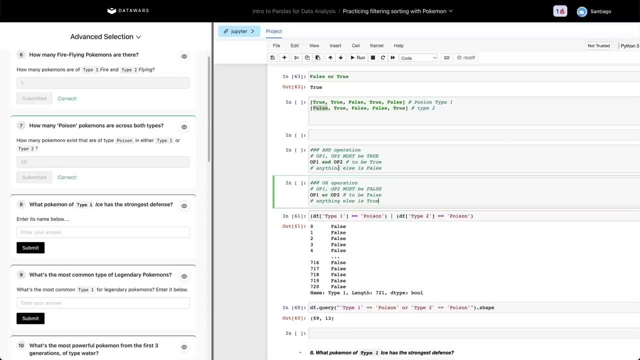 just flip things and that just works. That's the idea between Boolean algebra. You can just flip things true with false. In this case, true or false, Or false or true, True or true, All these things will be true. The only way to get a. 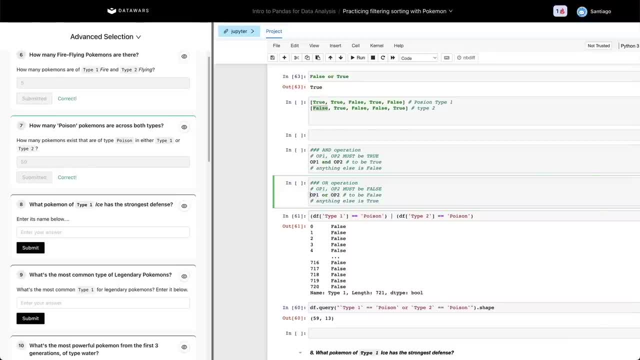 false. result back is: by both these things being false And going again to our logic here, we say: true or false is true and true and true is true. and let's do that. We align False and false is false, right? So these two are false. 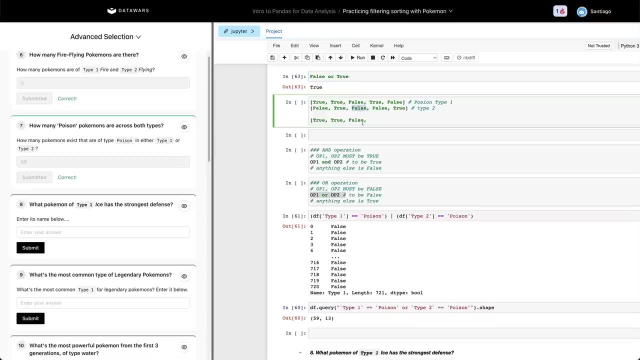 So this was fire. It was flying, so it's not poison. In this case, it was poison rock. I'm just making up types. It was, for example, flying poison, right? So that is also true. So true and true. 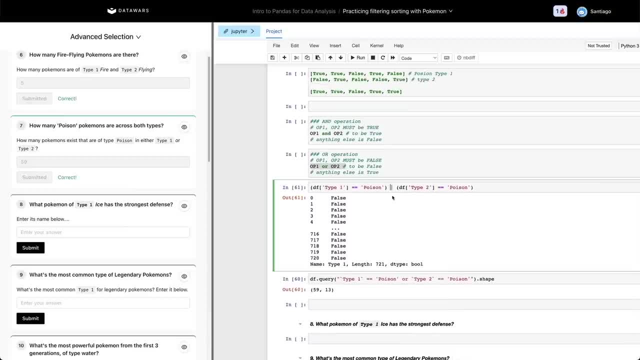 So what we're doing here with lock, we are generating the first Boolean array and combining it with the second Boolean array, with the or operation, And again, conceptually speaking, it works in this way. The result of this whole thing: if we wrap it in parentheses and do a sum, we're going. 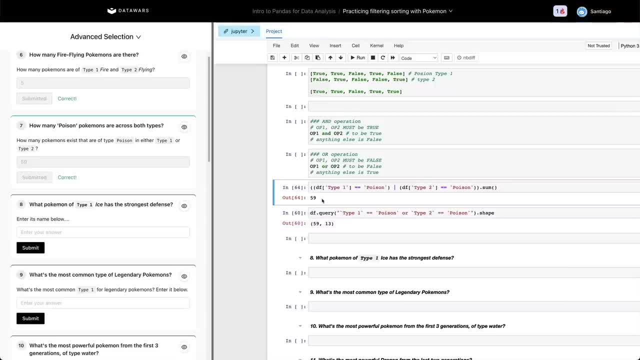 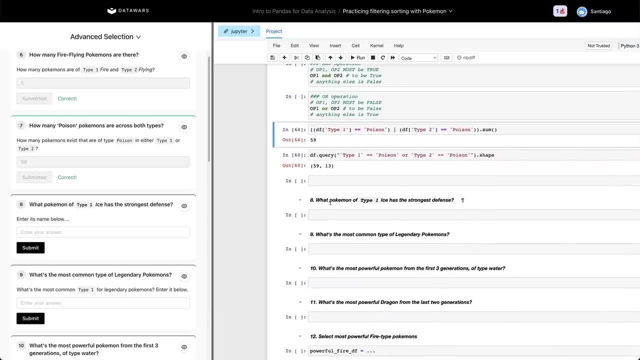 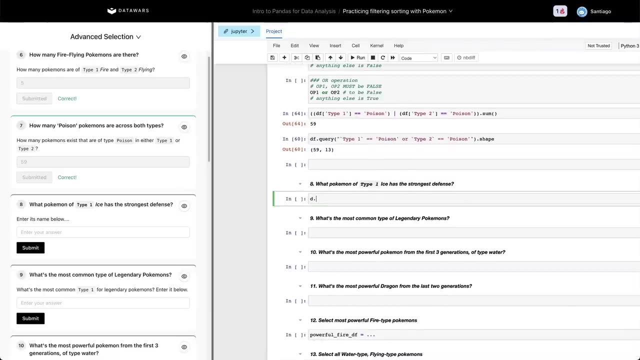 to get the same value out. Remember, these are just Boolean arrays. Okay, let's keep moving forward- What Pokemon of type one ice has the strongest defense? So we have to find- And you're going to- You're going to see that I usually start my activities doing dfhead. It's because 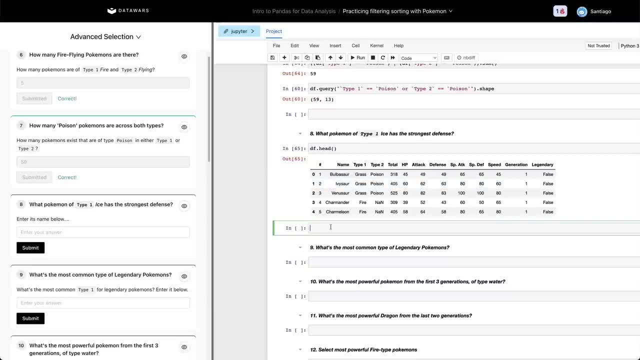 I need to take a look at the structure of my data. I'm going to do dflock type one, type one, sorry. df at type one equals ice. I'm going to start in this way. So these are all the Pokemon that have type one ice. 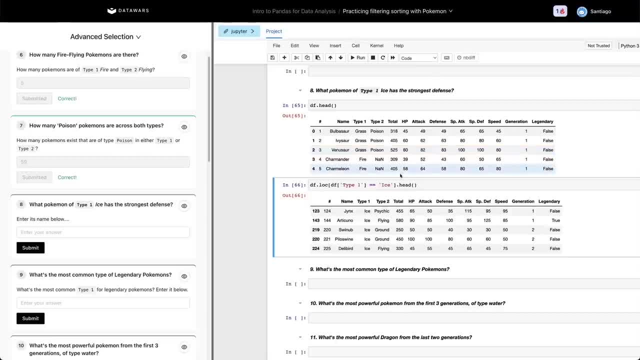 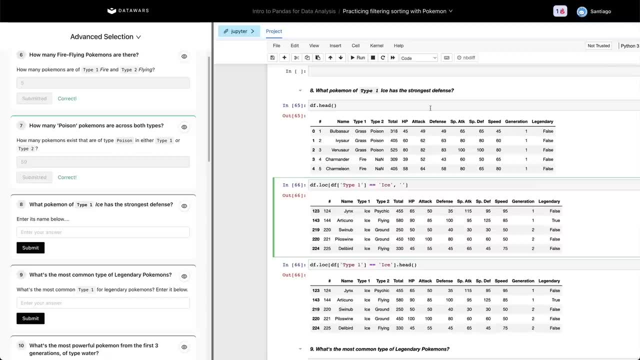 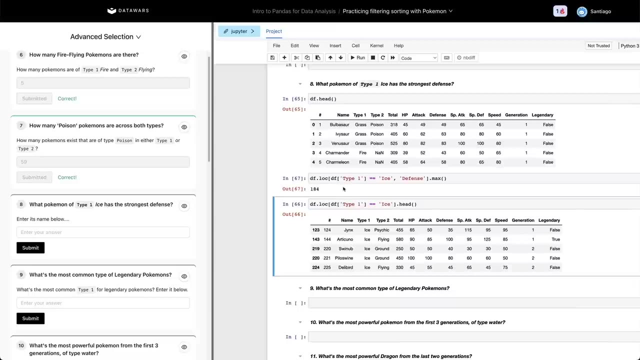 Now I can keep going By doing something like giveme1- here we can do- and the defensemax. The maximum defense of type one ice pokemons is 184.. I could extend this one by saying: givemePokemons that are type one ice. 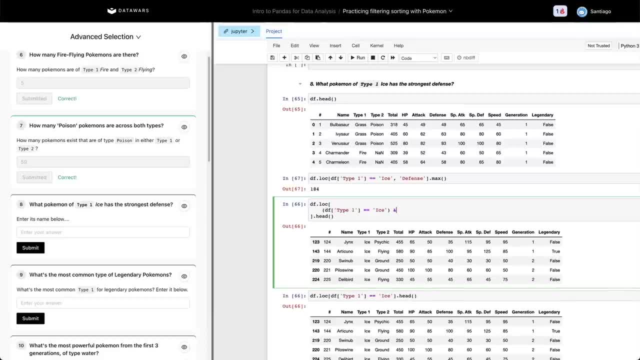 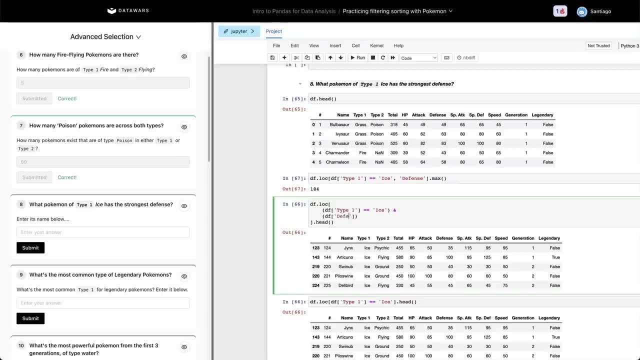 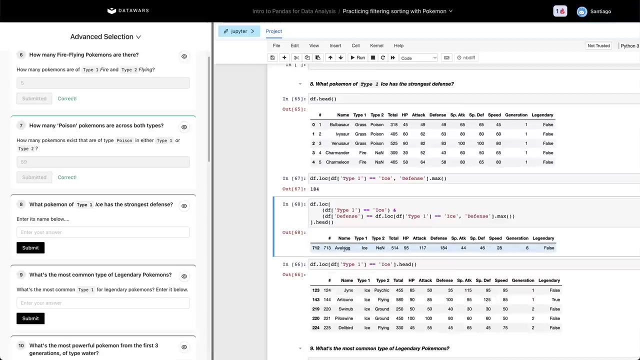 and here I'm going to use operation, because I want both things to be true and DF at defense is the maximum that I found before 184 and, if you let me, I'm gonna put everything together and I could do that and it's gonna give me just one Pokemon right. so far, so good. 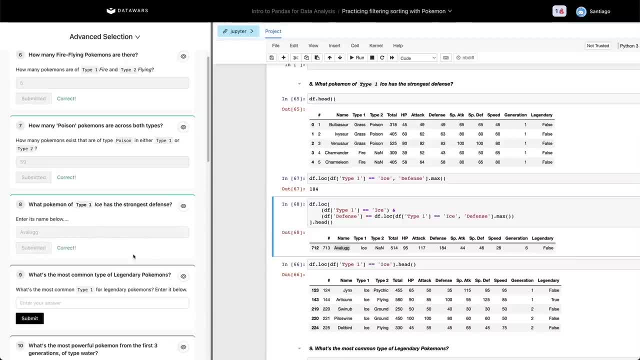 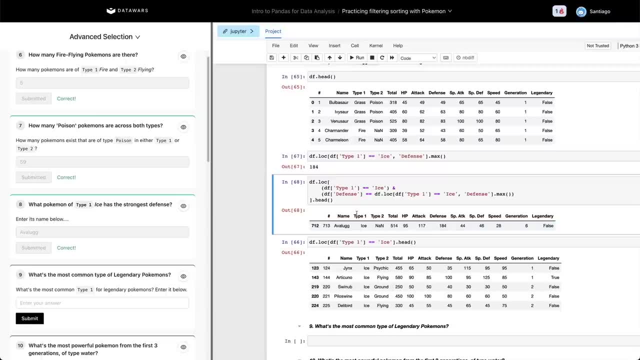 let's put it in here, see if it works. it worked, that was the correct answer. but now let me show you something a little bit easier. in this cases, we're looking for d1, like the most powerful, or the most powerful, like if we have, if we have. 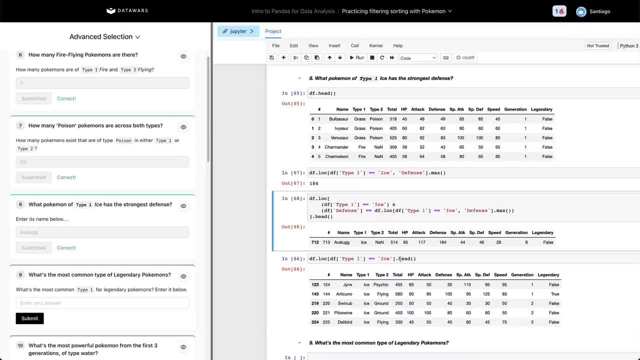 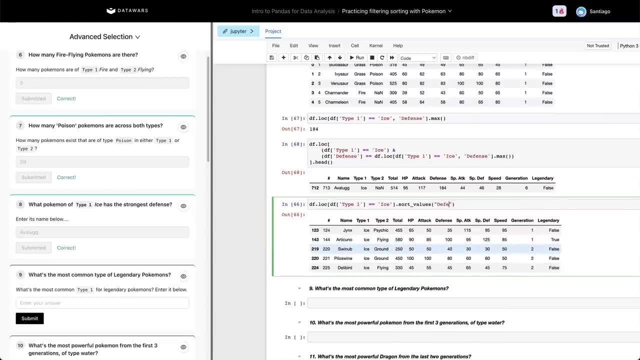 several, but we're looking for a maximum value. what we could have done is just sort values here. we're gonna sort by defense and we're gonna sort in descending order we want. let me show you the standard one. it's gonna show you the, the least powerful, like the. 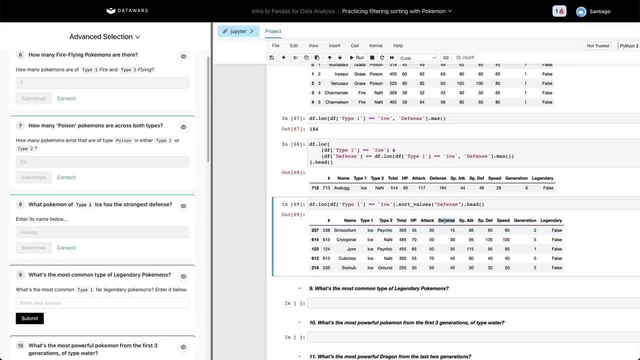 weakest pokemons first. that's because this is sorted by defense, but in ascending mode. but what i do is sorting descending mode to do that we're going to do. ascending equals false. and now we get the most powerful, the same result as before, which is of type ice. they have the 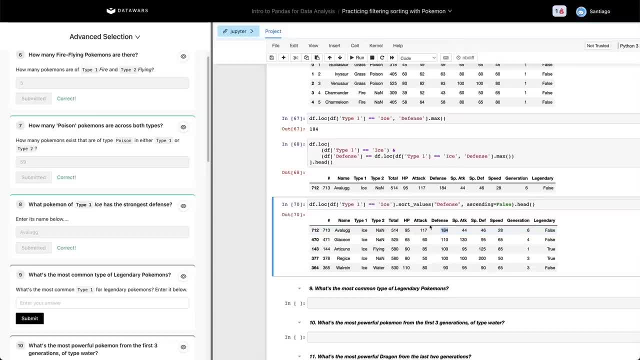 the most powerful one that we can see right here. so this is a more of a visualization. you know i'm doing some analysis with my own eyes so i can just, you know, get the first value here. it's not so programmatic. this is a little bit more programmatic. i could automate this thing. 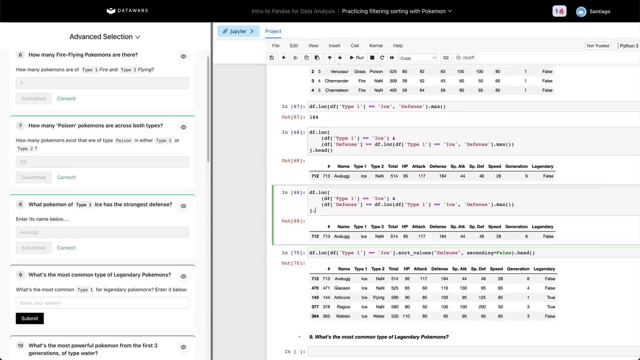 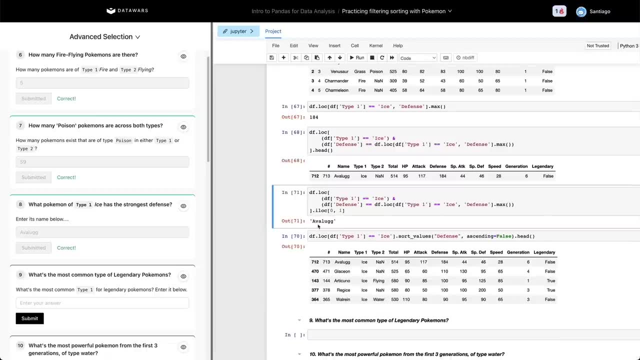 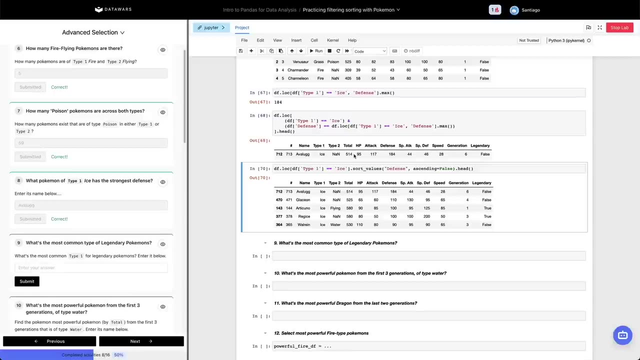 and i can do something like um, for example, I lock zero one and i have just the name of the first pokemon, the name. this is a little bit more programmatic, but again it's pretty much the same thing as before, as what we're doing serves the same purpose. 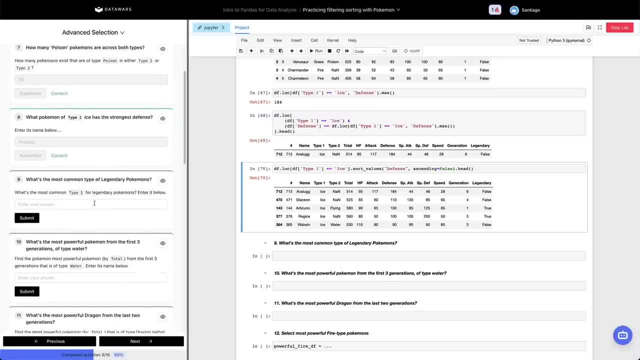 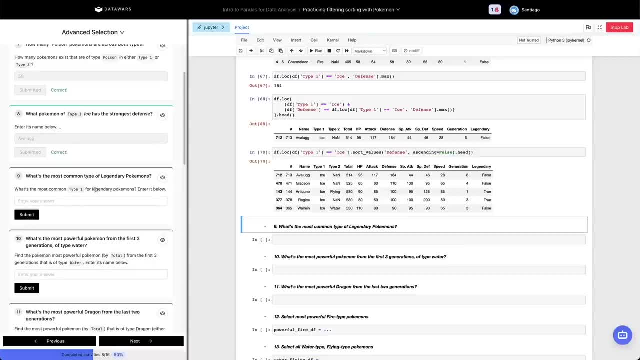 Okay, keep moving forward. What's the most common type of legendary Pokemons? What is the most common type of legendary Pokemons? What's the most common type one from legendary Pokemons? So what we can do is let's first lock all the Pokemons that are legendary. 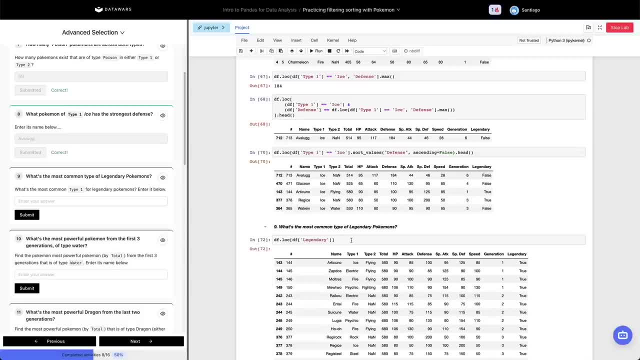 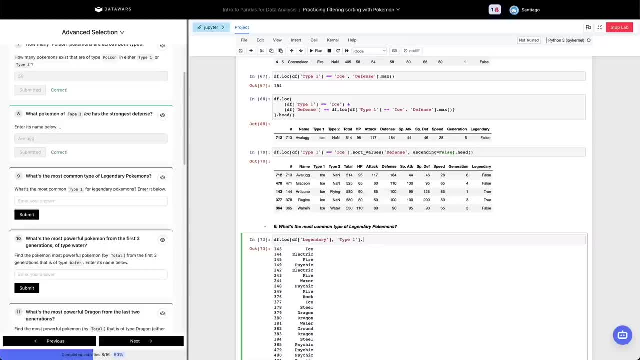 And we did this before. So this is gonna give us all the legendary Pokemons And now what we can do is do type one. This gives us the whole thing, And now we can do: just value counts And we can get that psychic. 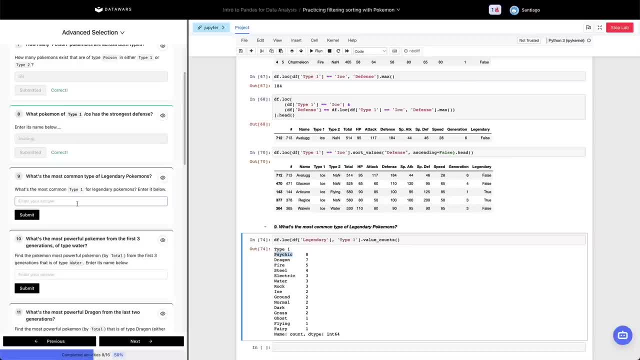 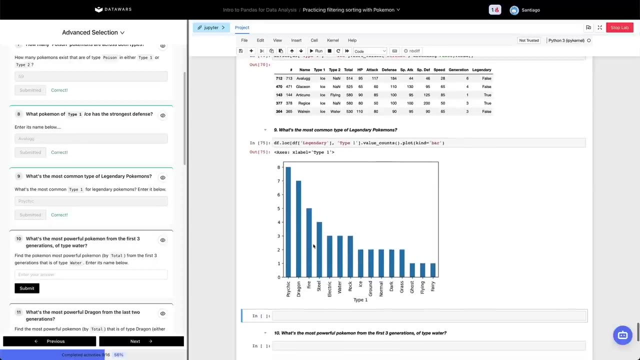 is the most common type of Pokemons And let's do that there. See if it works. There you go. You can combine this thing kind bar. There you go To do a little bit of a visualization, But in a way the result is correct. 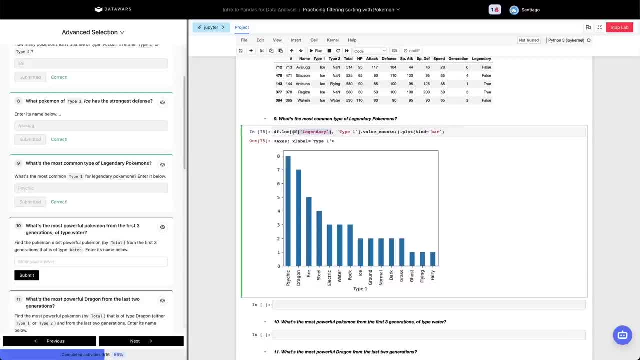 The important thing here in terms of filtering and all that, is that we filter by the legendary status, which is the Boolean array, And then we pass the type one column to get only that column, And then we got a summarization using a value counts. 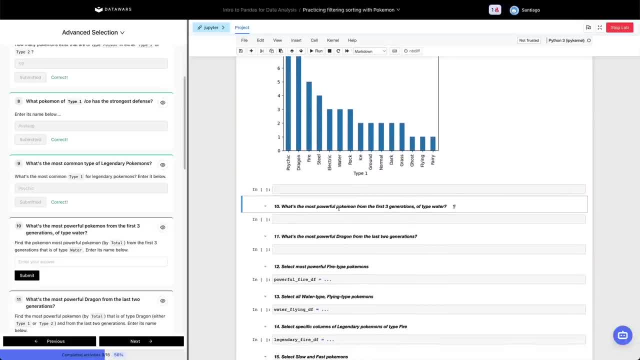 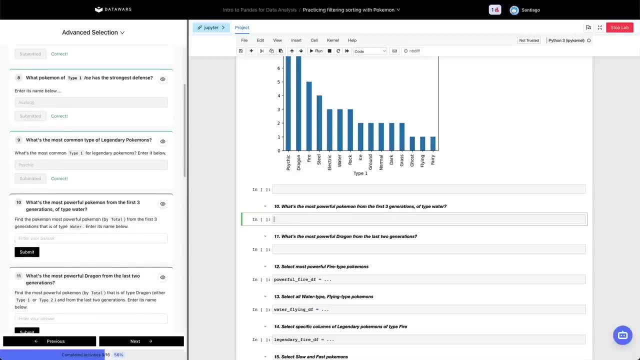 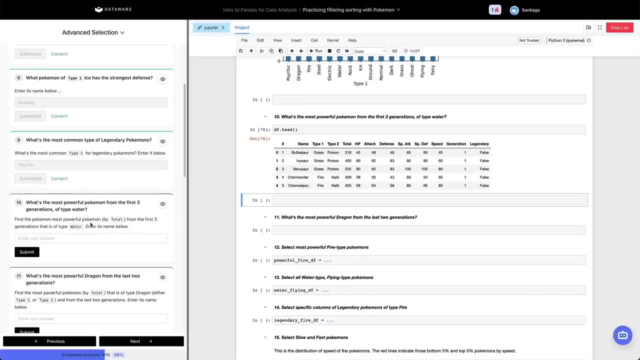 Okay, what's the most powerful Pokemon from the first three generations of type water? So we need to find the F, that head, As usual. So we take a look at the structure of our data, Find the Pokemons, the most powerful Pokemon by total. 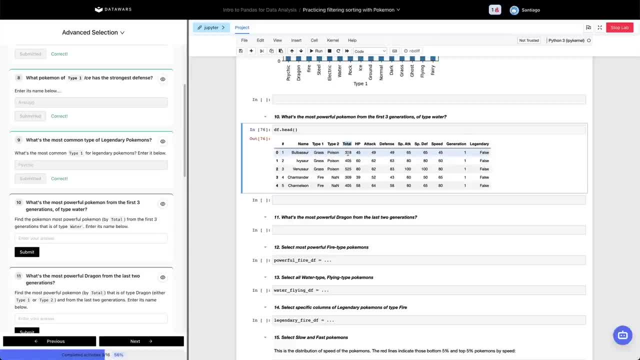 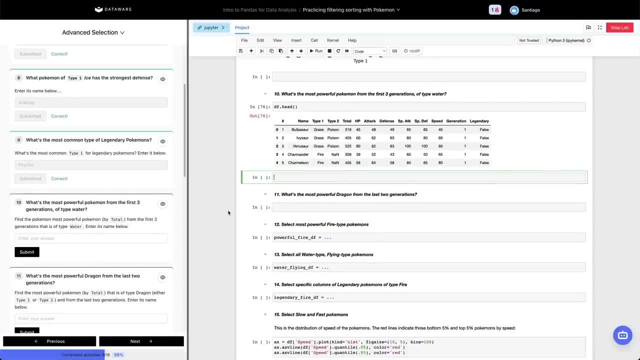 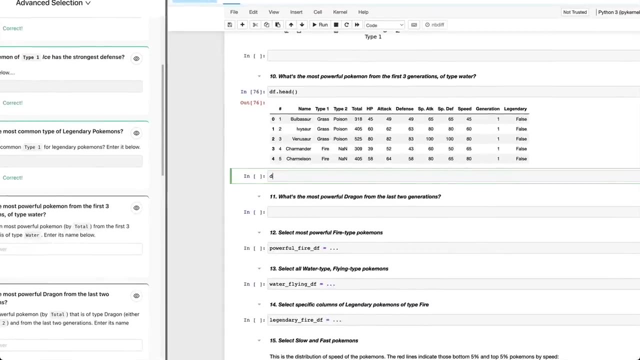 So we wanna find the total being the powerful representation here from the first three generations, that is of type water. So let's start step by step, with different conditions, To find, to filter. types of Pokemons are type water. That's simple. We're gonna do the F, the block, the F. 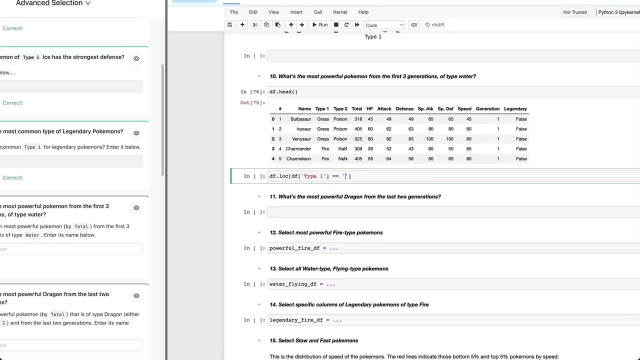 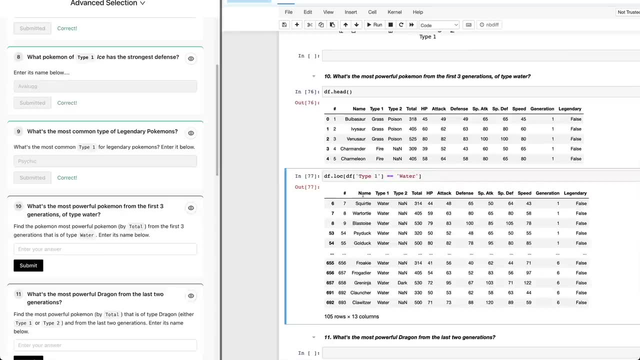 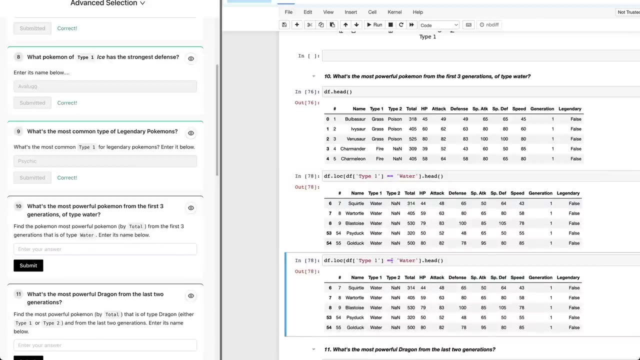 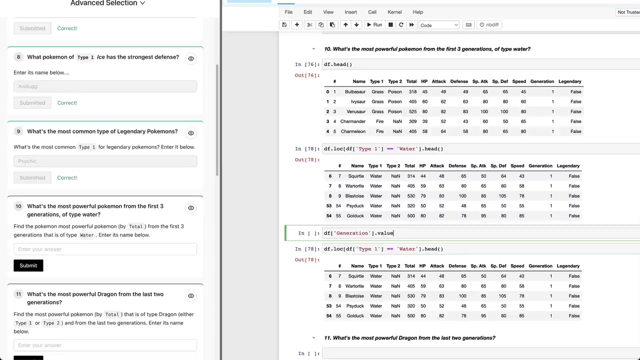 type water, And type one equals water. There we go, But now we have to combine it with the expression that is, from any of the first three generations. How many generations do we have Generation? we're gonna do now. value counts. We're gonna get the there are. we can actually 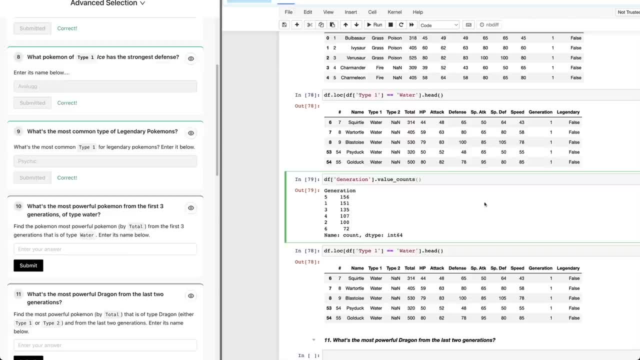 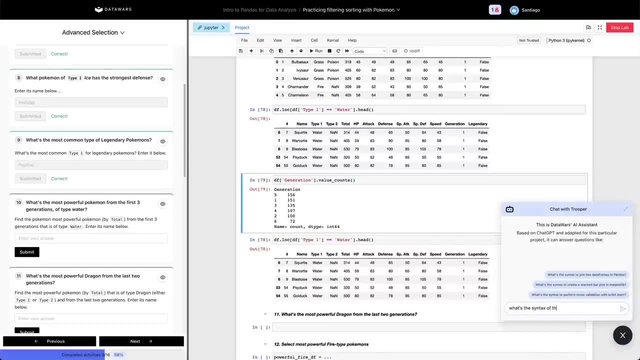 I think, let me see, let me see the. let me ask here what's the syntax of the value counts, value counts method, Because what I wanna do is not sort these values. We can visualize it in a quick VAR chart, to put it in a way. 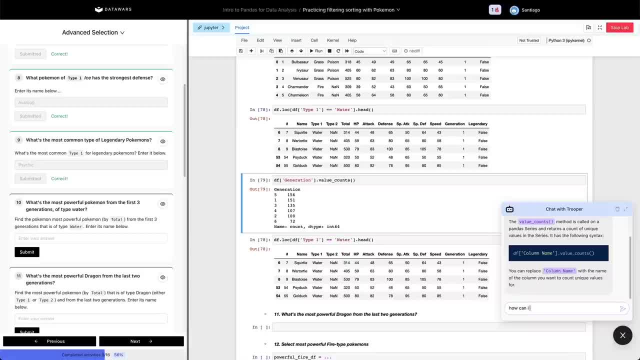 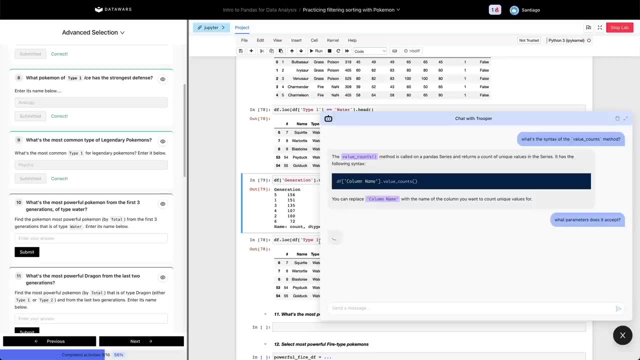 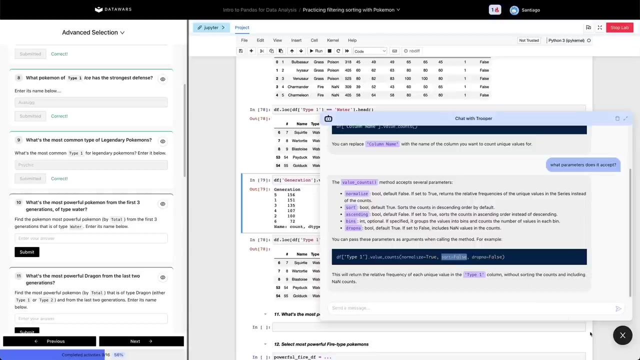 Value counts is the same, So I can. how can I? what parameters does it accept? I'm closer to find the documentation of pandas than asking the AI here. There you go. Sort. false is the method the one that I was looking for. 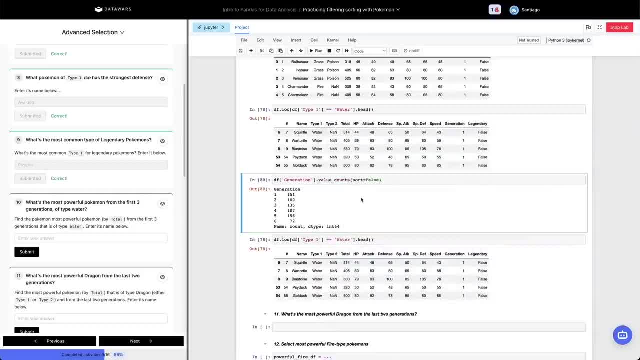 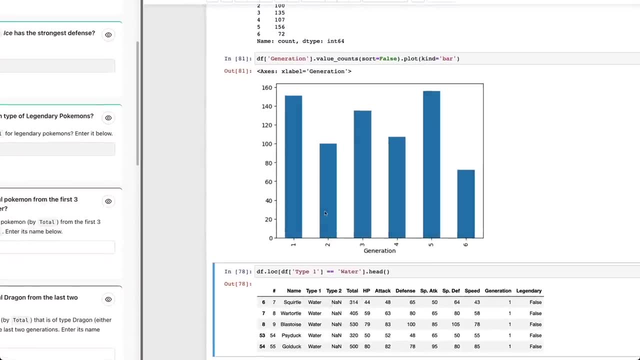 So let's do sort false. There you go. And now I'm gonna do plot kind bar. There you go. So these are the generations we have: One, two, three, four, five, six. This is a little bit. 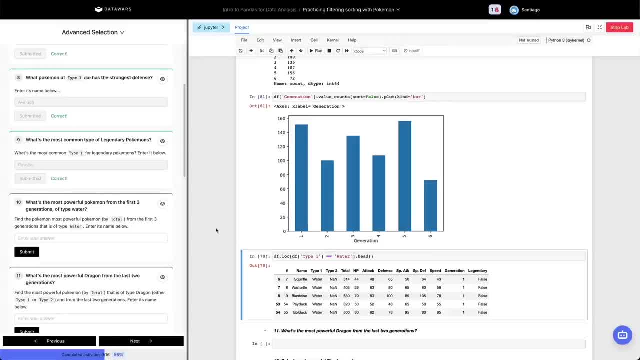 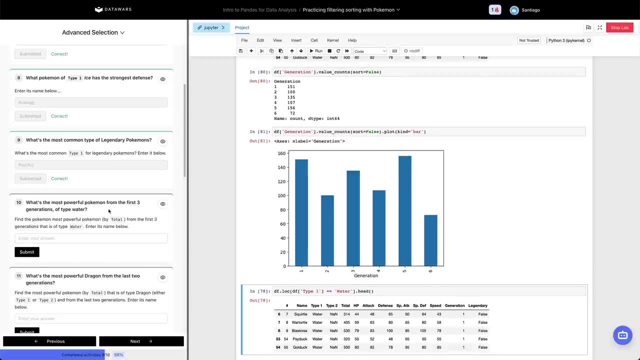 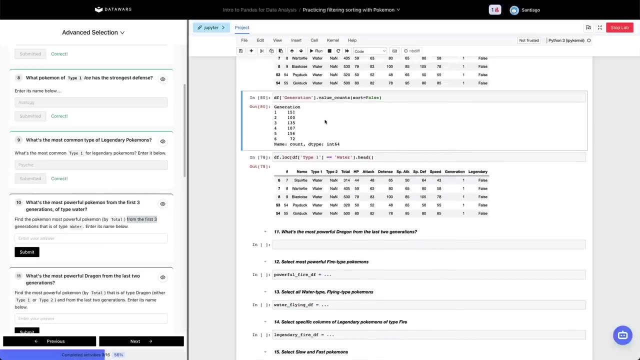 this is not useful for the exercise in reality. I just wanted for you to take a look at the generations. Basically, what it's asking us to do is the first three generations is gonna be generation one, two and three. Continue with our exercise. 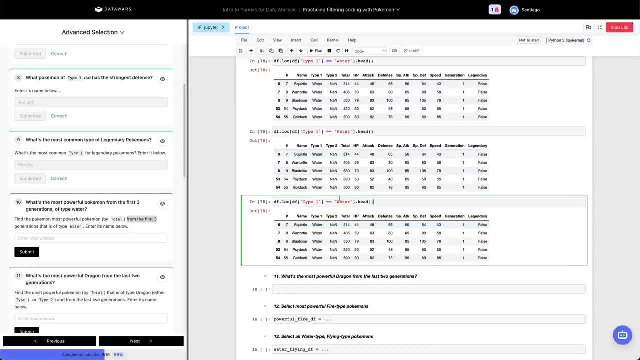 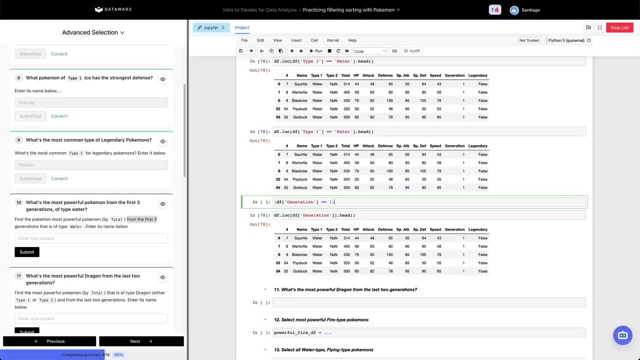 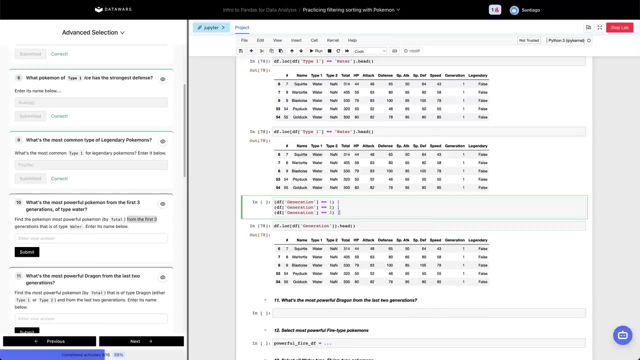 How can we get the documents of the first three generations? The way to do that is gonna be DF. We could do something like generation. Let me actually type it outside. We can do something like: generation equals one or or two or three. 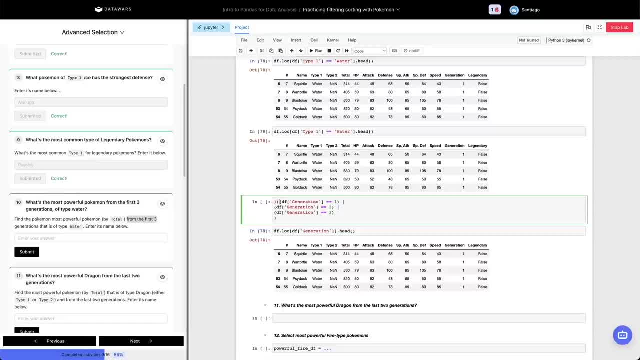 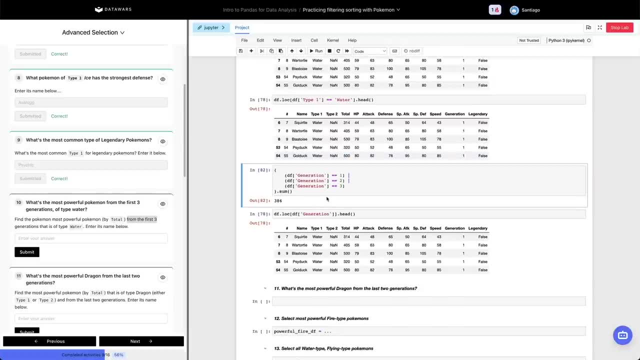 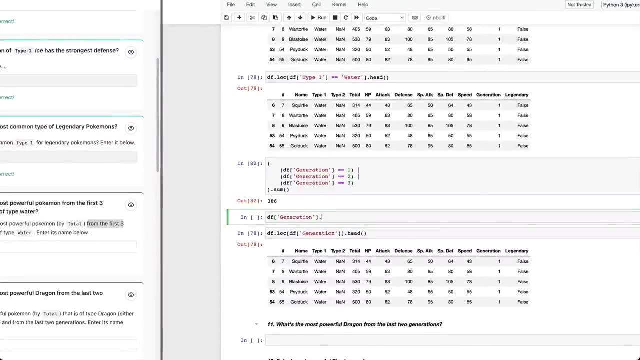 And we wrap this whole thing in parentheses. dot sum, There we go, But the reality is that it's a much easier method, which is DF at generation dot is in. So we're gonna pass here a collection: one, two or three. 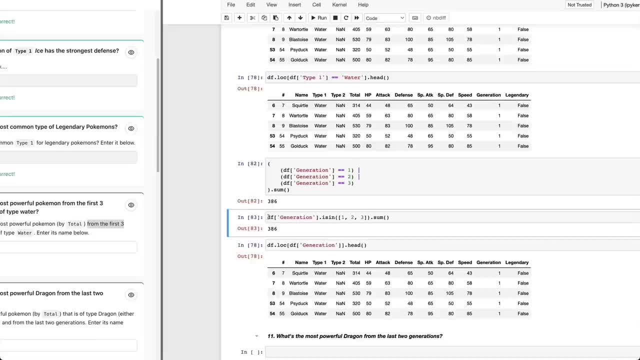 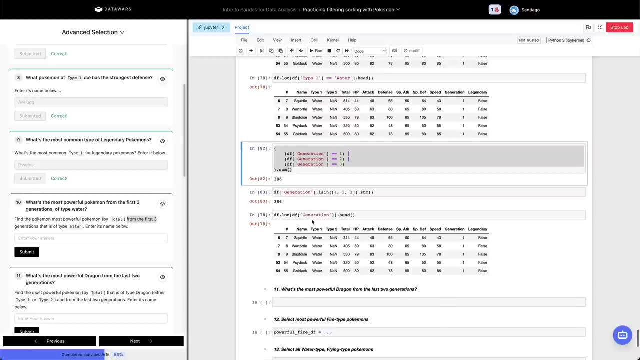 We're gonna get the same results. So it's basically the same expression as before. This value right here can take any of these forms, and that is good for us. That is the same as doing this full, OR So putting everything together. 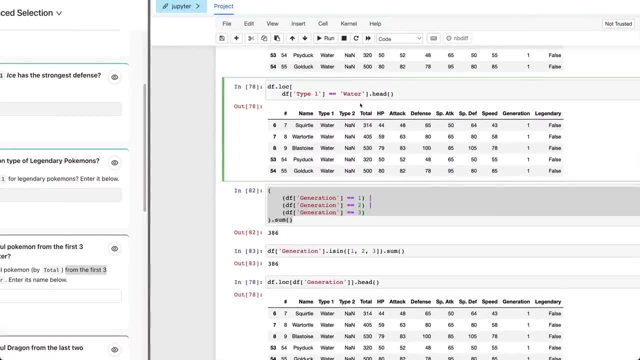 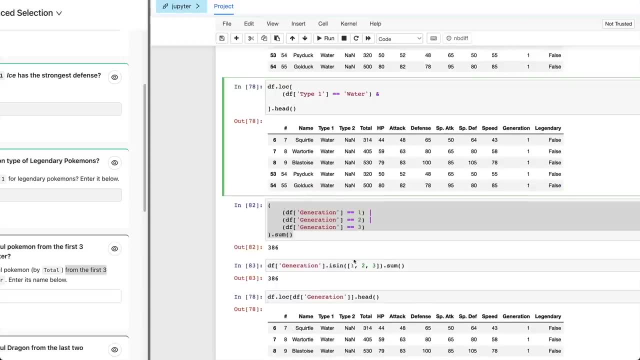 what we're gonna do is- let me zoom here and we're gonna break this into several lines- We're gonna do: type one is water and the generation is one, two, three. There you go, And I already forgot what the question was. 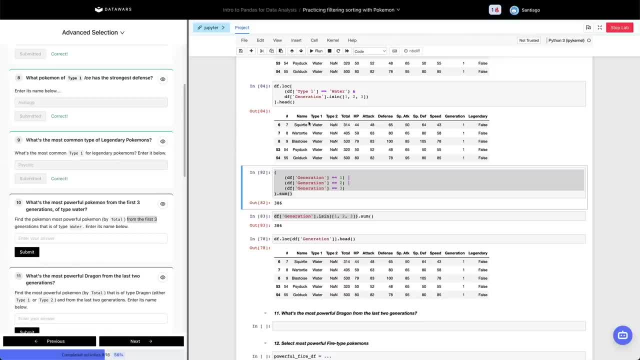 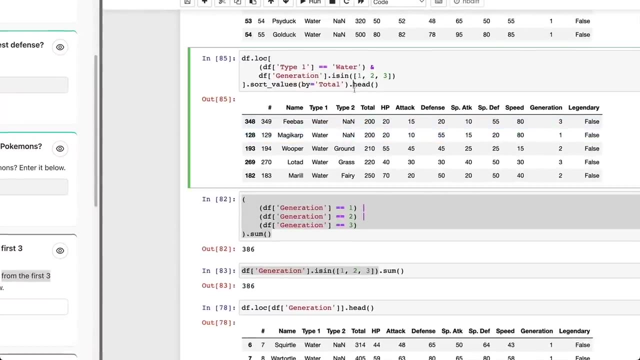 I forgot what the question was answering. What's the most powerful Pokemon by total? Here we're gonna sort values by total And, as usual, let me show you what it returns. Returns in a ascending mode. We actually wanna do it in descending mode. 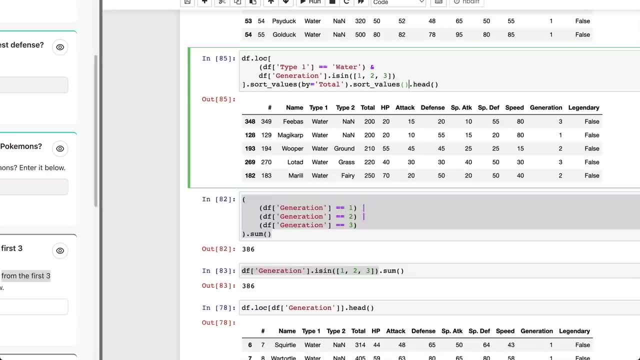 So we're gonna do sort values by: oh no, no, no, sorry, We already did sort values- We're gonna do ascending false and we're gonna get Kyogre- Kyogre- my English is bad. 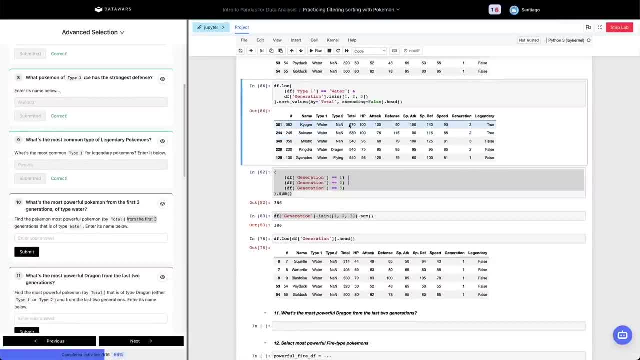 and on top of Pokemon's worse, is the most powerful Pokemon by far in terms of total. So we're gonna pass a value and see if it works. I'm gonna do a quick summary. The first one is this idea of just as usual. 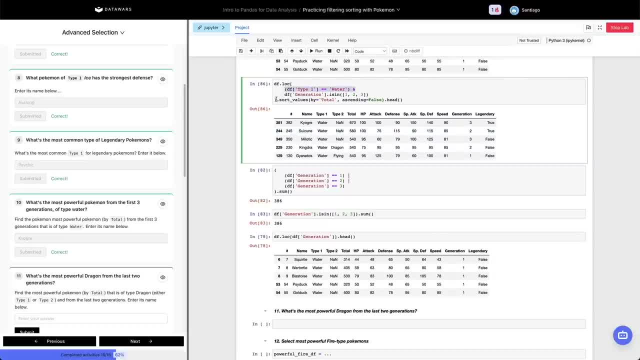 combining things with the Boolean array or sorting values to get answer. The interesting part is we're using this is in operator Right That lets you pass several values And it's basically a simple way to write an or statement. So let's say we're gonna get all the Pokemons. 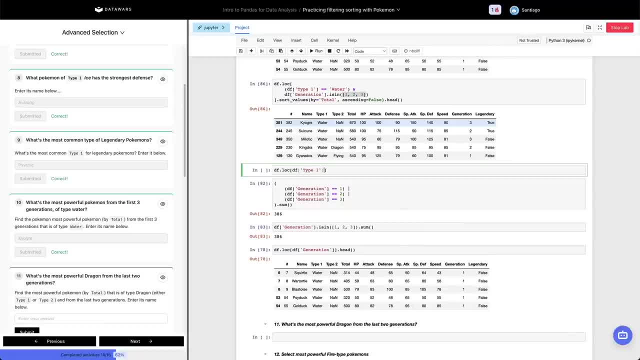 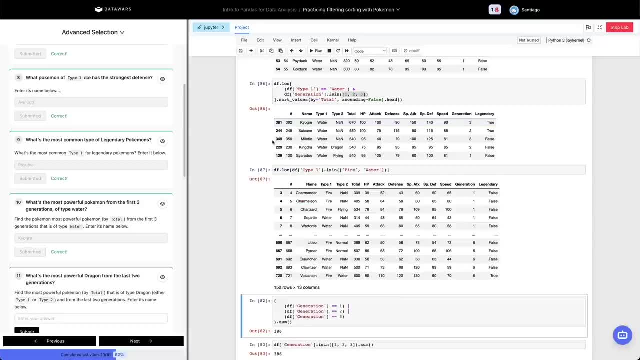 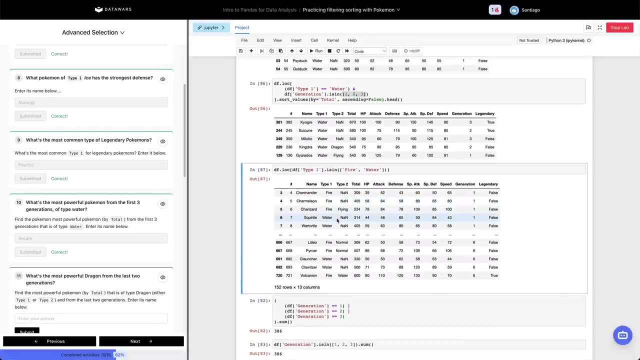 that are of type one, either fire or water, We can say is in and we can do here fire or water. So any Pokemons that are fire or water, It's basically this volume has to be in this subsets. Okay, moving forward. 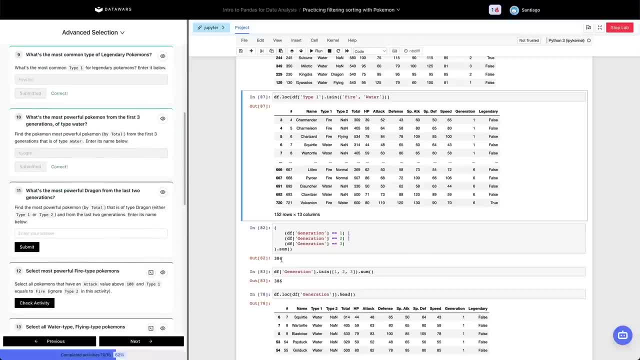 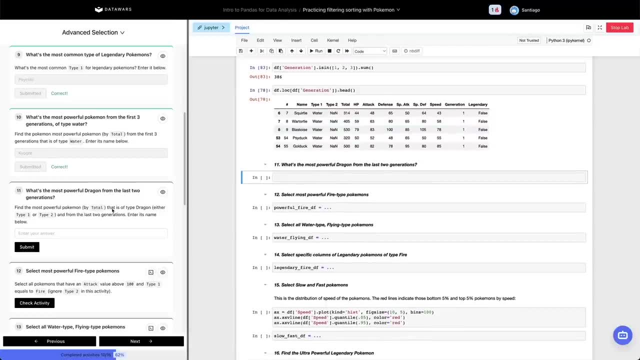 What's the most powerful dragon from the last two generations? This is getting interesting, So find the most powerful by total, that is, of type dragon, either type one or type two. So either type from the last two generations and enter its name below. 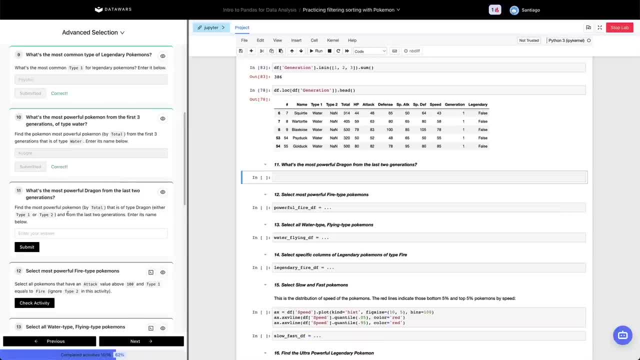 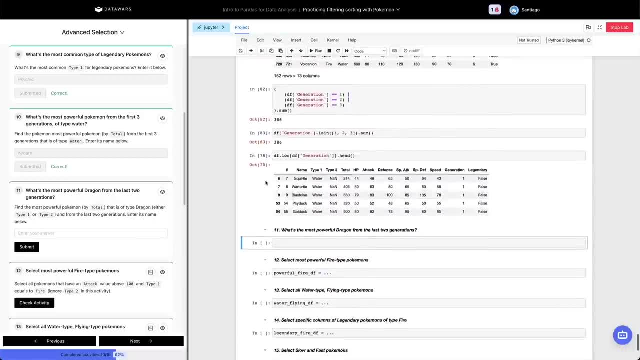 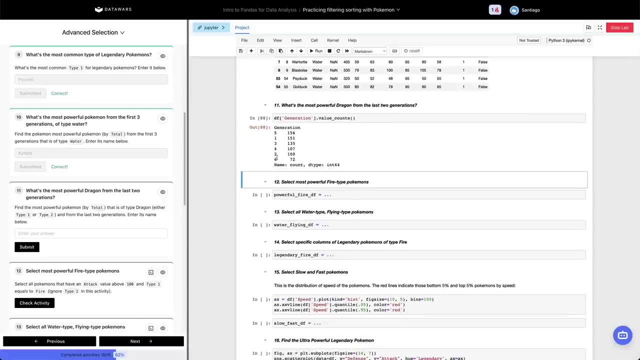 So it has to be a dragon, either in type one or type two and from the last two generation, last two generations We saw before The last the generations are- I already deleted it. Basically, generation value counts. There we go. 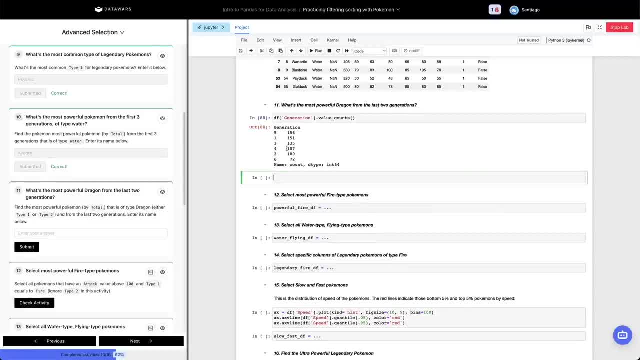 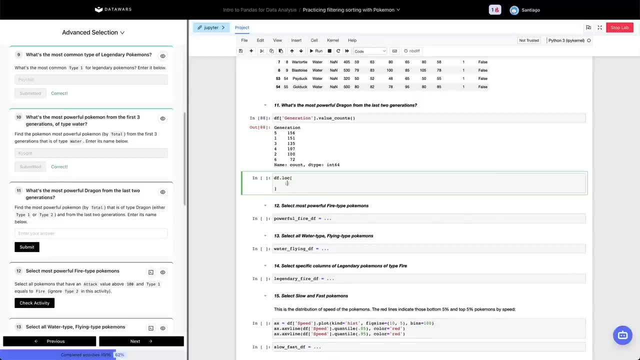 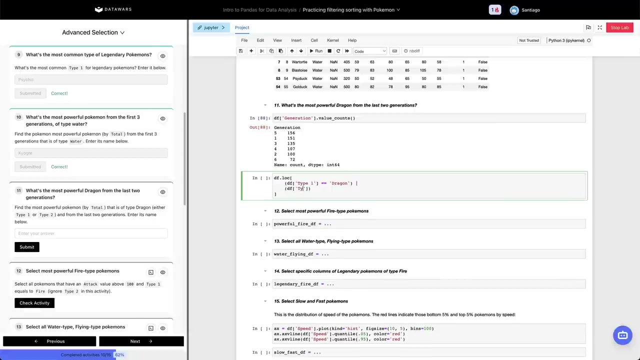 Is five and six are the last two generations. We're gonna write the whole thing now. We're gonna do, we're gonna break it in lines. I wanna say DF at type one is dragon, Or DF at type two is dragon And DF at DF at generation dot SN. 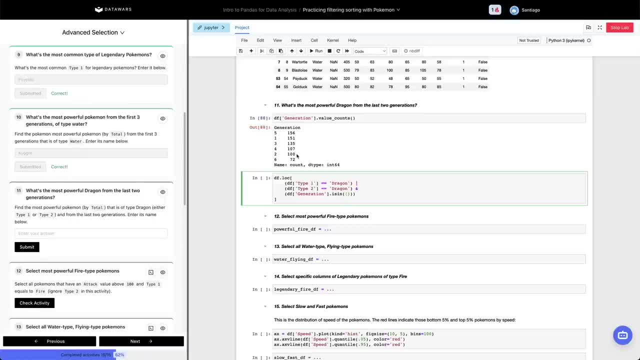 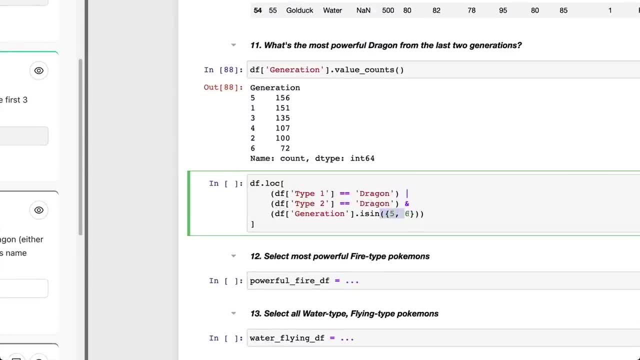 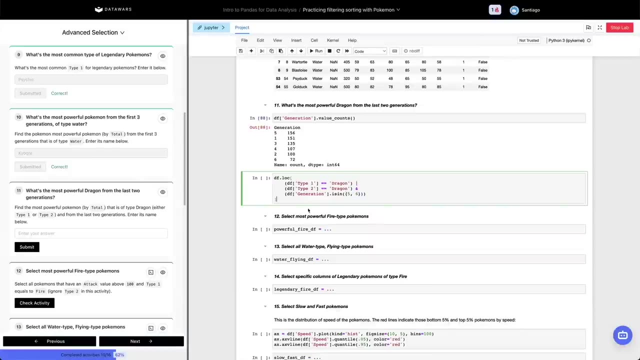 And here we have the last two generations, So it's five or six. And here, quick note, we are. I'm using here a set. You can pass a tuple, a list, whatever. I just pass an inline set because the most correct way of doing it. 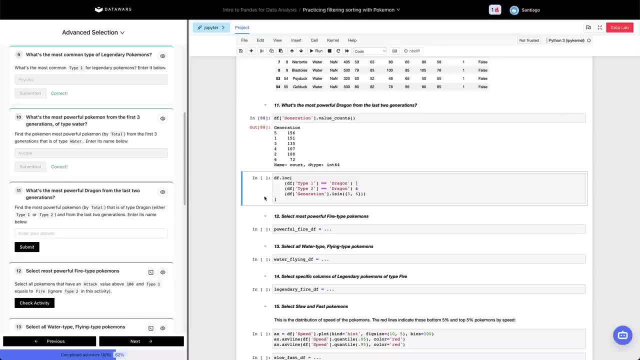 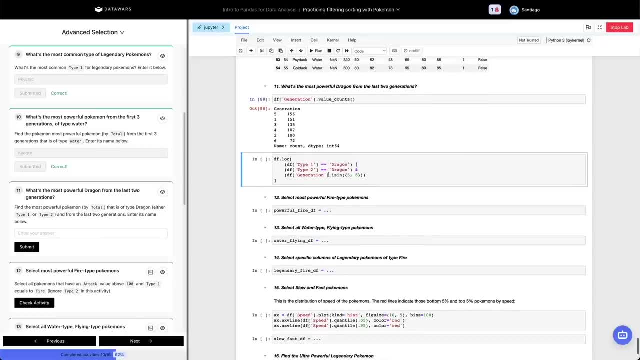 in terms of performance, I don't think it affects enough, but it's just the correct way of doing it. But anyway, in terms of solving the activity, let's go ahead, And the way we're gonna do is: I'm gonna just run this thing. 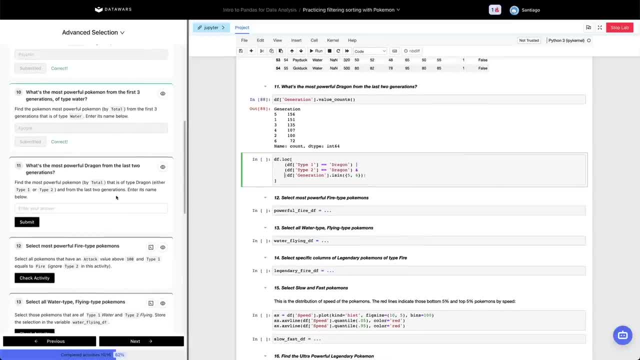 We have to find the most powerful dragon. We have to find the most powerful Pokemon in this set of being type one dragon, type two dragon and this generation five or six. But you're gonna find something interesting, So I'm gonna show you these results first. 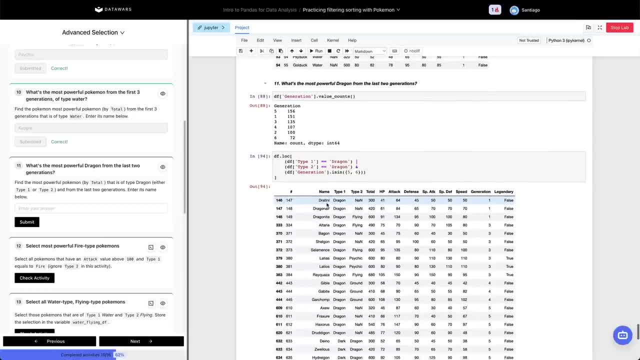 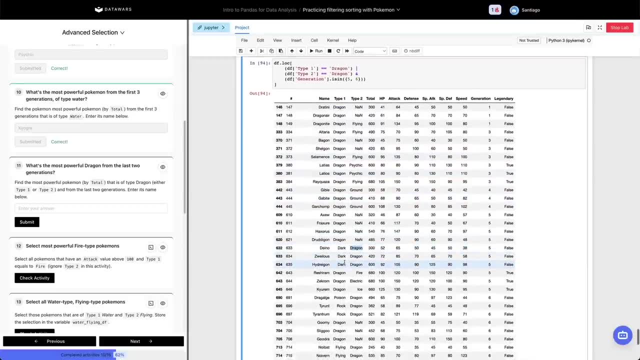 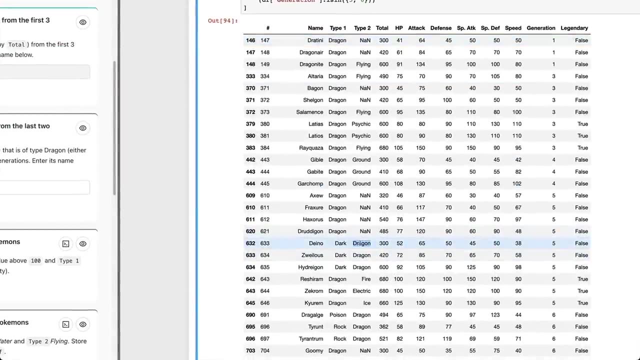 You're gonna see what we get. Type it's type one dragon, type two dragon. That is good. So let me show you the data: Type one dragon, type two dragon. So the first condition seems to be matching. but what you're gonna immediately see? 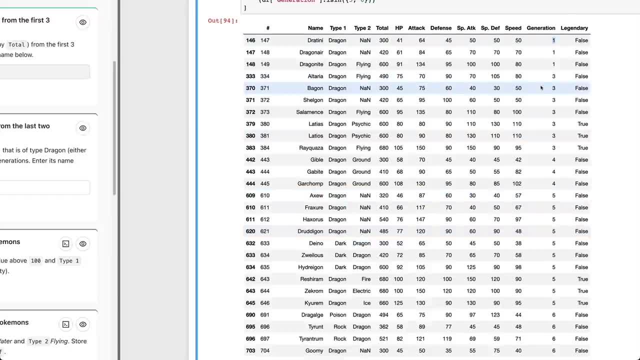 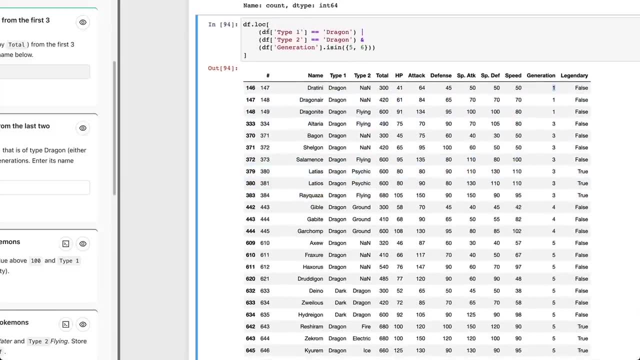 is that the generation is incorrect. We get Pokemon from generation one, three, four, And that is because we're combining the conditions that it's either or this thing, or and this thing, So the operators in the way they work, is that it did the operator of this thing that works. 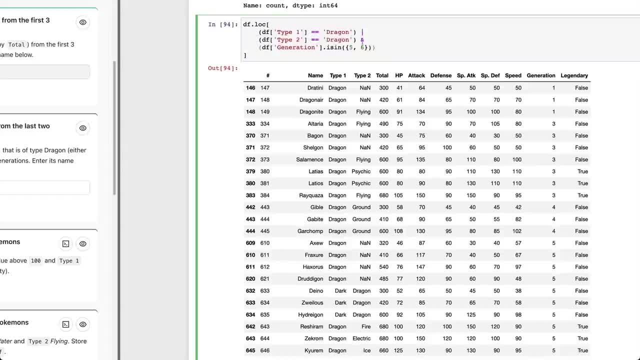 And then it did the operation of these two things. But that is not what we're looking for. The way we want it to work is to perform these two first. It's either one of these and this one in here. So to do so, what we need is to surround. 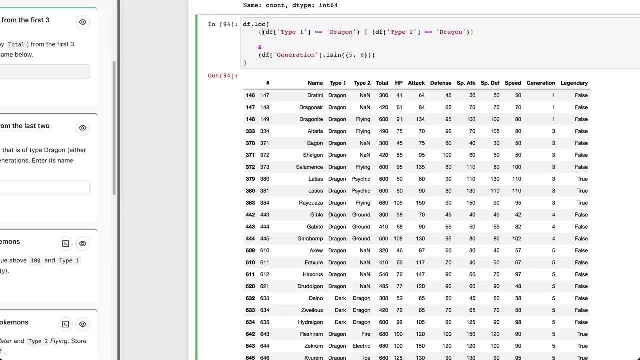 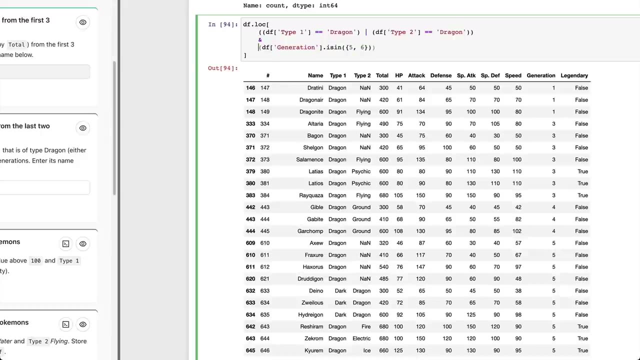 these two operations with parentheses, So it's like the order of the operations here is important. It's first perform this thing. It's either type one dragon or type two dragon, And we want it to be generation six or four. I don't know if this syntax worked. 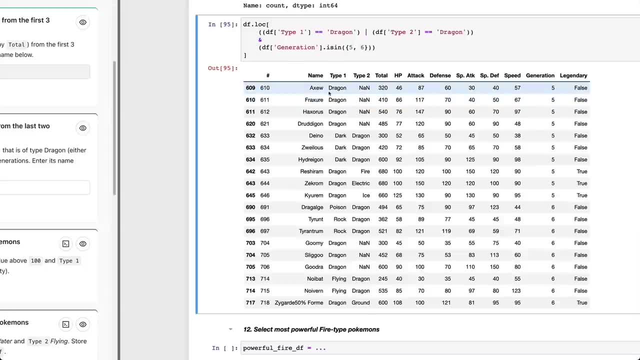 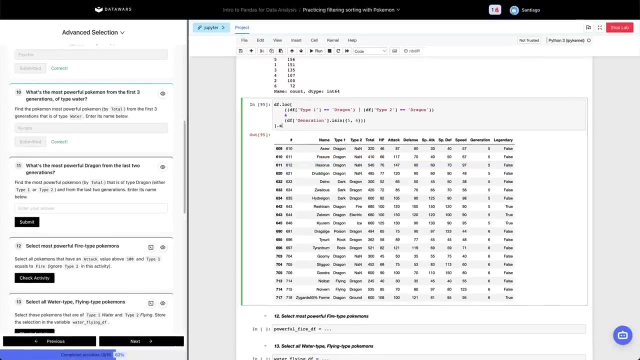 There we go, it worked, And now we can see that it's dragon in type one, dragon in type two, And the generation is only five and six. So this is the expression that we wanna get. Now the only thing we need to do is sort values. 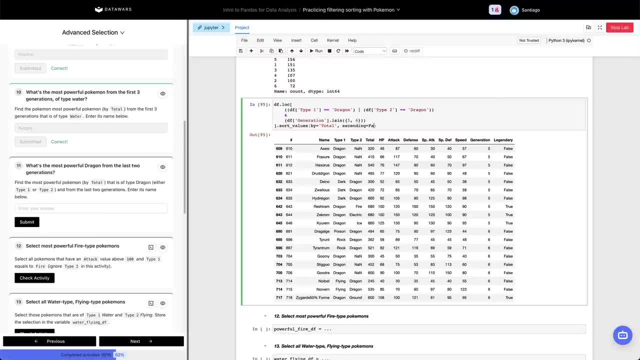 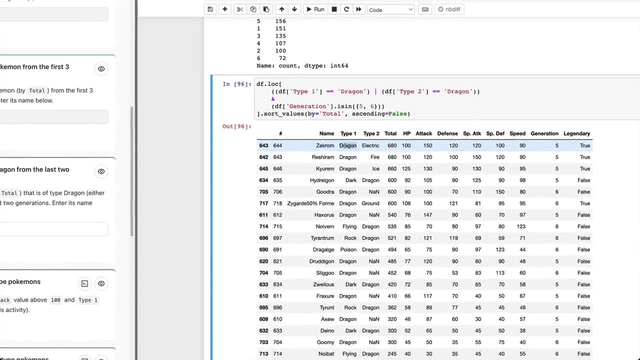 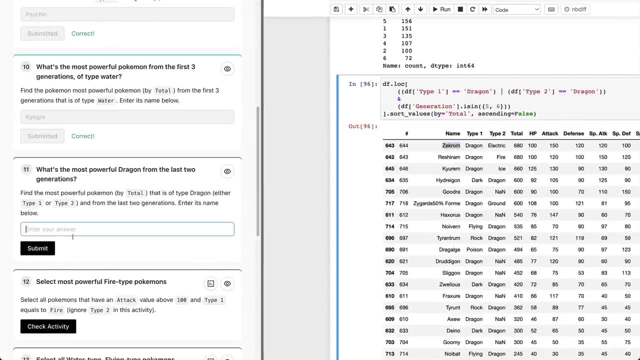 by total ascending false. And we get that. these Pokemon is the most powerful, one type one, dragon, type two, electric, that doesn't matter, And it's generation five. So let's try the answer right there And it works. 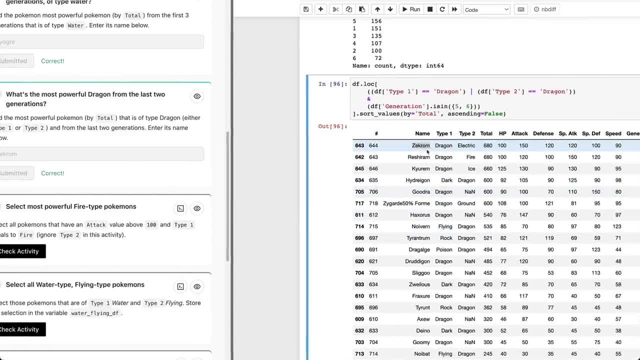 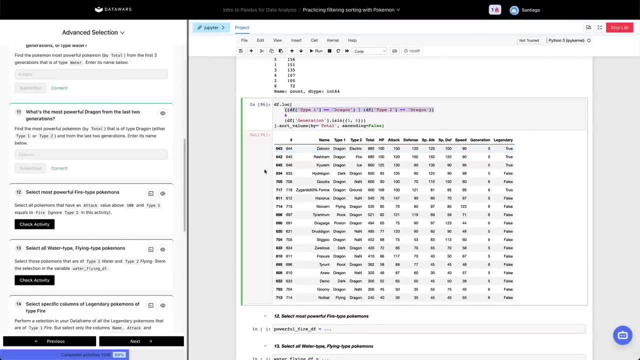 Okay, moving forward, and this is important. I don't think we have another activity in this project that has like the precedence, the important of the precedence or the order of operators, but it's an important concept. So just you know, remember parentheses don't hurt. 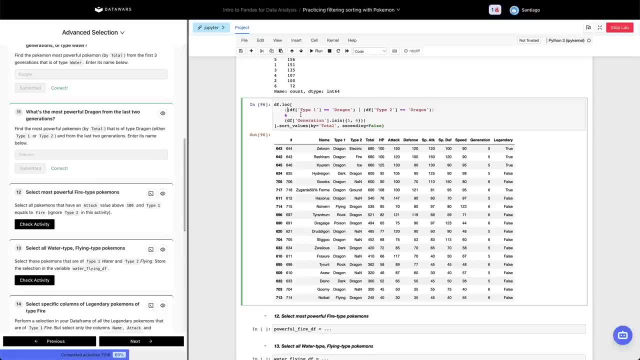 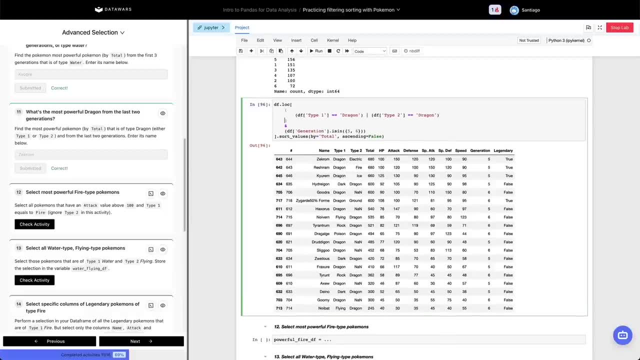 It's cheap to put parentheses. So if you have these complex expressions, just make sure you're surrounding the ones that you wanna run first with parentheses. You can indent, you can do all sorts of things, as long as you know it makes it look better for you. 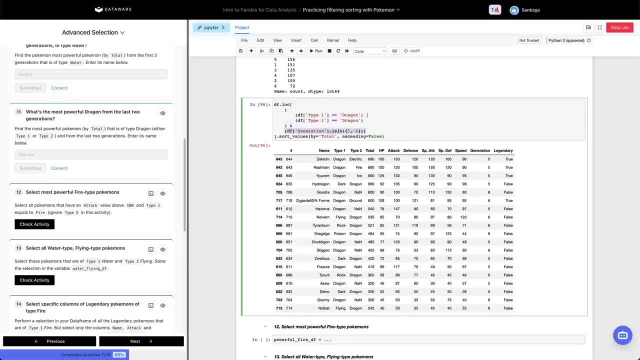 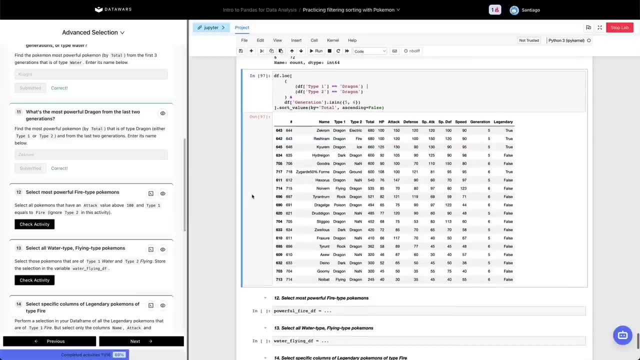 Could have used something like that. So is this thing And this thing You know? actually, parentheses are not necessary here. Anyway, just keep in mind. the precedence of the operations is important. All right, select the most powerful fire type Pokemons. 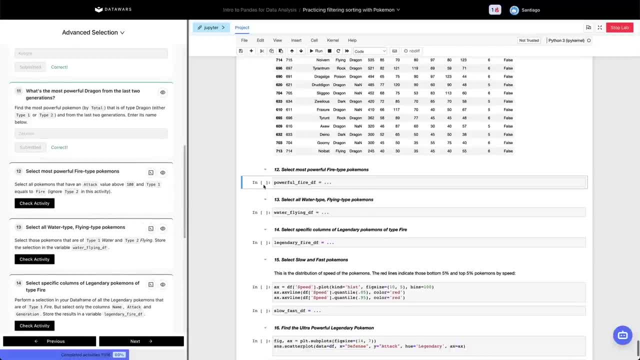 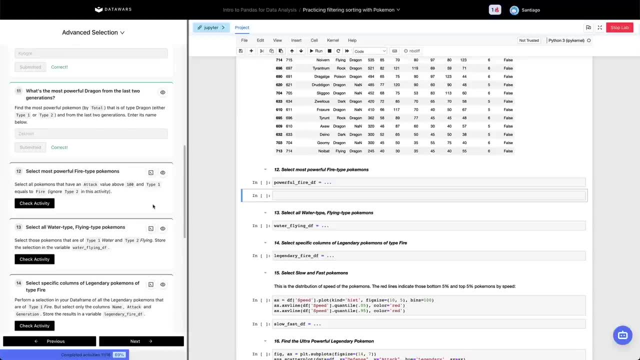 So here we're gonna say: select all the Pokemons that have an attack value above 100, above, and type one equals to fire, And we're gonna do dflog. We can actually do a query now. We're gonna do. 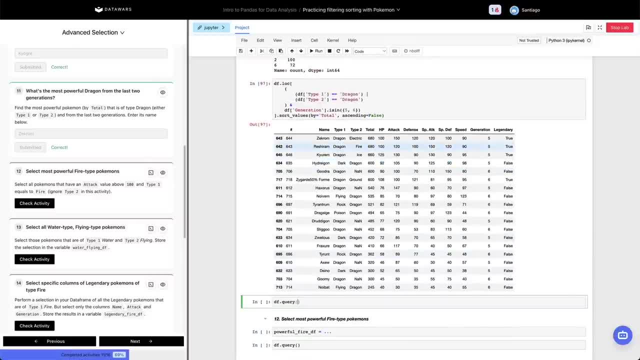 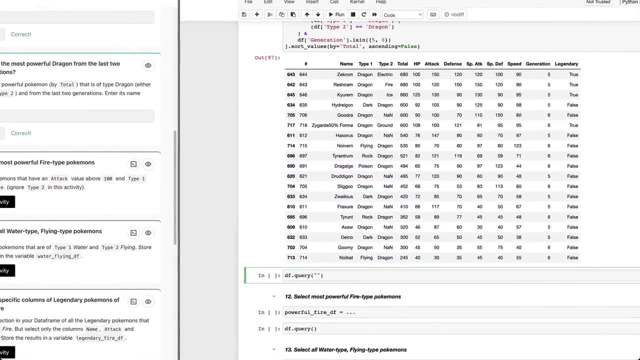 oh, by the way, we can solve this one with a query method first. So sorry, let's go back to the previous one. If you're pausing and resuming, you're hating me in this moment. Basically, we're gonna say we need parentheses here. 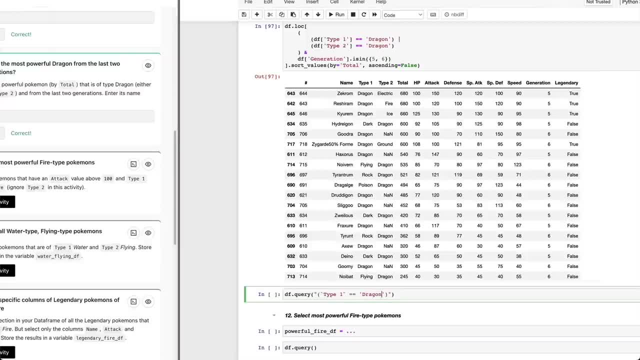 So type one equals dragon or type two equals dragon, And oh, we can't do the in here, We can't, We can't do the in. So we can do generation in five or six And we get. oh, we have to sort the values. 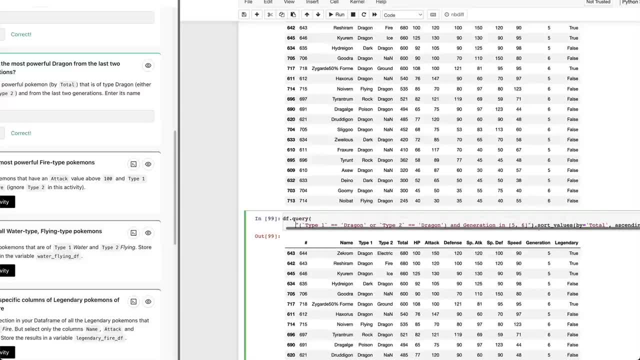 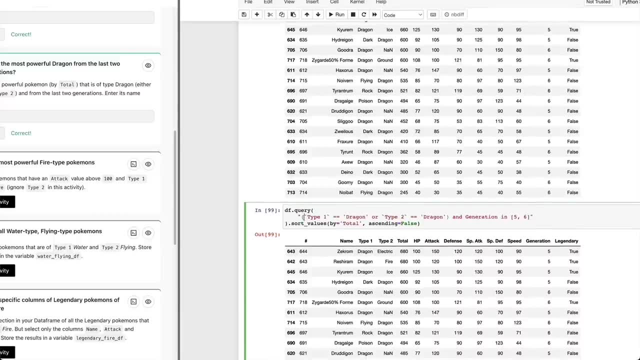 And we have the same result. Let me break this into multiple lines. It's difficult to read, But anyway, what you can see here is we are producing pretty much the same expression, and the order of operations is important: Type one dragon or type two dragon? 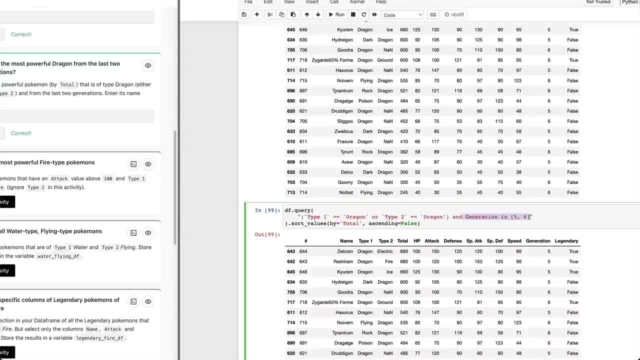 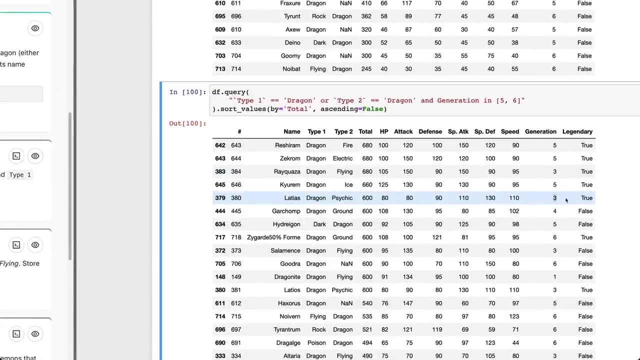 That's the first thing, And generation is in five or six. Let's see if it doesn't break when we got the wrong results Here. when we remove the parentheses, you can see that our Pokemons of generation three one. So this is clearly not working. 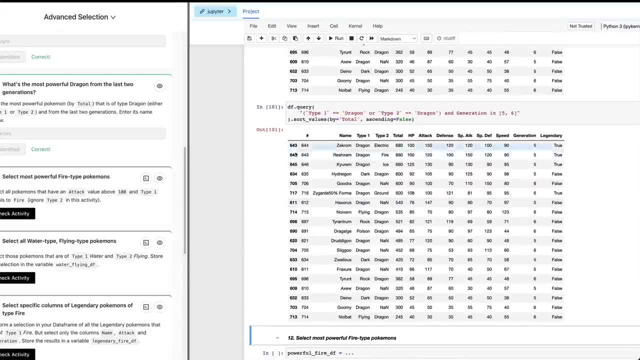 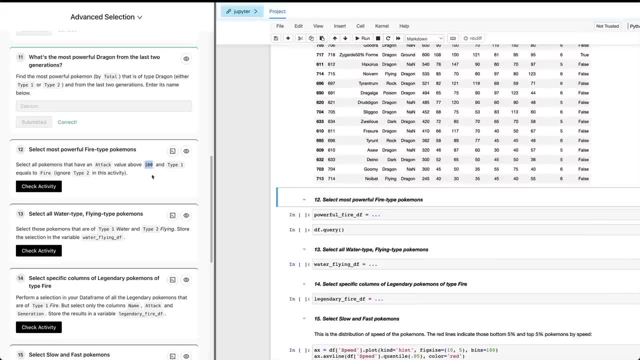 Have to go back and put the parentheses for the order, So sorry. Now let's move forward to the other one, Which was select all the Pokemons with attack greater than 100 and type one equals fire. We're gonna use a query. 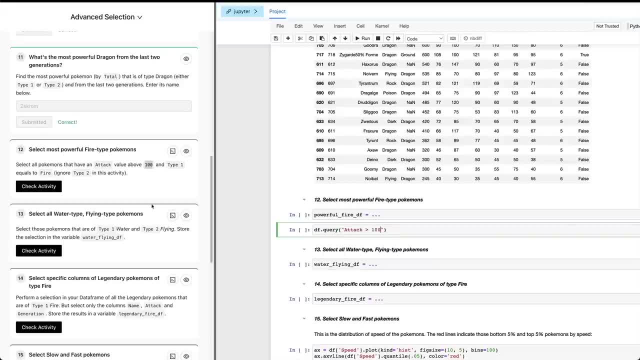 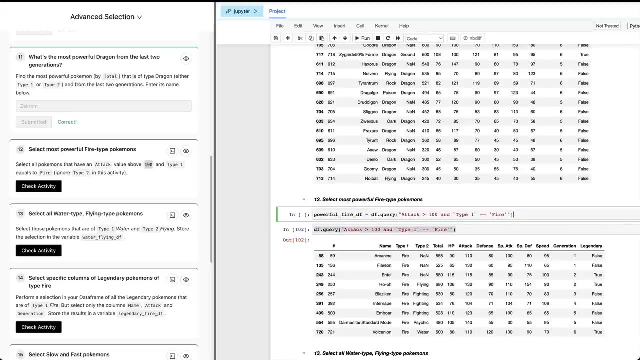 We're gonna do: attack is greater than 100, because it says above and type one equals fire. There we go. We're gonna run that thing and we're gonna assign it to our variable. Visualize it. Let's see if it works. 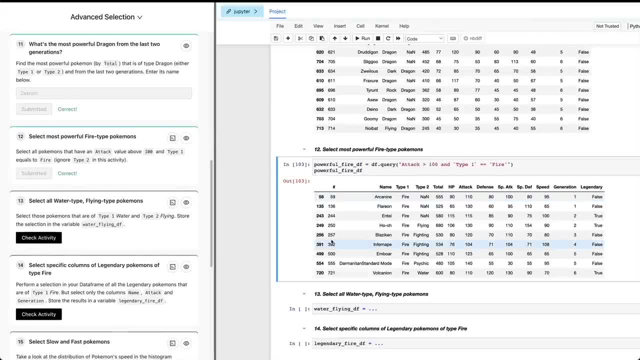 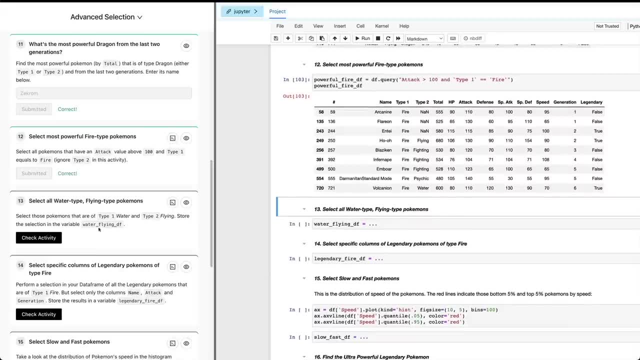 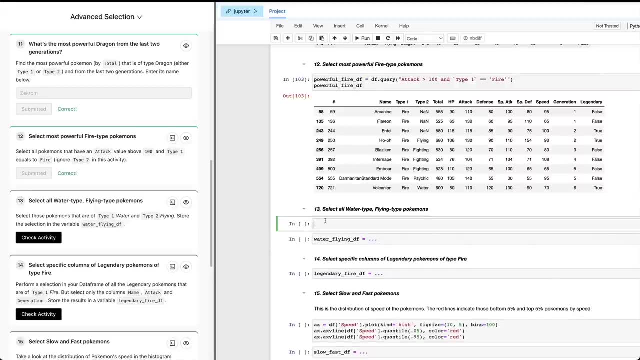 It worked, we're correct. Next one: select all water type flying type Pokemons. So select all those Pokemons that have type one for water and type two flying. We're gonna do pretty much the same thing as here. We're gonna do vfquery. 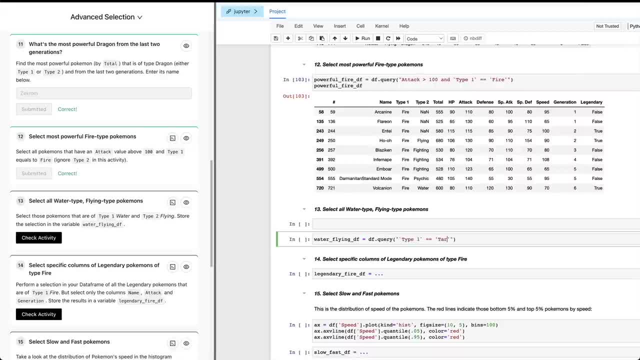 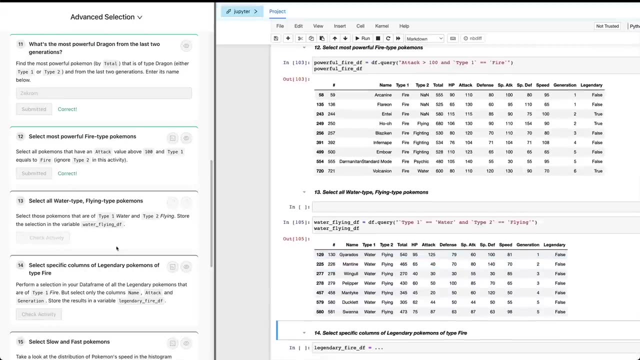 We're gonna do type one, water and type two flying, And let's see the data we get back- Water flying for both types And let's check the activity. There we go And finally- well, not finally- there are two, three more. 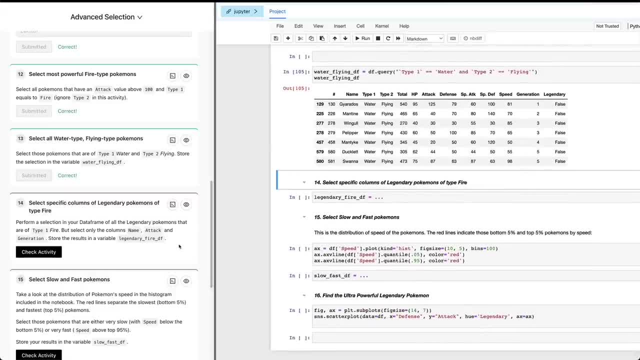 but select specific columns of legendary Pokemons of type fire. Okay, so this is interesting. Pause, now wanna solve it by yourself? It says: perform a selection in your data frame of all legendary Pokemons that are of generation, one type, one type, that are: 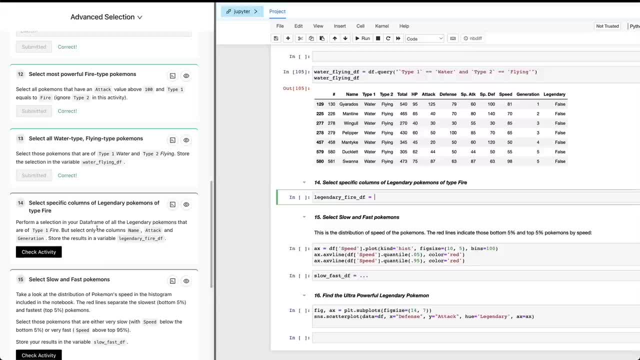 Of type one fire. sorry, but select only the columns name, attack and generation. So we're gonna do vflog, we're gonna use and there's gonna be a good reason that are: vf at type one equals fire and vf at legendary. 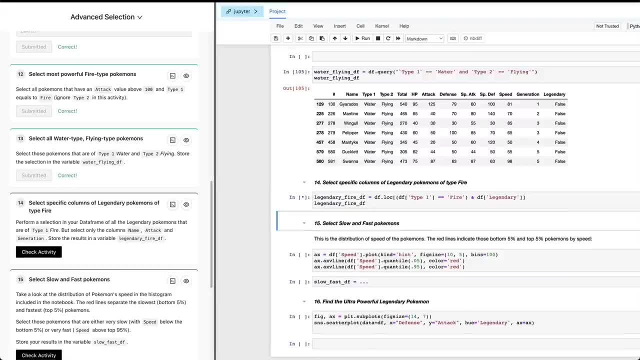 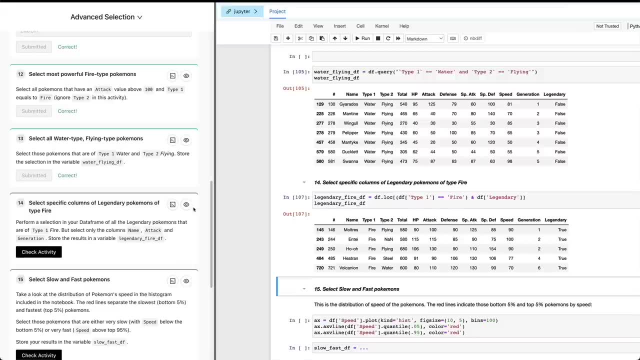 That's the first result. So type one, fire and legendary. I switched the order here but we don't wanna get all the columns, We wanna do just a selection. We say we only want the columns, And here we're gonna say name, attack and generation. 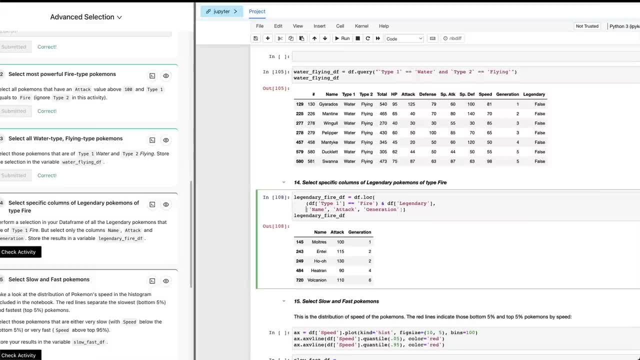 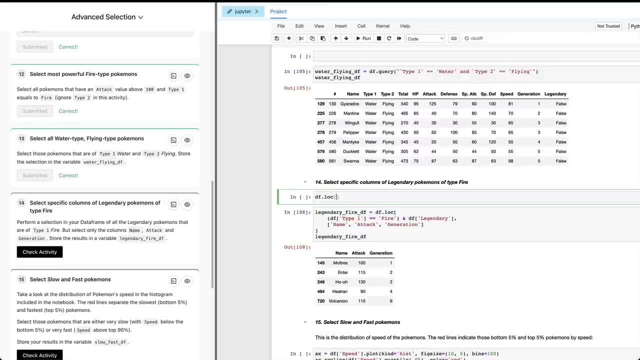 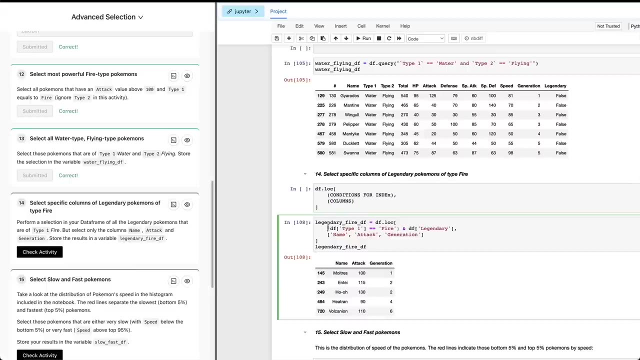 And let me break this, these two modes. So we get vflog, So we get it And we get the regular write dflog accepts conditions for index columns, right. So here we have, and let's actually do more parentheses. 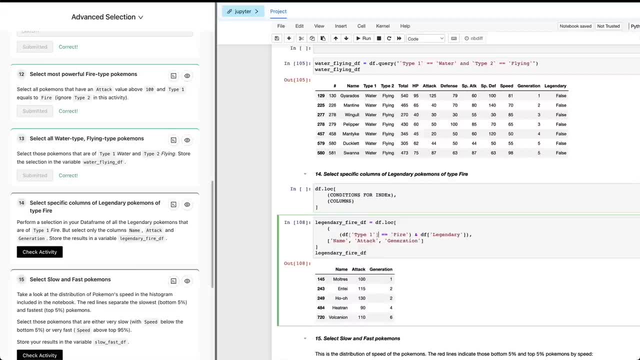 We don't need them, but let's do more parentheses so it's more clear of what we're trying to do. We need more parentheses. There you go. So this is the condition, and then it comes to columns And the final result that we have right here. 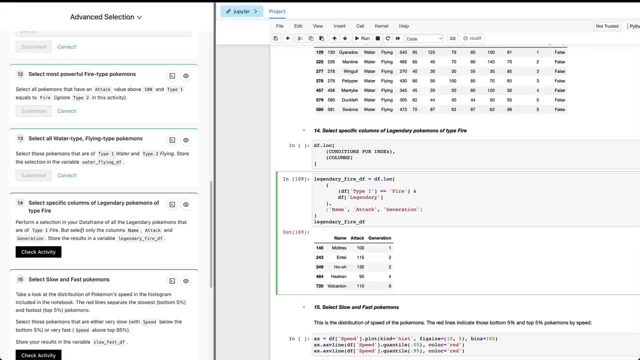 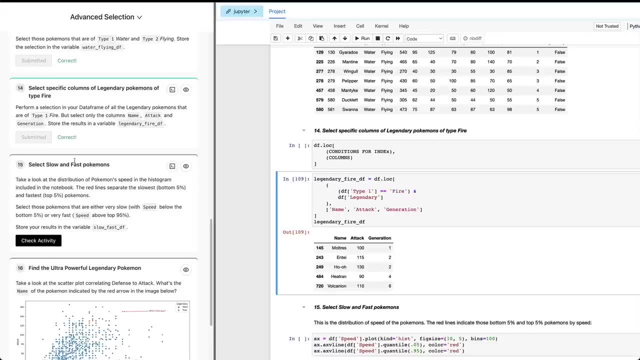 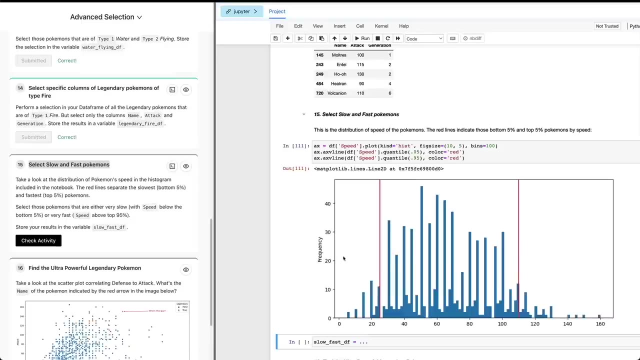 So type one, fire And legendary, And the columns are name, attack and generation. Let's give it a try, And that worked, as expected as well: Select slow and fast Pokemons. So this is getting interesting. now We're gonna see what this visualization shows us. 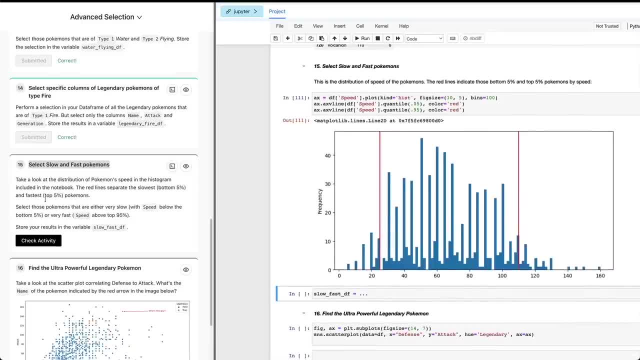 So select slow and fast Pokemons. We're gonna get all the Pokemons. Take a look at this region of Pokemons being in the histogram, including the notebook. The red lines separate the slowest, bottom 5% and the slowest. 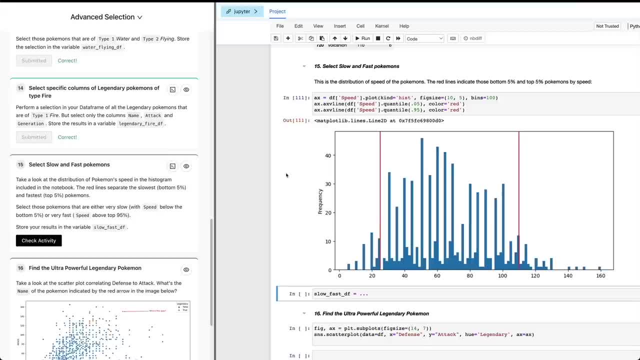 And the fastest top 5% Pokemons right here. So basically we create a histogram and then we plot two red lines in 0.05 and 0.95.. So it's the 0.05 quart quantile fifth percent and top 95th percent percentiles. 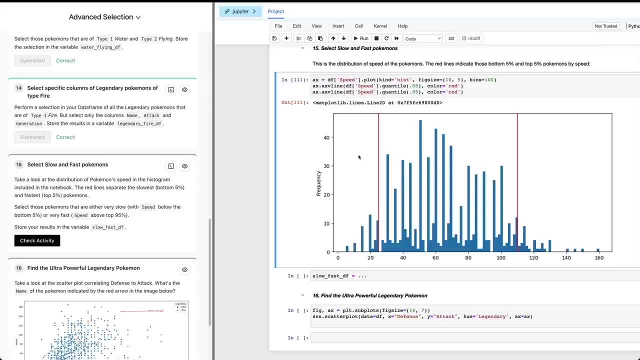 And what we wanna do is basically select those Pokemons that are either above this 95% or below the 5%, The two extremes of the distribution, let's say. So what we're gonna do is dflog And we have the values. by the way, 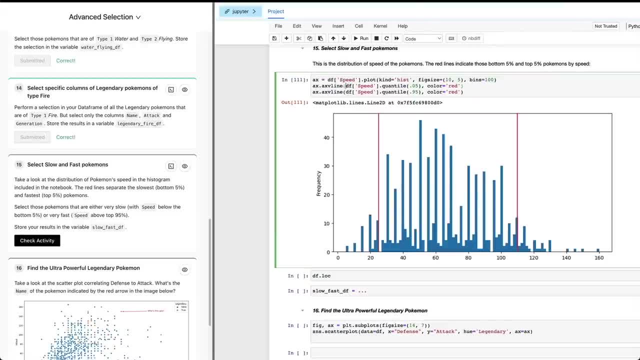 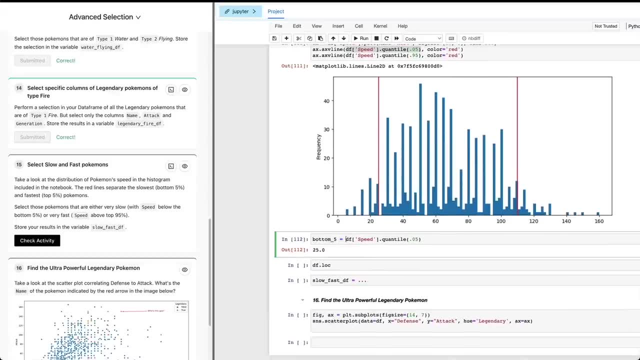 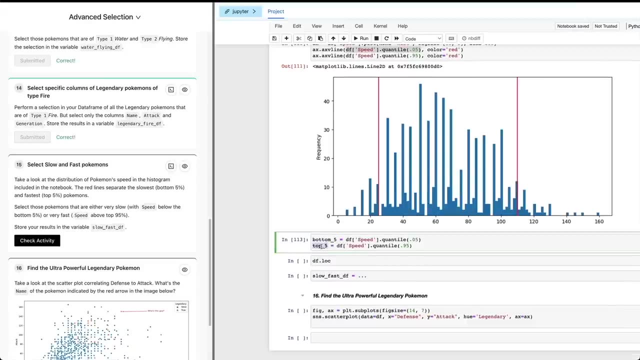 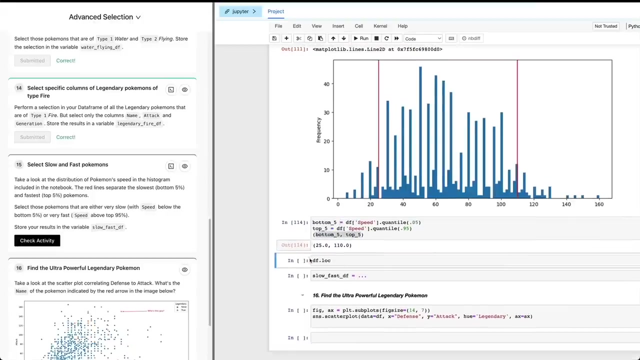 We can actually take a look at them. We can do here. Let's actually do this thing We're gonna do. bottom five is this thing. Top five is 95.. There we go, And let's show both top five. There we go. 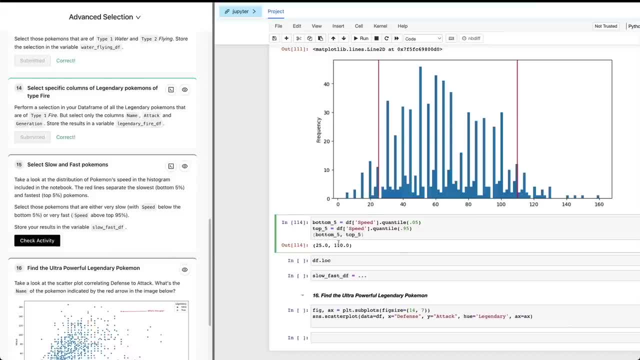 So we know that the cutoff for a very slow Pokemon is a value of 25.. The cutoff to be considered a very fast Pokemon is 110.. I'm gonna use first the dot log method We're gonna do dfaddSpeed is less than. 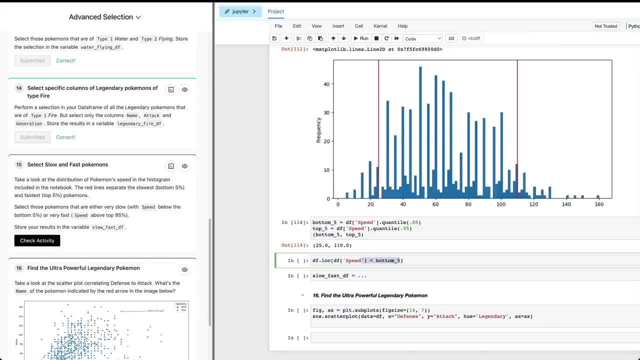 because we want it to be select. Where are we? The slowest Pokemon and the fastest Pokemon is very slow, with speed below the bottom five or very fast above top 95. So we want it to be this operation Or, and here's another one, very fast. 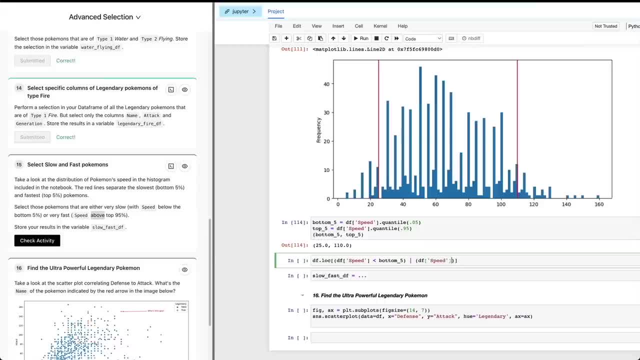 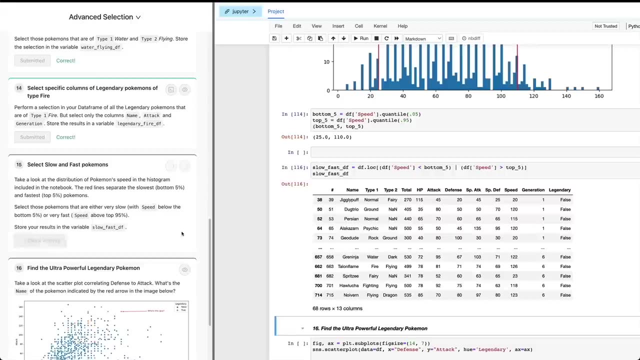 So it's gonna be, dfaddSpeed is gonna be greater than top 95. And let's put this whole thing here: Slow, fast Pokemon. There we go, there's our table, And let's try it out first to see if it works. 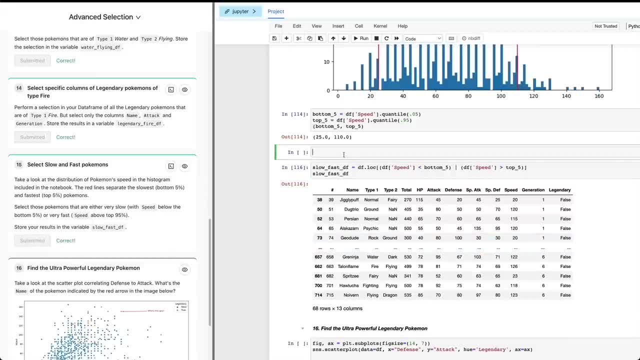 There we go. It works. But there is another way, which is basically using dot query method. What we're gonna do is dfquery, and you know this already. Speed is gonna be less than- And here to reference an external variable. 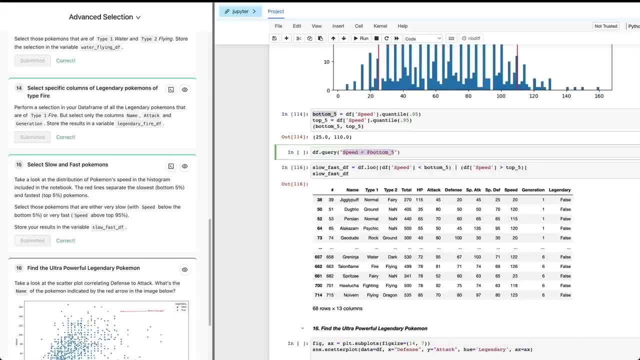 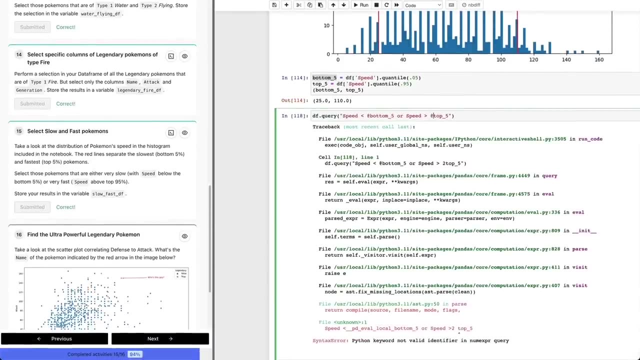 we've seen this already. we're gonna use the add symbol. So on this thing, we don't need parentheses or speed is greater than top five and we need the. there you go And we have the same result: 68 rows, 13 columns, the same result. you can trust me. 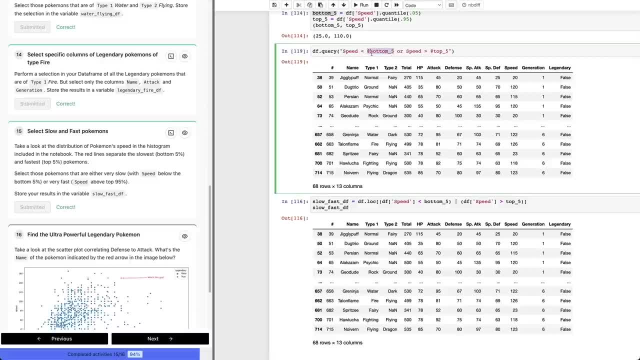 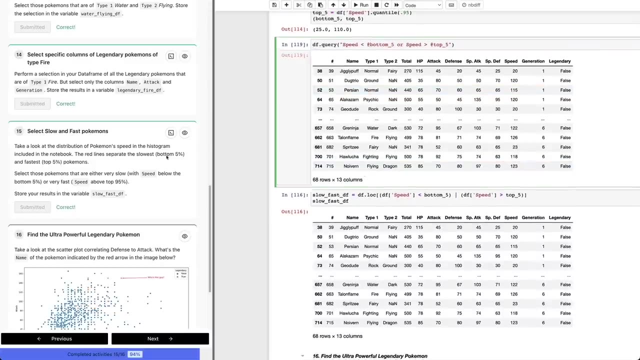 But basically the important point here is we are using an external variable and referencing it with the at symbol right To reference something outside of this particular query. Speed references the column the at this thing references an external variable we have defined before. All right, and I think we have the last one. 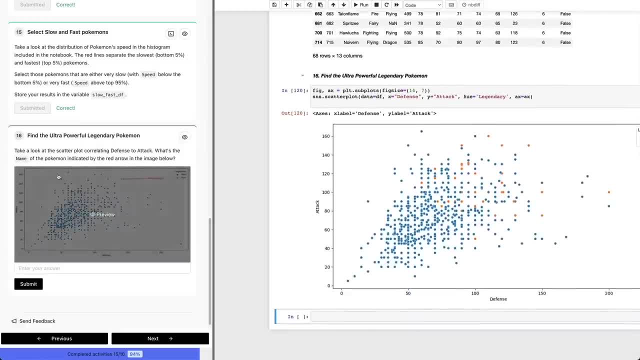 and this is a very interesting one as well. It says: take a look at the scatterplot correlating defense to attack. What's the name of the Pokemon indicated by the red arrow in the image below? So who's this guy Right here? 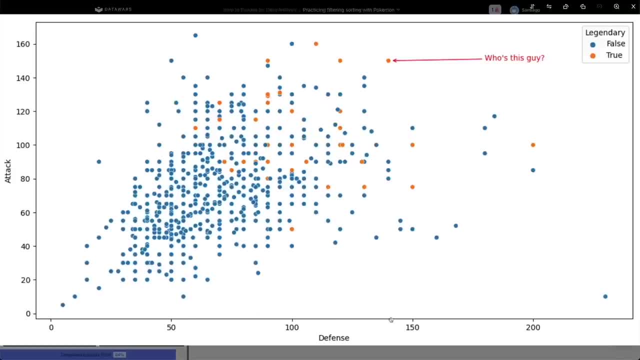 And it's a Pokemon that has a strong defense and a strong attack. So what we can do is sort by both values. So we have, like this case: first is legendary And second it has a very strong top attack and a very strong defense. 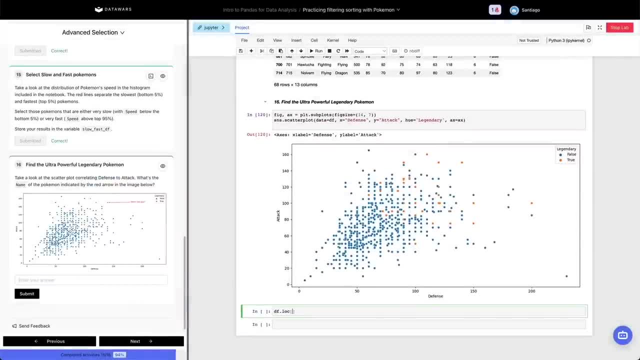 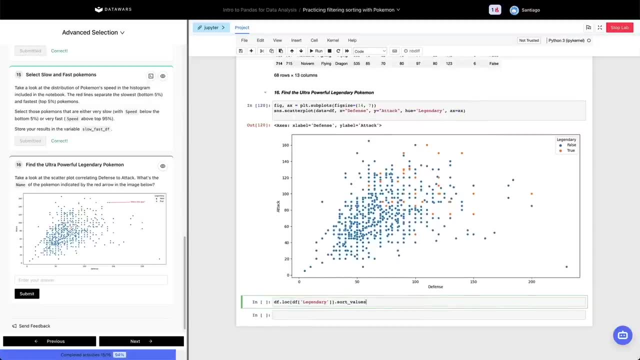 So let's take a look. The first thing we're gonna do is filter all the legendary Pokemons, legendary And sort values. We're gonna sort by doing by defense and attack. There you go by both those criteria, Or actually we can swap it defense. 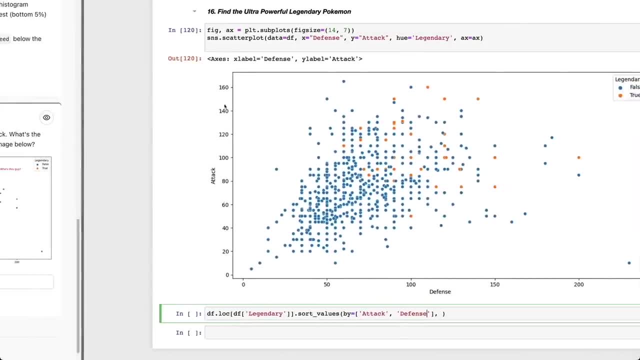 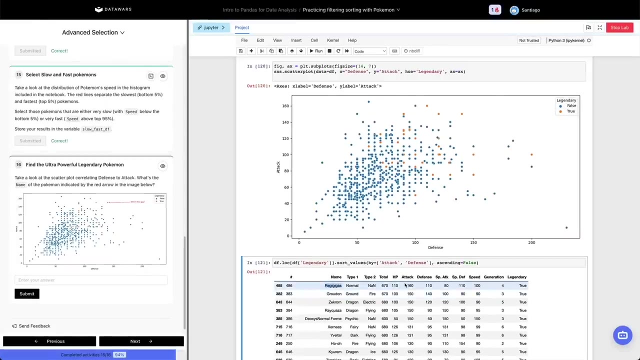 So we take a look at it in a more vertical way. So we're gonna sort in this way and then in this way, And of course we wanna do ascending. So we're gonna sort by this and we're gonna sort by this. 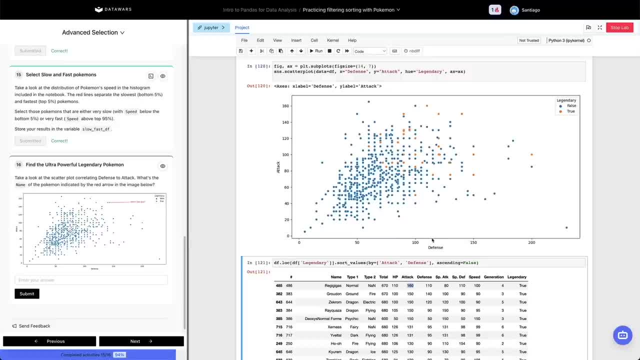 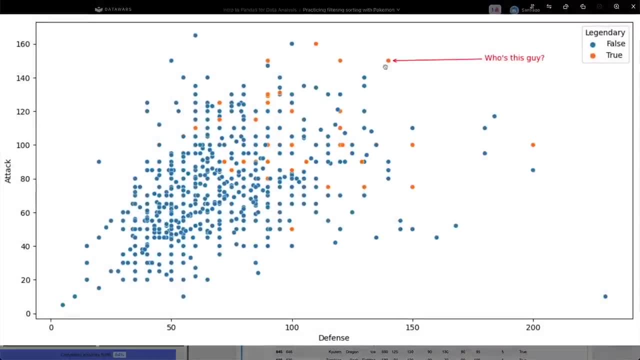 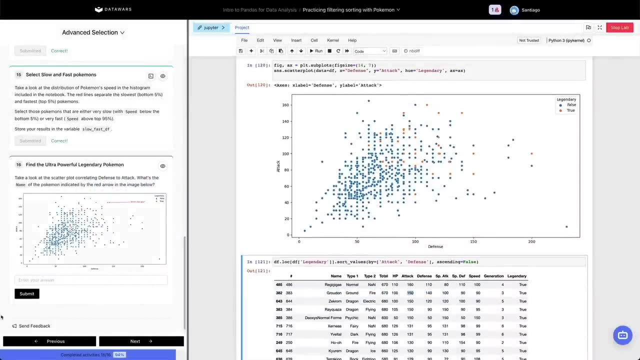 And in the right now we're gonna sort by this And since it's a high attack, then it's a high defense. So it's gonna be like this False, And here we have have these pokemon that has an attack of 150. so again, right here it matches and a defense. 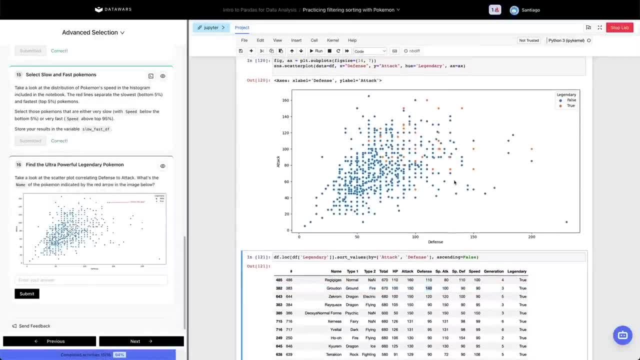 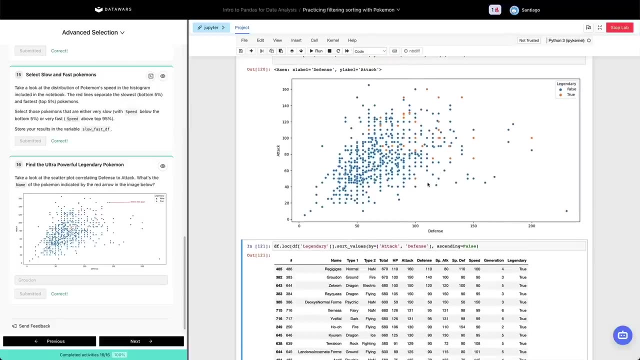 that is 140, so this one looks a lot better. let's try it out and see if it works and have our value, and there you go, all correct, all complete. but basically what we're trying to do here is using this combination of visualizations with the analytical power. we're filtering, we're 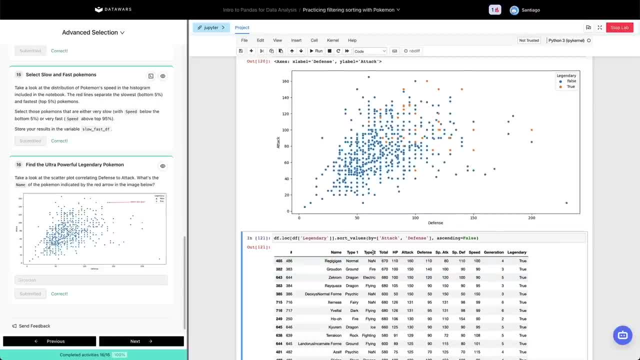 sorting and we're putting everything together to answer the question. so this was the whole practice about filtering and sorting pokemons. very interesting one again. if you have a chance, try to solve it by yourself, or there are a few more projects related to filtering and sorting all yours. let's keep solving more projects. 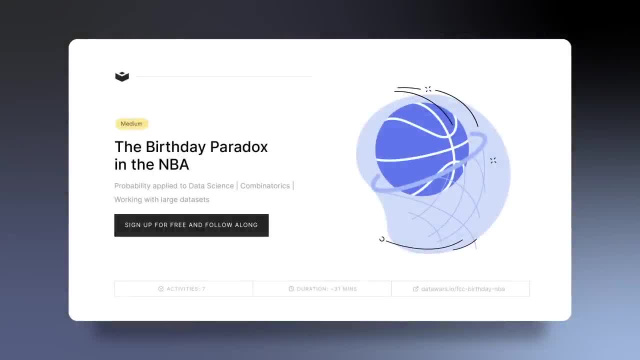 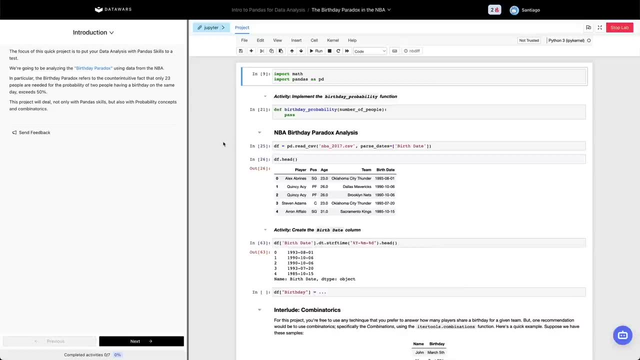 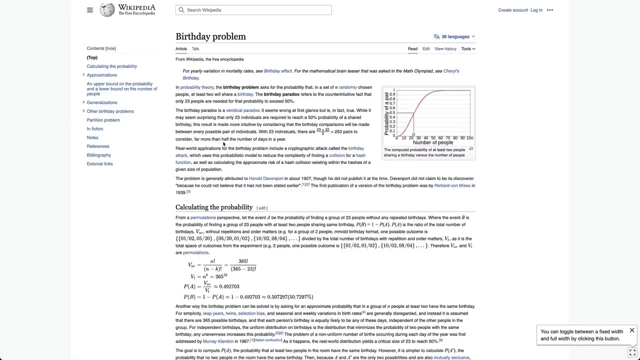 in this project we're going to be working with a pretty interesting problem, which is the birthday paradox. the birthday paradox comes actually from the birthday problem, which is a more general problem. that is basically answering the question: if you put n people in a room, what is the probability? 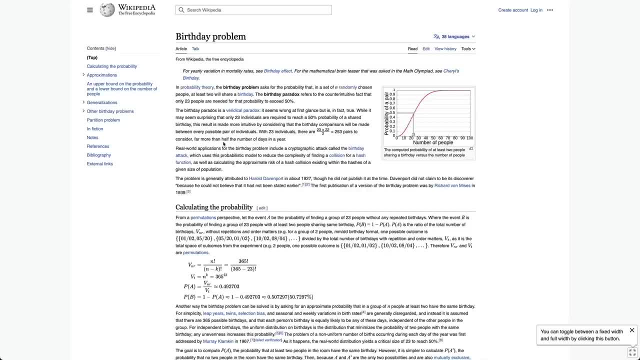 that two people share a birthday right. so, for example, i have 70 people in a room. what is the probability that two people share a birthday right? so, for example, i have 70 people in a room, that to any pair of two people within that room, within that room of 70 people. 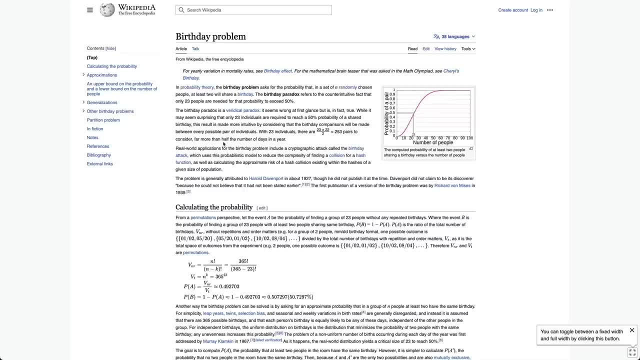 share a birthday and it's. there is a formula to calculate that birthday paradox, but it tells you, is that it's basically what is the number of people that i need to. i need to put in a room for that probability to exceed 50 and the counterintuitive fact that only 23 people. 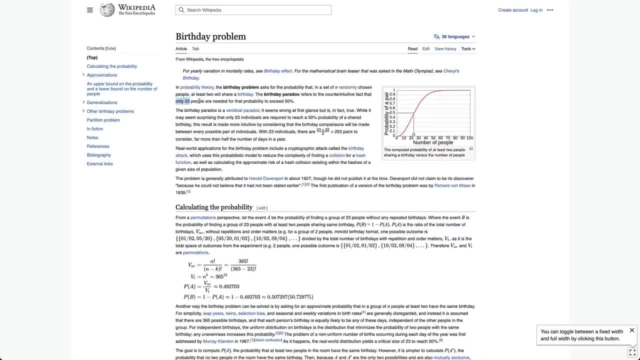 are needed for that probability to be above 50. so again recap: only 23 people in a room are needed for the probability of two of any of those people, any pair within that room, to share a birthday right. so only 23 people are needed for that probability to exceed 50. and this is a 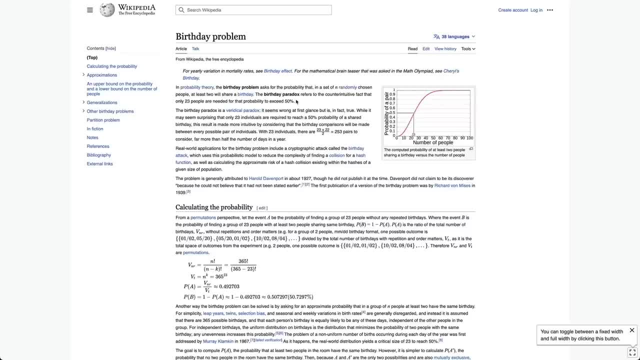 counterintuitive fact to be, i'm, at least to me. the first time i got asked this question, my reasoning was: well, what is the probability, sorry, what is the number of people that i need to be 100? sure that two people are going to share a birthday and the 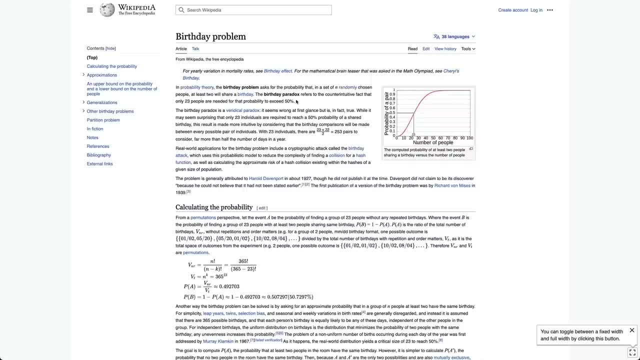 answer is, of course, 366. there are 365 days in a year, so for me to be 100 sure- probability equals one that two people share a birthday- i need to put at least 366. that's going to be 100 sure. so when i got asked, well now what is how many people are going to share a birthday? i need to put at least. 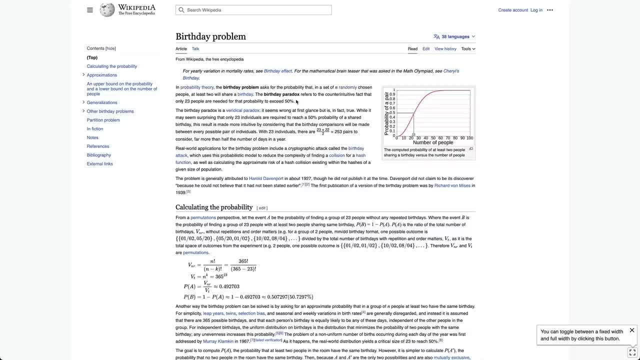 how many people do you need for that probability to be 50 percent? uh, my first reason it was like i don't know, 100, 150, half or 365, you know it's like. and then when i got the answer and i got to calculate, the answer is like obvious, it's just well, only 23 people are needed for that. 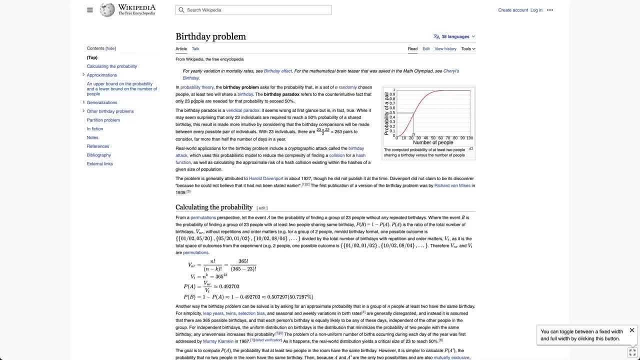 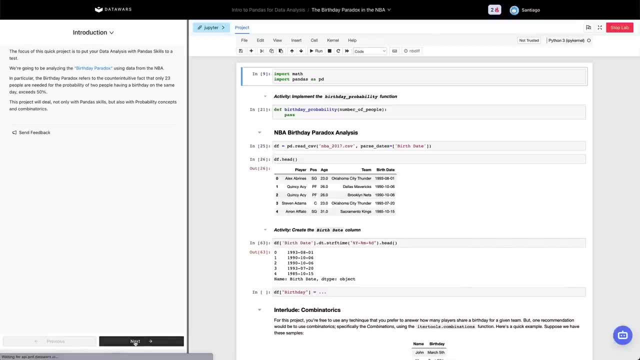 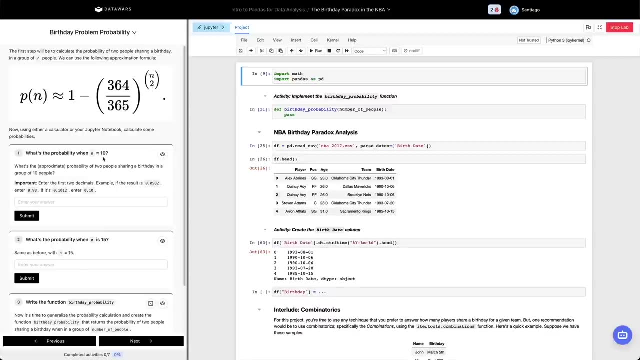 probability to be 50 and we will actually understand why in a second. so basically, this project deals with the birthday paradox and us calculating the birthday problem, the probability of two people sharing a birthday in a in a group of n people, um, and then we're going to apply that. 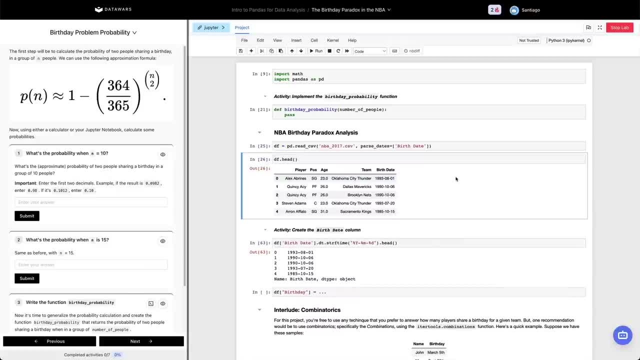 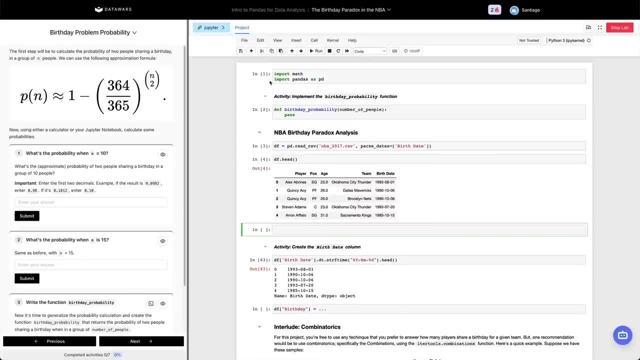 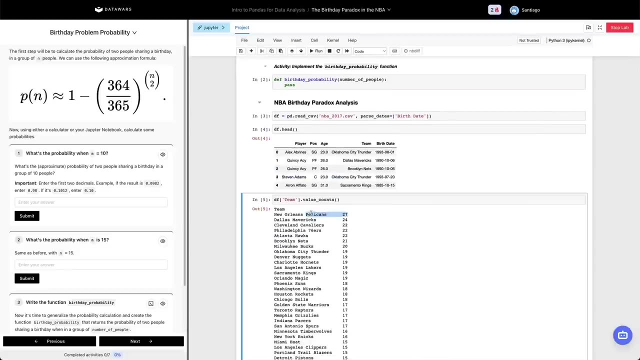 to nba teams and this is going to be a pretty interesting thing because the teams we have here we can actually run this thing. um, we can do df at team dot value counts. we're going to have teams that have 27 players, but then we have 24, 22, so we're going to see 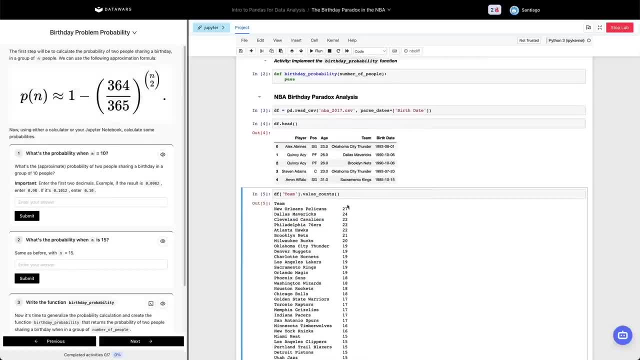 how many like if this probability stands, you know, if we're going to have here the probability of two people sharing a birthday in a team of 24 people, the probability is going to be greater than 50 percent. are we going to find matches here or here or here, etc. right, so that's going to be. 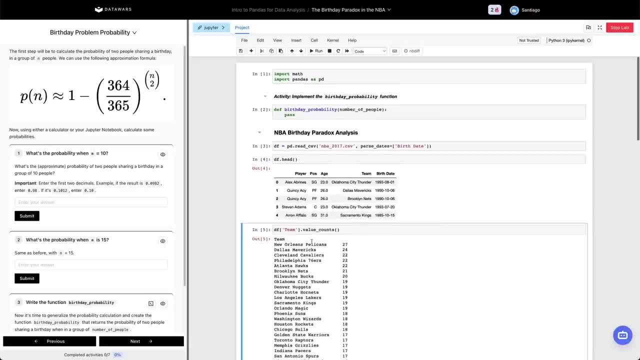 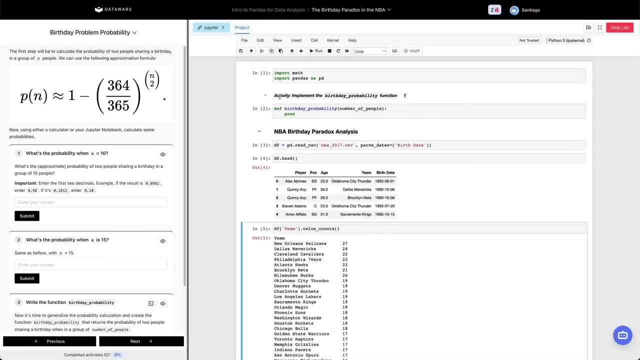 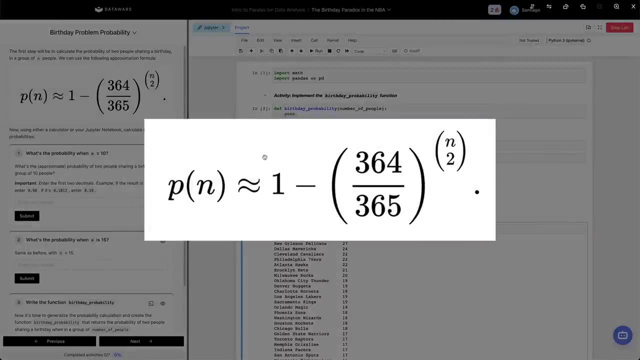 the problem we're going to deal with. but before we jump to the data, we're going to start with the calculating the probability and understanding the intuition behind this thing. the way we calculate this probability- and again is this formula- is: what is the probability of two people sharing a birthday in a group of n people? so we swap n here. we say, we put: 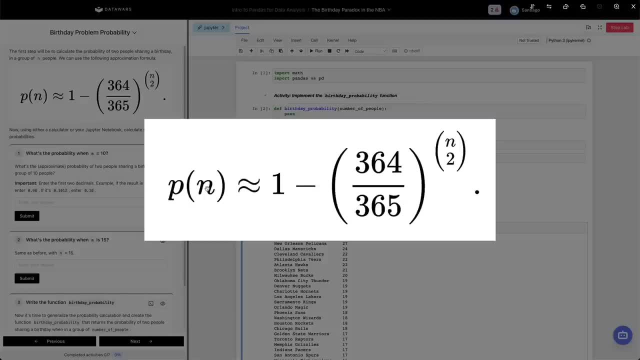 10 people in a room, 20 people in a room, 50 people in a room, and we get a probability back of uh, two of them, at least two of them, sharing a birthday. and the interesting part of this formula is right here is the combinations piece, and this is when 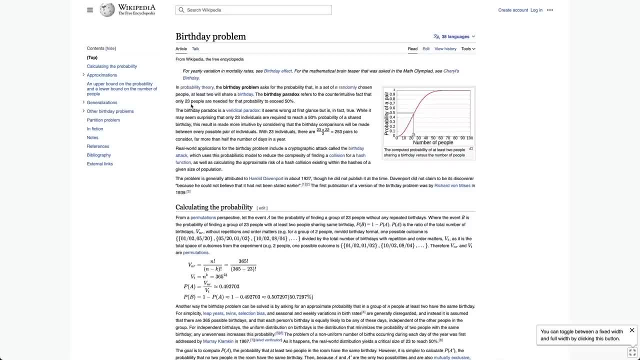 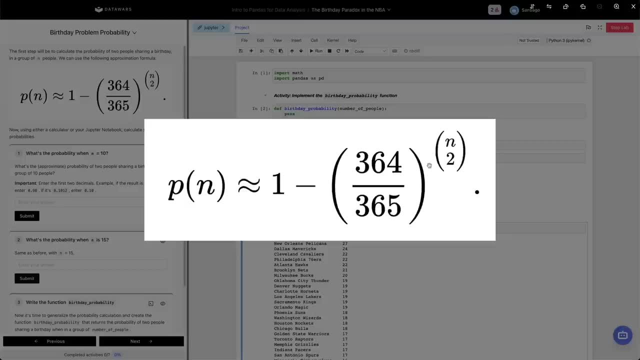 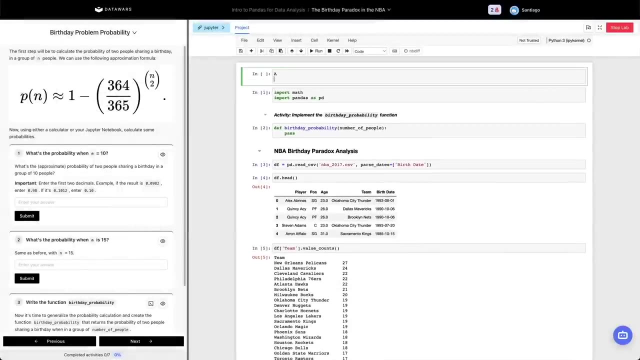 this, this number, only 23 is needed to get 50 percent. it starts to make sense once you take a look at this combination. uh, formula here and combinations just a week. a quick recap is: if you have um, a, b, c, d, e, people rob john mary susan. 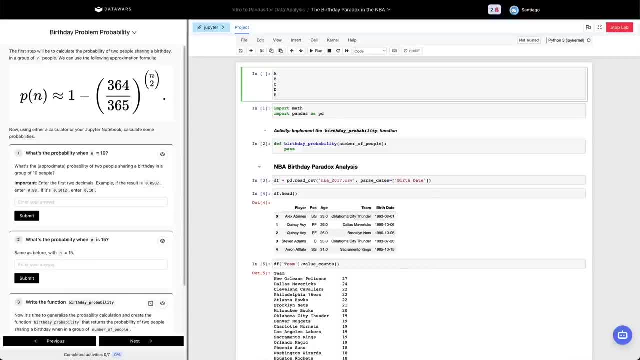 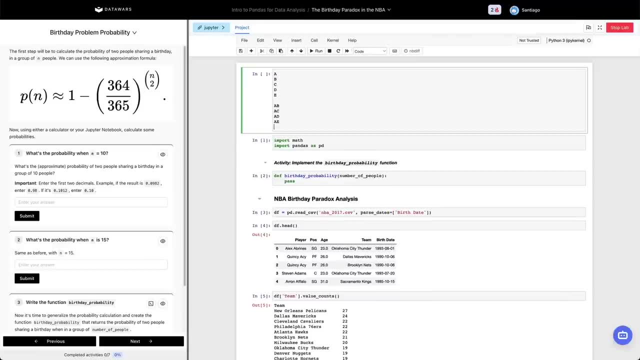 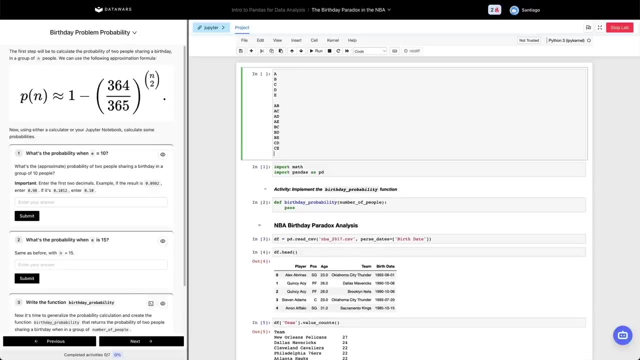 violet, etc. the way you can combine them is basically a with b, a with c, a with d, a with e, b with c, b with d, b with e, c with d, c with e and finally d with e. these are all the combinations you get so pretty quickly. if you start thinking in pairs of people, this number grows pretty quickly. 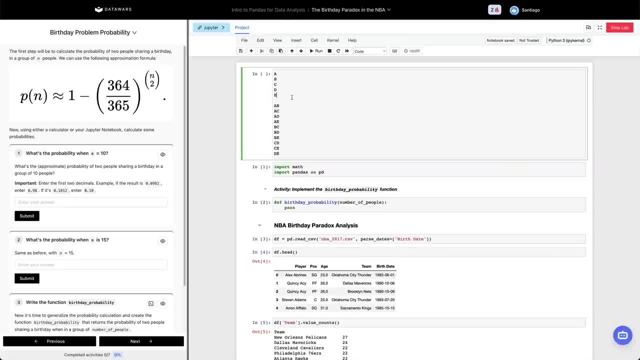 if you start thinking in pairs of people, you get a number that grows pretty quickly. if you start thinking in pairs of people, you get a number that grows pretty quickly. if i put just one more person here, let's say, one more person joins the room, i start adding. i will add five more combinations. 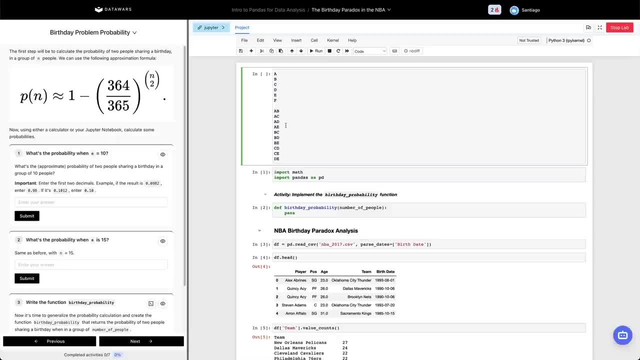 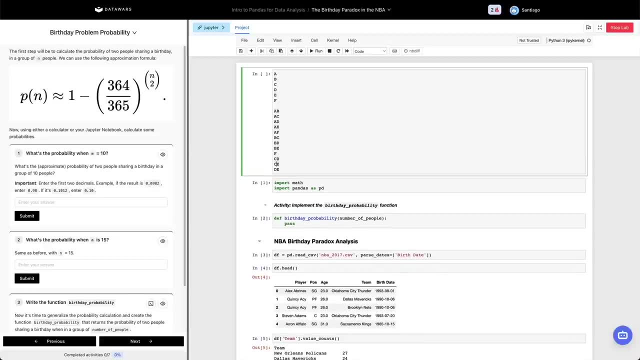 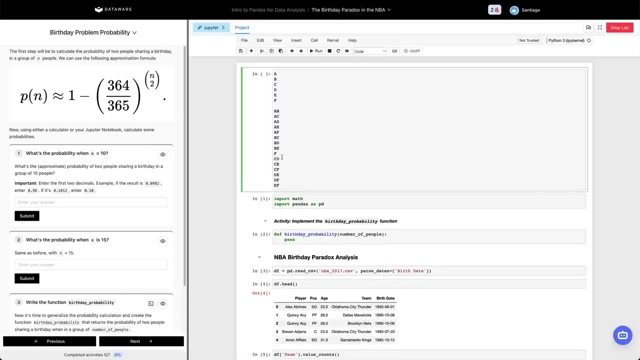 because it's f with a, b, c, d and an e, so it's gonna be um, it's gonna be a and f, now b and f, c and f and d and f and e and f. so one more person- uh, what did i do wrong here? one more person that i 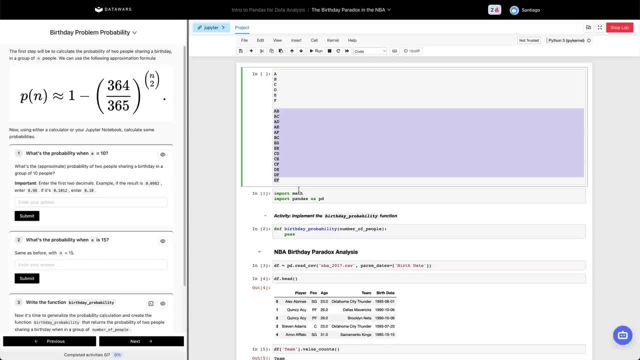 go to the room and this number of combination grows by the previous amount of people in the room. right, i add one more person- g, i'm gonna do g, f, e, d, c, b, a. right, it's gonna grow by six. i add one more person to grow by seven. it keeps growing, it keeps growing, it keeps growing. so that's why. 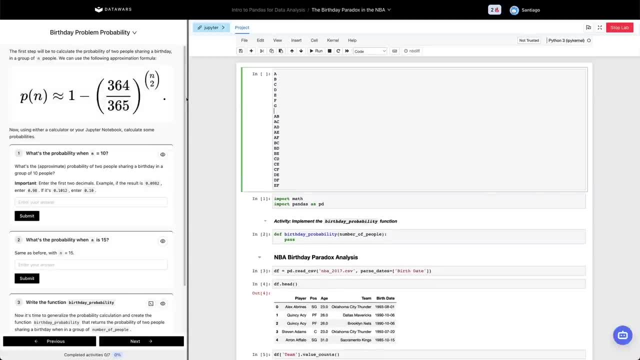 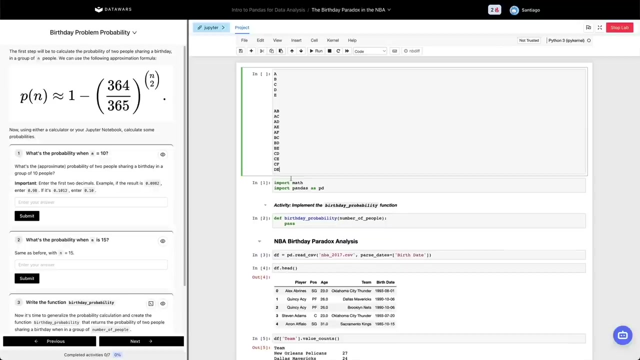 i- at least to me that was what made this problem- click and understand that it's a very small number, that we need only 23 for the probability to exceed 50%. we can actually calculate the combinations piece. so so let's get rid of this, and by F, so F is no longer. 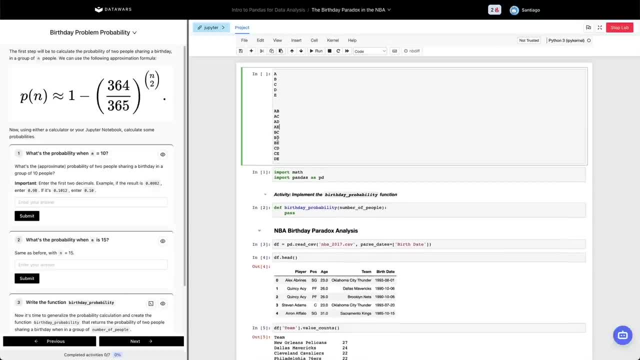 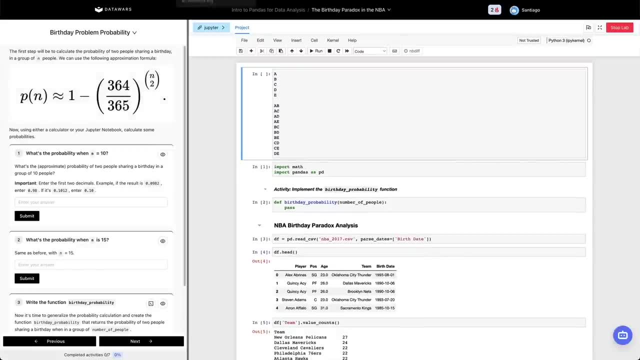 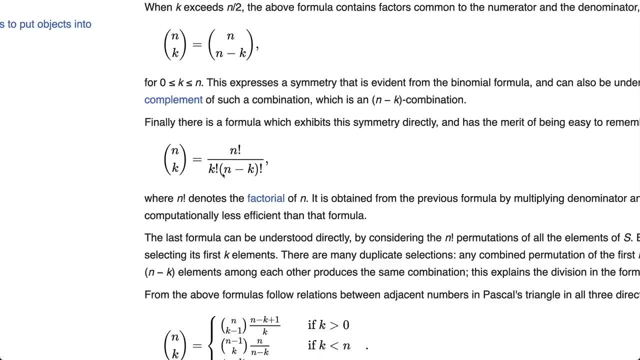 invited to our party. so we have ABCD and we can calculate the result of combinations of n taken by 2, and this is a pretty, pretty simple in a formula. it's n factorial divided by K factorial times n minus K. n and K in this case is 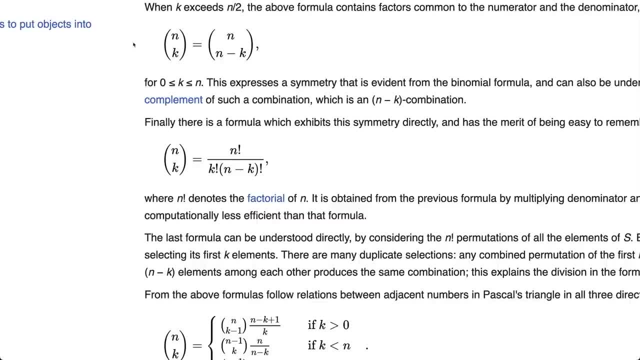 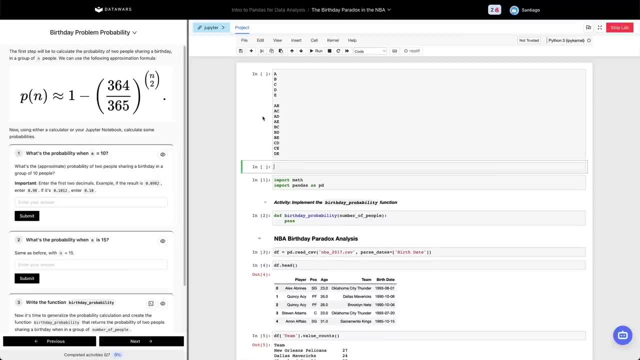 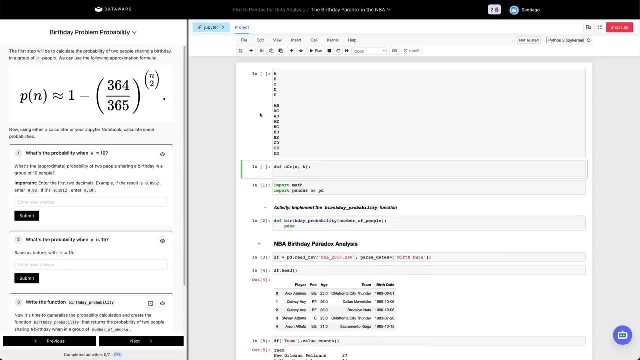 n people, or n taken by K. in our case gonna be n taken by 2, but we can very quickly hack this formula. it's gonna be that we call it n CR are of n taken by K, and the way it works is that we can calculate the result of the combination of: 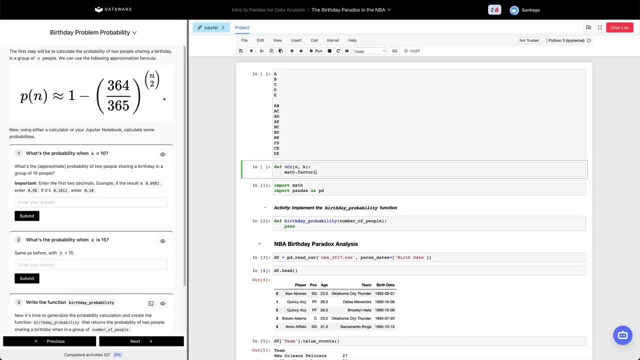 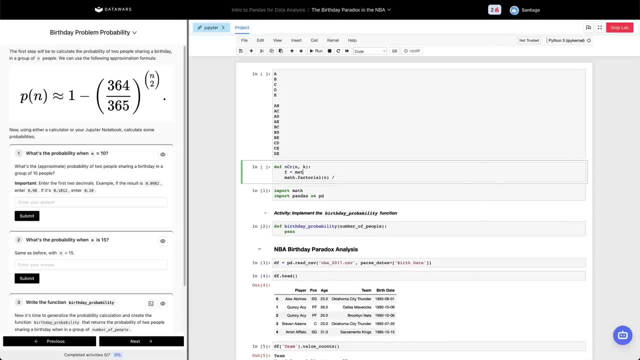 n and the way it works is we can just do math dot factorial of n divided. and if you let me, I'm gonna do something just here. shortcuts is the beauty of Python again. just assign a variable to a function, factorial of n divided, factorial of K times factorial of n minus K, and I will return this whole. 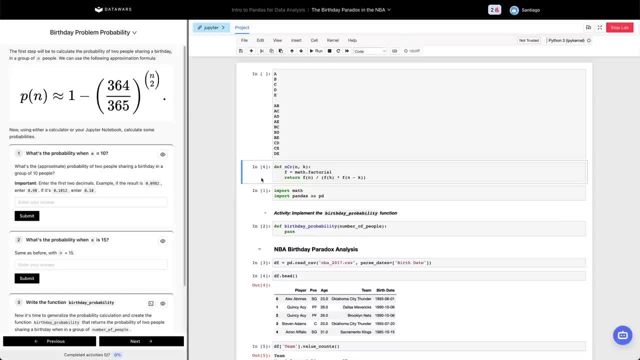 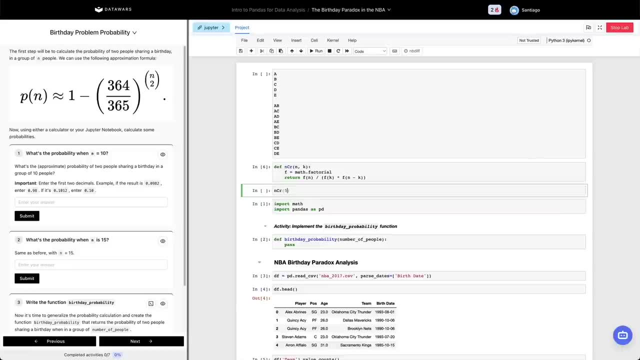 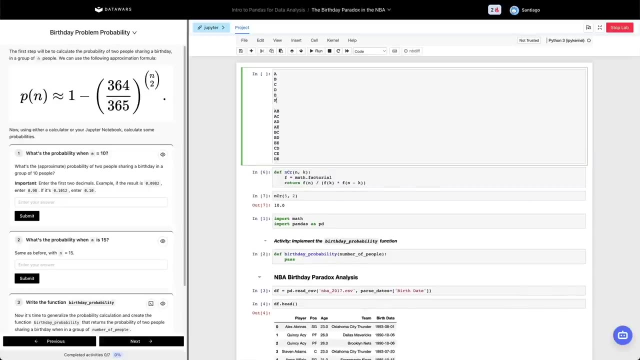 thing we have, that the combinations of five people and CR of five people taken by 2 is 10. we said: if we are a sixth person, this thing is gonna grow by five, right? so it should grow by 5, and I have now six people- 15 was that, if we add another. 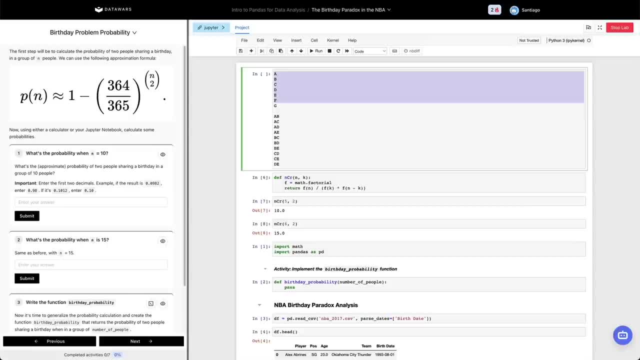 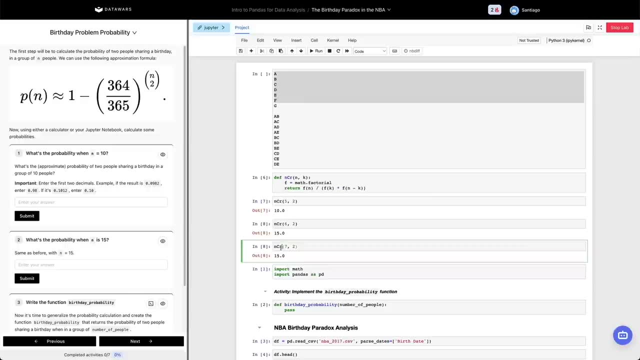 person right here. this thing is going to grow by all these previous one, so it's gonna be by six more. So we're going to do: if we have seven people, this should grow by six, should be 21.. There you go, So we're calculating this thing on the fly. 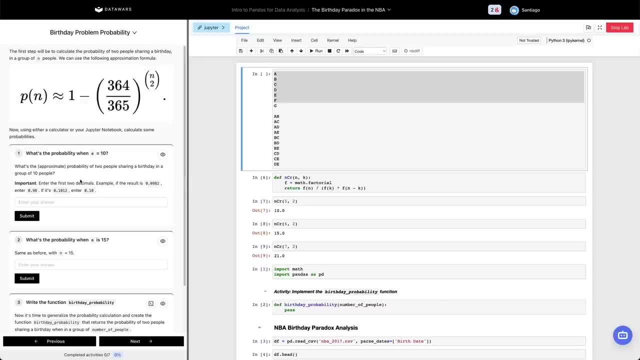 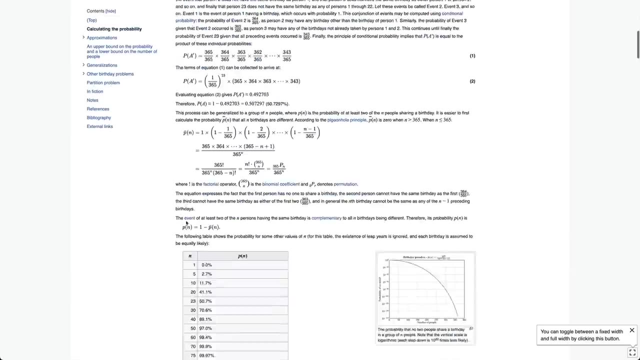 That's the way it works. So now let's get to the activities. In this case, the project is asking us to calculate the probability right When n is equal to 10.. And we can actually take a look at. there is a table here. 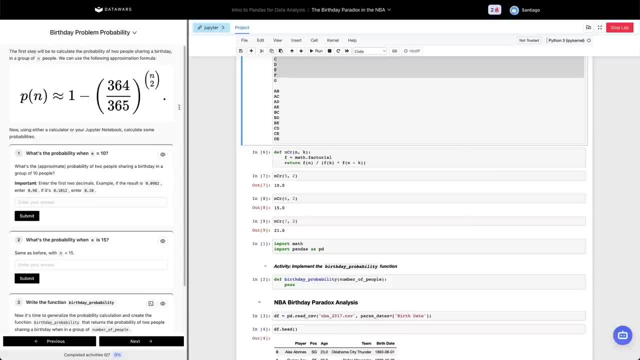 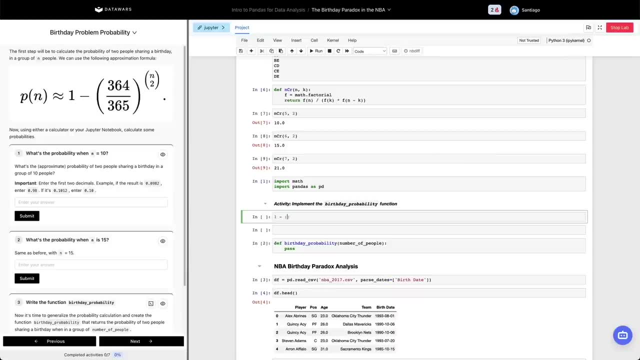 We can kind of cheat: that is the value, but we can calculate it ourselves. And to do so, what I'm going to do is something like: we have 1 minus 364 divided by 365.. And here we're going to do, we're going to use our formula, or, sorry, our function- that we calculated before. 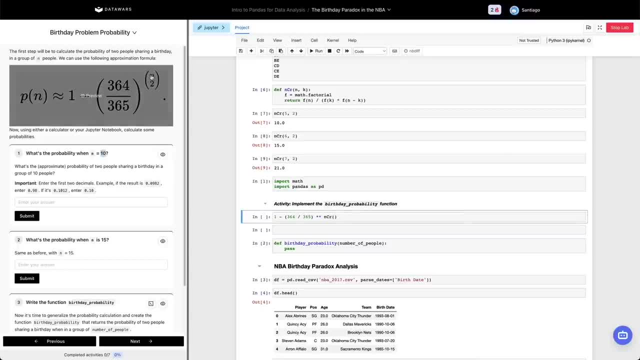 that is equal to 10 people taken by 2.. So n taken by 2, in this case n is going to be 10.. So we're going to do 10 taken by 2.. And we're going to use parentheses here, just in case. 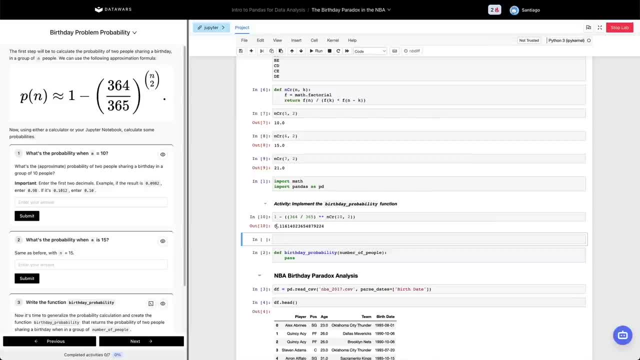 And our probability is 0.11614.. In the table was 0.7.. I don't know how they computed it, what rounding they did, but it's pretty much the same value. Let's see if this is okay. It is okay. 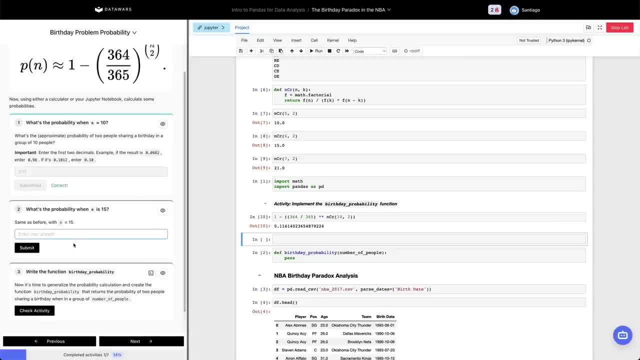 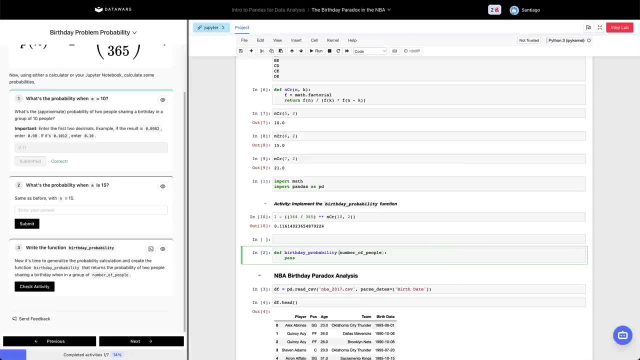 It's asked us for now Equals to 15, but I'm going to go ahead and it's asking us to implement the function. So, given number of people, calculate the function. so we can do it generically And the way I'm going to do it, it's just going to do return this thing. 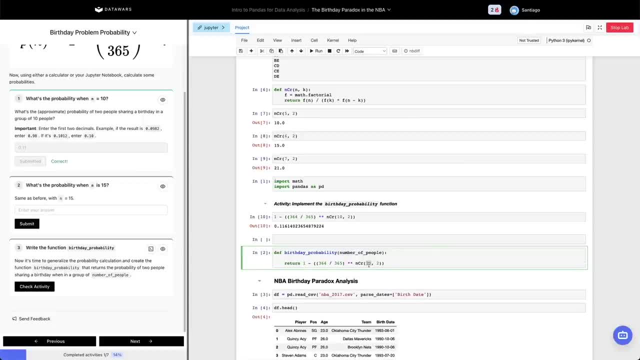 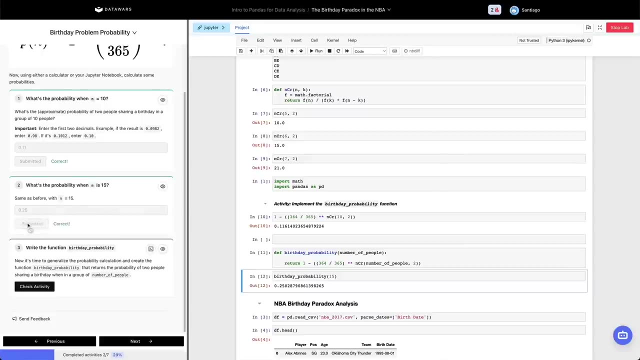 And I have to swap just one parameter. that is here: number of people. There we go, And now we're going to do birthday probability of 15.25.. And we'll put here 25.0.5.. And it worked as expected. 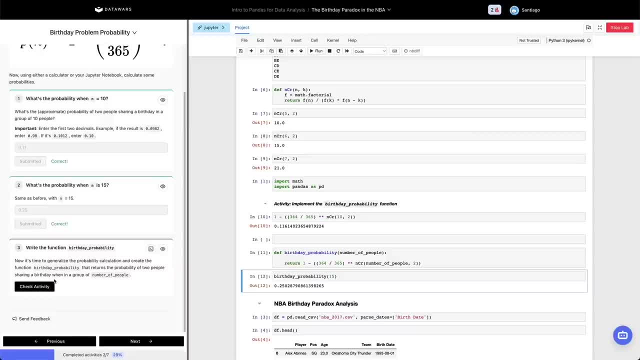 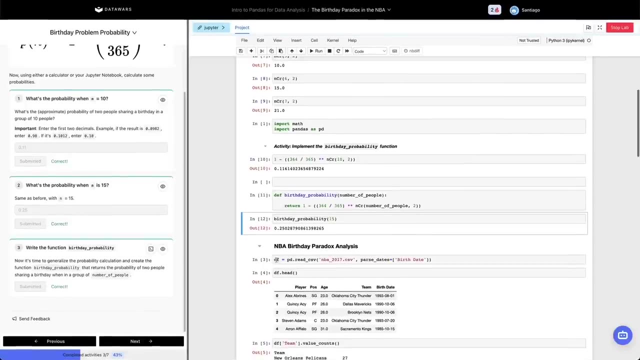 And we can check. now the birthday probability function all at once And it worked as well, So we're good to go. So again, this was quick recap For this project, not to be extremely mathy, but it was just a quick recap of the birthday problem. 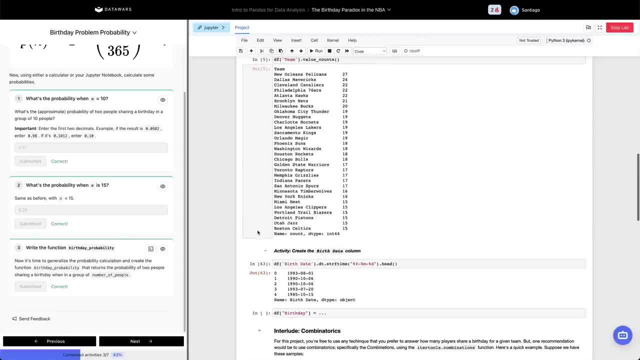 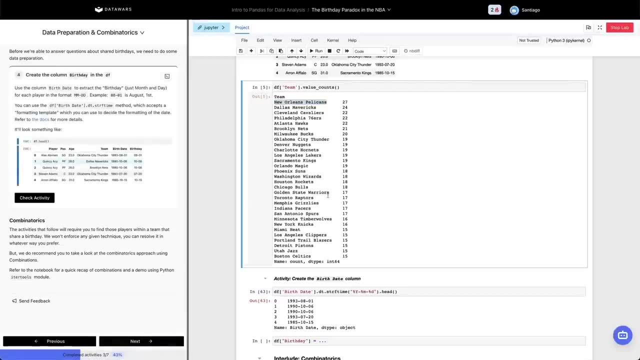 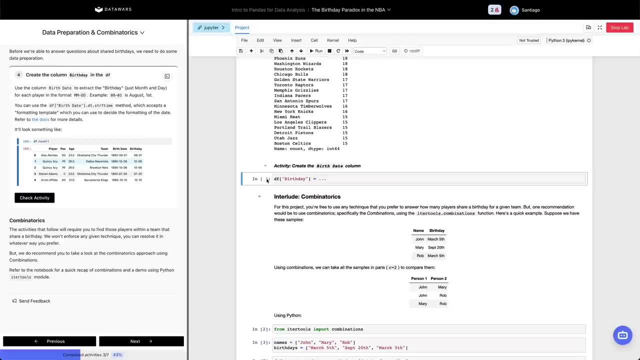 And now we're going to apply that to our data set To see how many people within a team share a birthday, if any right, It's going to be a pretty interesting one. So the first thing that we're asked to do, I'm going to delete this thing. solution is: we need to extract. 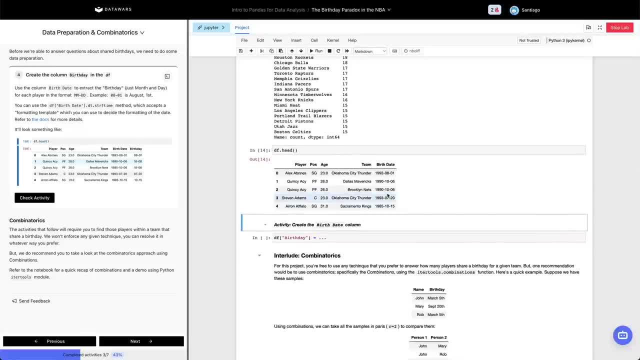 Let me show you again the data frame. We're going to extract the birthday birthday from the birth date function. So date is the actual date Day, month year- We want to extract only the birthday right. So for two people to share a birthday, they just need to be month day. 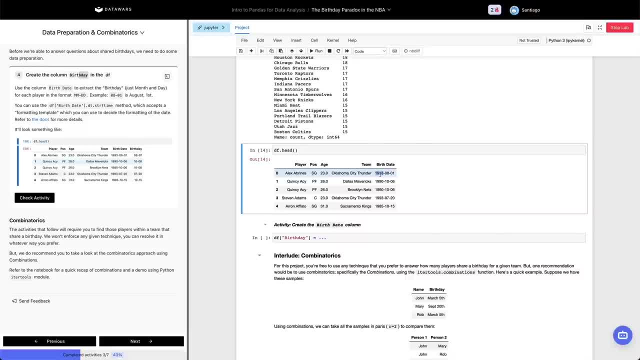 It's like: hey, my birthday is September 29.. Yours is September 29.. We share a birthday, but potential is going to be different years, That doesn't matter. So we need to extract here the month and the day from this data frame. 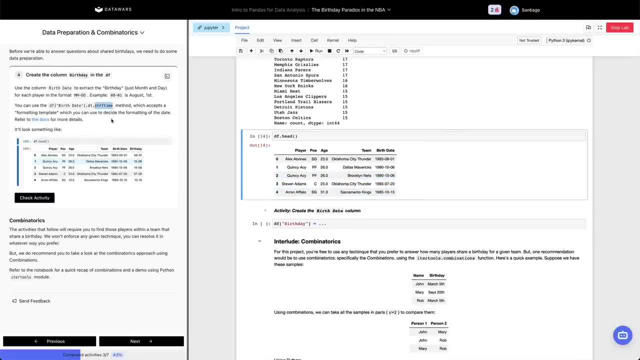 To do so, we can use the strf time function, String format time function. That is actually part of Python. In this case it's implemented for a tuple And it's implemented. Let me show you this here. It's implemented in the column birthday with a DT special accessor. 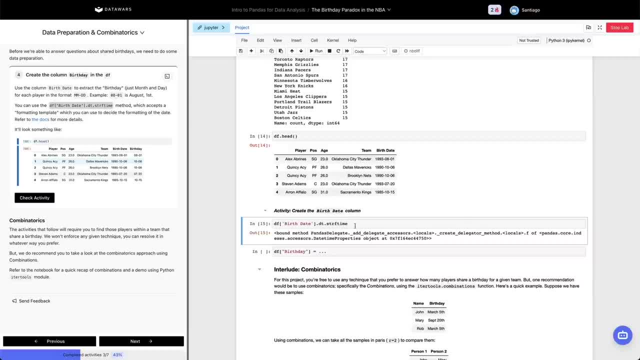 Don't worry too much about it. The only thing we have to do just go ahead and Google the syntax to get this thing, to get this format as expected. The way it works is: This function is going to receive a formatting So, for example, we can get the year and the day right there. 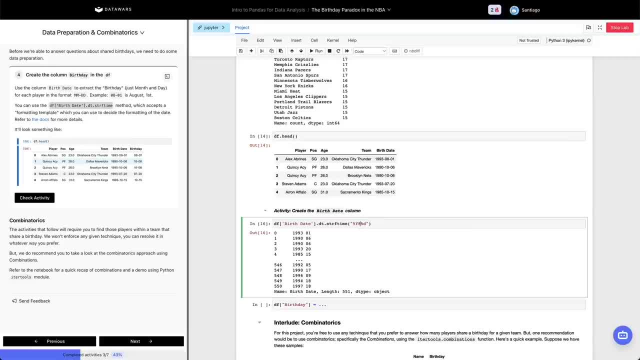 We're going to get they and year, And here we can put whatever we want. We can put an at sign and hello world, And it's just going to be a formatting. It's going to format this string That's going to replace with special values, starting with the percentage symbols. 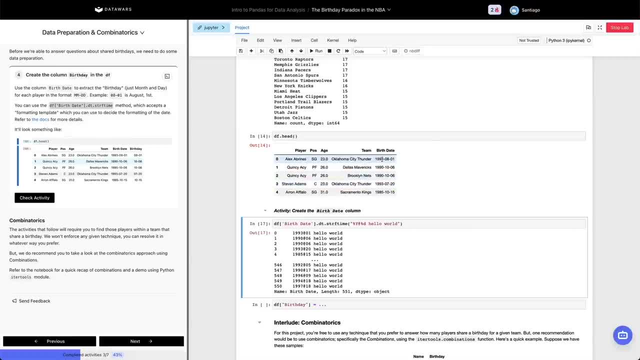 And the question now is: How can we get only month and day. This is what it's asking us for birthday? We can actually go ahead and ask our assistant. We can say: how can we format the column birth date in the format month day? 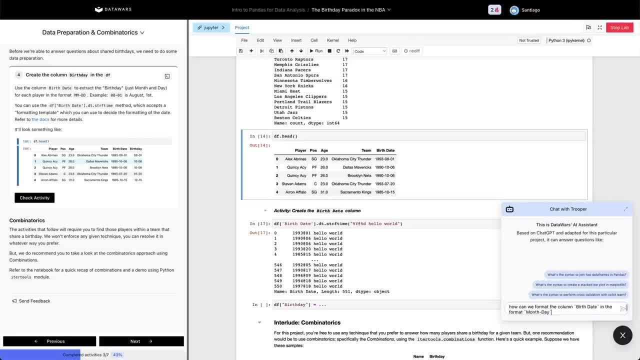 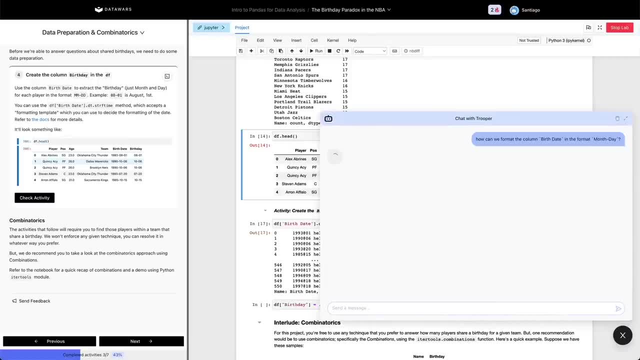 Do we have month day without space? And let's just go ahead and ask the question I'm going to criticize here. There you go And we get pretty much these formats, Um, pretty interesting. uh, because it's actually the- the correct answer. 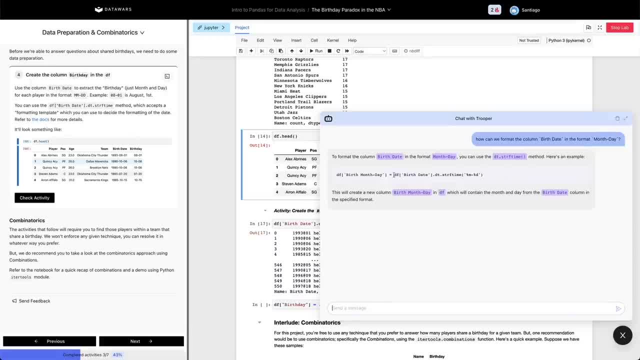 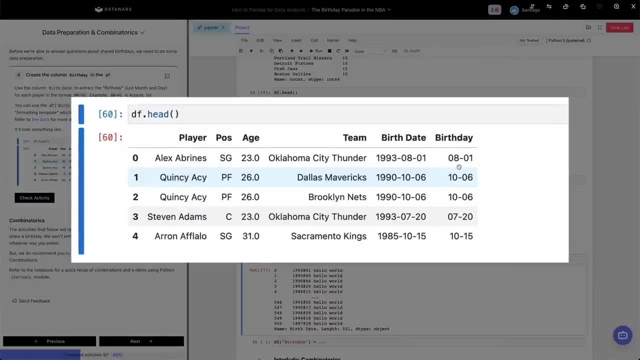 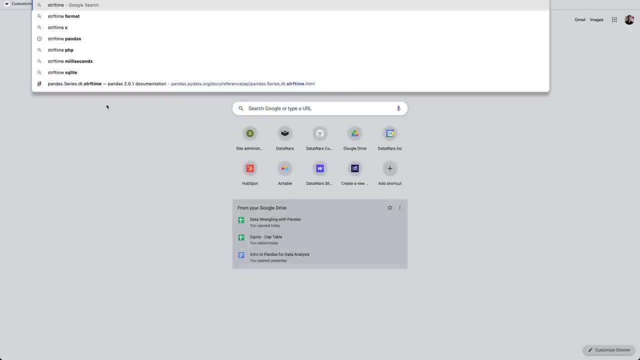 Um, and let's try it out. Can I copy this thing? We're going to, there we go, And this is the correct format. So you can see. um, if you want, you can Google. we can say: um, STR of time pandas are going to find this method. 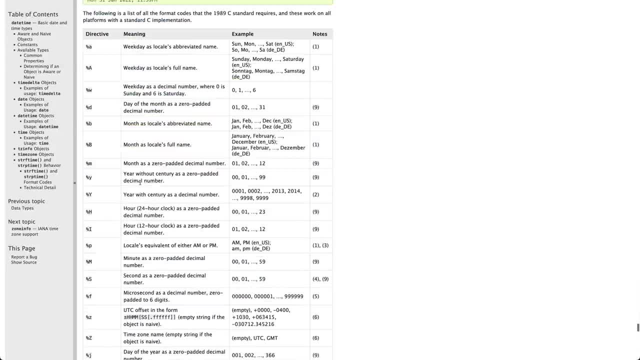 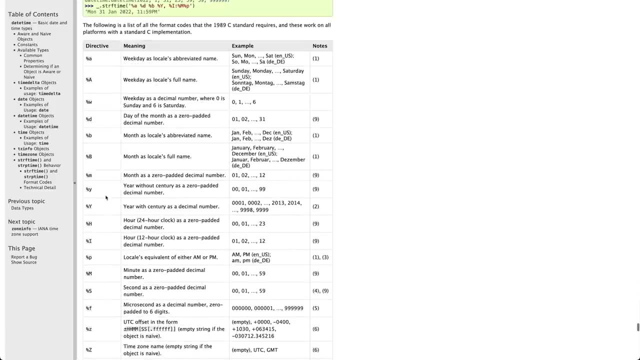 We can hear, find Python string format documentation And here you can validate that percentage D is going to give you the day with leading zeros, which I can't find. but but trust me, There you go, Day of the month and zero padded, and then we're going to use percentage month, which 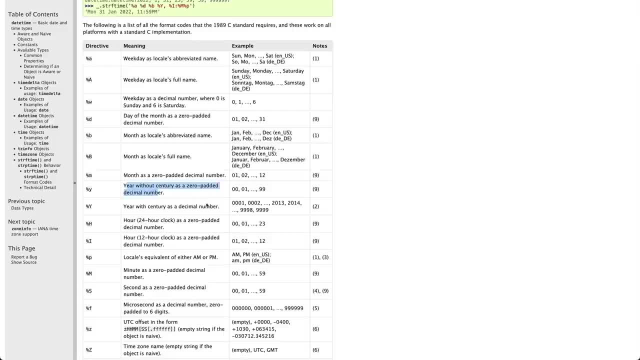 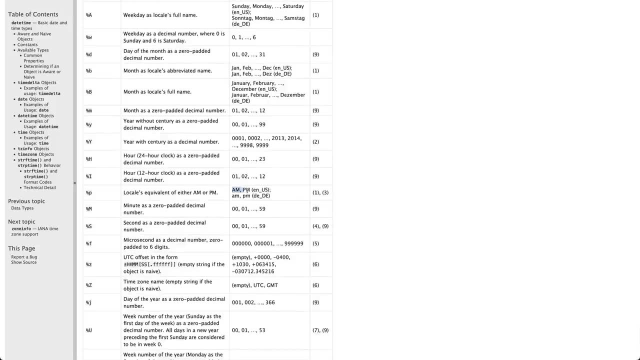 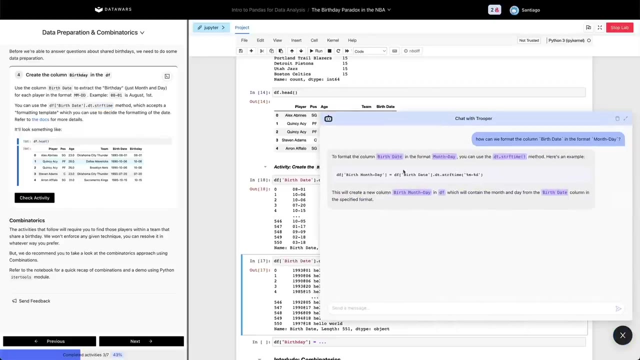 is zero padded, And then you can get year. you can get year with the four digits Um, you can get uh. day of the week. you can get and PM four times Again, you can do any formatting you want. in this case we only need the um month. 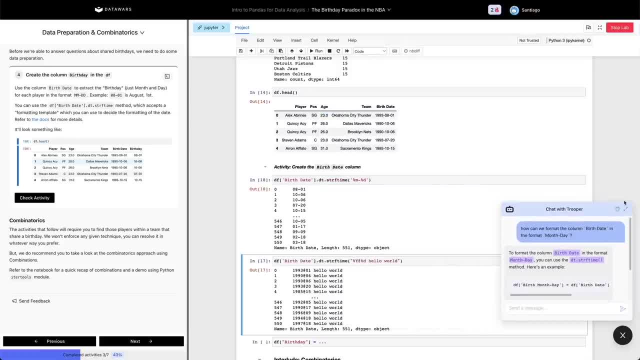 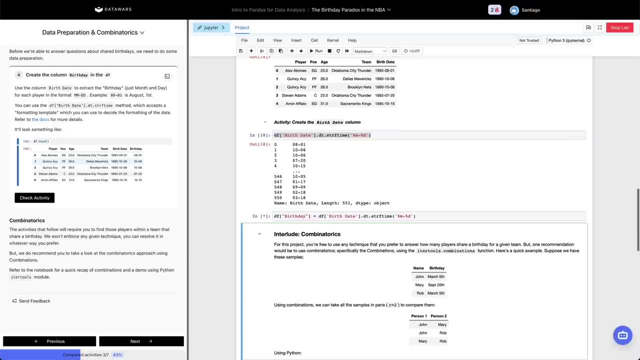 and day. So this is the format that we are looking for. Close this one, And now we're going to assign this value here. Okay, We're going to check. We're going to check to see if it works. There you go. 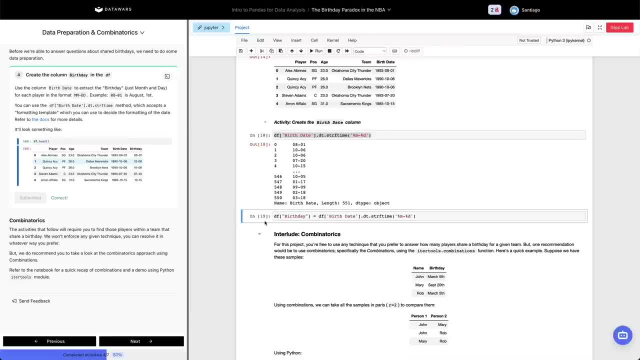 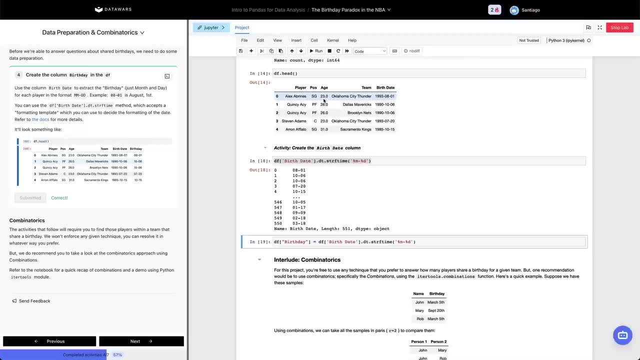 It works. Now we know already what we want to answer is how many or which players or how many players within a given team. this is important. share a birthday, So we need to separate all the players within a team and we need to find the. 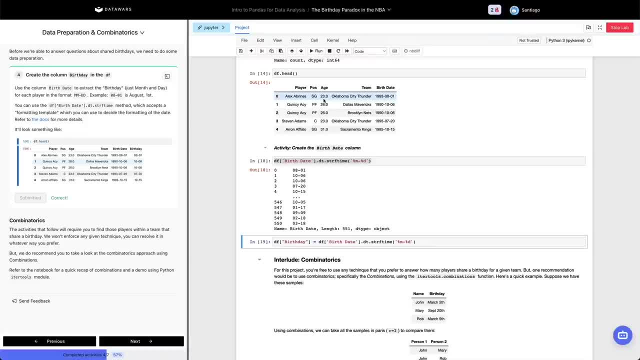 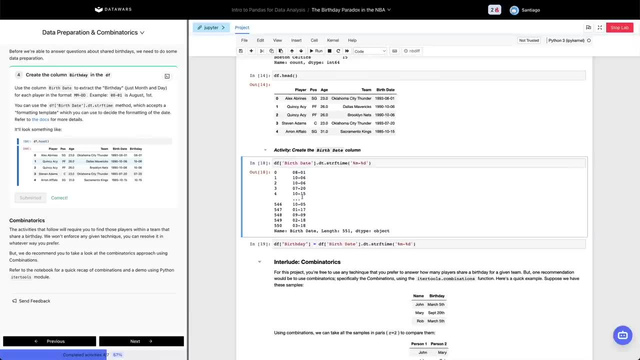 ones that um share the given birthday. We could potentially Think about these problem in different resolutions, For example finding duplicates within a team doing group by operations. but those are all, at least given the the, the project we're solving now. things are a little bit. 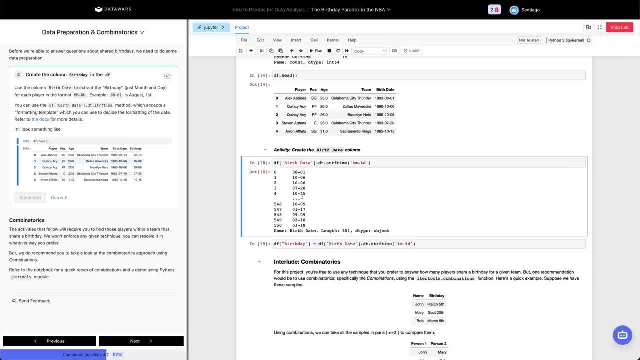 more advanced And, basically, what I want to communicate with this particular project is that sometimes we can find clever answers, clever solutions that will pretty much give us the same results, And the one we're going to do here is we're going to use combinations. 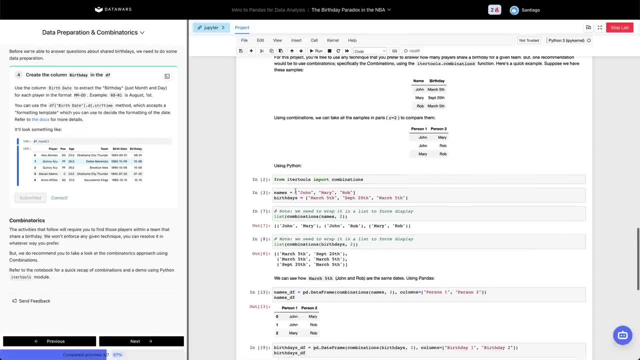 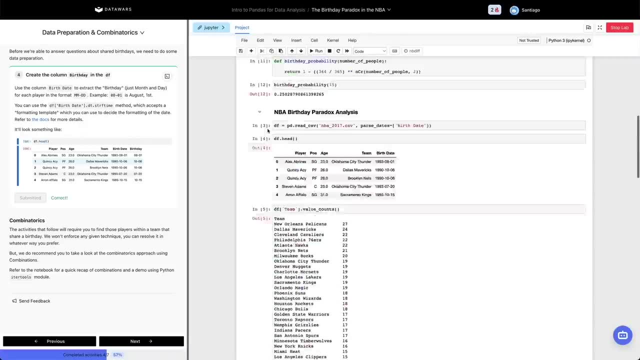 community targets to pretty much solve the same problem. And here we have an example: Um, we have the built-in combinations uh formula and we have something built in. We didn't have to actually write the one we did before, but just for the sake of the example, we did it. 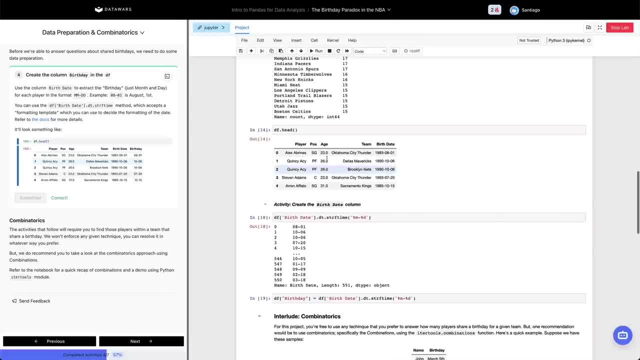 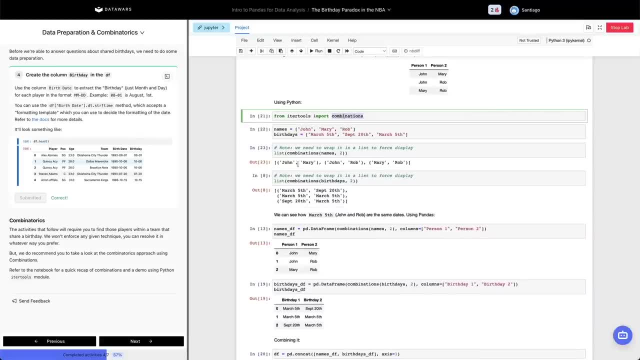 And here the way to think about it. forget for a second about the NBA players. the way to find these people matching Is: first: we're going to use this combination function, but it does. it puts it aligns combinations within a given collection. 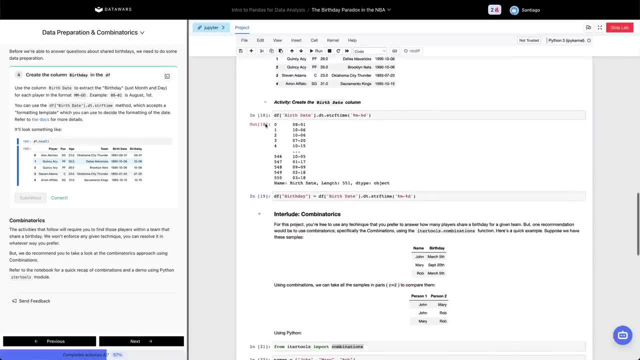 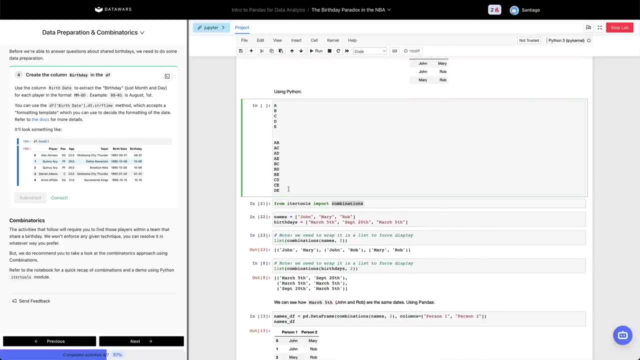 So the same thing we did here with our people. So combinations, right here this thing. So remove F and G. There you go. It's going to put a with B, a with C, a with D, a with E, B with C, et cetera. 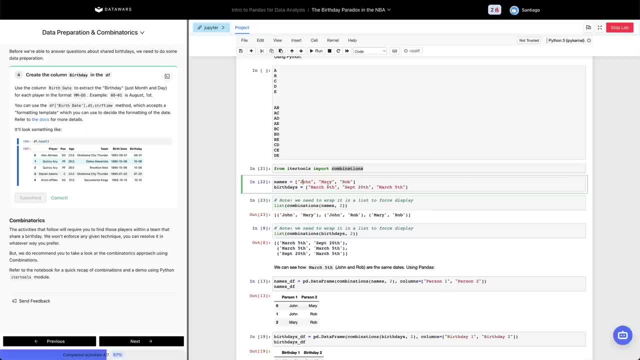 It's doing the same thing here: John with Mary, John with Rob, Mary with Rob. We can Add someone else, We're going to add Susan, we're going to add Violet and we're going to add, and then we're going to do as again: John, Mary, Rob. 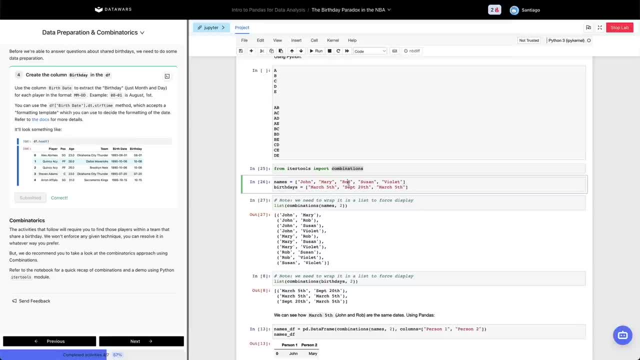 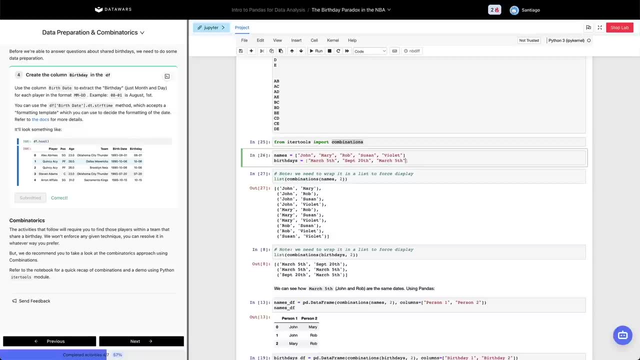 Susan Violet, Mary Rob, Susan Violet, Rob Susan Violet, Susan Violet. Those are all the combinations, And then we have all the birthdays. So let's add two birthdays, Let's add on July 20th and let's add um. 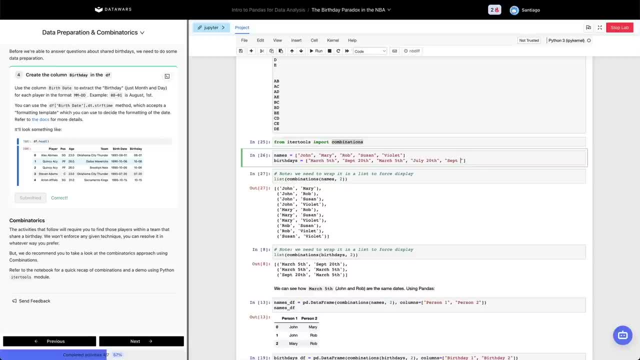 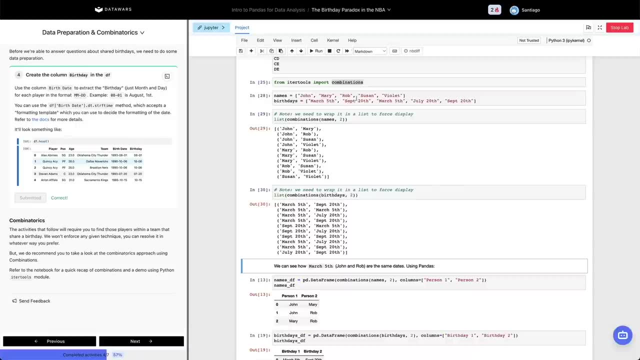 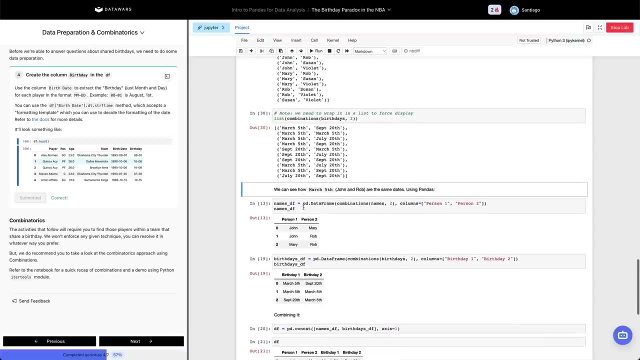 September 20th. So we have another repetition. There you go. It's going to do March 5th, September, March. It's going to do the combinations again, And then what we can do is we can put together these things with a little bit of pins. 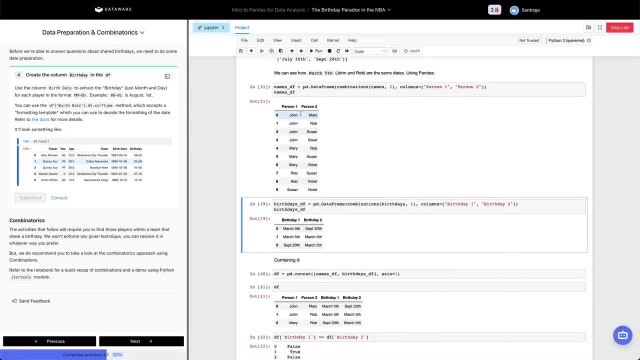 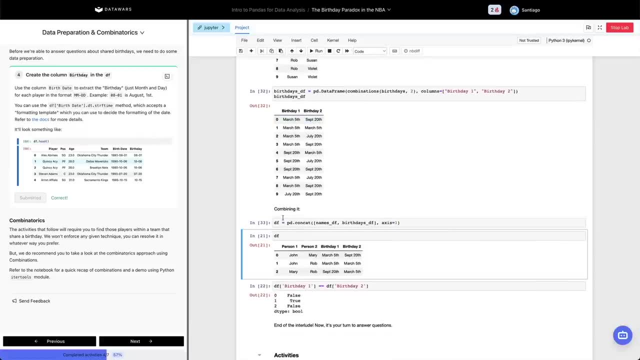 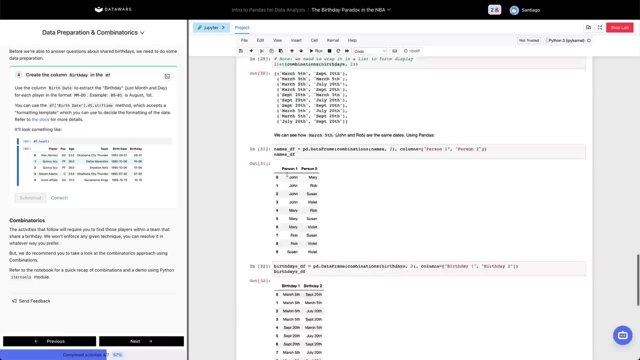 We can create these separate data frames aligning these people and aligning these birthdays, and then combining them all together with this simple operation. Oh, and I just realized that I have overwritten our original data frame, but it doesn't matter, We'll have to read it, reread it. 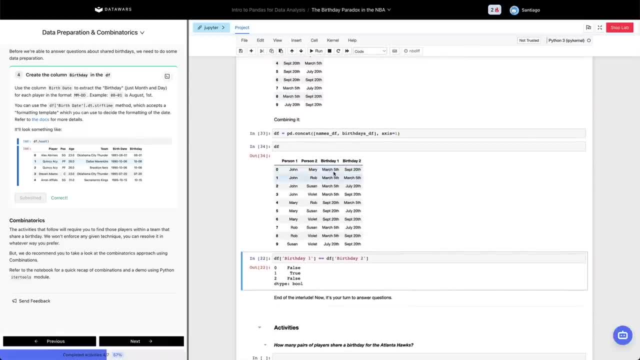 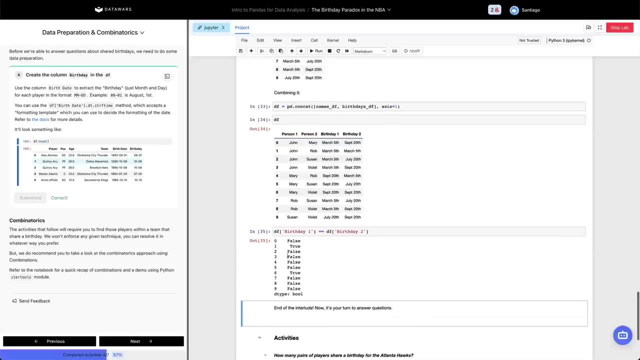 Um, and now we have all these combinations of people, their birthday, and now we can just ask which ones of these people are matching. And we have that one and six are matching. So one is John and Rob, because they are March 5th both of them. 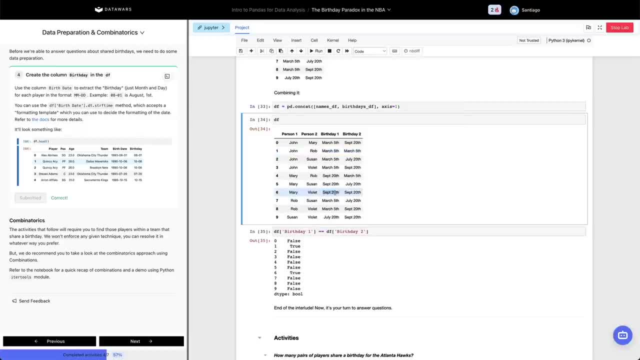 And six Is Mary and Violet, because they're both September 20th right, And we can apply the same reasoning, the same solution for our NBA data here. What we're doing is we're not doing any group by operations, We're not doing any algorithmic nested for loops that could potentially work. 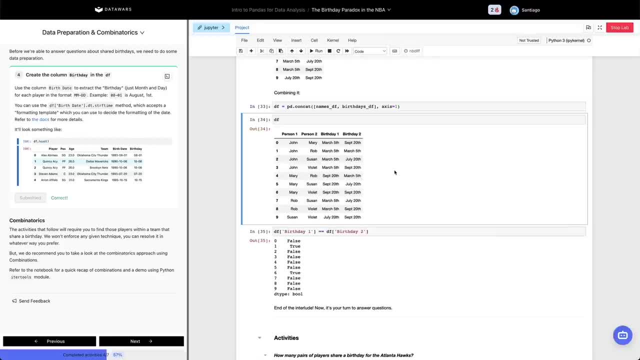 What we're doing is we're being very smart and using combinations to reshape our data. We're going From- let me do a little bit of a drawing here, if you allow me. we're going to do- we go from a small data frame with uh one, two, three, four, five people were reshaping it's. we're creating these long formats with all the different combinations. 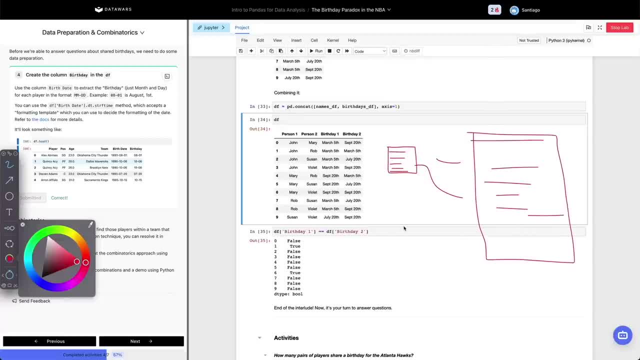 And now we don't need to algorithmically like iterate this thing over and over and over again. We can just answer data by finding Chunks here. How many which um combinations here are true? in this case It's a one. no, I'm not good drawing one. 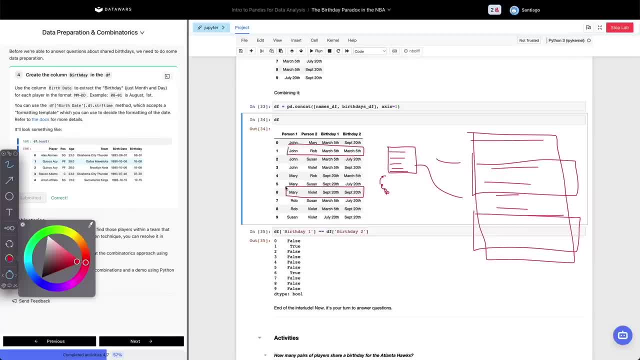 And six. what I'm saying again- and we're going to move forward in just one second- is: sometimes you need to work smart. You need to understand your data, reshape it, be creative in the way you work with your data to resolve the problem. 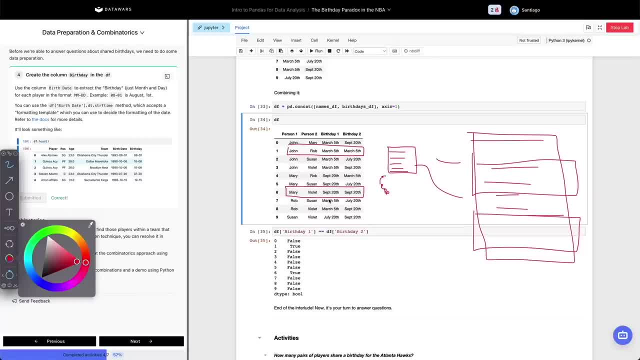 And there's going to be a lot more scalable than think it Algorithmically Because, trust me, when you start working with big pieces of data, these solutions that are more declarative are going to be more scalable than algorithmically. We cannot paralyze an algorithm. 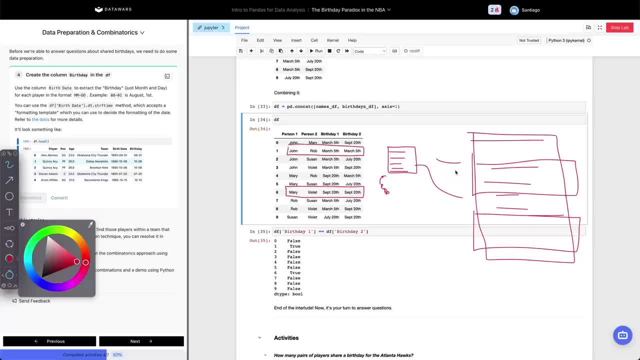 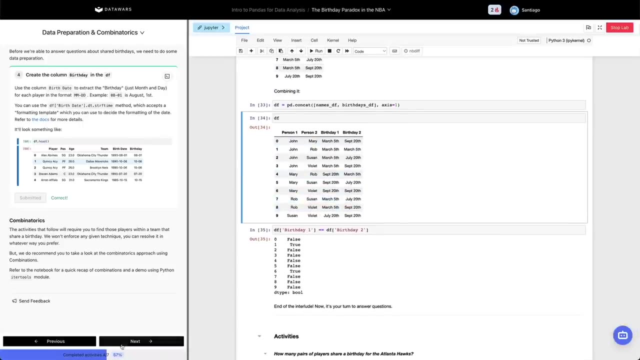 We could potentially break this thing. Imagine you're working with millions of records. You can put this thing into different servers and check it in parallel. That could be completely possible. but anyway, I'm. I'm getting ahead of myself and we're going to work now by solving the activity. 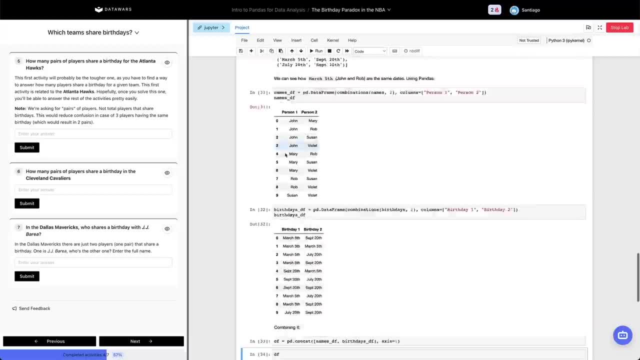 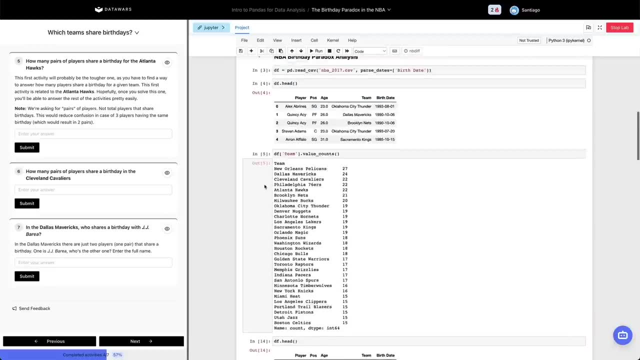 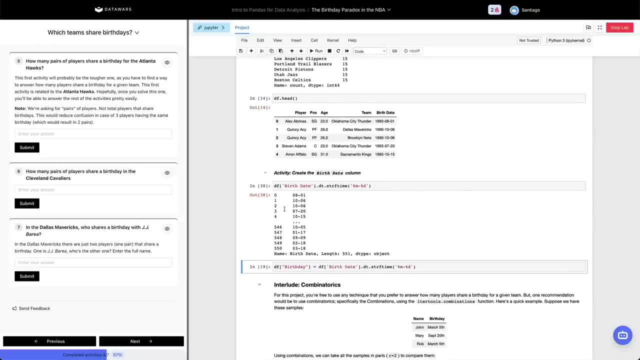 That we are asked in this particular project. So, as I told you, I am stepping over this data frame, I'm going to re-read it again- Where is our data frame right here? And we're going to recreate our birth date um column. 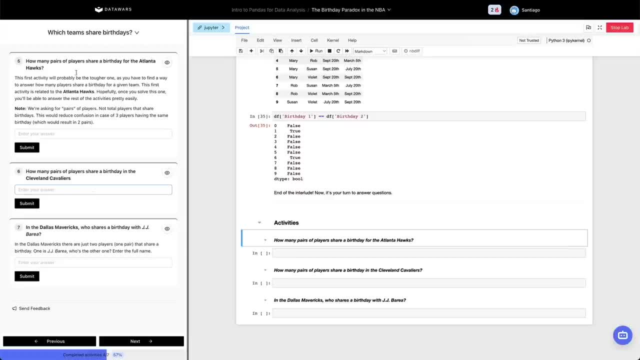 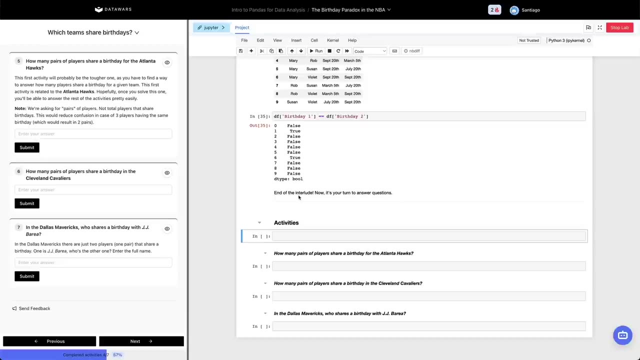 There you go. We're going to go straight to the activities. How many pairs of players share a birthday for the Atlanta Hawks? And again, we want to use the same solution as before to do so. The first thing we have to do is to um only get the players from the Atlanta Hawks, because we don't want to compare every player with every player. 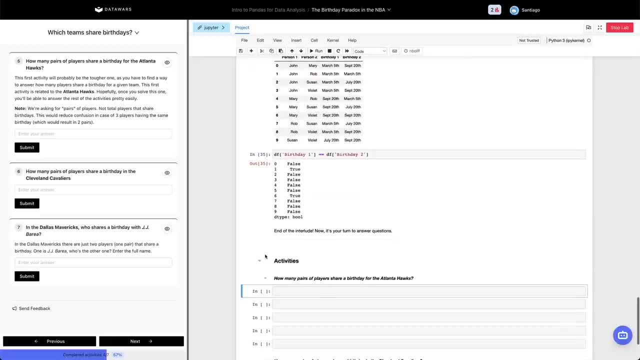 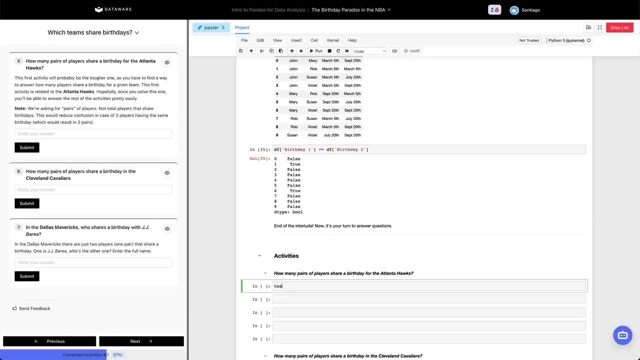 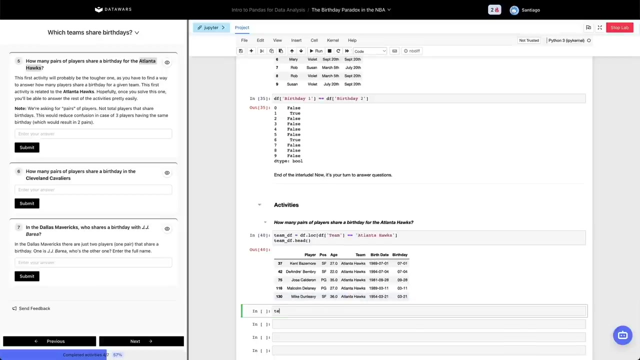 And it's going to be like a huge number, right. So we want to get, uh, we actually have, um, the number of players in the Atlanta Hawks going to be- let's put it in a, in a Variable. it's going to be dflog, dfteam equals. uh, let me copy directly from here and that's: we have teams, dfshape, we have 22 players. 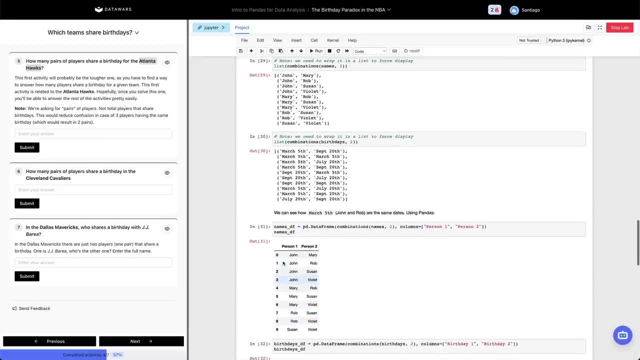 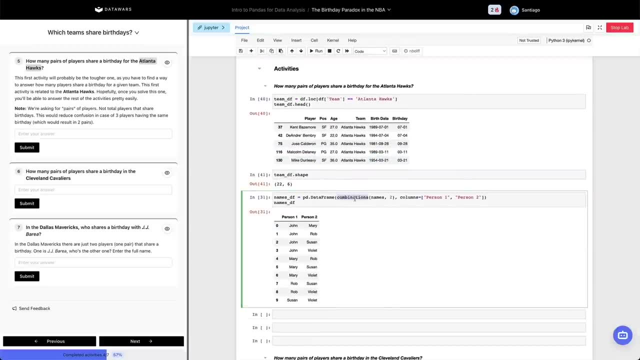 So now, what we're going to do is pretty much the same thing we did before. Um, I'm going to do. I'm going to copy this thing. I'm going to paste right here. I'm going to do: instead of combinations of names was a variable we defined. 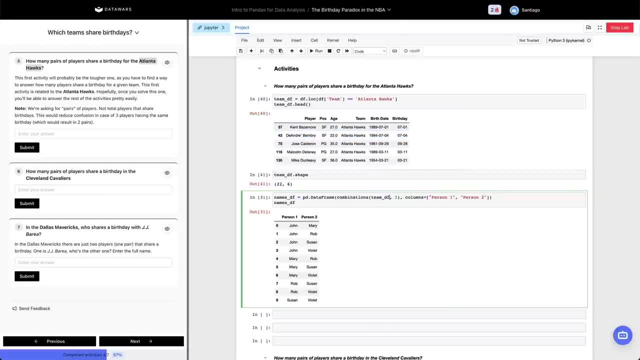 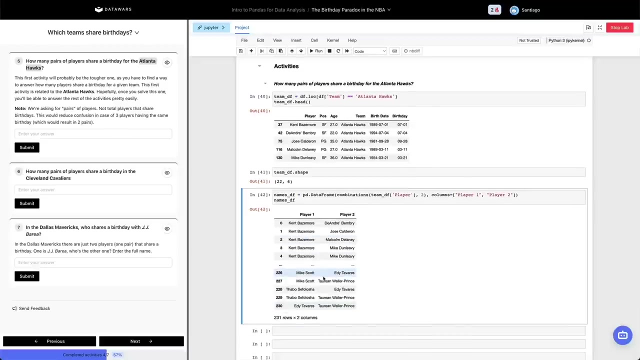 What I can do is just do team dfs at um, team df at uh player Here. I'm going to put player one and player two. There you go, And I have the correct resource. One interesting comment here: completely on the side of um, we were QA'ing this project with someone that's resolved the project and make sure that the quality is good. 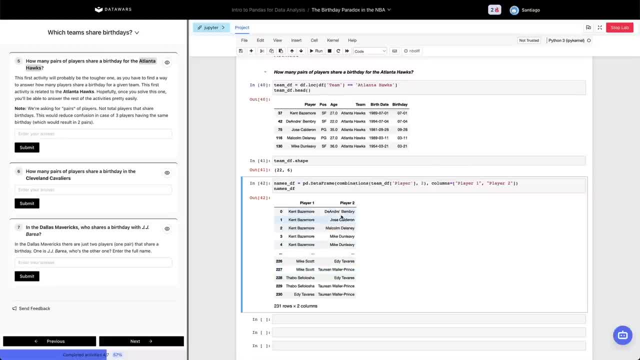 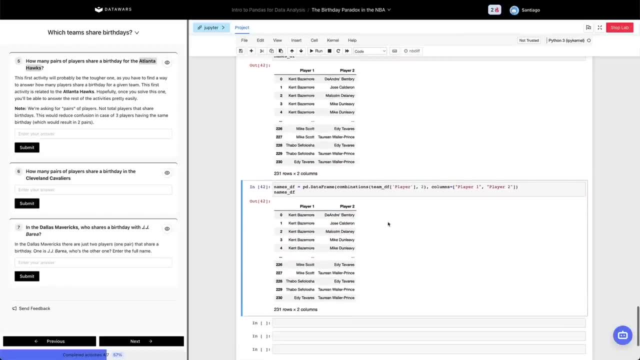 There are no errors, And this person was finding an error and saying: I have too many. I have too many names, Right, Um, and I don't know what's going on. And it was a very impressive like problem that the person was using df instead of team df. 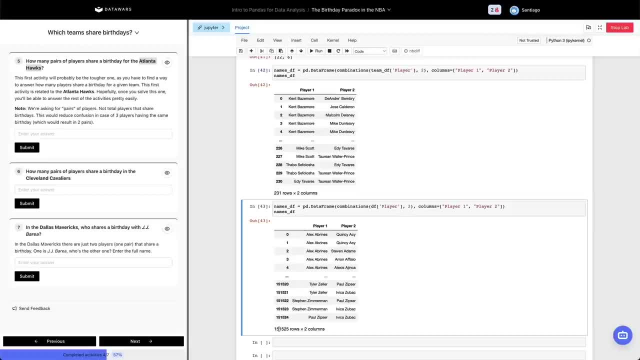 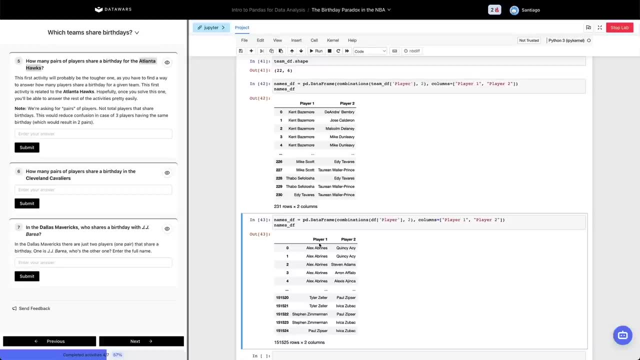 And it said like: Okay, Like I have, is this possible? They have 150,000 rows. And this is an interesting piece because it's like you have to kind of understand the big range of data you're working with, Like we were. we were working with Atlanta Hawks and we needed to create these combinations of players. 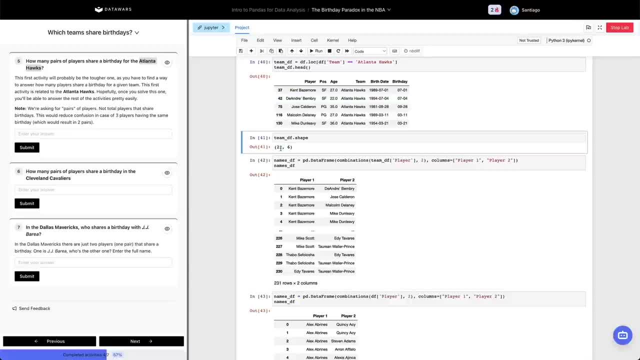 And we need to. we have 22 people in Atlanta Hawks. how many combinations of pairs you can create, And this is It's important to understand, to have a range, a quick ballpark estimation of what data you're working with and what should be the result. 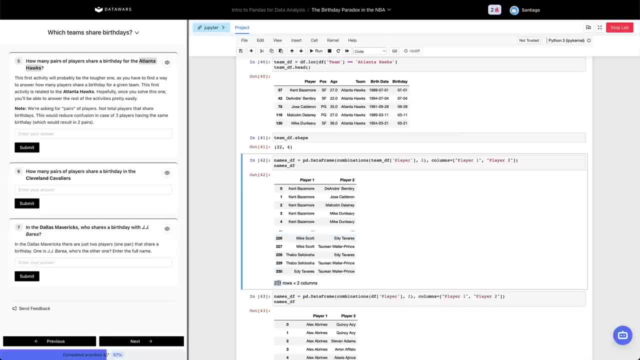 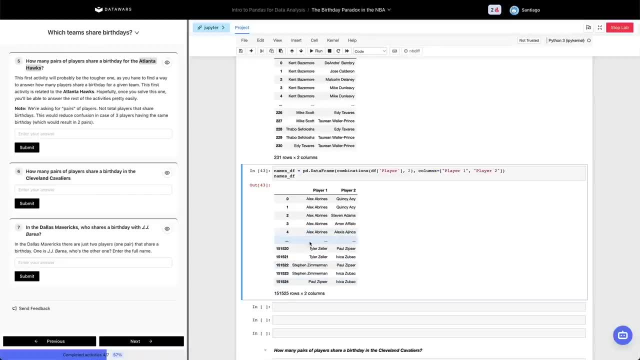 Because I honestly don't know if it's 231, but I do know that 100,000 is too much. It's definitely too much, way too much. So this hints is like understanding the data you're working with is kind of quickly gives you an understanding that there is a mistake in something you did right. 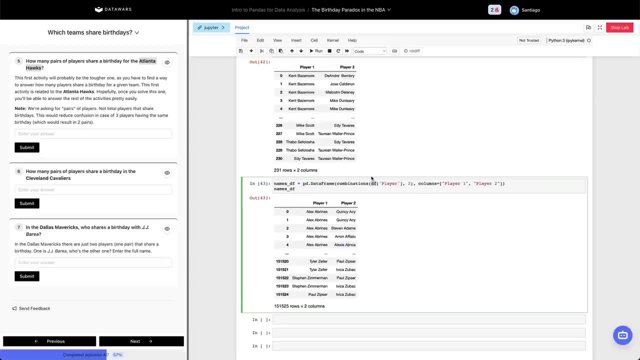 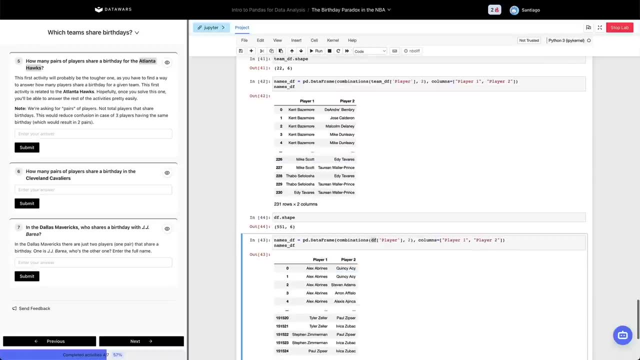 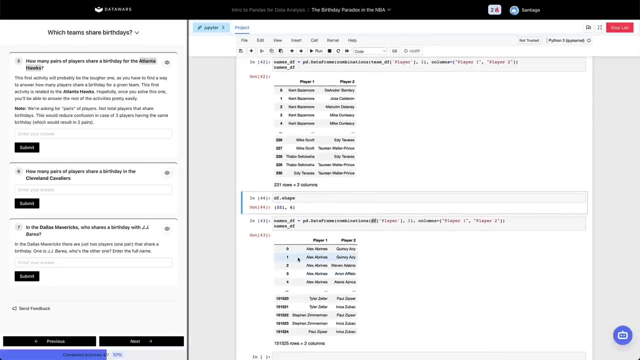 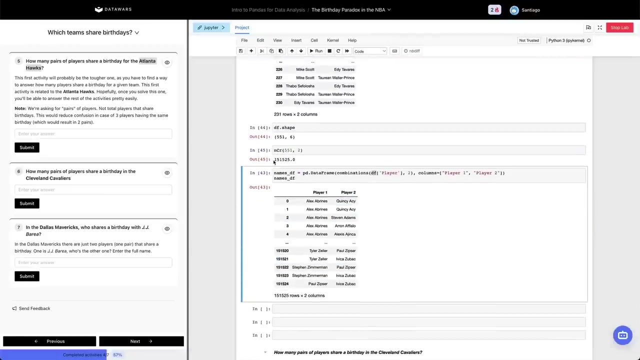 So if, If you forgot, you were filtering by the Atlanta Hawks and you wanted to create pairs of only these 22 players and instead you created combinations of 551 players, that number grew by a lot. We actually have our formula NCR of 551 taken by two is the same number: 151,525.. 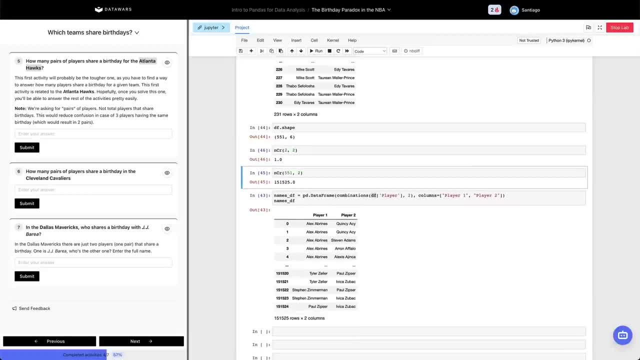 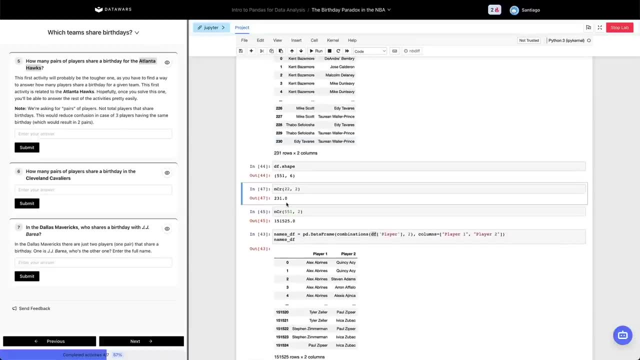 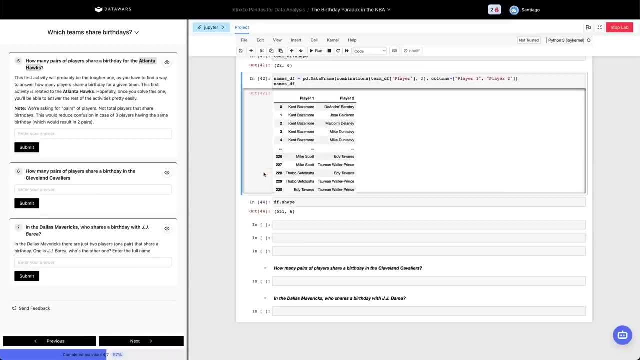 And NCR Of 22 players. 22 players in the Atlanta Hawks give us 231 rows, So this makes a little bit more sense. So anyway, just a comment on the side. I meant is like again having understanding data we're working with. 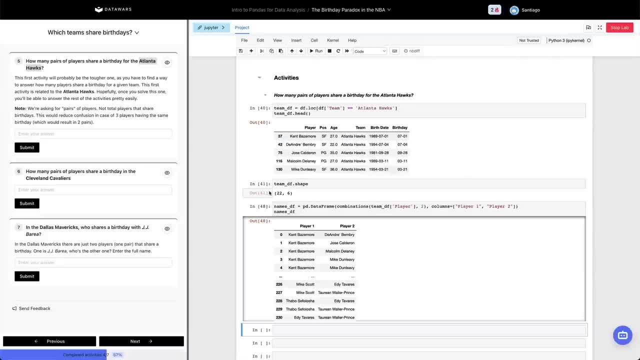 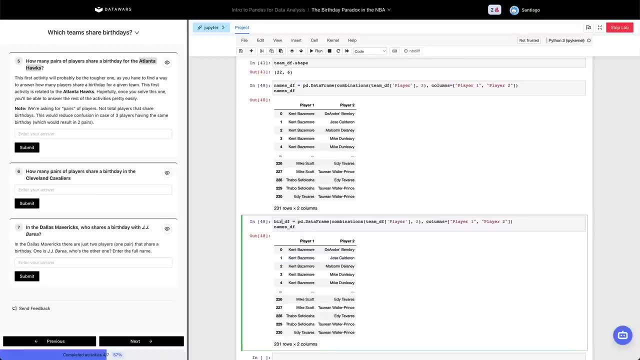 So let's go back rerun this thing. The name's DF And we have the 231 rows. I'm going to do the same thing for the birthday, Birthday and, And the birthday Here, and this is going to be birth day. 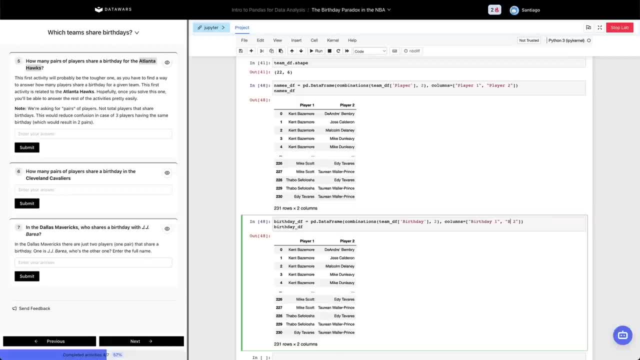 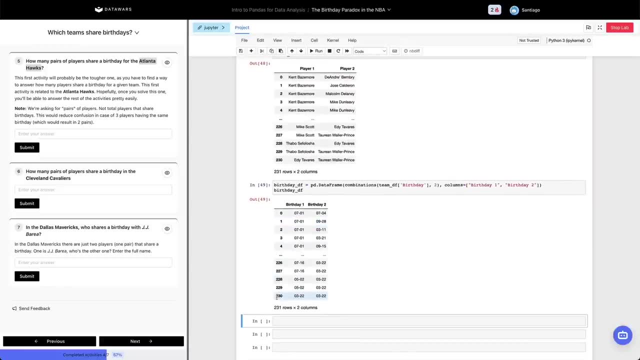 And here we're going to do: name it birthday one and birthday two And finally we're going to put, by the way they are aligned, 231, 231.. We're going to combine them with the same concat operation we did before. 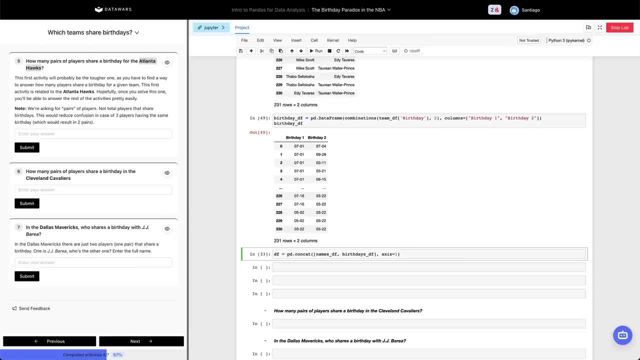 I don't want to overstep the name, So I'm going to do check DF and the names and birthday. And now let's take a look at our data frame. We have the combination of the player and the birthday of each one of the players. 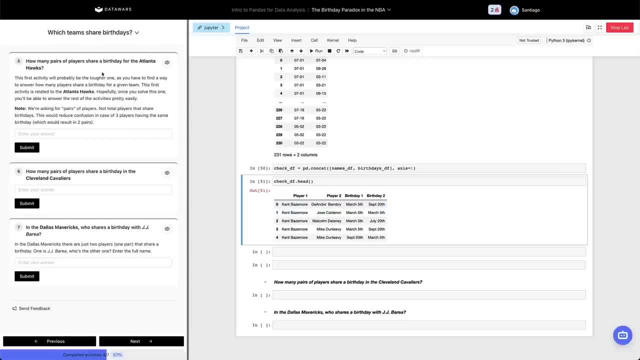 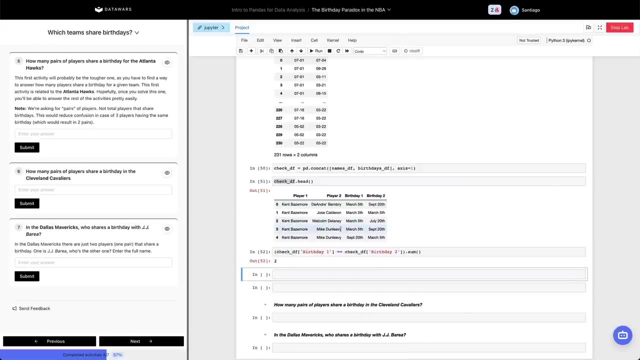 Now we can ask the question: how many pairs of players share a birthday, for the plan The Hawks are going to do is a birthday. One is equals to birthday too, And we're going to sum this whole thing, It seems like there are two players. 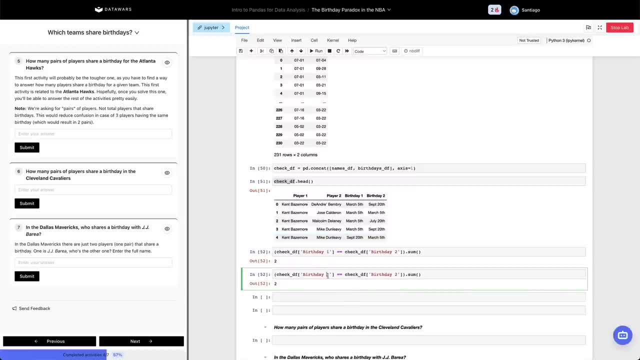 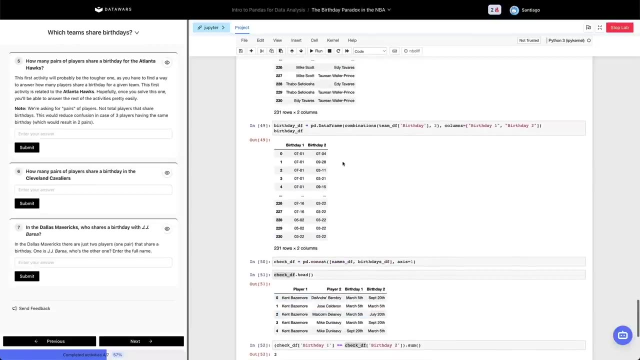 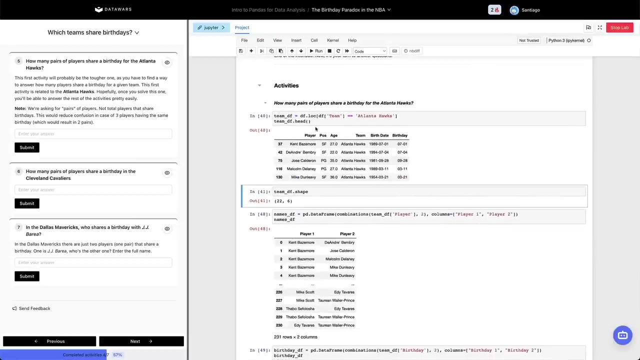 And then what we're going to do is dflock this thing. No, check the air. There you go, We have these two players. So team DF: Let's see if all the variables are correct, because I might have done something wrong here. 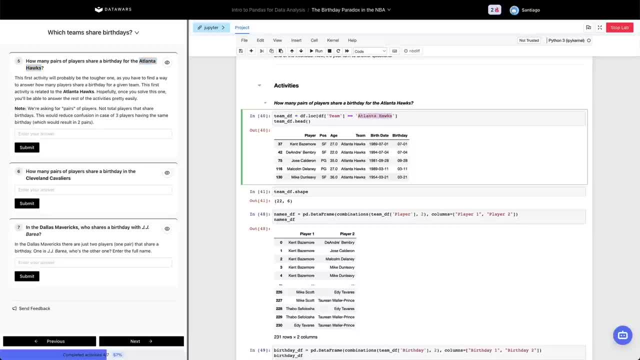 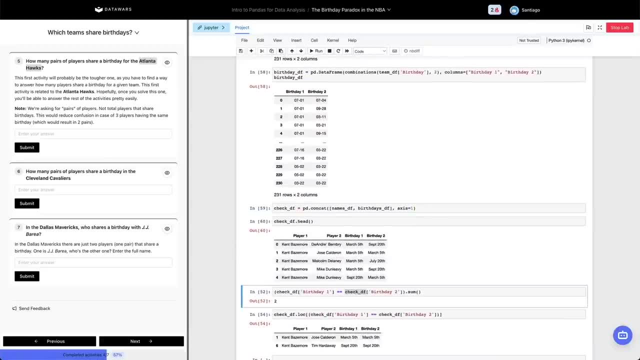 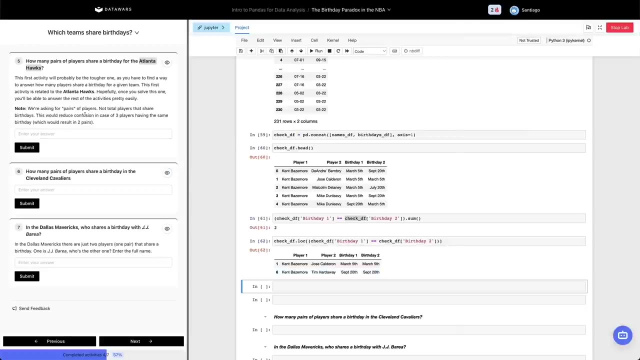 Quick recheck: team DF. Okay, Okay, Okay, Okay, Okay, Okay Okay, We have birthday Check DF And we have two players, Two pairs. Let's go ahead and try the answer. Two players there, Wrong answer. 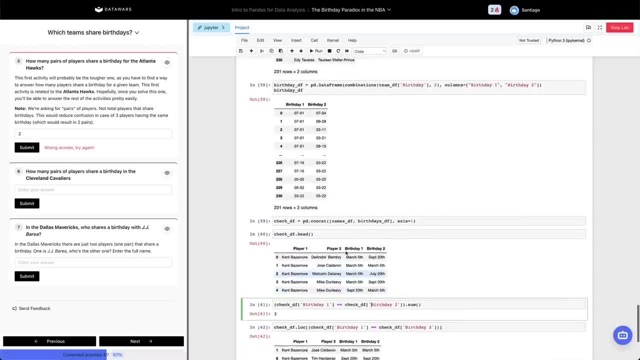 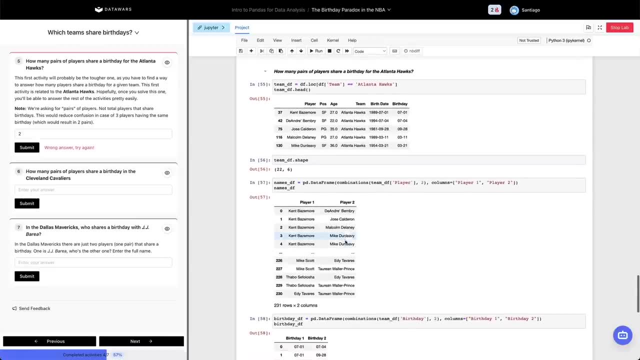 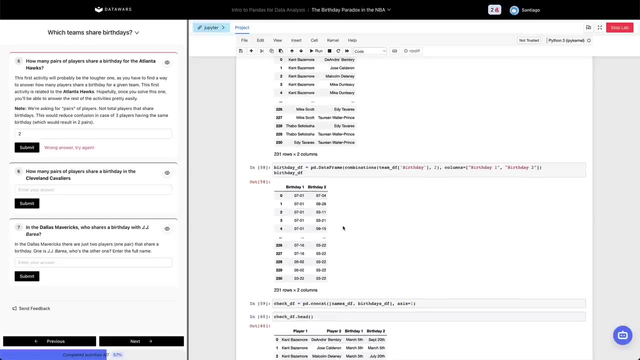 Try it again. Let's go ahead and recheck our thing. I don't want to overstep the name. I want to make sure I use the rock team and then we have the player and the. oh, this is a very unlucky mistake. it's a very unlucky mistake for sure. 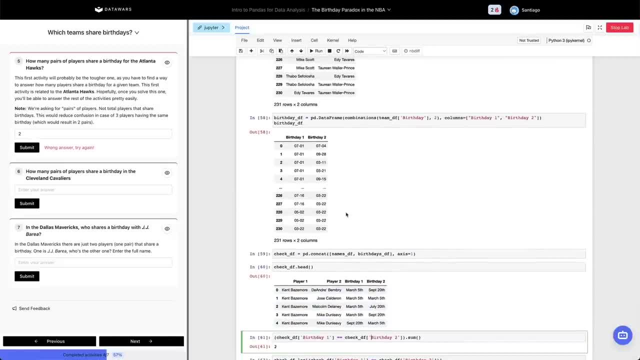 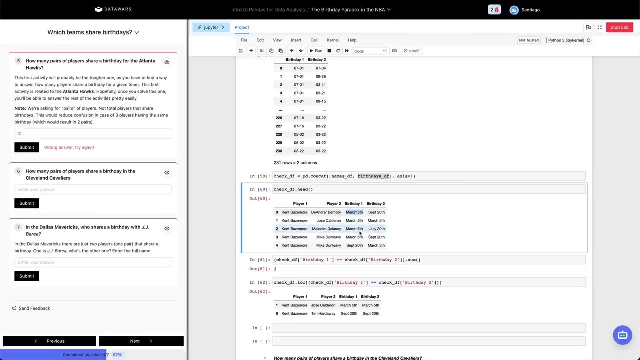 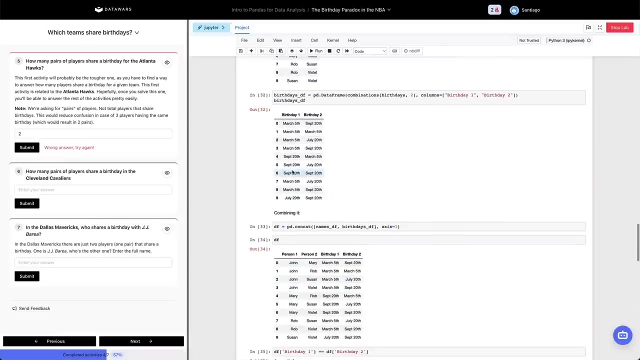 what I'm checking right here is birthday and using birthdays and check the dates that we have in this particular point. this is just bad naming on my side. I used the, the old data frame that I used for the sample, and the dates are in this format. that is September 20th, whatever, and I just 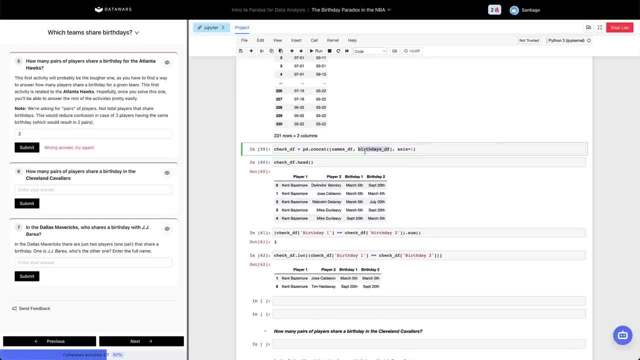 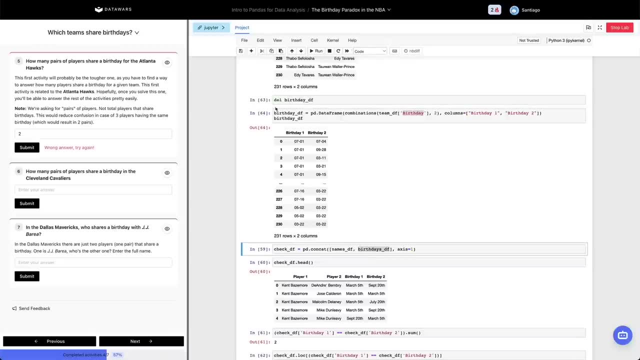 recreate the data frame that I used for the sample, and the dates are in this format. that is this thing for the entire data frame. so my mistake, let's go ahead and delete birthday df and delete it, and we're going to use this variable name now and try to recheck it. 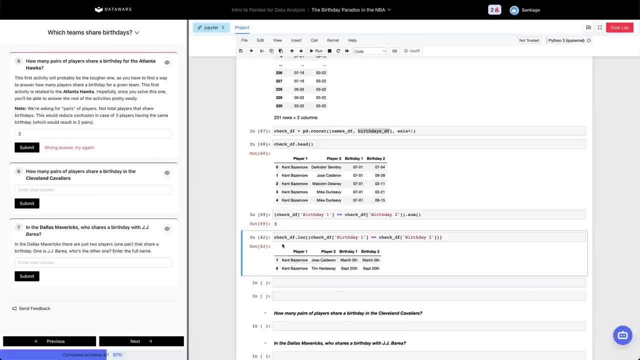 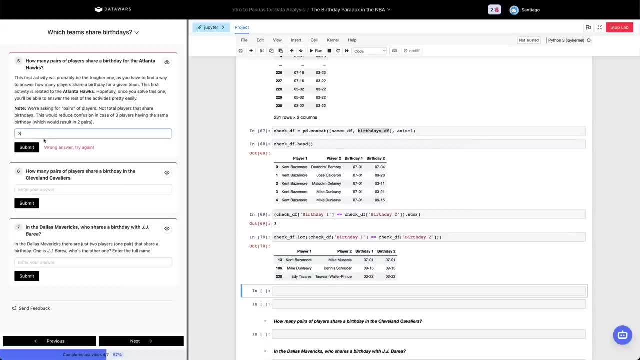 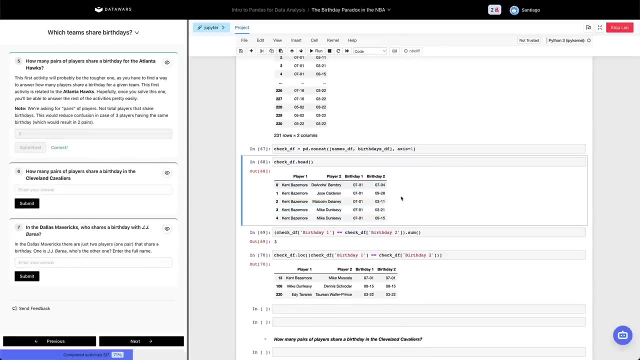 and seems that we have three now and effectively we do have three people. let's try it out now and see if it works. now it works, it's again. the previous mistake was just using bad variable names. I should have used something like testing a combinatorics, birthday or. 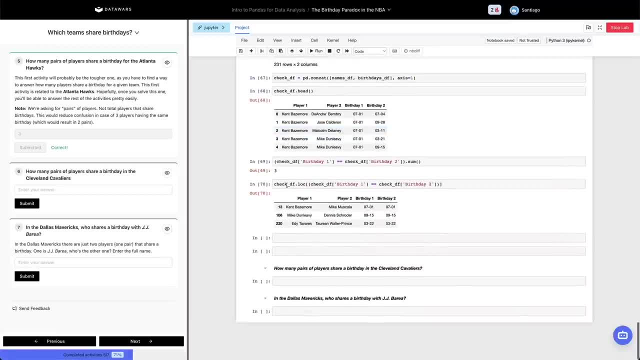 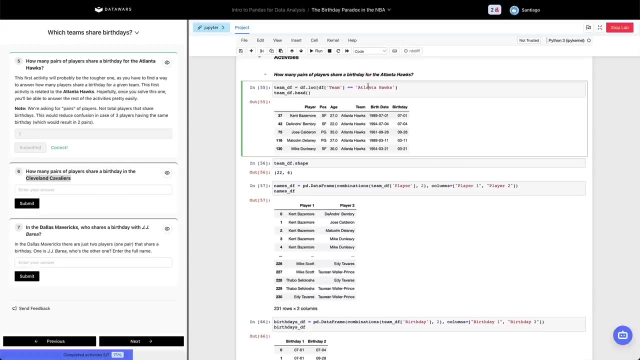 proof whatever, instead of the real variable names, but we have just fixed it. how many pairs of players are birthday in the Cleveland Cavaliers? so this is pretty much the same thing we did before we're going to. we're going to change the date. we have 22 people. it's going to be the same probability. 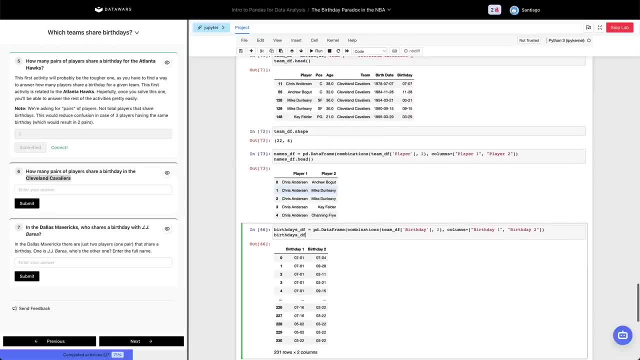 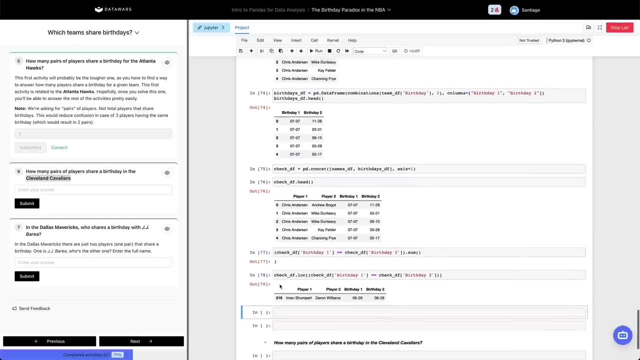 as in that now we're going to do that now and we have only one pair of players that share a birthday that's going to be june 26th, so we're going to just one pair and that worked. and finally he says kanji is lost, so we're going toPC. this equation here means if this right here. 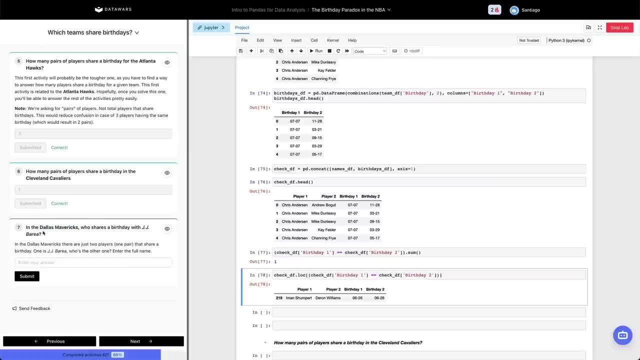 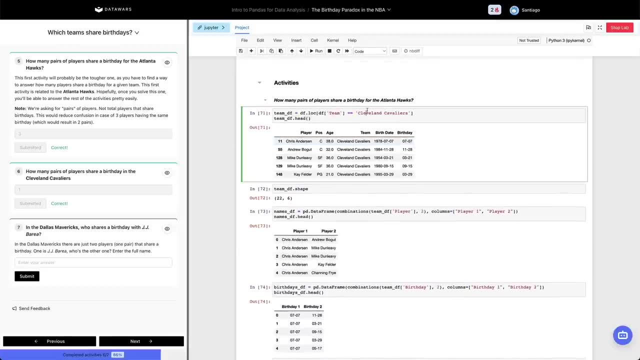 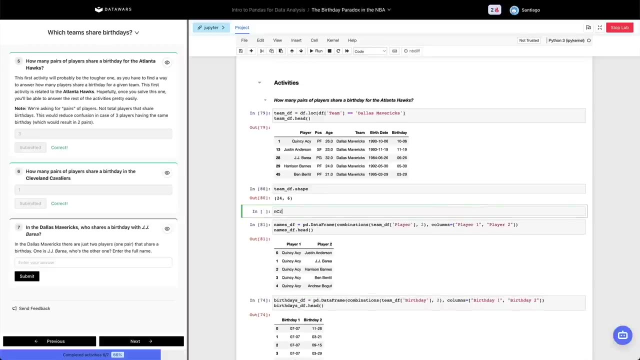 Finally, we got asked in the Dallas Mavericks who shares a birthday with JJ Borea? What we're gonna do is rerun our code. I have 24 players. What is the probability here? NCR of 24, NCR 24 taken by two. 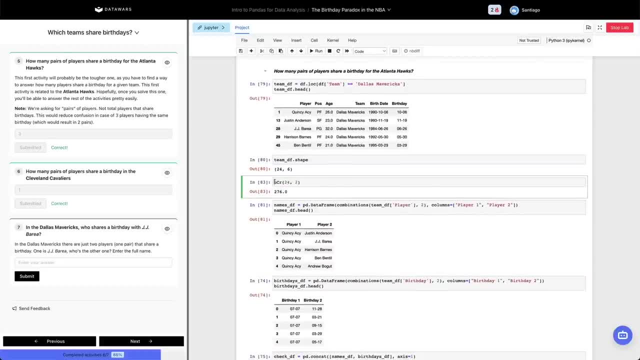 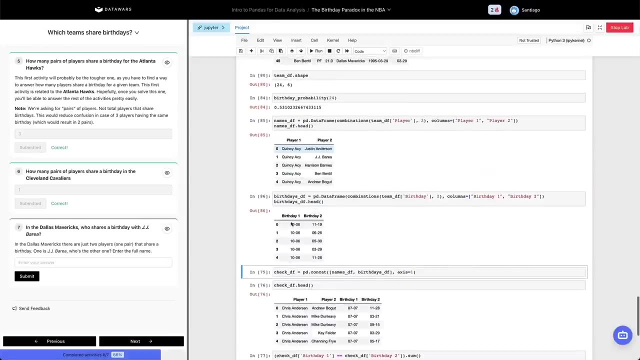 And we have 276, 276 combinations. No, we actually wanna do the birthday problem There. we have a 0.53 probability of two people sharing a birthday. Let's actually go ahead and do it, And we have one shared birthday. 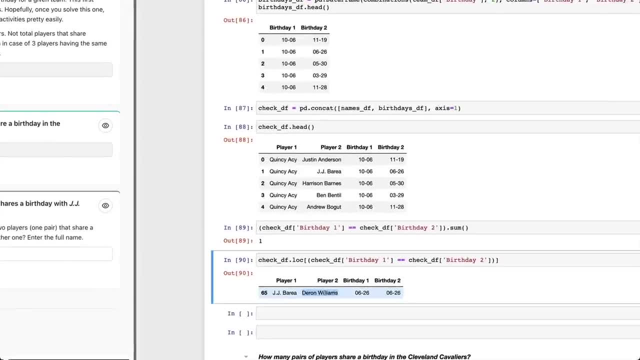 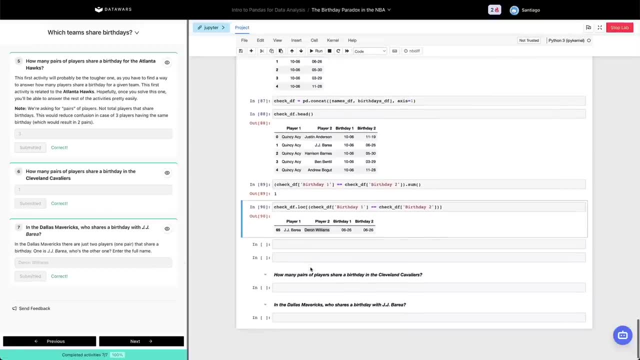 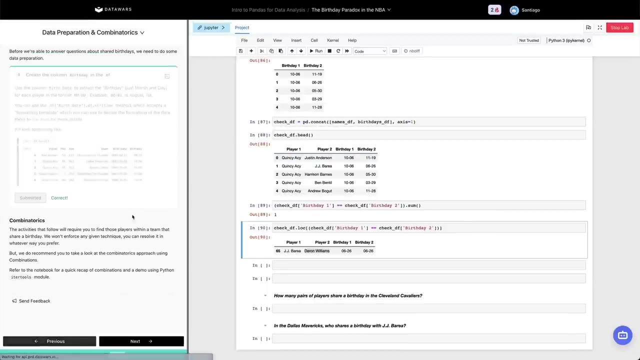 and it is JJ Borea and Deron Williams on June 26 again, And that is the final result. So anyway, a few things we saw here. I think it's pretty interesting the way we have solved the project without using any algorithmic imperative. 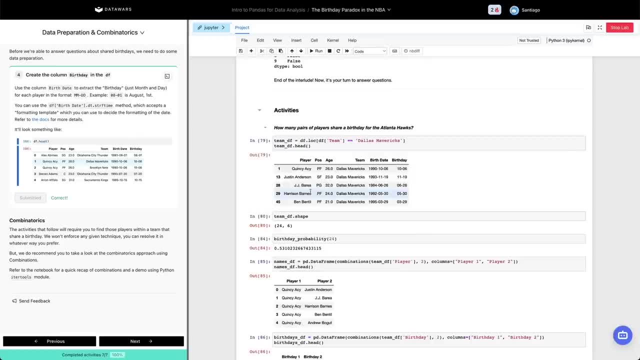 and nested for loop solutions. We used a data driven approach, thinking about how we can expand this data kind of a map, reduce sort of solution that I think scales pretty well. And also I made a few mistakes- few mistakes that i think were um interesting to see live, um and the fact that we're combining 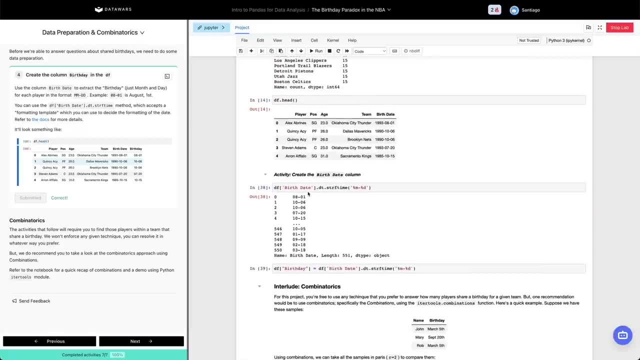 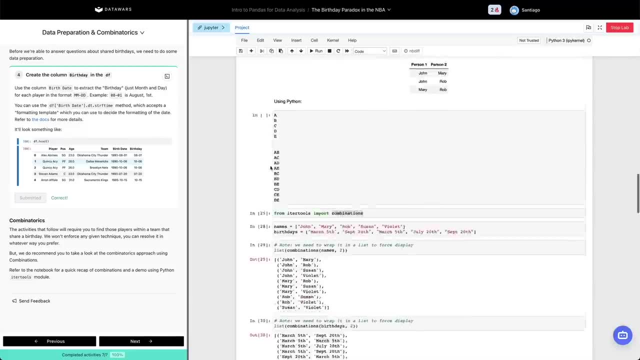 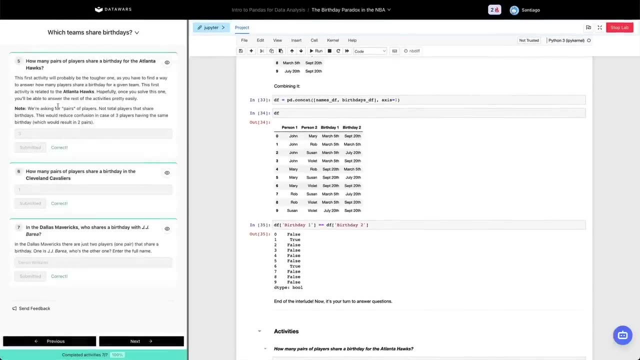 these conceptual things, resolving these conceptual challenges, mixing it with real data. we validated that. this birthday paradox. you know we have two or three themes, teams- sorry, we found it for at least three teams right here: um, atlanta hawks, cleveland cavaliers and dallas mavericks. that. 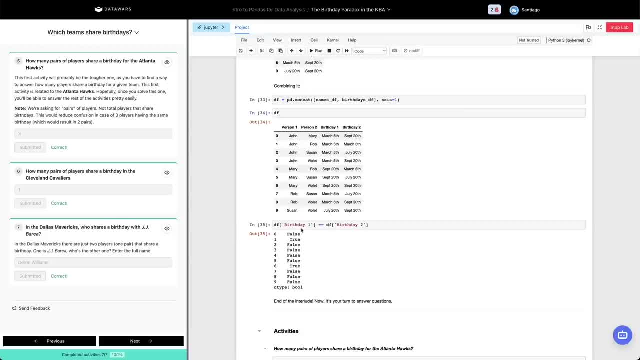 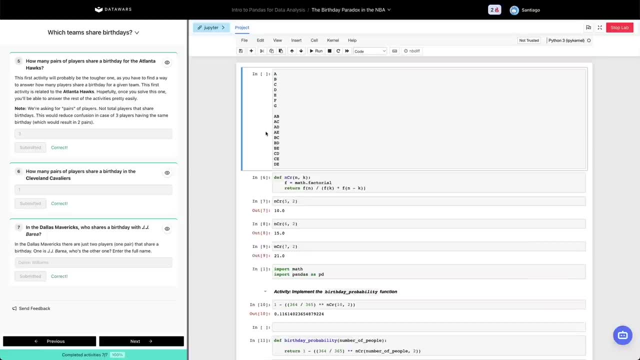 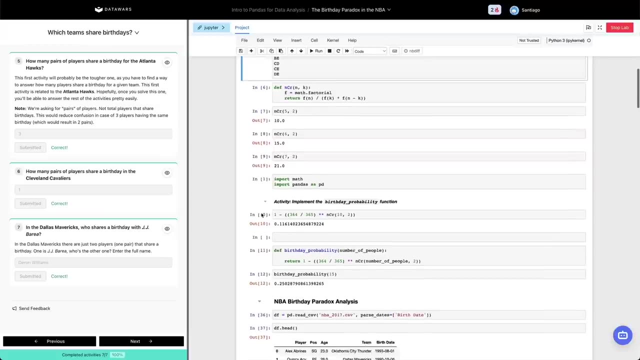 there were pairs of people, pairs of players sharing a birthday, so that that is pretty interesting to see, something that is statistically proven or the probability is, is is high enough. now we see how the resolution in the real data in the world, in the real world data also applies. 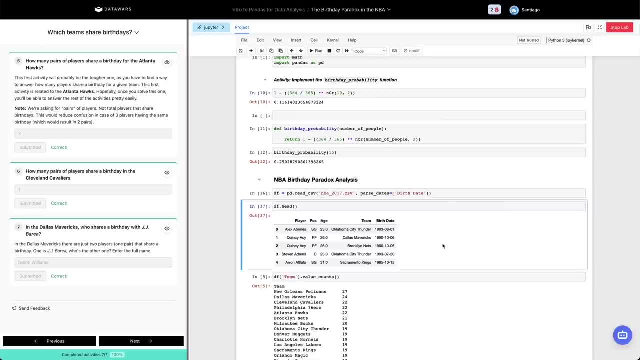 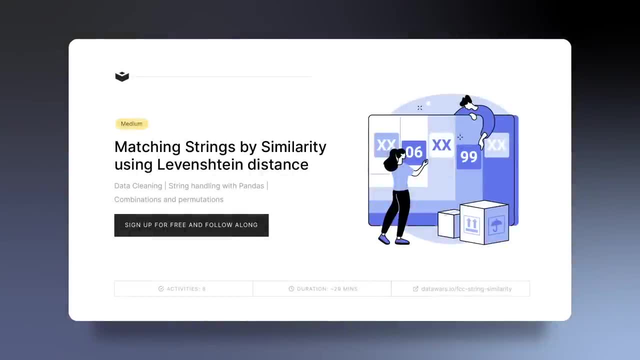 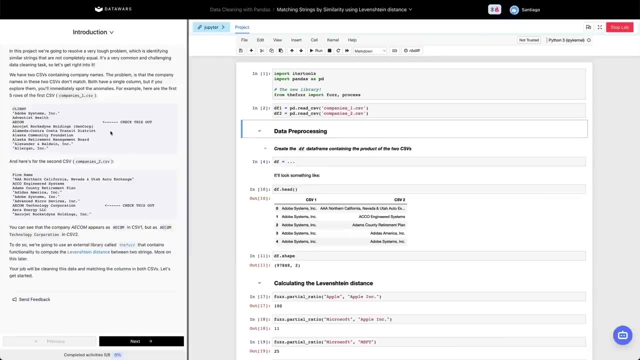 so, anyway, try to take a look at the project by yourself and try to resolve it by yourself, um, and let's keep exploring more problems together. for this project, we're going to be combining our data cleaning abilities with our string handling abilities, and these two skills together are extremely powerful when it comes to the process of 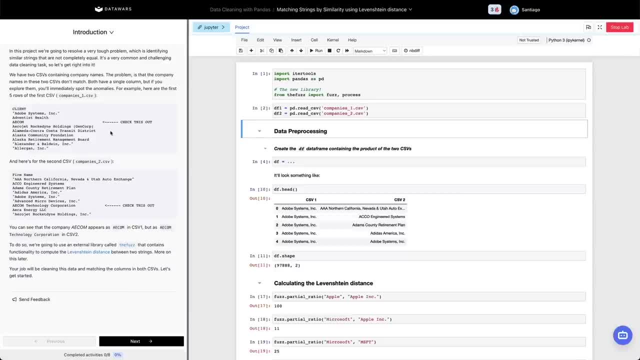 handling data that is coming from the real world. so so far we've done a few projects that had a data was pretty much perfect. we didn't have to do much handling munging of it. but that is not the real world usually when you are collecting data from different sources. 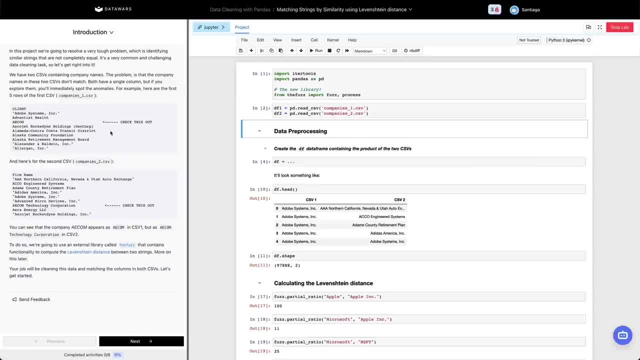 you're pulling it from different apis databases or it's even human generated. we're going to be dealing with a lot of strings and, as those are going to be different sources and humans make mistakes, we are going to have differences between these, these data points, and when strings are. 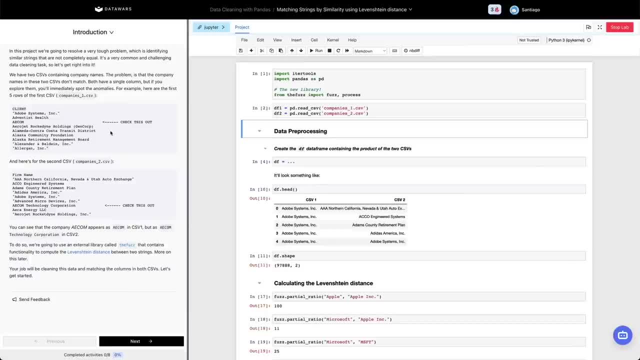 involved, and humans are involved, and multiple sources are involved. the result is pretty much problem. we will always face a little bit of an issue in terms of the data we're working with, so it's very important to have these sharp skills of data cleaning and string handling. 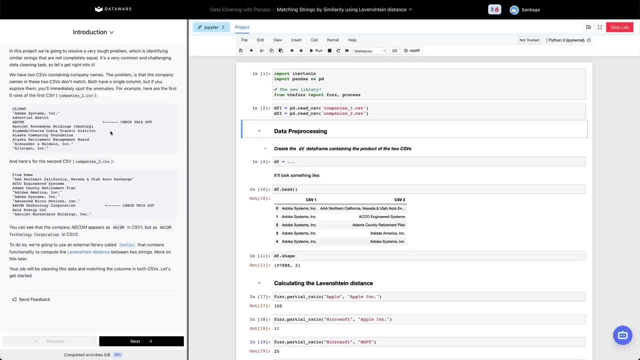 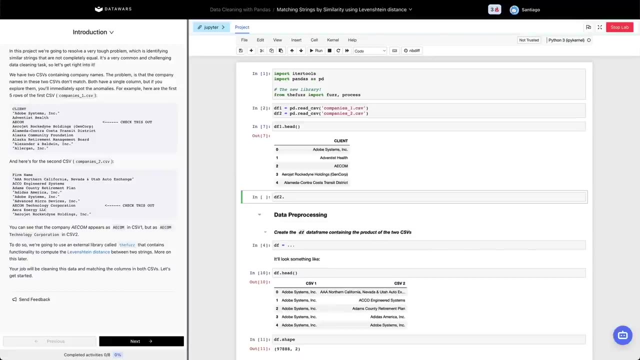 that's what we're going to be practicing for this particular project. let me tell you what we're going to be working with. we have two data sets, that they are explained here, but i'm going to just go ahead and show you the the first few roads of both of them here. there you go and what you're going to. 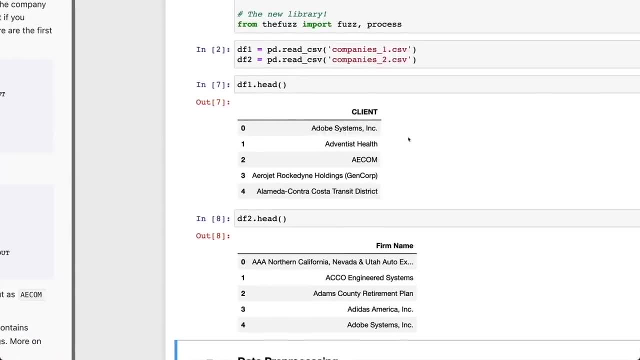 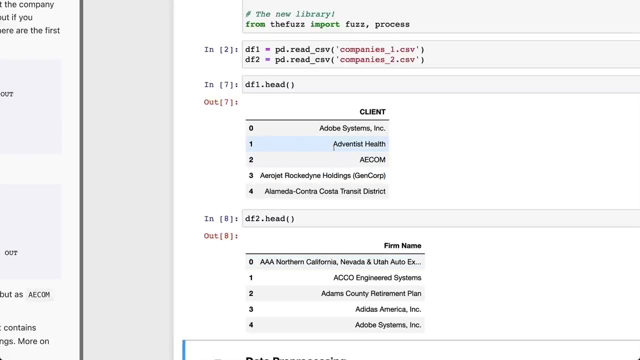 find is that these two data frames, or these data sets that we're going to be working with, are going to come from different sources, but they have pretty much the same information, that is, company names. what changes is that? the way these company names was inserted, input is different, so the 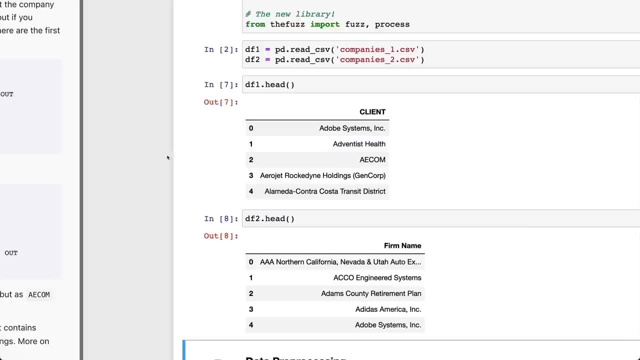 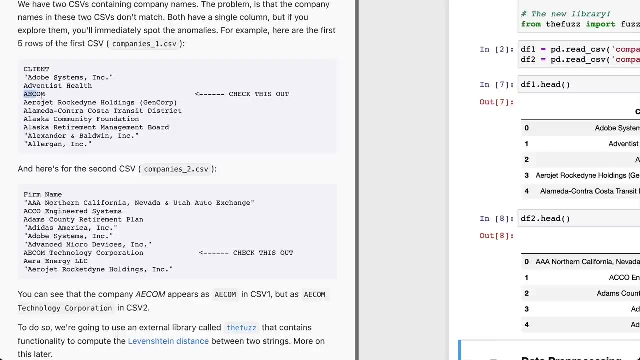 companies by themselves, like the strings by themselves, are going to have differences, but the companies are going to be the same. so in this case we have, for example, from the first data frame, this company is pretty much the same thing as this company, but here has it has a full name and here has, just, you know, a shorthand. so it's. 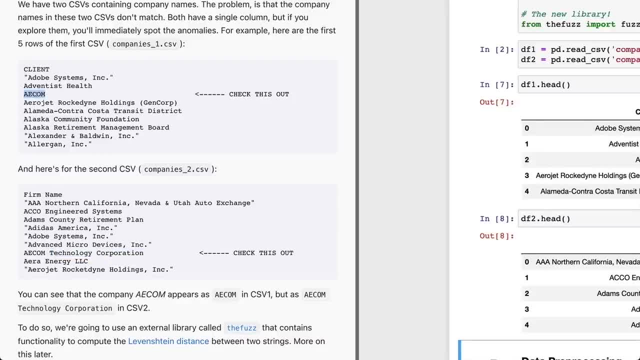 like saying apple. apple is not the real name. the real name is apple inc. dot. right, that's the real string. as a human, it's pretty easy for me to understand that this company refers to this same company. right, it's just pretty basic. but the question is now: how can we make that programmatic? 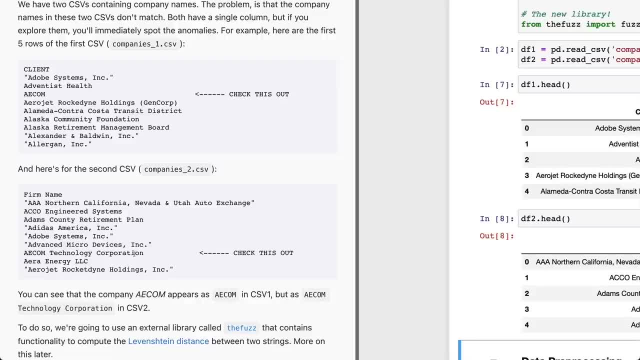 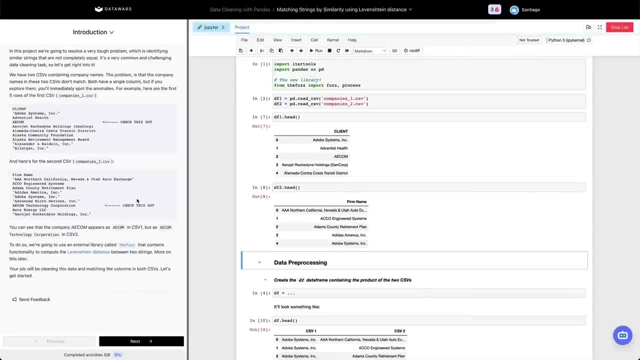 how can we build this sort of artificial intelligence to find the companies that are matching, so we can match the strengths and, of course, continue with our analysis from these two data sources that are coming from different sources? the answer is: no artificial intelligence, yet we're gonna use a. 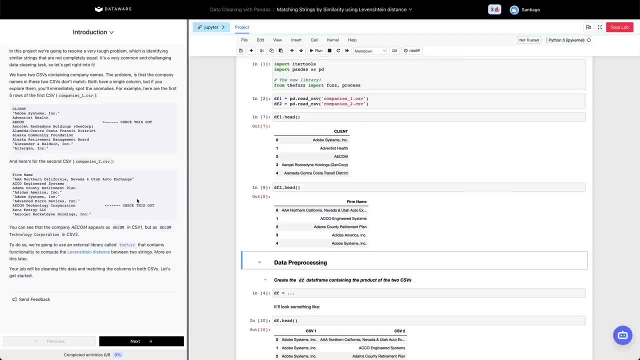 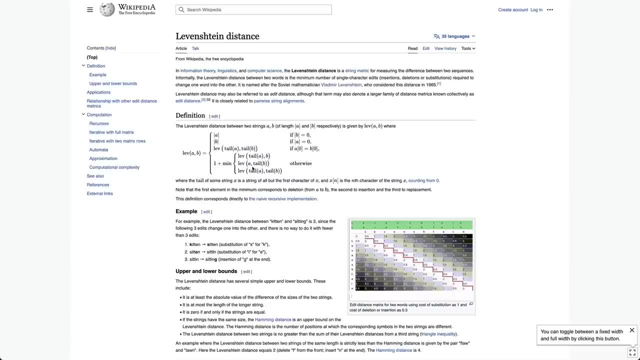 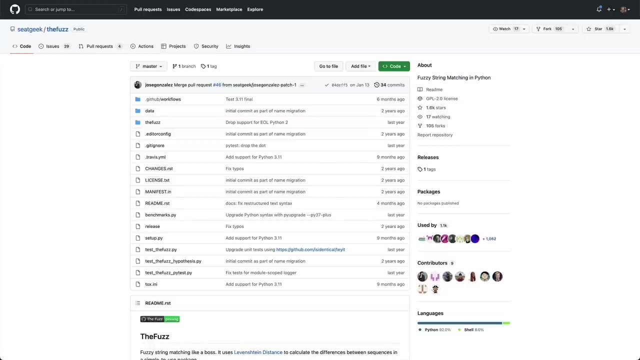 pretty simple, heuristic, uh, this um deterministic method, which is the levinstein distance. it's a simple formula that basically will give you a number on how different two strings are, and the good news is that this distance is calculated. this formula is already implemented for us in a package that is already installed in our lab that is called the. 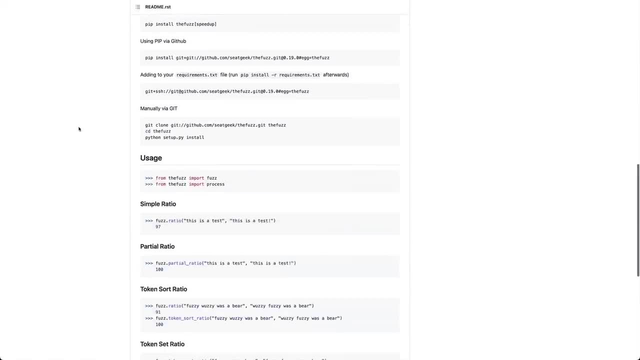 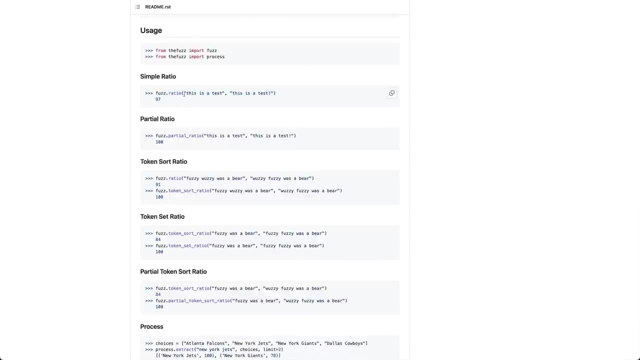 fuzz and the fuzz has a couple of very simple methods. we can take a look right here: um ratio and partial ratio. that will give you kind of a, a similarity or a distance if you want, between the two um, two strings and new bonds. in this case i think it's easier to think about in terms of similarity. 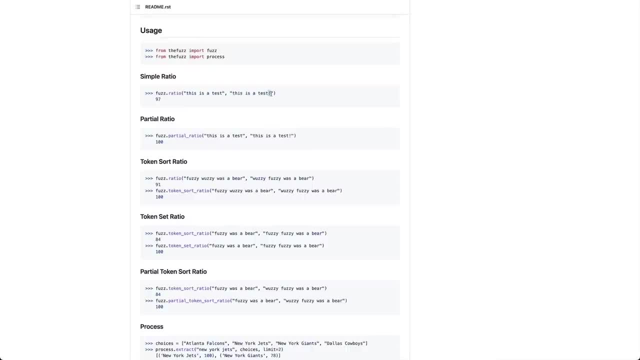 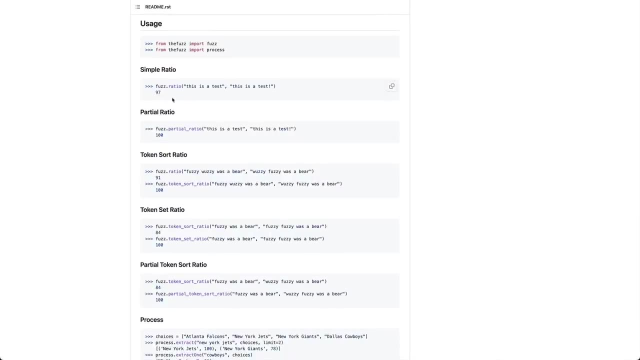 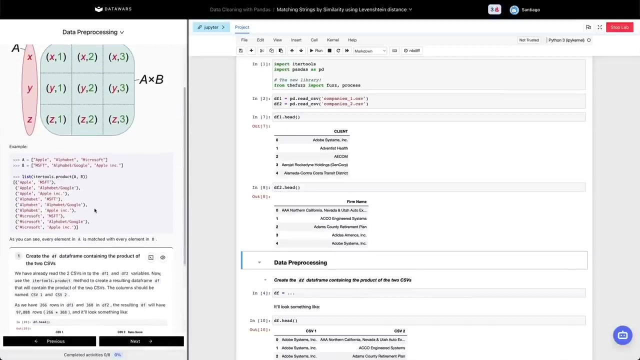 right, so these two strings are pretty similar. the only thing that changes, uh, is an exclamation mark, so the similarity is pretty high- 97.. so, um, we're going to be using this library to compute this distance, so let's move forward with, uh, the first couple of activities and the first thing that we 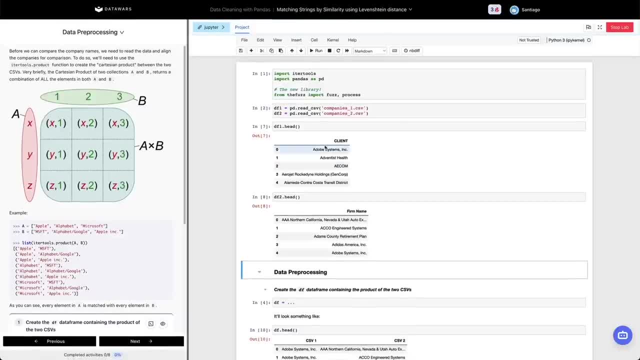 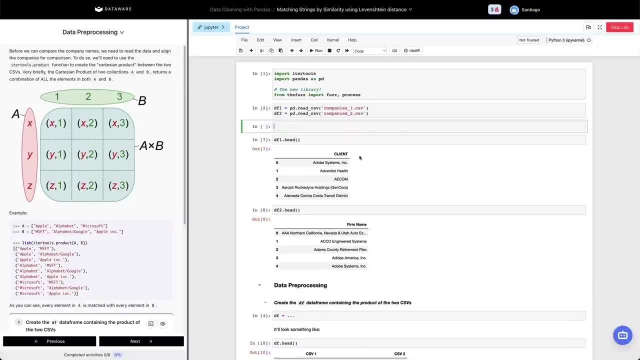 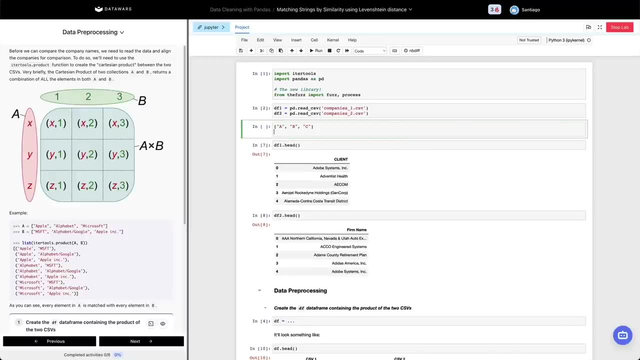 have to understand is how are we going to match these uh companies? we could do something like a four loop nested right. so let's say we have uh, two companies, so a and b, three companies and c, and we have um, a, a, inc and b and brothers and c, and how can we? 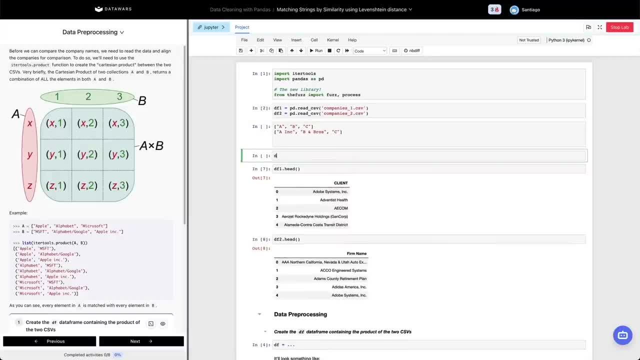 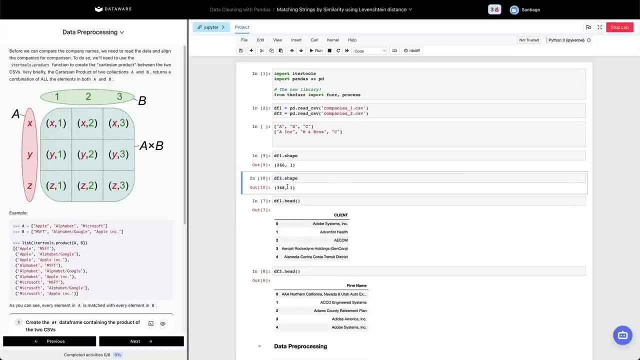 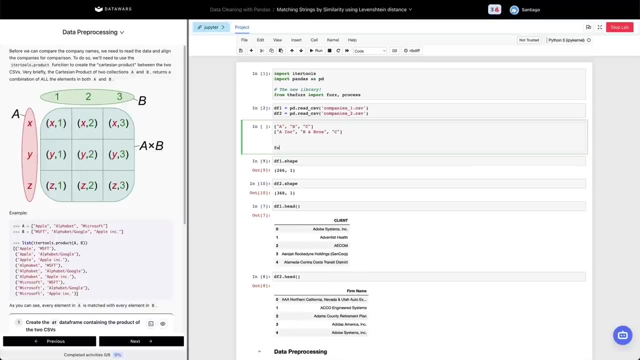 match. of course we have more than those. we could actually take a look. we have shape of the f1. we have 266 for the first one and 368 for the second one. but the way we could do it is with kind of a nested for loop. we could do something like four uh c1 in companies. 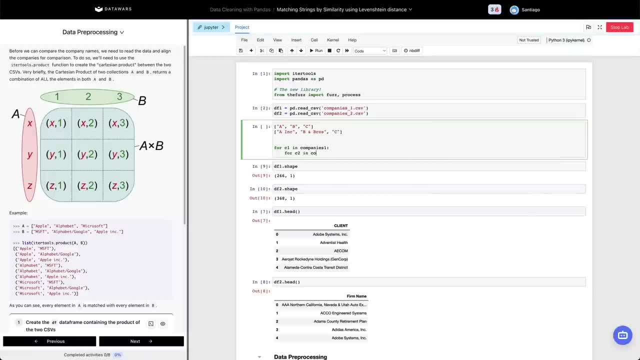 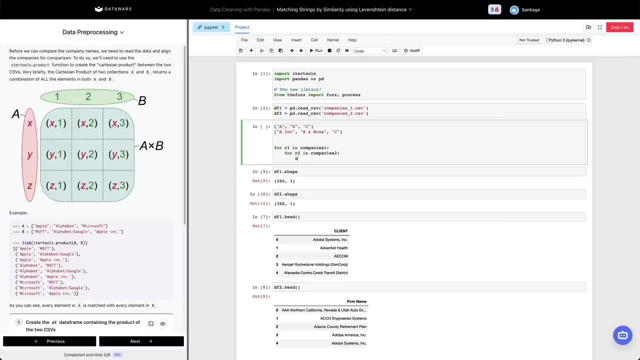 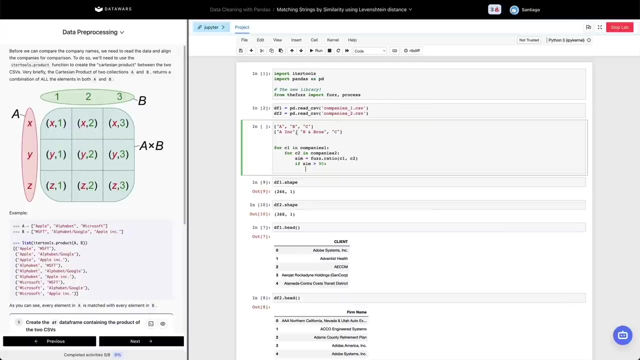 one and four c2 in companies, two right, and we can do, uh, something like distance, let's, let's see. similarity is equals to. let's just use some quick, um, quick zoodo code here of c1 and c2 if sim is greater than 90 um and we can store these things. let's, let's make, we're gonna make something like: 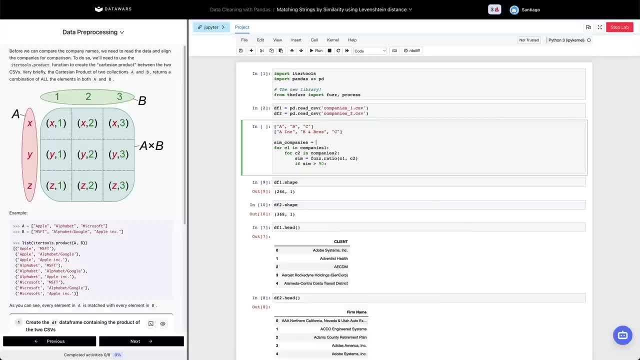 companies, similar companies. we're gonna do uh, similar companies. dot append. we're gonna put c1 and c2. but this algorithmic approach doesn't let us visualize the data and see and do a little bit of an analysis of what, how the data changed, how the data is represented under the hood. we're gonna 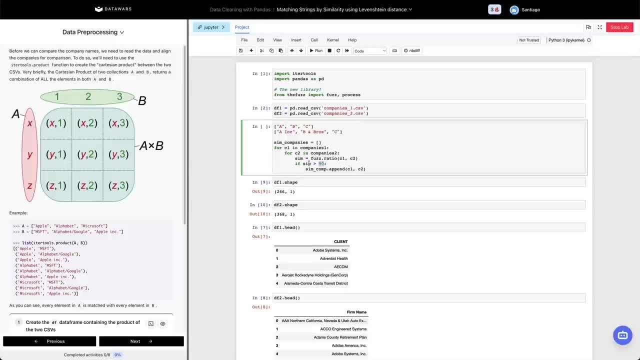 just do these hard cuts in 90 without the ability to see if maybe there was an 89 that was fairly good and don't don't don't worry about the number itself, because i mean 90, 89, 85.. this approach, algorithmic imperative approach, is not extremely, it's not very analytical, in in from some point of 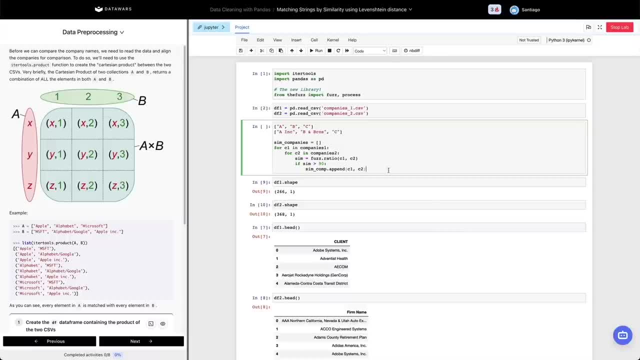 view, it's not easy to see why or how things are working behind the scenes, so an alternative way that we're proposing for this particular project is to create the combinations of the columns and pretty much do this same process: match every company with every company. a with a ink b. 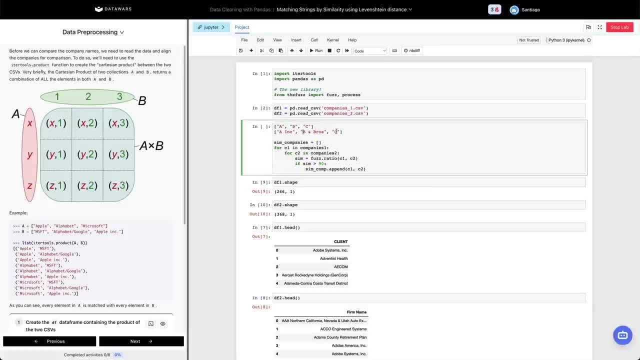 and bros and c b with a ink b and bros and c c with a ink b and bros and c match every company with every company, and to do that there is a very simple method, which is the eater tools dot product method. so we have imported the eater tools method and we're gonna do here. let me remove this thing. 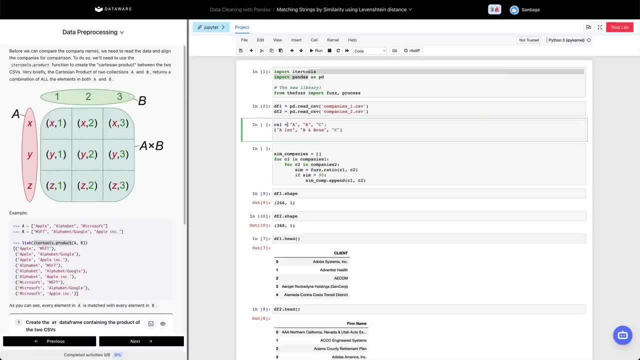 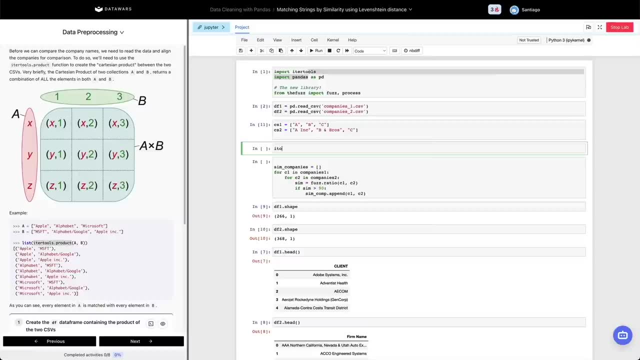 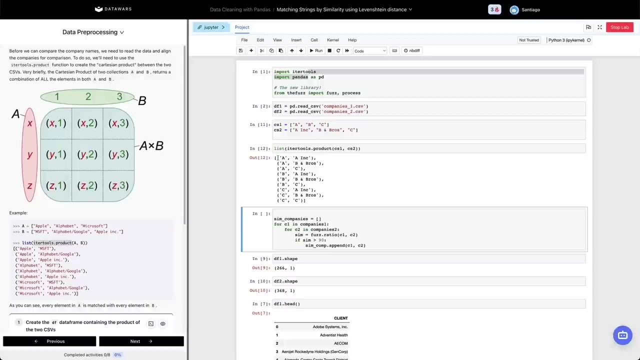 and we're gonna do companies one and companies two. these are plurals. i'm gonna do ether tools. ether tools dot product of c1, cs1 and cs2, and we need to wrap this thing in a list to visualize it. there you go and we have pretty much the combinations of everything with everything. 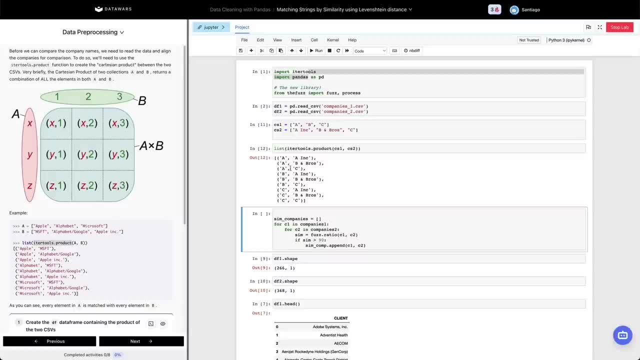 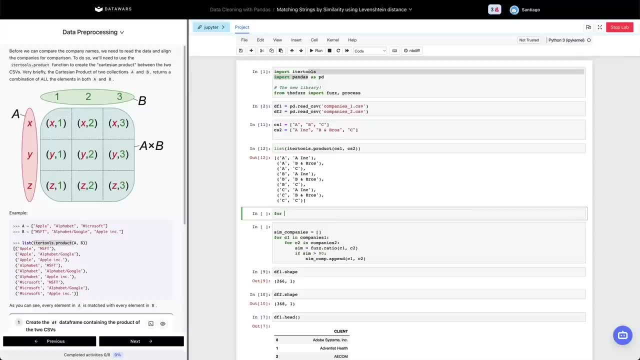 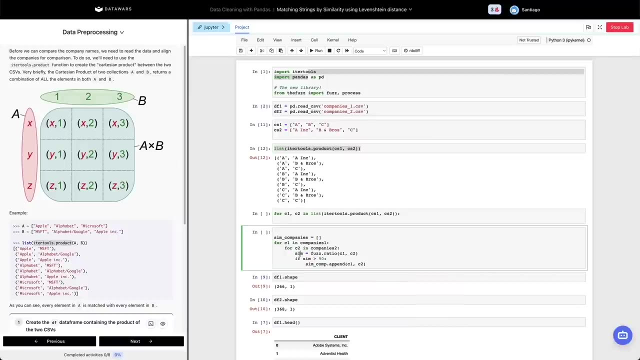 which is again what we were, uh, wanted to do. so now what we can do is we can just pretty much do four at a time. um, so let's say we use an imperative approach again, we're gonna do four- c1, c2 in this thing, right, and now we can say pretty much the same thing we were doing before. we can compute. 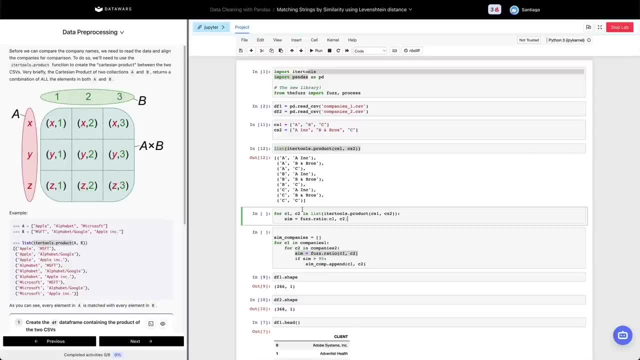 the similarity of these two companies, but the result is we went from a nested computational intensive for look to something that is a declarative- uh, expressive- approach. In this case, we're generating the data And now we can do some different things. If we think about this thing in a data frame, we could potentially add a third column. that is the. 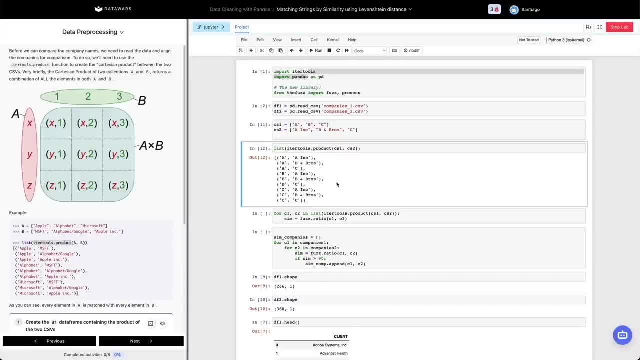 similarity. So now we're going to have a ink and the similarity column And now we can start doing some analysis. we can filter all the values that have greater similarity. we can do a, we can do some plotting, for some of the components have some certain similarity we can visualize, we can 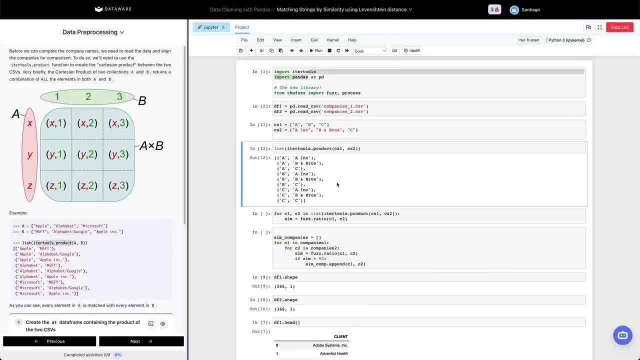 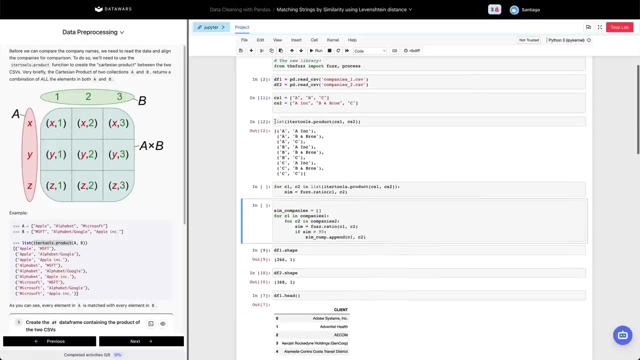 explore- we can analyze the data in a more declarative, analytical way than just doing a simple- not simple, but just a more rudimentary- naive iteration or imperative algorithm. So let's move forward, let's get rid of all these things, And we're going to start approaching the first. 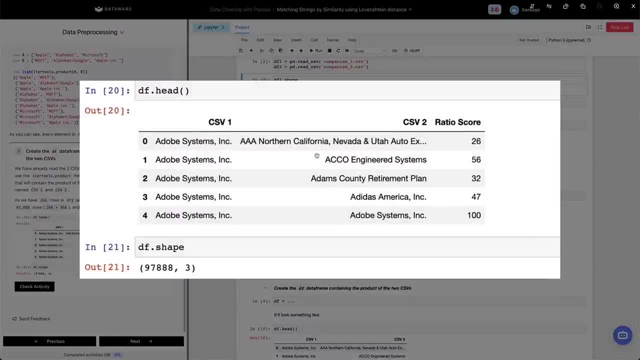 activity, which is basically asking us to build that data frame, build this data frame that contains the companies Of- sorry, the contains all the companies from CSV one and the product of CSV two, and also compute the ratio for all of them, right? So we have to put these two things together. the first thing, 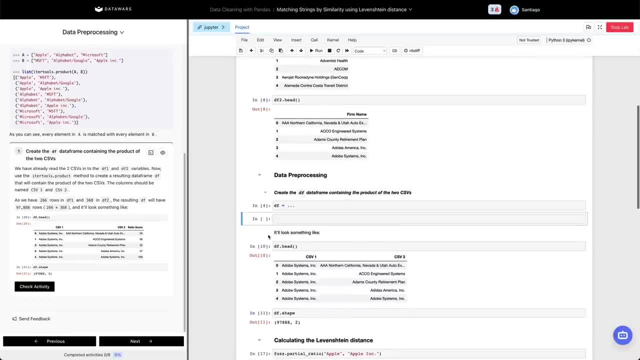 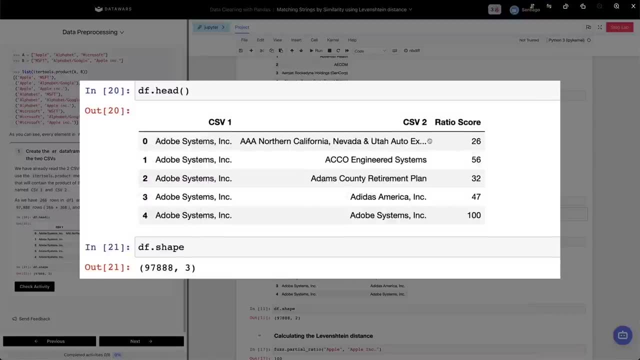 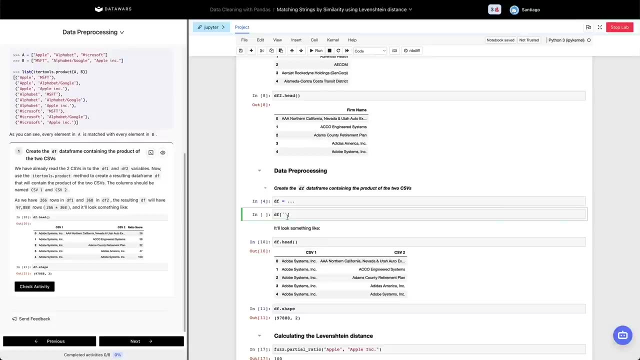 we're going to do is we are going to do DF at. we're not asked for the ratio right here. this screenshot is incorrect. we're just gonna compute. we're going to just compute the product and create the large CSV. So what we're going to be doing here is we're going to do the F. 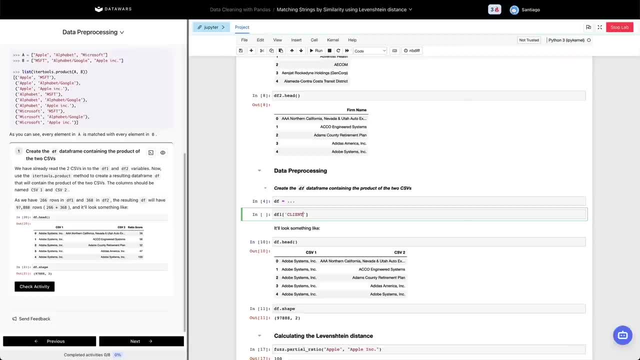 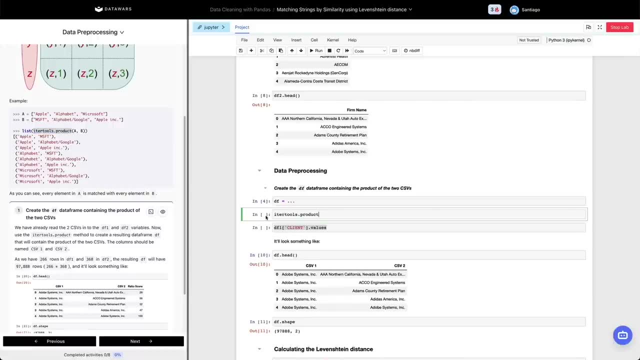 one, add client, client, the values. that's going to be our first list. So remember, we have either tools that products. here's the syntax: collection one, collection two. So we're going to pass for collection one, we're going to pass the row for the for the F one and for collection to the F. 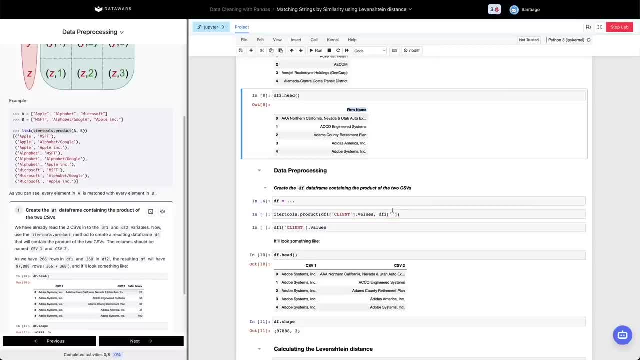 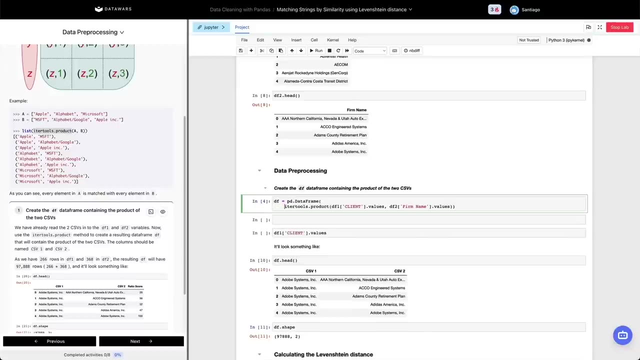 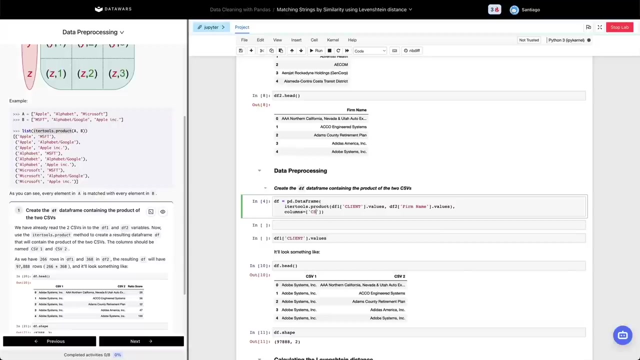 two We're going to pass. then it's firm name, dot values. We can pass this whole thing to a data frame, PD, dot data frame, this whole thing, break it into a different row and we can say column names, columns. it's going to be CSV one and CSV two. 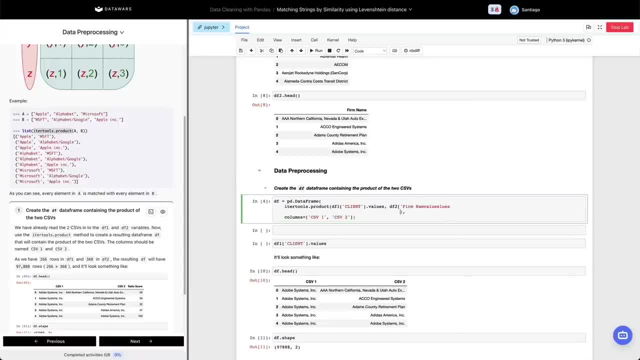 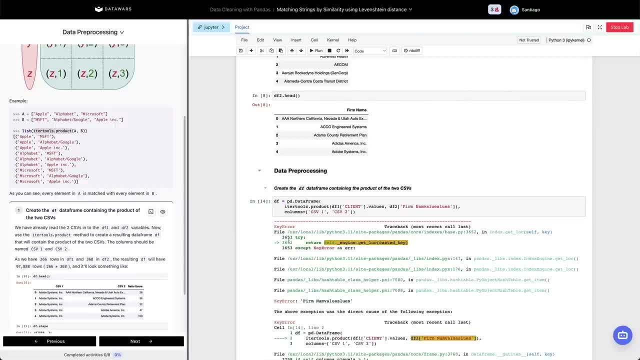 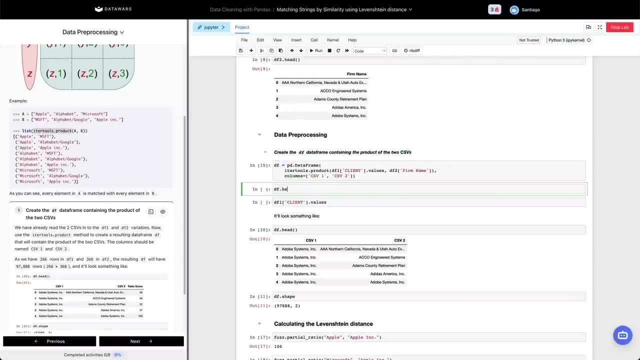 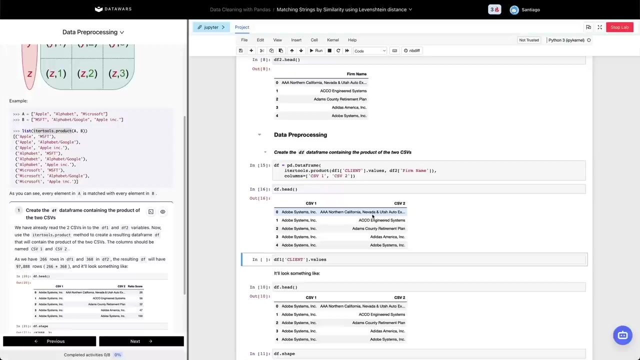 And I have a non matching parentheses Because I'm need to close that one, And we have an error with columns, no firm name values, And there we go. Sorry, we have a few mistakes. This is pretty much the regular process of data analysis or data processing, And now what we see is we have created 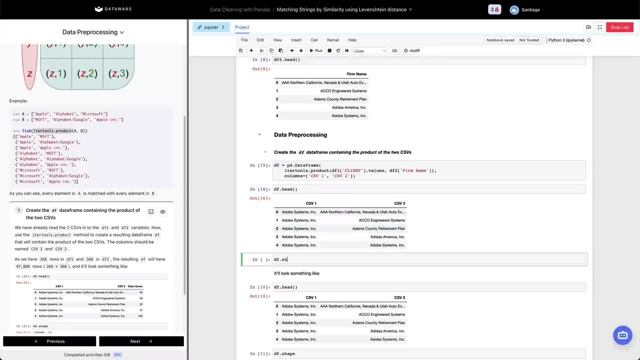 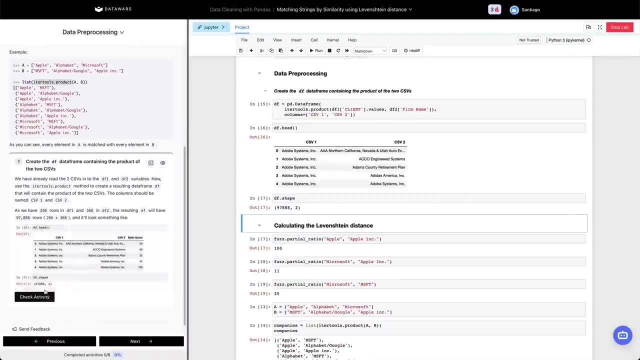 this huge- let's actually take a look- the F shape, This huge data frame with the same expected rows as the one we have right here- 97,000 rows- which is going to be the result of the product of the F one shape and the F two shape. So let's give it a try and see if it passes. There you go, it worked, So So. 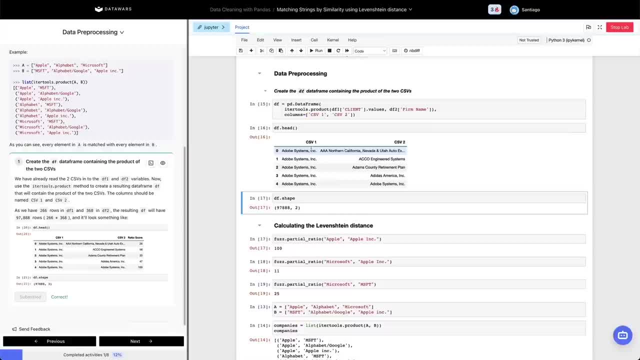 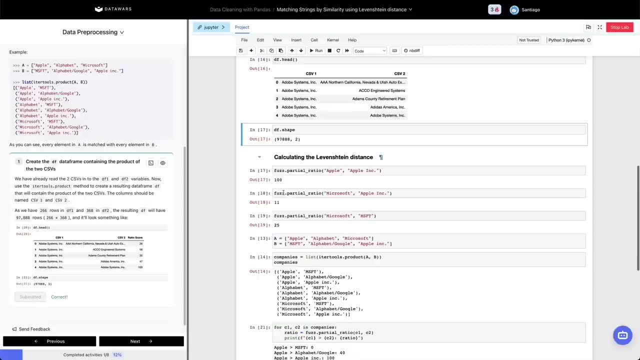 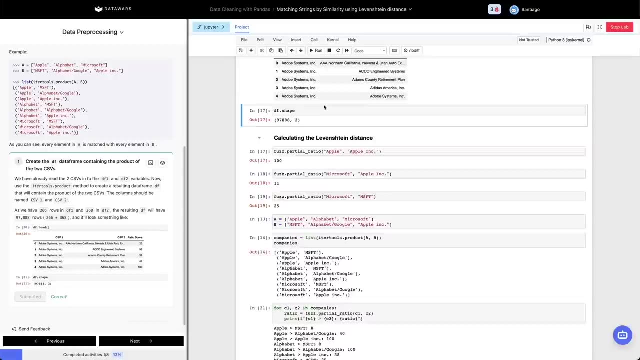 far so good. We have our product of different company names, so we can do a little bit of matching. Now we are going to apply the range, the Levenstein instance right, to compute the similarity between the company, So of. 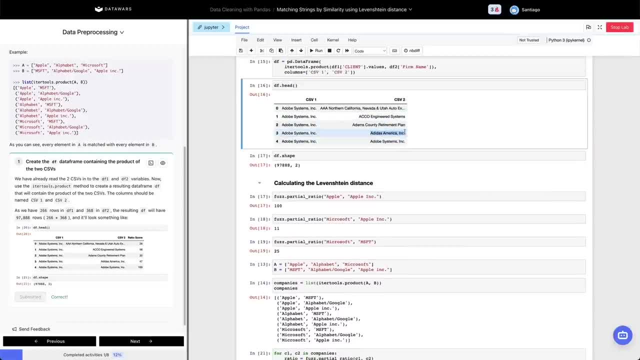 course, the similarity between these two is going to be a lot. the similarity between these two is going to be 100.. I mean, sorry, the similarity here is going to be pretty low, the distance going to be pretty high, the similar is going to be pretty low. They similarly, in these two companies- Adobe for both of. 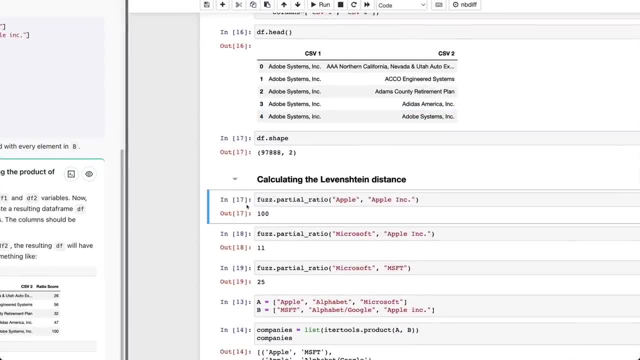 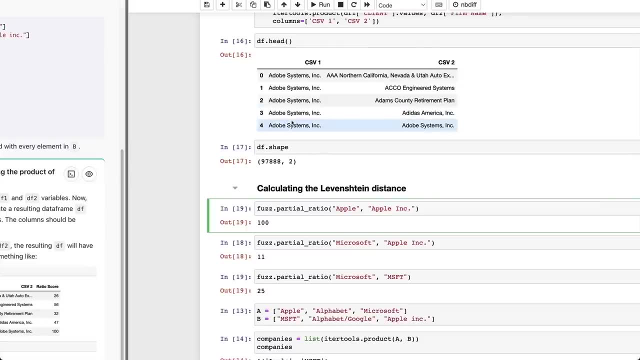 them. it's going to be pretty good. So we're going to use using these library for files dot partial ratio. partial ratio because the companies have white spaces, So it's gonna pretty much compute the the words in different orders And these might be helpful. All right, So what we're going to do here? 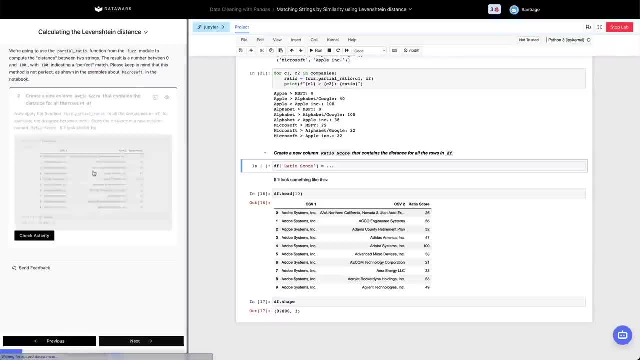 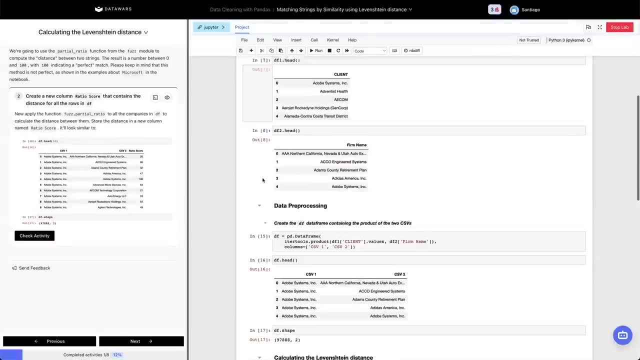 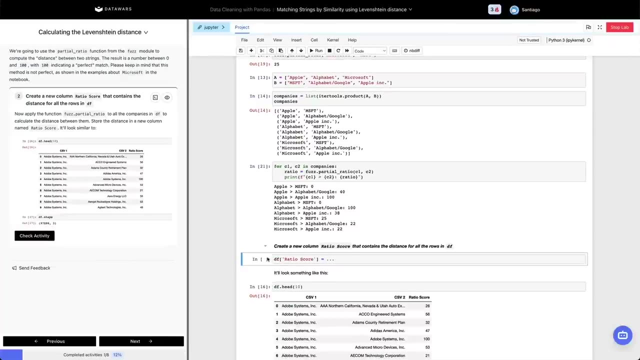 is, we're going to compute the, the ratio score, and we're going to swap to the activity first. So this is the second activity that is asking us to compute the ratio score. We have, right there, we have the ratio score here of these two companies. And how can we do that? Well, it's pretty simple, as we already have the. 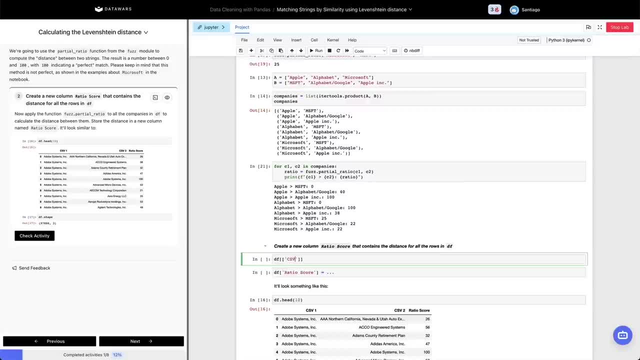 values. So we have the F. we can just do values here, Values, And we can do something like, let's say, score equals fuzz dots. partial ratio of C1 and C2 for C1, C2 in the F dot values. 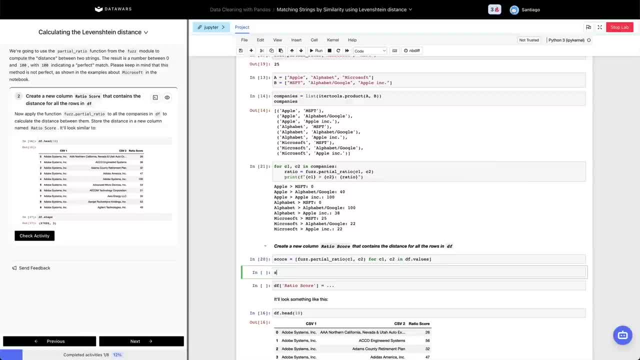 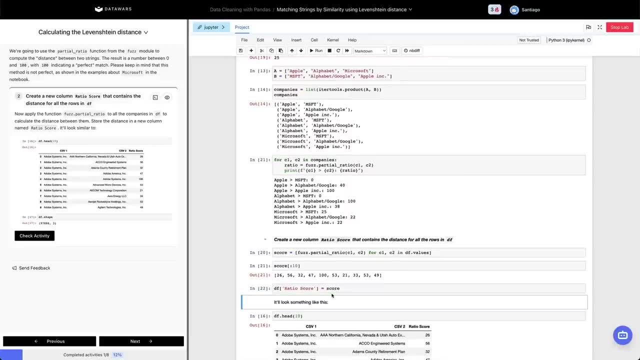 It's going to take a little bit of a moment. There you go. We can get like the first 10 scores And we can now basically apply that to ratios guard and take a look at the different ratios And now we have that Adobe. 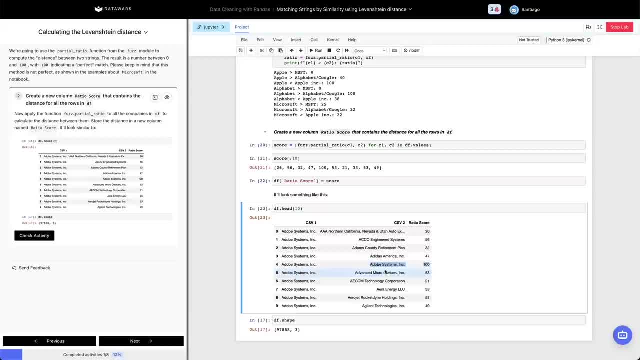 systems, right, obviously has a 100% similarity, while something like Adobe with advanced micro devices Inc has a lower similarity. right? the only thing similar is probably the ink and the individual individual characters. Alright, so so far, so good. The first part of this process is understanding how we 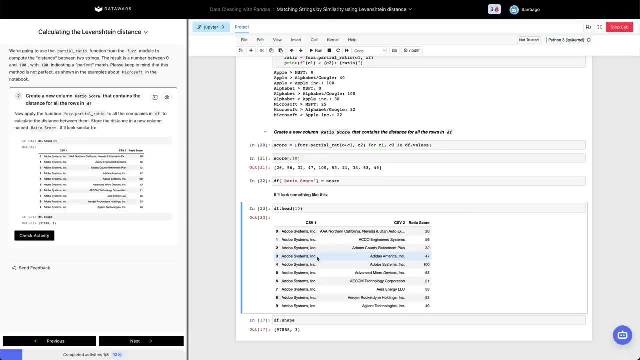 created a declarative, descriptive approach by transforming our data and working with a different foundations, like we move the floors, like we started with these two different data frames And now we have just a single one that has these very useful column with the combined ratio of the: 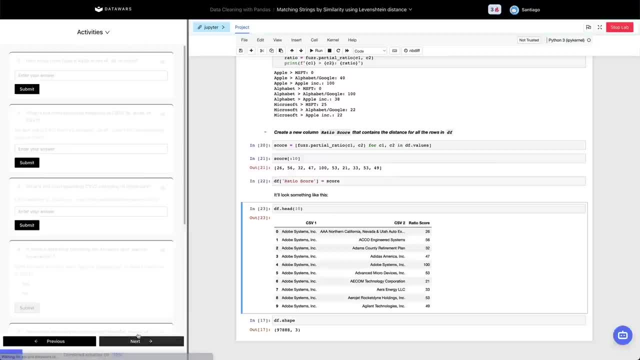 similarities of each of each company. So in this case we have a single one that has these very useful column with the combined ratio of the similarities of each of each company. So now let's move forward with a few more activities, And this is pretty much the whole data analysis process. 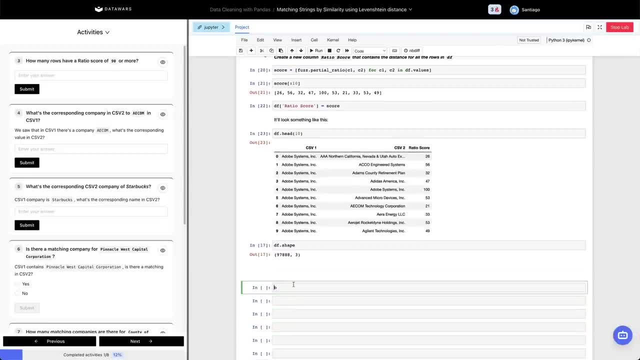 I'm gonna create a division here and we can get started. How many rows have a ratio score of 90 or more? And this is gonna be dflog: df at ratio score greater or equals to 90.. And let's take a look at that. 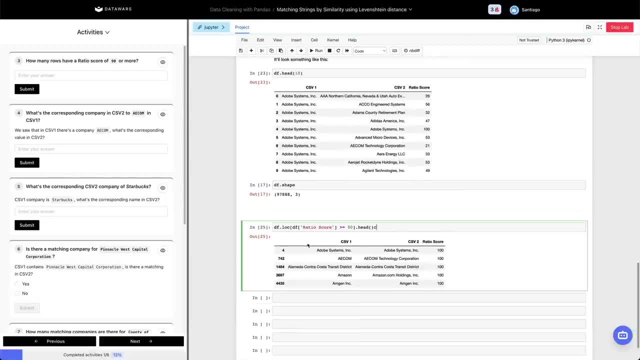 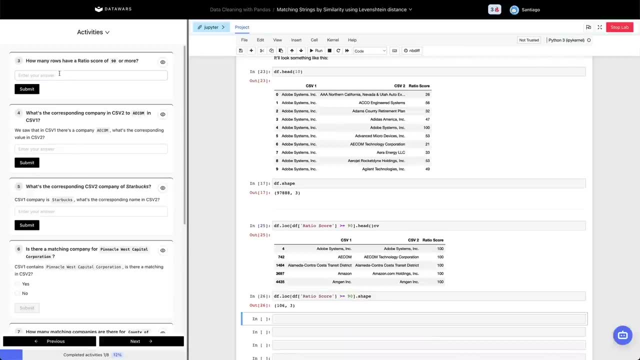 I made a mistake. There you go, And we can now check how many we have. And we have 106 companies. There you go. What is the corresponding company in CSV2 to a EECOM in CSV1?? And this is the one we pretty much saw here at the beginning. 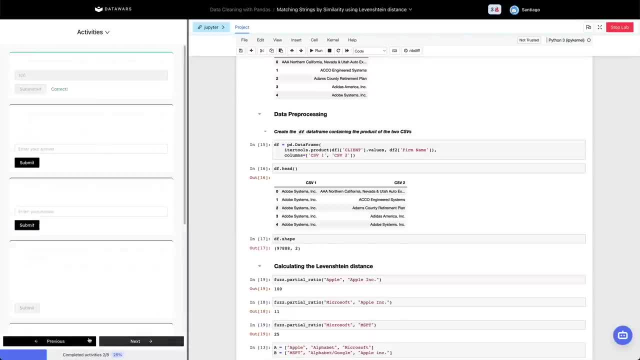 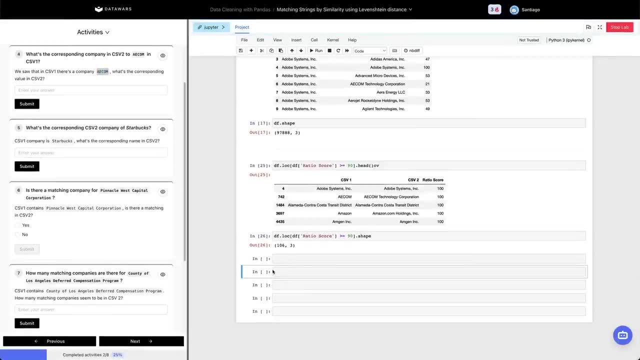 This one right here, But let's go ahead and give it a try. There we go. So what we're gonna do is we're gonna find we're gonna do dflog or let's actually use query, So we change things a bit. 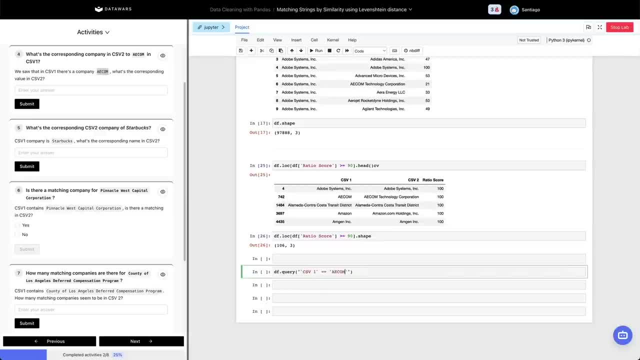 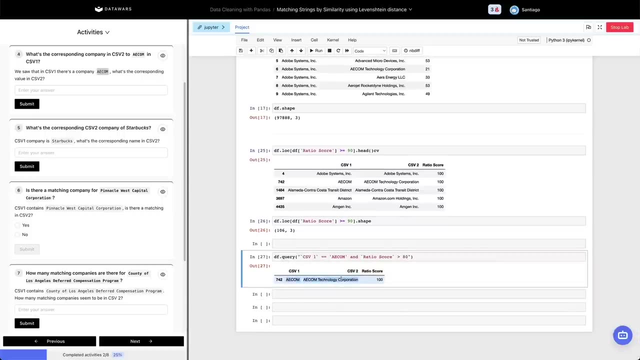 We're gonna do. CSV1 is equals to this one and ratio score is equals to what, Or greater than what I'm gonna say. let's say 80 to take a look, There we go. So these two have a 100 ratio score. 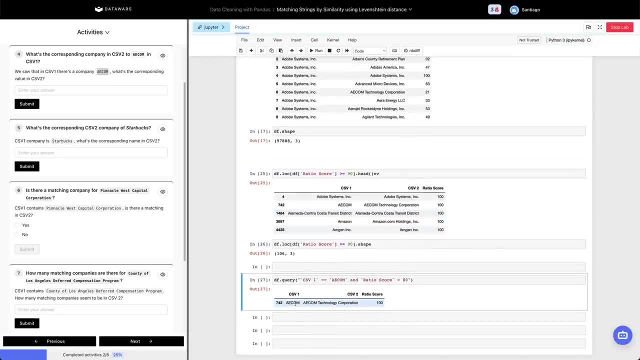 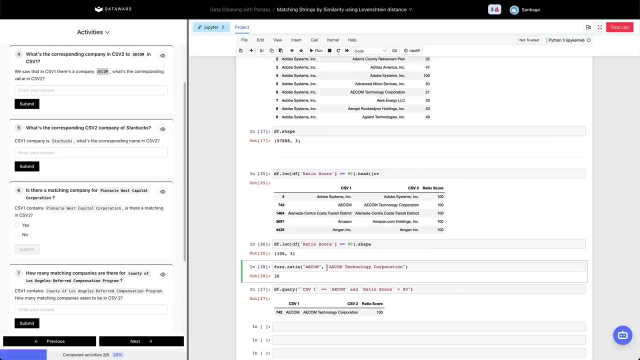 because, again, we're using a partial ratio. If we were using a for ratio only ratio, this is gonna be lower. It's actually 30. And that's because there is, in reality, there is a lot of dispersion or distance between these two words. 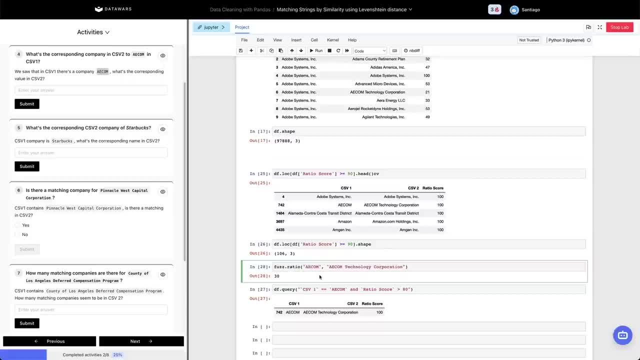 There is no much similarity. like again, to the human. there's a lot of disparity or distance between these two words. There is no much similarity. human eye: there's a lot of similarity here because we can zoom in and just focus on these two words. 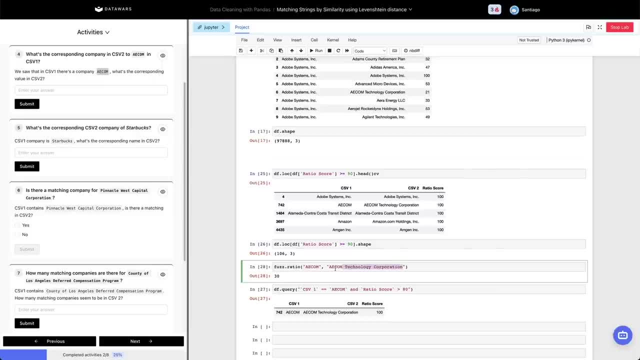 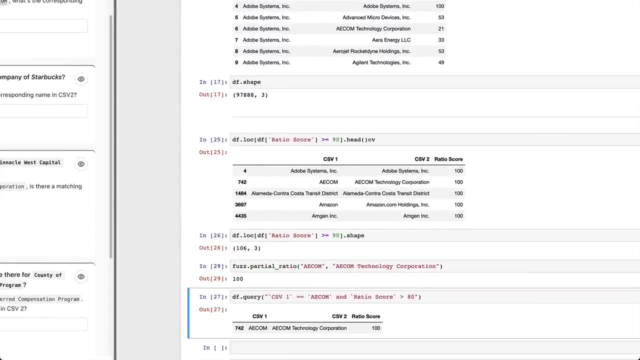 but if you think about it's like this whole thing makes the second string completely different, and that's why we use the partial ratio. partial ratio, which now gives you a 100 score, because it's doing the same thing we do with our eyes, which is basically focusing attention in different. 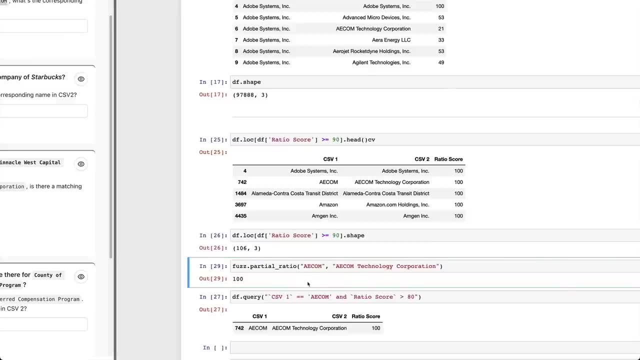 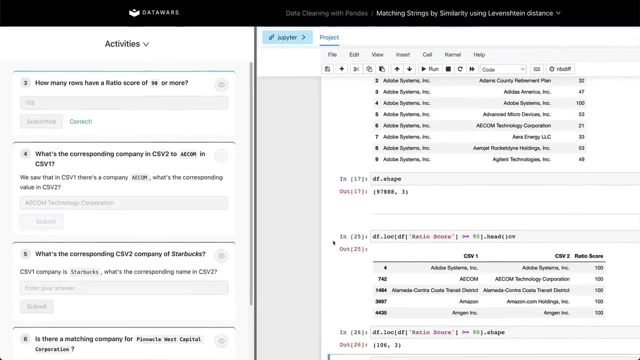 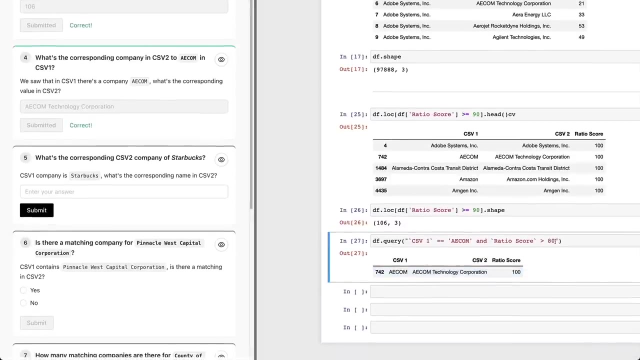 words right, and give you the combination of individual words. so anyway, uh, let's try it out. this should work as expected. um, and basically here's like we are. um, we are basically trying to understand what's going to be the kind of value that is going to make us right, decide if 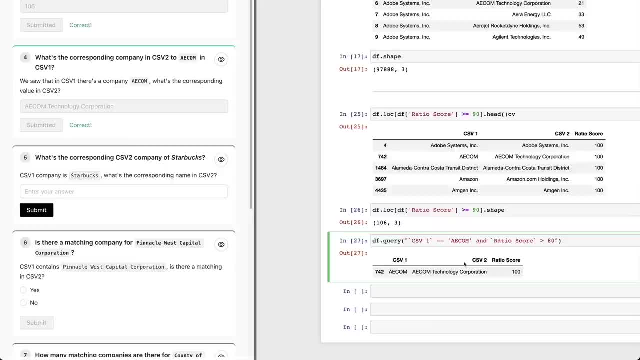 a company, programmatically speaking, right in an, in an automated way, if a company name matches now the company name, it's like: where's the cutoff value? um so, csv1 company. the fifth activity is starbucks. what's the corresponding company in csv2? we're going to do the same thing and let's 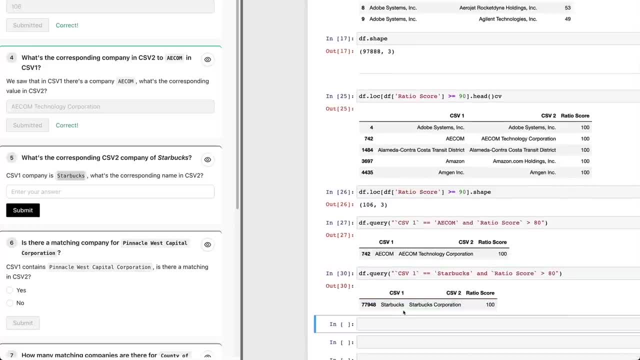 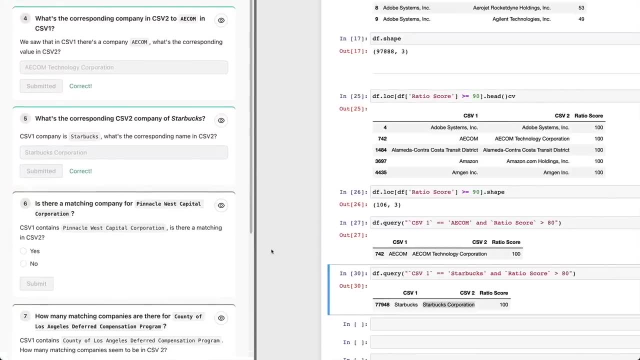 keep the ratio equals to 80, and we have that it's starbucks, starbucks corporation and let's enter it right here. it works. but again, the ratio score was 100 and 100. so by doing some analysis we can start understanding how this um these different 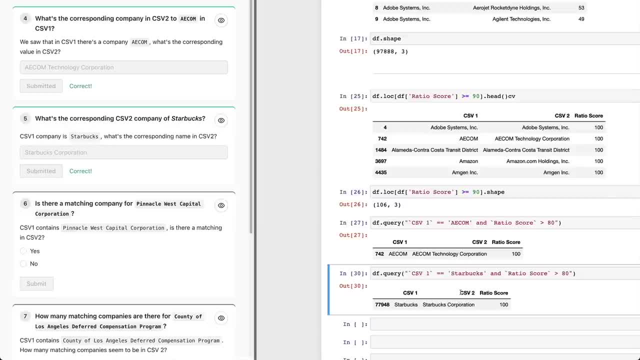 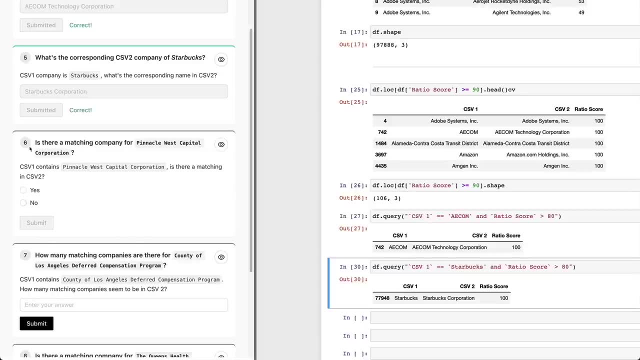 ratios are going to be distributed, something that i'm gonna do in at the end, just as some other activities. so activity number six, is there a matching company in pinnacle west capital comp corporation? so let's copy this thing once again and put that, and there aren't. 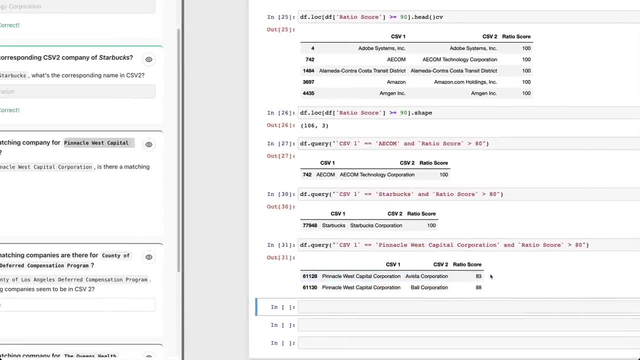 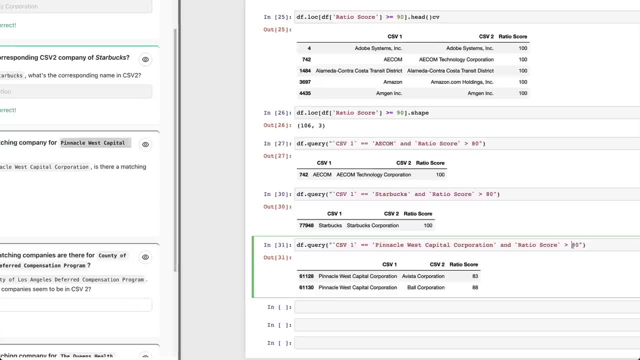 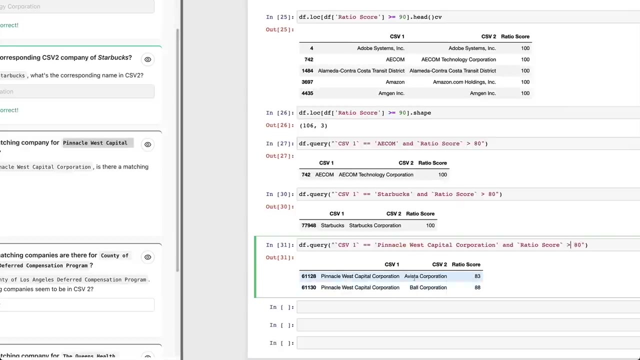 like, definitely these two are not related. but but we see, right here, just because i randomly chose, uh choose, i'm randomly choosing to use 80 as as the ratio score to do the cutoff. it's like there are two companies that have nothing to do with pinnacle west capital corporation, but they have. 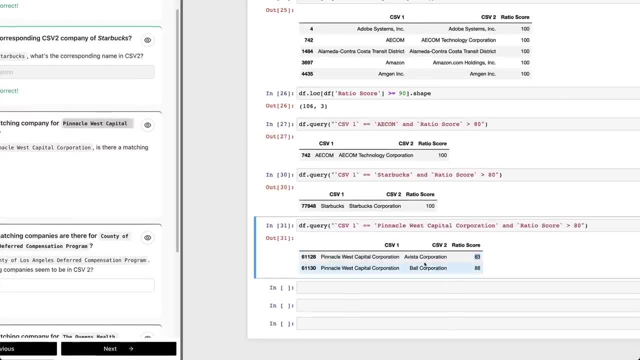 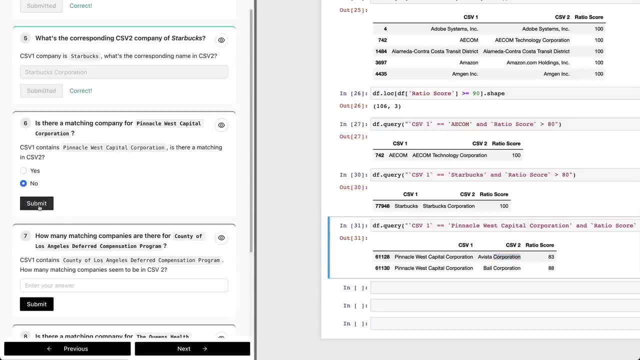 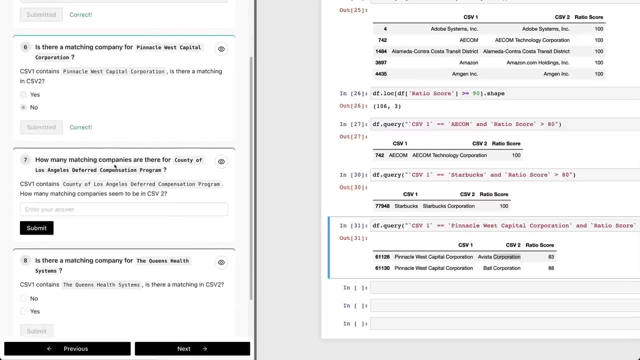 a ratio score of 83 and the answer is that because they have. they have the corporation word, so we have to be very careful. so i'm gonna say here: no, let's see what's the answer. that works, um, and let's move forward. seven activity: how many matching companies are there for county? 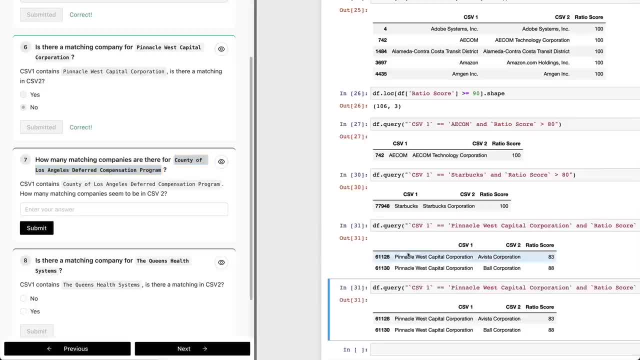 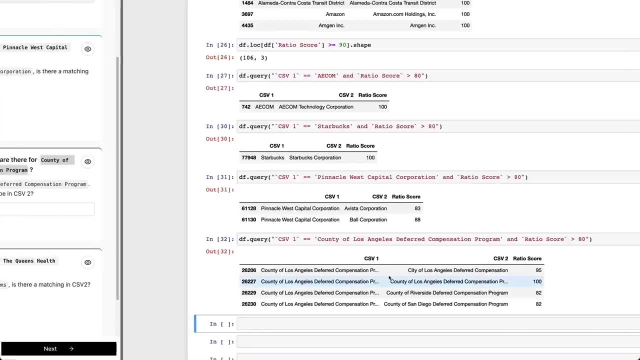 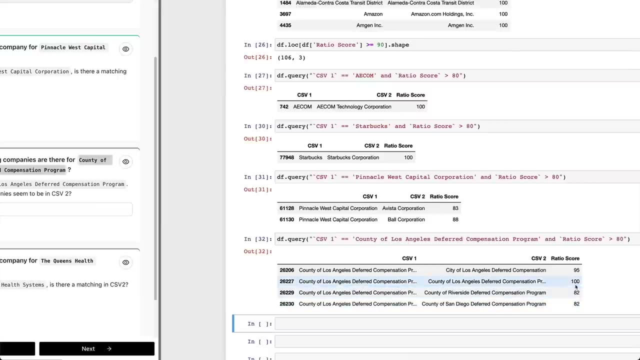 of la blah, blah blah, and now we're gonna put this thing and we're gonna keep the ratio equals 80, so we can take a look and keep understanding what we have. um, so there is a very clear difference here. um, two companies that have a value of 82 and two companies that have one 100, 195, so above 90. so 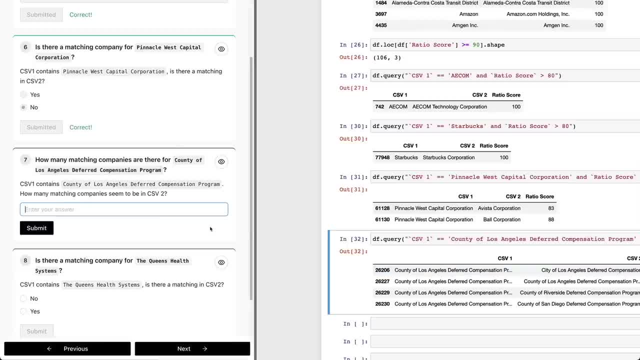 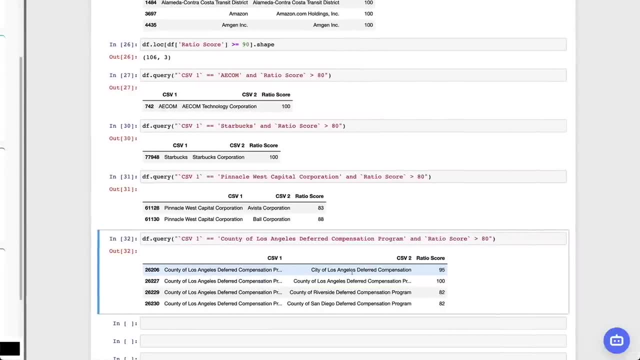 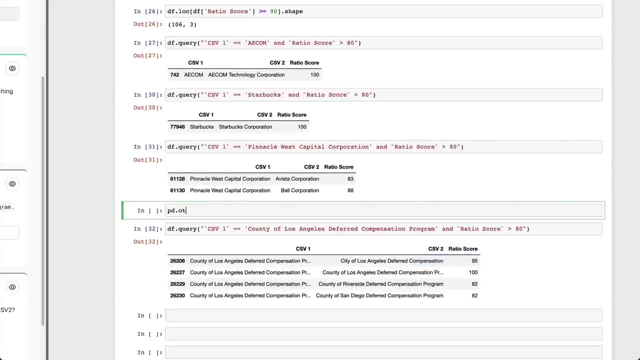 i'll be tempted to say two. here there are two companies- that's much the name for county of los angeles. blah, blah, blah. um, we should take a look at the full names so we can do that. um, with pdoptions options, maybe i can ask our ai assistant. 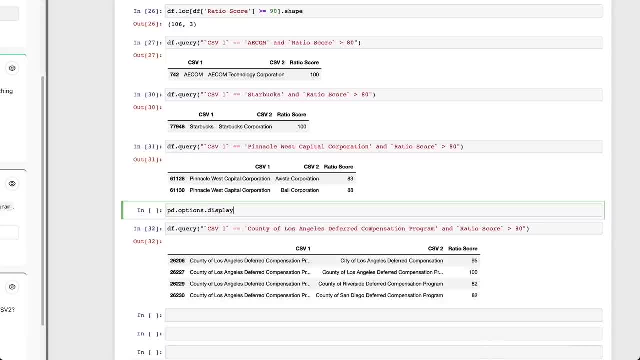 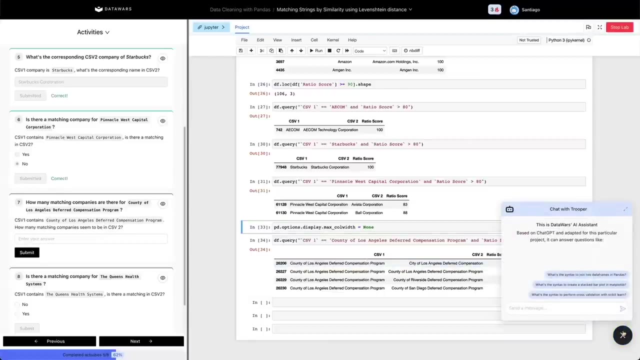 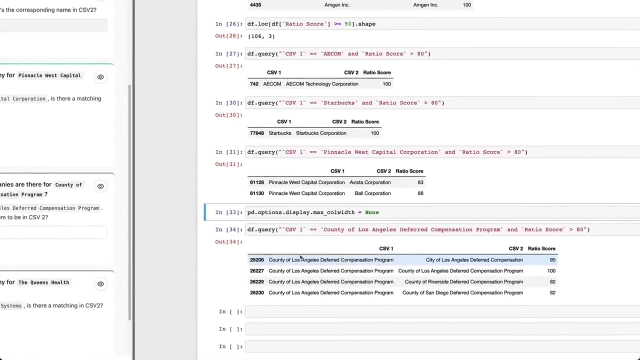 if i don't remember, this display max, max, max call with none. there you go. that was one um. if you ever have the dub, you can just ask the assistants, go for it. don't worry in googling or asking the ai assistant, because that's pretty useful um. and here now we can. we can take a look at them and we say 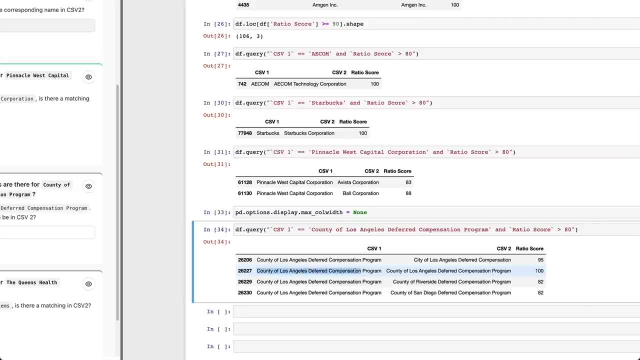 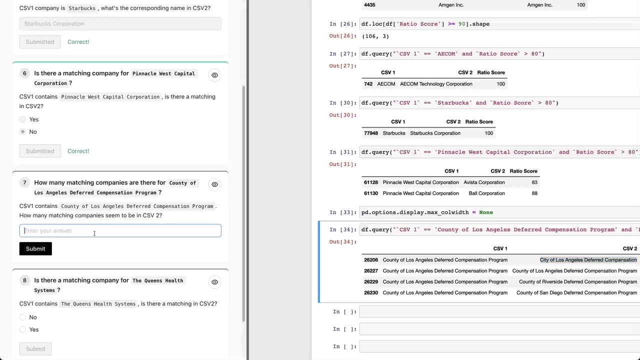 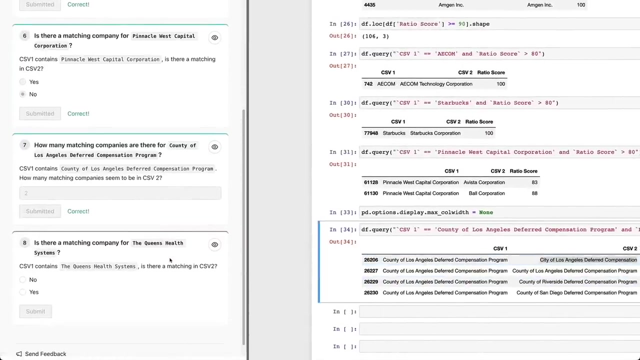 county of los angeles deferred compensation program, county of los angeles deferred compensation program and then we have city of los angeles. so i'll potentially say how many companies seem to be in csv and we're gonna say two. there we go. they seem to be the same company or they're not. 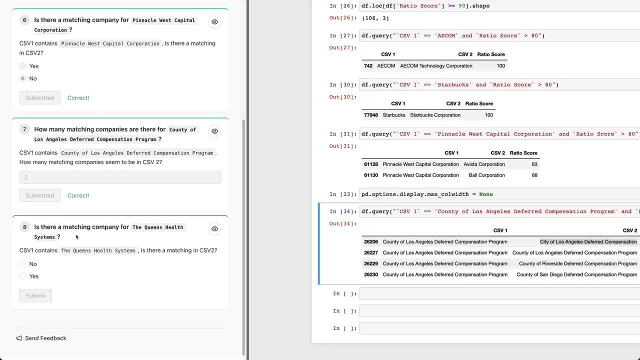 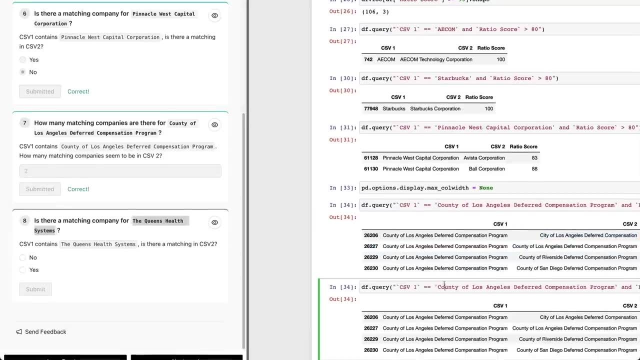 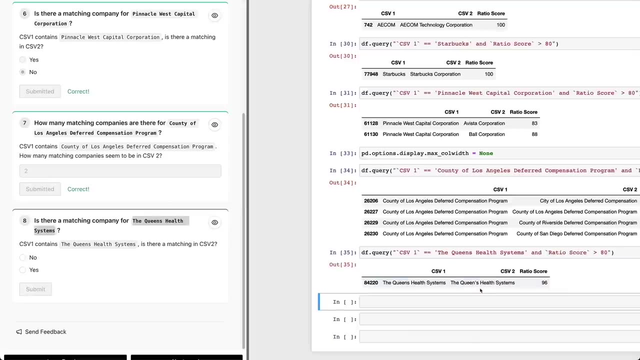 companies, entities, to put it away. so, finally, a activity. is there a matching company for the queen's health systems? what we can do here is run pretty much the same operation and we find the, the queen's health system just with the apostrophe, and the s so is. 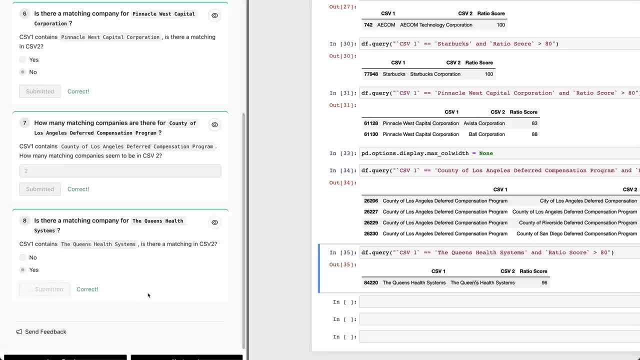 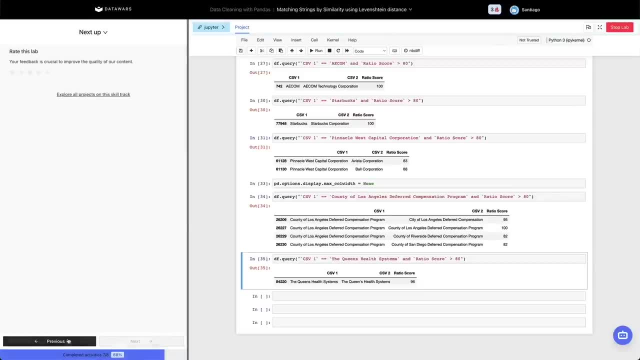 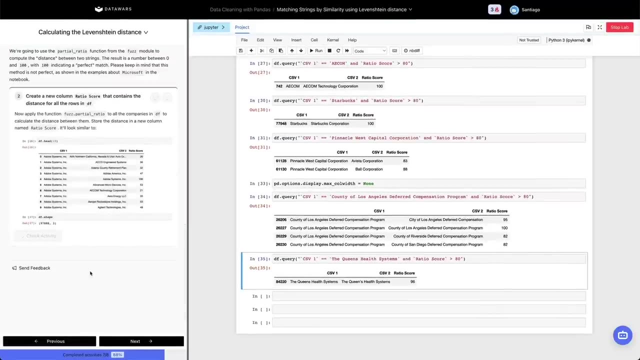 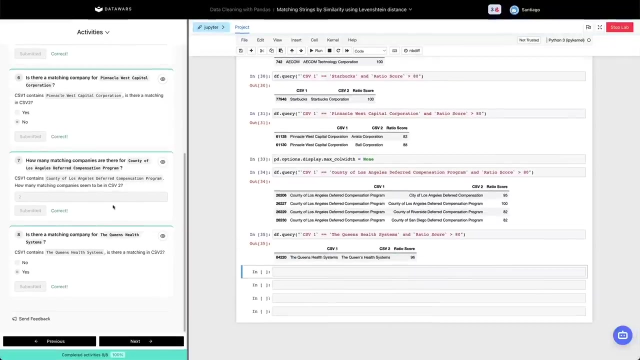 there a matching, we're gonna say yes, and by doing this analysis- and we have, i think we're missing one activity. i think i have completed. oh, let's check this activity. there you go, we have no more activities to complete, all the project passed. but by performing this analysis, so first we did. 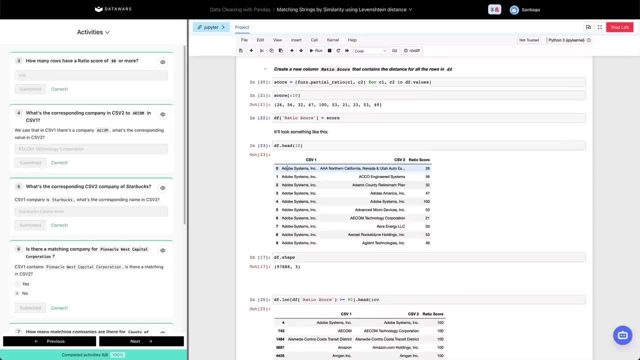 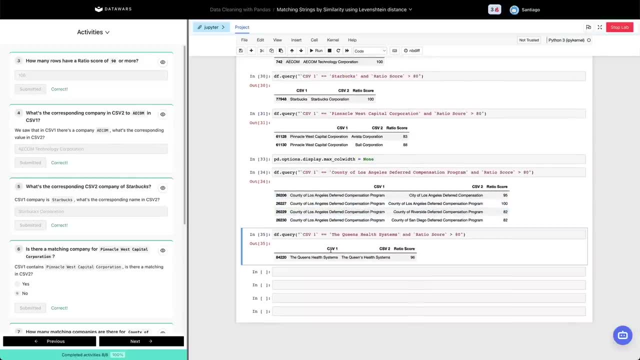 a little bit of data wrangling, we did a little bit of uh, managing to get to the ratio score, and now we're kind of close to start generating the, the final csv, if you want the final csv, if you want to find a representation of what would be the matching companies- and here we don't have an activity in- 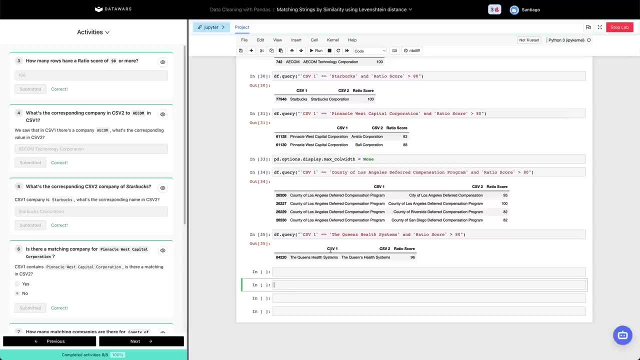 this particular one on purpose, because there is still a data cleaning process that it's kind of annoying. it could take a little bit of time, but we can start taking a look at. we're gonna say, for example, dflog, df at ratio score greater than 90, right, and we can take a look at how many companies 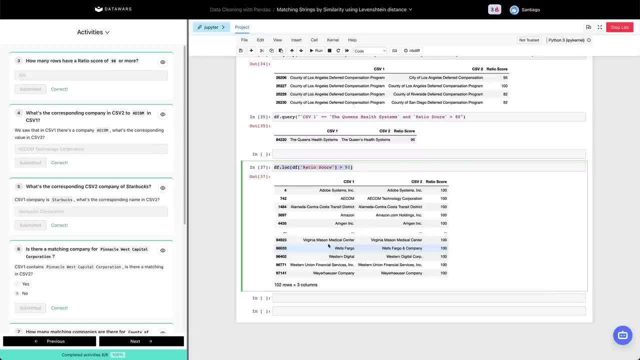 are matching that uh, that, uh, that query. we can go one step further, and when you're doing data cleaning, something very useful to do, at least to me, is to start visualizing your data. so i'm going to do ratio score and here i'm going to plot kind kind hist. 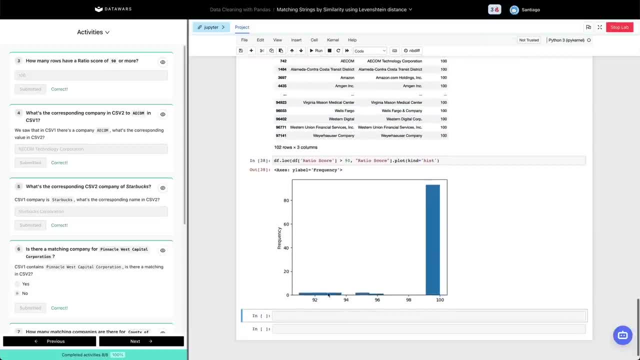 and you're going to see that, if a ratio surpasses 19, most of the data that we're going to be using is going to be the same as the data that we're going to. most of the data that we're going to be using is going to be the same as the data that we're going to. 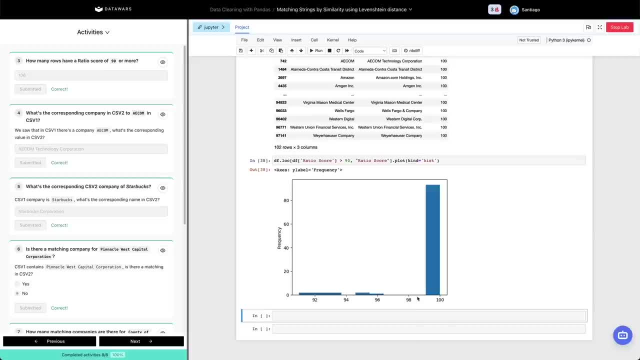 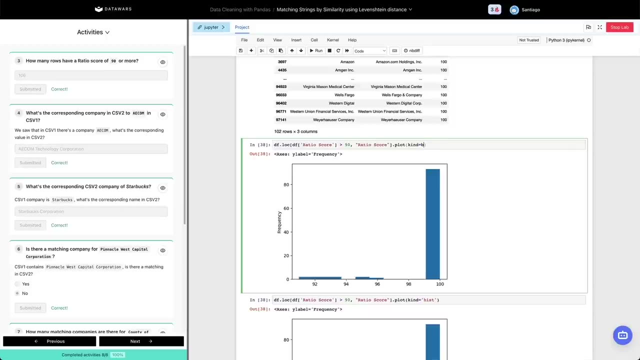 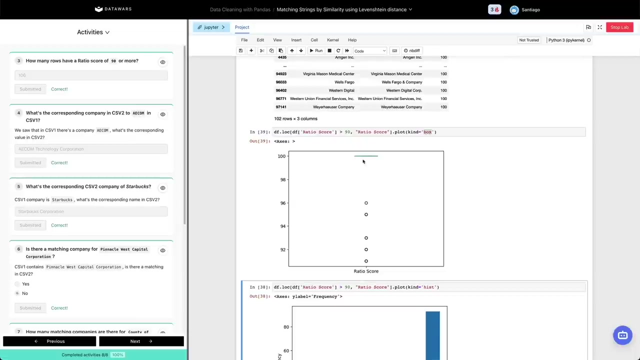 have. the samples are going to be between 98 and 100, so it'll be interesting to see what companies we have here. let's actually um, we get. we can actually take a look also at a box plot. so we're going to do box and we have pretty much the same results, like everything is concentrated in the 100. 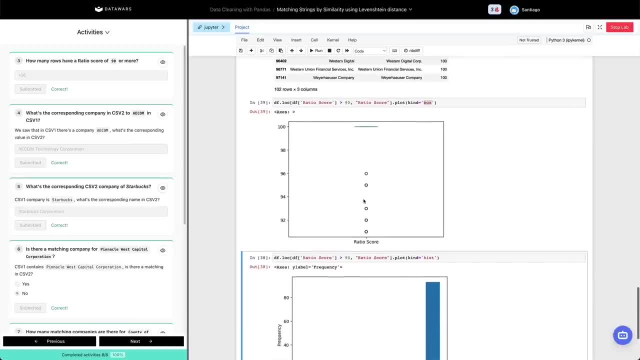 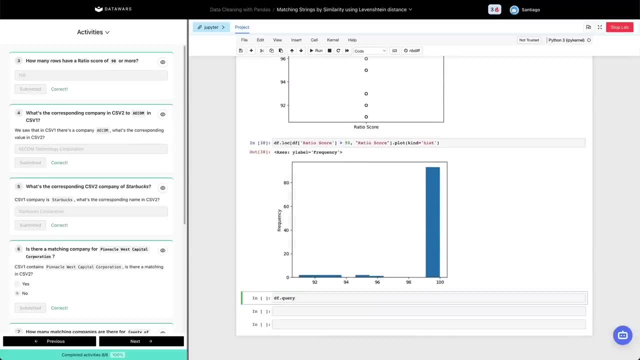 and then we have a few samples in 96, 95, 93. so let's actually take a look at those and we're going to say the f dot query. let's do query now where ratio, ratio score is greater than 90 um and is less than 97. let's say: 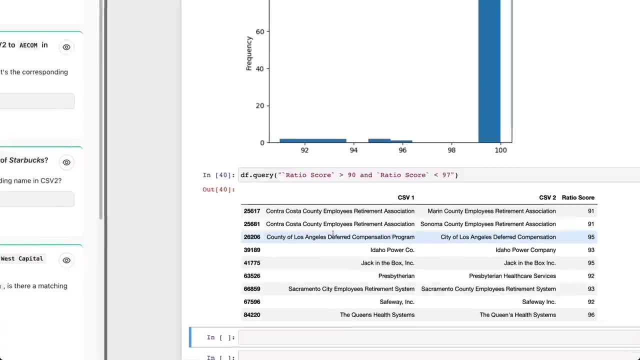 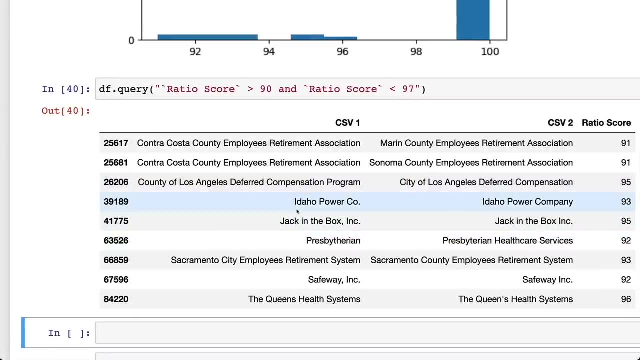 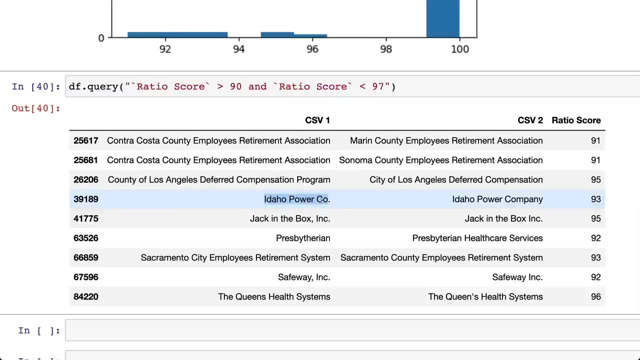 and now we can take a look at what's going on in here, and this is again. this is the data analysis process, so in this case we have one that seems to be very compelling. this one is pretty much the same thing idaho power co is. it's the same as idaho idaho power company. 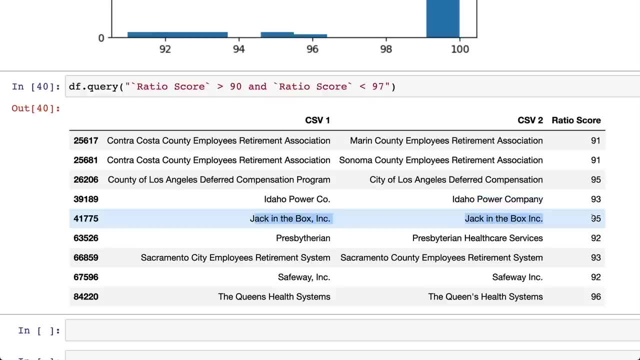 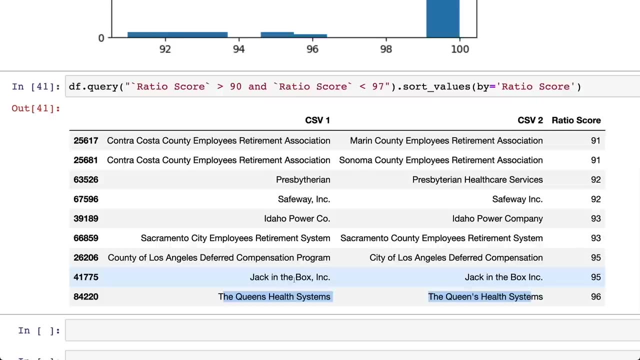 jack-in-the-box inc and jack-in-the-box inc with 95, let's actually sort my bar. let's sort values by ratio score and we're going to start with. the ones are like, less like or more likely. so the queen's health system pretty much the same thing. jack-in-the-box pretty much the same thing. 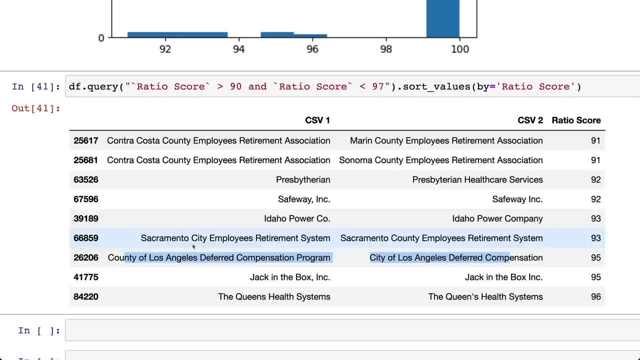 county los angeles, and cita the whatever we did before: sacramento city, sacramento county. of course we have to understand if the city and the county for us are represent the same entity or not, but nevertheless, idaho power company is the same, safeway inc is the same. these two are. 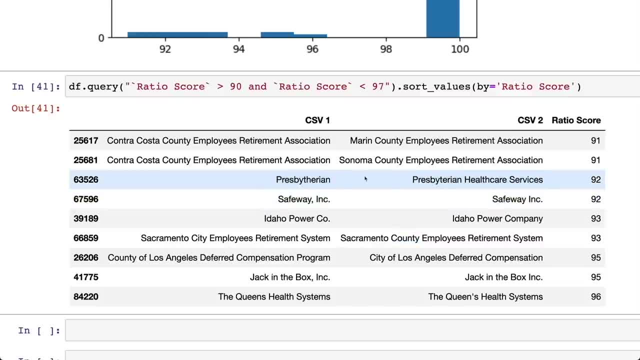 probably the same, but now we're getting into a little bit more of the same thing. so let's see if we can get into the range of what would be the same thing here and let's actually try to see how we're getting in with this one. if we're getting into terrain that it's a little bit. 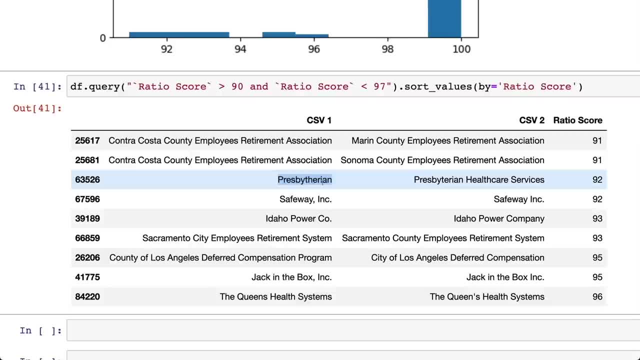 less clear what's going on here. so i'm not so sure- and this is because i don't know the business we're running- if this um company or institution is the same as this one right here- potentially right, but this is where you have to start to ask. so 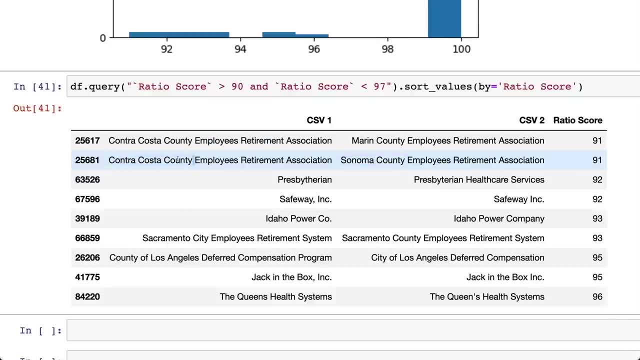 these are different. Again, I don't know the business, but I'll bet that these two companies are not the same. The same thing with, again, Contra Costa and Marin County. So I'll bet that these two are definitely not the same, While there is a little bit of a mixed ground between. 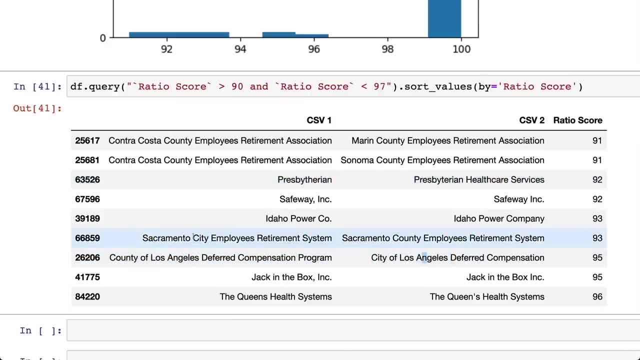 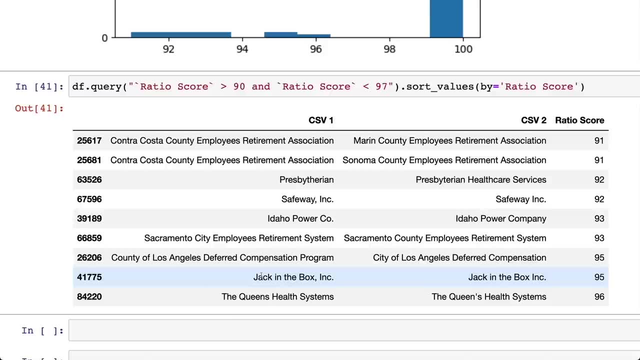 let's say this one and these two in terms of if city and county and city and county are the same institutions, And then there is no doubt in the last two. So, basically, this illustrates the real process of data cleaning, which is, first of all, if we would have done this process before. 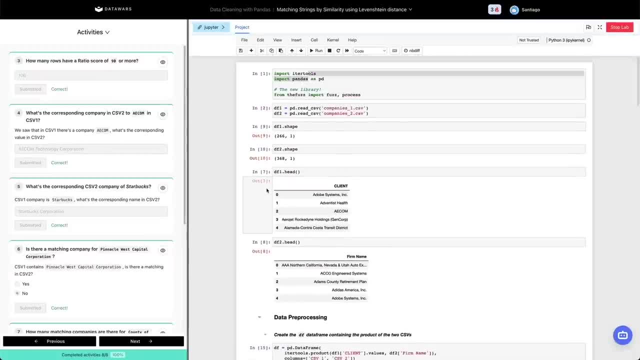 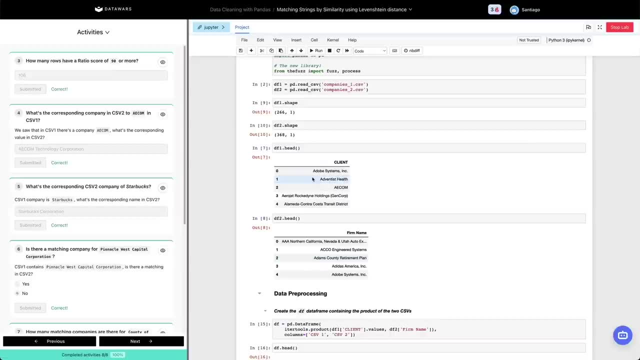 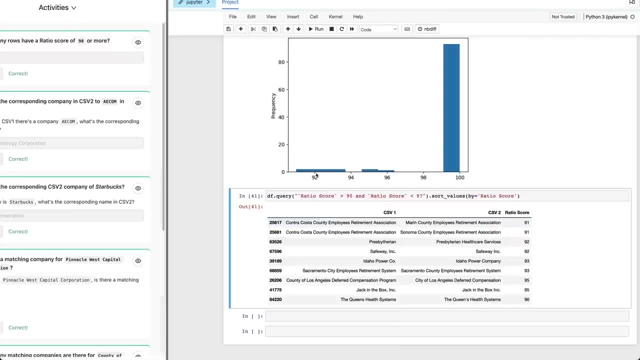 there was a nested for loop that I deleted. Remember nested for loop for company one in companies one for company two in company one. When we do it manually, it's very hard to visualize this. So what we did right here was by first reshaping our data and having a clear picture of all the 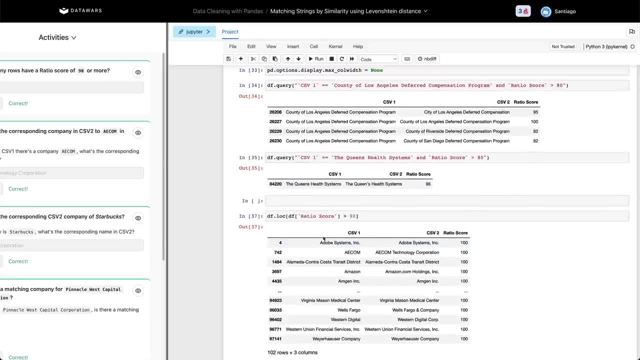 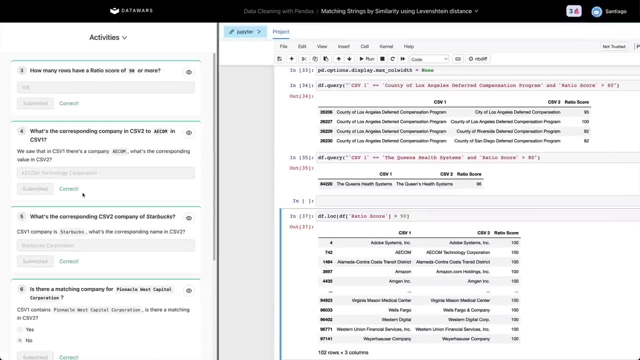 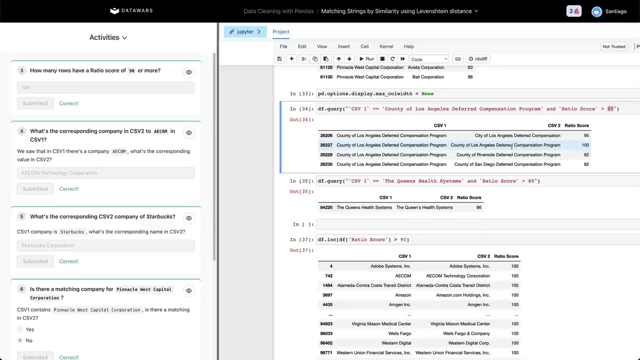 data we had, we were able to create a more descriptive representation. We calculated this ratio score company. We started doing some analysis. We answered some basic questions like: can we find a company here there? Can we find this cut of value? We know I just chose 80,. 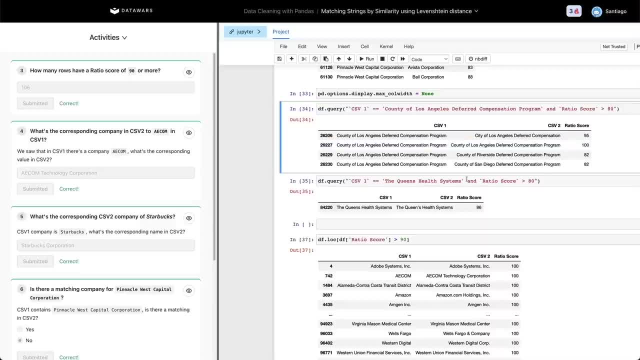 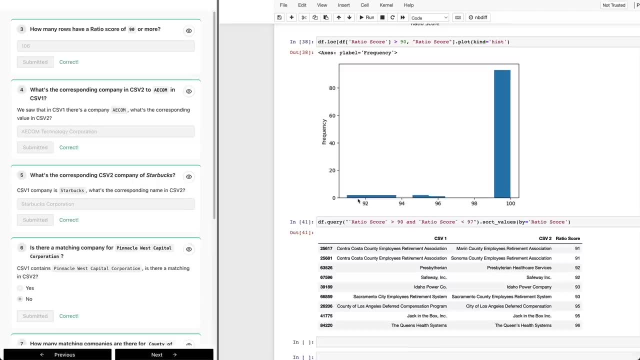 but we could have used 75 and see how it went. And then we took a look at the distribution of the ones that seemed to be more likely And we found this middle ground. It was something like we probably need to go back. 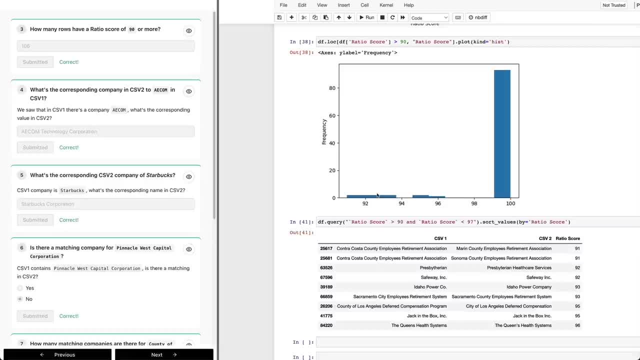 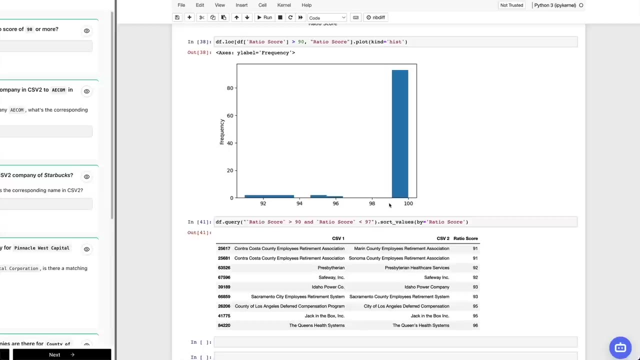 to whoever is running the business, or just Google it and start understanding the data that we're dealing with, Because data cleaning, at the end of the day, you do need a ton of domain knowledge. I can't just clean data with my data cleaning techniques without understanding data that I'm cleaning. I 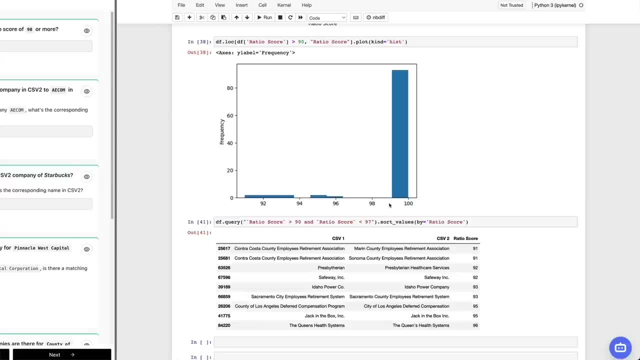 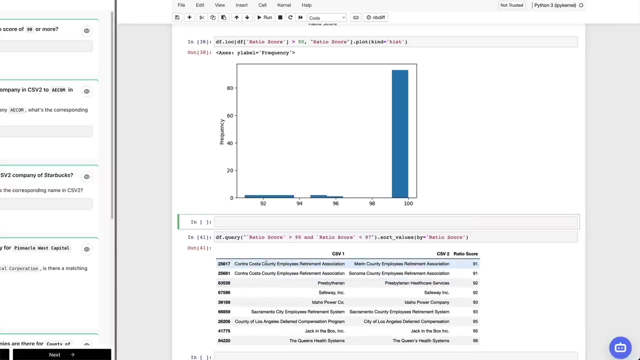 might be a great data scientist, but if I'm cleaning biological data or data from a physics lab, I will have no idea what data I'm working with, right? So that's a very, very common case You have. you know you're working with a high tech and you have measurements from instruments. 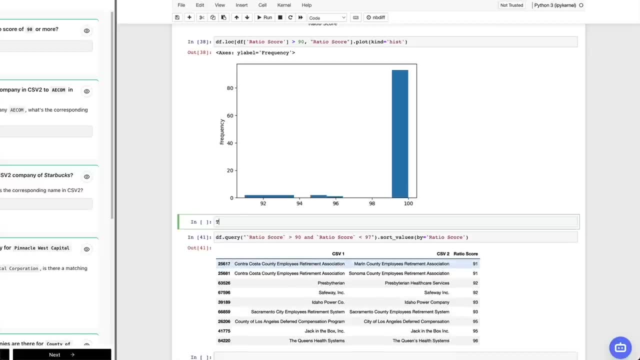 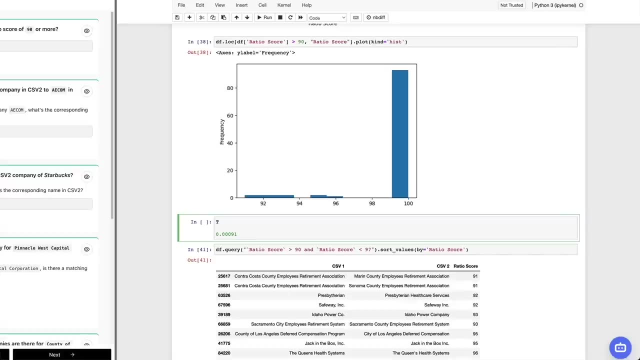 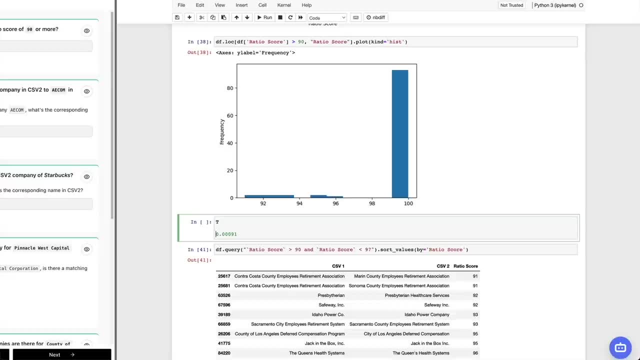 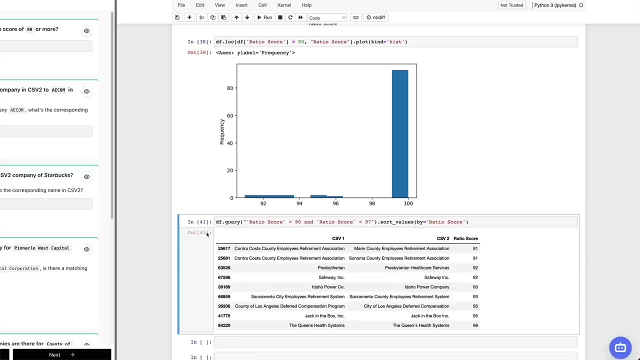 physics guy comes and says: hey, this is completely wrong, You're missing the columns. The T value should be in the orders of hundreds, not in the orders of I don't know very small right. So I need to understand the data. but to understand the data, to understand the domain, to be able to 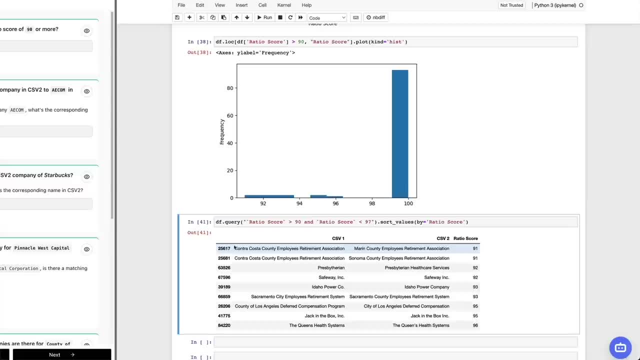 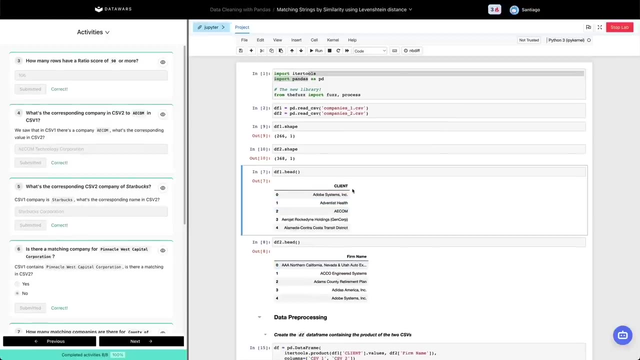 Google things to be able to go to the archives of the company. I need to put that in a good representation that allows me to do that, And that's what we're doing with these representations that we have created. So, anyway, I have talked a lot so far in these projects because for data, 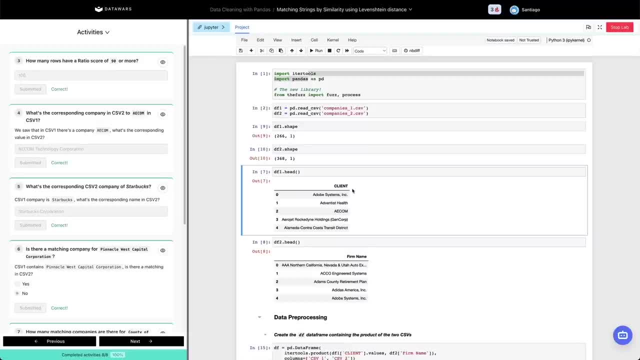 cleaning- this is the most important thing- is being able to reproduce your experiments, visualize and understand what's going on. Take a look at the project, try to resolve by yourself or keep working with other capstone projects we have for data cleaning. It's a very fun activity, pretty. 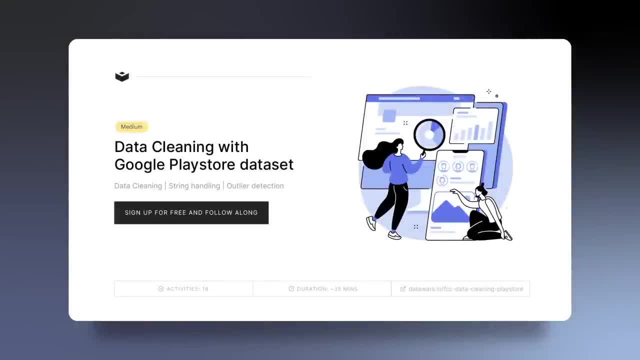 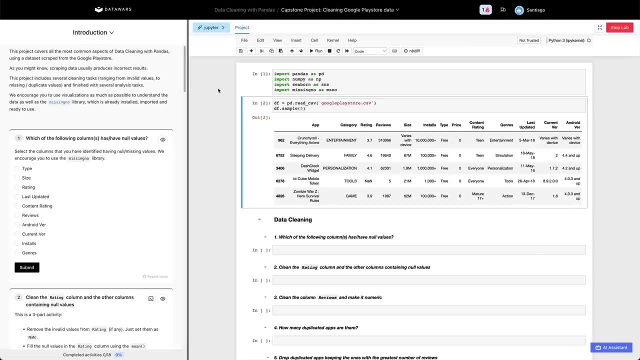 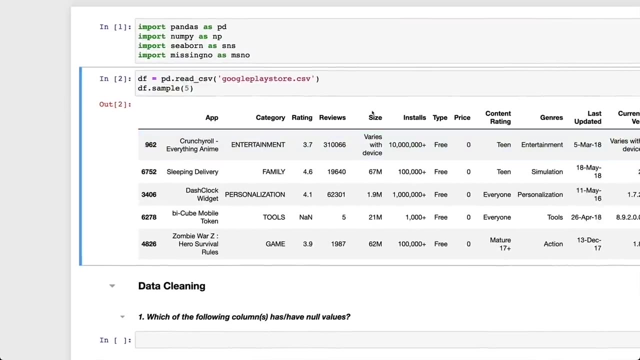 much all the time. This project is focused on data cleaning and some data analysis after the data is clean, And it's a very interesting one because the data that we're using it comes from someone that scraped- right, just scraped the HTML out of the Google's Play Store, right? So, as you might, 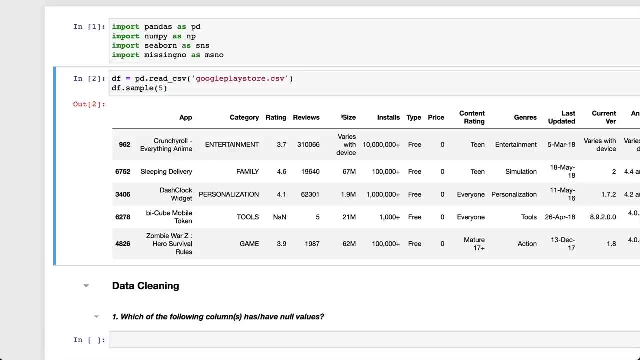 remember you're scraping data, you should be worried of issues in the resulting data, because I mean web pages are not extremely structured. they change a lot. So if you have a scraping job that takes time- because I mean we have a lot of reviews here- we have like 10,000 apps that were 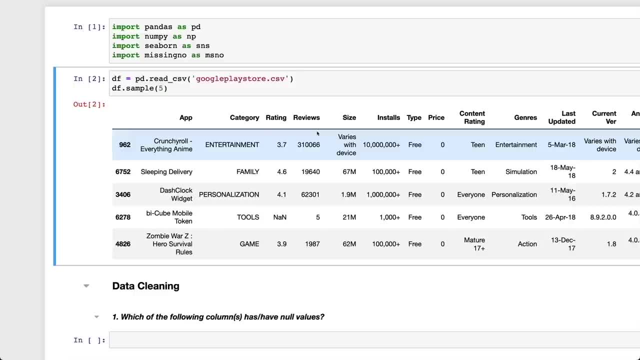 scraped from the App Store. that's gonna take time. it's not that you can just hit a button and that's gonna complete in just a second. it will. it might actually complete in a matter of weeks, because Google bans your IP- the one that it's scraping, of course. this is, I think. 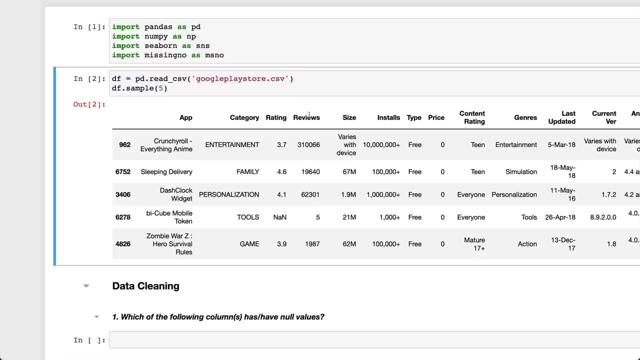 this is even illegal, right, but someone has done it And again it's gonna take time to scrape, and time equals that things might change, you might duplicate, you might scrape the same app two times, so results might not be ideal, to put in a way. So the way we are gonna, we're gonna. 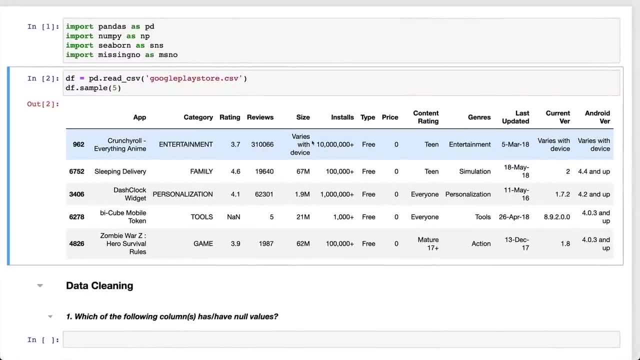 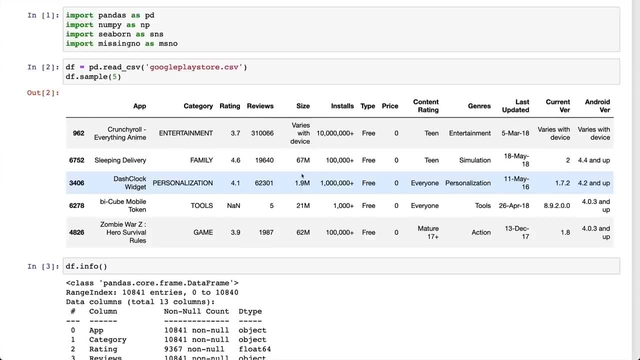 go with this is first understanding the data we're dealing with. So that's pretty much the first step. we're going to do dfinfo And we're going to kind of brace for impact here. it's like we know that there might be things going on wrong. So the first thing is we have 10,841. 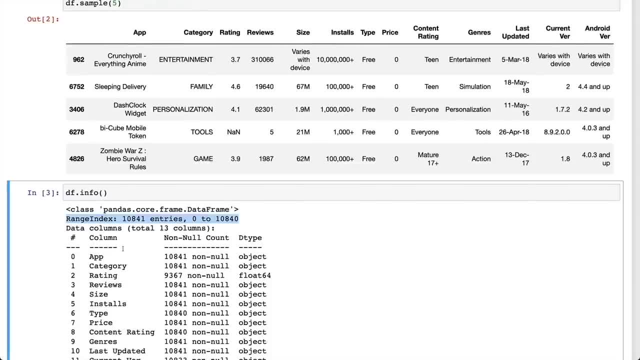 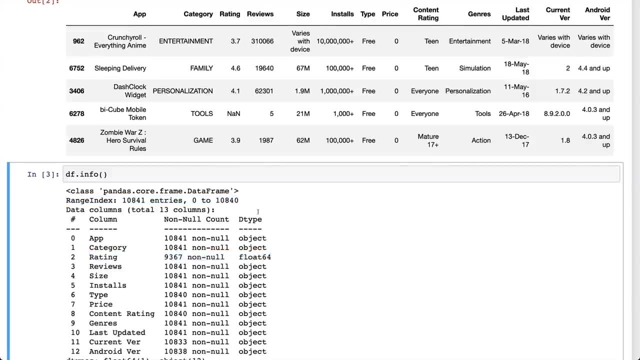 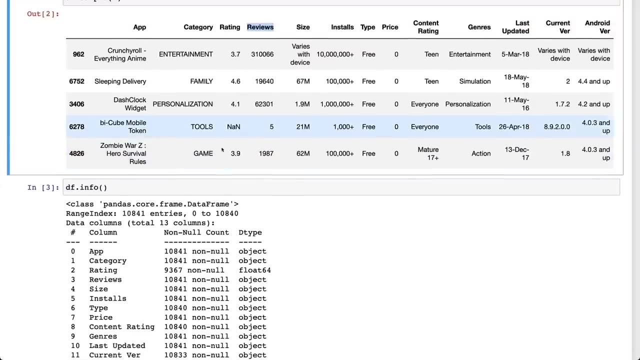 entries the total end number in the index and then we quickly see that rating has far less value. So there are no. there are no values here. Also, we see something like, for example, reviews right here, which should be numeric, and or rating, which see that rating is actually numeric. So this is a good. 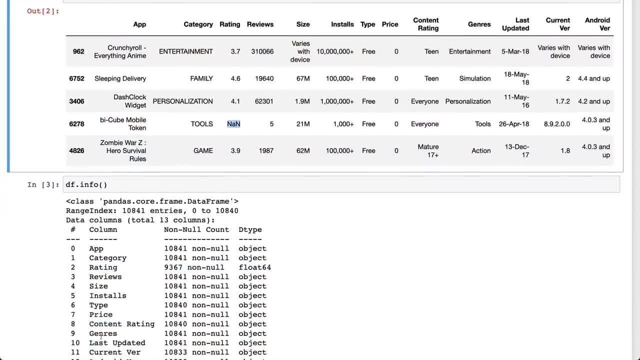 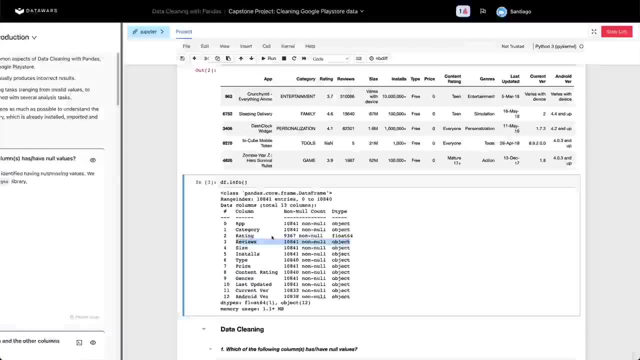 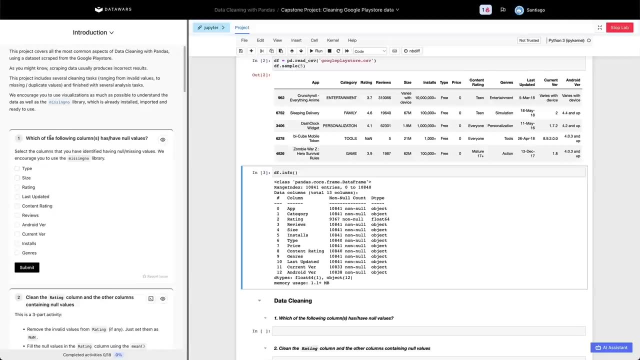 thing, but there are no values. Then we see that something like reviews, in this case right here, that is not numeric, it's an object, it's a string. So what's going on in here? That's a question we're asking ourselves. So let's actually get started with activities. And it says which of 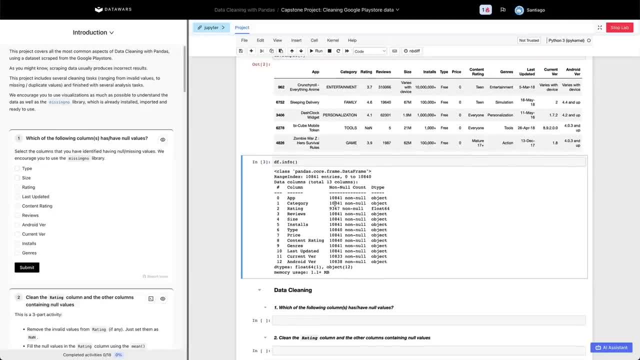 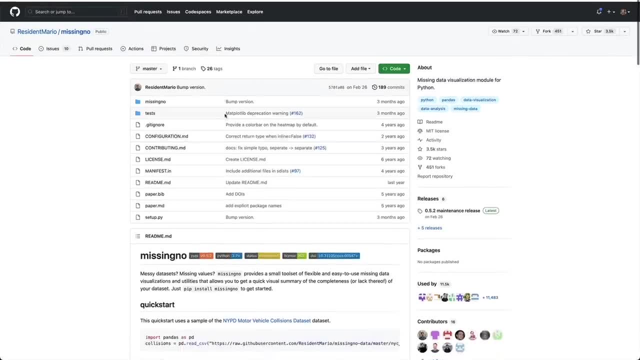 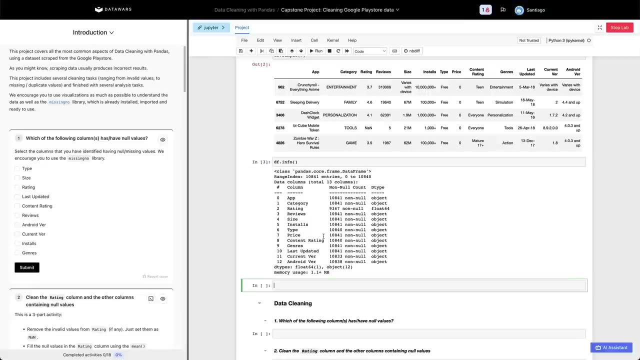 the column following column or columns have no values. we quickly saw that rating is one of those. We can use the missing NO library, this one right here, missing NO, just a- gives you a quick visualization And, as usual, I like to start my analysis with a quick visualization when I'm 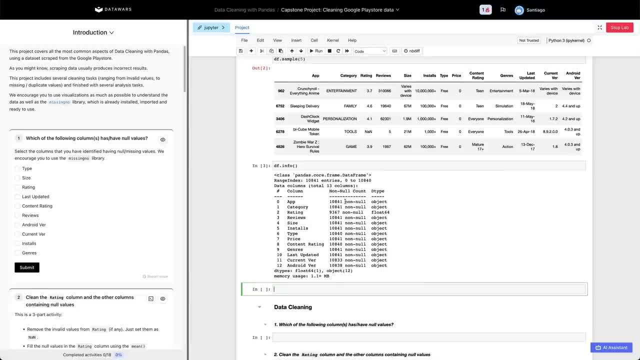 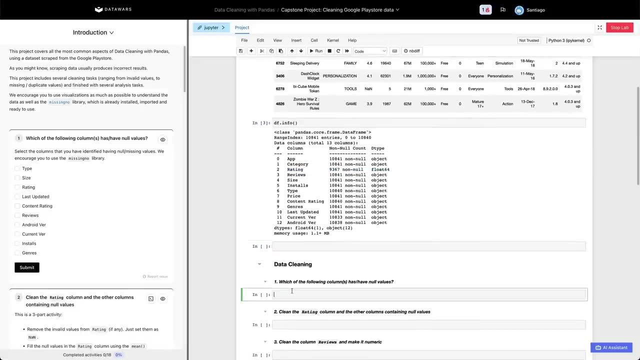 working with, with something trying to understand the data. a quick histogram box plot one of these missing values. visualization is recommended. The second stage is doing an analytical review of what's going on, etc. So let's do a right here missing. And now we have import. we have already. 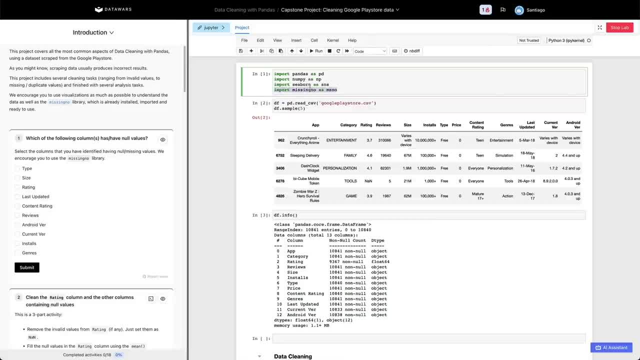 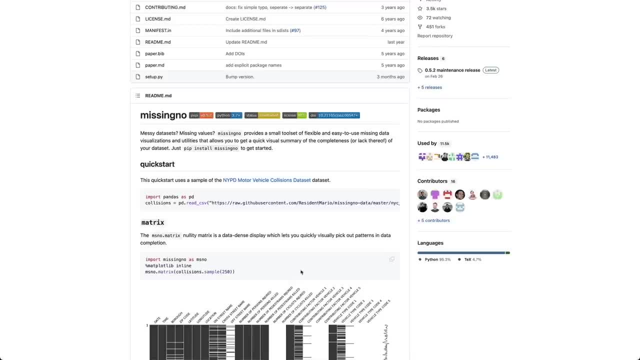 installed the app for you or the library and it's already imported here at mess. And oh, we're going to do a bar. matrix is the most common one. Like this one. I'm going to do a bar and we're. 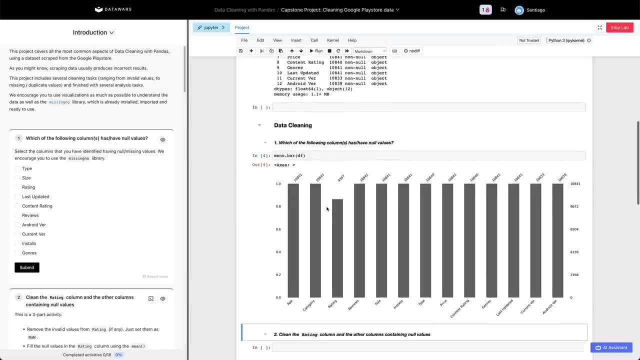 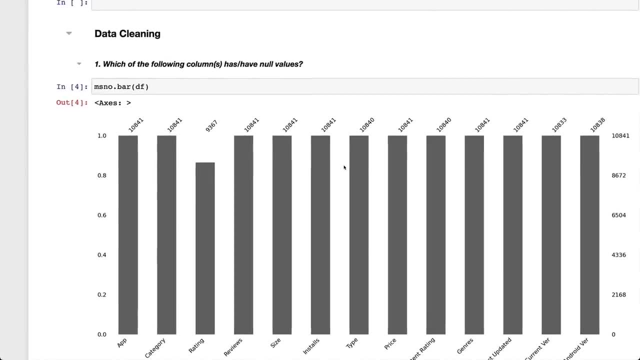 going to do the whole data frame, going to show us that very quickly, that rating. it has a good chunk of missing values right there. What else? Well, there are a few here, but it's hard to see with the bar and. 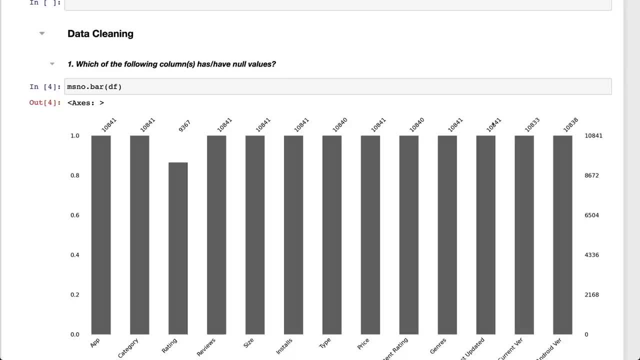 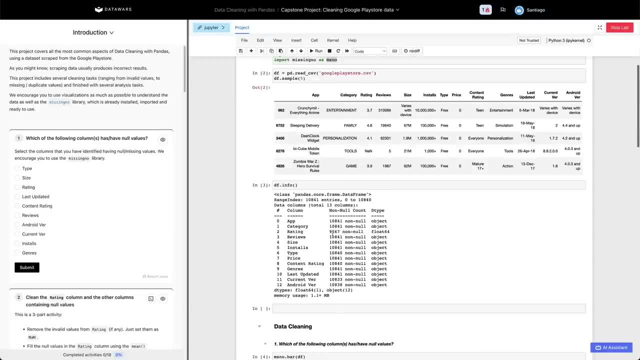 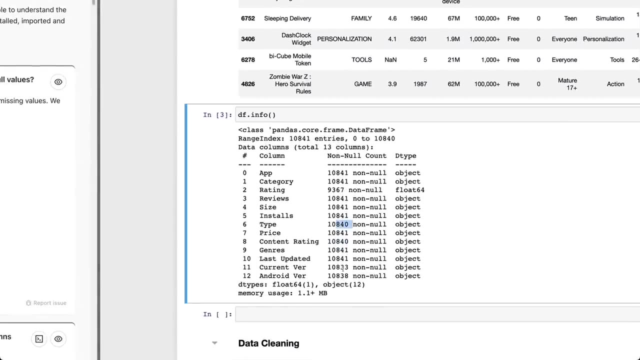 one here, 841 missing value here, And this is: this is hard to read because the bars don't help. So now we can switch to something analytical. And of course we kind of saw that because we have 1040, 10, sorry- 840, 840, 833, which we know that the full index has 10 841.. 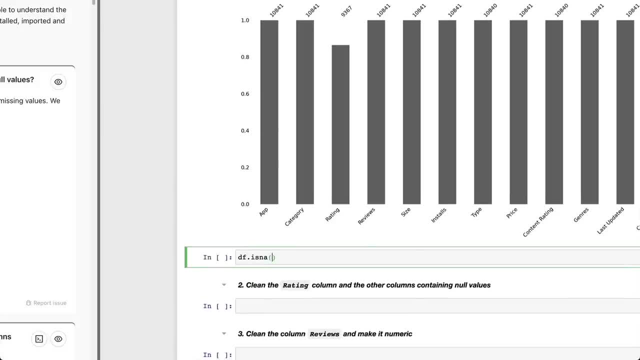 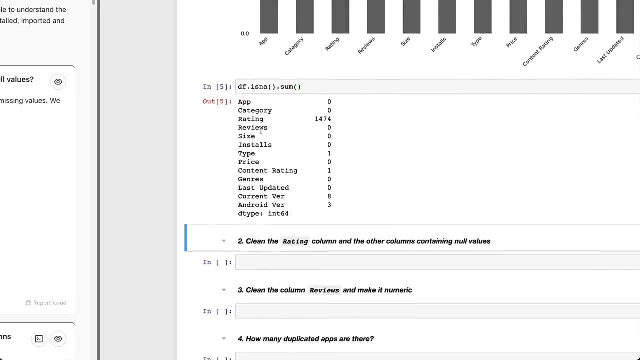 But to do so with an analytical way we can just do isn't a I can do no summon And that's going to give us- there you go really quickly- the apps that have the columns that have no values, And we can sort. 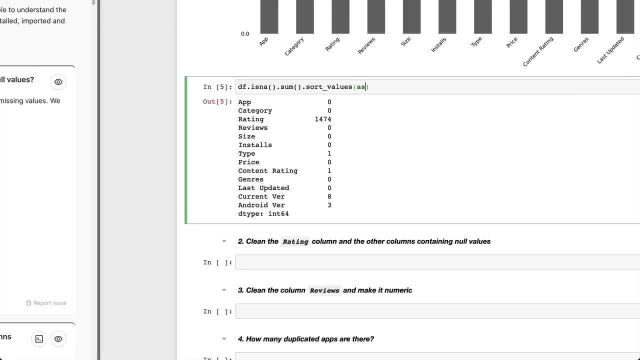 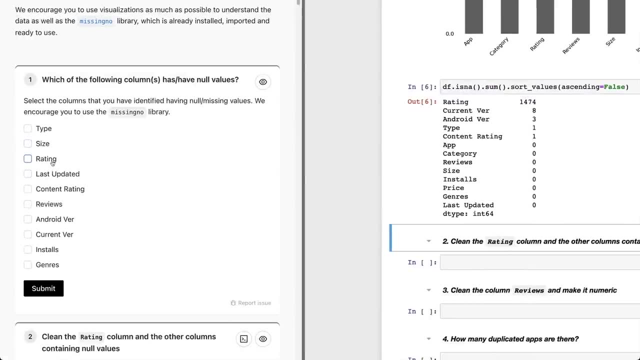 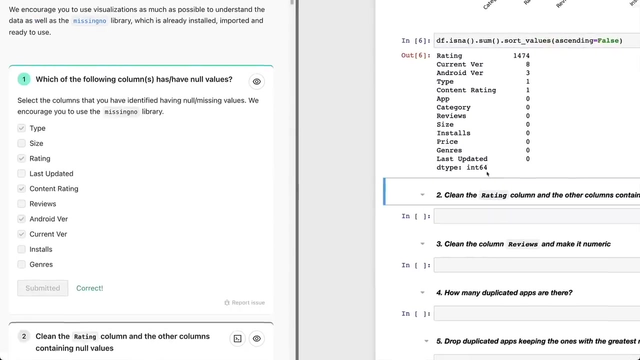 this doing sort values: ascending false. There you go. So we have here we can start answering rating, of course both versions. So type on Conson rating, type and count and rating. There you go. both are now cling, there you. 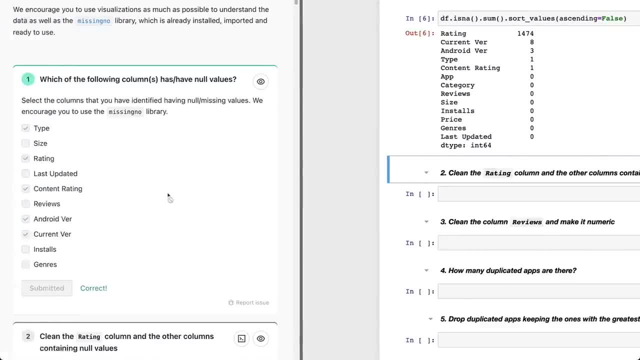 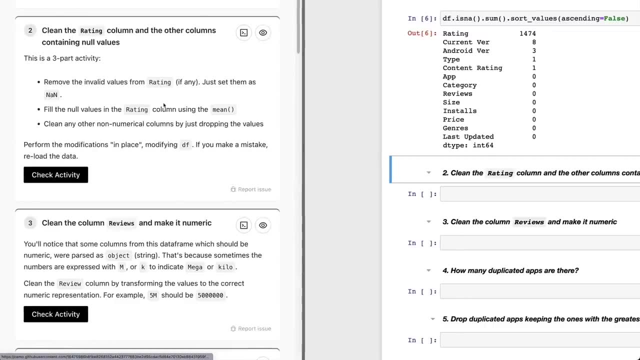 go are no values in all of them. So now second second activity, and this is again as usual. I encourage you to pause right now transfer by yourself, because it's an interesting one. So three part activity: remove the invalids values from rating, if any. just set them as n sending, okay. 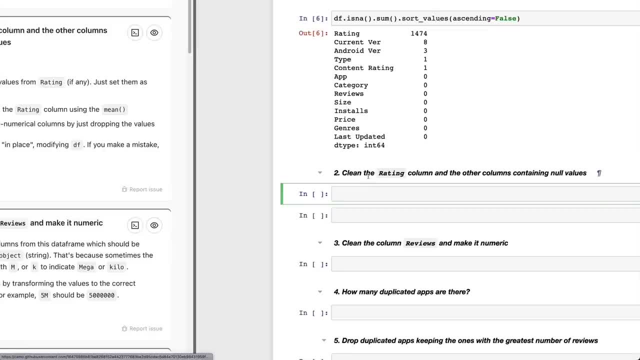 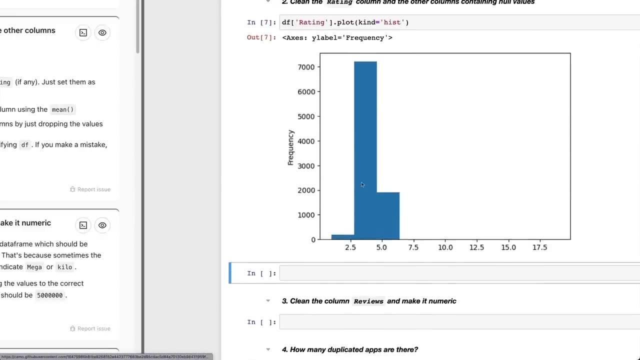 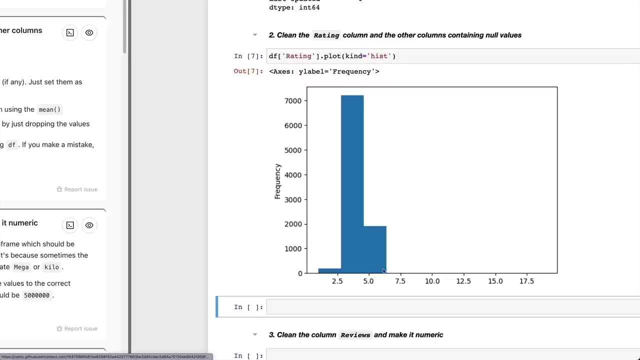 invalid value values. and let's take a look at rating. we're gonna do now again as usual. we can start with a quick visualization at rating dot plots, a kind histogram, real quick, and it doesn't look so. so might be okay, but we already see that there are some that are above five, which is of course not. 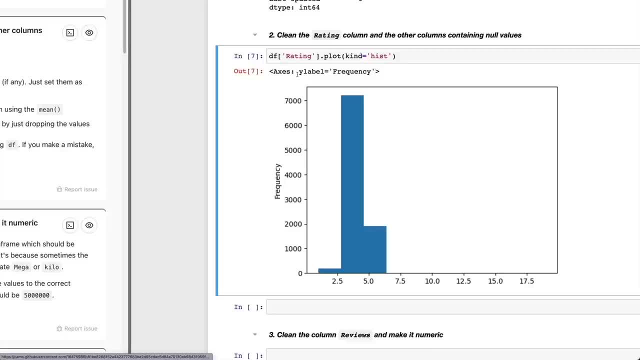 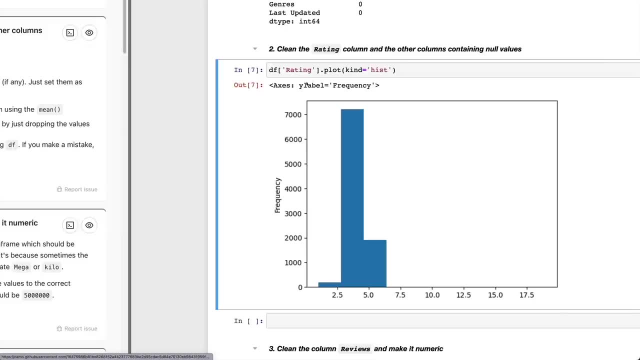 a valid rating- and this is my usual comment- you have to understand data, you have to understand the domain you're working with, to do correct data science, because we know that the rating of an app goes from like zero to five, or actually from one to five. so if you have anything above five or below, 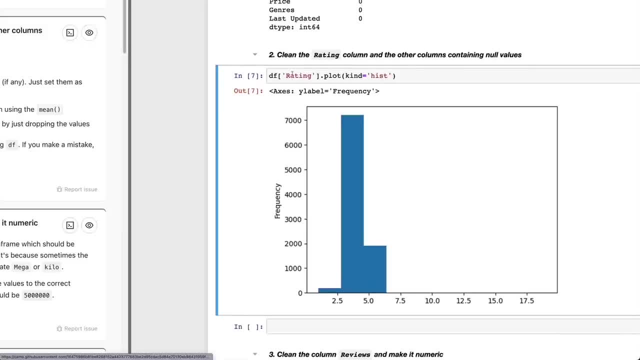 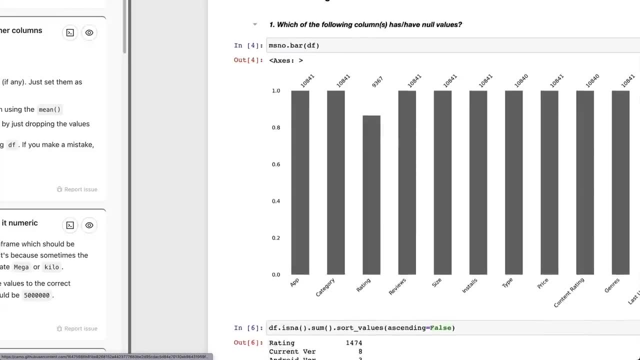 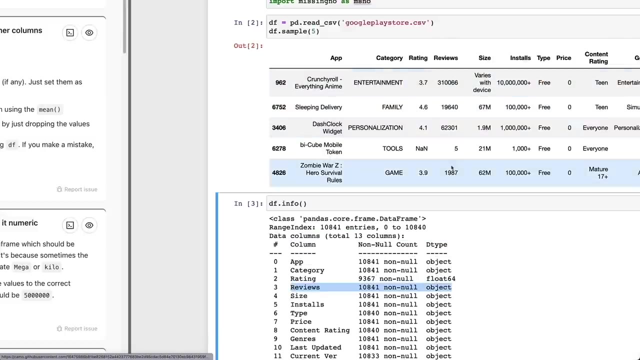 one, they'll be invalid. right and it's. it's a number. so the the column is okay in terms of the type. first check that. for example, we saw already that reviews wasn't, so reviews is an object. this is already here. reviews they it seems to be numeric, but then when we check the analytical version with info, we quickly see that it's not. 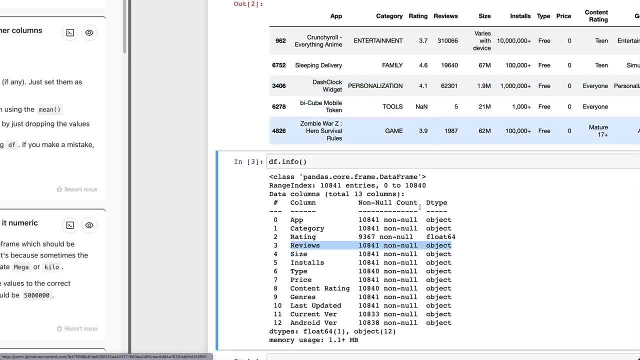 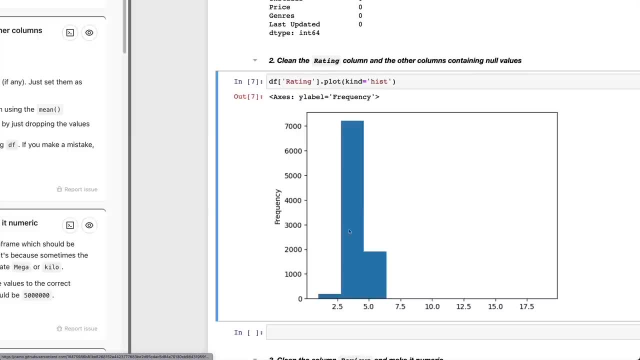 parsed as a number, so now it's raising suspicious. we're going to take a look at that later. but here, rating: we understand our data and we know that the top the, the maximum number that a rating can be, is five and this goes above five. so that's clearly invalid. let's turn this thing. 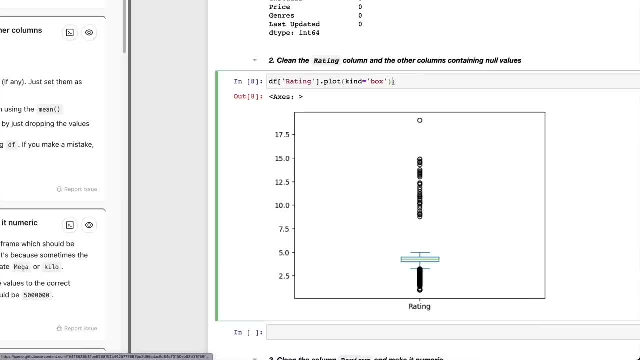 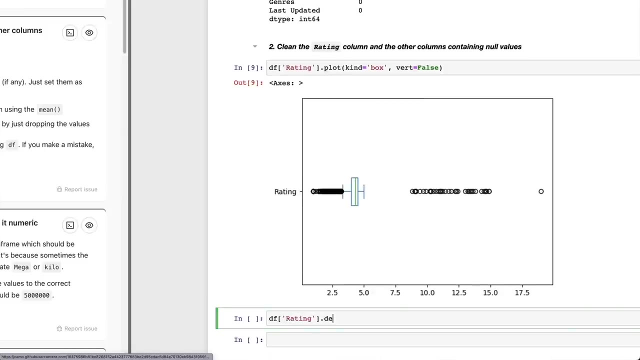 into a box plot. we're going to, we're going to do vert false, and now we can clearly see that there are a bunch of samples that are completely invalid. let's take it now to the analytical version. we're going to do rating, we're going to do describe. there we go and we have. 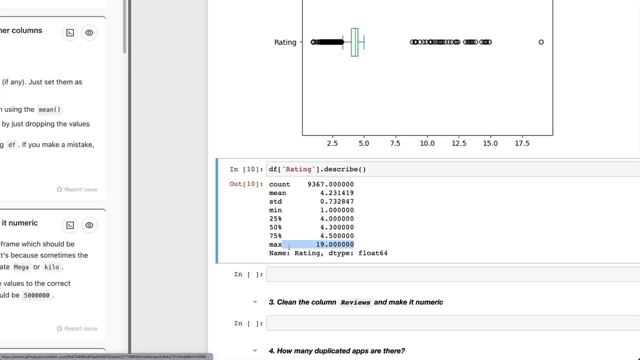 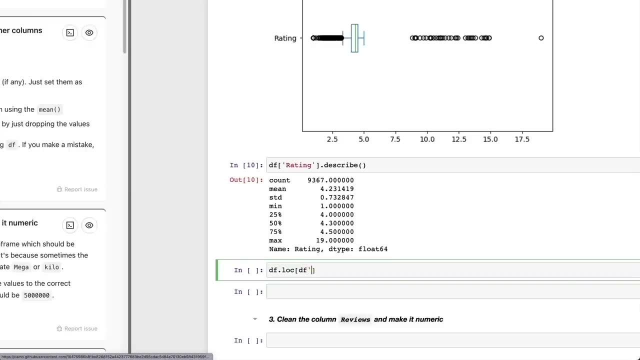 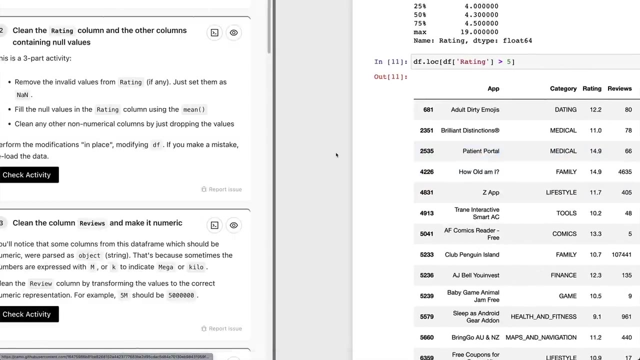 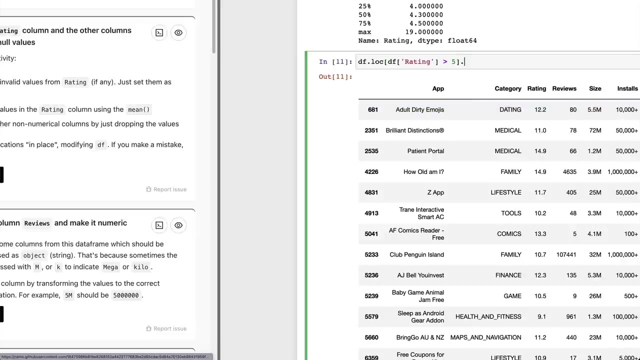 maximum value, which is uh 19, definitely invalid. all right, let's check it out. to say, dflog df at rating uh greater than five, and there are a bunch of apps here and we're going to need to claim these apps and the rules set them as nan. that is it. so here, um, we're gonna do these apps at rating. 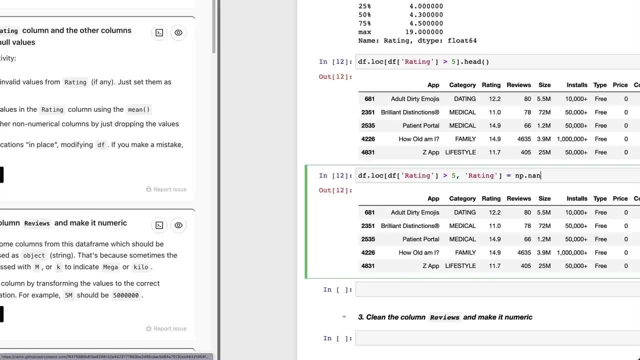 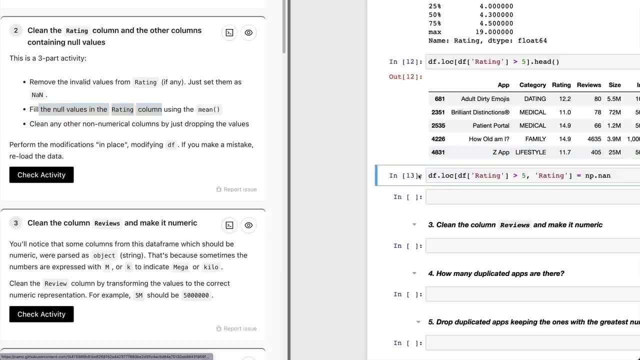 we're gonna do equals to npnan, that's it. but then it says: fill the null values in rating. so the ones we have just done and the other one, because there were like a thousand apps without a rating using the mean. so basically, what we're going to do here is we're going to do df at rating rating, uh, dot mean we're going to use. 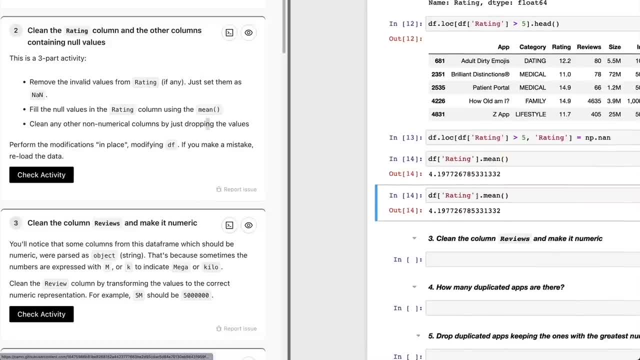 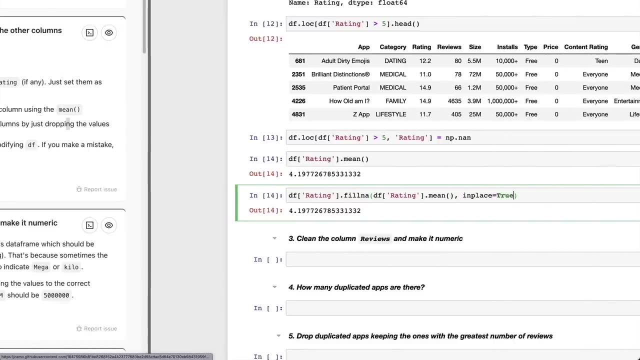 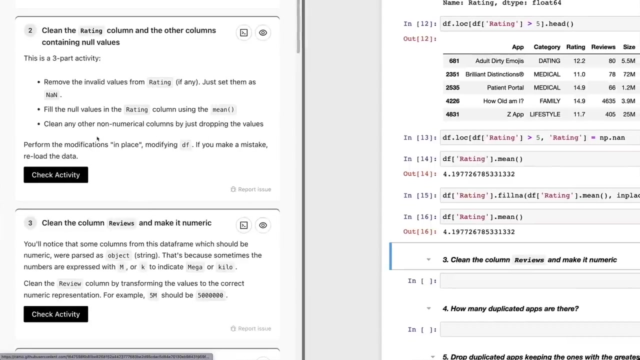 this value, i'm going to say df at rating dot fill. i'm gonna, okay, keep that rating dot fill na, with this value in place, equals true. and now it's pretty much the same thing. um, and now it says we can't check that yet. because it says: 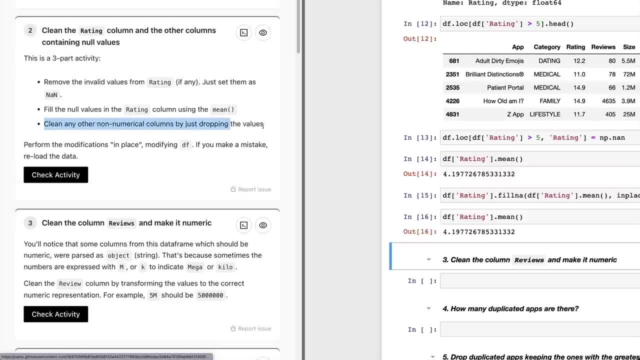 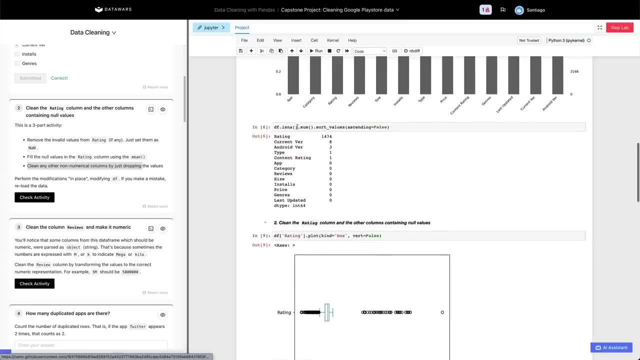 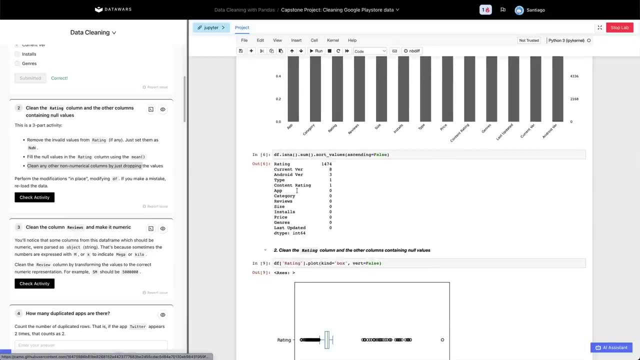 clean any other non-numerical, non-numerical columns, but just dropping the values. and this is understandable because we we don't have so many, so we're going to do df at rating, dot, fill na. we have 10 000 apps in total, like 10 841 apps, but there are apps like occurrences, rows, symbols. 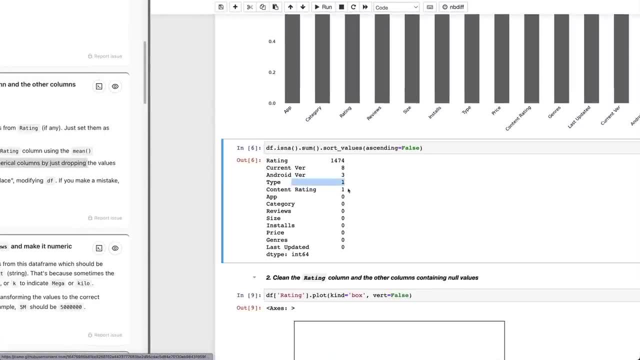 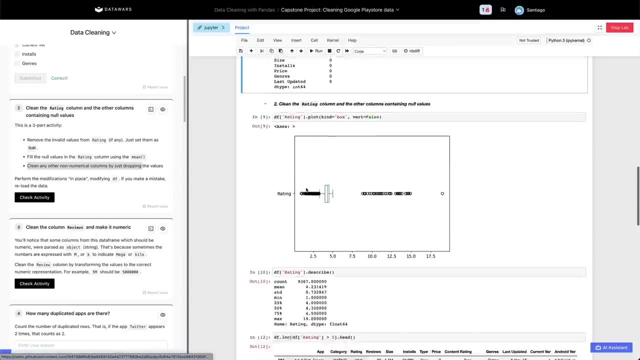 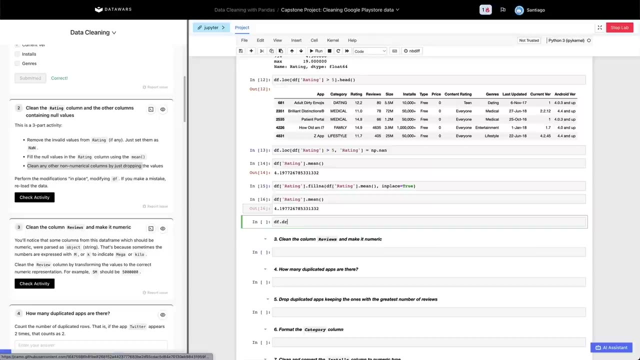 but there are only a handful- like 13- 13 apps that have either a missing version, a missing type, a con rating. so it's not that bad. we don't have so many missing apps, so we can just get rid of them. that's basically what this, this activity, is saying. so we're going to say df, dot, drop na. 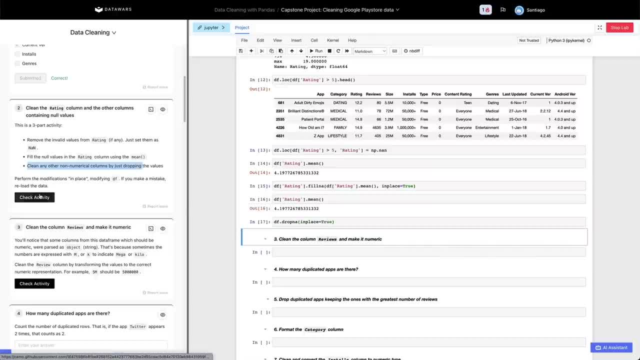 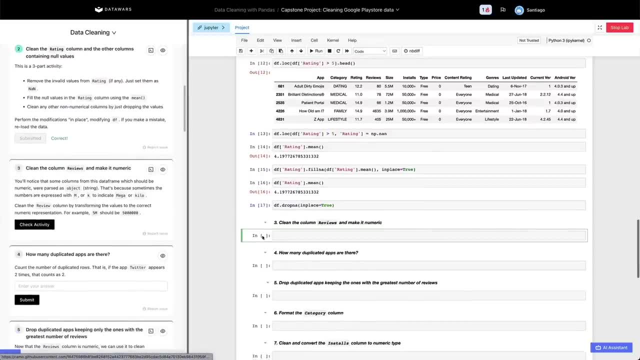 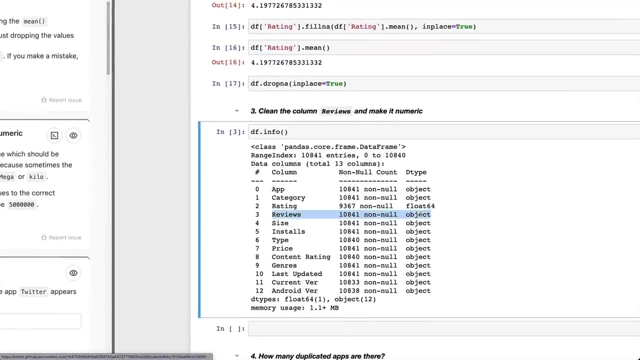 in place. true, that's it, and that works all right. moving on to the next one, reviews. we already talked about reviews. we saw that it's that it was parsed. let me take this right here. it was parsed as an object. pandas is going to try to parse any column as a as a number. okay, this is by definition. it's going to try to. 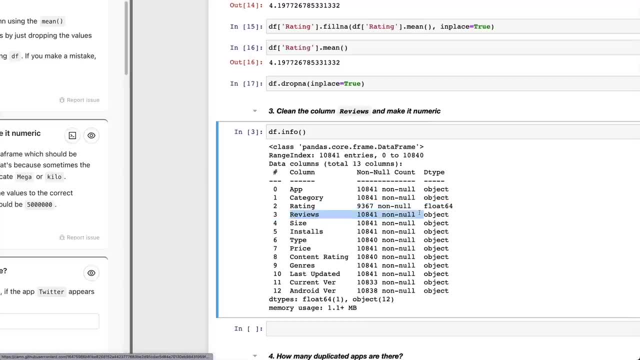 parse the column as a number. if it can't, because the column is not a number, they're string, they're invalid characters, it will just default back to object and that's it. that's exactly what happened here. but again the question is like where we take a look df at ratings. 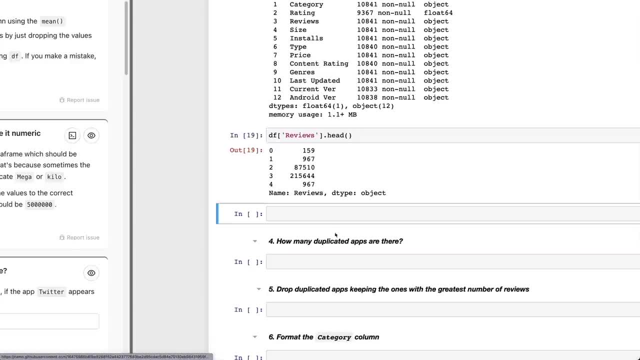 now reviews dot head and they look numbers as numbers, but it's an object, so let's check it out and see what happened. we can actually double check doing a to numeric to numeric, and we know this is gonna fail because somehow, i mean pandas was not able to parse the number, so there is no. 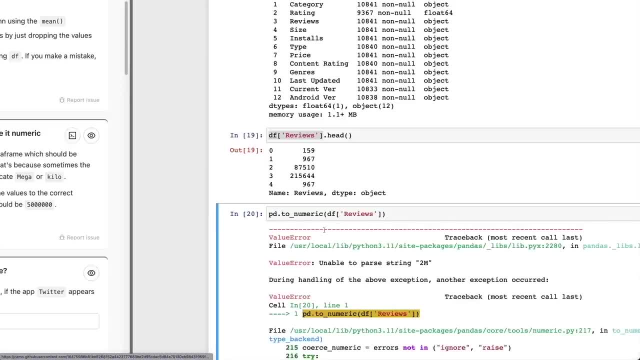 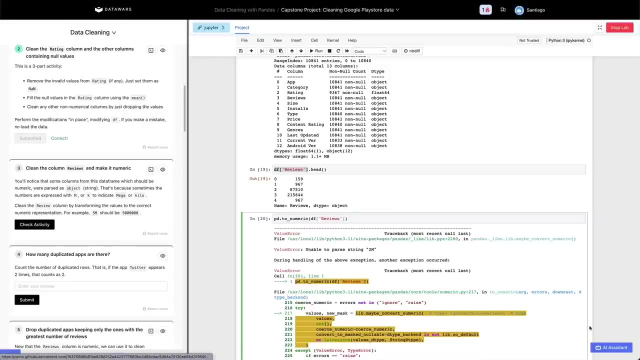 way this is gonna work. it didn't because basically there are values here are invalid. so somewhere in this list of ten thousand apps there will be um values that are not fully numeric and let's explore for that. a good way to explore for that is- i have my ai assistant here- that i asked earlier. for example, what is the syntax of pd? 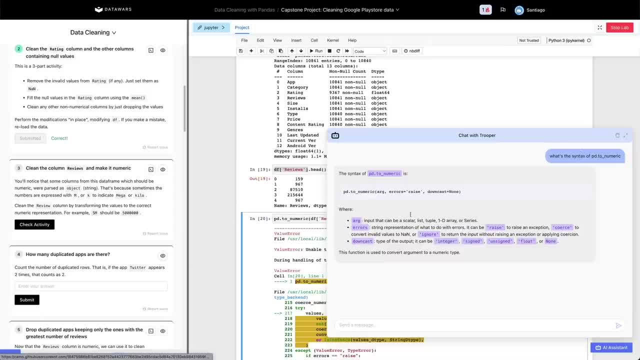 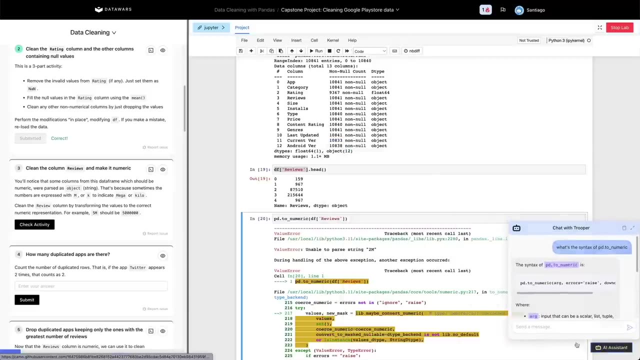 to numeric. when i was just checking this, this project to resolve, and it's telling me that there is this method which is: i can pass an optional attribute which is: errors equals squares, right here, and that's gonna, instead of raising errors with a you know loud red message, he's gonna turn the no values as the evolved values, as nams. so basically, that means: 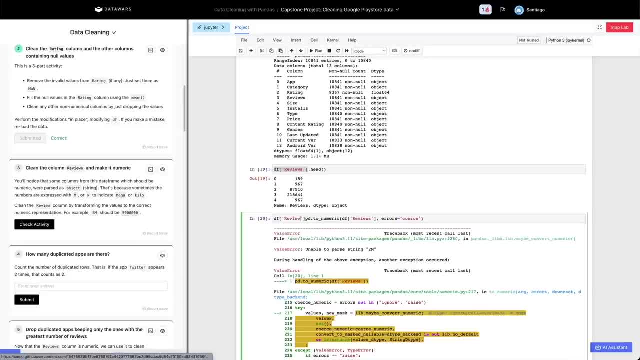 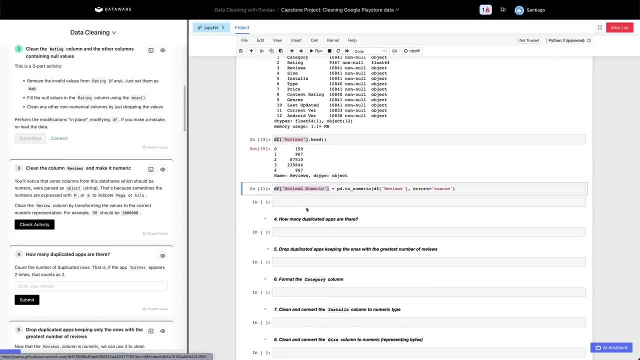 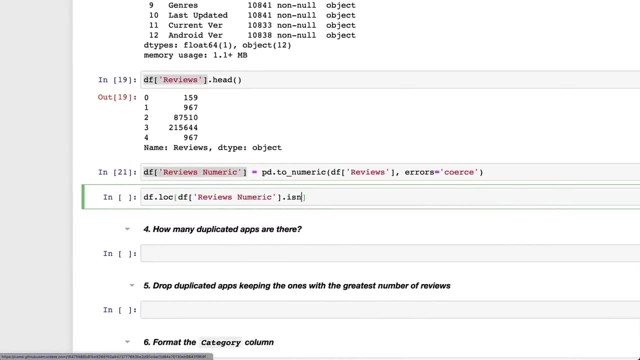 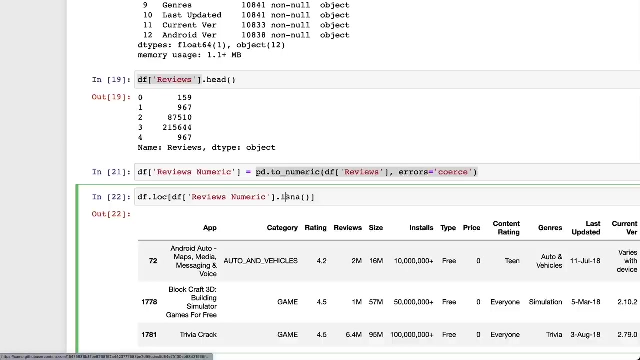 we can do that. i can create a new column reviews numeric. that is a result of that, and now i can say: dflock, show me the rows in which these row they have. this column that i have just created is nan, because that means that wherever there is a non-value, no value missing value in this new column. that is because 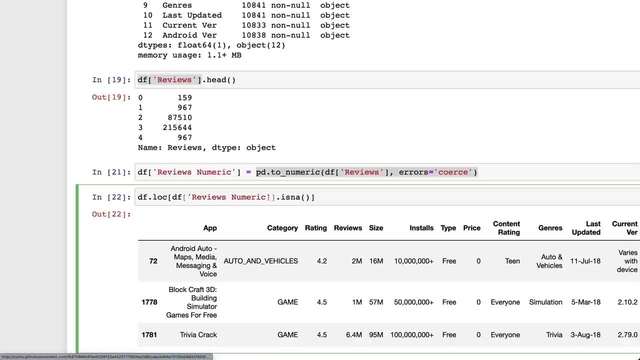 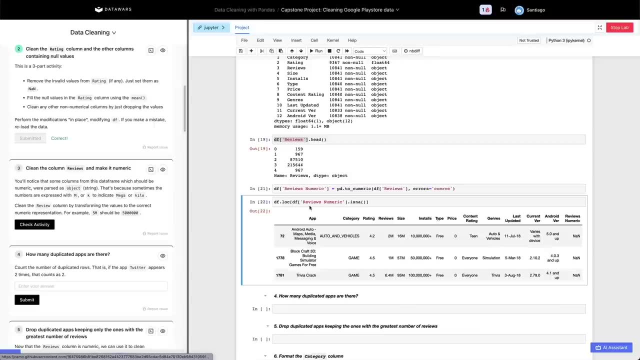 there was a number there that wasn't that pandas couldn't parse, and when it couldn't parse it, it just assigned nan, and that is basically what is happening right now. so we can see that this is an right here. reviews: numeric is an, an, an, an. we can take a look at the actual reviews and we see that. 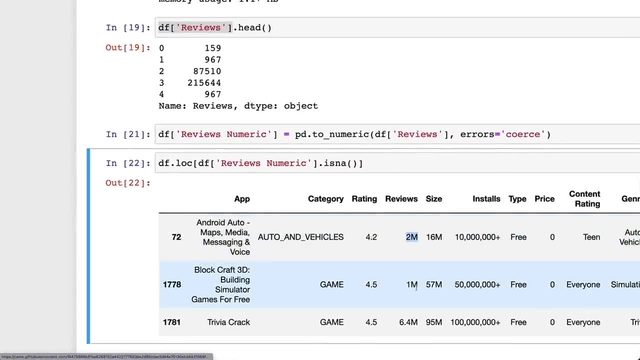 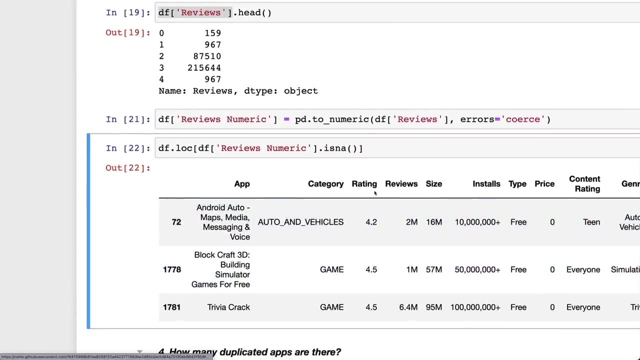 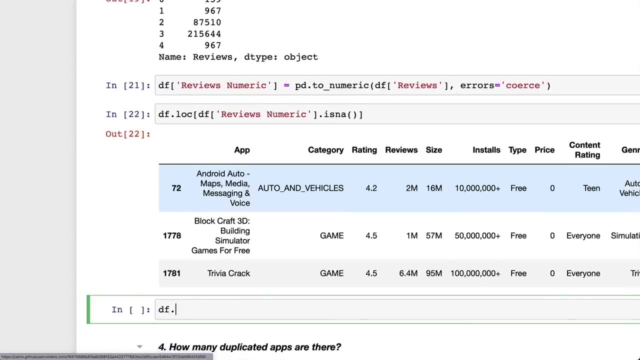 there is this m value here, symbolizing for millions. So 2 million, 1 million, 645 million. we want to turn this thing into numbers. To do so what we can do is df ads, let's say df dot log, df ads reviews dots. I could have just on df dot log at 72.. Here we can do, I'm not. 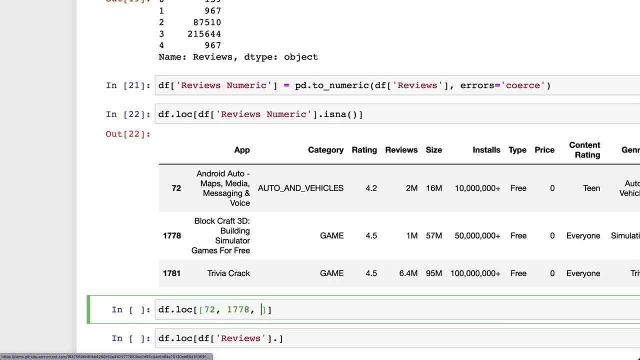 gonna do it, but I can just do 178, 1781.. And I can just do 2 million, 1 million ad reviews, of course, here reviews, but of course it's not very scalable. So I'm going to do something else, just just. 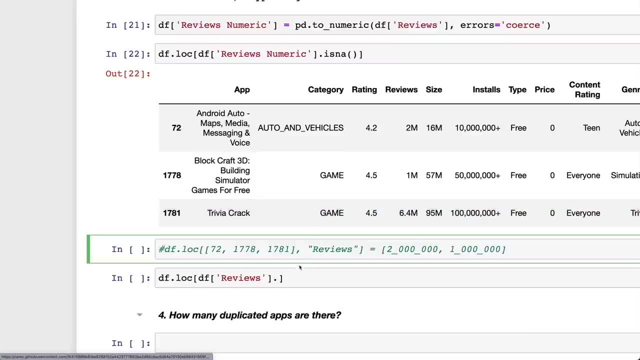 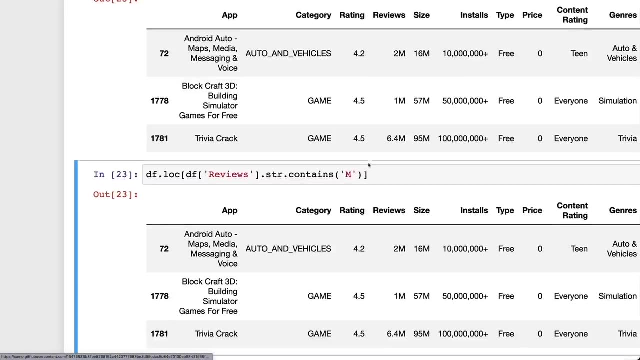 making automatic to put it away automated, like it's going to be completely generic And this is what we're looking for. So, basically, find me all the reviews that contain contains an M Right. so these are the invalid values. What are the reviews now? 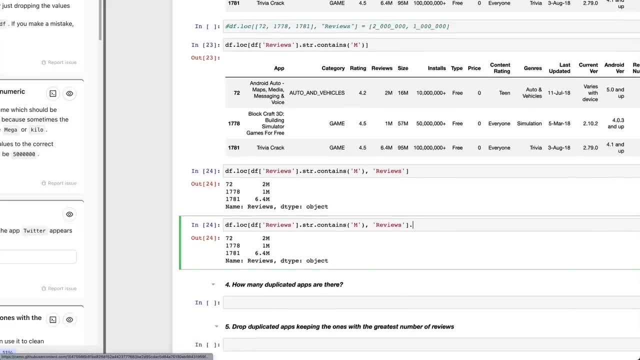 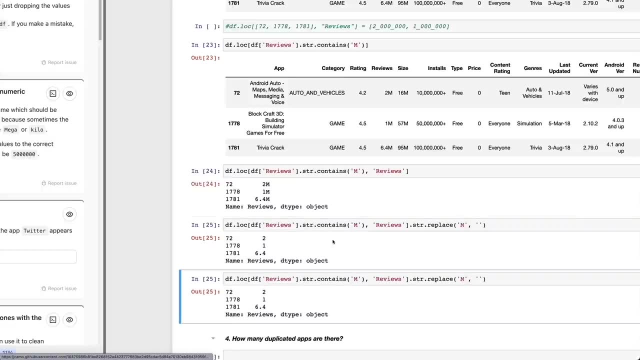 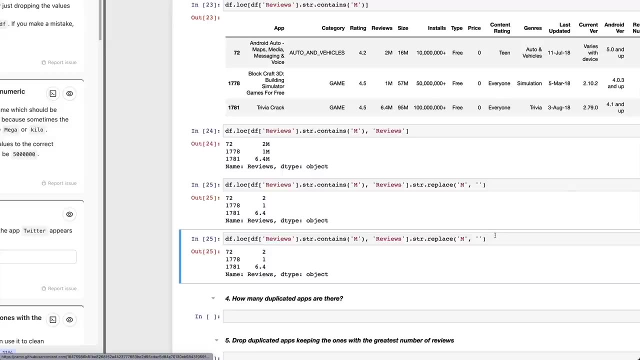 There you go, And now what we can do is dot, str, dot replace. we can do m with nothing. So it's going to remove the m and I'm doing this step by step- by the way, I could have just done in just one line, but I'm showing you a step by step resolution. And basically we can now turn this thing into numeric p, dot, two numeric of this thing. There we go, But we saw there was 2 million, So we need to multiply back to 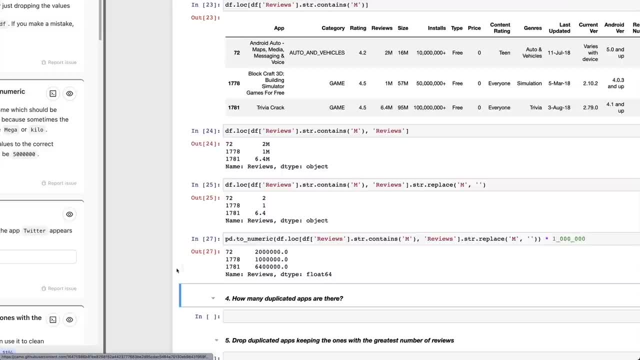 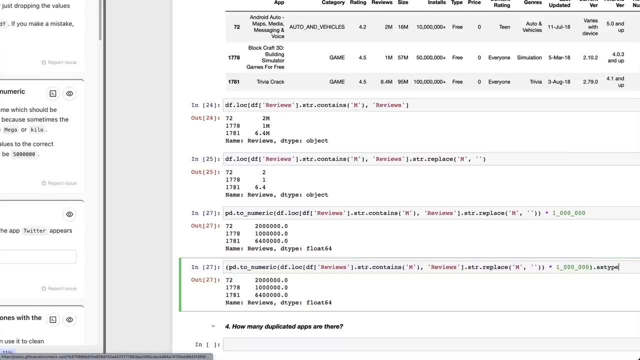 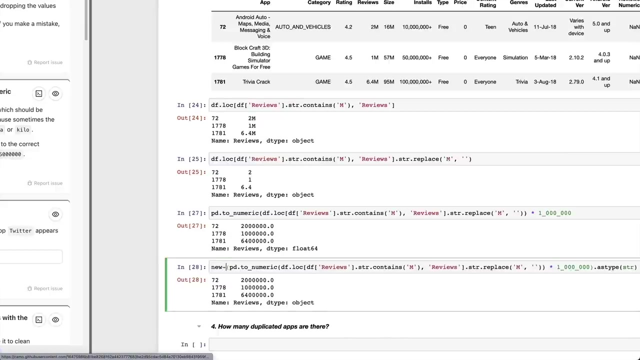 1 by 1 million. We have the value, But we want to assign this thing to the reviews column, which is a string type. So it's usually recommended to turn this whole thing back as type str. So we want to make it a string, Because now we can take these values: new reviews, new reviews, And there you go. 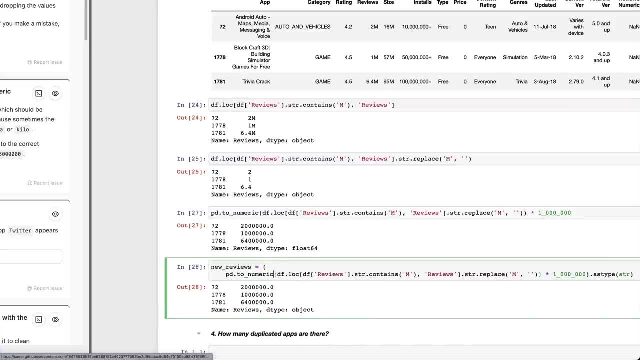 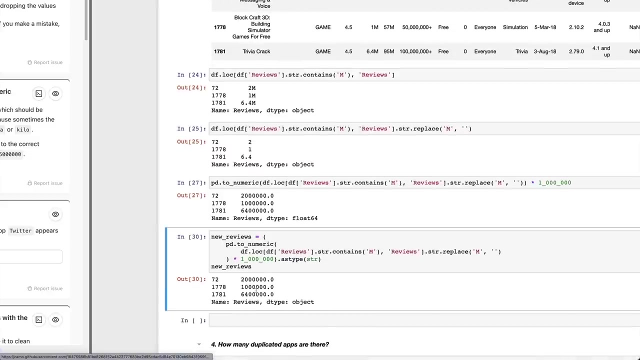 We have to break into a new line, break into a new line. There, These new reviews did it work? Let me put it right here: New reviews There. These reviews basically want to assign them back again to which one? this: 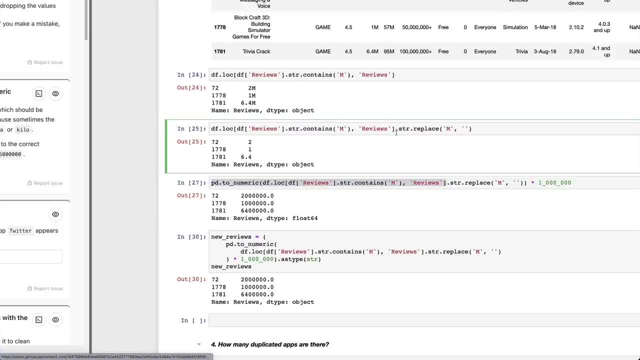 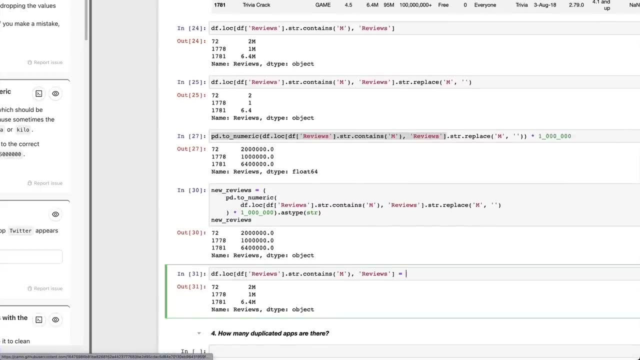 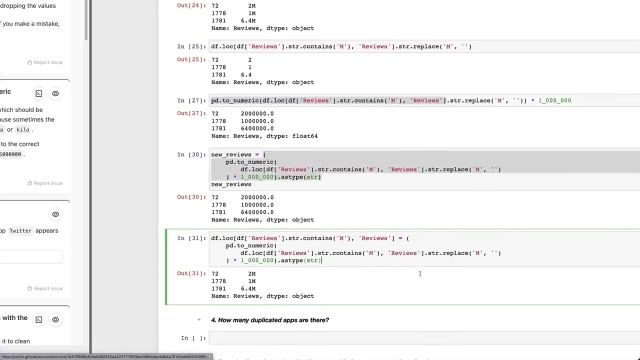 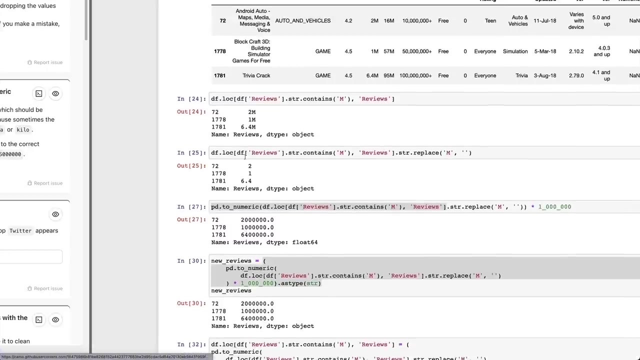 is No, this. I'm already making a mess of myself These results. So basically, when I get these things, I want to assign it the previous value. right, So we can do. do you want to do the whole thing? Let's do everything just one line, as I promised. We're gonna do that. Let's see if it works. So now we can look again for this column, these apps. 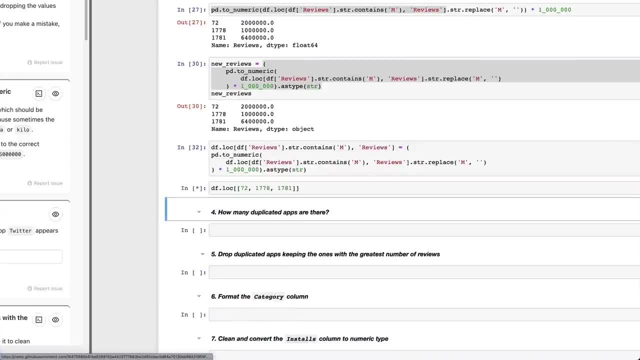 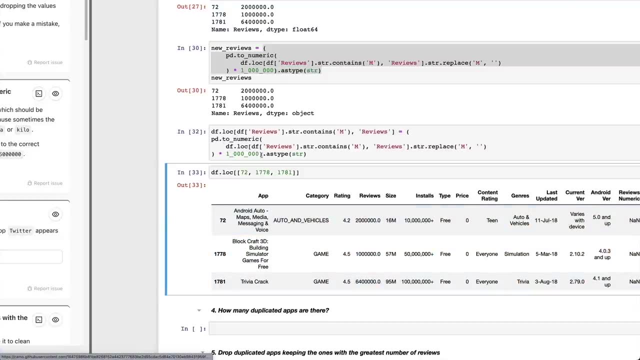 And let's take a look at the whole row. I guess now that the reviews have been correctly cleansed, But so far this is just a string right? We have not, which is, we have just fixed the three occurrences which we could have fixed 1000 occurrences, because, again, this method is pretty generic. it works for pretty much anything. We are going to turn the whole thing now to a number, So we're going to do PDF add reviews. Let's check first. 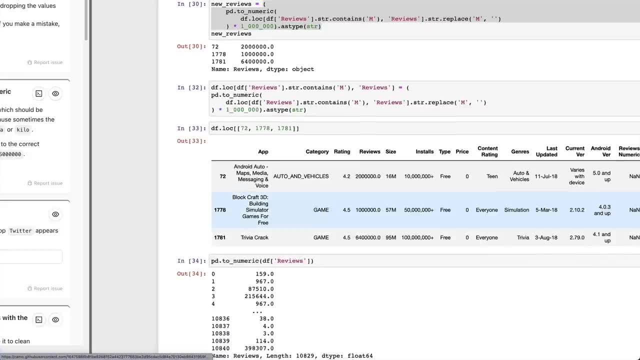 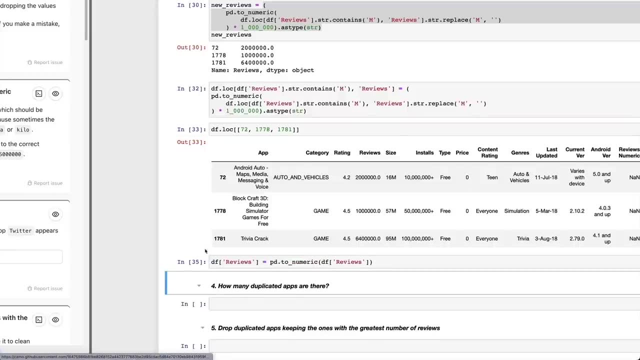 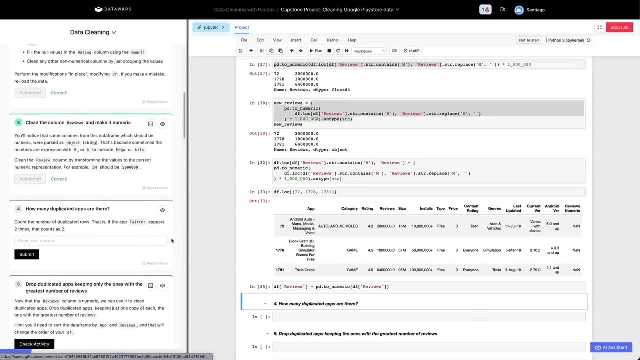 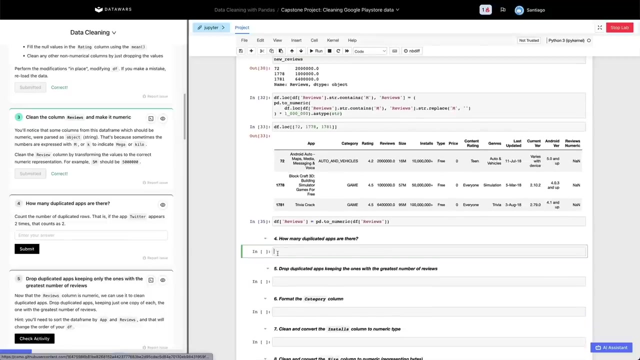 To numeric. There you go, It worked, So it didn't raise an error. That is good. We now can assign that back to reviews and check our activity. Finally, finally- and it works Okay, moving forward to the next one, How many duplicated apps are there? And in this case, is asking us for the total duplicated apps. Let me do a quick recap of the duplicated method. Undo duplicated apps. 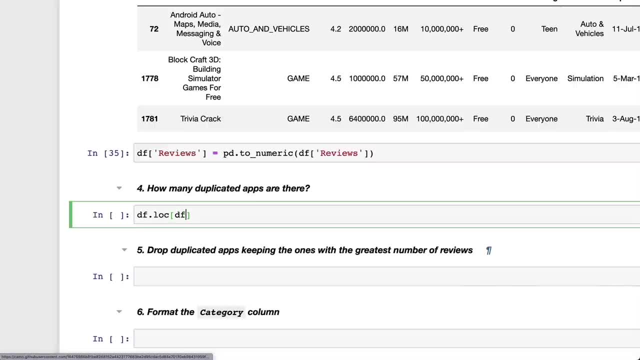 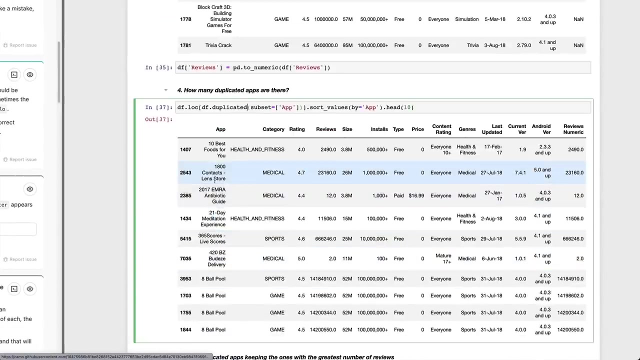 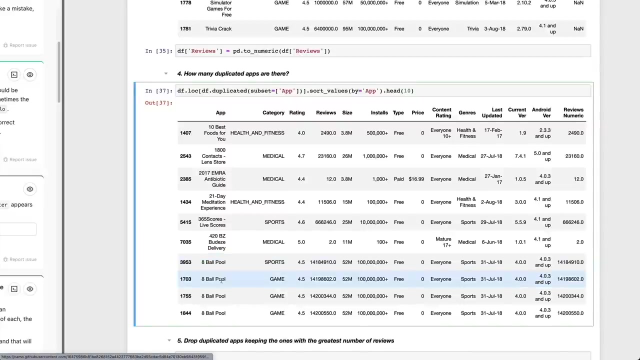 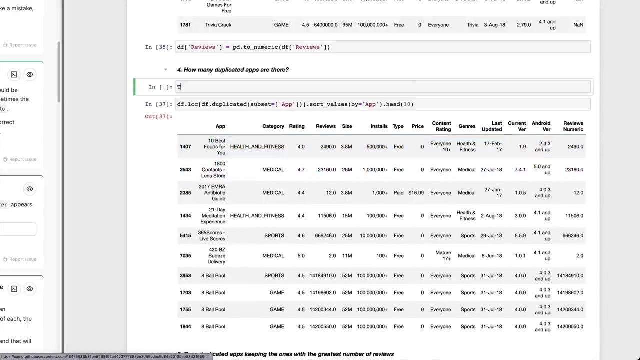 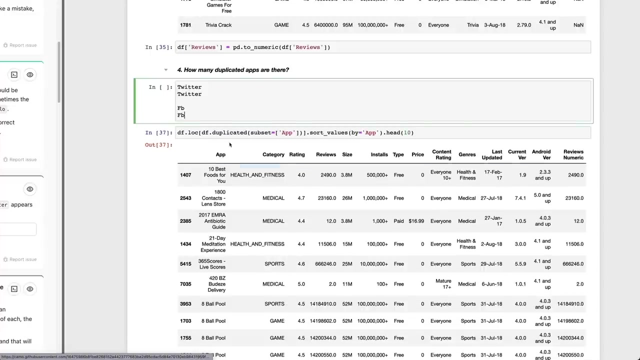 And df dot log, df ads, duplicated subsets, up sort sort values by up, And then there you go, we have all these apps out. here is the occurrence that I'm looking for. So basically, here, eight ball, pull, um, so what it shows by default, if you have, so, if you have, for example, Twitter, Twitter, you have Facebook, Facebook. what this method is going to show you is only this one is duplicated and only this one is duplicated. That happens because, I mean, this is the real one For pandas, the first occurrence like the real one. the second one is a duplicated one. 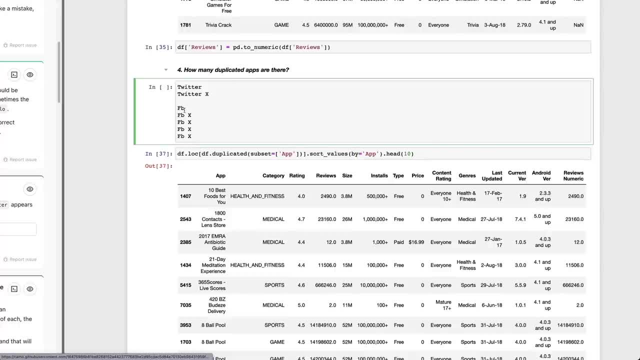 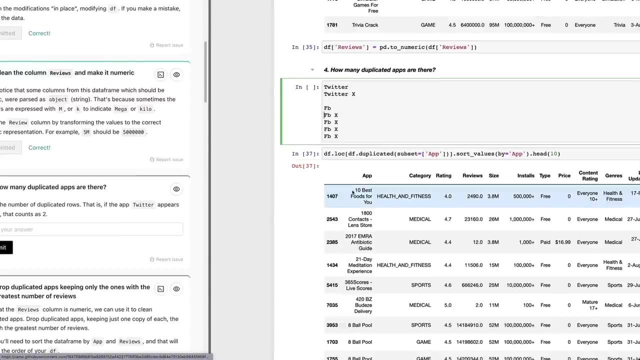 The same if you have multiple apps. So if you have six occurrences or five, whatever, 12345, there is one good and four are duplicated. That's basically what pandas does by default. In this case, activities asking us for the dip for different behavior is saying: if there are two occurrence of Twitter, that should count as two. you want to mark like Twitter is here is two times duplicated. To do so, what we need to do is pass a. 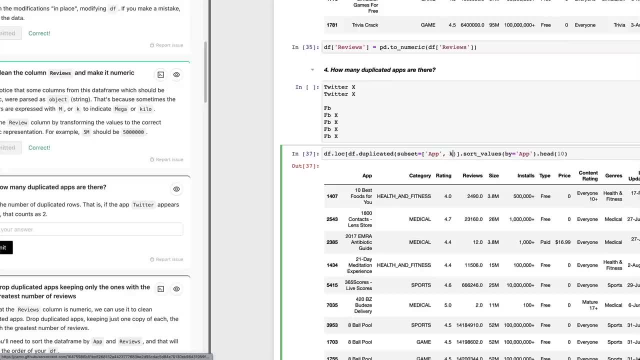 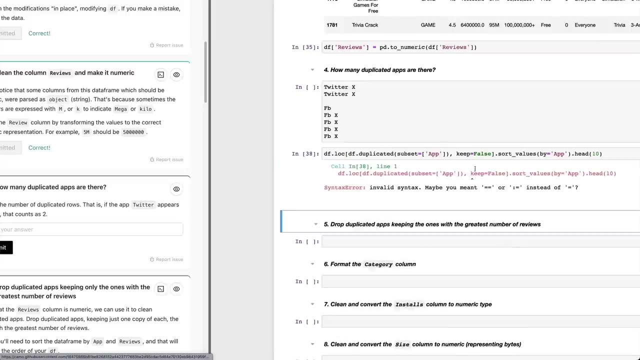 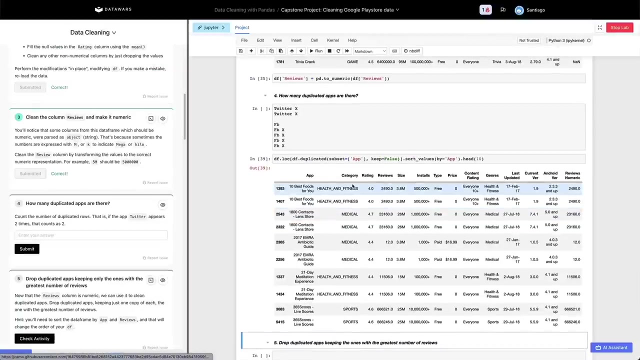 parameter, which is keep- Sorry, I already made a mess- keep faults And somehow- because that should go inside the parentheses- There you go, And now it seems that it's a little bit more interesting in this case, because we have every occurrence of the given up. 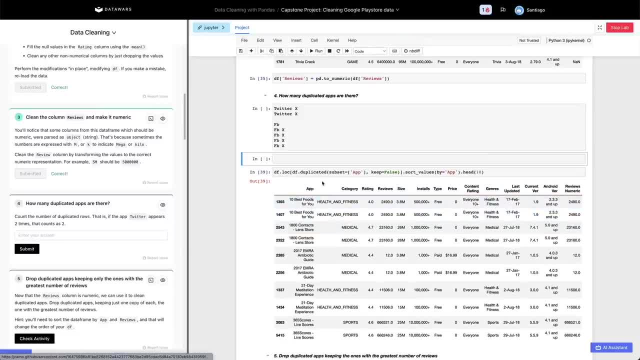 and there is also one more thing to comment here- is that let's say, you have this app and you have the number of reviews, which is 19 100 for one of them and the other one is 19 100. there you go. so these two rows for pandas are completely duplicated, these two rows. but if you 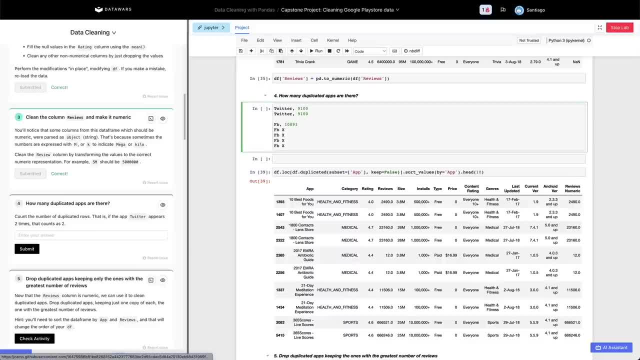 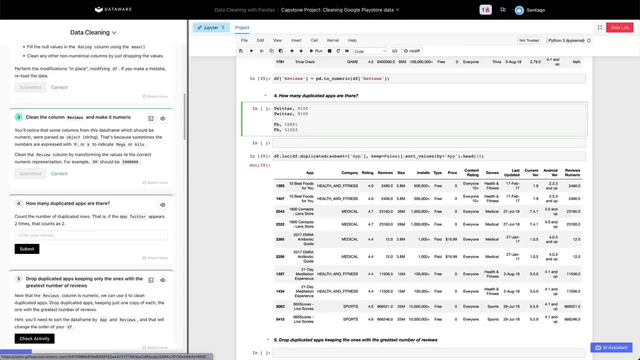 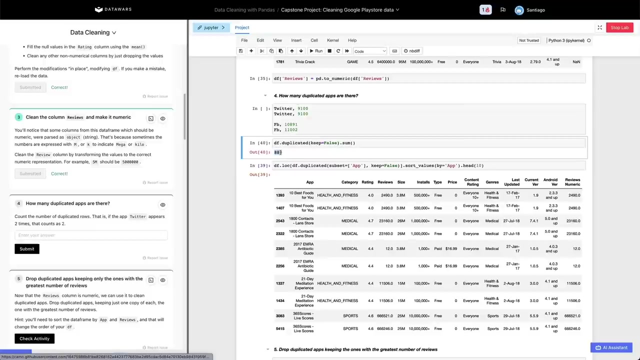 have something like, i don't know, 10091 and 11002. if you have these two rows right there, if you just do df dot duplicated, let's do keep false. some by pandas, by default is going to tell there are 18 800. sorry, 880 duplicated rows, but for 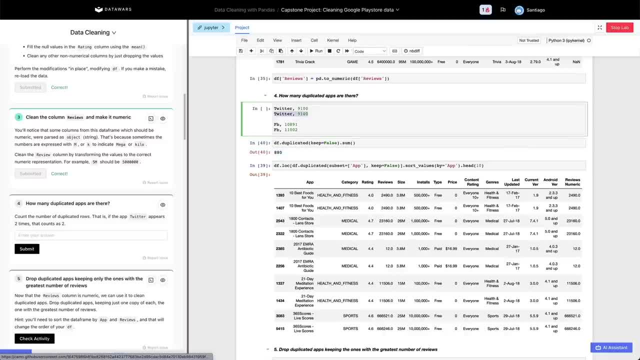 you this to be counted as duplicated row, the whole thing has to be the same. So in this example this would be just two. These two are duplicated, but these two here are completely different rows- to me That's what Panda says- because the values are different. 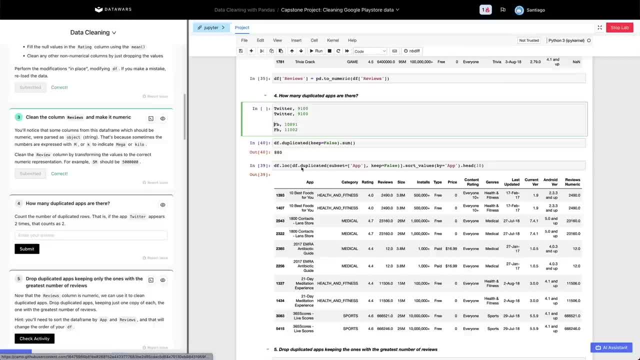 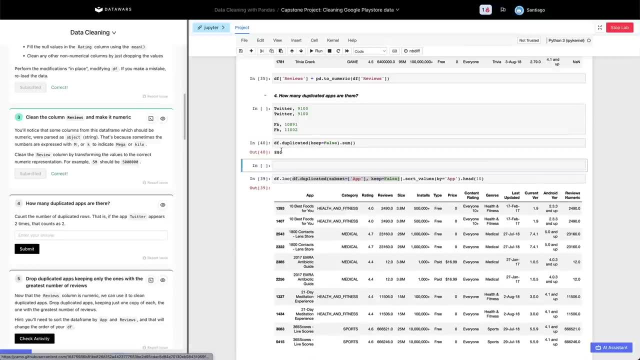 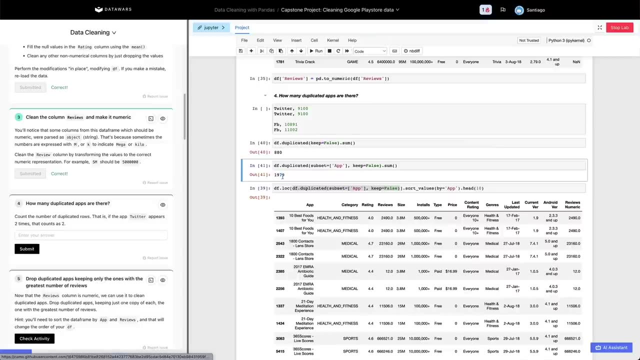 For us to say: we wanna count duplicated apps. we need to do these subsets app, right? So let's do thoughts, copy this thing. Now we're gonna do there, And now we can count 1,979 apps Because again there are some rows. 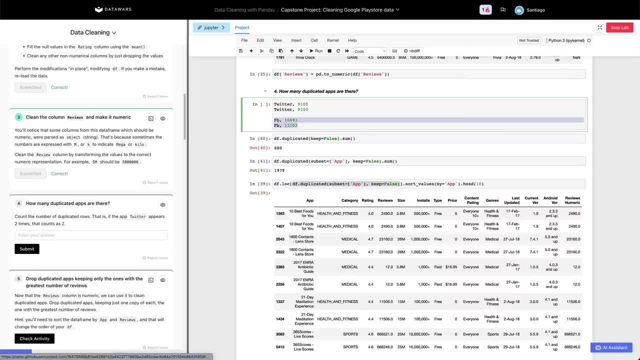 that are completely the same. There are some rows that are different, at least in some other column, but the app is the same. Let's actually try to visualize that I can say, and it might take me a while, and it's not this thing. 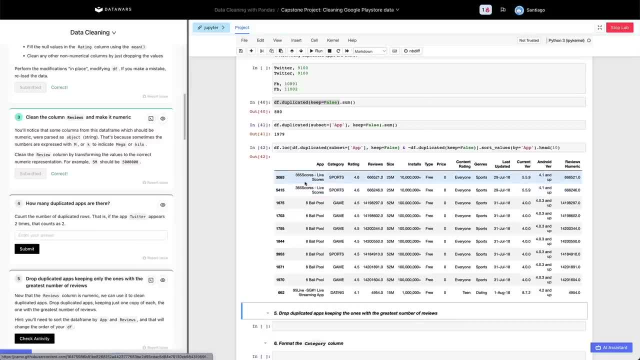 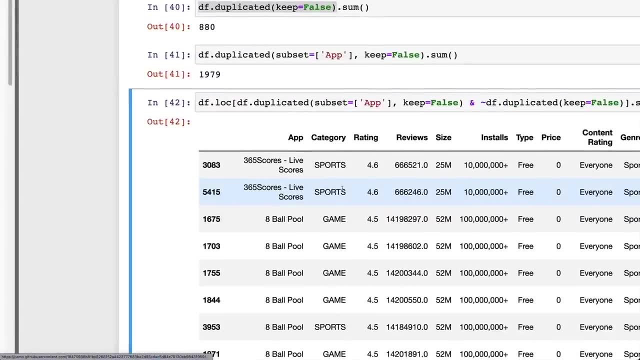 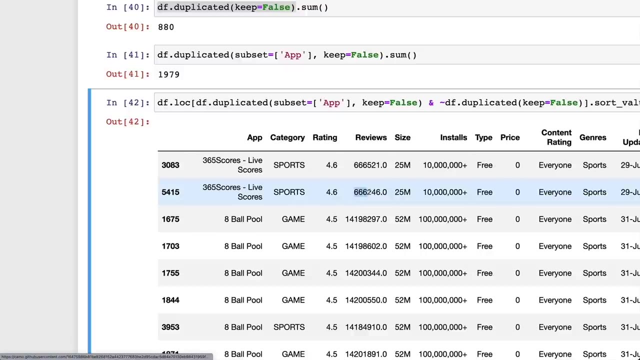 There you go, that works. So, basically, these are the apps that are duplicated, but there is something different between these rows. So, for example, between these two rows there is something different, and it's here the reviews. This one has 666-521, and it has 666-246.. 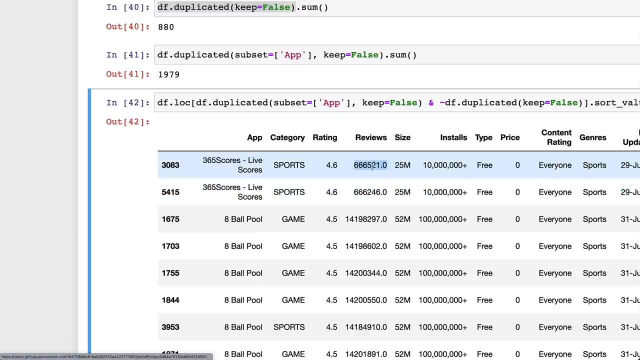 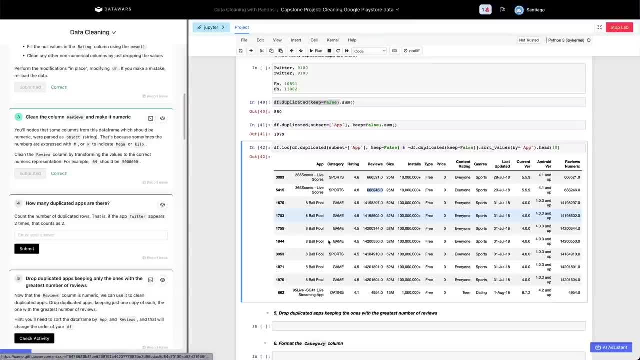 So this one has more reviews than the second one. And again, remember where the data is coming from. It's coming from the scraping process. So there is a chance that this app was scraped two times at two different points in time And, of course, we have a duplicated rows. 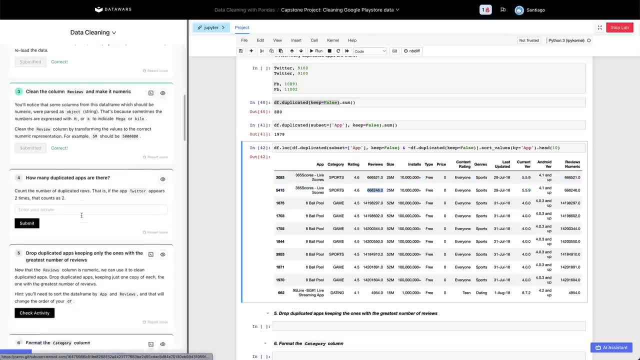 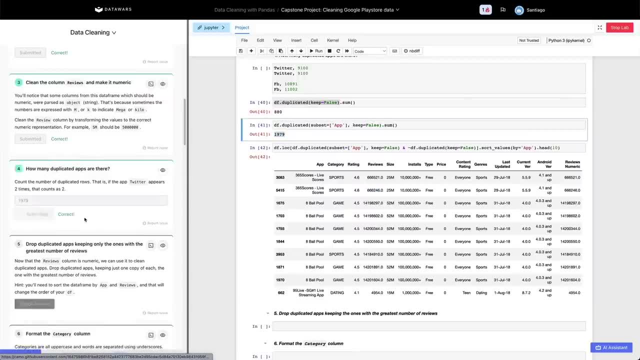 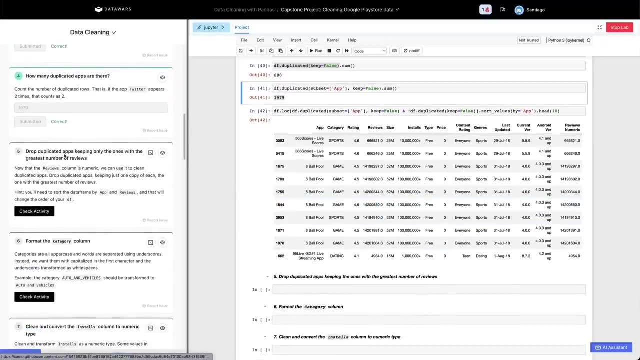 with different data. Anyway, let's answer the activity: How many duplicated apps? but counting them whole, do we have 1,979,. let's check if that works And it goes. it works. Next activity: drop duplicated apps. 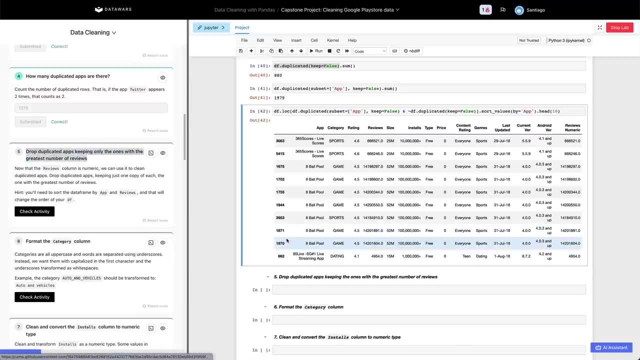 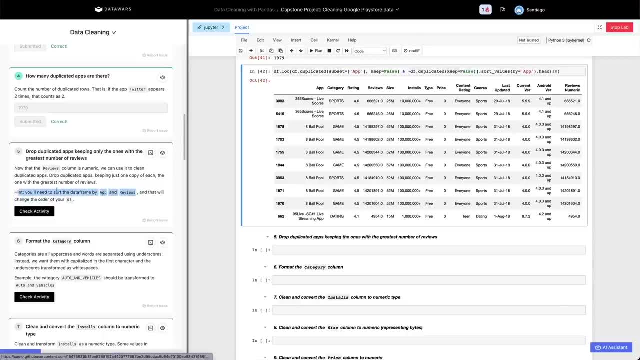 keeping only the ones with the greatest number of reviews, And this is a very interesting one. You will need to sort DataFrame app and reviews and that will change the order of the DataFrame. That is fine, because what is gonna happen is- and again you have to understand- 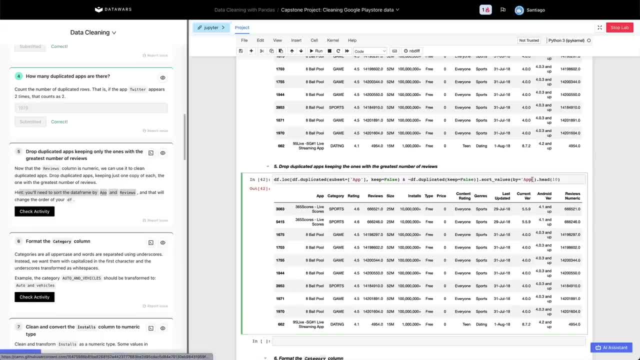 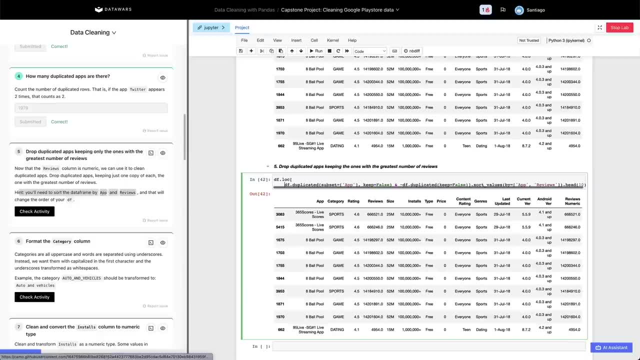 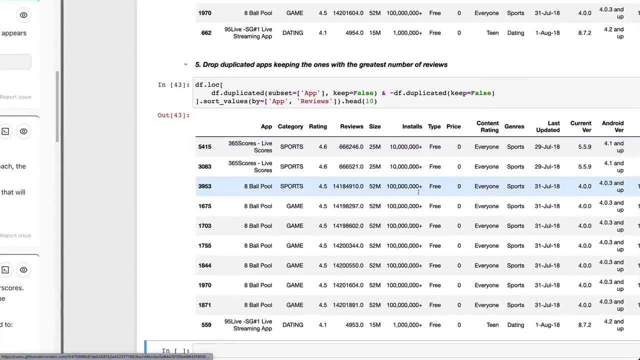 let me copy this thing once again, but I'm gonna sort now by app and by reviews. These lines are extremely short. There you go. So what happens here is that we have again this scraping process that potentially scraped two times or more than two times. 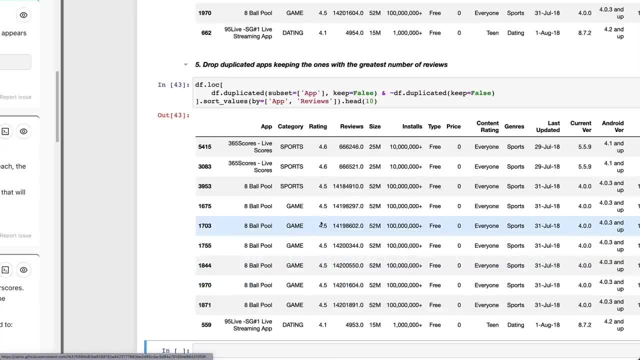 we have like two, four, six, seven times And the reasoning- at least what I'm thinking- is that the scraping process took like an entire week And somehow this person scraped the same app multiple times. but there is one important hint, at least to me. 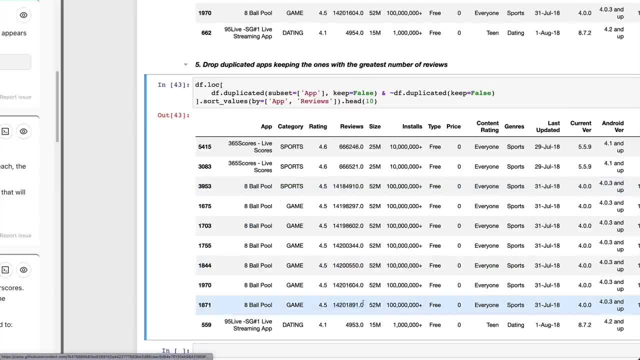 which is that the number of reviews in an app is probably always going up. right, It's like you will seldom delete reviews that you've done in an app. I don't know if that's even possible. potentially it's possible, But basically what I'm thinking here is that 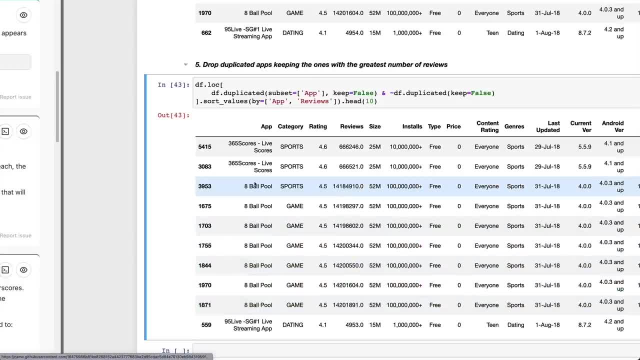 and basically what the activity is asking is that we wanna drop duplicates And what is the freshest copy of the scraping process? What is the app that gets closer to the real number today And that is potentially the one with the greatest number of reviews? 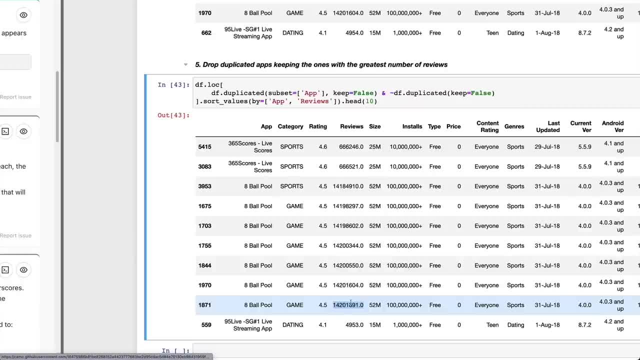 the one with the most reviews Because, again, the reasoning is that this was scraped on Monday. this was scraped on Tuesday, Tuesday, Wednesday, Wednesday, Saturday, Sunday, right, Because all these apps have a different number of reviews and this one the one below, right. 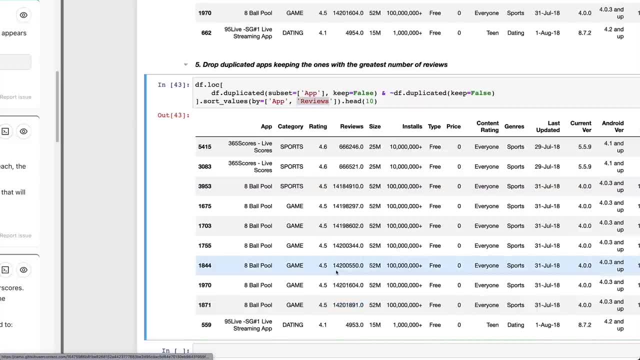 at the bottom, because we sort by reviews, has potentially the greatest, the highest number of reviews. It's potentially the freshest copy of the app from the scraping process. let's say So. what we have to do here is we can sort this data frame in this way. 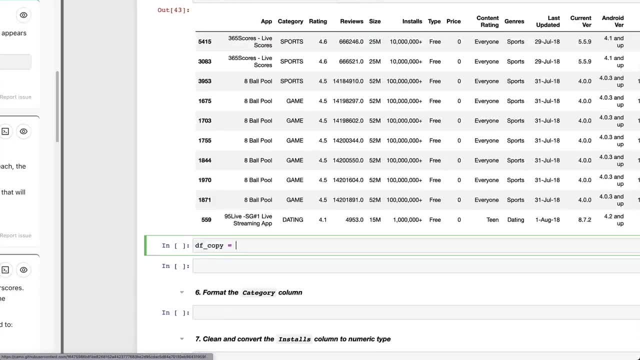 So we can do. let's keep a copy. This is a good technique. As we're changing the data frame, we're making several modifications, it's a good practice to keep a copy in memory, just in case you can always go back to this copy. 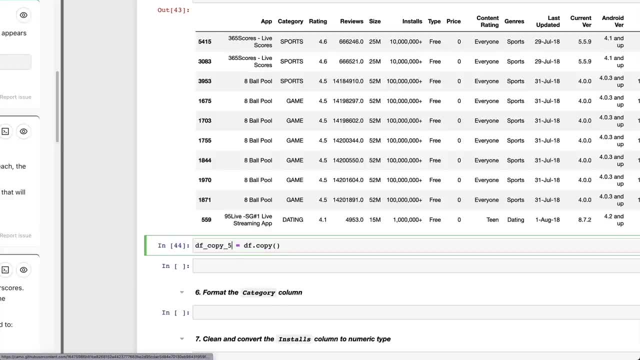 The way I do, it is just copy. I can put a number like this: is activity number five, df copy five or df copy before removing revision or something like that. And I usually just comment it out immediately, because if I execute this cell again, 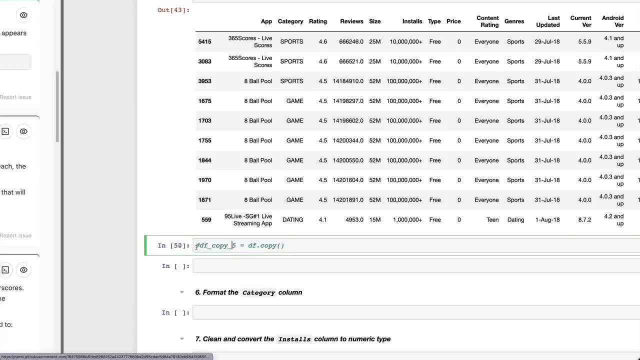 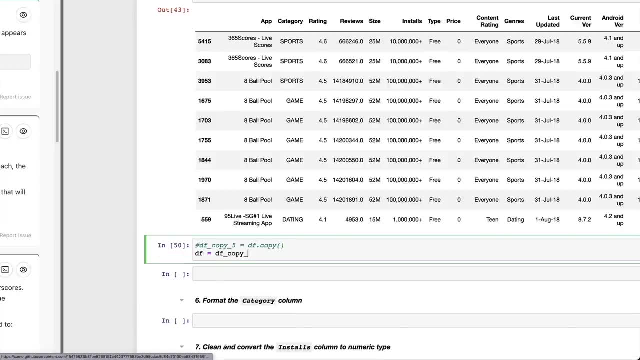 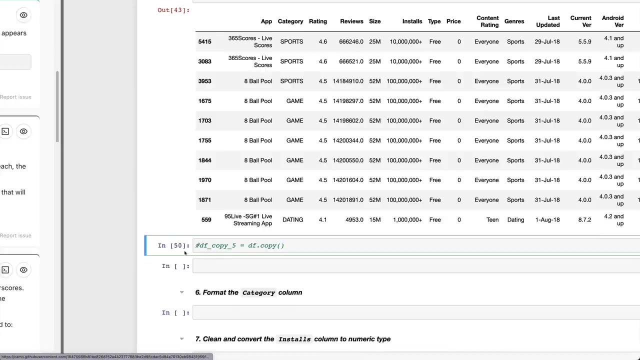 nothing happens, I don't hurt my copy. So again, if we make a mistake we can always roll back. we can do df equals df copy, five, dot copy and we have back again the data in this previous stage. But anyway, let's keep moving forward with activity. 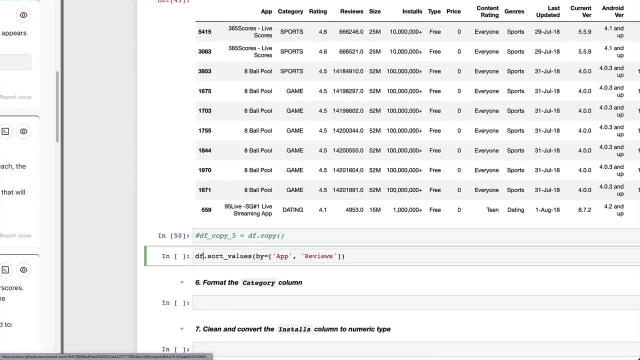 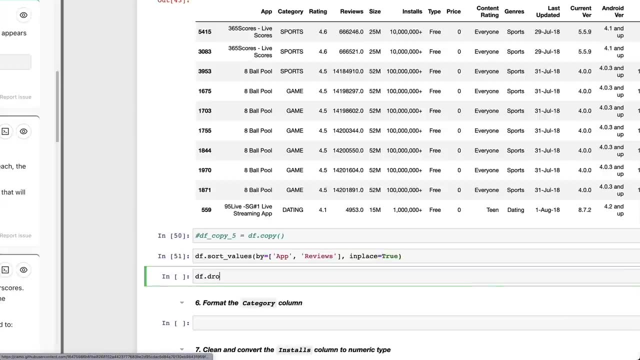 What we wanna do is we wanna sort the values, So dfsortValues- appReviews in place, true, And now we're ready to do dfdropDuplicates- drop duplicates. there we go, We're ready to do this thing. But the interesting part is that we need to say: 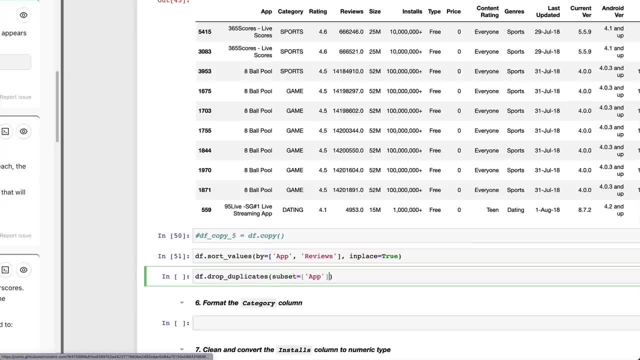 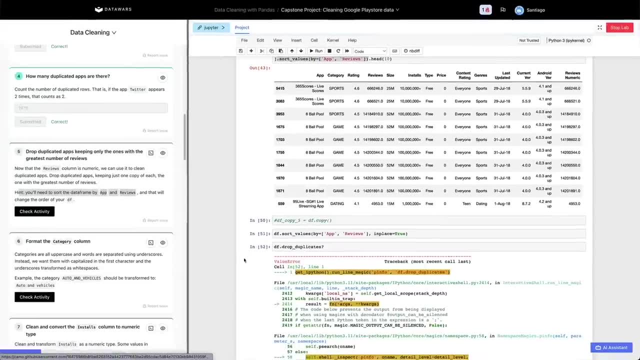 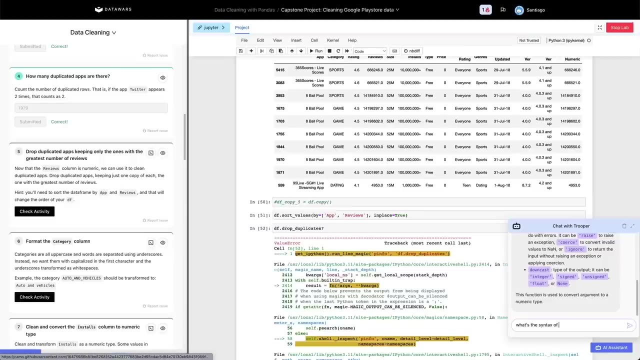 subset is by app and there is a parameter in drop duplicates which is chase. I don't know why the documentation is not working. what's this syntax of the after drop duplicates? let's quickly, I could also do something. I don't know. if you know this trick, like to help this method. 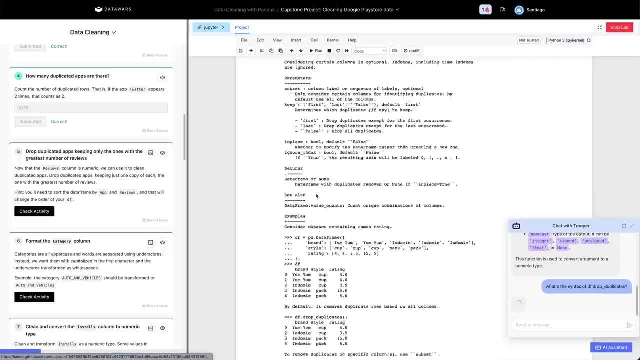 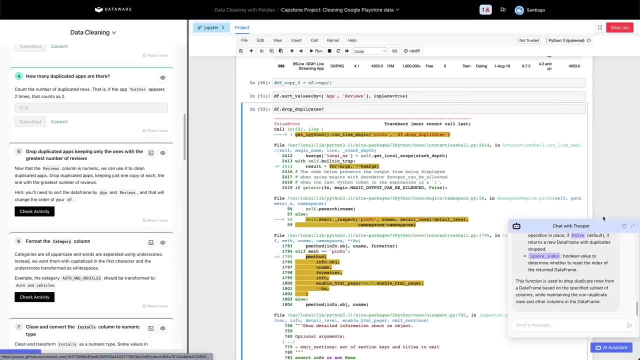 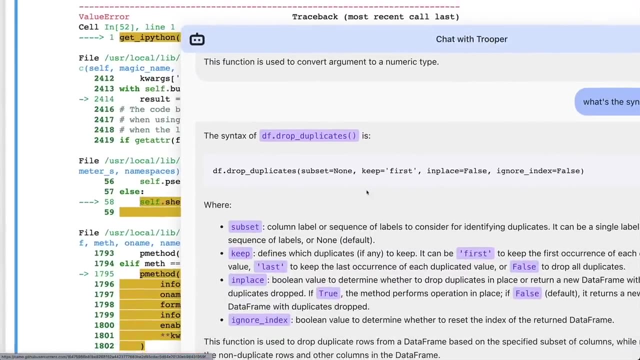 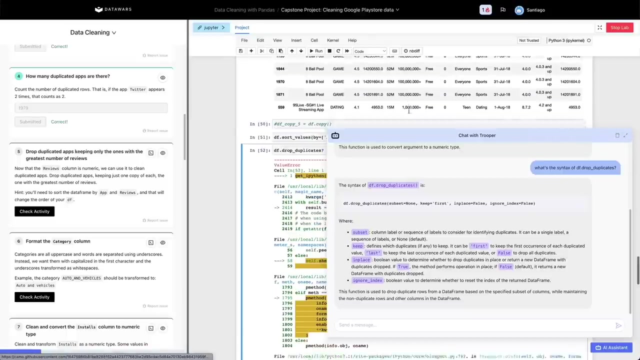 right here gives you the help that should work with the same as this one right here. but let's wait for the systems. try to read of this. there you go and there is this parameter, which is keep first, and what keep first does is basically we. the way pan is gonna gonna work is it's gonna find the duplicates. 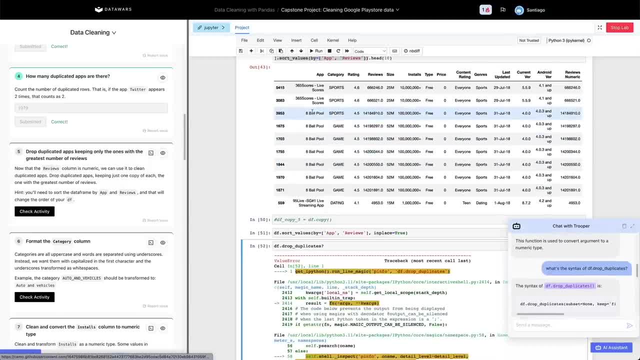 right. in this case, eight ball pool is the app right. in this case, eight ball pool is the app right. in this case, eight ball pool is the app is gonna again. one is gonna be marked. is gonna again. one is gonna be marked. is gonna again. one is gonna be marked. as good. everything else is duplicate, but 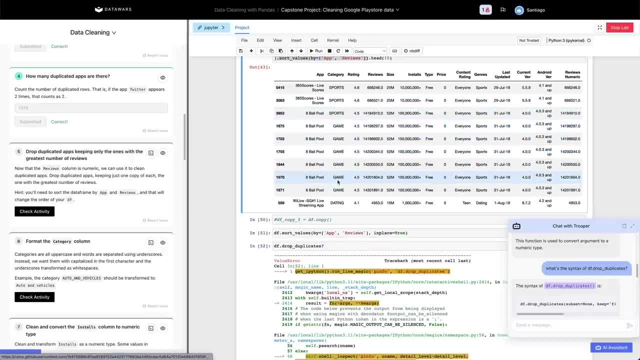 as good, everything else is duplicate. but as good everything else is duplicate. but the question is which one is marked as. the question is which one is marked as. the question is which one is marked as good in this case, as we sorted the data. good in this case, as we sorted the data. 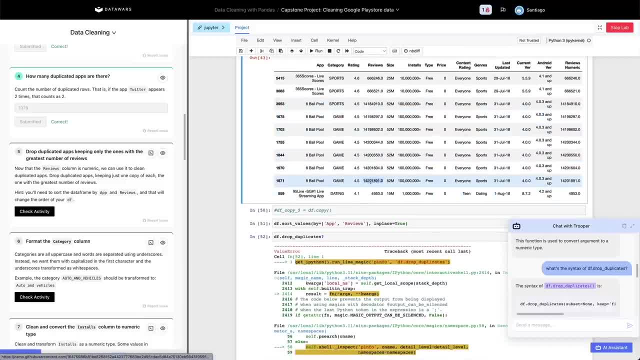 good in this case, as we sorted the data frame in this order, that the one at the frame in this order, that the one at the frame in this order, that the one at the bottom is the one with the with the bottom is the one with the with the. 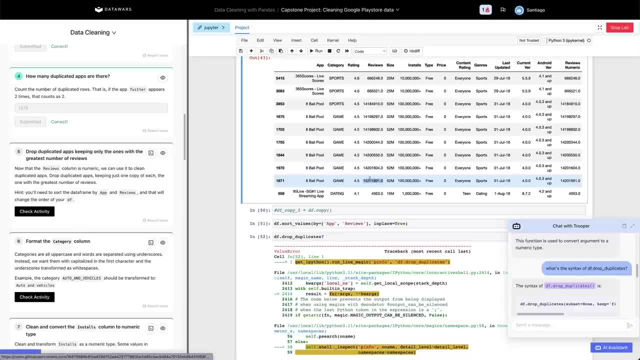 bottom is the one with the with the greatest number of reviews. we want to do greatest number of reviews. we want to do greatest number of reviews. we want to do a keep last. we want to remove all this a keep last. we want to remove all this a keep last. we want to remove all this. and when I keep only this copy: okay. 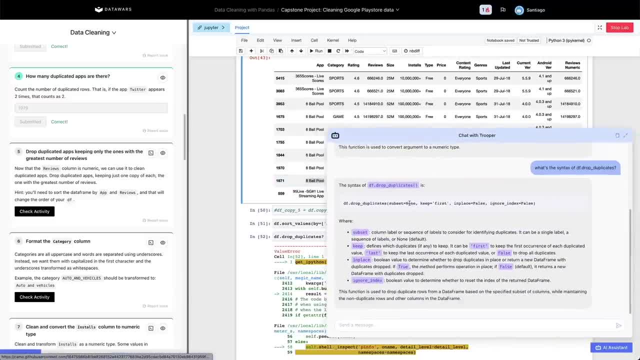 and when I keep only this copy, okay. and when I keep only this copy, okay. that's again the syntax. let me show that. that's again the syntax. let me show that. that's again the syntax. let me show that to you for a sec, right here, keep last. 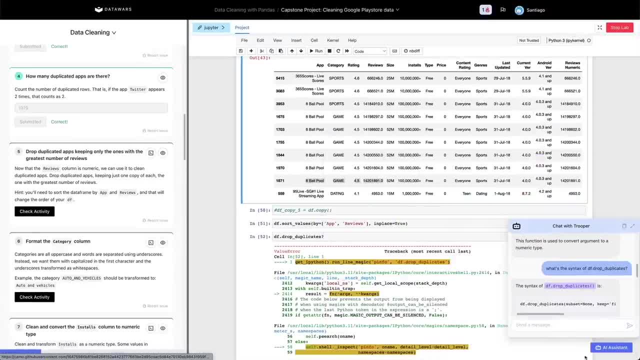 to you for a sec right here. keep last to you for a sec right here. keep last. that's what we want to do, so let me, that's what we want to do, so let me. that's what we want to do. so let me close this and we're gonna do drop. 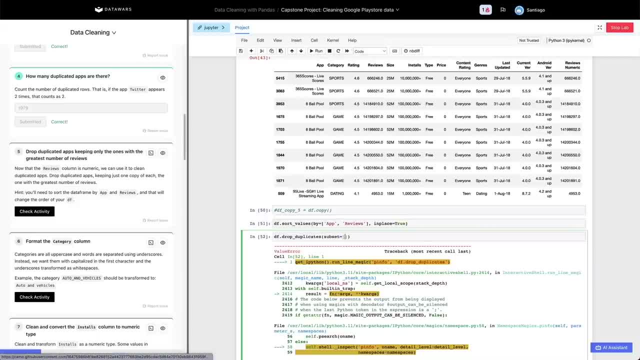 close this and we're gonna do drop close this and we're gonna do drop duplicates subsets up. I do keep last. I duplicates subsets up. I do keep last. I duplicates subsets up. I do keep last I do in place. true, and this is when we're do in place. true, and this is when we're. 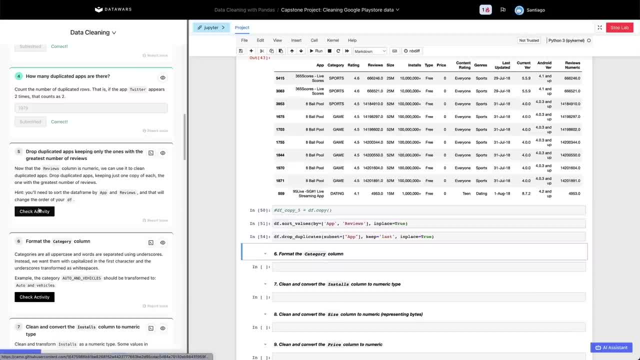 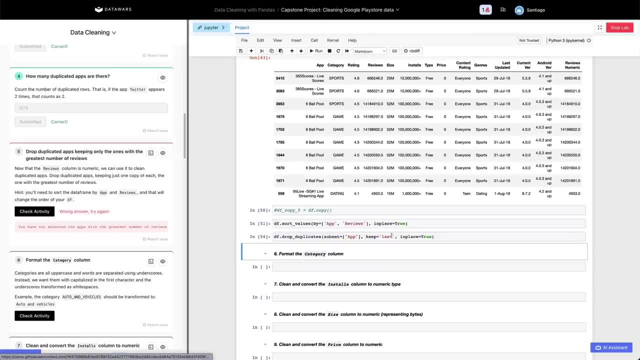 do in place. true, and this is when we're changing the data frame again and we can changing the data frame again and we can changing the data frame again and we can now check the activity. and it didn't now check the activity and it didn't now check the activity and it didn't work. it's strange and potentially could. 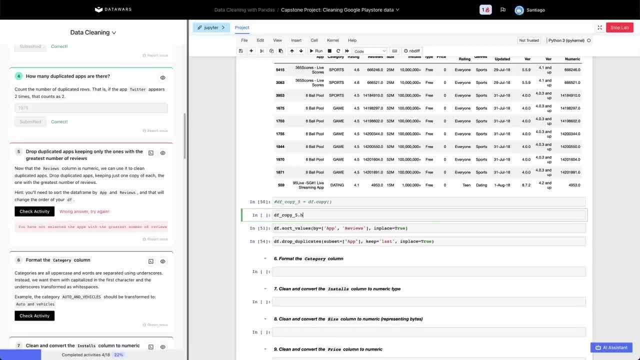 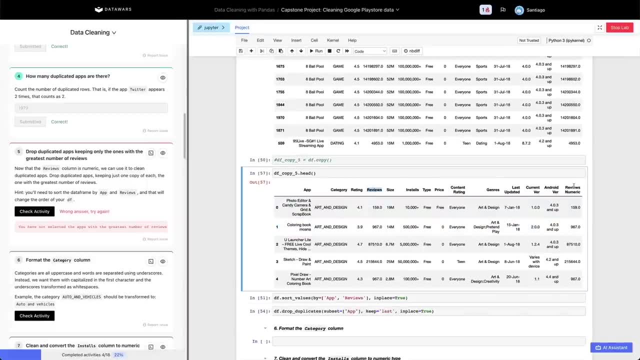 work. it's strange and potentially could work. it's strange and potentially could go back again to the copy and we can try. go back again to the copy and we can try. go back again to the copy and we can try once again. and reviews: Oh, potentially. once again. and reviews, Oh, potentially. 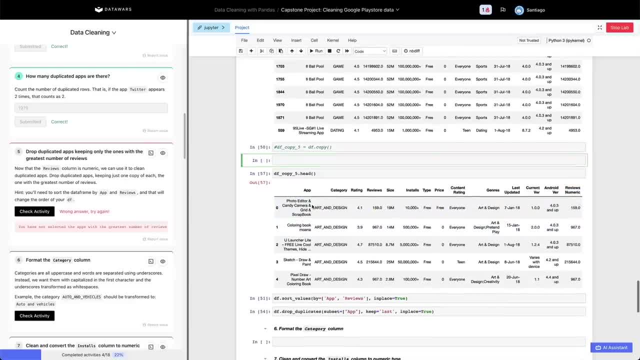 once again and reviews: Oh, potentially, this activity is checking, this activity is checking, this activity is checking, that might be it. so let's keep the copy. that might be it. so let's keep the copy. that might be it. so let's keep the copy what it is. let me just try this out, DF. 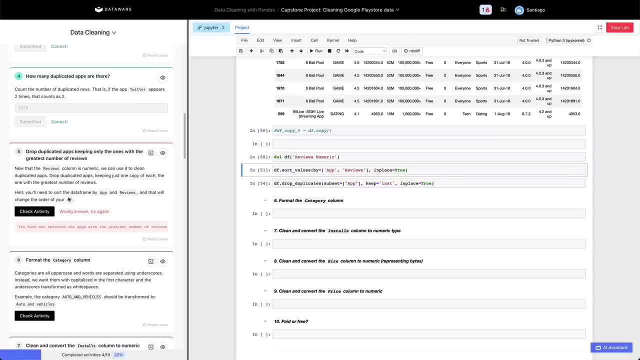 what it is. let me just try this out. DF what it is. let me just try this out. DF- arts or use numeric. let me get rid of arts or use numeric. let me get rid of arts or use numeric. let me get rid of this column and check the activity once. 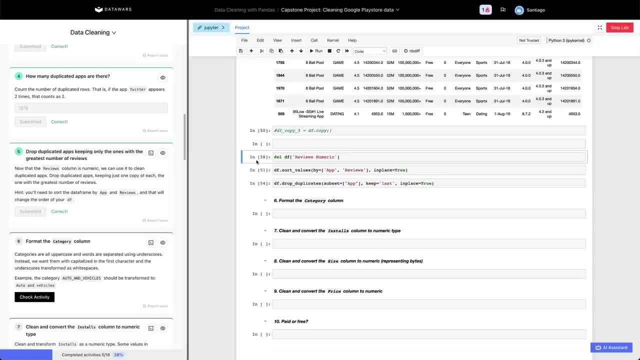 this column and check the activity once this column and check the activity once again. there you go, it worked. my mistake again, there you go, it worked. my mistake again, there you go, it worked. my mistake was not supposed to create a new column, was not supposed to create a new column. 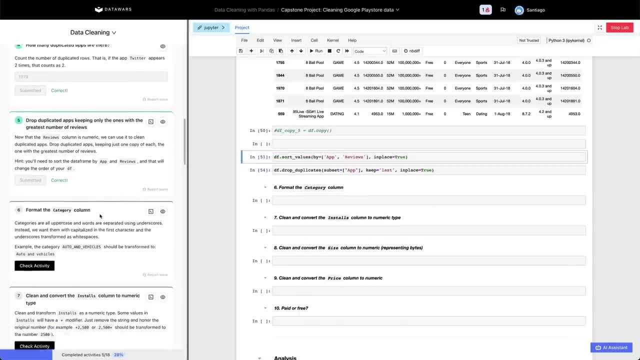 was not supposed to create a new column, which I did okay. moving forward format, which I did okay. moving forward format, which I did okay. moving forward format. the category column. this is an the category column. this is an the category column. this is an interesting one because let's take a 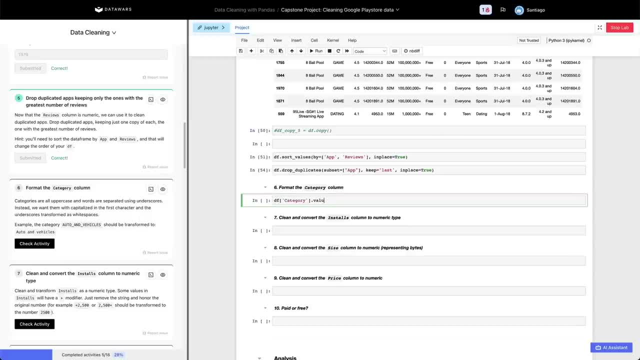 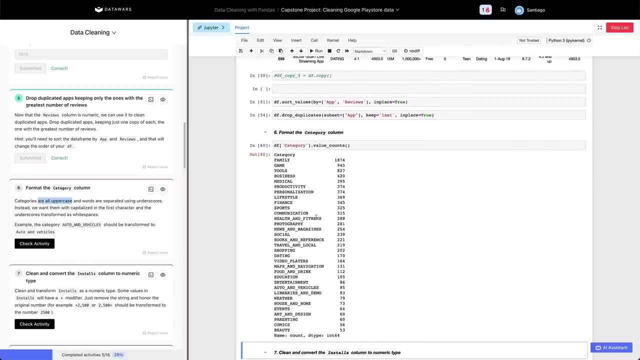 interesting one. because let's take a interesting one, because let's take a look at category first counts. there you look at category first counts. there you look at category first counts. there you go: category all uppercase. yes, they're all go. category all uppercase. yes, they're all. 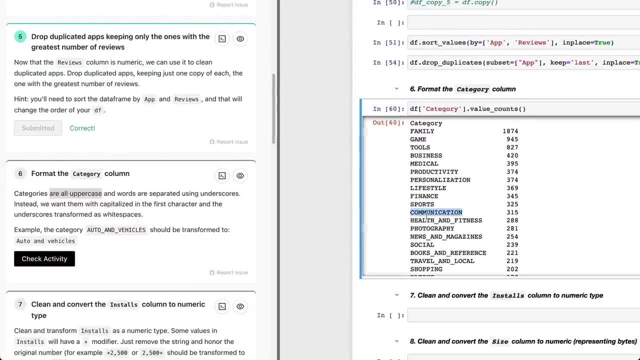 go category all uppercase. yes, they're all uppercase, we can see that. and it says uppercase. we can see that and it says uppercase, we can see that. and it says that white spaces are actually. where are that white spaces are actually? where are that white spaces are actually? where are you seeing underscored? for that we can. 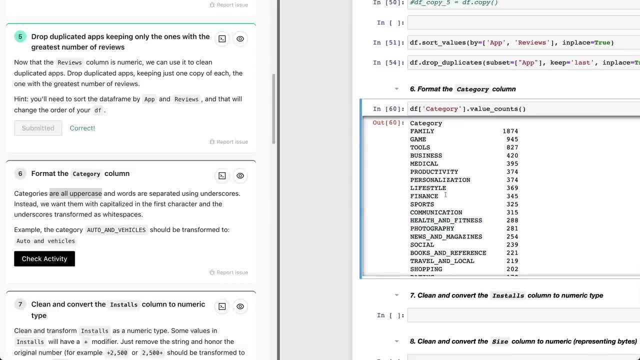 you seeing underscored for that? we can. you seeing underscored for that? we can check that as well. I have to change that. check that as well. I have to change that. check that as well. I have to change that. we have to make this thing remove. we have to make this thing remove. 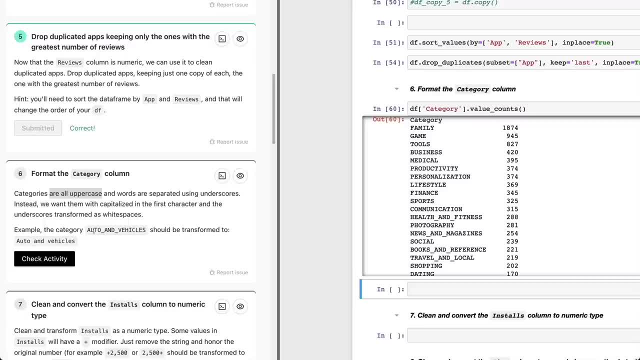 we have to make this thing: remove the uppercase: just use white spaces and the uppercase just use white spaces and the uppercase just use white spaces and capitalize it so autumn vehicles in this: capitalize it. so autumn vehicles in this: capitalize it. so autumn vehicles in this format becomes autumn vehicles in these. 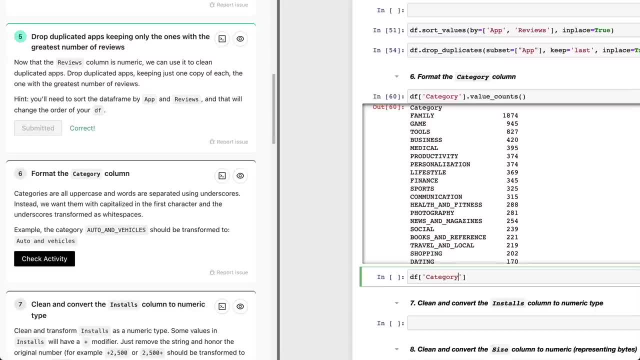 format becomes autumn vehicles in these format becomes autumn vehicles in these formats. so we're gonna do this very formats. so we're gonna do this very formats. so we're gonna do this very quickly. no, any category is equals to the quickly. no, any category is equals to the. 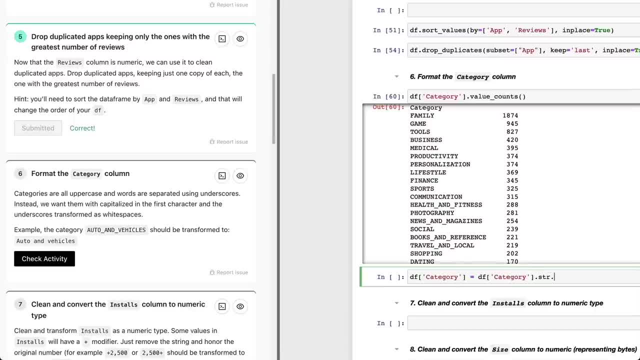 quickly. no, any category is equals to the effort category dot STR to replace, and effort category dot STR to replace, and effort category dot STR to replace. and we're gonna replace here the underscore, we're gonna replace here the underscore, we're gonna replace here the underscore with a white space. that's the first. 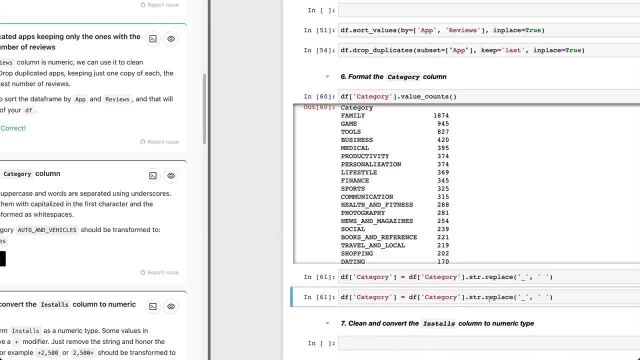 with a white space. that's the first with a white space. that's the first replacement. we're gonna do the second one replacement. we're gonna do the second one replacement we're gonna do. the second one is: we're gonna capitalize the whole. is we're gonna capitalize the whole. 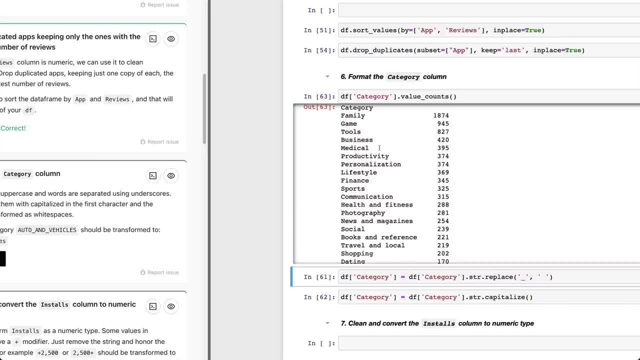 is we're gonna capitalize the whole thing and now we're gonna check we can thing, and now we're gonna check we can thing, and now we're gonna check we can check again this thing. and where is check again this thing? and where is check again this thing? and where is autumn vehicles, autumn vehicles, ideal. 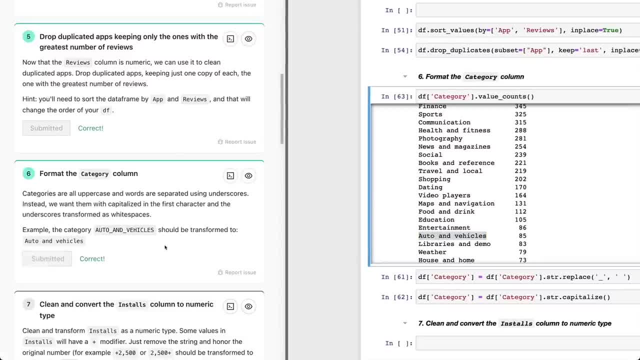 autumn vehicles- autumn vehicles- ideal autumn vehicles, autumn vehicles- ideal, it's gonna be the same. let's check it, it's gonna be the same. let's check it, it's gonna be the same. let's check it out and it works as expected. okay, out and it works as expected okay. 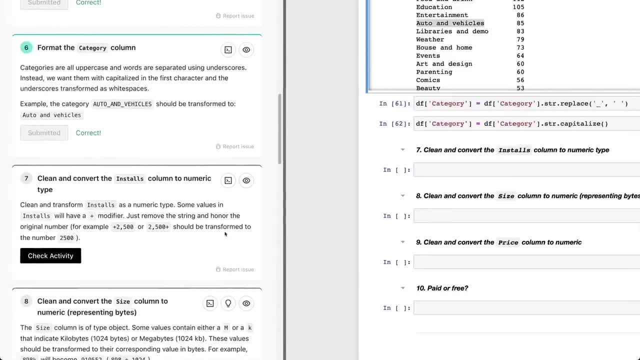 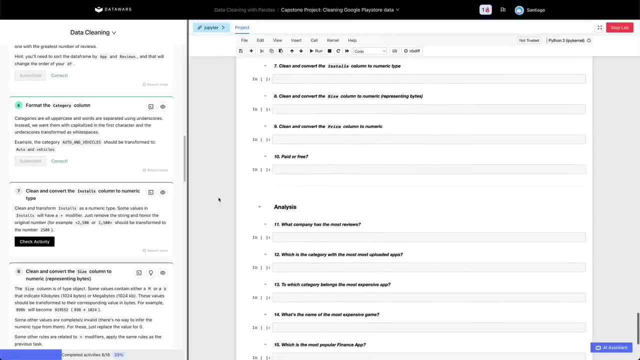 out and it works as expected. okay, activity number 7: clean and convert. the activity number 7: clean and convert. the activity number 7: clean and convert the installs column to numeric type. get rid installs column to numeric type. get rid installs column to numeric type. get rid of this. there we go: clean and convert. 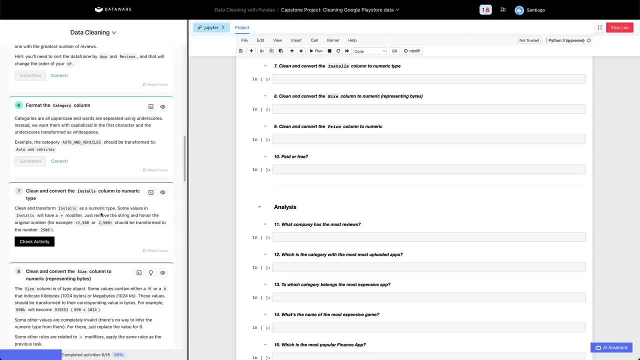 of this: there we go, clean and convert. of this there we go, clean and convert. installs columns in America. cleans some. installs columns in America. cleans some. installs columns in America. cleans some values that have a plus modifier. just values that have a plus modifier, just values that have a plus modifier. just remove the string and honor the original. 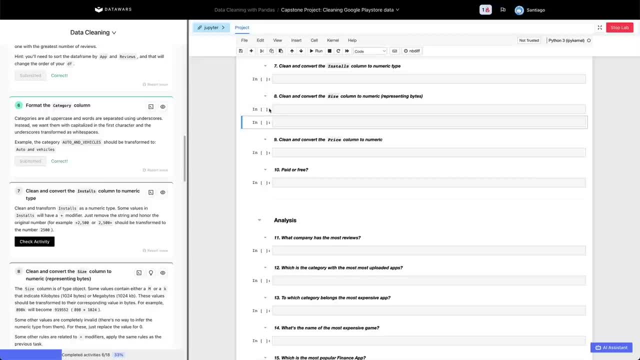 remove the string and honor the original. remove the string and honor the original number. okay, so as usual, we can do number. okay, so, as usual, we can do number. okay, so as usual, we can do something like I don't want to create a, something like I don't want to create a. 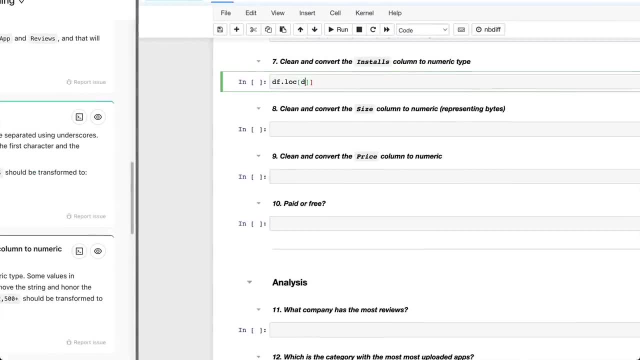 something like: I don't want to create a new column, so I'm gonna do the F? dot lock new column. so I'm gonna do the F? dot lock new column. so I'm gonna do the F? dot lock the F we're gonna do. remember the PD. 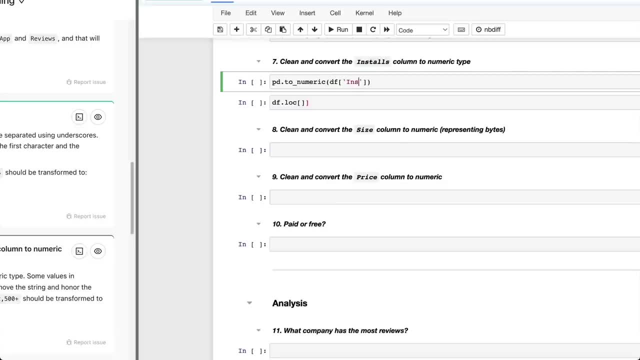 the F, we're gonna do remember the PD. the F, we're gonna do remember the PD. dot to numeric of the F at installs. dot to numeric of the F at installs. dot to numeric of the F at installs. errors squares right, all right, it is an. errors squares right, all right, it is an. 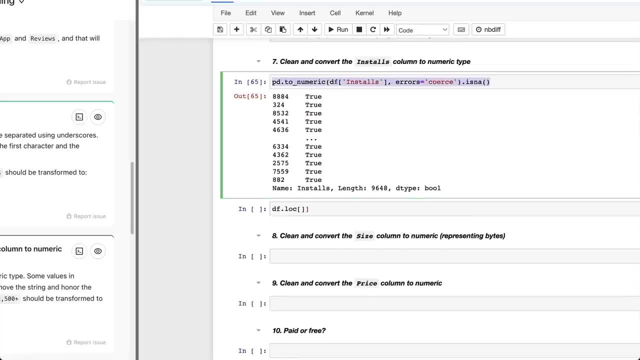 errors squares right. all right, it is an a. so, basically, the opposite cannot the a. so, basically, the opposite cannot the a. so, basically, the opposite cannot. the rows that cannot be parsed as a number. rows that cannot be parsed as a number. rows that cannot be parsed as a number. well, look, use that for a selection, we're. 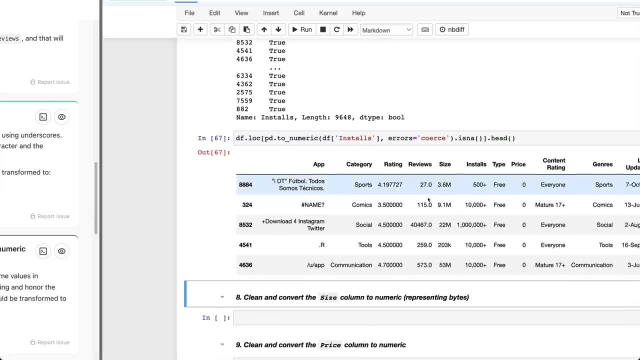 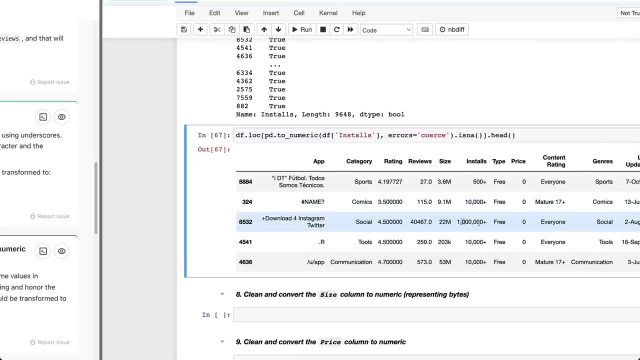 well, look, use that for a selection. we're well, look, use that for a selection. we're gonna do a head real quick and installs gonna do a head real quick and installs gonna do a head real quick and installs 510,000. with a comma separator: 1 million. 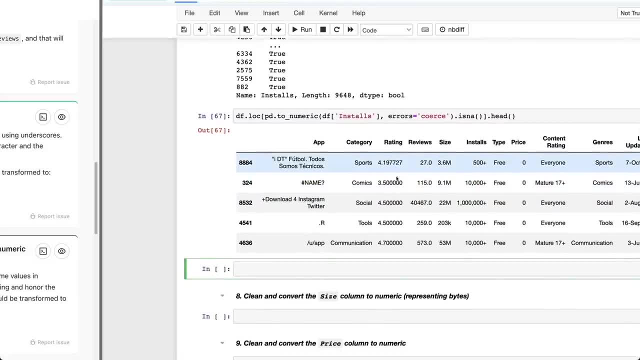 510,000 with a comma separator: 1 million. 510,000 with a comma separator: 1 million, the plus with the comma separator, so the plus with the comma separator, so the plus with the comma separator. so basically what we can do, and I think I 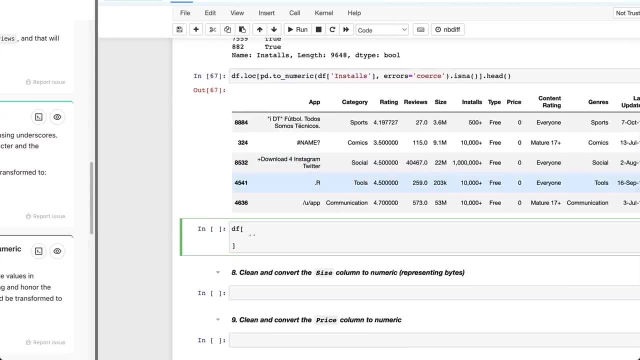 basically what we can do, and I think I basically what we can do, and I think I could do this whole thing in just one, could do this whole thing in just one, could do this whole thing in just one line, would be the F at: oh my bad, my. 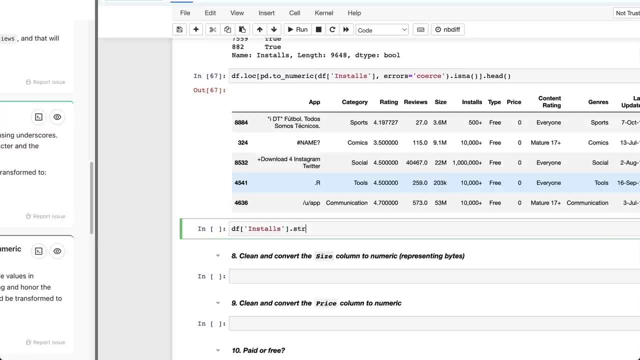 line would be the F at: oh my bad. my line would be the F at: oh my bad. my button installs, not STR, to replace. I'm button installs, not STR to replace. I'm button installs, not STR to replace. I'm gonna replace the plus symbol with. gonna replace the plus symbol with. 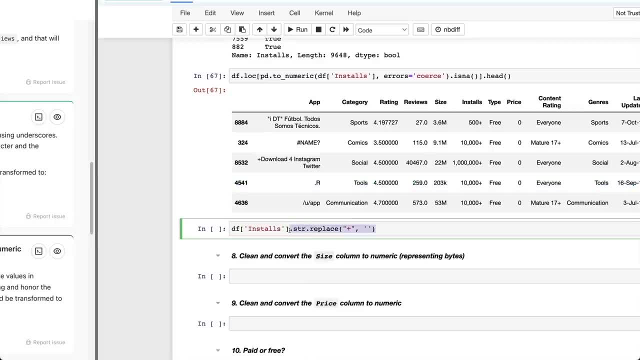 gonna replace the plus symbol with nothing. we're gonna remove it and just nothing. we're gonna remove it and just nothing. we're gonna remove it and just change the whole thing. change the change, the whole thing. change the change, the whole thing, change the command, and we're gonna do comma with. 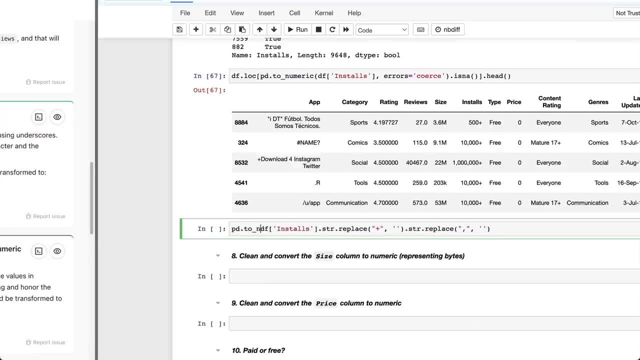 command and we're gonna do comma with command and we're gonna do comma with nothing. we're gonna separate that, so nothing. we're gonna separate that, so nothing, we're gonna separate that. so what I do PD dot to Merrick of this, what I do PD dot to Merrick of this: 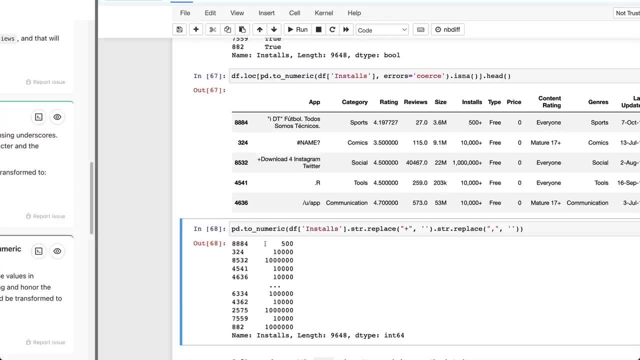 what I do. PD dot to Merrick of this whole thing. there you go, seems it's not whole thing. there you go, seems it's not whole thing. there you go, seems it's not. failing, so that means this is working. failing, so that means this is working. 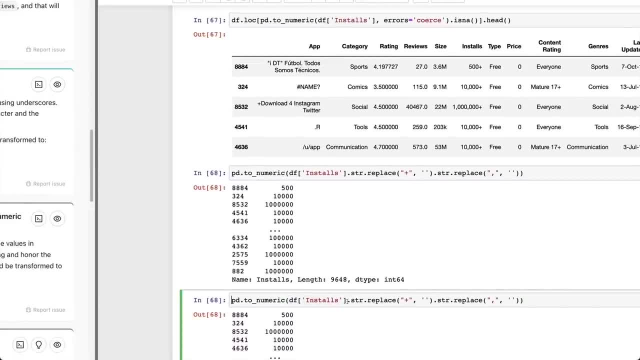 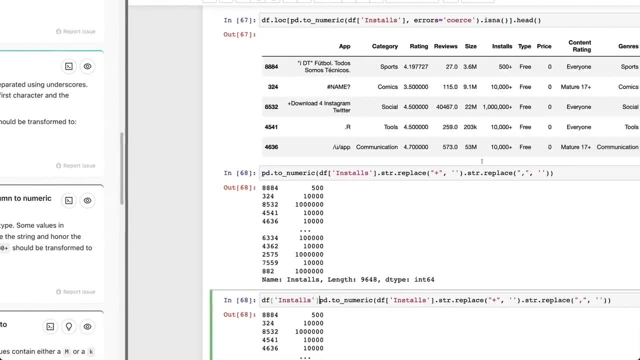 failing, so that means this is working and finally we're gonna sign this thing. and finally we're gonna sign this thing and finally we're gonna sign this thing to installs. let me see if there is to installs. let me see if there is to installs. let me see if there is anything else. no, that is perfectly fine. 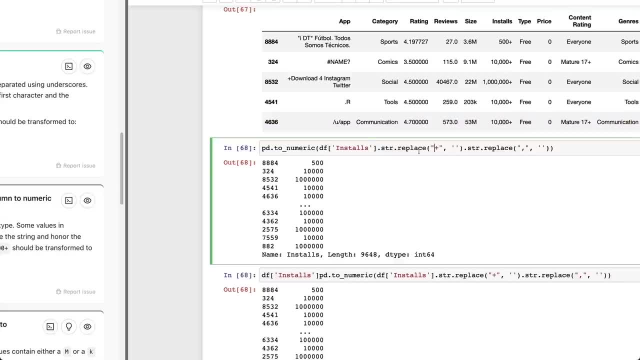 anything else? no, that is perfectly fine. anything else? no, that is perfectly fine. there is no M right because I, only I. there is no M right because I, only I. there is no M right because I only I only remove the plus symbol and the comma, only remove the plus symbol and the comma. 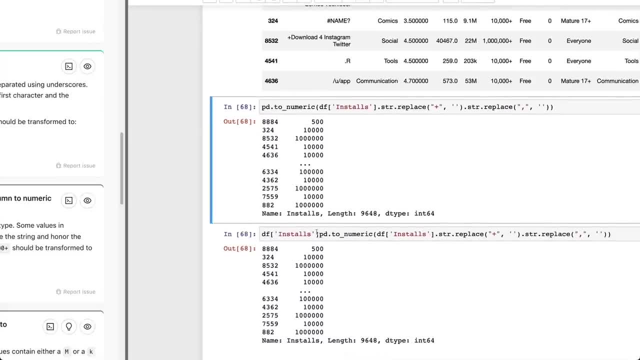 only remove the plus symbol and the comma. and that just transformed to numeric, so. and that just transformed to numeric, so. and that just transformed to numeric, so it seems like I'm Faye, I'm safe, sorry. it seems like I'm Faye, I'm safe, sorry. 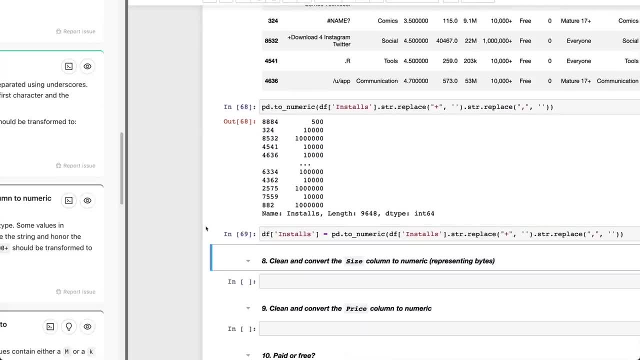 it seems like I'm Faye, I'm safe, sorry, and we're gonna know I'll sign this to and we're gonna know I'll sign this to and we're gonna know I'll sign this to. installs and check the activity and it. installs and check the activity and it. 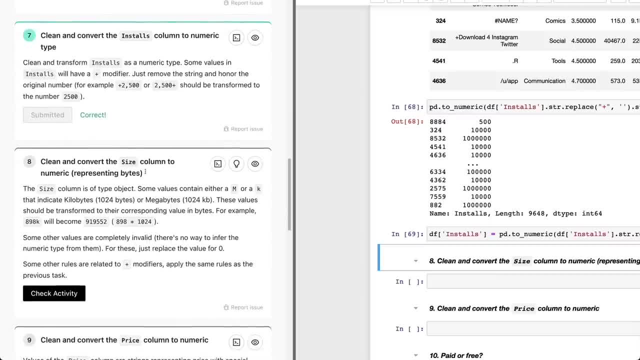 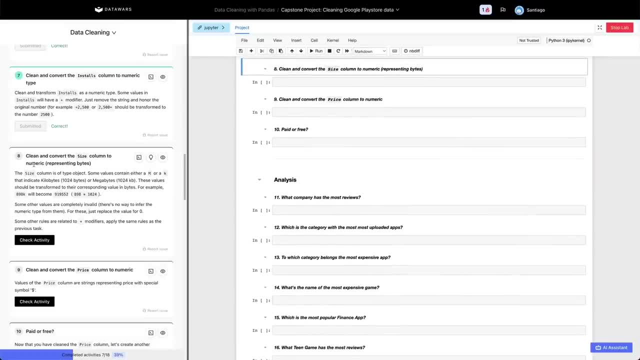 installs and check the activity and it works clean and convert activity number: works clean and convert activity number: works clean and convert activity number. eight, there, there you go, let me center eight. there, there you go, let me center eight, there, there you go, let me center its activity. activity number eight, clean. 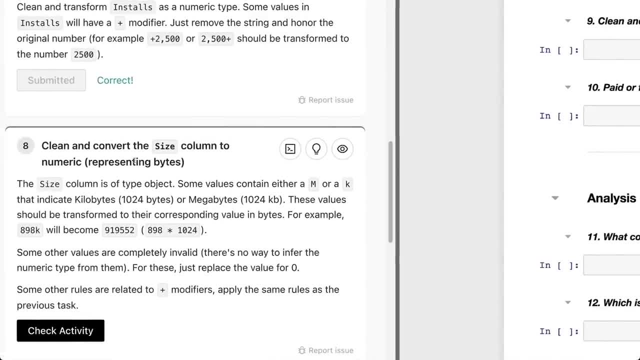 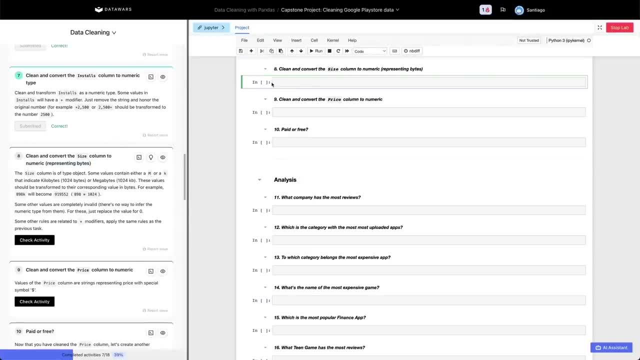 its activity activity number eight: clean. its activity activity number eight: clean. convert the size column to numeric. convert the size column to numeric. convert the size column to numeric. representing bytes size. columns of type. representing bytes size. columns of type. representing bytes size. columns of type objects: some values are either M or K, so 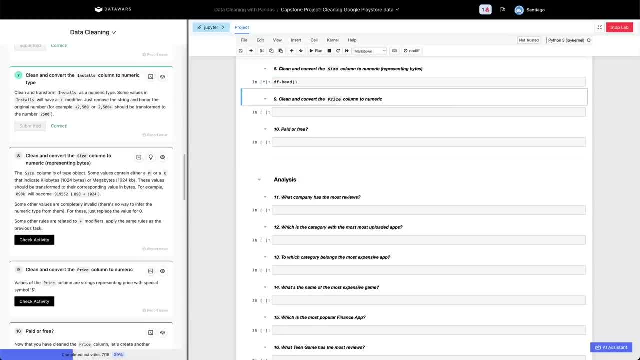 objects, some values are either M or K. so objects, some values are either M or K. so that's basically megabytes or kilobytes. that's basically megabytes or kilobytes. that's basically megabytes or kilobytes. let's take a look at our data frame once. 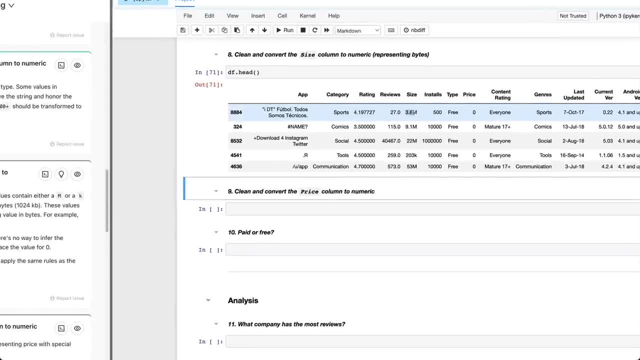 let's take a look at our data frame once. let's take a look at our data frame once again. there you go. sign size: this is 3.6. again there you go. sign size: this is 3.6. again there you go. sign size: this is 3.6 megabytes, 9.1 megabytes, 203 kilobytes. we 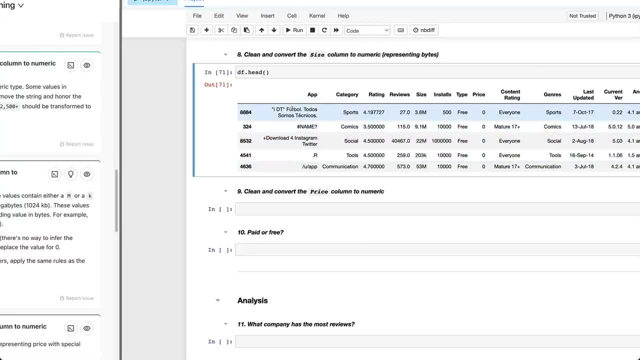 megabytes, 9.1 megabytes, 203 kilobytes. we megabytes, 9.1 megabytes, 203 kilobytes. we want to turn this thing into a, into a. want to turn this thing into a into a. want to turn this thing into a, into a bytes. it seems right when I turn this. 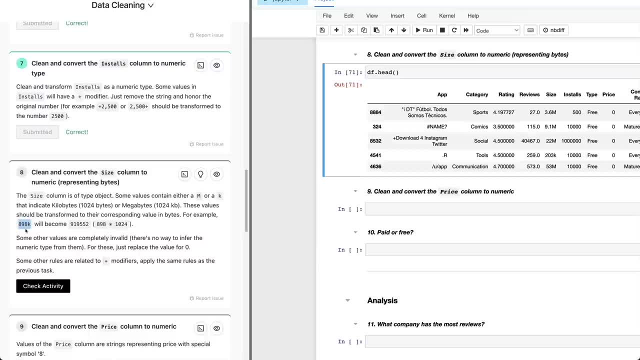 bytes. it seems right when I turn this bytes. it seems right when I turn this thing into bytes, 9 898 2 will become thing into bytes 9 898 2 will become thing into bytes. 9 898 2 will become this thing, which is the bytes thing that. 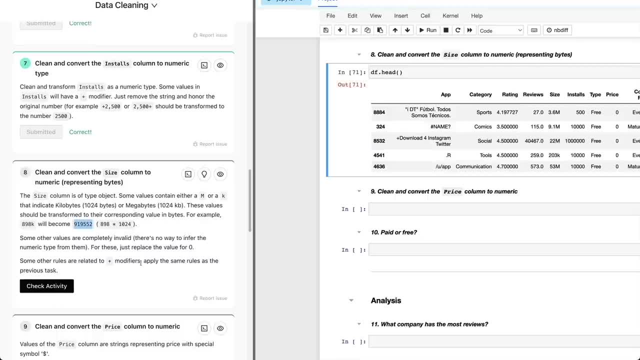 this thing, which is the bytes thing, that this thing, which is the bytes thing, that is that is good. some other rules are I is that is good. some other rules are I is that is good. some other rules are I. remember supply the rules as previous. remember supply the rules as previous. 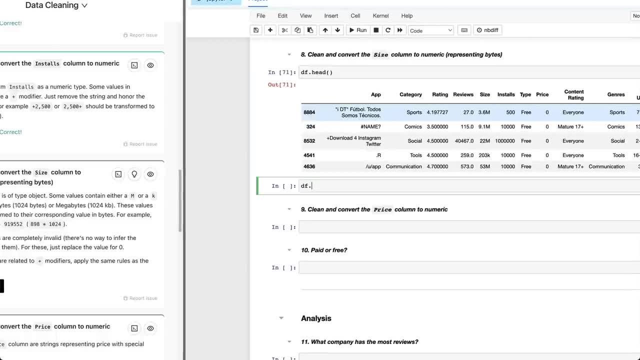 remember, supply the rules as previous tasks like the one in the plus. so if we tasks like the one in the plus, so if we tasks like the one in the plus, so if we do the F PD time, let's do the F dot lock. do the F PD time, let's do the F dot lock. 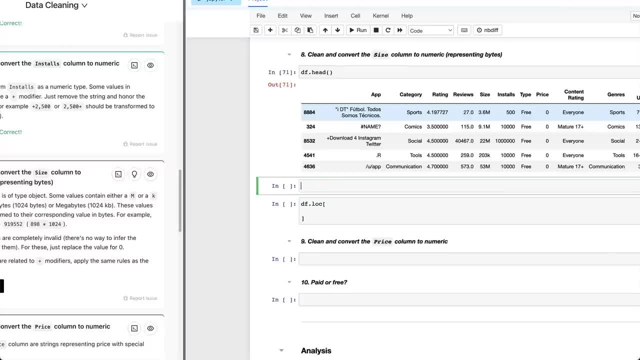 do the F PD time. let's do the F dot, lock the F and do PD to numeric. and I think the F and do PD to numeric and I think the F and do PD to numeric and I think it is a good time to keep a copy the F. 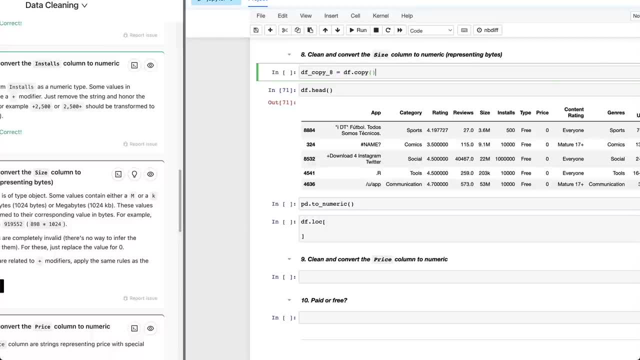 it is a good time to keep a copy the F. it is a good time to keep a copy the F. copy H the F that copy, there you go. copy H the F that copy, there you go. copy H the F that copy, there you go. Oh my bad. 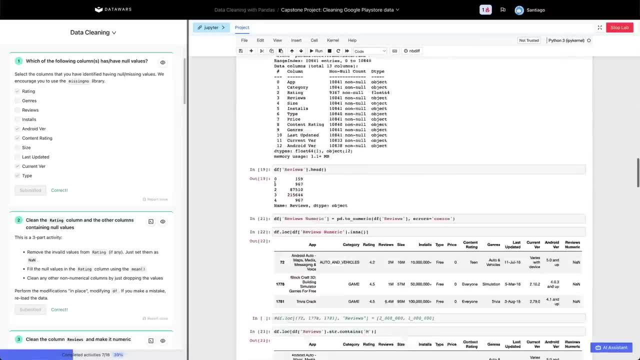 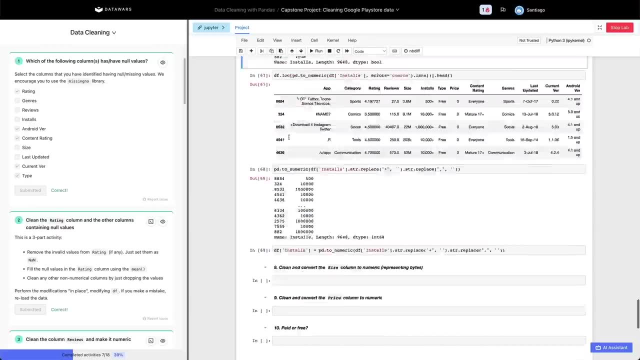 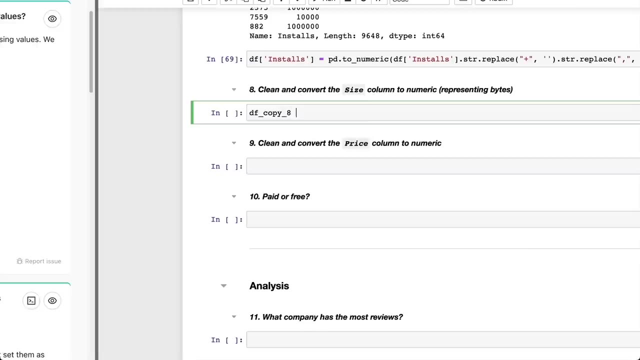 Oh my bad. Oh my bad. reloading, reloading, reloading, scanning, reloading, reloading, reloading, scanning, reloading, reloading, reloading, scanning, scanning, scanning, scanning. where were scanning, scanning, scanning? where were scanning, scanning, scanning, scanning? where were you size? we didn't save the you size. we didn't save the you size, we didn't save the notebook, the F copy. H equals the F, the copy. 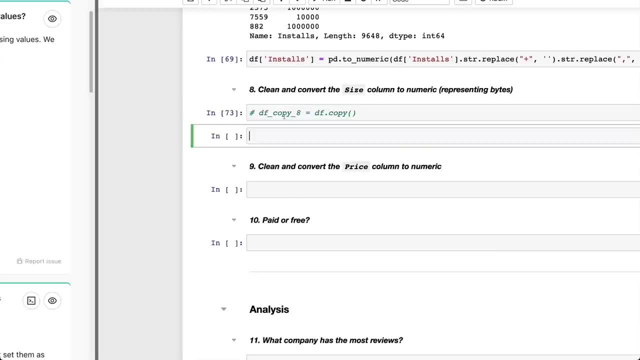 notebook. the F copy H equals the F the copy. notebook. the F copy H equals the F the copy. H notebook. the F copy H equals the F. the copy. H equals the F, the copy. and we're gonna comment that, and we're gonna comment that, and we're gonna comment that out and, as usual, we're gonna do the F at. 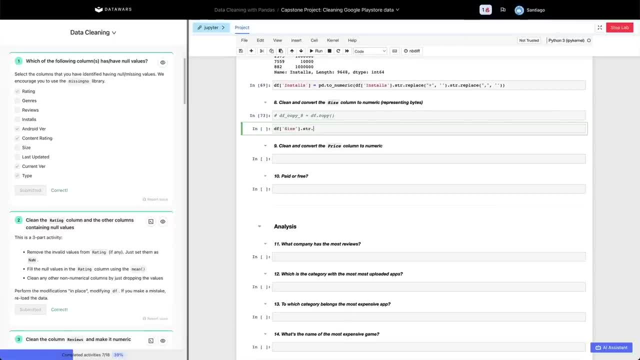 out and as usual, we're gonna do the F at out and as usual, we're gonna do the F at size dot. STR dot replace M and with size dot. STR dot replace M and with size dot. STR dot replace M and with nothing. and STR dot replace K with. 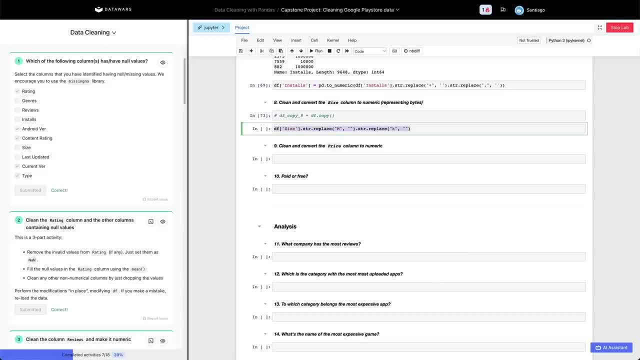 nothing, and STR dot replace K with nothing and STR dot replace K with nothing. we don't want to do that right nothing. we don't want to do that right nothing. we don't want to do that right now because we want to convert this thing now, because we want to convert this thing. 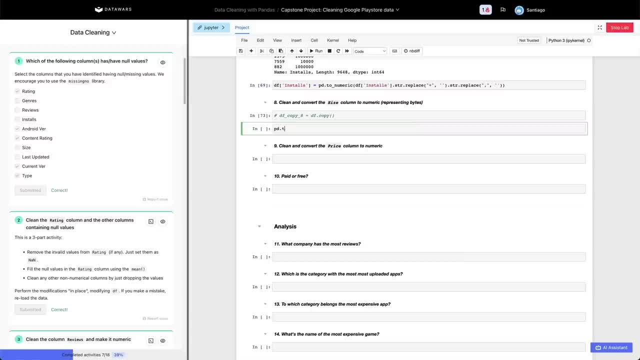 now, because we want to convert this thing to the real numbers. but for now, if I do to the real numbers, but for now if I do to the real numbers, but for now if I do PD to numeric of this thing, what happens? PD to numeric of this thing, what happens? 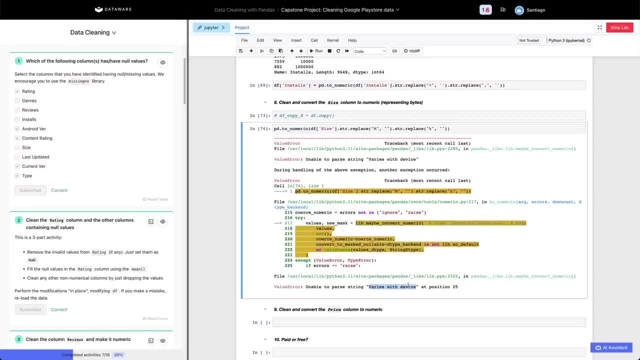 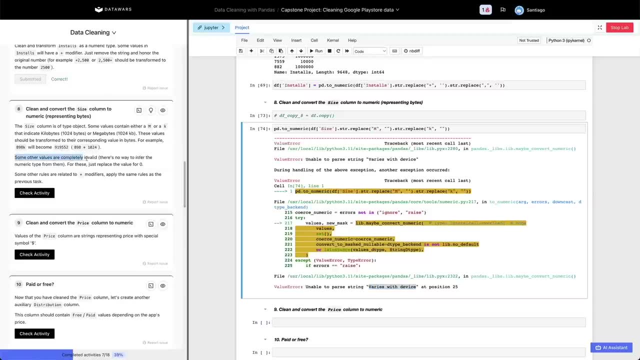 PD to numeric of this thing. what happens? unable to parse string: var, var, var, var. unable to parse string var, var, var, var, var. unable to parse string: var, var, var, var, var is with device. so that is because some is with device. so that is because some is with device. so that is because some other values are completely invalid. 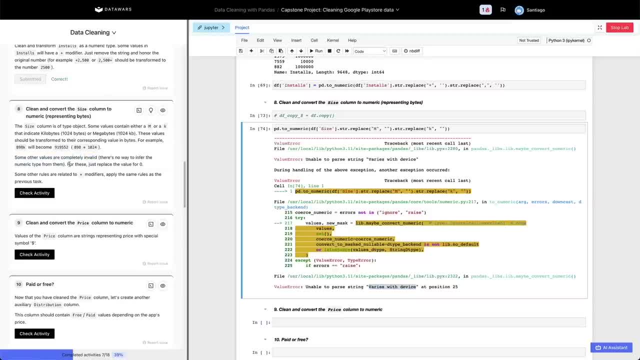 other values are completely invalid. other values are completely invalid. there is no way to infer numeric type. there is no way to infer numeric type. there is no way to infer numeric type from them. so these are to replace with from them. so these are to replace with from them. so these are to replace with zero. okay, so we can start right there. we. 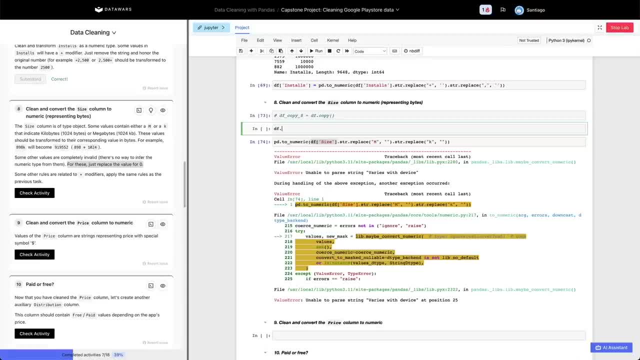 zero okay, so we can start right there. we zero okay, so we can start right there. we can say the F, the F dot lock, the F at can say the F the F dot lock, the F at can say the F the F dot lock the F at size equals or, as with device dot shape. 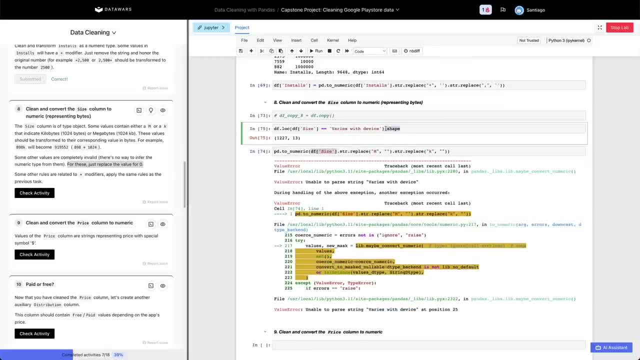 size equals, or, as with device dot shape, size equals or as with device dot shape. how many? oh, okay, a ton. so there are a. how many? oh okay, a ton. so there are a. how many? oh, okay, a ton. so there are a ton of these sort of apps. and here want 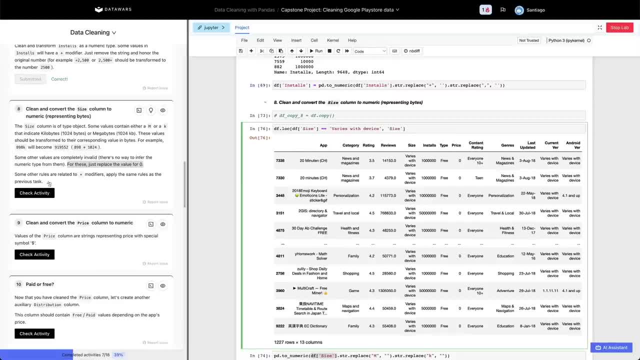 ton of these sort of apps. and here: want ton of these sort of apps. and here want to do that, these column size for that, to do that, these column size for that, to do that, these column size for that condition should be zero. so I'm gonna do. 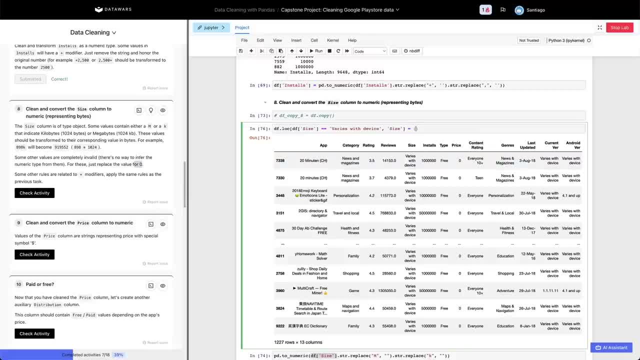 condition should be zero, so I'm gonna do. condition should be zero, so I'm gonna do just I'm gonna do zero as type STR. as just I'm gonna do zero as type STR. as just I'm gonna do zero as type STR, as usual, usual, usual, remember. 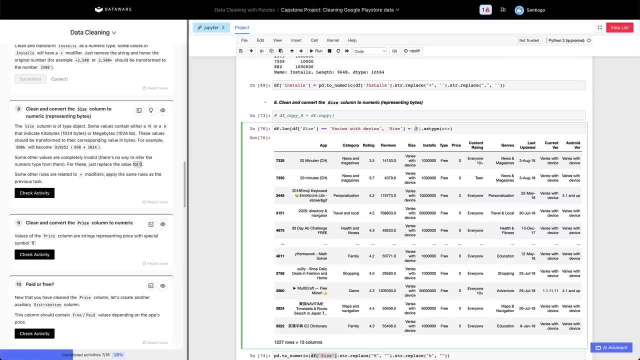 remember. remember. thoughts- this is not gonna work. thoughts- this is not gonna work. thoughts- this is not gonna work. potentially PD- this might be fine. let's potentially PD- this might be fine. let's potentially PD this might be fine. let's let me try it out. if it doesn't work, we 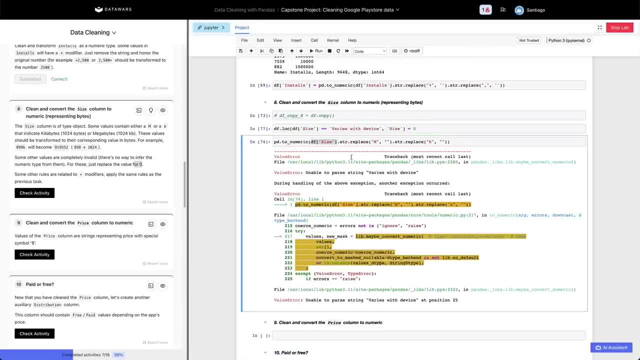 let me try it out. if it doesn't work. we let me try it out. if it doesn't work, we have the copy as usual. we want to keep have the copy as usual. we want to keep have the copy as usual. we want to keep the values to string. the F at size is: 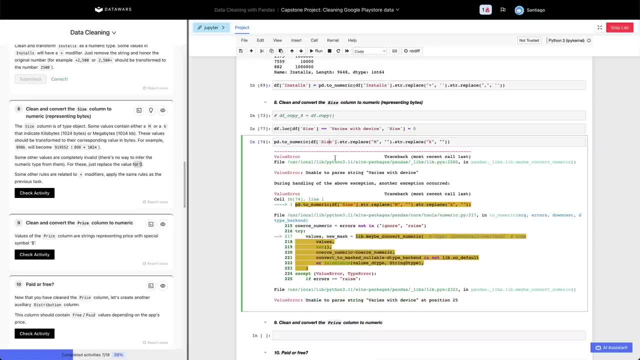 the values to string the F at size is. the values to string the F at size is: is still an object. that's good, and now it is still an object. that's good, and now it is still an object. that's good, and now it seems that it's working. 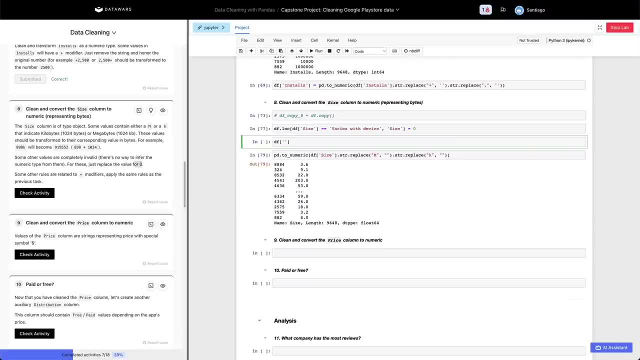 seems that it's working. seems that it's working. so there you go. it seems that it's working. so there you go. it seems that it's working. so there you go. it seems that it's working. the F adds the F that head. we only. the F adds the F that head, we only. 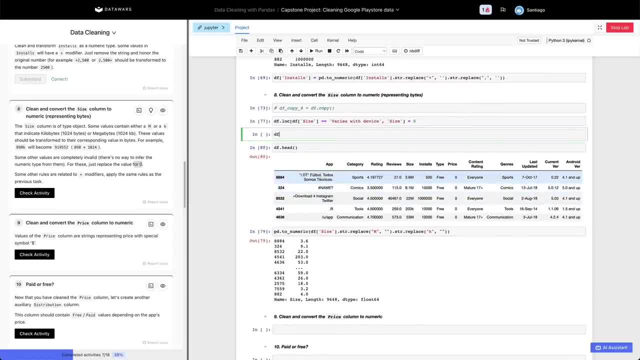 the F adds the F that head. we only have to replace our their DF dot lock the F. have to replace our their DF dot lock the F. have to replace our their DF dot lock the F. at size dots. STR dot contains a. at size dots. STR dot contains a. 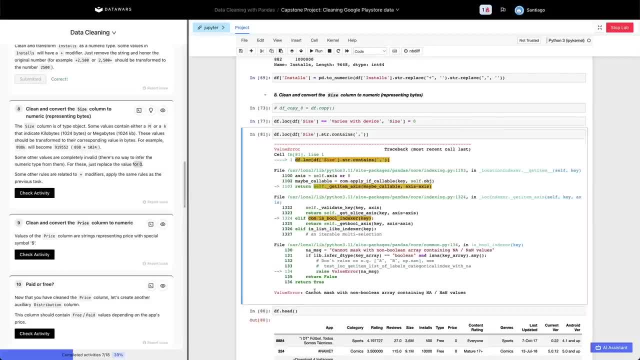 at size dots. STR dot contains a comma. can I must know? contain it? no, I we we comma. can I must know? contain it. no, I we we comma. can I must know? contain it. no, I we we. made a mistake. let me go back again. made a mistake. let me go back again. 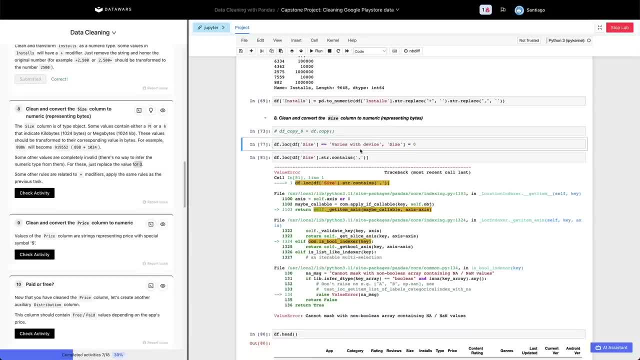 made a mistake. let me go back again: copy, copy, copy, copy, copy, copy, copy. this is a good thing we're gonna. this is a good thing we're gonna. this is a good thing we're gonna basically say PD- the series 0 thoughts. basically say PD- the series 0 thoughts. 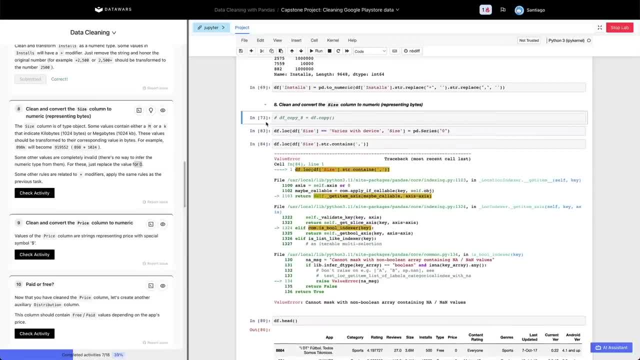 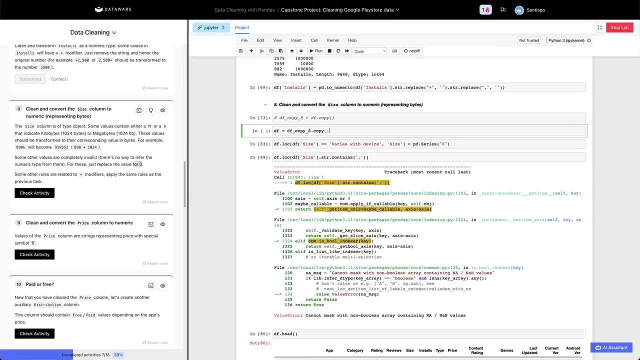 basically say: PD, the series 0 thoughts and I. we made a mistake again, the F and I. we made a mistake again the F and I. we made a mistake again the F, copy, copy. there you go because we might copy, copy there you go because we might. 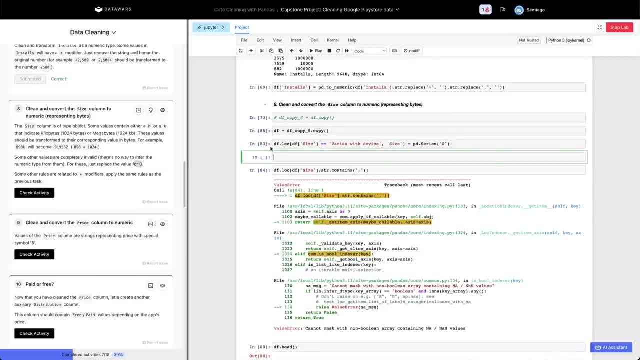 copy, copy. there you go, because we might not be able to assign it, so what? I'm not be able to assign it, so what I'm not be able to assign it. so what I'm gonna do is just gonna do. is just gonna do is just more string handling, which is the usual. 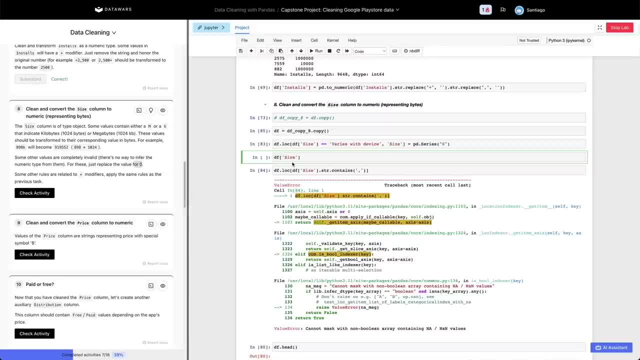 more string handling, which is the usual more string handling, which is the usual way of doing this process, which is the F way of doing this process, which is the F way of doing this process, which is the F. at size equals the effort size dot STR. at size equals the effort size, dot STR. 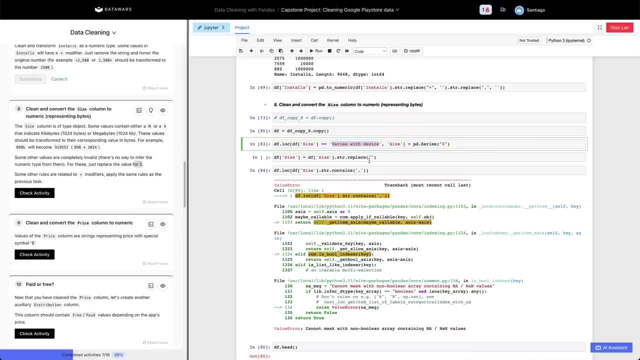 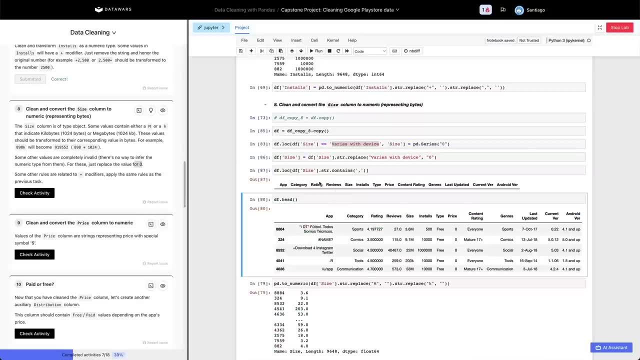 at size equals the effort size. dot. STR. that replace. I'm gonna replace this. that replace, I'm gonna replace this. that replace, I'm gonna replace this whole thing. or is with size for a zero in whole thing, or is with size for a zero in whole thing, or is with size for a zero in this way. there you go and there you go. 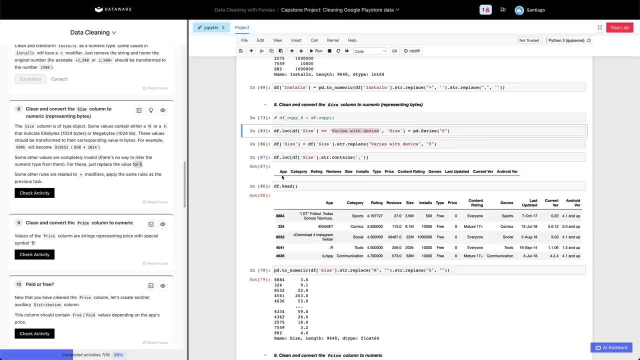 this way, there you go and there you go. this way, there you go and there you go. it works. so the copy is saving us, so it works. so the copy is saving us, so it works, so the copy is saving us. so there is nothing with a comma, that is. 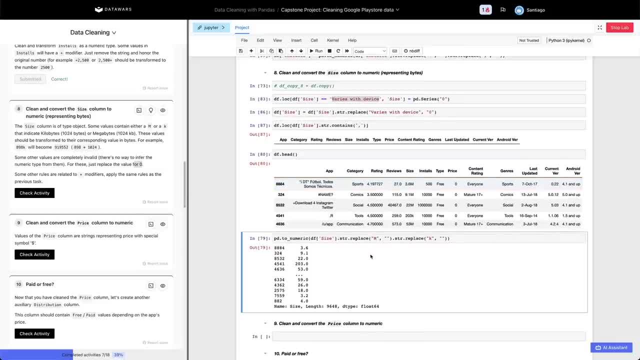 there is nothing with a comma. that is, there is nothing with a comma. that is good, and it seems like we can good and it seems like we can good and it seems like we can potentially convert if we fix the issue, potentially convert if we fix the issue. 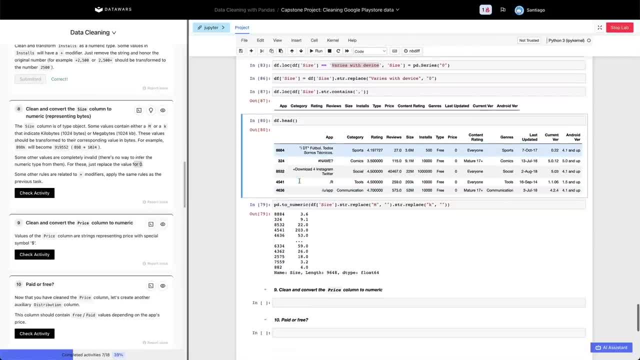 potentially convert if we fix the issue with the M on the K, let's go ahead and do with the M on the K. let's go ahead and do with the M on the K. let's go ahead and do it once again. we did it already this. 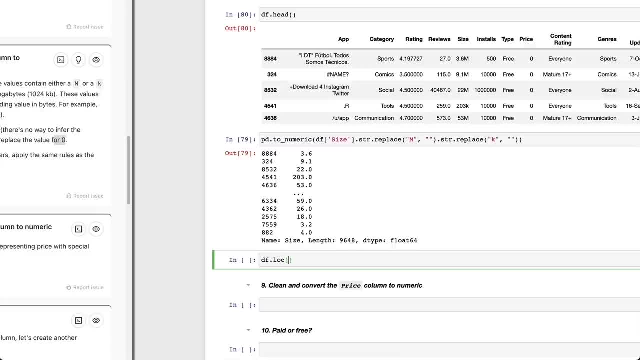 it once again. we did it already. this it once again, we did it already: this process. basically, what we're gonna do is process. basically, what we're gonna do is process. basically, what we're gonna do is the F that lock. let's start with the. the F that lock. let's start with the. 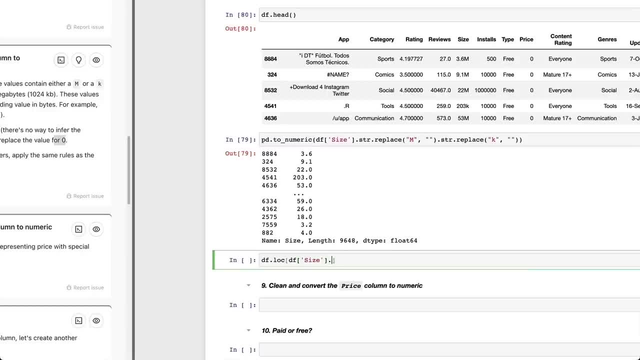 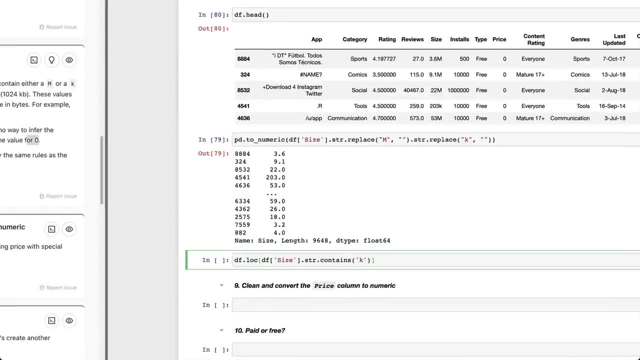 the F that lock. let's start with the kilobytes: the F at size dot STR. that kilobytes the F at size dot STR that kilobytes the F at size dot STR that contains the K: okay, lower lower case K. contains the K: okay, lower lower case K. 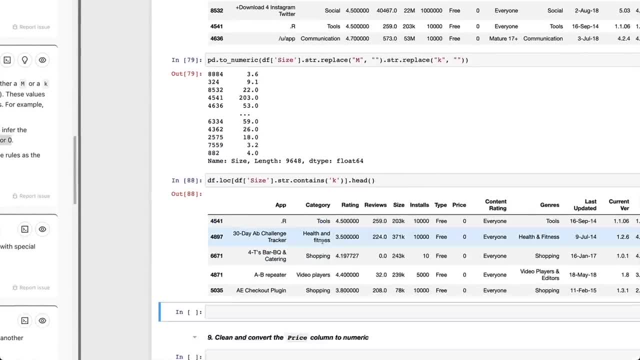 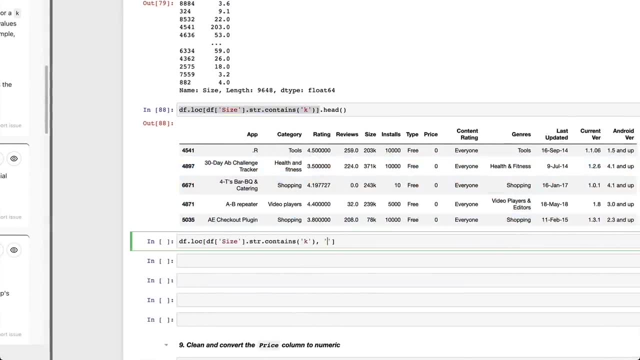 contains the K: okay, lower lower case K. really quickly, let me check that and really quickly, let me check that and really quickly, let me check that. and what we're gonna do now is we are gonna. what we're gonna do now is we are gonna. what we're gonna do now is we are gonna take these reviews no size. that's what. 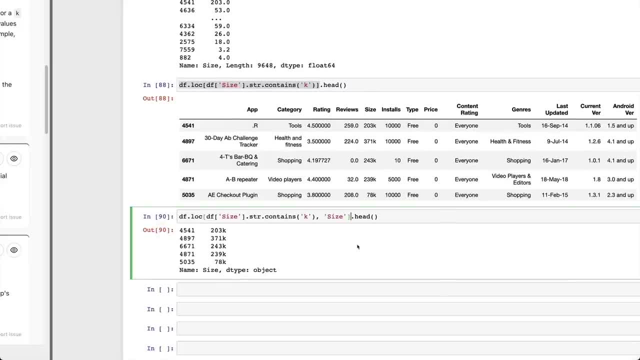 take these reviews: no size. that's what. take these reviews- no size. that's what we're looking for and basically we want, we're looking for and basically we want, we're looking for and basically we want to convert this thing. we're gonna to convert this thing, we're gonna. 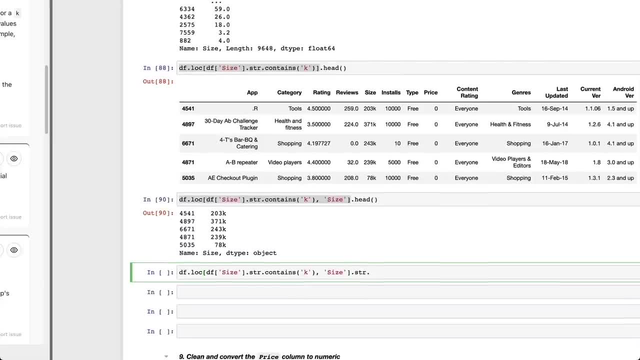 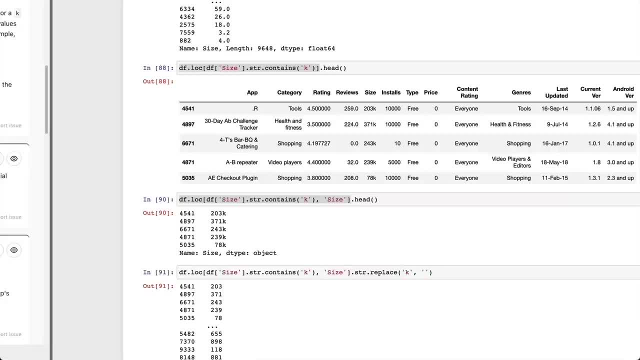 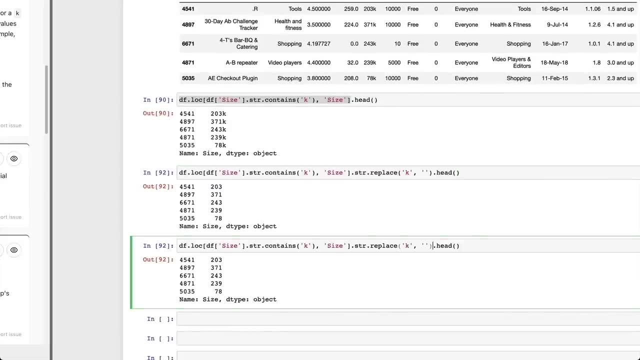 convert this thing. dot STR thoughts replace the. convert this thing: dot STR thoughts. replace the K with nothing right. we want to go we K with nothing right. we want to go we K with nothing right, we want to go. we want to now turn this thing into numeric. 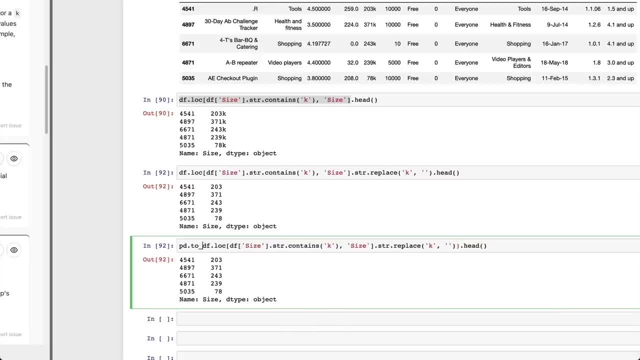 want to now turn this thing into numeric. want to now turn this thing into numeric. PD dot to numeric, there you go. but these PD dot to numeric, there you go. but these PD dot to numeric, there you go. but these are kilobytes and what the activity is. 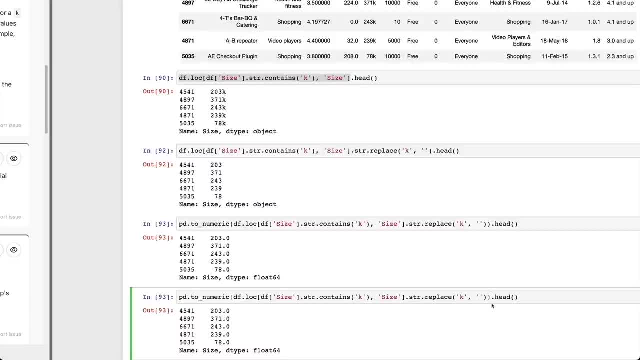 are kilobytes and what the activity is are kilobytes and what the activity is asking us is for megabytes. so we're asking us is for megabytes. so we're asking us is for megabytes. so we're gonna do now. sorry for bytes, these are. 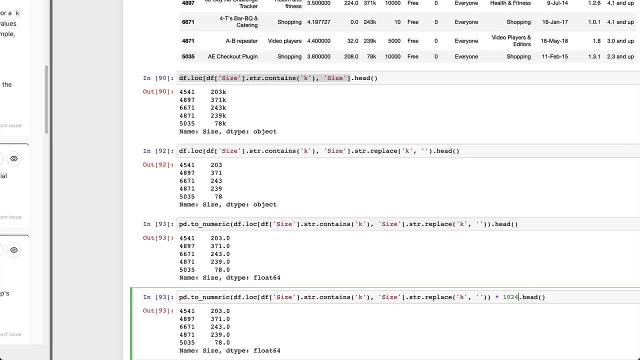 gonna do now sorry for bytes. these are gonna do now sorry for bytes. these are kilobytes. is asking out for bytes. they, kilobytes. is asking out for bytes. they, kilobytes. is asking out for bytes. they have to multiply this whole thing by. have to multiply this whole thing by. 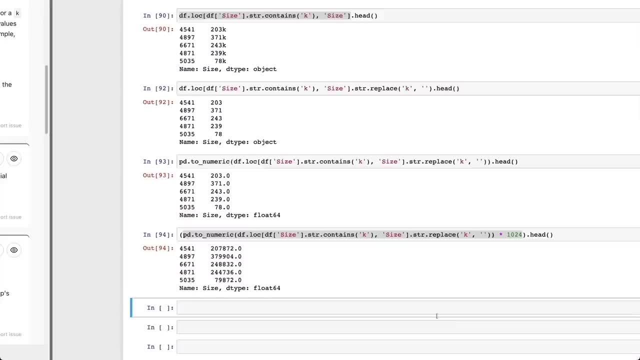 have to multiply this whole thing by 20: 10 if 10, 24, and now these are kilobytes: 20, 10 if 10, 24, and now these are kilobytes: 20, 10 if 10, 24, and now these are kilobytes. so basically what we are able. 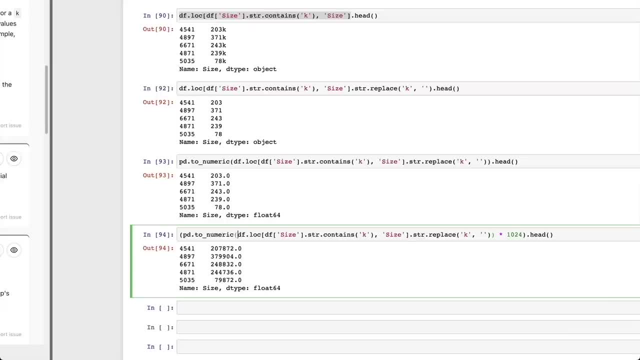 so, basically, what we are able, so basically what we are able to do now is as usual we're gonna get to do now is as usual. we're gonna get to do now is as usual: we're gonna get this thing, those sizes, and we're gonna this thing those sizes, and we're gonna 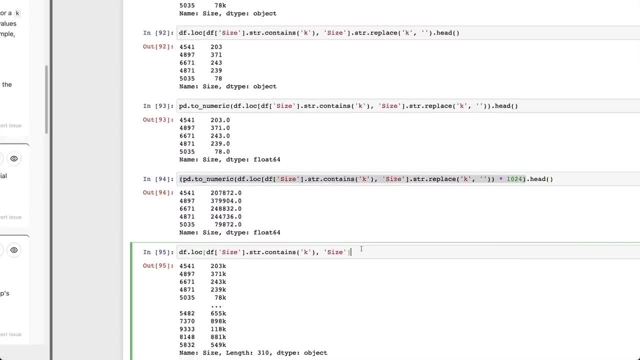 this thing, those sizes, and we're gonna assign them to this thing right here, and assign them to this thing right here, and assign them to this thing right here, and this is gonna be a long string and the this is gonna be a long string and the this is gonna be a long string and the size of the lines is not great. there we 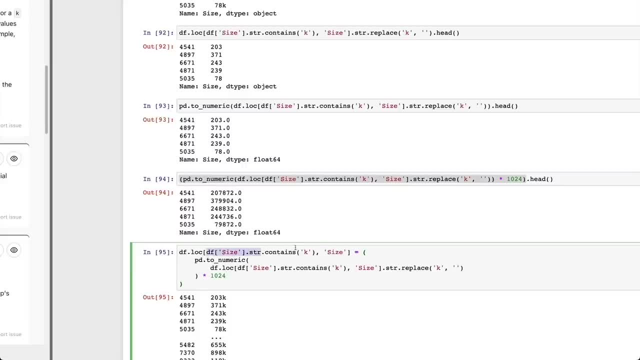 size of the lines is not great, there we size of the lines is not great, there we go. so what we're doing is selecting all go. so what we're doing is selecting all go. so what we're doing is selecting all the rows that have a K, turning dot K to. 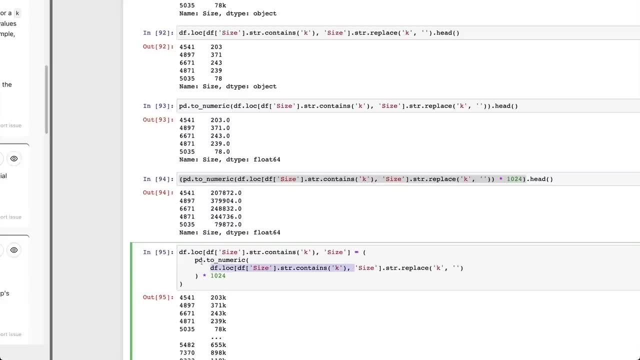 the rows that have a K turning dot K. to the rows that have a K turning dot K to a. removing the K turning into a number. a removing the K turning into a number. a removing the K turning into a number. multiplying it for 1024. because 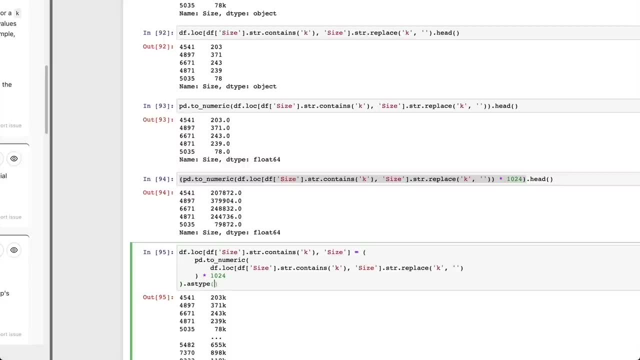 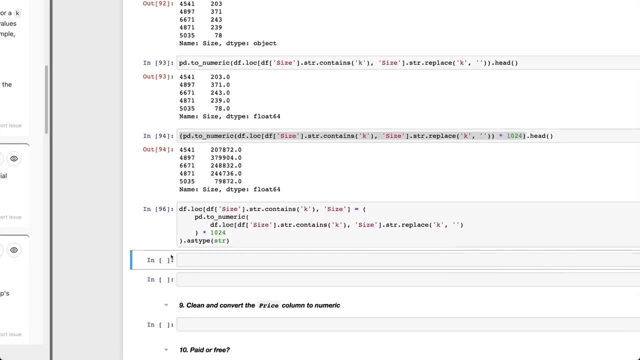 multiplying it for 1024, because is going to be bytes, And at the end, as usual, we want to keep that as a string. There you go. We're going to do the same thing now with megabytes. I'm just going to replace m. 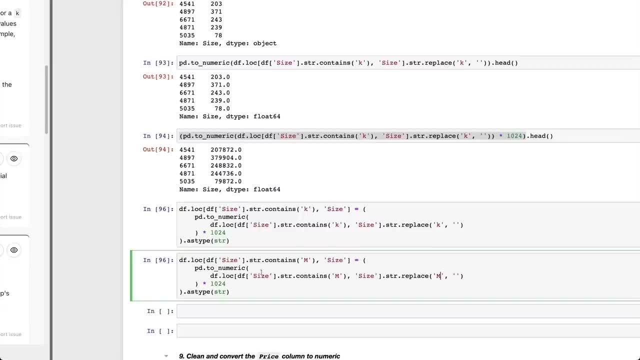 m, m and m, m, m, m, m. And of course here is 1024 times time, 24 for megabytes. I'm going to do that. Finally, PD to numeric of DF at size it works. Let me show you. 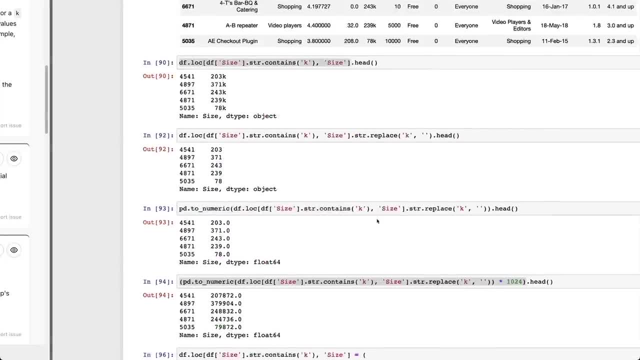 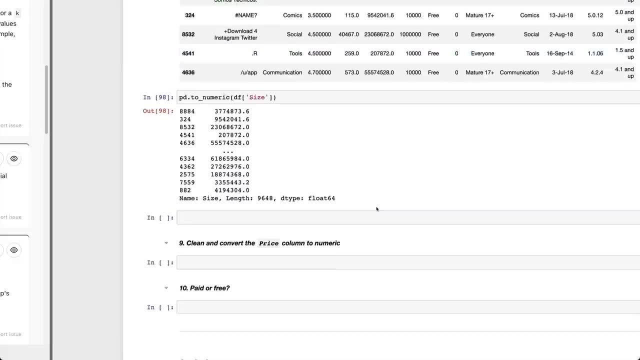 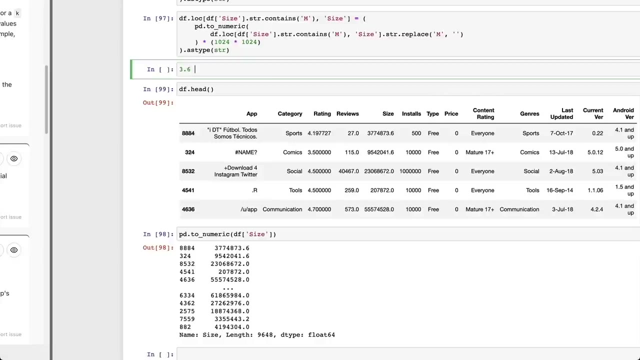 the size now. So this was three something. maybe we have a copy here. size is pure 3.6. And so that is 3.6. And this one right here was 3.6. m. So 3.6 times 1024 times 1024. 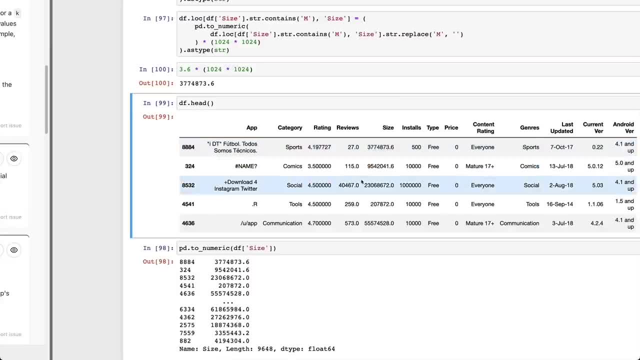 is pretty much the same value we have right here, So it's good, But it's still an object because we're using strings for everything, which is a good thing. Keep strings, keep strings, keep working with strings until you're good. I'm sure you want to convert that into a number. 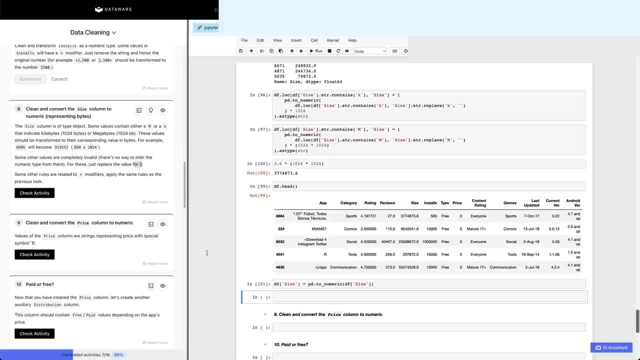 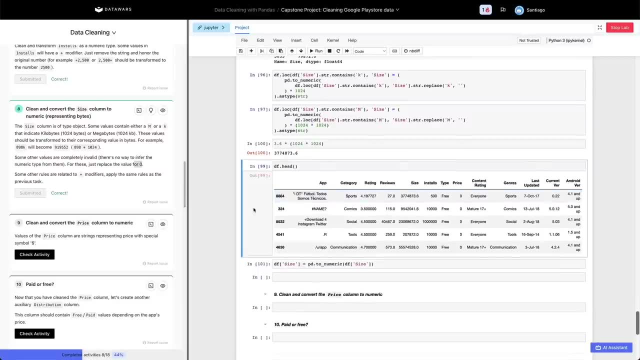 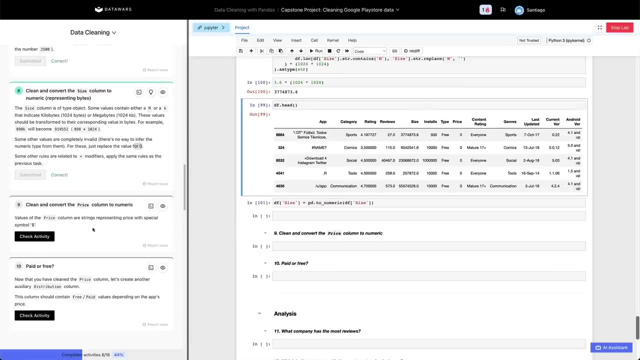 we can do that right now. And let's check the activity. This was a long one, took a little bit of wrangling, There you go, But finally we have successfully claimed it. All right, moving forward, clean and convert the price column to numeric. 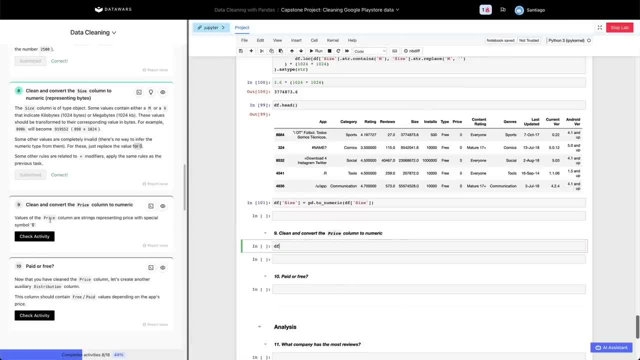 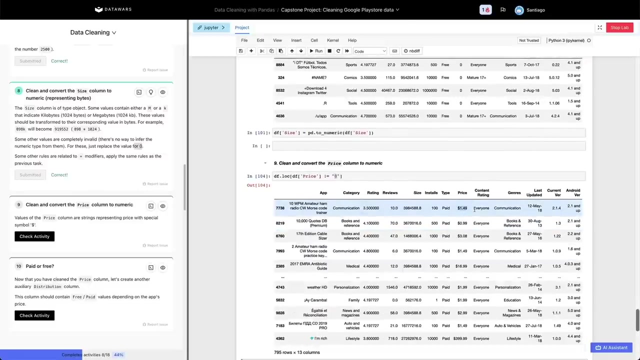 clean and convert the price column to numeric. The value represents with a dollar symbol at price dot. different zero, The f dot block. we're gonna check a few prices. That zero is a string. There we go: 1.49. Seems to be good. Let's check if there is one that has a comma or anything like. 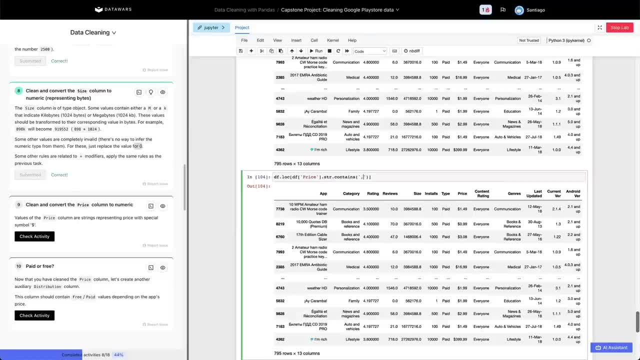 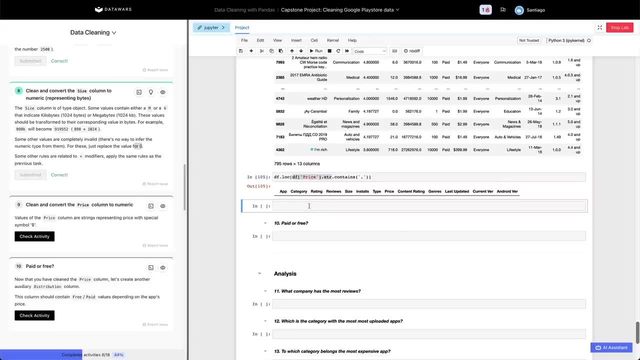 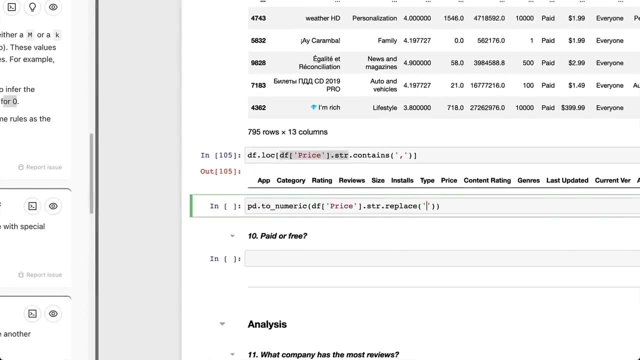 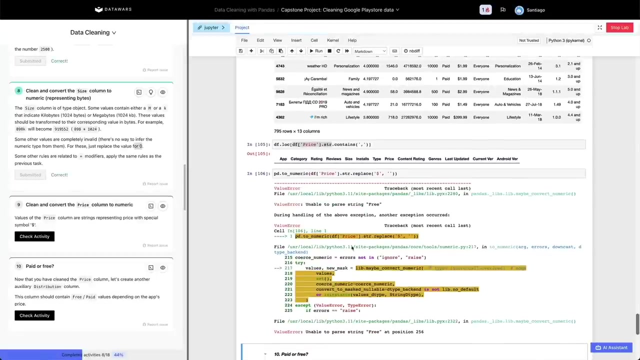 that contains a comma, nothing. So I think we can just let's, let's try it out. What if we do p.0, the dots- I mean Chris eyes here to numeric of this thing- dot replace dollar symbol with nothing, just dots, oh no. therefore. well, the values? oh because. 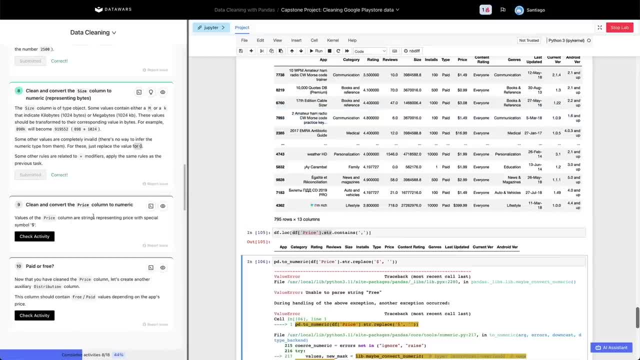 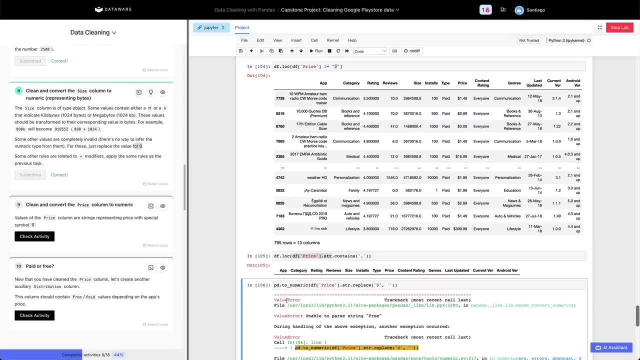 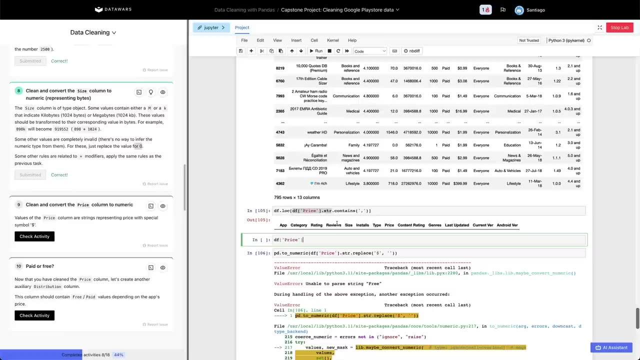 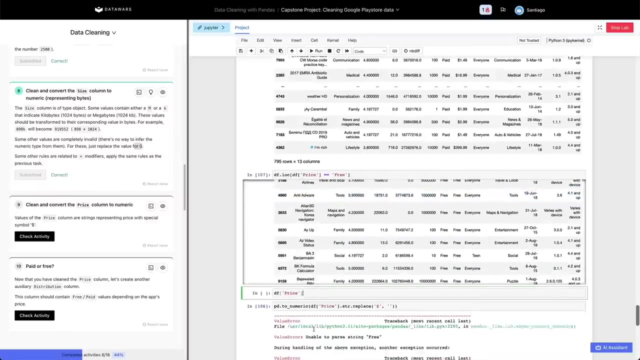 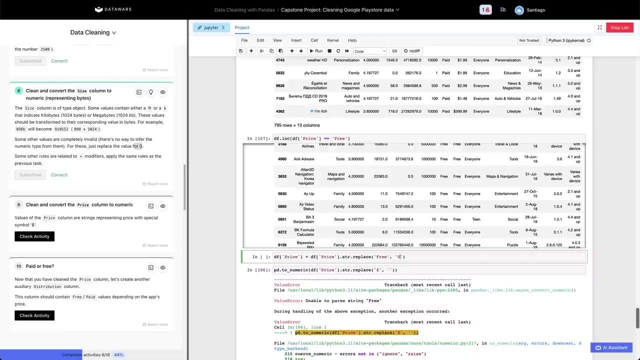 there is a bunch. of price equals free. yeah, symbol that is for prize. all right, so we can do the effort prize you can actually check free. yeah, there are a bunch that are free, so the effort prize equals the effort prize. dot STR. to replace free with a string representing 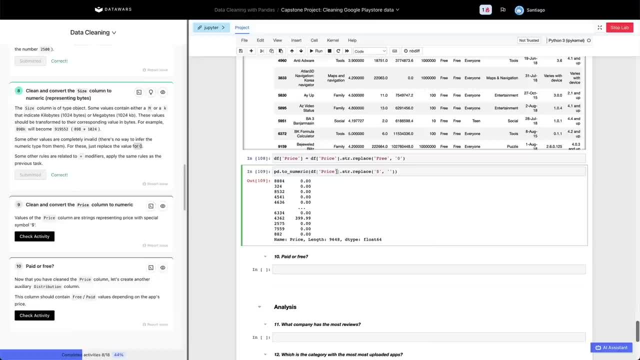 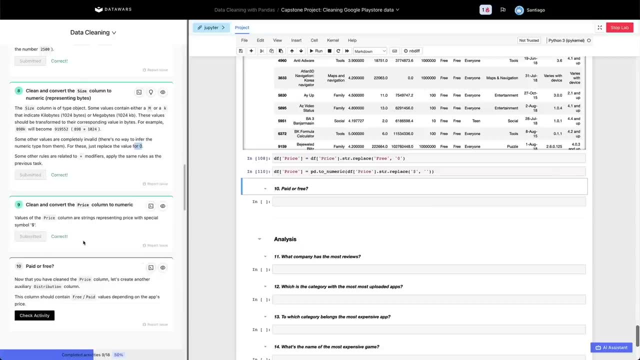 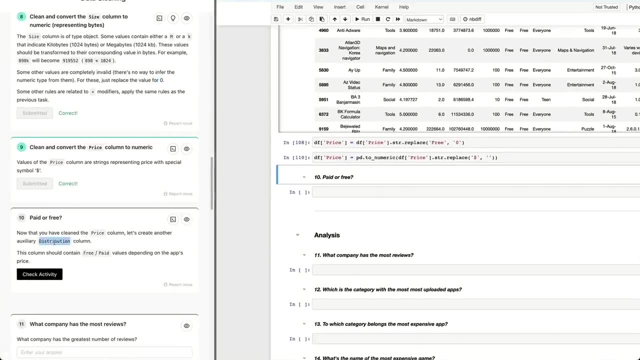 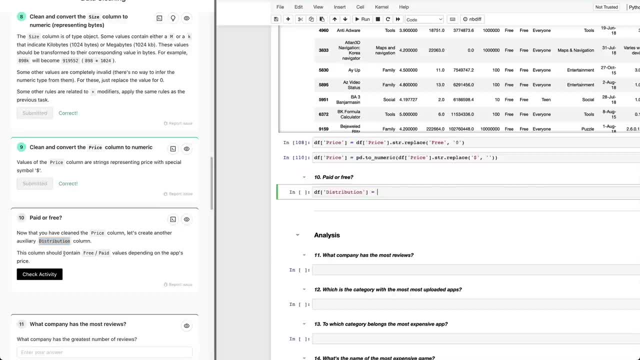 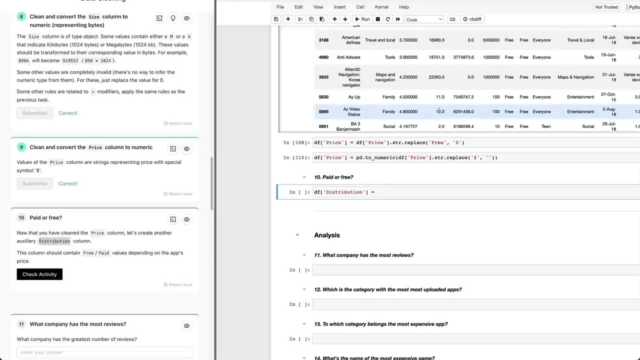 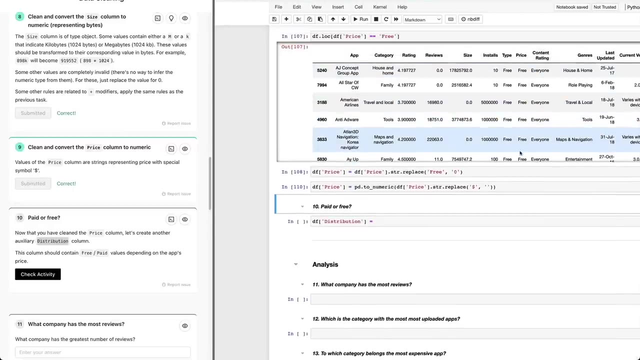 distribution equals. the college could contain free 횡 valleys vending on the app's price. so this is a good one. we could eat rates over each prize price right over the whole data frame of price and just assign one thing or the other. we could use an apply function, we could do something like equals. we could do the effort. 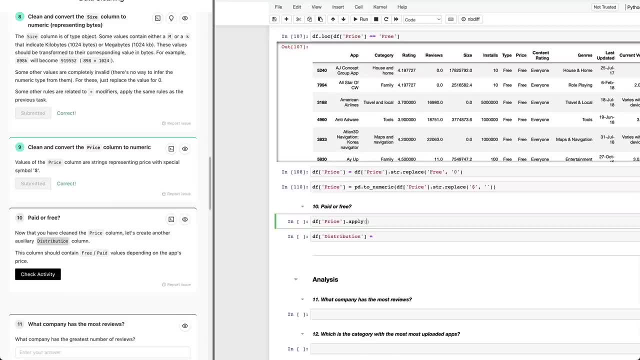 price: dot apply a lambda with a price P and put we can free if P is greater than zero, else paid, and do that and I could assign that distribution as it is. let me check just as we're doing it, but there is. 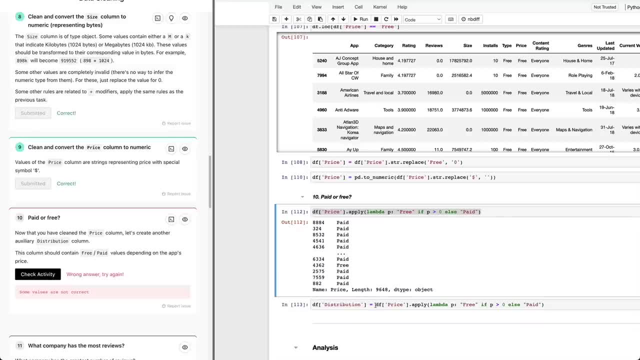 no, didn't work. actually that's a good thing because oh, paid it's on the other way, it's paid if other way is free. I just- and that's why I don't like the apply one and potentially 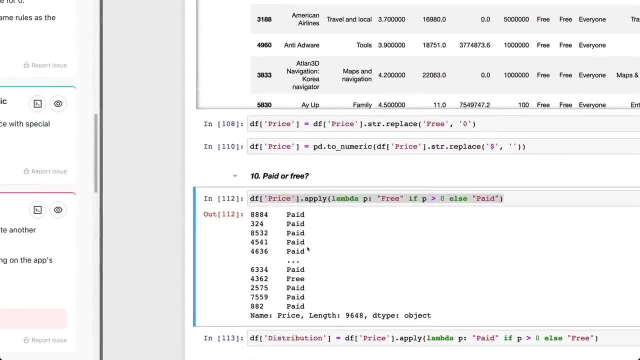 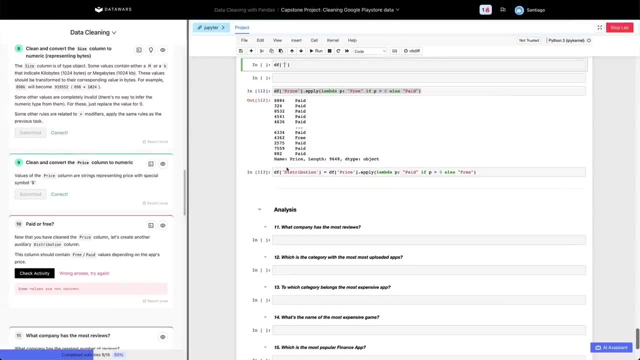 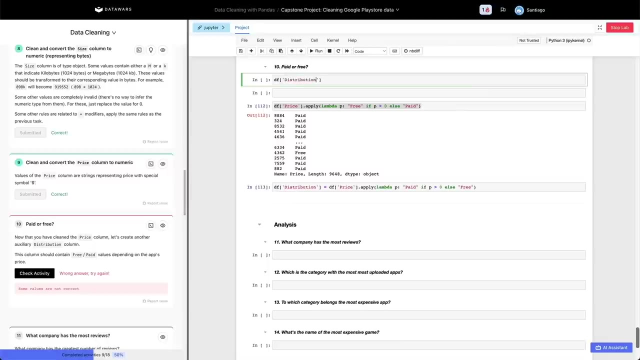 at this stage. if you're just still doing data cleaning, you might not know this method. but there is another, simpler way that is just hacking pandas, which is I will initiate. let's actually see if this works. first distribution or no. I want to use my method, so distribution is going to be. 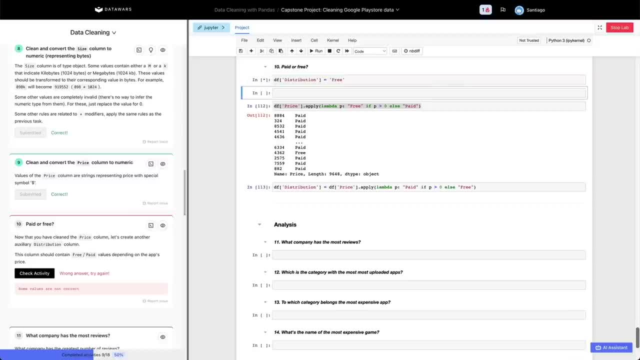 I'm going to say distribution is like everything is going to be free, like let's start that way. it's free, we can check the activity, it is not going to work. no, didn't work, but then we're. 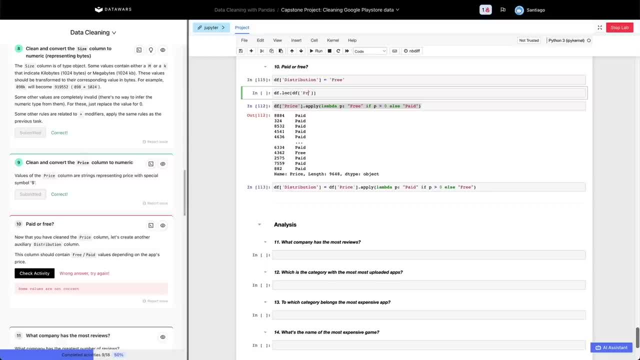 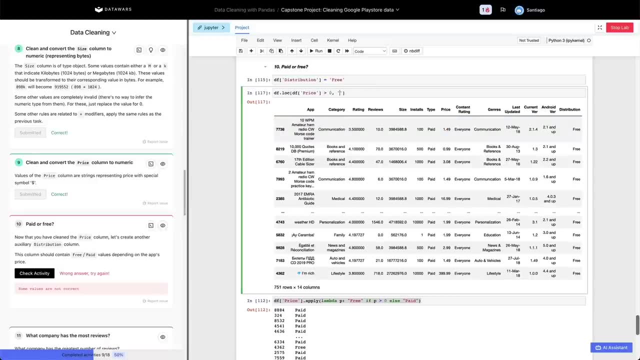 going to say is: df, dot, lock all the apps that have a price that is greater than zero, right that? so price. here we're going to get the distribution column. I want to send that to paid. that way now we can check the activity. 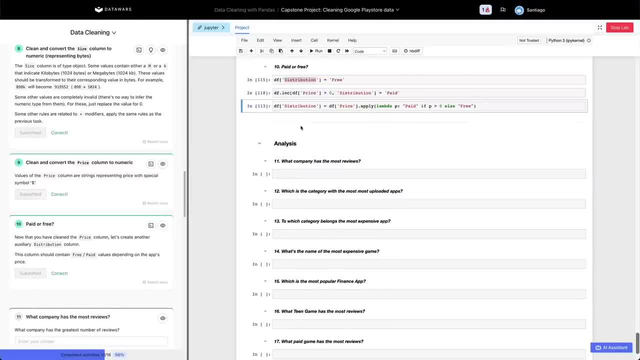 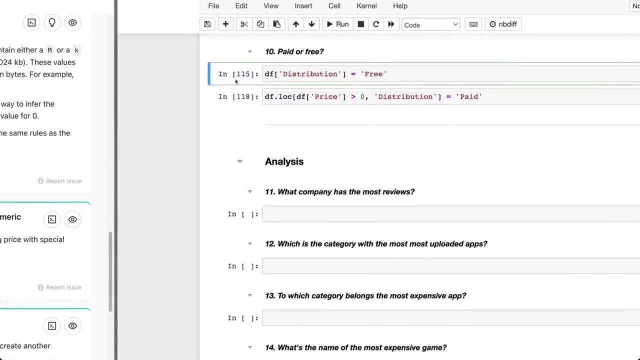 and that works. so the way- and I'm going to get rid of the apply for a sec- the way- this method, which is again the most convenient, is just if you have a few rules, what you can do is just. 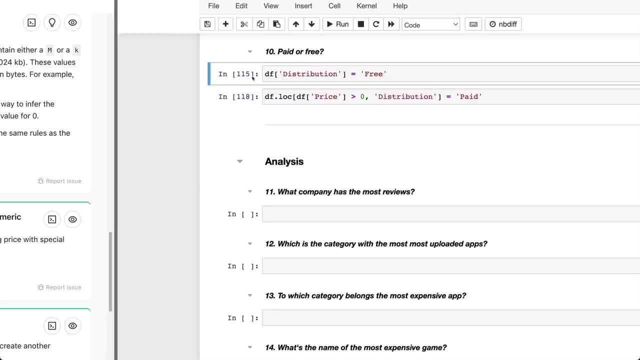 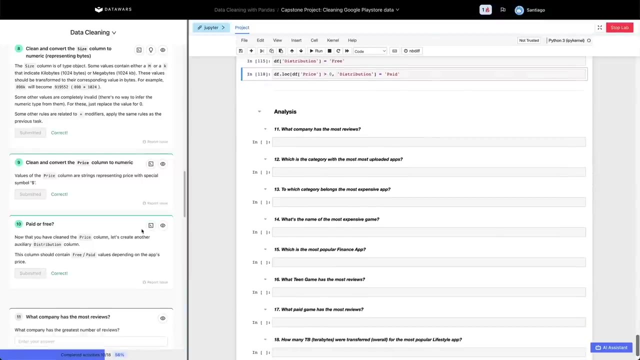 you know, start with the one that is going to give you like 70% of the apps are free, and then just work your way creating other conditions to replace the others. this is a very common technique. all right, now that we have finished with data cleaning, we can just do a quick analysis to 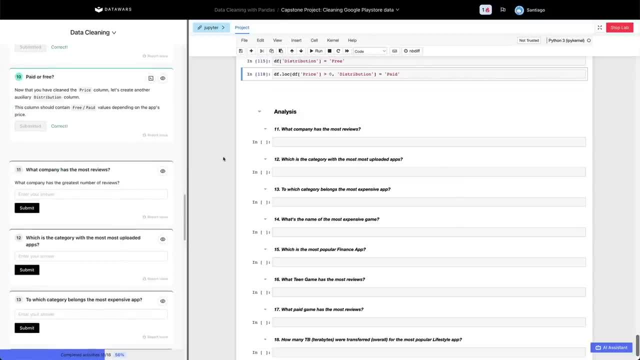 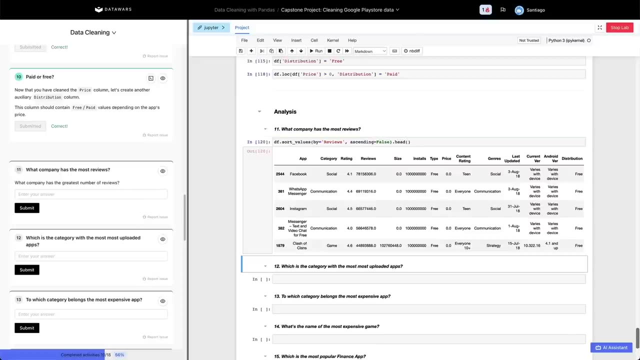 answer all these questions. so what company has the most reviews? we can do something like df dots: sort values by reviews. ascending falls head. by the way, as usual, this is a good time to stop the video. Let's try to resolve it by yourself. I will just, you know, move very quickly over all these. 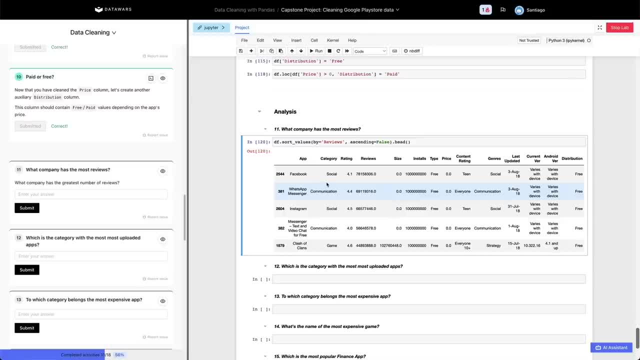 activities, because this is more analysis that we've done. I think it's still interesting, but if you can try to resolve by yourself first and then take a look at the solution, I've done so. the first thing is the app that has the most reviews. this works also, as usual. 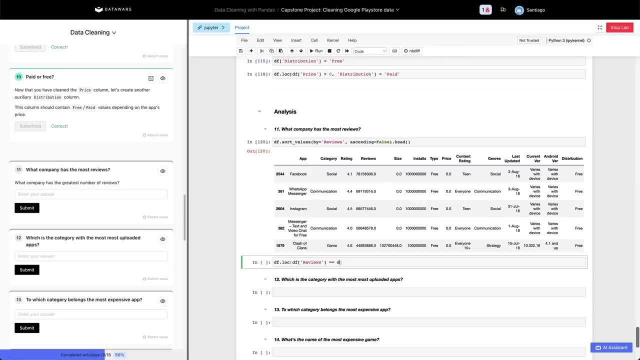 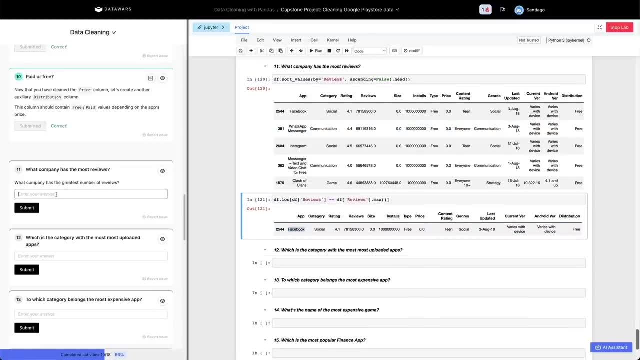 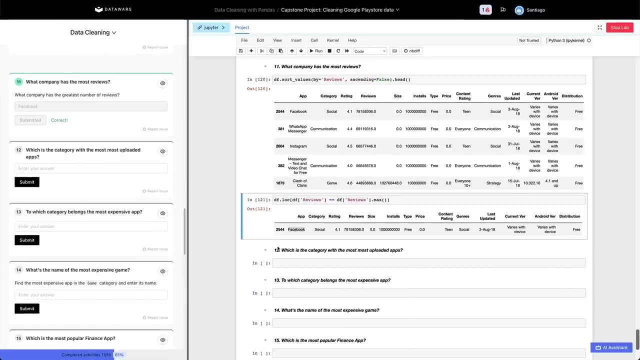 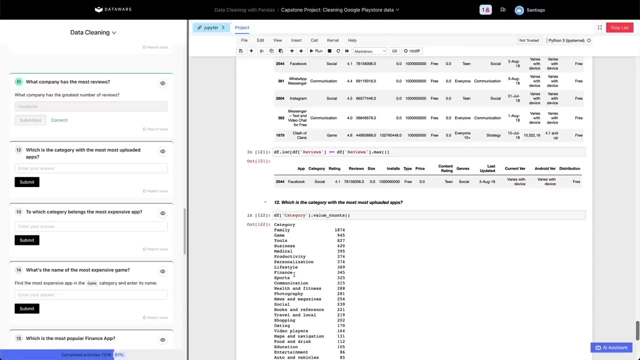 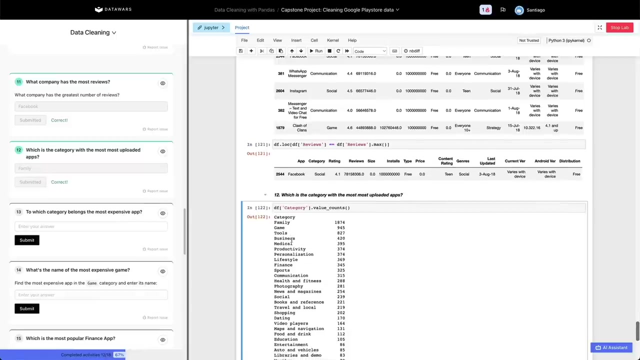 df at reviews equals df at reviews, dot max. that is Facebook Good, which is the category with the most uploaded apps, and this is df at categories: dot value counts. family is the category, it seems, with the most. there you go. apps to which category. 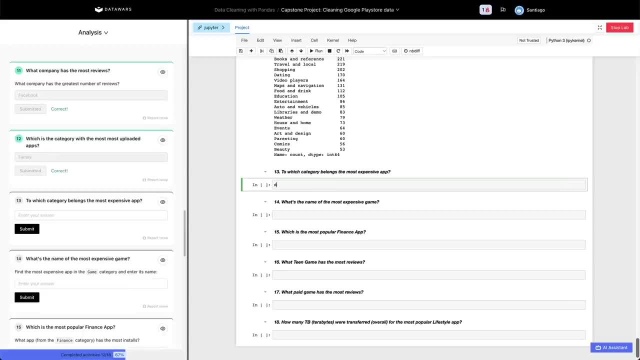 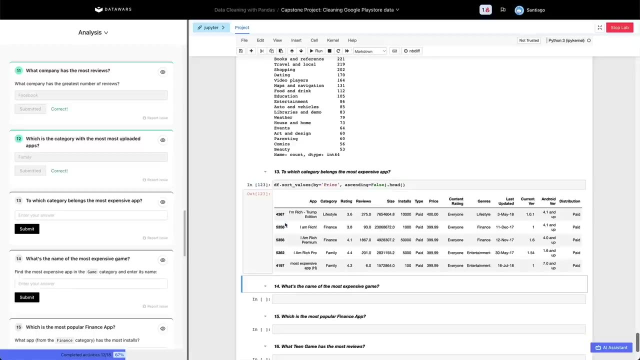 belongs the most expensive app. so we can do df, dot sort values as usual by price. ascending falls dot head. and I'm rich: Trump edition lifestyle. what's the price? $400 for an app. okay, I'm gonna do that and it worked again. 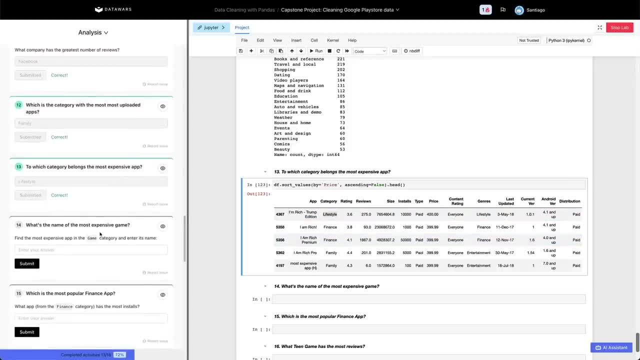 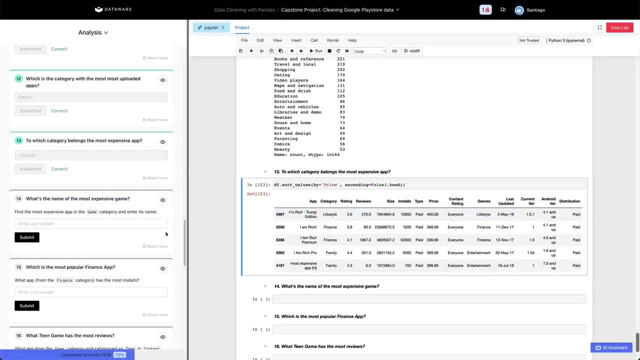 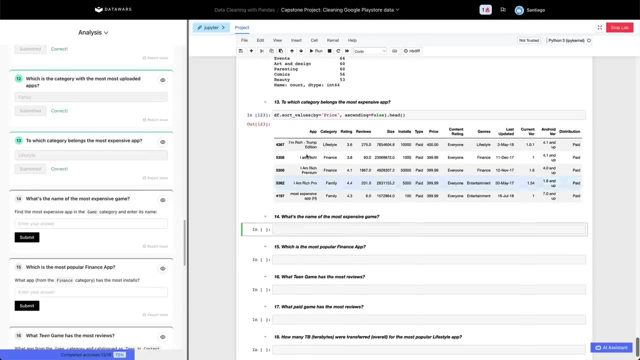 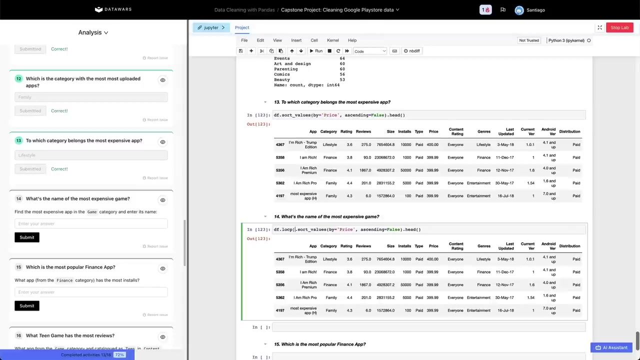 it's a live type application. What's the name of the Most expensive game? What's the name of the most expensive game? Find the most expensive app in the game category and enter its name. so, basically, we're gonna do the same thing as here, but we're gonna lock here. we're gonna do, we're gonna do query. 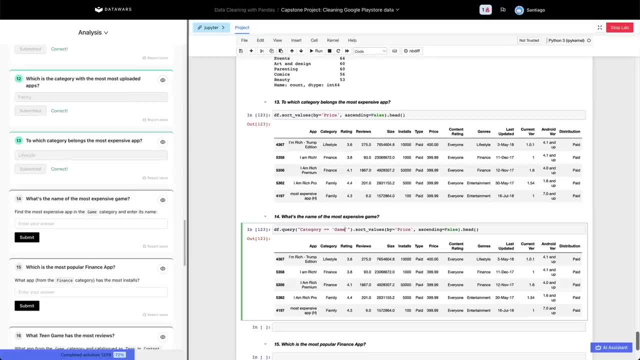 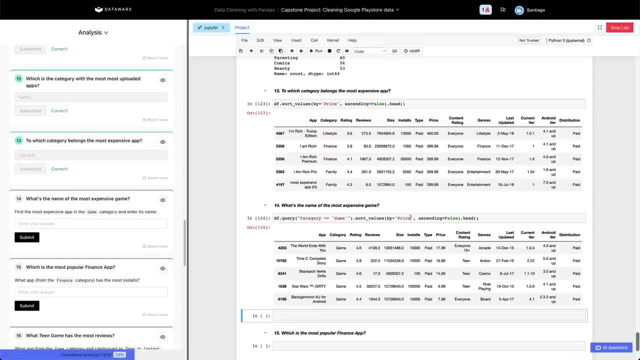 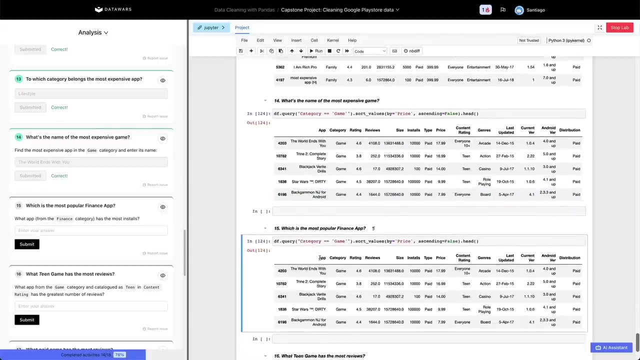 where the category is game and the game seems to be find the most expensive app in the game category, the world ends with you, it seems. there you go, which is the most popular finance app. so basically we need to first filter by finance. so category's gonna be finance. 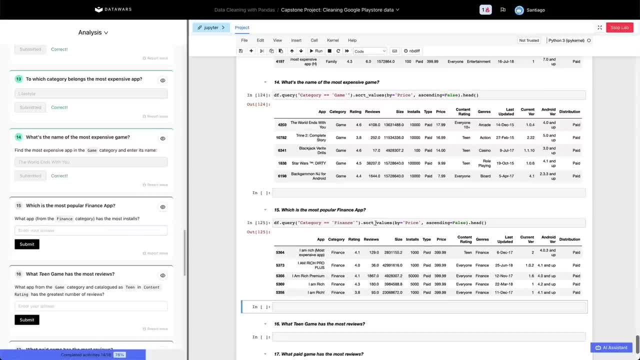 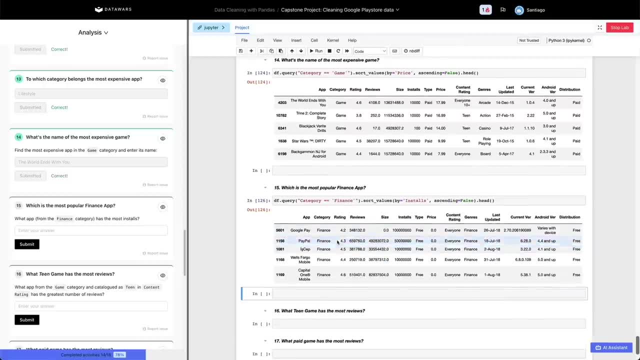 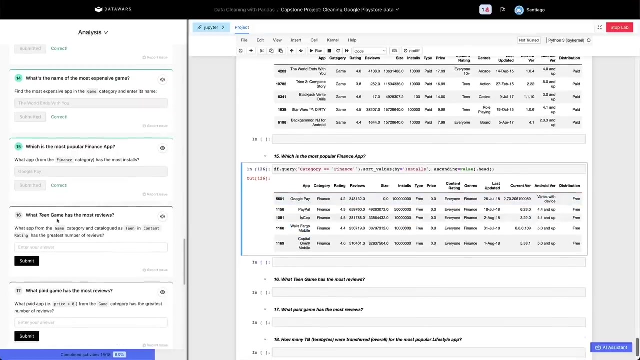 and then it says with has the most installs. so we have to sort by installs and that's. it seems to be in finance. the most popular app- which is kind of obvious, i hadn't thought about that- is google play, google pay- sorry, that makes total sense and that activity also passes. what team? 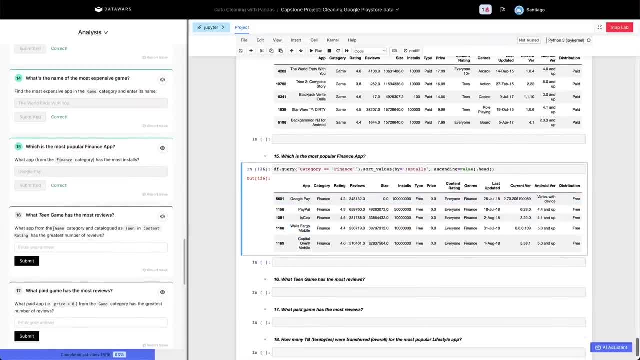 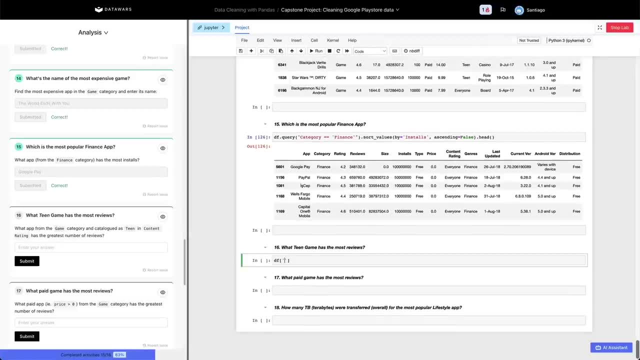 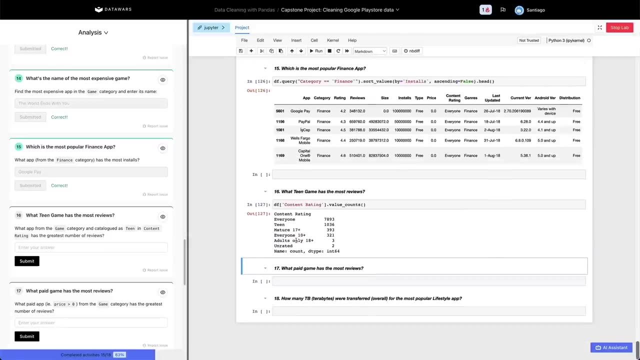 game has the most reviews. so what up from the game category and catalog as team in content rating. so df, at content rating the value counts. we haven't looked at all the content ratings yet. uh, teen, okay, so we're gonna find. we're gonna find the app from category equals game, it seems. 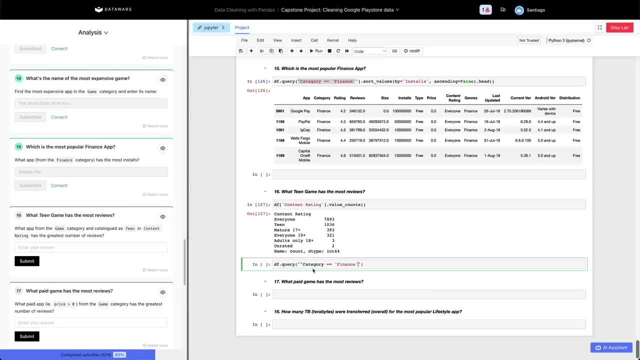 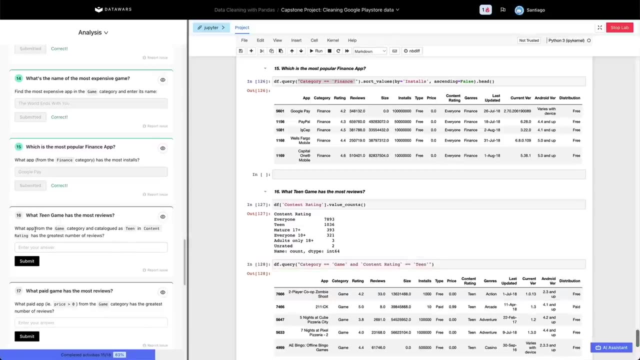 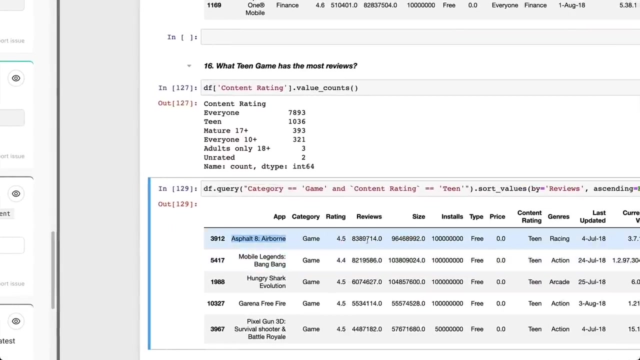 uh, category game and content rating equals team thoughts and we're gonna find the one that has the greatest number of reviews or the maximum number of reviews, and sort values by reviews ascending falls. first five: asphalt 8- airborne seems to me seems to be the most popular in terms of reviews of. 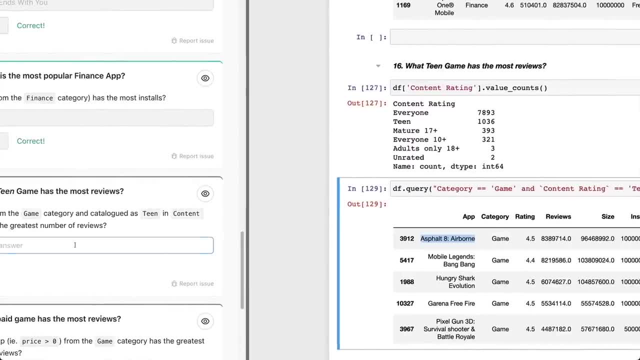 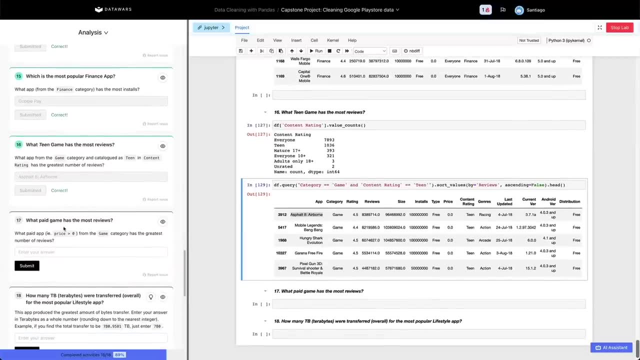 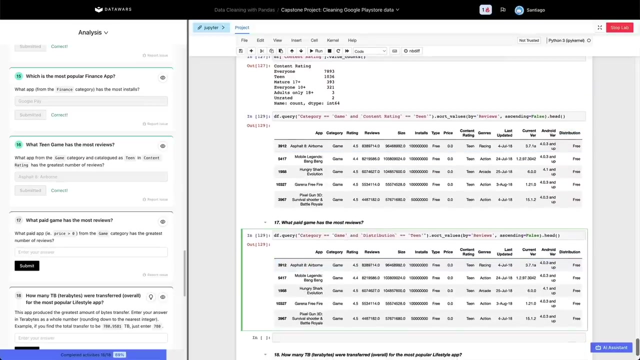 all the games, our content rating team. let's take a look. yep, that worked as expected. what paid game has the most reviews? so we have to find a game that's, let's say, let's use our distribution column column that is here paid and has the 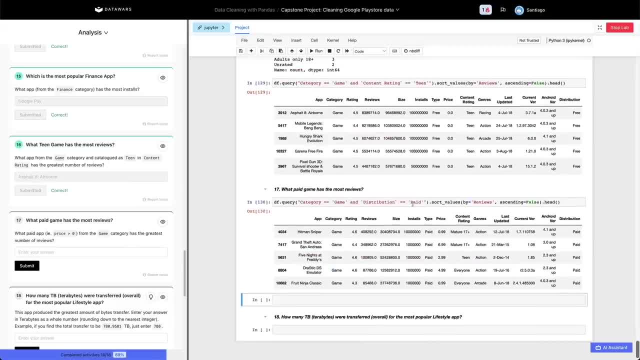 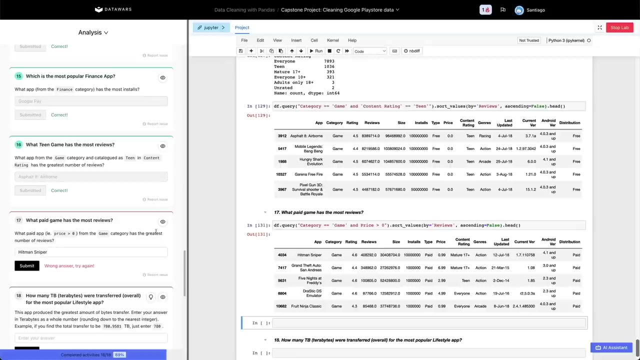 most reviews and it's going to be the same thing. okay, um, distribution paid and it's again. it has the most reviews. price equals greater than zero by reviews ascending faults, hitman sniper- no, because we probably need. and price creating zero. what paid up from the game category. 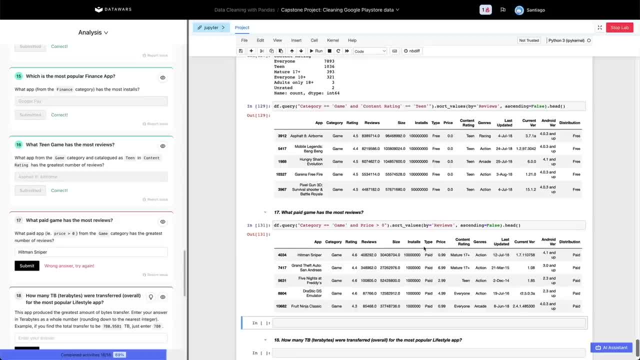 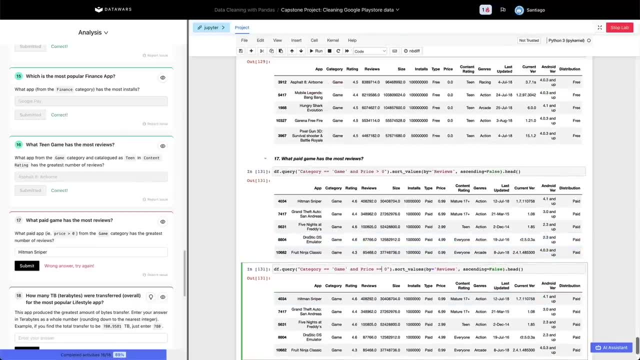 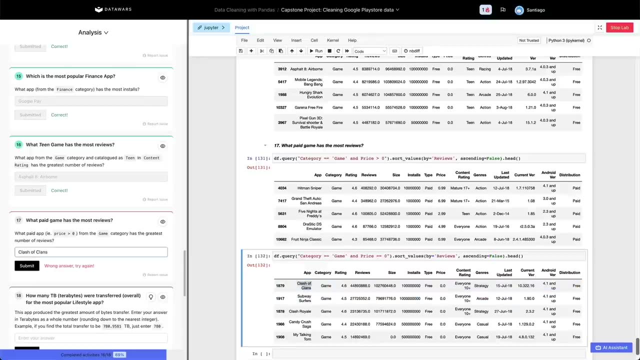 category game has the greatest number of reviews. huh, what if cache of clans? let's, let me try this, because i found an error. yeah, so this activity should be what free game has the most reviews, so we have to fix that. ideally, by the time you're watching this, that has already been fixed. 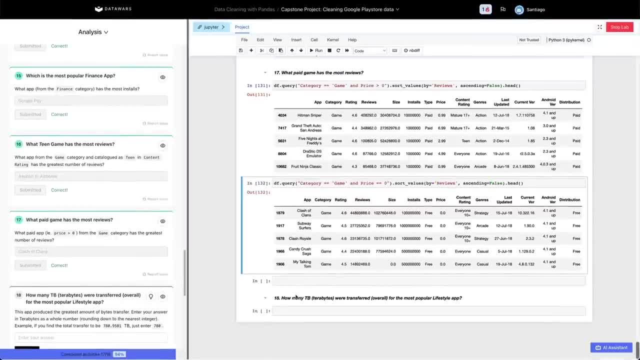 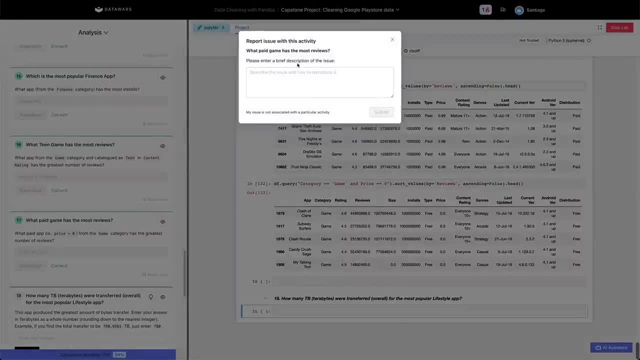 so let's keep moving forward. finally, how many terabytes we can actually report an issue right here? for the previous one report an issue, the activity is asking for uh paid apps, but the solution is for free apps. here let's stop, because we already know that uh, the apps do need to purchase. 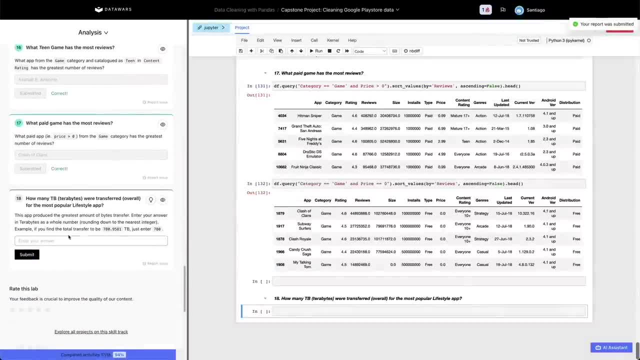 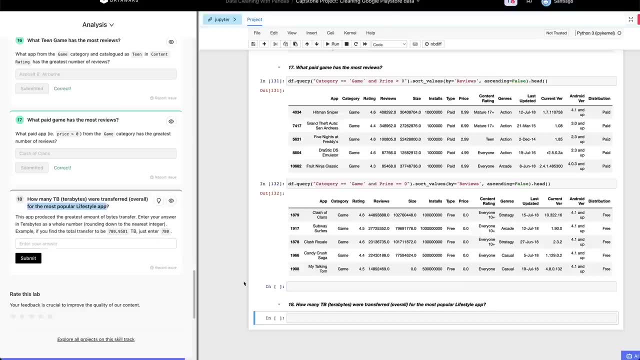 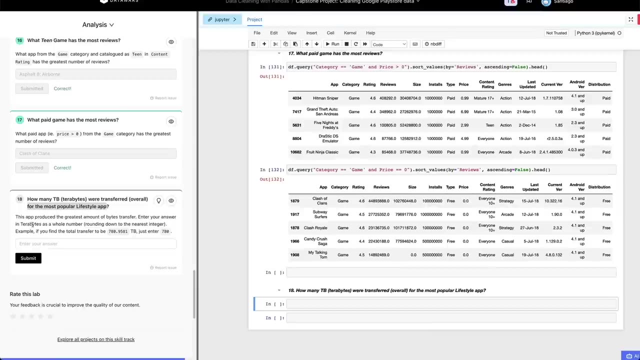 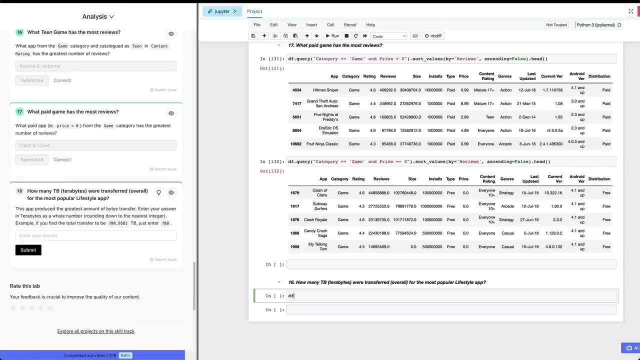 the app. so another example why this is happening to me: because some services are not yet fully Rome, this is like 20%, and you know there's that, but that's nothing new. it's an p physical app and so的話, uh point, just enter 780.. So the app most popular is going to be the F dot query. we're going to say: 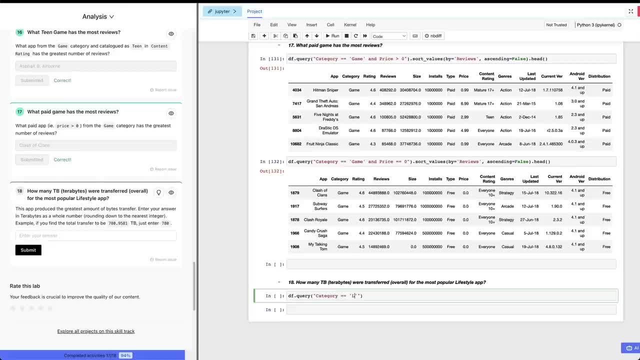 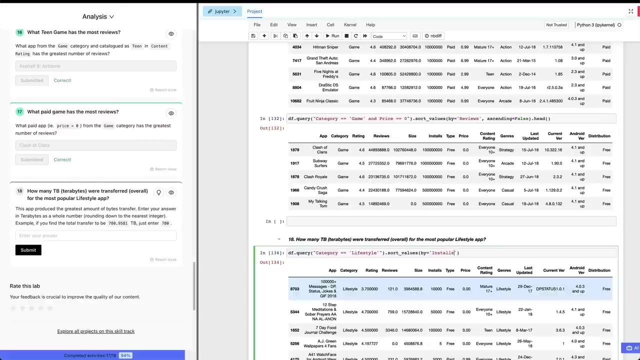 as usual. category equals live style. Yes, no, what's the name? The live style. There you go. sort values by short values by by installs is the one that produced it. So this is the app that I was installed in the greatest amount of times, like most times, And 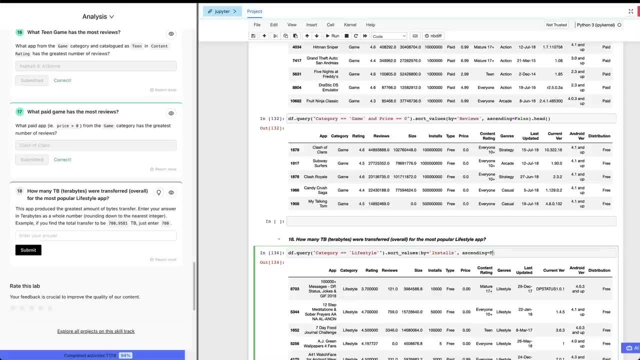 we're gonna do ascending falls and do i log zero right on. let me show you that first. So Tinder was the app that we launched this time. Yeah, you would what? which app, I guess. Well, from the thing, yes, Yeah, are you kind of working on, say, like OEM Region here in the 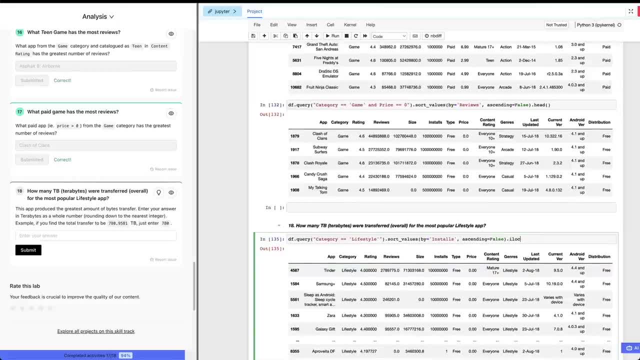 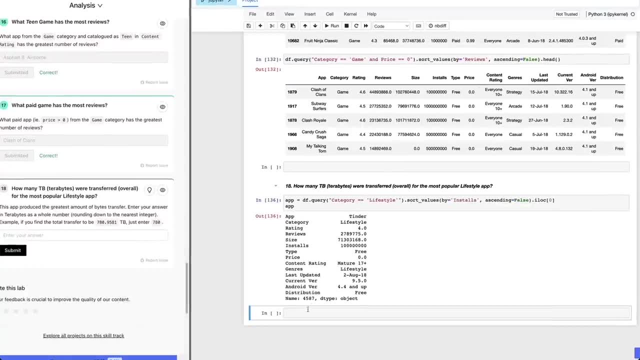 ế sonst dialogue. Yeah, there's a few accounts that I can change it to. Yeah, there is one from an app with the most installs. i'm going to do that. i locked zero so i get this first row. i'm going to show you app. these are app and now we have to do app. so this app wants to install this many times. 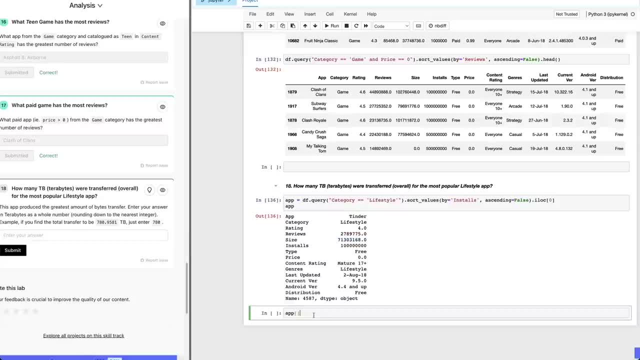 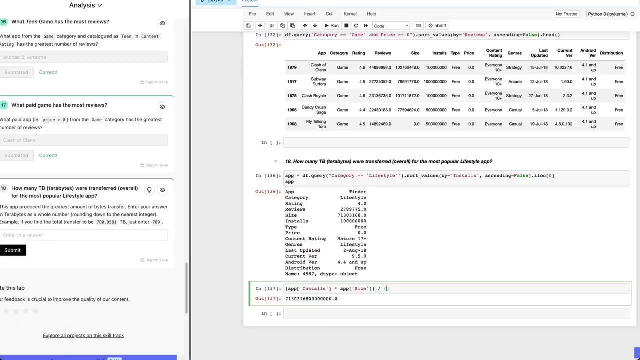 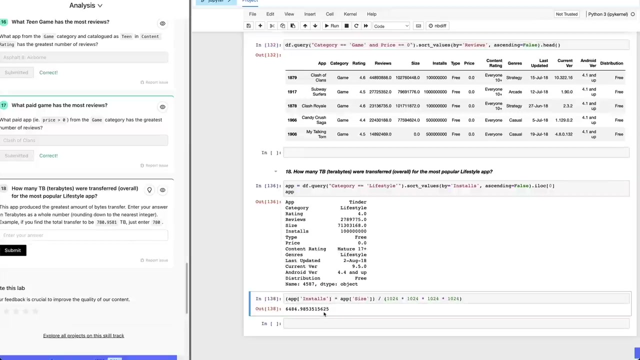 and the size? is this size in bytes, right? so that's going to be up at installs times, up at um size, right? but this is in bytes. we have to divide until we reach terabytes. it's going to be kilobytes, megabytes, gigabytes, terabytes. there we go. so let me show you the previous one: these many bytes, these many terabytes. 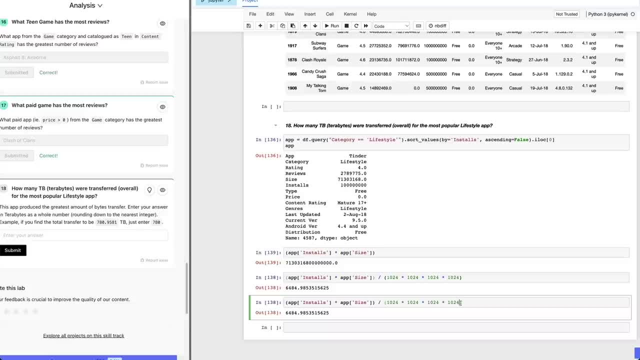 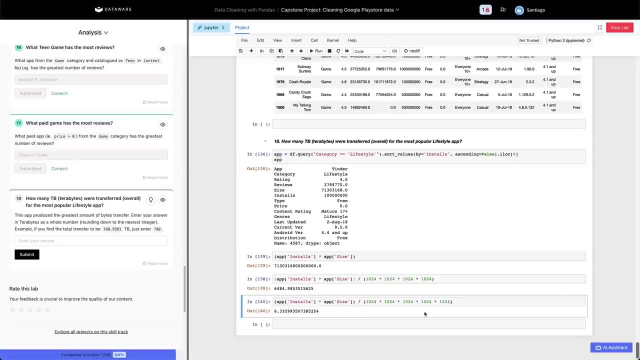 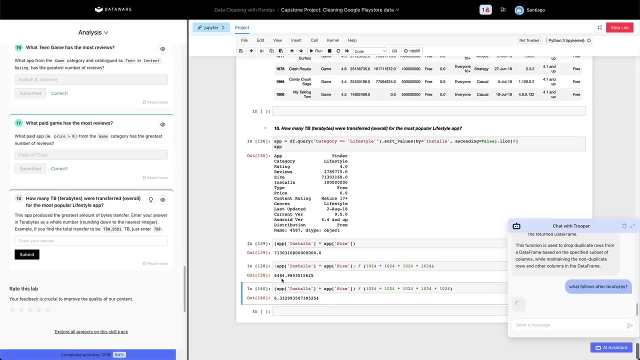 change transferred and i think what do we have? we can, we can actually do it in the the following, so six, i think it's petabytes, so we can ask the assistants, just in between, what follows after terabytes. um, so, basically, this is the answer in terabytes. it says to just enter the whole. 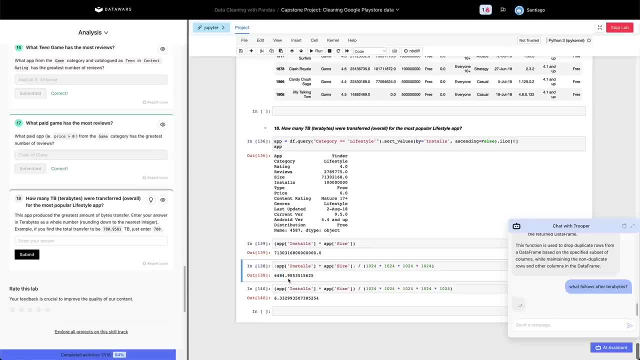 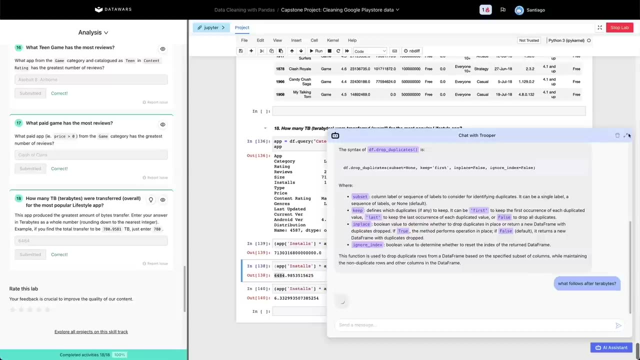 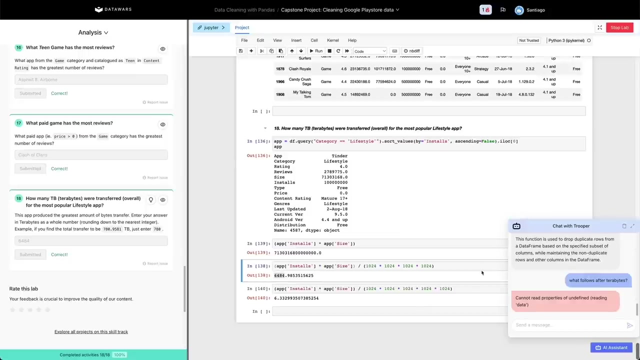 number rounding down, so we're gonna put just six, four, eight, four. there we go and this is still working. i can see if we can answer real quick. i think it's petabytes that follows terabytes, but it's a kind of well, it broke anyway. the greatest, the app that produced. 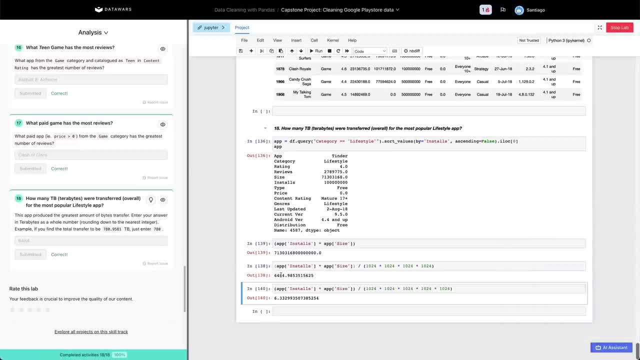 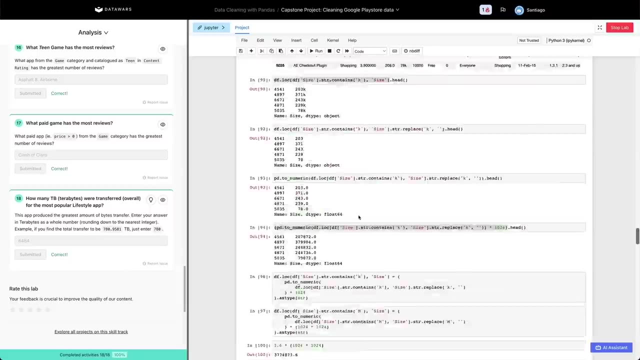 terabytes is the app that produced terabytes, so we're gonna put just six, four, eight four. the biggest amount of data transferred in that case was tinder with 6 000 terabytes, which i think is 6.3 petabytes. i think i'm not sure anyway. um, this is a great project. we did a lot, remember we? 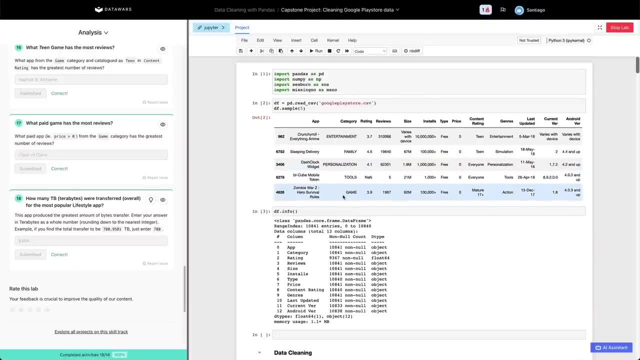 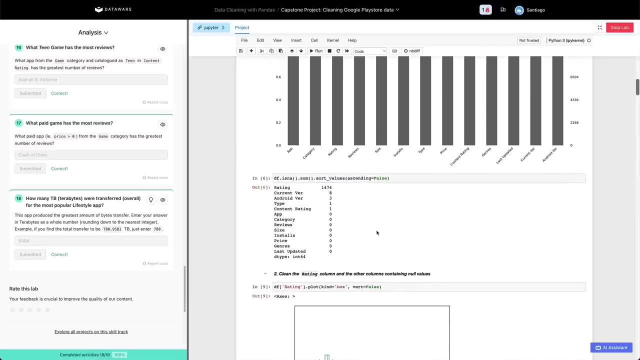 started with the whole data craning process which, as usual data, we had a lot of detective work. we had to find out why some of these columns were incorrectly parsed objects. that was suspicious. we started removing things. turning to the metric, as usual, keep trying to keep everything. i think there. 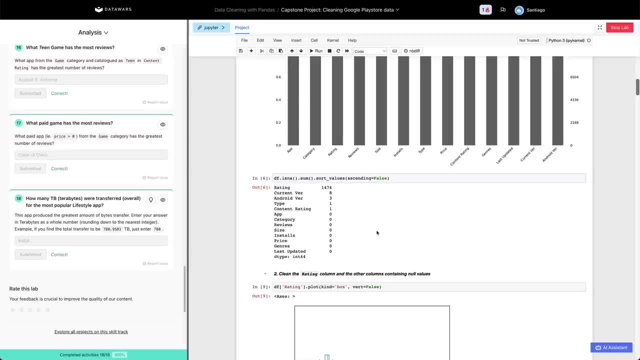 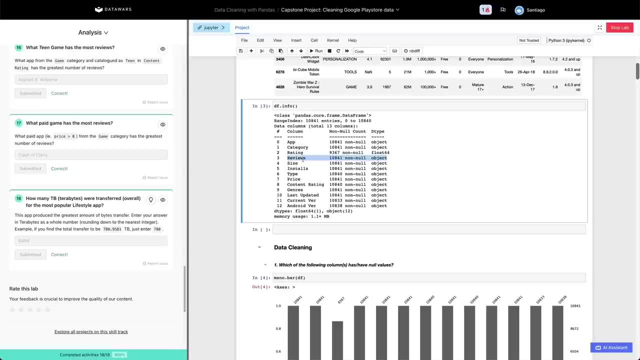 are two or three very important things that i'm trying to transfer to you here, and the first one is that, um, this detective work, you know, trying to turn things to numeric and try to find out where the issue is, removing things and doing this iterative work. the second one is, if you're 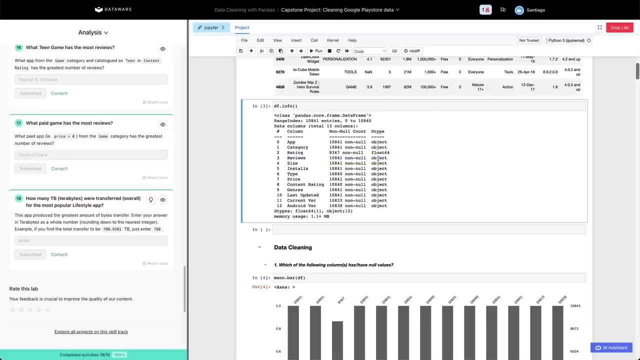 modifying data frame, always keeping copies. we were able to fix an issue by keeping copy um. and then the third one is keeping everything as string until you're safe to turn it back into a number. the same thing is going to apply if you're turning something into a date, first, you know, keep. 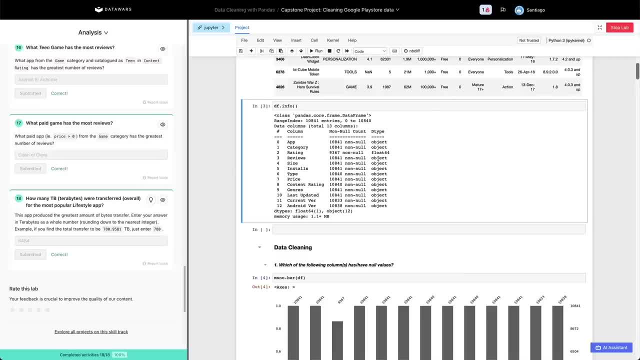 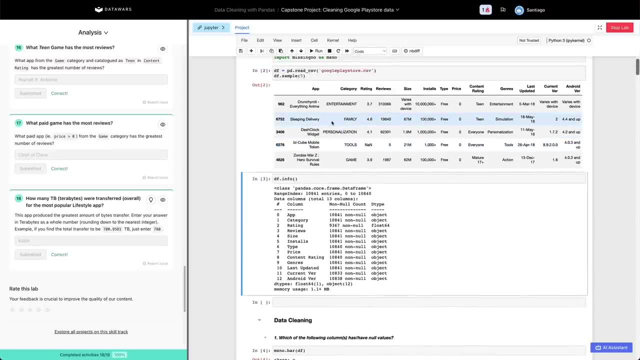 working as string, string strings until you're ready to turn it into a number. but anyway, i think this is very interesting process. also the same: the whole idea behind where the data is coming from. it was scraped, so we were finding the duplicate data. we were assuming that the app 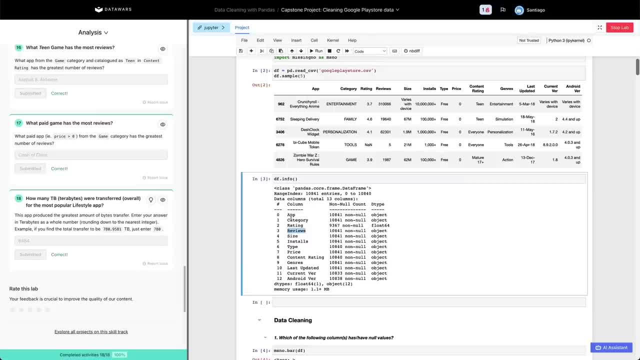 with the most reviews was going to be the app with um. that was the freshest copy. so doing all these. you know, analysis based on our data is basically data science process. so if you are comfortable with this, congratulations, because you're you're pretty, pretty, pretty close. 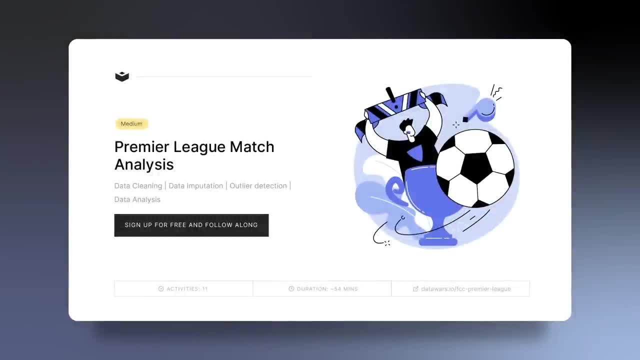 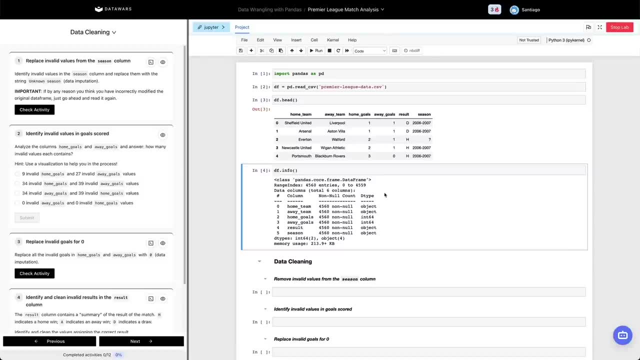 in becoming a data scientist. now, for this project, we're going to combine our data wrangling, data cleaning skills to finally perform some data analysis using group by operation. so it's a pretty interesting one, the data that we're working with, the data we're going to be analyzing. 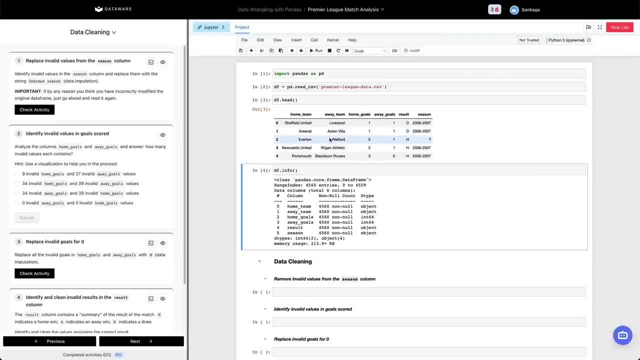 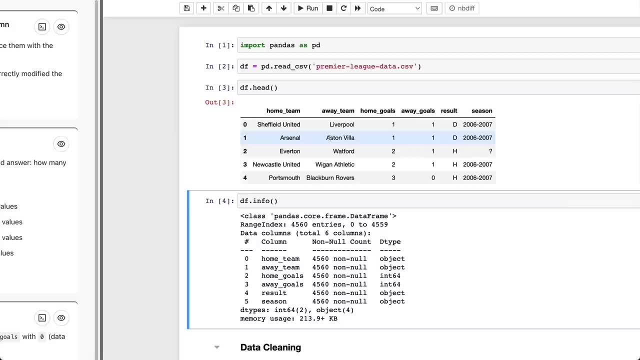 is going to be the data that we're going to be analyzing and we're going to be analyzing the data information about premier league matches. the premier league is the top tier top flight football soccer league in england, potentially in the world, and the data set we have has information. 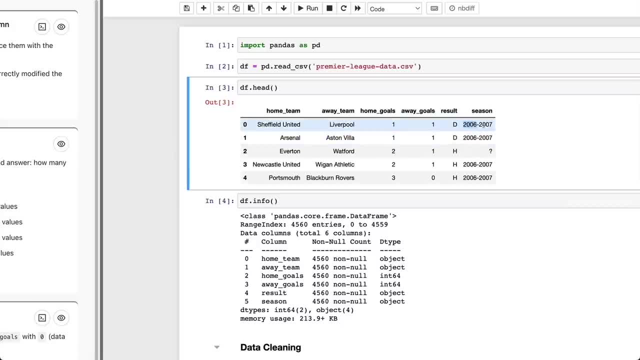 about matches from multiple seasons, starting 2006- 2007 season. um, and it's a very, very interesting data sets because we have the teams played and the goals scored and the final results. so, um, anyway, we're gonna start one by one with the activities, as usual. i want you to just pause if. 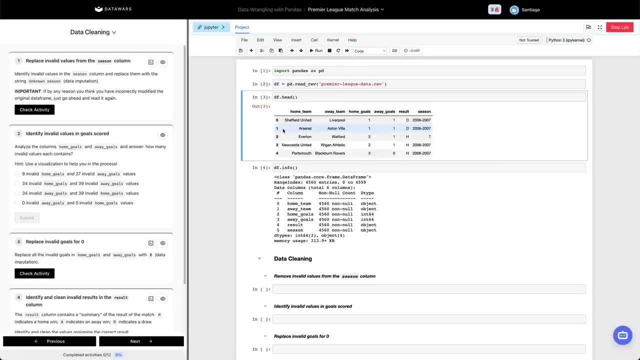 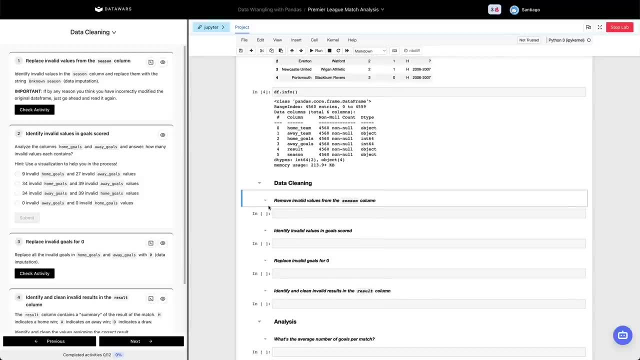 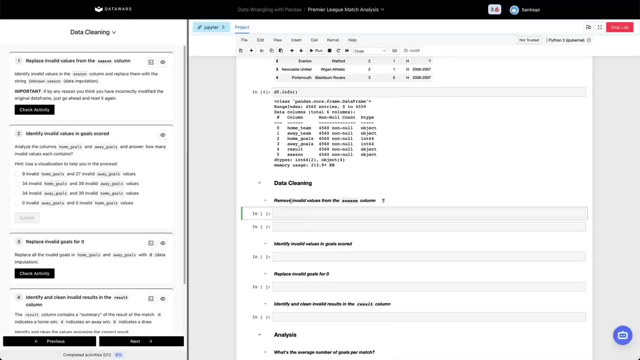 you want to resolve them by yourself. um pause, resume. pause resume as you see me perform the the different activities and you can borrow some ideas from my solution. so let's get started. replace invalid values from the seasons column. and before we can replace invalid values we have. 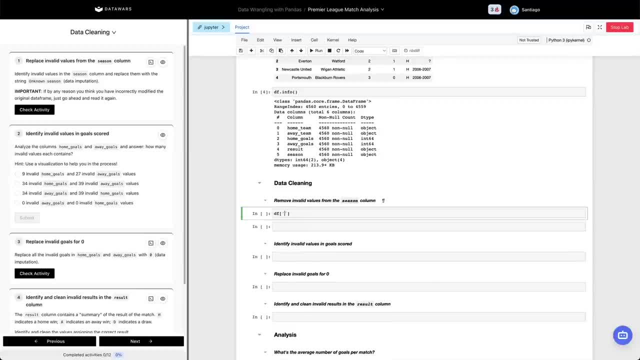 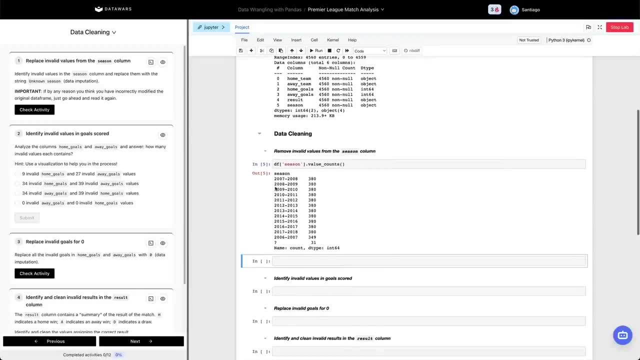 to identify the invalid values. to do so, we're gonna. we're gonna take a look at the seasons. we're gonna do here: value counts. there you go, let's see that, um, there are 2007, 8, 2008, 9, 9, 10, etc. but then we have this question mark here. so this is one of one of the 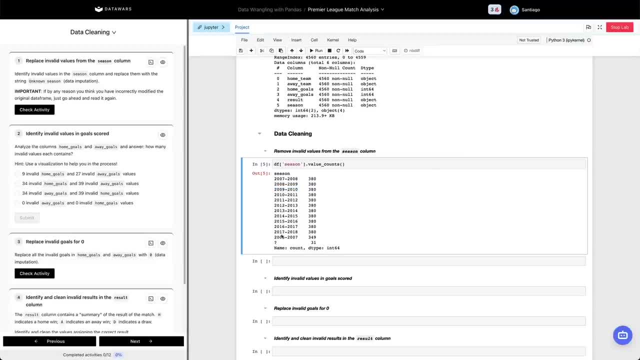 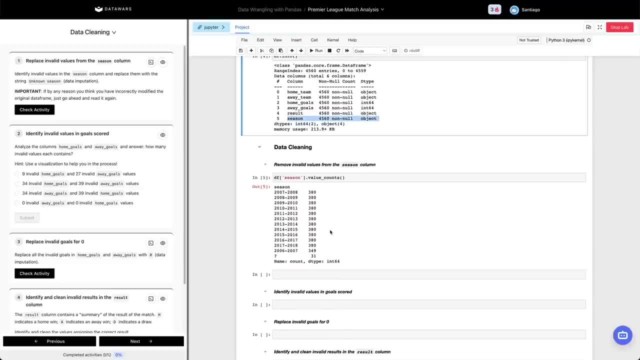 first examples of an invalid value in a column. in this case, um, it's a string column of here string column and the invalid value comes because this is a question mark and of course it's not within the format of the question mark. so we're gonna do: here, value counts. there you go, let's see that. 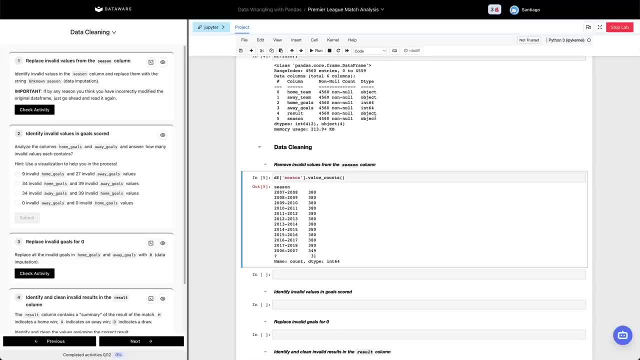 of the season. there is no enforcing in these strings, they're just strings. but we can see very clearly that there is a clear pattern, a format that is an integer, dash an integer, and of course the question mark doesn't match that. so we have to claim those values and replace them. 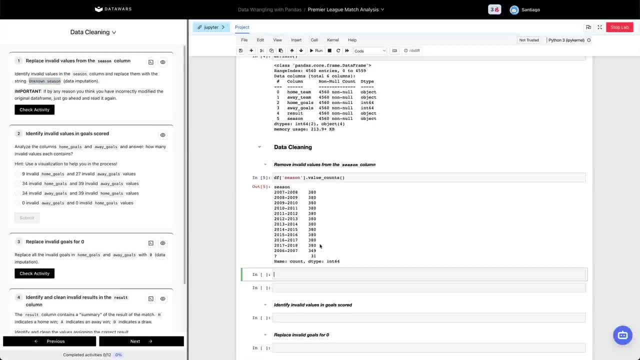 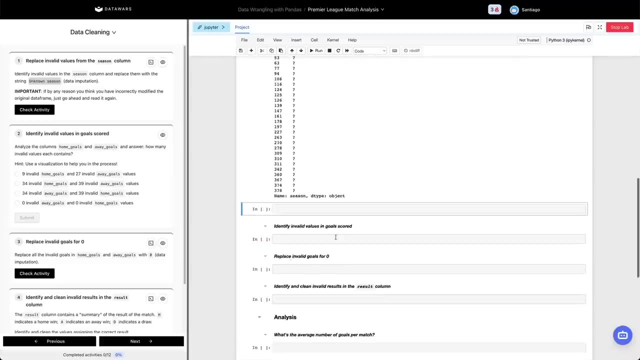 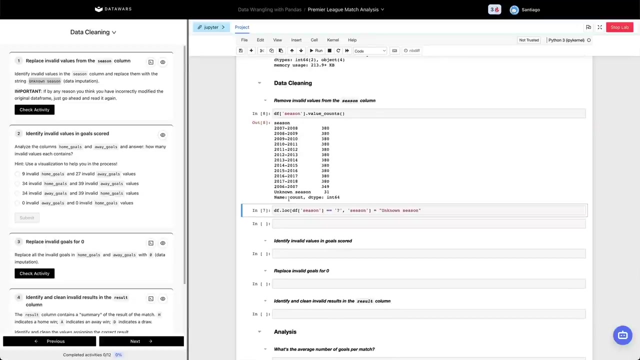 with the value unknown season to do that. what we're gonna do is df dot block, pause. now, if you want, uh, df at um season equals question, mark the season value. there you go all these values. we're gonna replace them with unknown season, and now they should be removed. let's check the activity to see if it works. 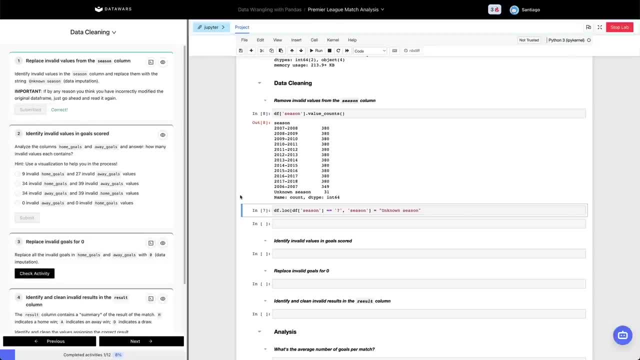 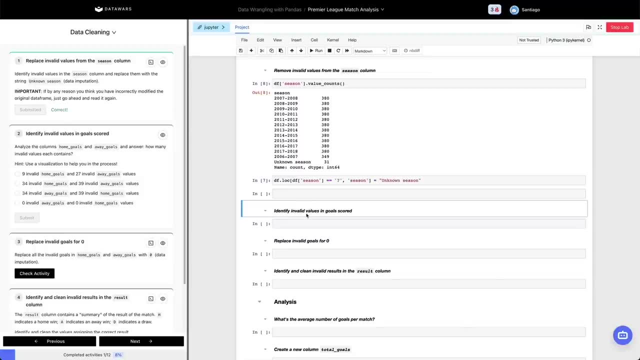 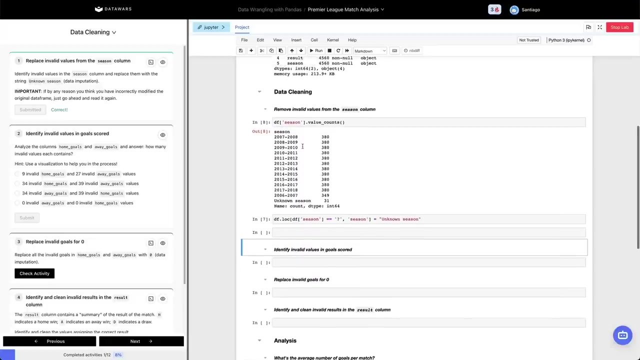 it works so we can keep moving forward. identify invalid values in goal score: this is a pretty interesting one as well because it deals with a little bit of data cleaning, but conceptually speaking, the the data cleaning process- like the decision tree that i'm running in my mind- is different because to identify invalid values in goals, i'm gonna take a look first again. 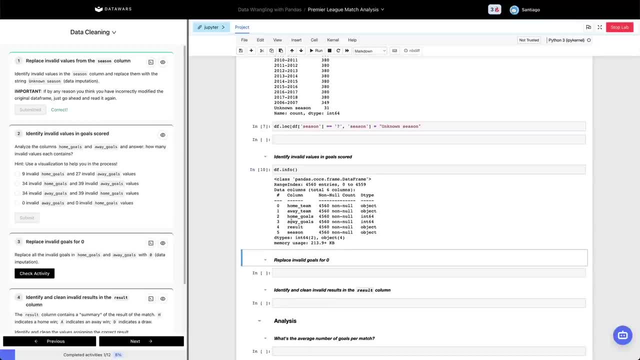 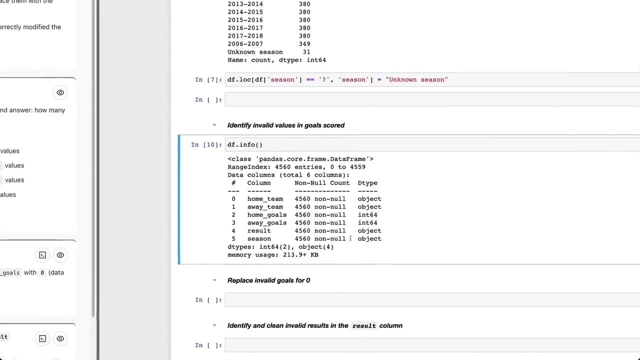 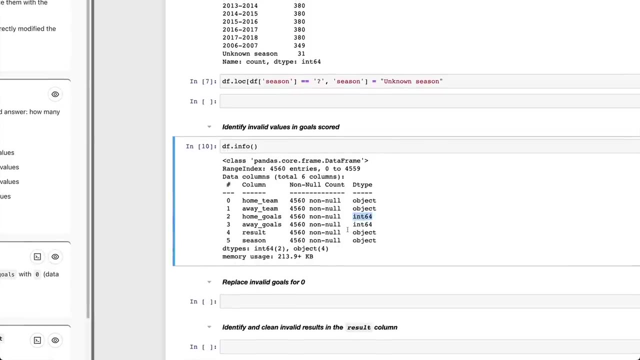 at the info method and you're gonna see that both home goals and away goals are integer numbers. so that is. that is correct. those are supposed to be integers. so how could we have an invalid value here? it would be different if, for example, we see an object here, because that means that 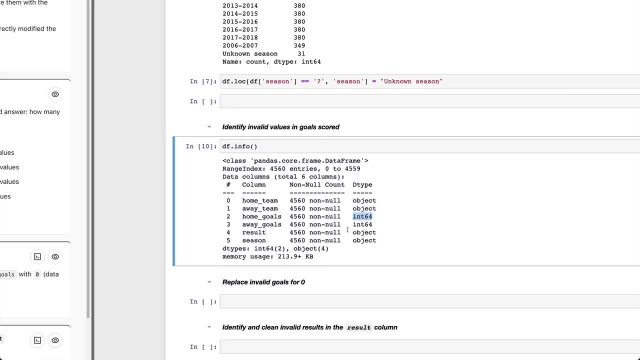 pint has found something. it cannot be parsed as an integer, so it turns it into a string, right, um? but in this case they're all integers and that's pretty much valid. now what we're gonna find is, given that the we have identified the value type, which is an integer, and the column, 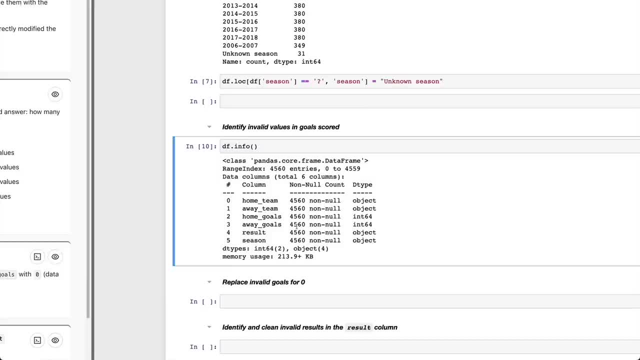 itself is an integer. what is the next column? that is called the tag and that's what the Flickr code does in일. What is the next process? What is the next decision we have to make? Well, if the data, if the range of potential values is met right. So there are a few other projects deal with some other things, But, for example, we have rainfall. you know, that's something that can take a given value. 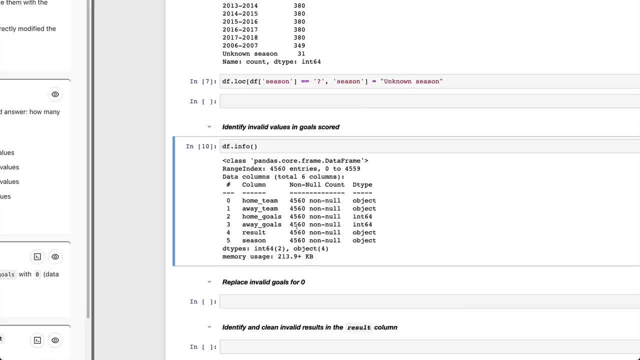 We have, for example, power, electric power in a house. you know the valid values are going to be between, I don't know, zero and 110,, 115. But there are valid values for everything And we have a range now as a second step to define the validity of that column. 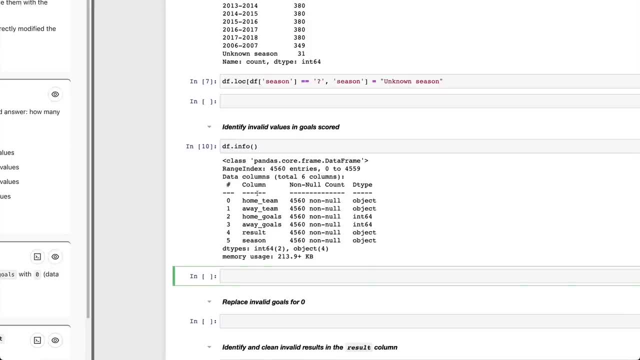 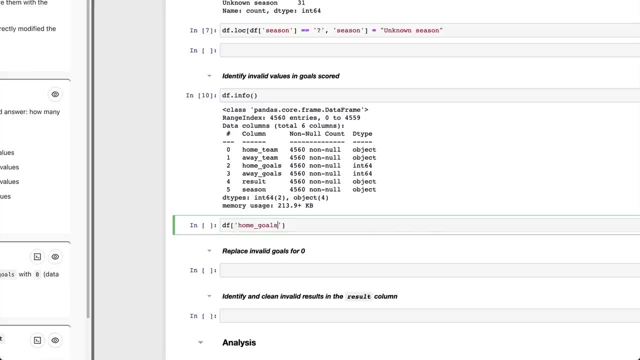 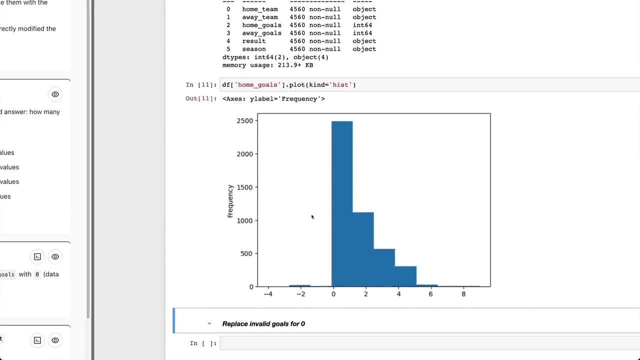 So to do that, what we're going to do is just use a little bit of plotting to aid in the process of identifying these invalid values. We're going to do df at Home, home goals and a plots kind. First we're going to do a histogram And we can quickly see that there are some values that are invalid because they are below zero. And in a football match the minimum value, the minimum goal score, is zero. We don't see anything weird on the right hand side. we don't see any stream goal count If we see something like, for example, 20,, 25,, 30,. 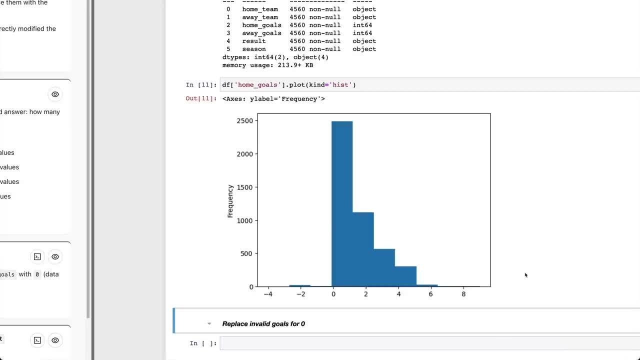 that is a little bit more difficult, because it's valid in terms of a range, But it's an outlier. So is there possibly a Premier League football match in which we're 20 goals scored? I mean, it's possible. It's highly unlikely, And that's the third step when we have to start digging a little bit more, understanding the value Again. hopefully, or thankfully, in this case that doesn't happen. 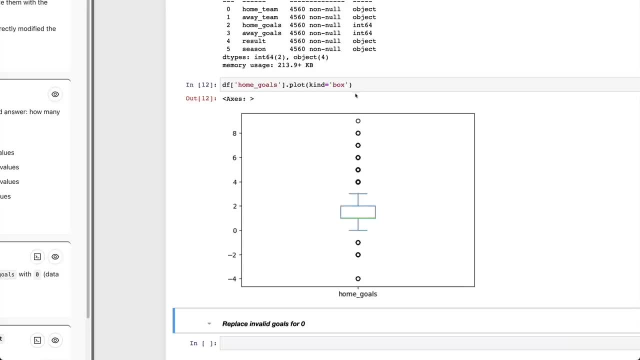 into a box plot So we can visualize it. I'm gonna swap it to be horizontal and do vert falls. There we go And we can see pretty much the same thing. Most of the goals are going to be concentrated here And we have a few samples below zero that are invalid. I'm gonna add a way goals down To visualize, away goes And we can also see like this is the the zero line we can also see here. so the standard zero lines and the 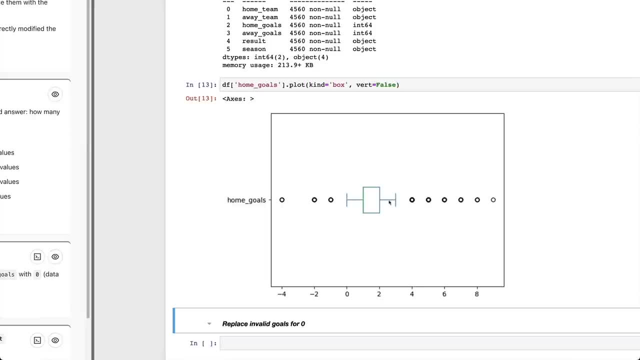 isson values for the side is like the tall one. Okay, so we can see that our information sample is below that theta value we were saying. So if we react to that, then it will100 times incatc, misschien, with lots of. 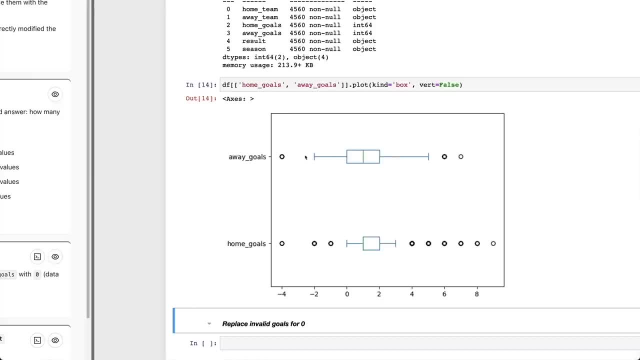 reading, isn't it like? this is the zero line. we can also see that there are a bunch of invalid values right here. Interestingly, the way goals are all shifted to the left. that means that home teams tend to score more goals. 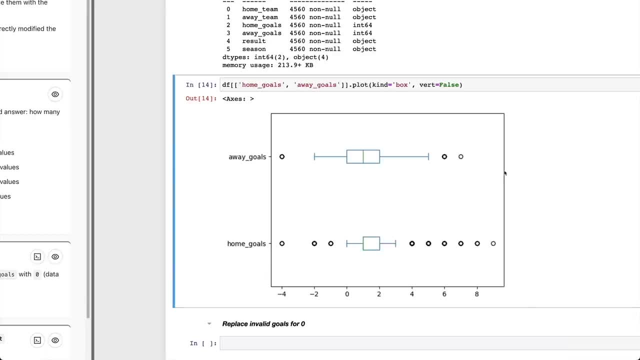 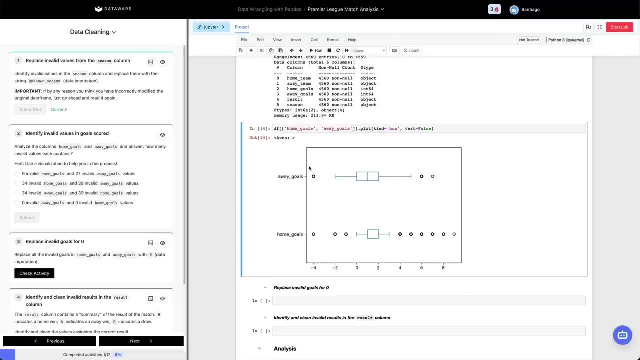 which makes sense if you watch football or soccer. So we have pretty much understood the validity of the column. We know it's an integer, We know that it has a range because we know the sport, And we have identified that there are values that are outside of that range. 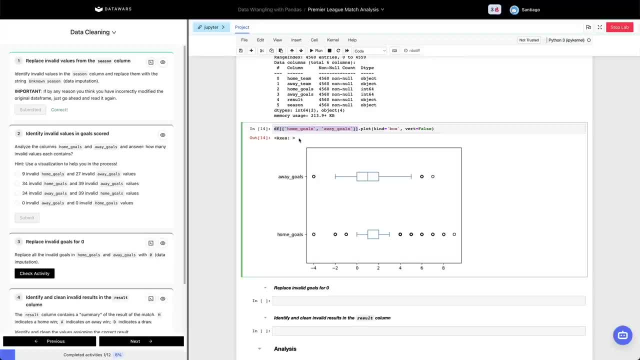 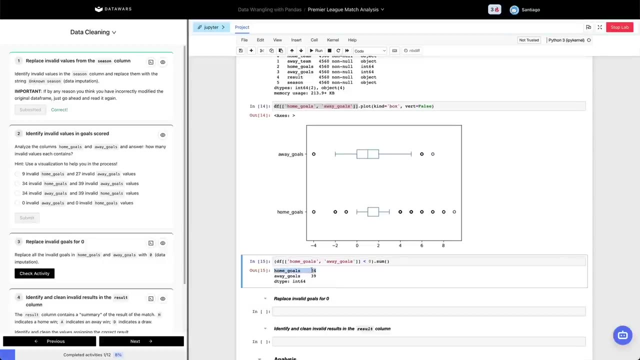 So now we have to take a look at them, And here what we're going to do is we're going to do that are less than zero And we're going to sum that And we have 34 home goals that are invalid and 39 away goals that are invalid. 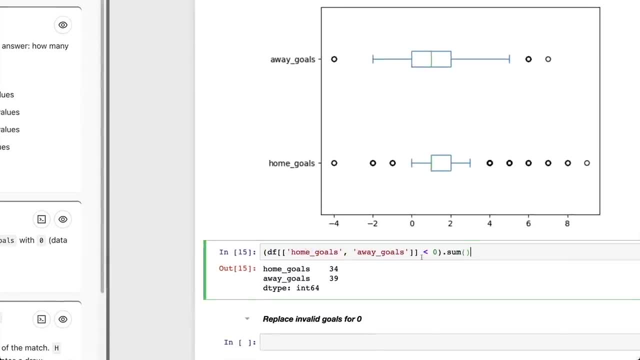 Sometimes people have issues with this sort of thing that I did. If you want to think about it in a different way, we can do something like dflock at home goals is less than zero, Or df at away goals is less than zero. We can take a look here at the different ones. 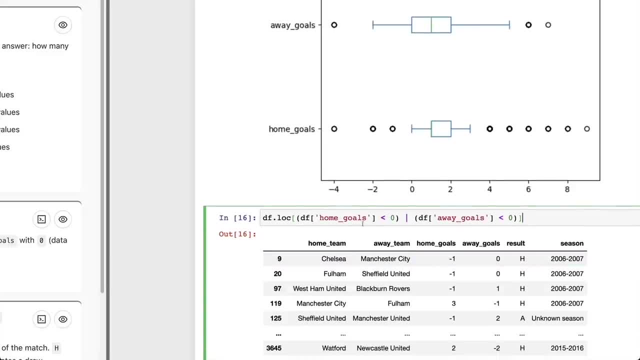 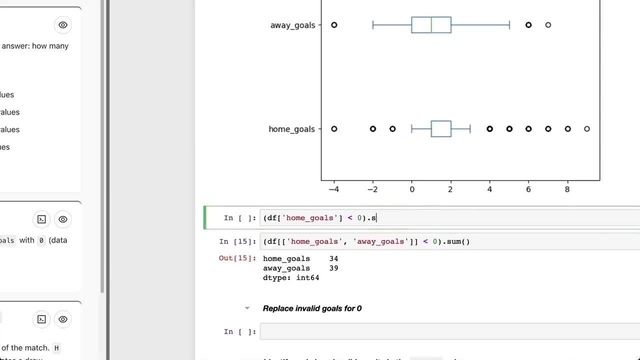 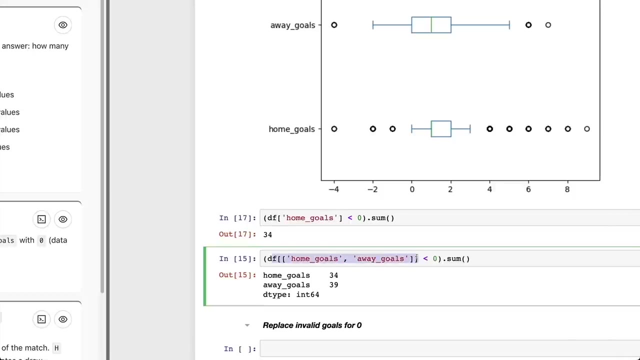 We can start finding how many we have. Or actually we could say something like: it's easier if we do something like shape here or some here, We have only 34.. But the result of this expression is a data frame. We can do pretty much everything altogether. 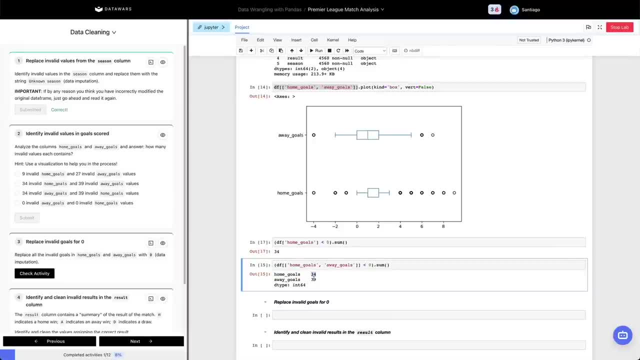 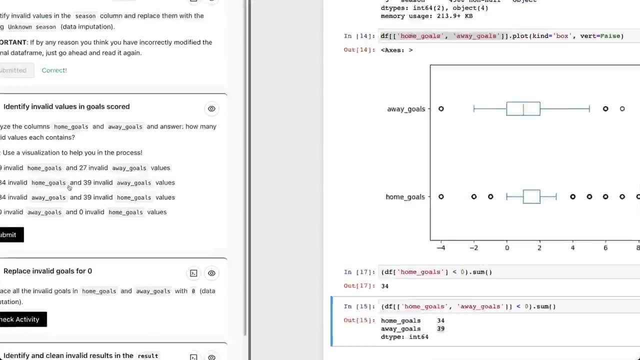 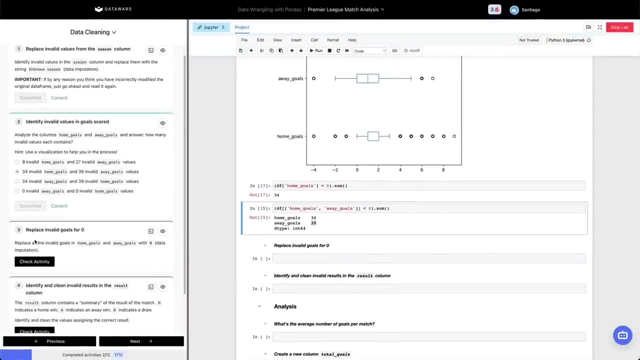 And now to answer home goals: invalid: 34 away 39.. So that's going to be 34 home goals, 39. 39 away goals. And let's check the activity. And it worked. Now moving on with the third activity. 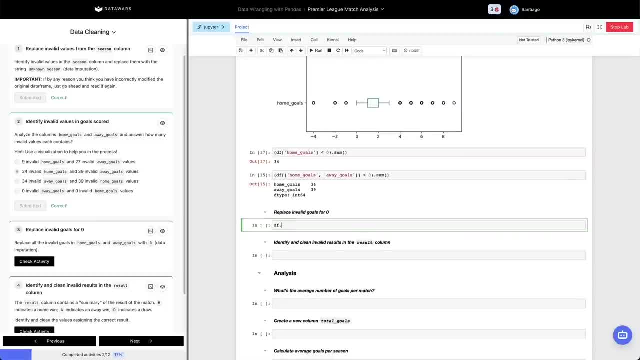 It's pretty much the same thing we did before. We're going to do dflock, df, at home goals that are less than zero. We're going to home goals. We're going to that thing. We're going to replace them all with zeros. 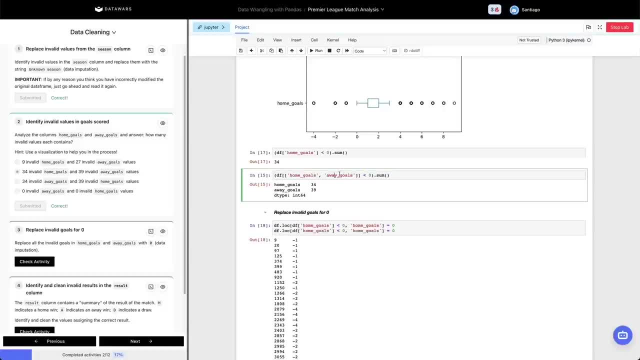 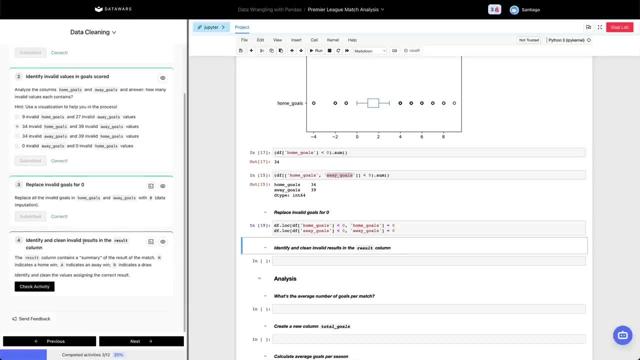 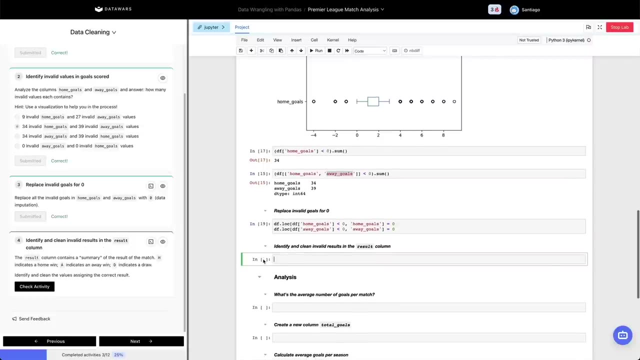 We're going to do the same thing with away goals And we're going to check the activity And it worked. Identifying cleaning value results in the result column And this is a very interesting one because we can keep looking at the different data cleaning scenarios. 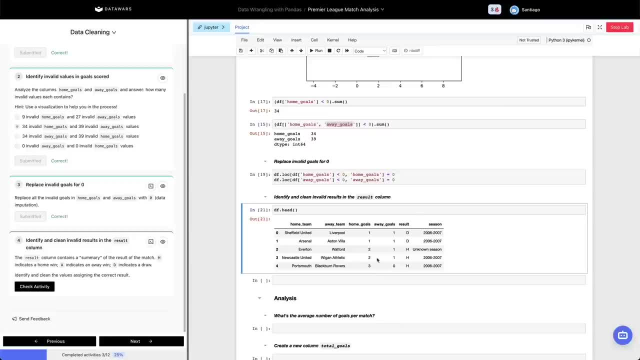 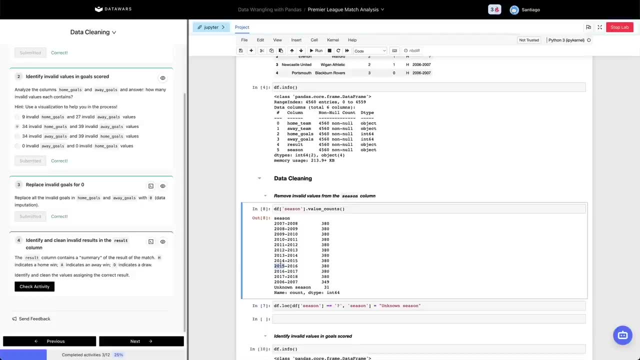 or techniques we have to approach. We had one that we had just simple strings and we had to find a pattern. There is a pattern: Year dash year. This year is the year before this year, right? So there is n dash n plus one, a four-digit integer. 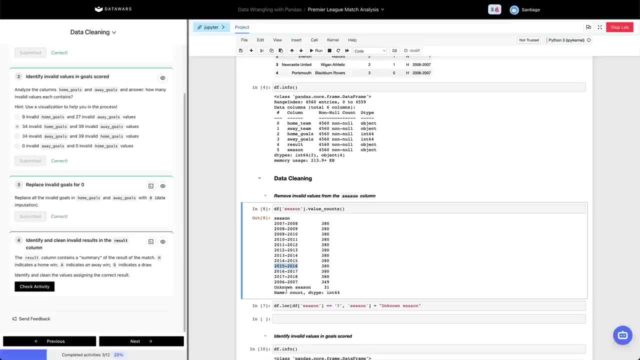 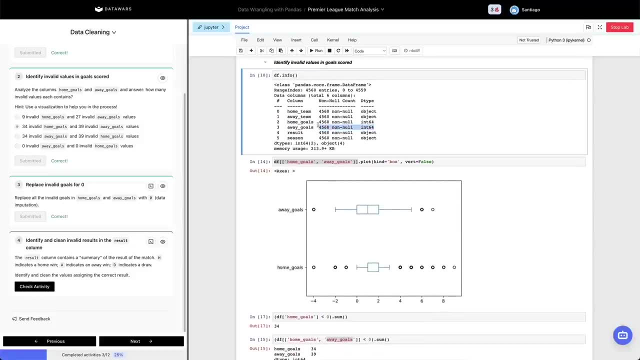 There was a free-form pattern here and there was a pretty clear value. It was invalid, It was a question mark. We then jumped to a integer, which was the correct value type or the correct type of value for goals, But then we had a given range that was available. 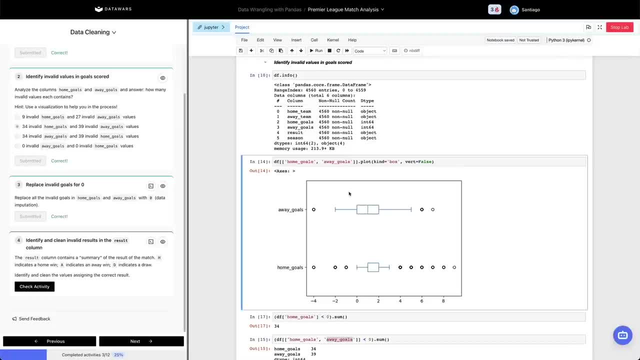 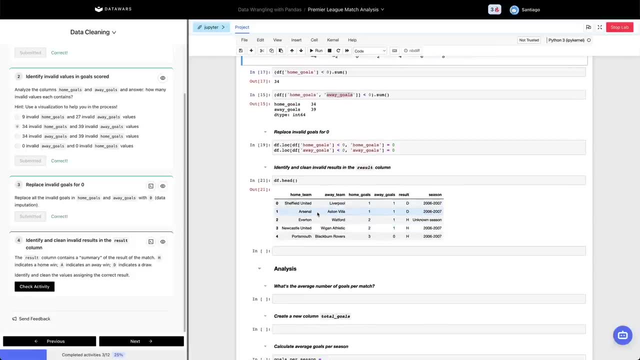 It was valid And, of course, there were values that were outside that range which made it invalid. Finally, we have the one that we're trying to deal with here, which is the result one, And the result column is interesting because what we're going to find value counts. 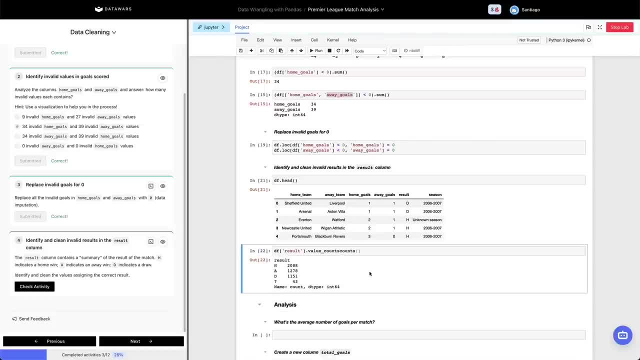 it took a little bit of time. The idea- oh, because you know it's not auto-completed, but the idea is that value counts- is, let's say, a categorical variable. It's not, let's say it's a categorical variable. 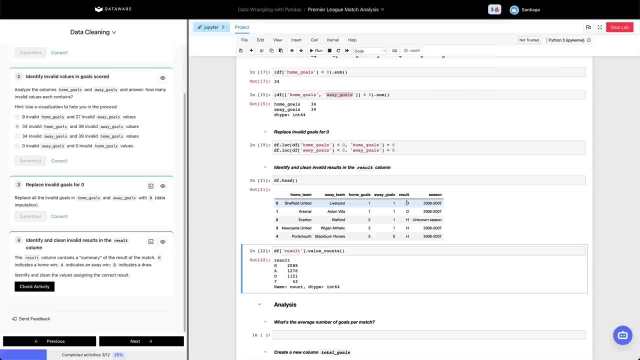 The values that we can take in result are restricted. It's either H for a home victory, A for an away victory and D for a draw, And that's it. Anything outside of that range is considered invalid, And these are usually the simpler to put it in a way. 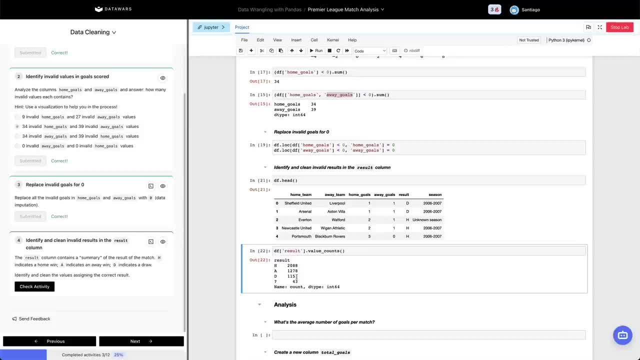 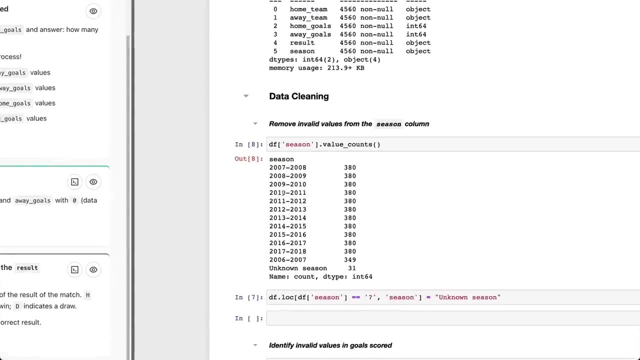 values to not to claim but to identify at least. But we can quickly see if a value is outside of this subset of potential possible values. These are the only three possible values. That is different again from what we saw before with the seasons, because we have to apply a pattern here. 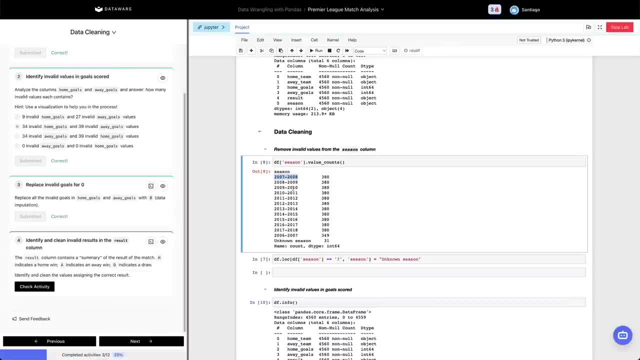 This is just a free-form string. There's a pattern underneath So we can have any value. We can have, you know, 19,, 15, D, 19,, 51, for example, something like that. So that's a little bit more difficult. 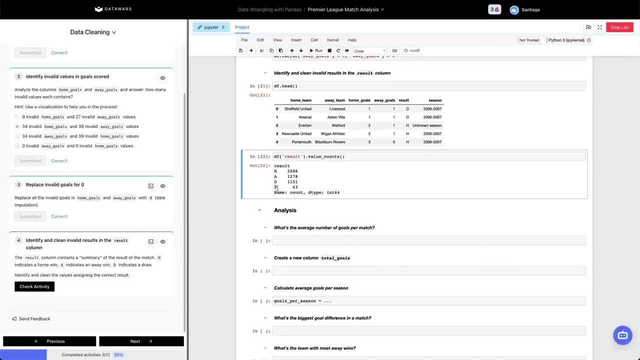 But again, in this case, it's pretty obvious that everything that has a question mark is an invalid result. Now, how can we clean that? Well, we already have the. we can already calculate this result. The result column is a calculated column. 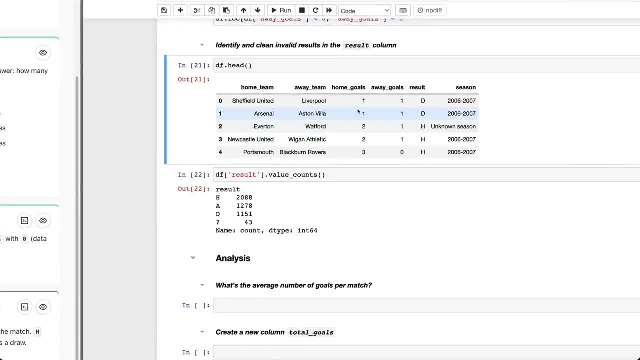 because you can just get that by computing the result yourself. You know, one one is a draw If the value is here, and the value is here and the same if there is a number, an equal number of goals, that's a draw. 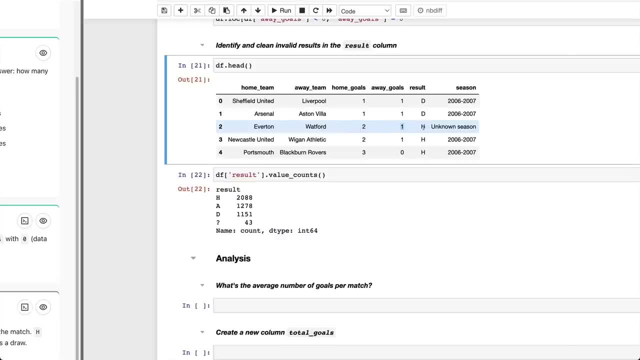 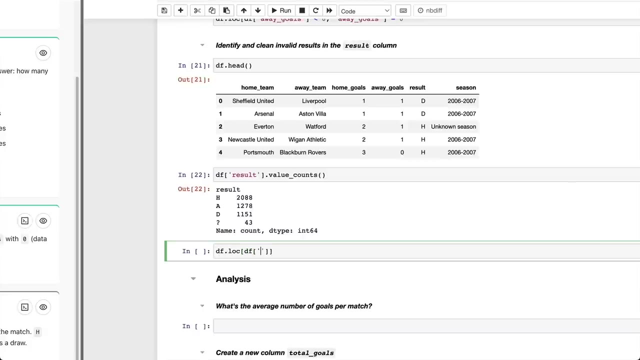 If the home goals are greater than the away goals, that's a home victory, And if the away victory is greater than the home goals, that is going to be an away victory. So how can we fix that? Fairly easy, We can do dflock, df at, for example. 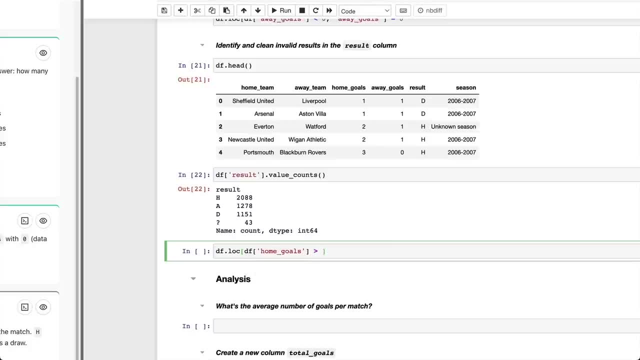 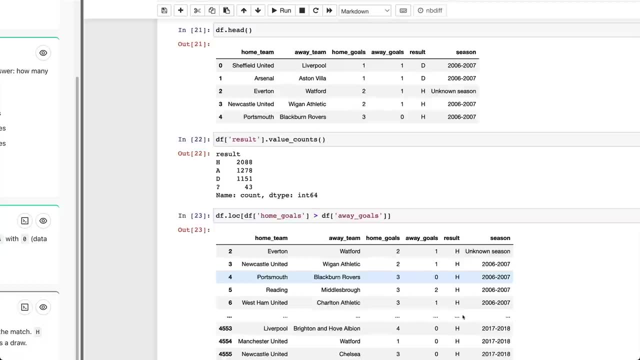 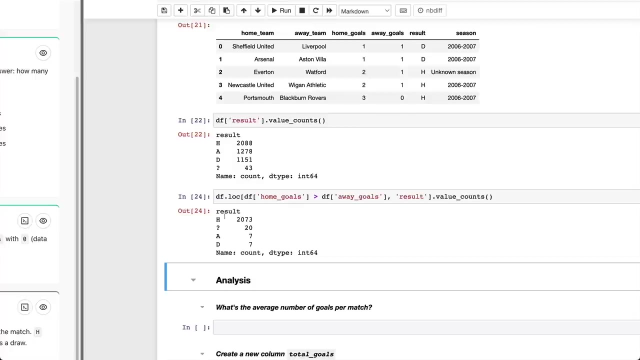 home goals greater than dflock df at away goals. There you go. These should all be. all these results should be. we can do. assault value counts. All these results should be valid, right, So they should all be. sorry an H. 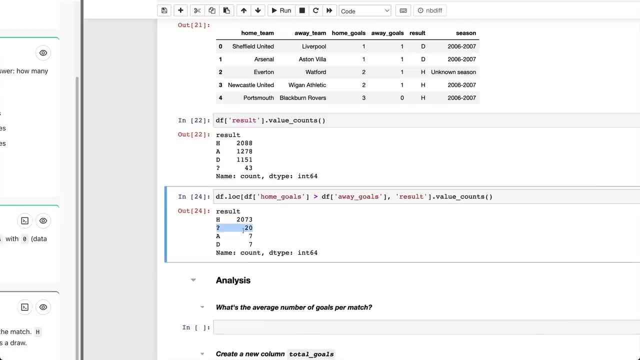 but we not only have this question mark, we also have invalid values, because we can calculate the results. So this is why this is a pretty interesting activity. So now what we can do is just here to like, step over the value, and we know that it's going to be a home victory. 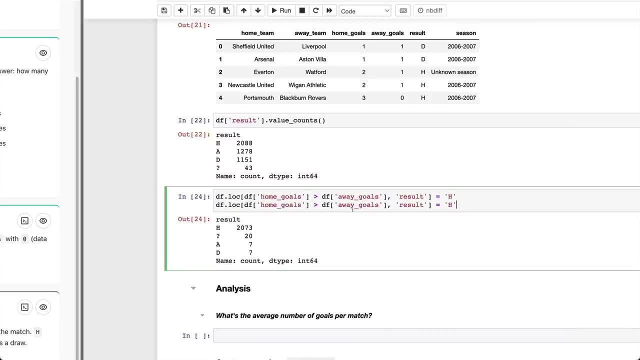 And we can do the same thing for pretty much every other possibility. We can say: if away goals is greater than home goals, that's going to be an away win, And finally, if- let's put here- if home goals is equals to away goals, that's going to be a draw. 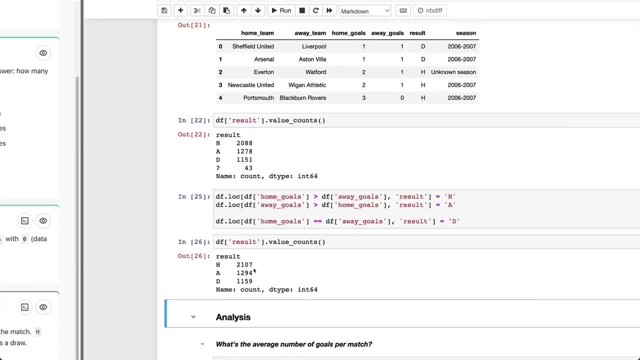 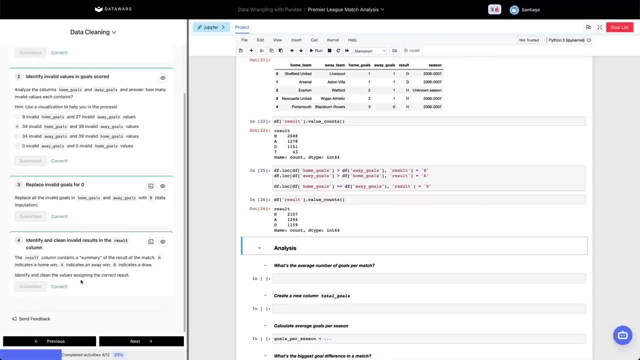 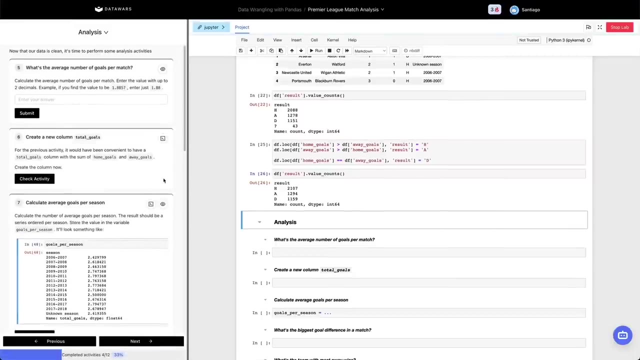 That's pretty much the same thing. Now we can count again and we have the possible values. Let's give it a try and it works as expected, All right. moving on to the analysis piece, This is when we start doing some interesting analysis. 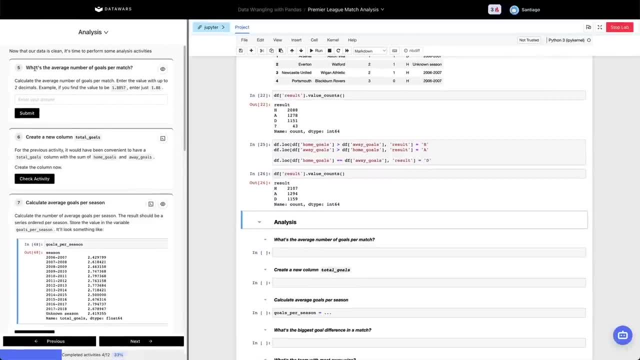 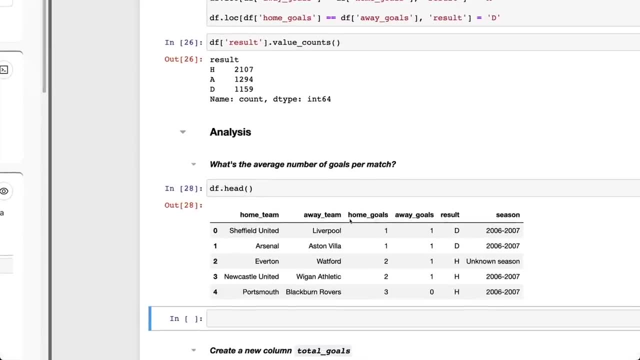 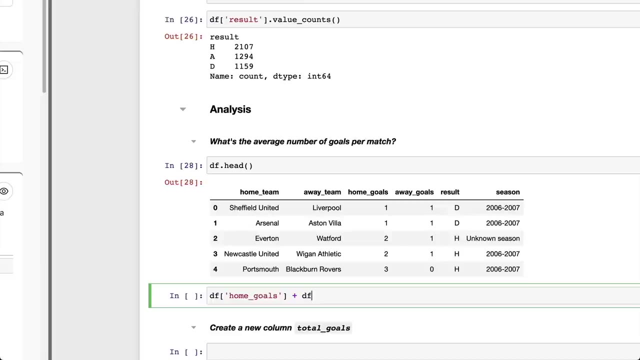 with group, by activities and all that. So what's the average number of goals per match? And we don't have that value. goals per match. We don't have it, but we can easily calculate it on the fly. So home goals, DF, at away goals: we have that. 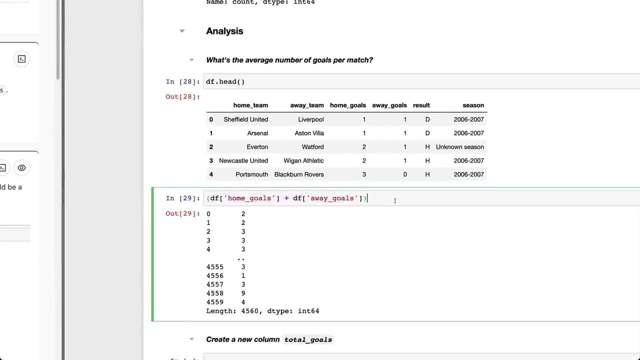 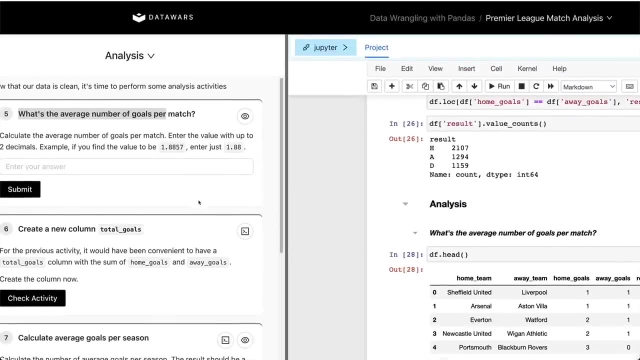 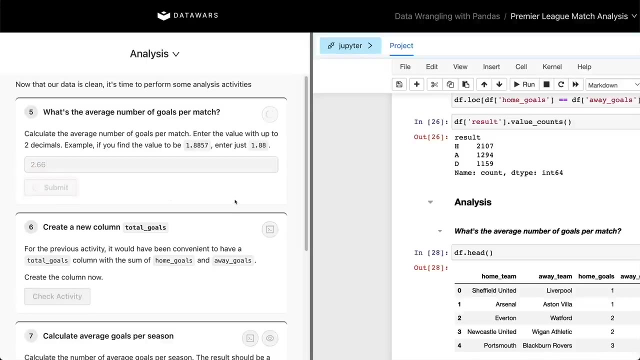 And we can, sorry, zoom out. We can here have the average very quickly And the activity is asking us calculate the average number. I'm put it with two decimals, That's 2.66.. If I'm not mistaking, I'm not saying it 2.66.. 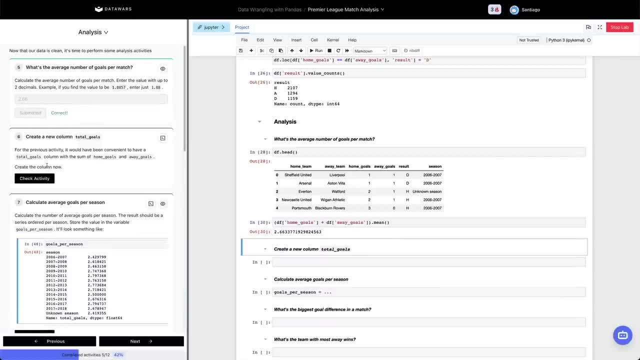 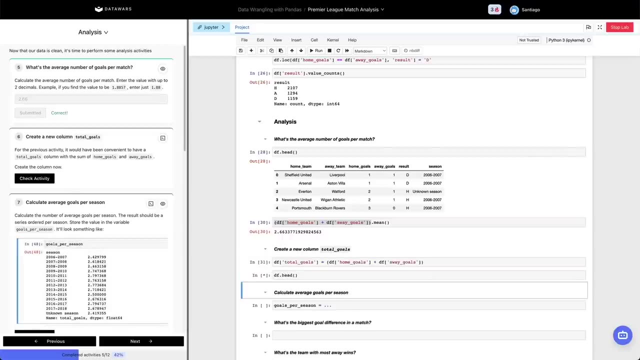 And the activity works. Next one: create a new column- total goals. So now it's pretty much asking us to create a new column, DF at total goals, bypassing this thing And total goals. there we go And we can check the activity real quickly. 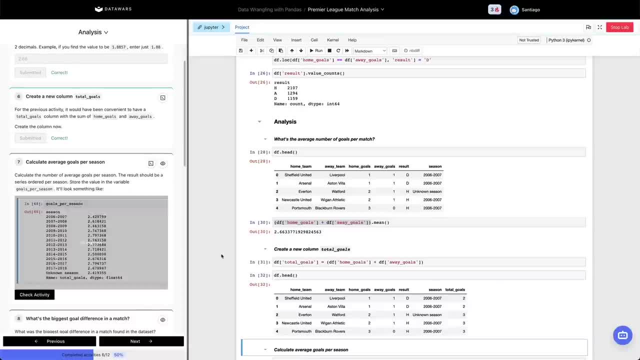 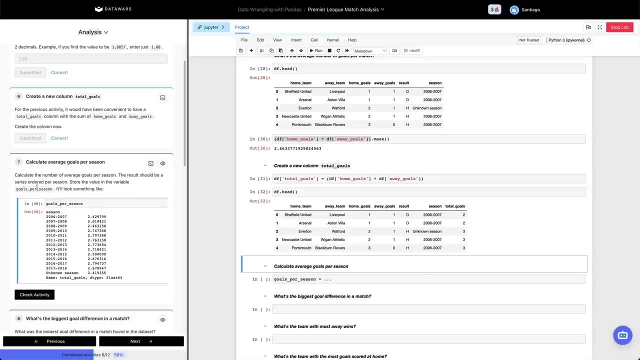 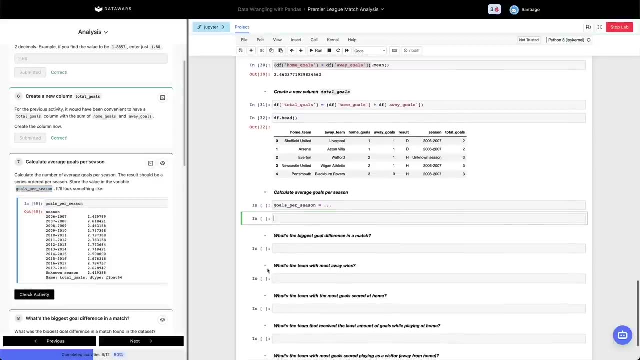 And it passed as expected. Now calculate average goals per season And we have to sort the values by season And we need to sort in the goals per season variable. So the way it's gonna work, it's gonna be. let me zoom in. 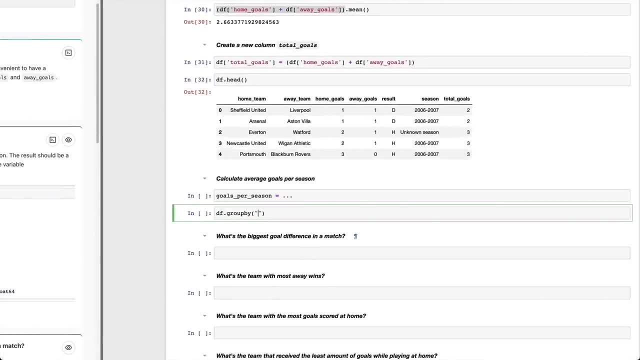 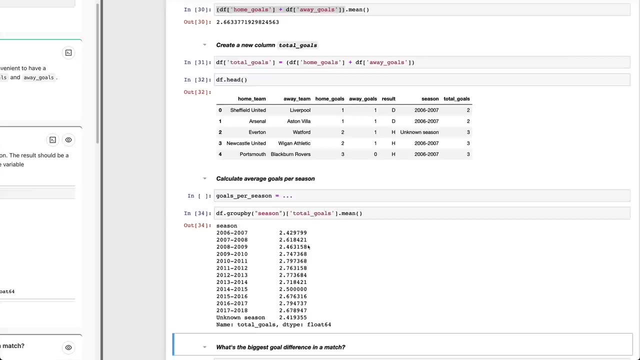 What I do: group by season. And here we're gonna get total goals, We're gonna get the mean. There we go. We need to sort these by the index. That's the season name, So there's gonna be sort index. 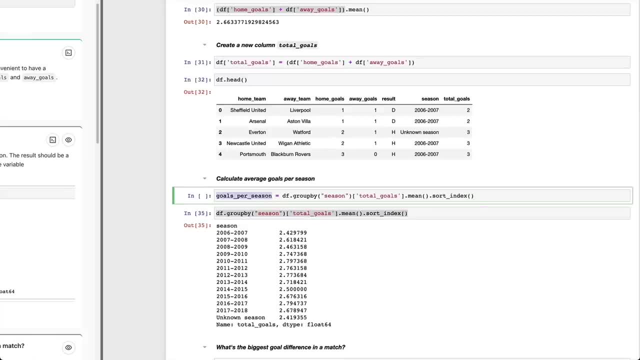 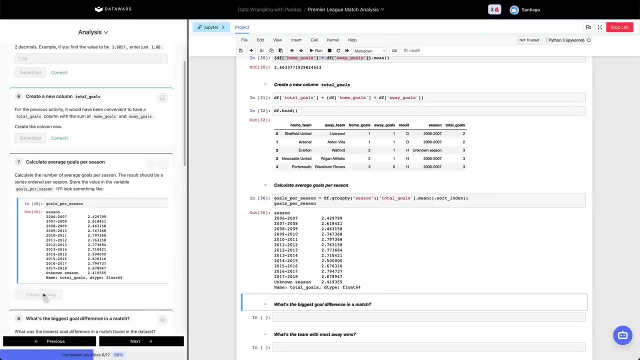 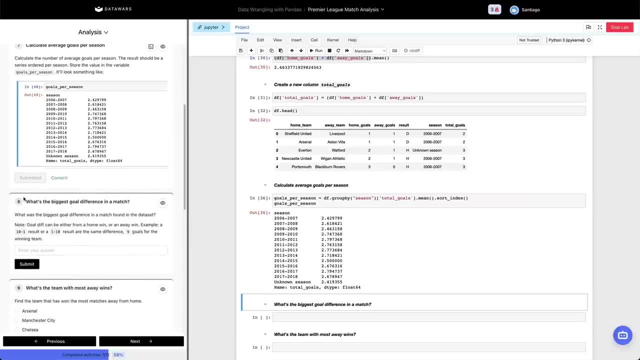 which gives us the same result. just we were lucky enough And we can store that in the goals per season variable. Let's check the activity and see if it passes. There we go, It passed. We are good to keep making progress. What's the biggest goal difference in a match? 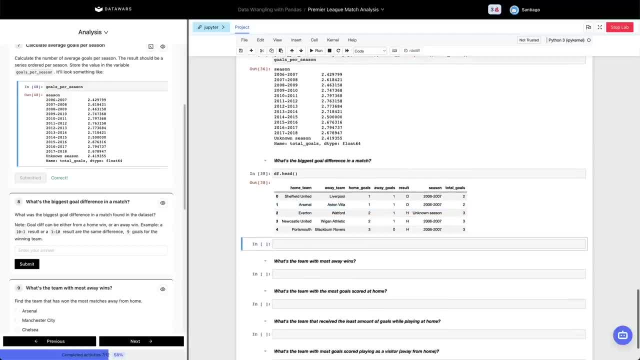 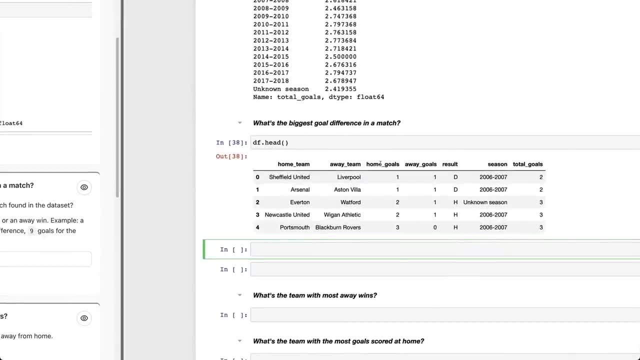 And this is an interesting one as well- Why We have two potential results: when home won or when away won. right, We have a home victory and away victory And we have the difference of those two, So we have something like DF at home goals. 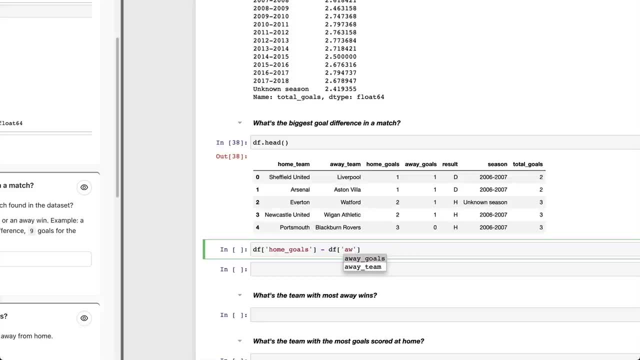 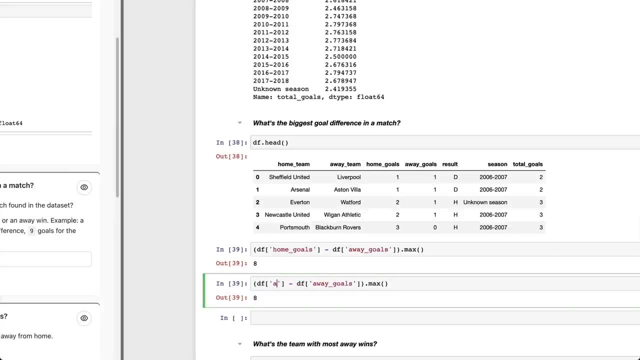 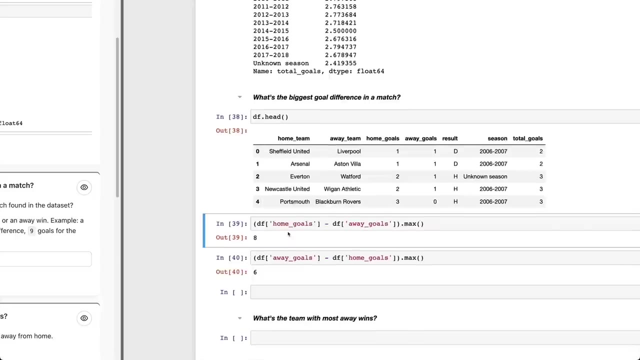 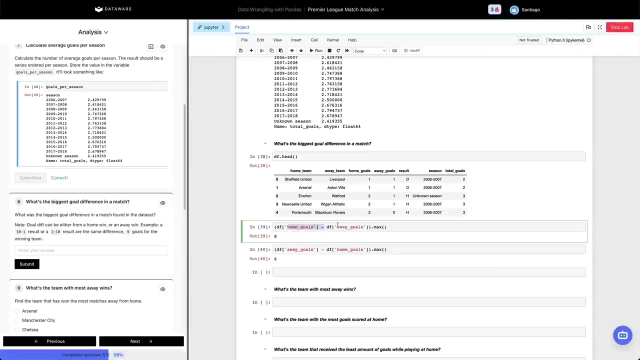 let's say minus DF at away goals, And we can do here something like max. right, We could do the same thing by doing away goals and home goals, And then we have the maximum. So this is the maximum difference in the biggest goal difference for a home win. 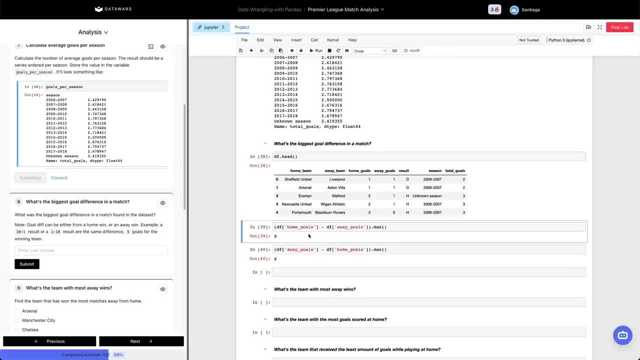 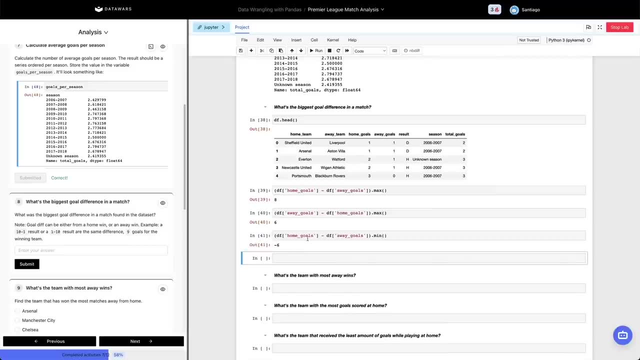 And this is the biggest goal difference- for an away win. We could have used the same value here to do something like max and min, And that's gonna be minus six right, Because in this case it was an away win, the way side won and that gives us a negative result. 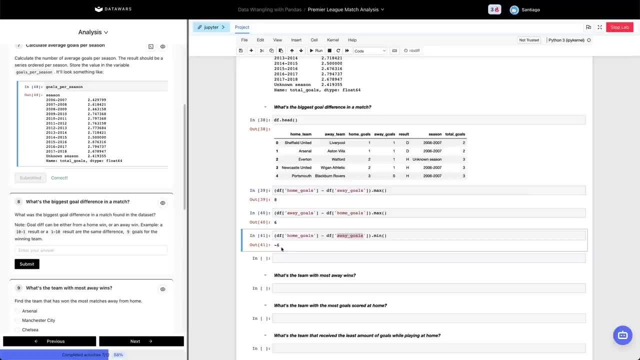 But basically, if I don't care about the symbol, because basically what I care is the magnitude of the value- eight or six, that's a magnitude of the value- Then what I could have done is just do it's something like do absolute. 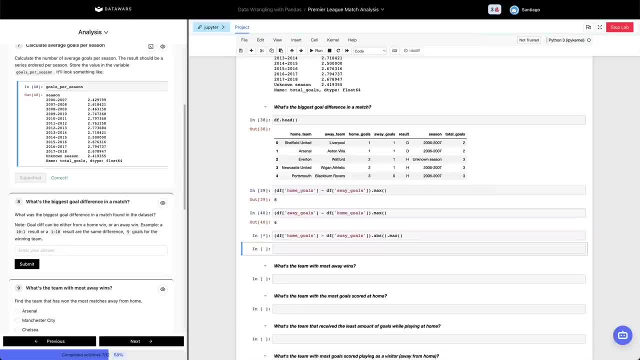 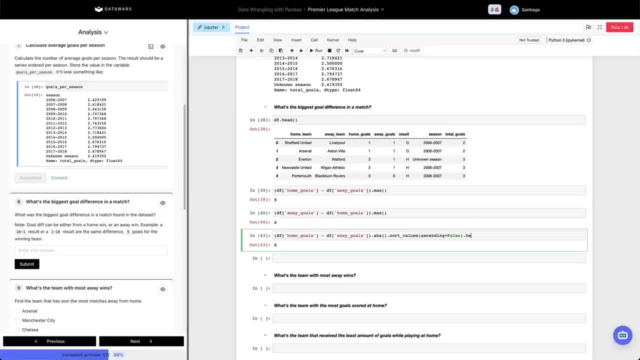 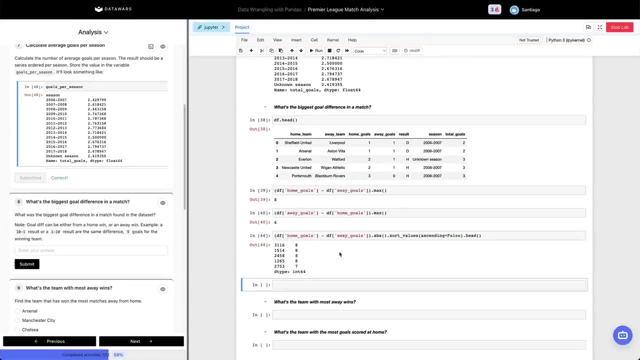 there you go, And now we can get the max value. Or, to put it in a way, we can just do sort values, ascending false head. we can get the results here. So anyway, we arrived to the same results using different techniques. 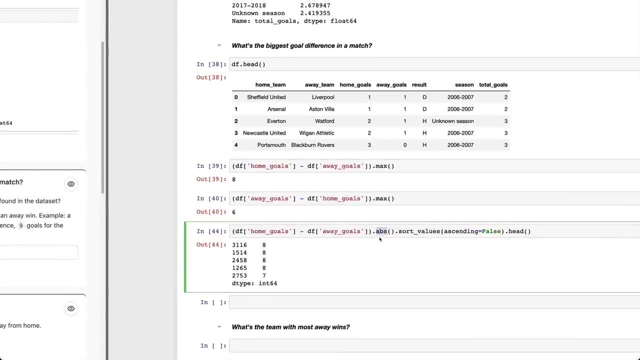 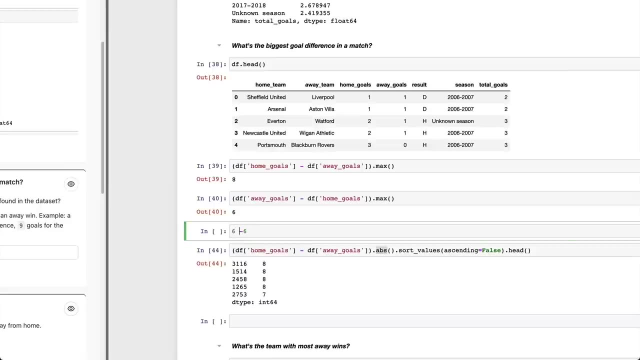 Basically the most interesting piece for me at least here, is for you understanding the absolute method, Because again, it's six or minus six. in this case, it's the same for us because we care about the magnitude, the goal difference. 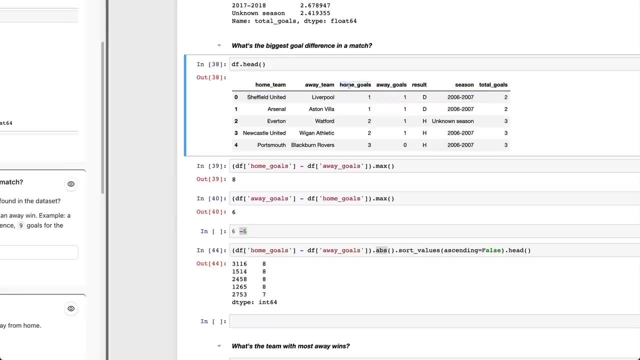 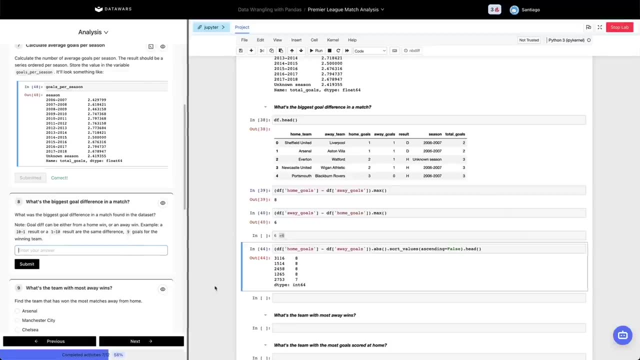 We don't care if it was the way team that won or the home team that won, right. So the absolute method will give us that magnitude. Let's try with eight. anyways, It was pretty obvious that it was a home win If you know a little bit about football, soccer. 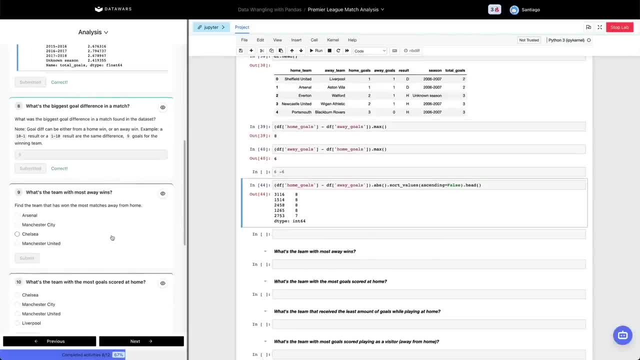 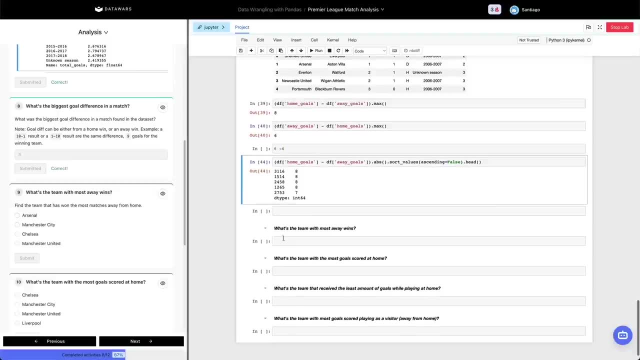 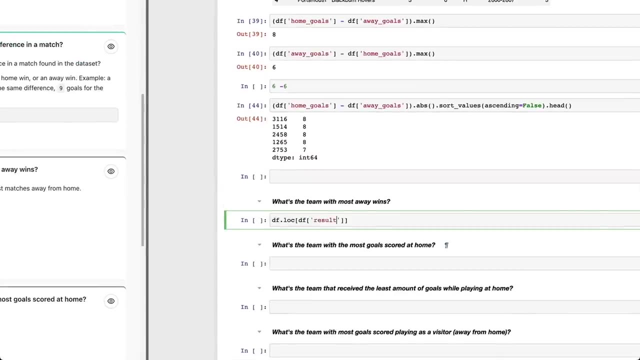 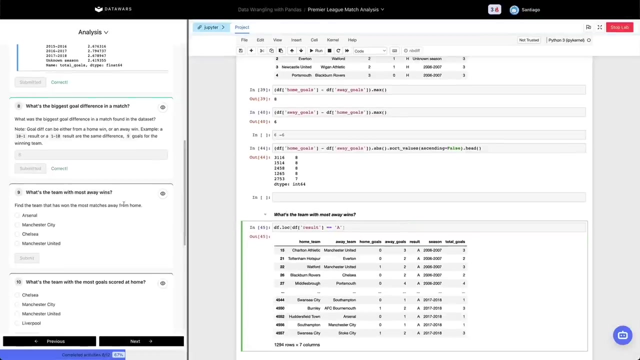 those are case. Okay, moving forward, What's the team with most away wins, Away wins- And this is a very interesting one as well- Why We could start doing something like dflog. dfresult is away. right, We have all the away team away victories. 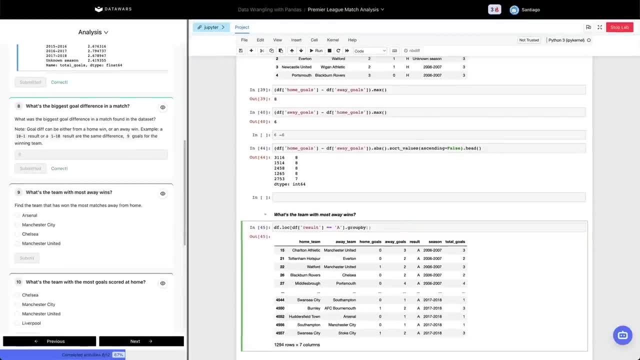 Now we can group by the away team, because basically what it's asking us? what's the team with the most away win? So this is an away win. Who was the team? It's basically away team And now we can just add: resultsize. 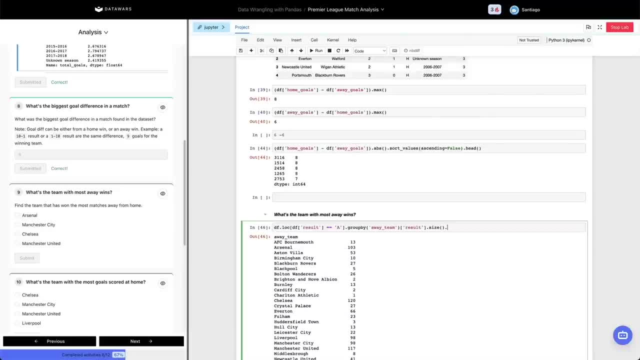 and we can get, oh, we can sort values by nothing, because this is a series ascending false. And let's do just head. And we have that. the team with the most away wins is Chelsea. Let's give it a try first. 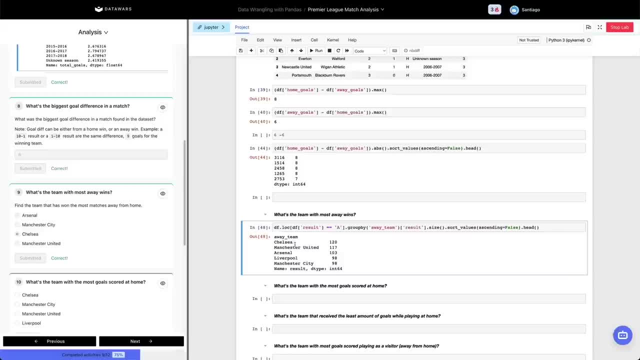 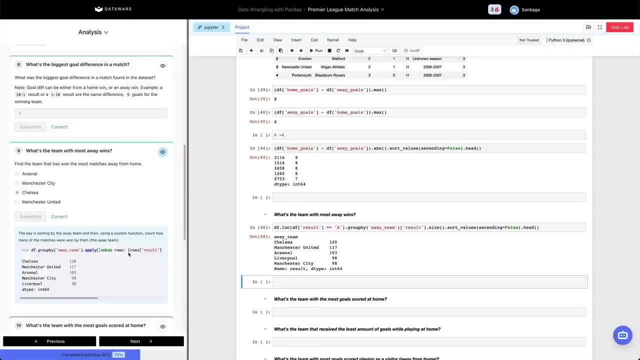 And then I'm going to show you something different, a different way to calculate this thing. There you go, work. There's a different way, And it's actually the solution proposed here, So I'm just going to go ahead and reveal it. 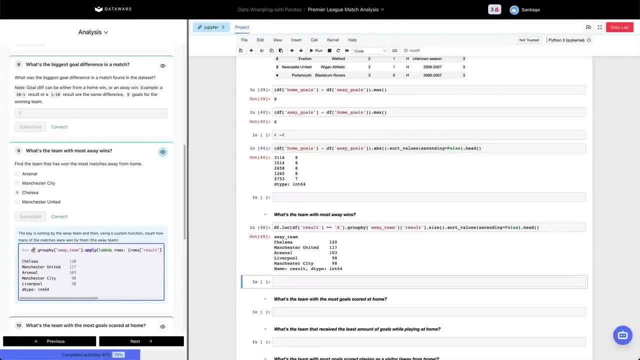 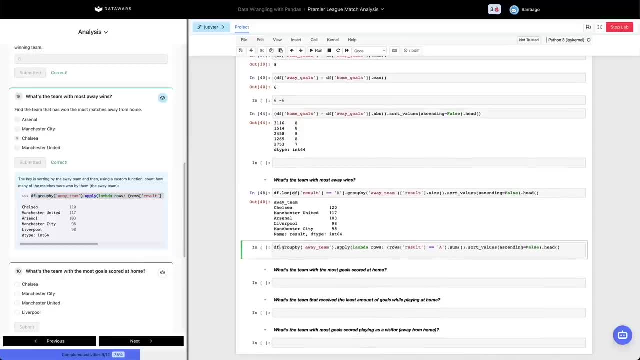 And we can. I can just copy and paste these things- We don't waste so much time- And I can explain it to you right here. Basically, what is happening here is we can group, by the way team, And when we do this grouping, we're going to have 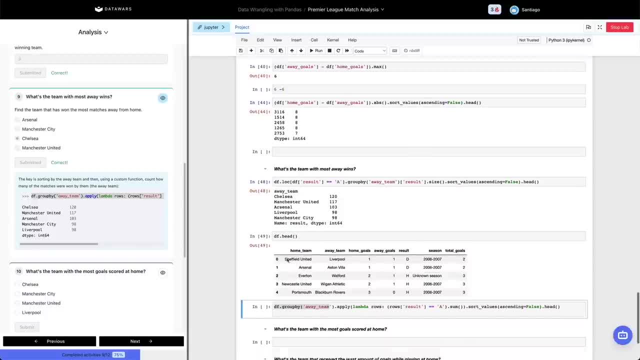 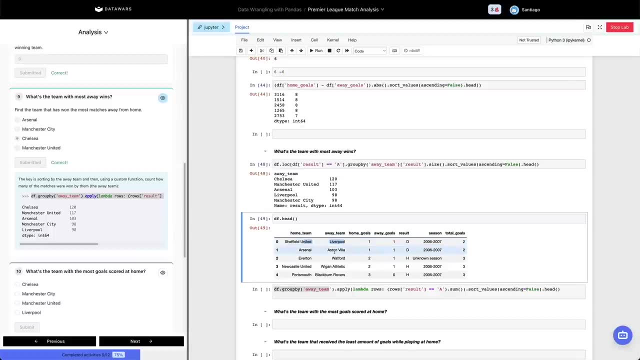 the head. we're going to have all the results for an away team. So for Liverpool, we're going to have these results and pretty much any other result from Liverpool, And that's going to include draws, home victories and away victories. So, basically, what we want to do is we want to group. 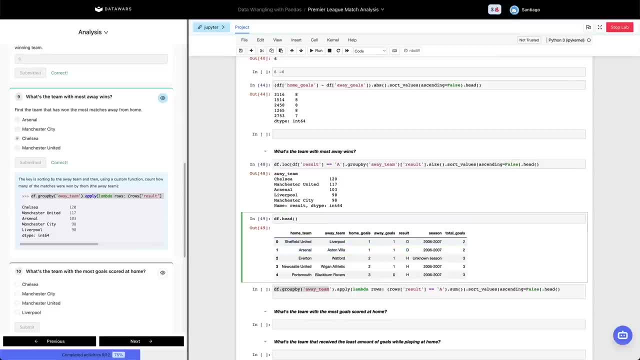 we're going to get this group, that is- let me get here- Lock. if at away team is Liverpool, as they say, There you go. So when we group by away team, we can, we create, we create like we have. so we have this full data frame. 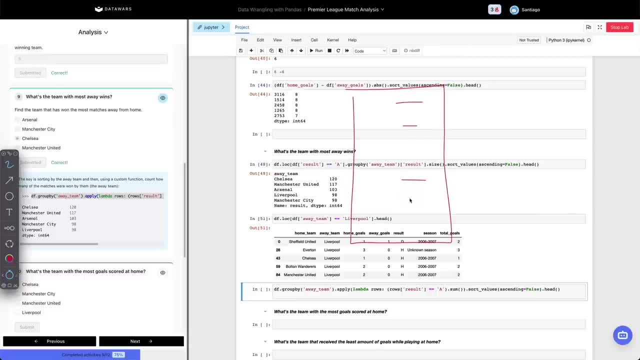 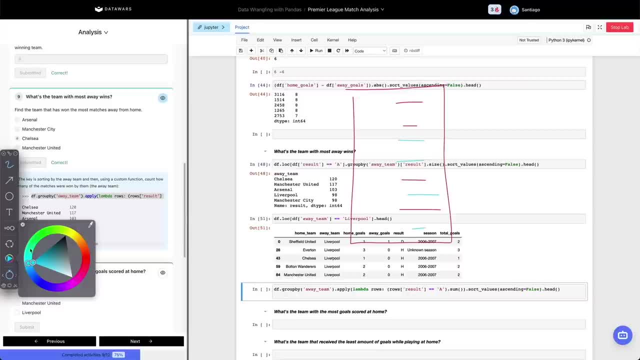 Manchester City, Manchester City, And we can get another football team from the Premier League Can get here. Wolves Wolves is another team. Wolves, Wolves, Wolves Wolves. What the group by operation is going to do is going to identify. 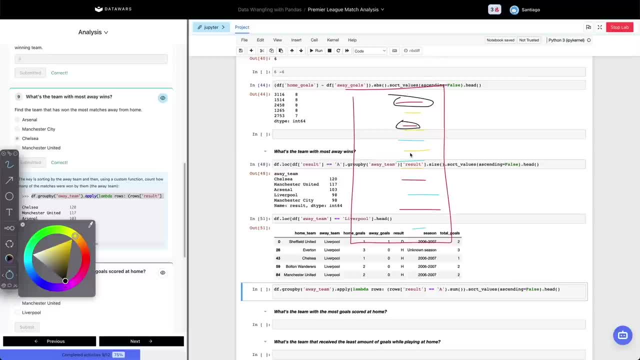 we're going to use black. It's going to identify the values that are the same and it's going to pre-package them right in this. I don't know if you've heard about it, but the term is splits, apply, combine. 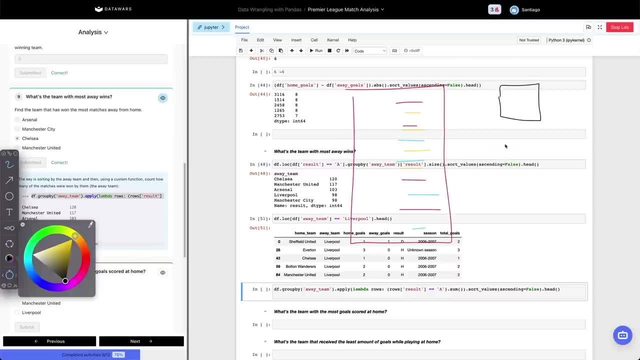 is going to create tiny groups with the different samples that meet their grouping criteria. So it's going to put all the Liverpool, all the Liverpool matches here. it's going to put put all the Manchester City matches here. It's gonna put all the Wolves matches here. 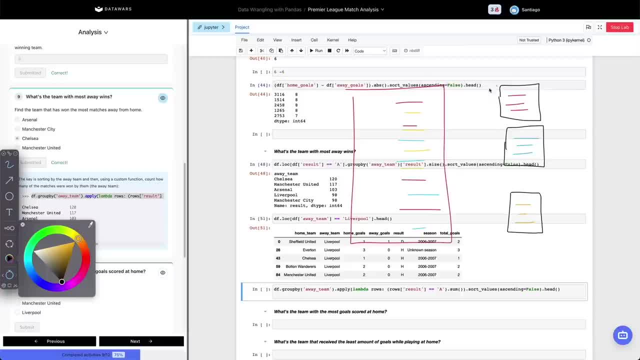 It's gonna give you the option now to work with this thing. So now we can do, for example, now get me the away goals and do a sum, Or give me the results and give me the size. We can do any operation with these subgroups. 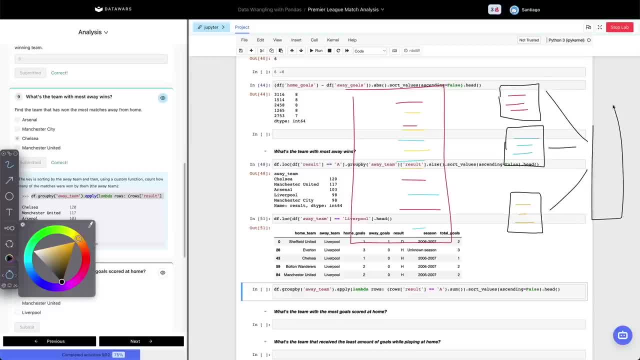 And then it will assemble them again in a table and it's gonna say: Liverpool, whatever, Manchester City whatever, Wolves whatever, or Manchester United whatever. Again, it's gonna combine all these small pieces that it has created. But before we do the operation, 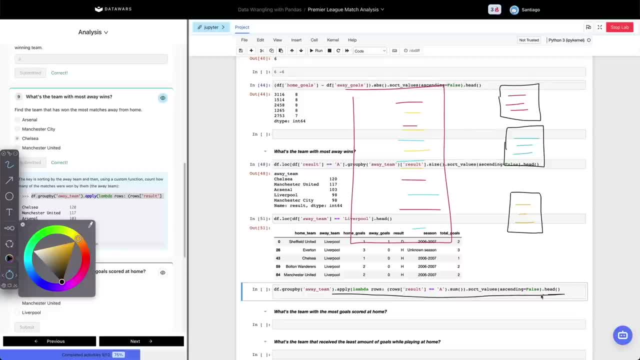 we have the chance to run a custom function and that's the apply one right here, So we can run, we can pass this custom function that is gonna be run in each individual group, And what the custom function does is it gets all the rows. 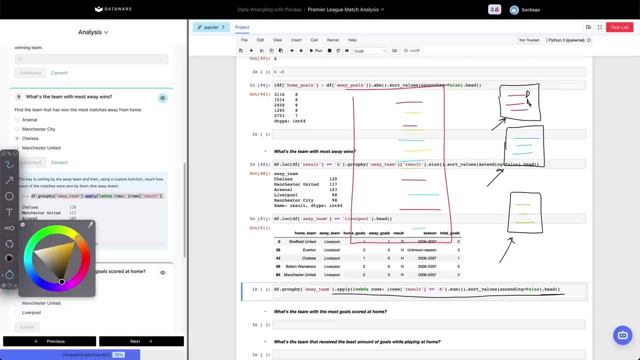 So here it's gonna get a draw, an away win, a home win, an away win, et cetera, And we're gonna perform the operation that we want, which is counting the ones that are an away win. So we're gonna get only the ones that are an away win. 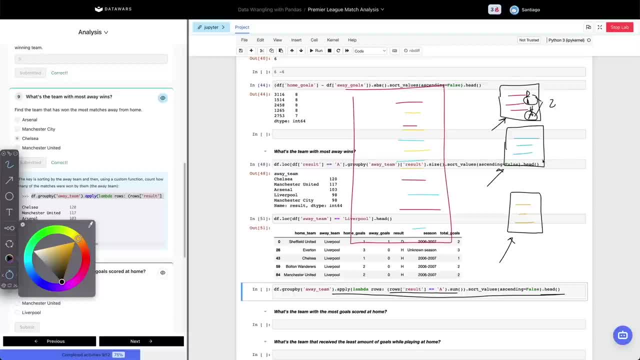 We're gonna do a sum and we're gonna return that value. So here's gonna be two and here's gonna be, for example, just one, And here's gonna be- I don't know- zero. We're gonna get just one. 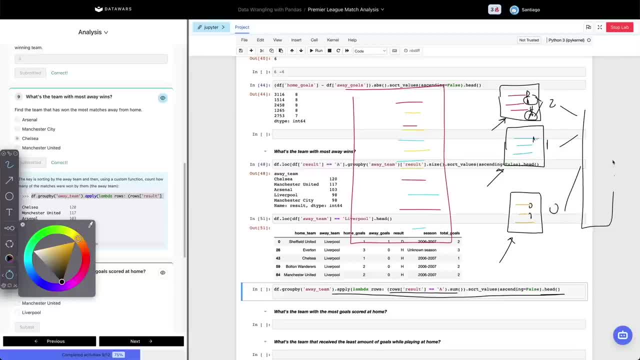 Finally, Pandas by itself just takes care of saying Liverpool two, Manchester City one and Wolves. that's too many Wolves. zero, right The combination at the end. And that's the way that function works. Let's clear this whole thing, unrun it. 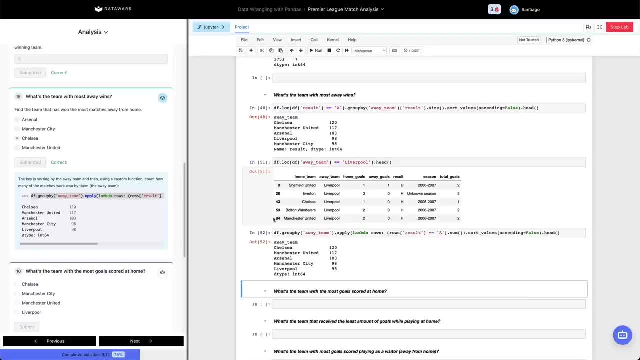 And we get pretty much the same results as before: Chelsea, Manchester United, Arsenal, et cetera. So the way to think about it is: you can filter your data before starting, or you can perform these operations after you have grouped the data. 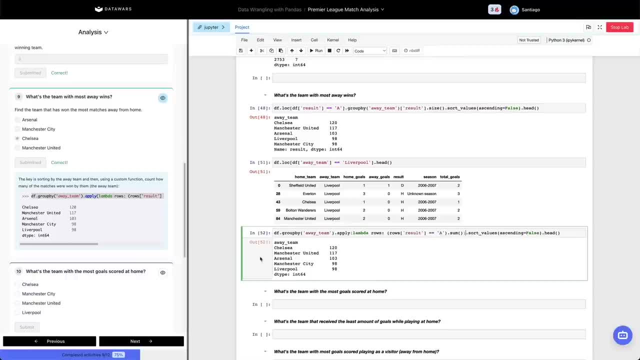 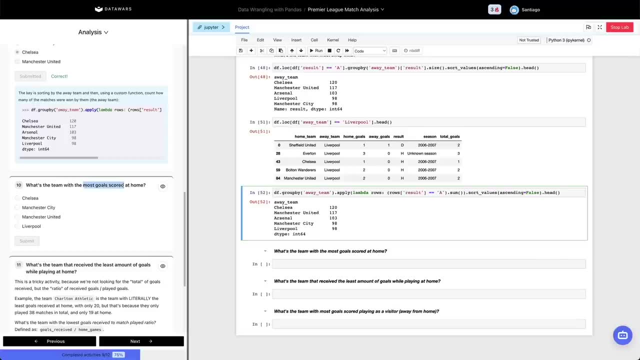 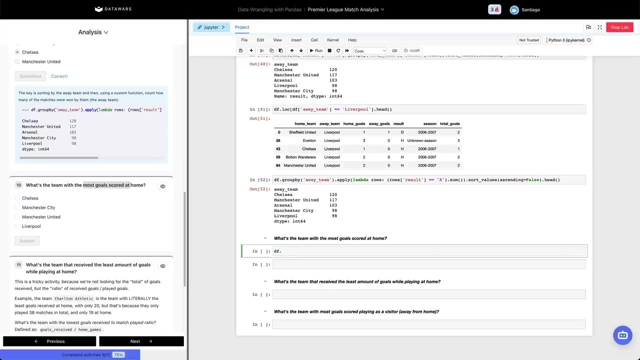 with the individual groups that you had before. Okay, that's it. Let's keep moving forward, because we have just three more activities to go. What's the team with the most goals scored at home? So this is a pretty interesting one as well. 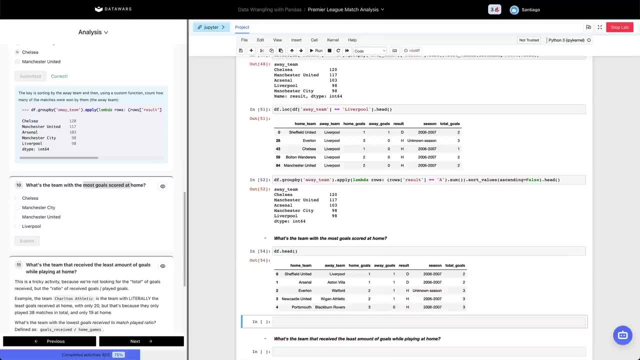 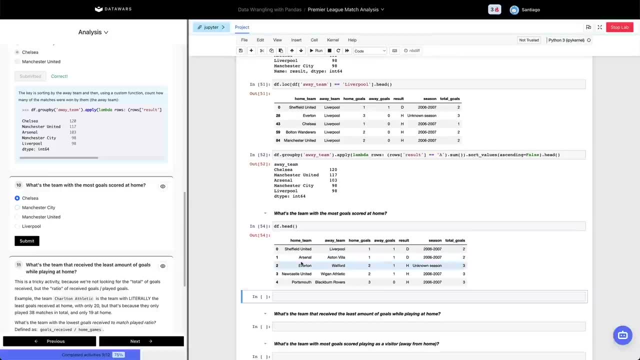 Let me get head. you take the time now to pause the activity and solve it by yourself. I selected Chelsea, I don't know why, just a mistake. But again, take the chance to pause and do it by yourself. Basically, it's asking: 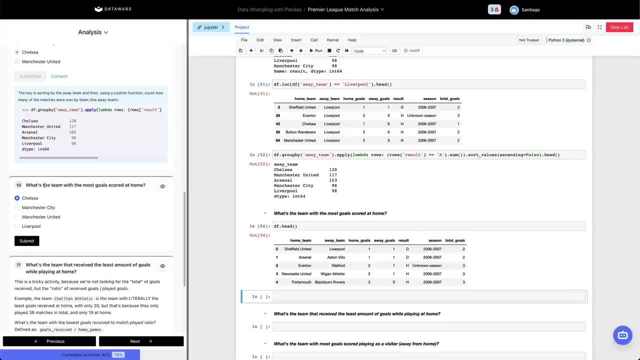 what's the team with the most goals scored at home? So it's basically the home team. We have to group by home team, home team And we have to count these home goals. So here, just count home goals And we need now to get the sum. 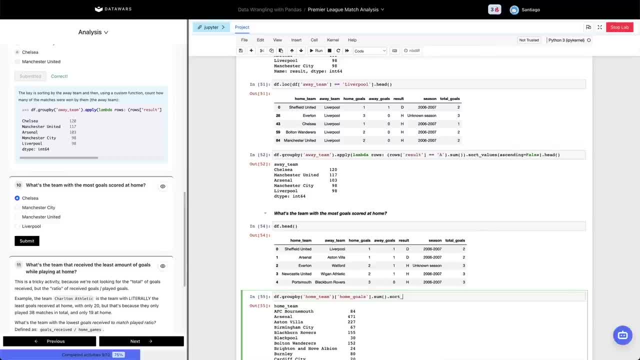 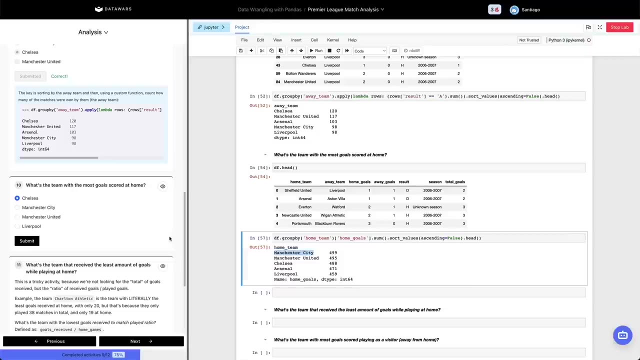 We're gonna get the whole thing, but of course we need to sort values by ascending false And we're gonna get head. There we go And we have that. Manchester City seems to be the goal with most the team- sorry- with the most home goals scored. 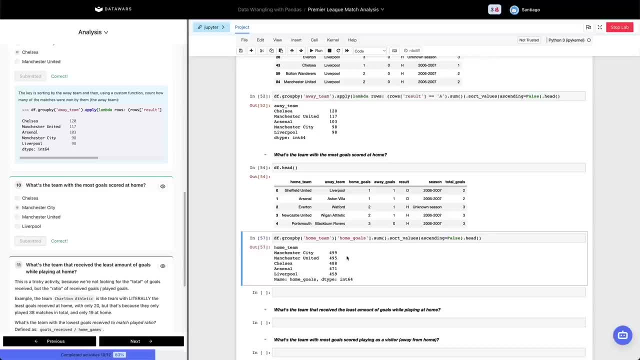 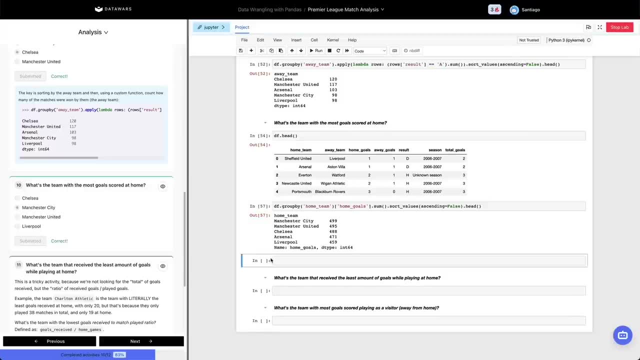 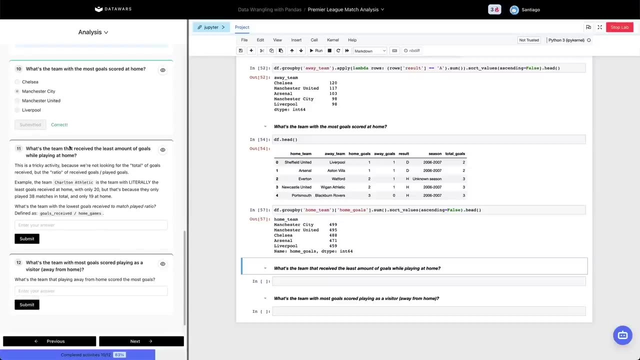 So let's try that out. And that is correct. A pretty dangerous team in attack, Manchester City for sure, especially now. This is outdated, especially now. Okay, second to last, what's the team that received the least amount of goals? 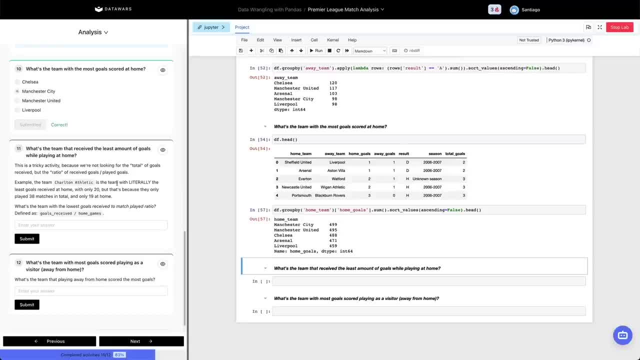 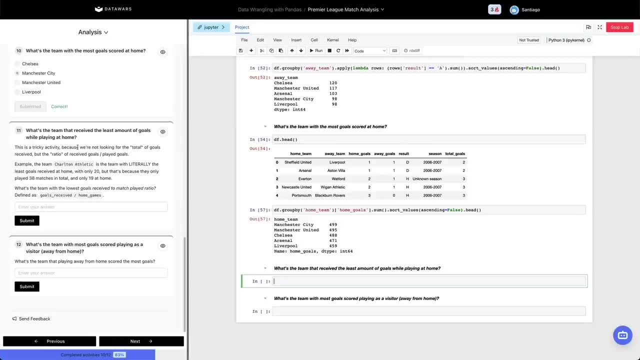 while playing at home. And this is also a very interesting one, because if I was just naive, I was going to do something like df: the team group by home team. What's the team that received the least amount of goals while playing with home team? 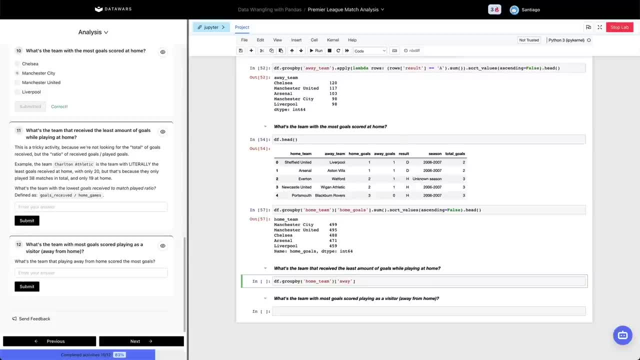 By home team. what's the team that received the least amount of goals while playing home team? and I'm gonna be away goals. so it's team playing at home, away goals. but some sort values, head, there you go. so charton at play athletic ha only. 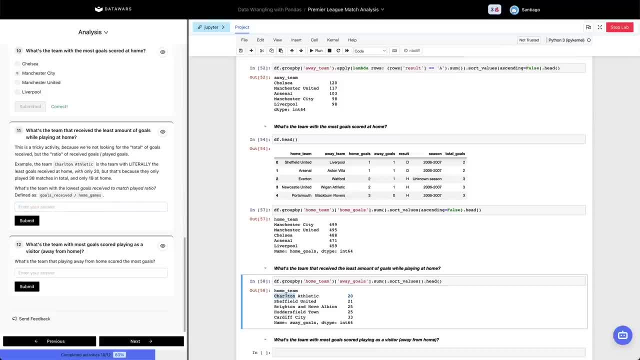 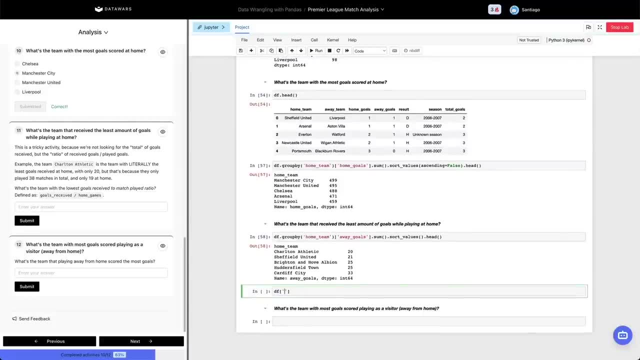 received 20 goals. right, but the. the reality is that a only play DF that lock the F or no, let's do DF at home- team equals charton. very, there you go that some they only play 19 games at home. so it's interesting, because what these 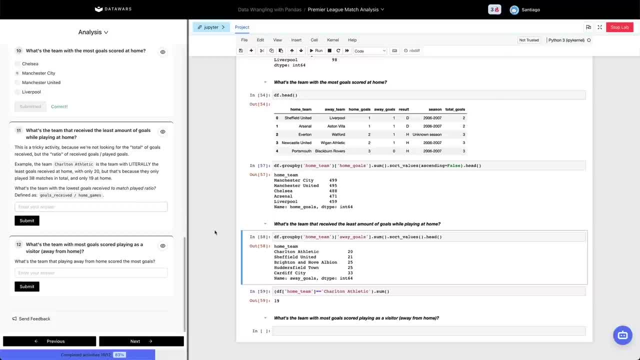 activities. asking us is for the ratio of goals received over home games and I think, if you have not pause, I think it's a very, very good moment to pause and try to resolve it by yourself. but anyway, let's just do it. we're gonna start first, we're gonna keep the same group by operation, but we'll try to get. 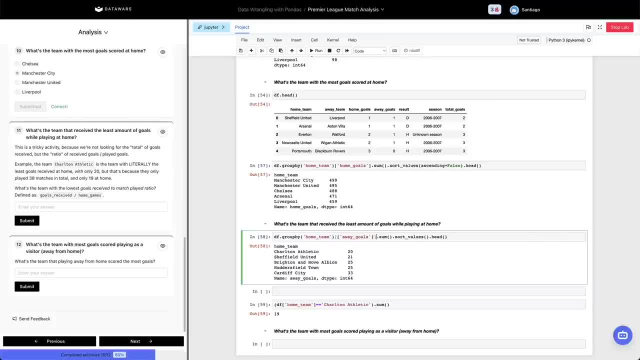 two things: we will try to get the total goals they received and the total matches they played. so we're gonna get, we're gonna get a, a, a way goals and we're also gonna get first. we're gonna get just here: home team. I have two different operations for that. we're gonna use the aggregation. 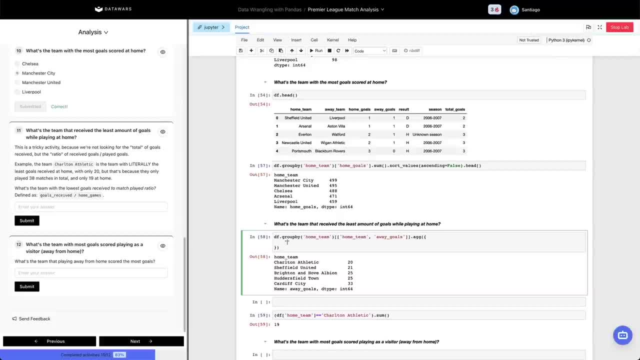 method and when I use a dictionary and we're gonna say for home team, perform the size operation, for away goals, perform the sum operation. let's take a quick look at what we have. there we go, we're gonna sort values by by, by home team. that's actually not sending falls by home team. I did. 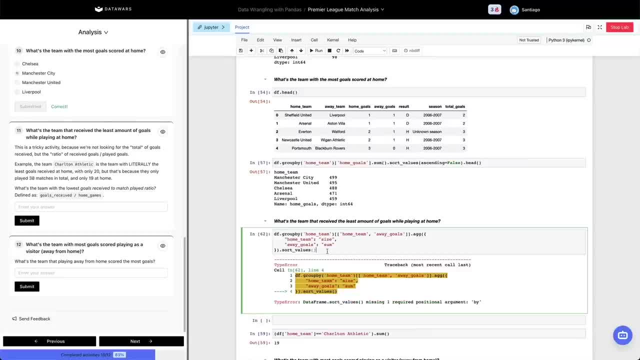 something wrong here? why bad sort values by home team shouldn't be around here? it is important to keep in mind that when I don't send it, this is just trying to get everything together. how final, whatever. right now we have a second team and the Baque team and we're not just gonna be popped out by the home team and 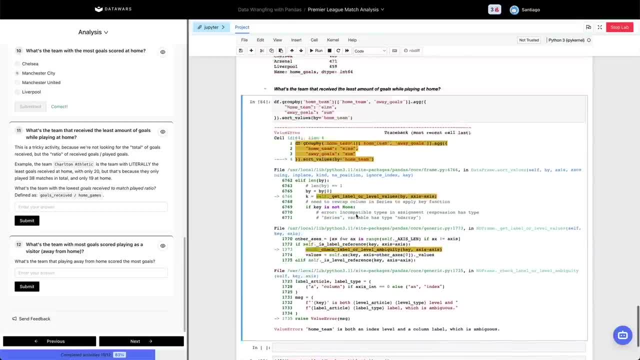 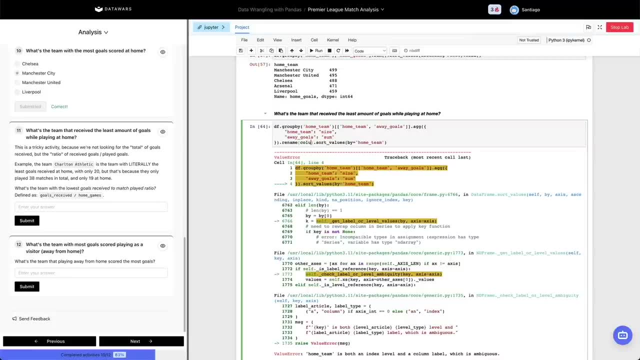 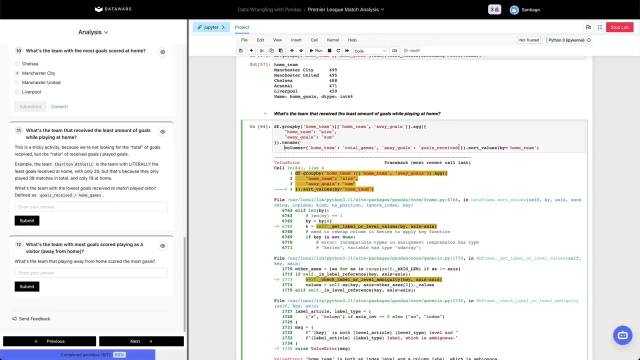 why is? oh, because it's both. so let's replace, replace uh rename, rename uh columns. we're gonna call home team um total matches to total games. i'm gonna put away goals equals goals received. there you go um. let's break this in a couple of lines really quickly and ascending false, there you. 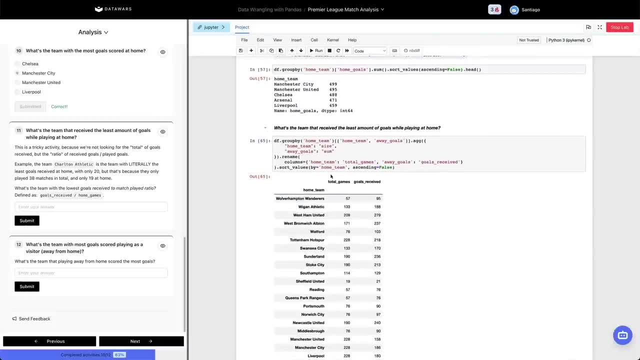 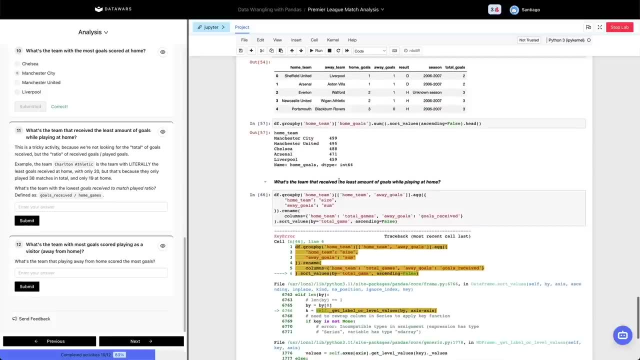 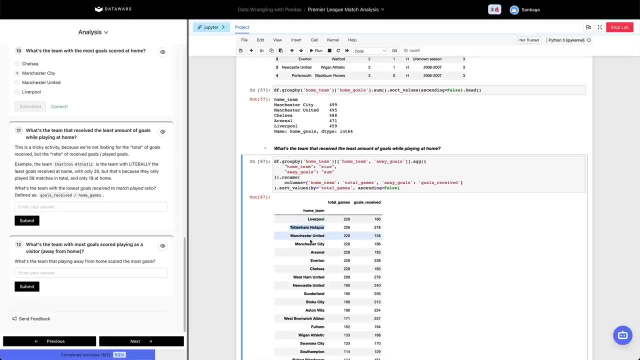 go um total games. no, because this is total games. now, games, there you go. so liverpool, tottenham, so these are the usual suspects, right, the teams that have always played at the top of the premier league. um, what we can do now is sort by two things. we can sort by goal, by, sorry, by. 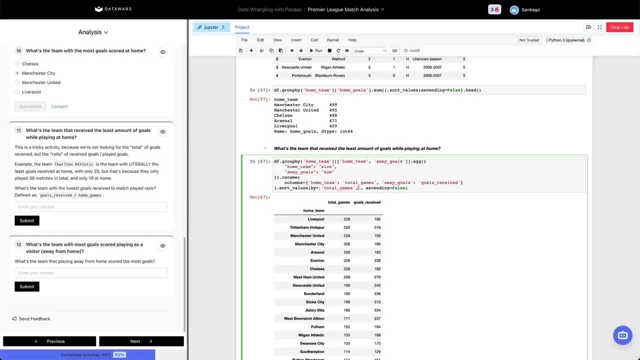 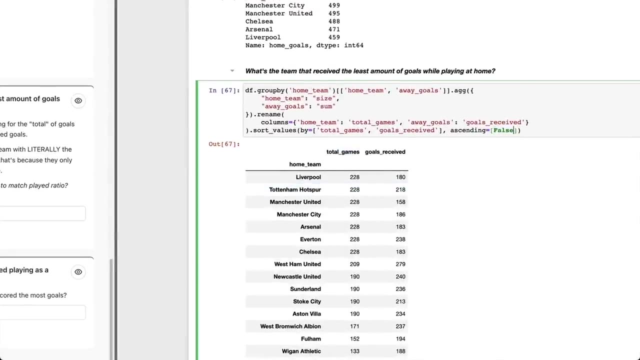 total games and we can also sort by goals received. but we want to flip the sorting here. we want to get all the players that- oh sorry, all the teams that played a ton of games, so ascending false. but then we want to get the ones that receive few goals. so we're going to be ascending. 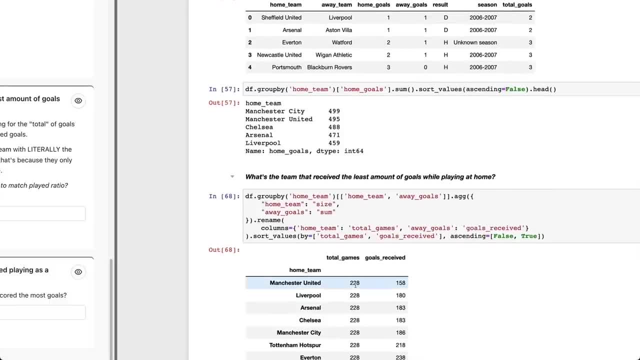 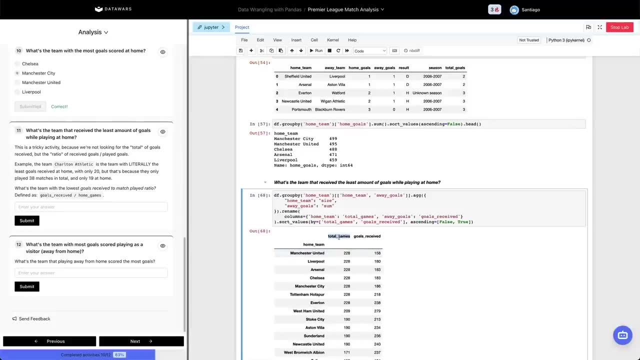 true, and now we're going to get the manchester united um. manchester united is a team that played the most games with the least goals received. we can- let's say we can- rename this thing. we're going to do something like: um, we're going to call. 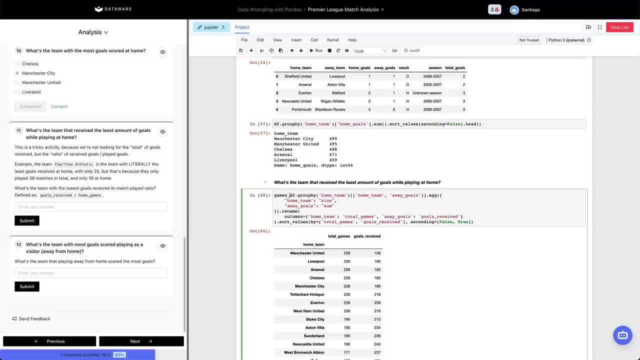 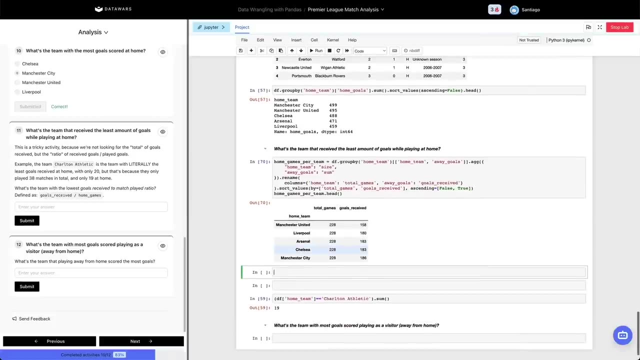 it um games per team games, home games, low end home gamesята games per team and call that um head. we could do something like um ratio. what's going to be? it's going to be goals received per match, and we're going to call this thing. we're going to be the result of. 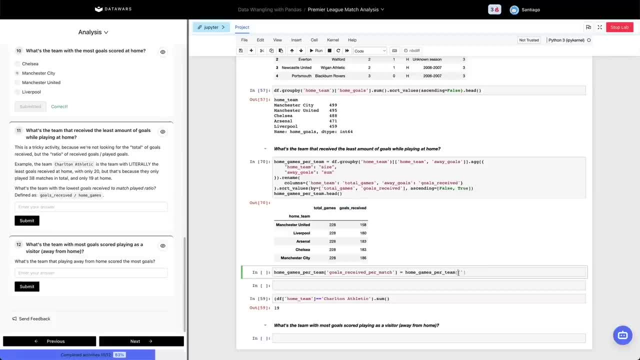 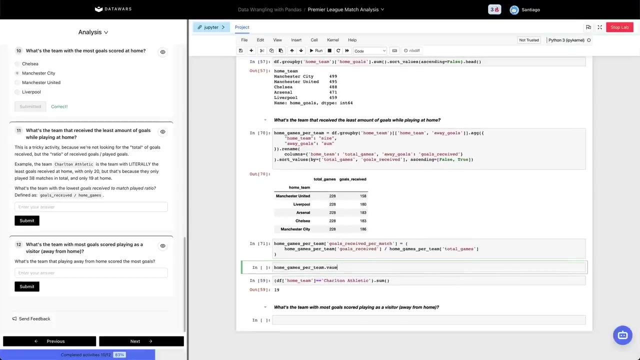 team at goal received, divided by home games per team at total games. And let me break this into multiple lines so it's a little bit more readable. And now we're going to do pretty much the same thing as before. But we're going to do is value, sort values by goals received per match Head. 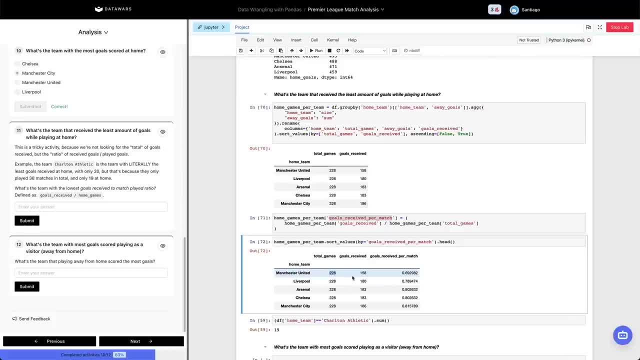 I get the same result, just Manchester United with the best ratio in terms of goals received per match. It's actually tried out. because I haven't tried it out. Let's see if it's the team we're working waiting for. that is correct, Correct, Wow, Basically what I'm saying. 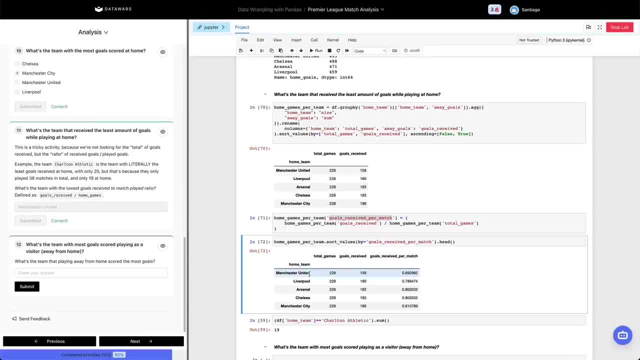 here is that we tried. we first got we have for the same grouping operation. we competed two different things: total games- sorry, total goals received those away goals because it was the whole team. But we also competed how many games they played, So same. 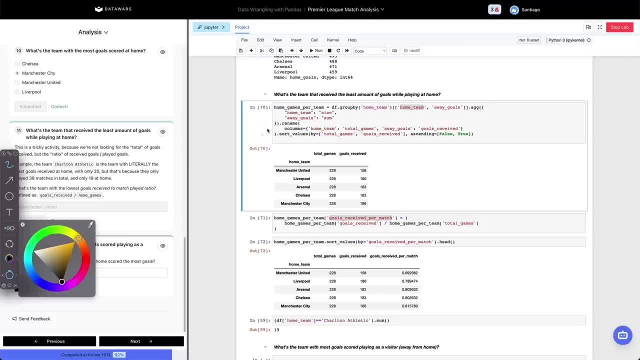 group by operation. if you allow me a very quick draw: right, we have like the big chunk of the teams And then we did like this separation of small, small groups for home teams. But then we competed two different things for home team. This gave us the size for their way. goals is gave us. 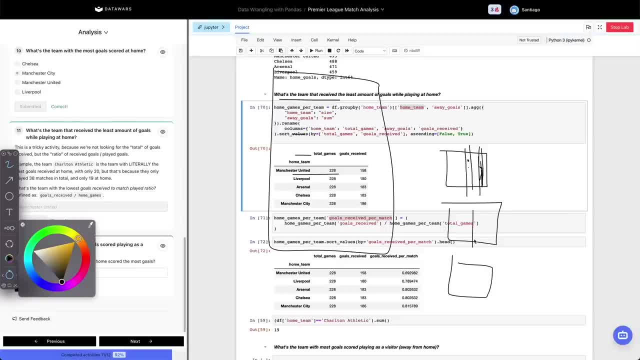 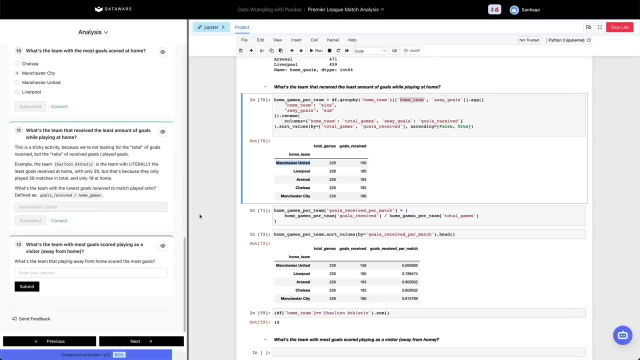 the sum right, some, some all the way goals. And we did these two operations in all the individual chunks to compute the final results. We quickly identify Manchester United as the one meeting the requirement of activity. But we went one step further to actually compute these. 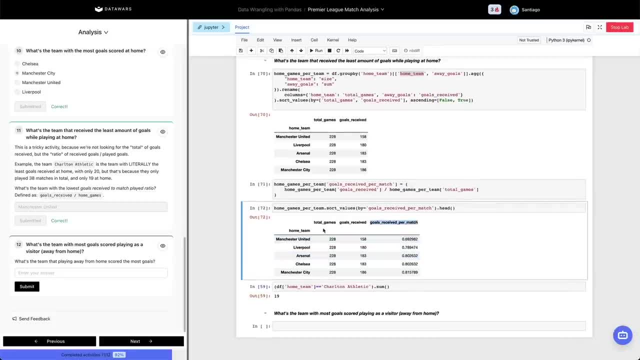 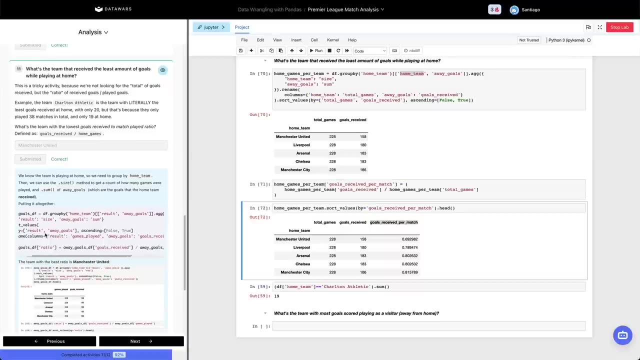 goals received per match value. Why is that? because if we want to make this thing analytical and potentially automated, we need it. we need an analytical way. What else there is, I think we can take a look. I think there is a pretty interesting solution here. Now I thought that we had a 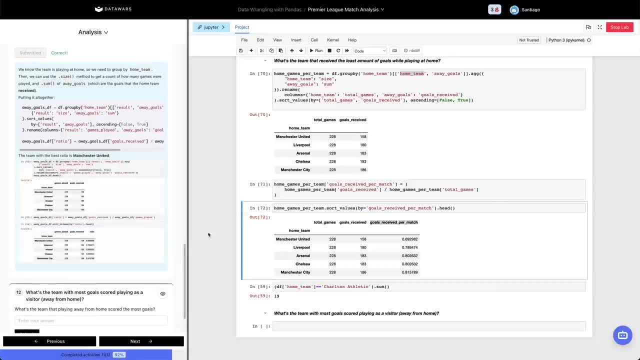 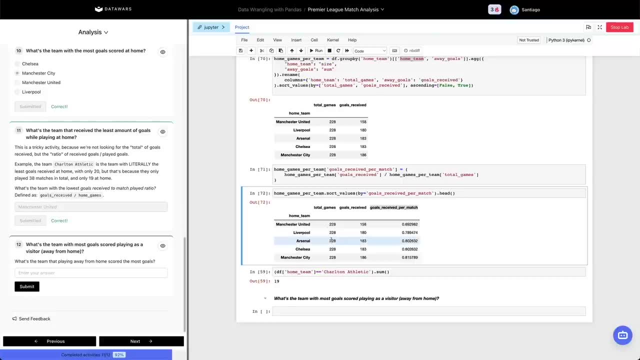 solution that had everything in a one liner with a apply operation. it is potentially doable if you want to give it a try, But I think readability matters in this case. And finally, what's the team with most goals score? playing as a visitor away from home? And this is going to be pretty much the same thing as before. 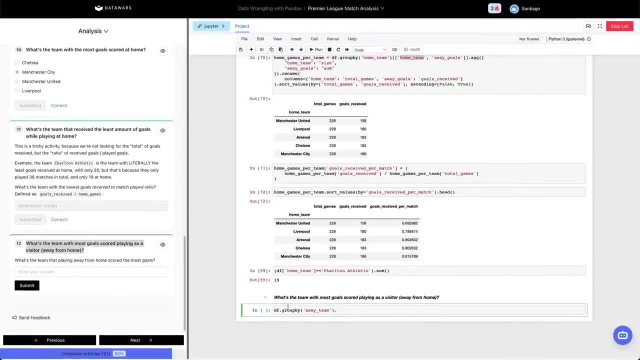 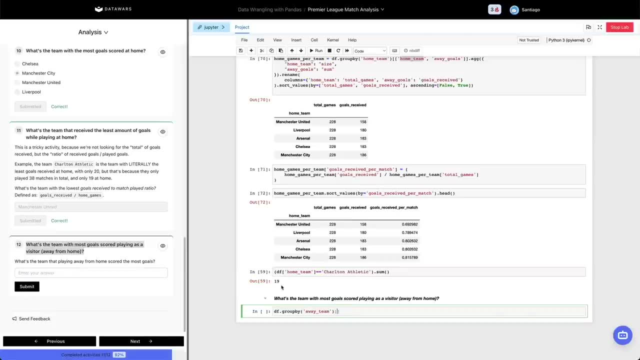 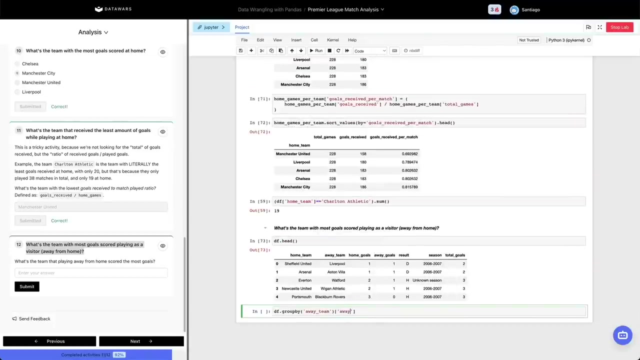 group by away team And we're going to get the team playing away from home score. more goals are going to get goals Go. I forgot already the name of the columns. It's away goals, Away goals, Away goals. sorry, And what we're going to do is some. 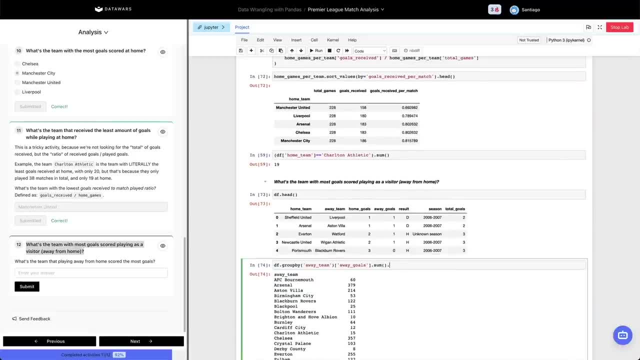 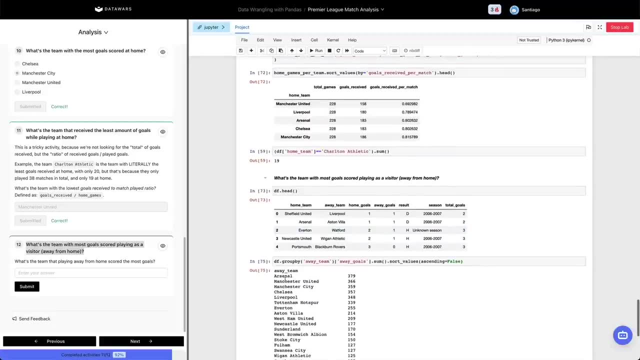 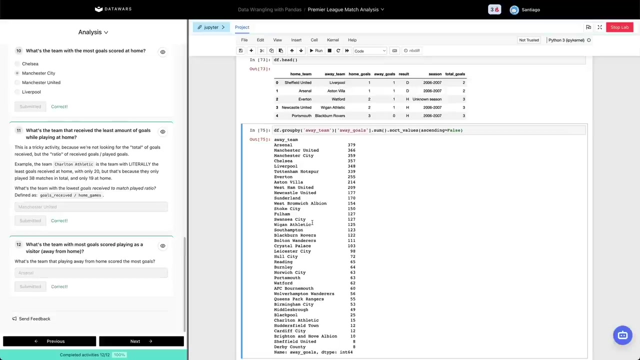 get a preview, And now we're going to do a sort values ascending falls, And it seems to be Arsenal. Let's give it a try And it passed And we completed our projects. So this was pretty much the the activity we started. 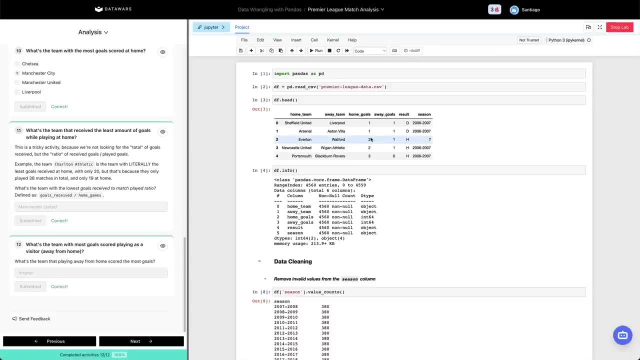 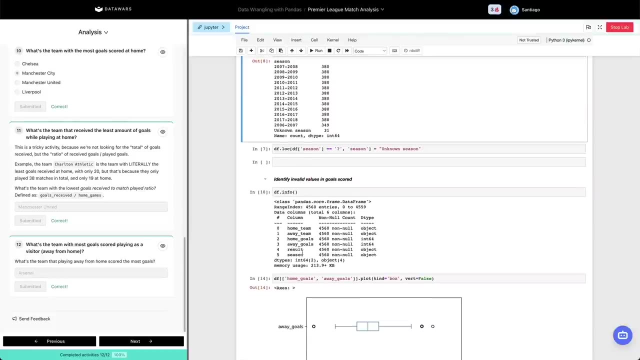 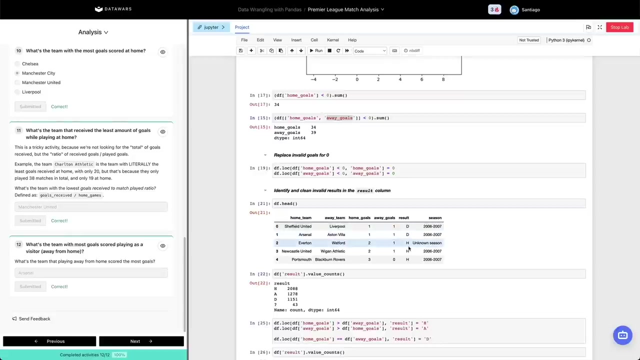 with a little bit of data cleaning, data wrangling. pretty interesting Because again we had a good variety of different issues with our data. we have the issue of the invalid seasons was just a string invalid pattern. Then we move to the invalid count of goals, which is an integer out of range. Then we claim the categorical result variable. 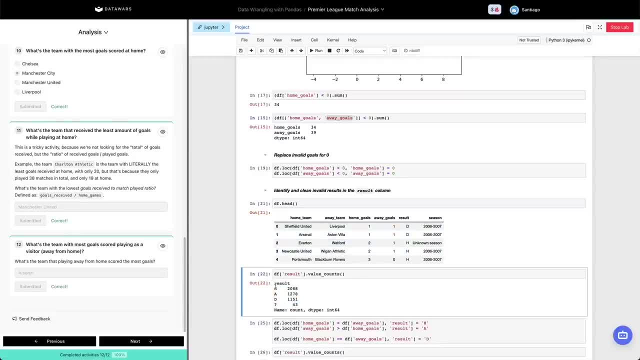 was just a potential, just a result categorical. So the result should be in this, in this subset. we had a way to clean that up and explain hole numbering, But once again the fee home score this year is huge. So this would be worldwide premium rate. 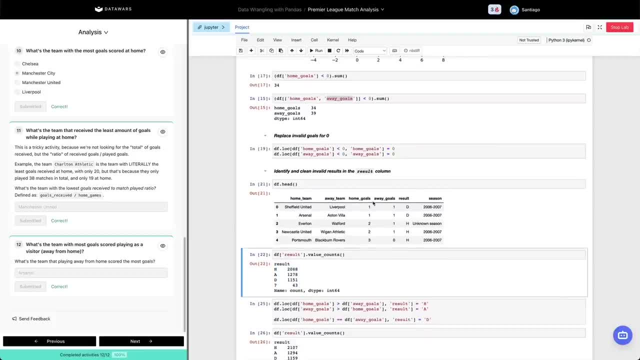 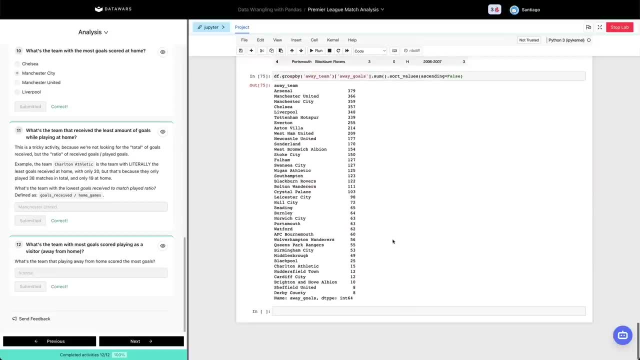 So again we sort of we Twimlay had the ability to give you subset. We had a way to clean that by just calculating something else in the data frame. That was a good thing. And then we started with a bunch of group by activities, all very 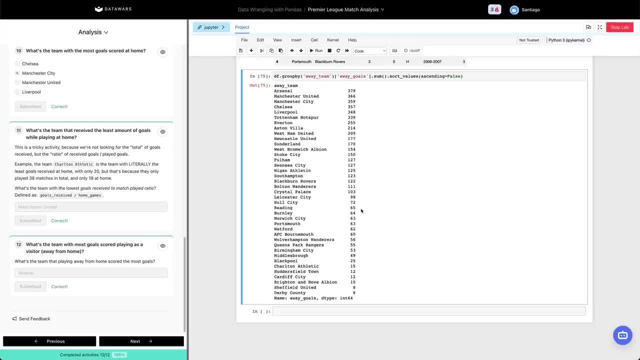 interesting, So take a look at yourself if you want to replay it. In other case, we have a bunch of other projects dealing with data wrangling and group by and all these operations. This is a very interesting project that combines some data wrangling skills. 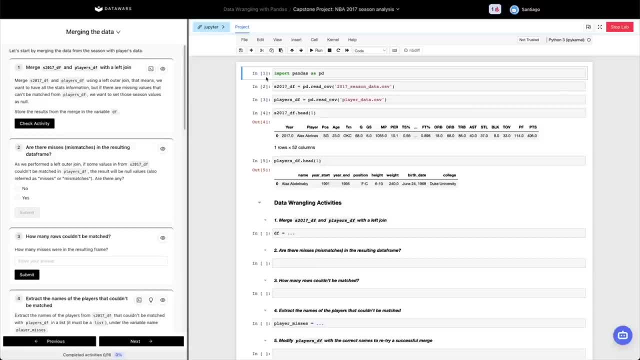 which involves merging data frames, creating new columns with some data cleaning skills, And it's going to require you to take a look at the data and do some cleaning to make those merge work And finally do some analysis. some question answering with group. 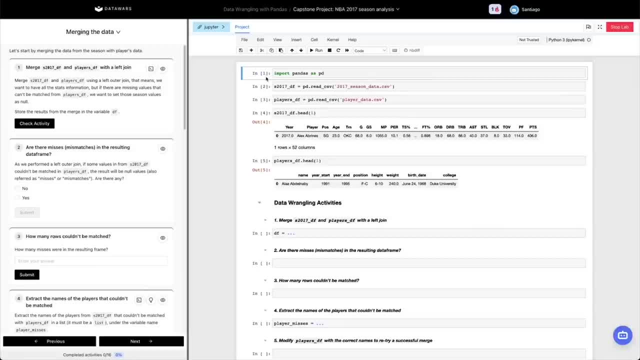 by operations, with transform operations, So it's a very, very interesting project for sure. As usual, I encourage you to pause the video, first try to resolve it by yourself And then, of course, take a look at the solutions, because maybe I'm 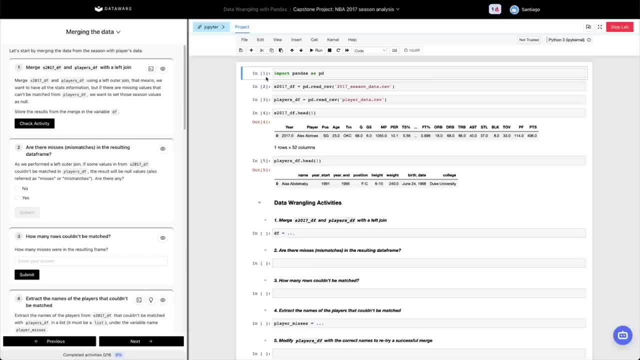 choosing a different way of what you're doing and you can see something different. So, with all that said, let's just get started. I have the first few rows executed already, as you can see, And let's take a look at the data that we're going to be working with. 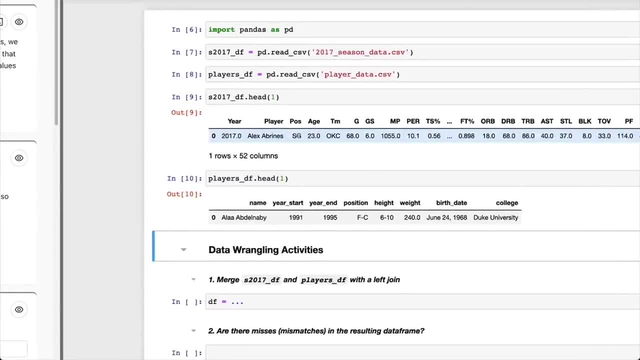 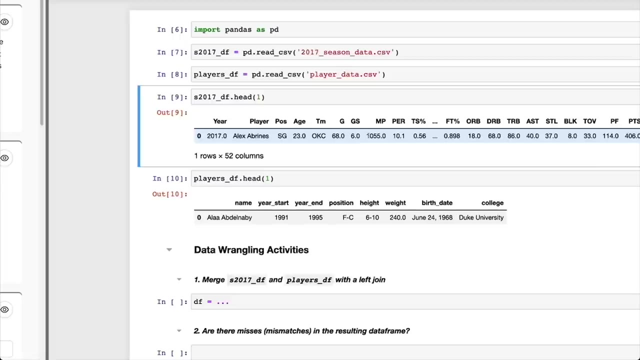 In this case, we're going to be working with NBA basketball information And basically we have the 2017 season stats. that's going to be in this data frame right here, which involves the usual, you know, just information for each player as an aggregate of the whole season, And then we have a player's DF data frame that. 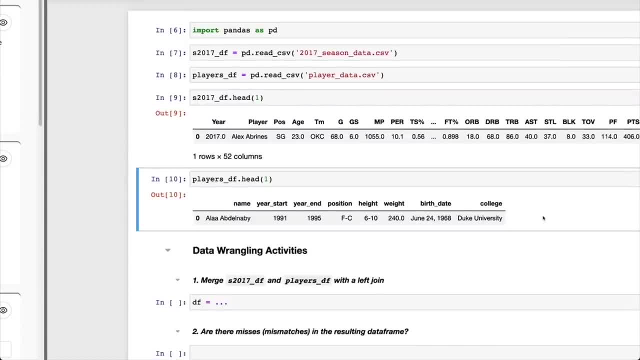 includes the personal information of the players, so their name, their weight, birthday, college, etc. The important piece here is that the player's data frame contains information about all the players in the registered history of the NBA, So that's from like 1950s. The information in the 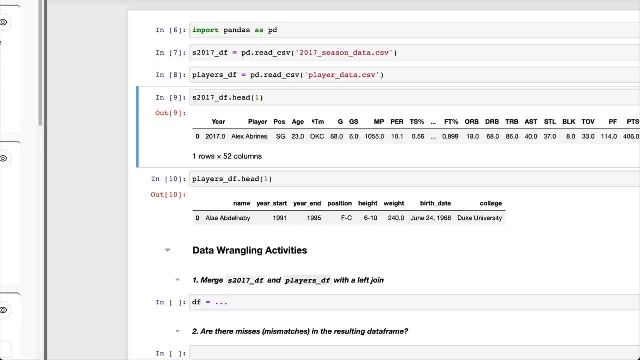 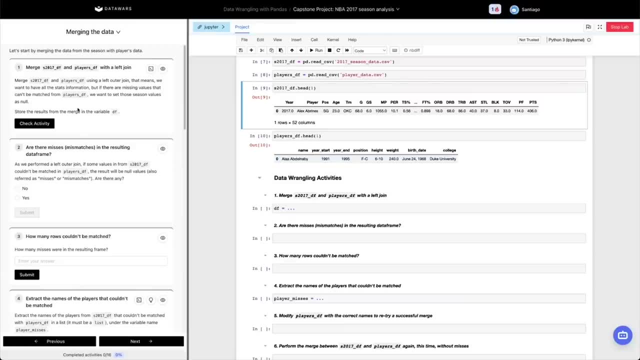 seasons only from 2015.. And then we have the data frame that contains information about all the players in 2017.. So we're going to start by doing a merge, but, of course, going to be an interesting one, because we have to merge in a specific way. The first activity, and here again, encourage you. 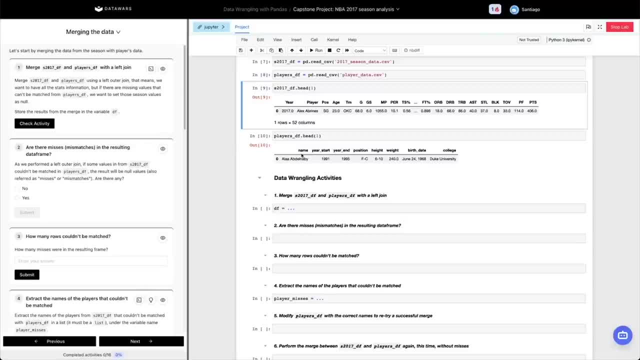 to just pause- involves merging data from the 2017 season with the players but performing a left showing. So basically, we want to include here in our seasons DF data frame. we want to include the personal information from the player. We want to bring the data to our existing data frame from this particular season. Okay, so as you, 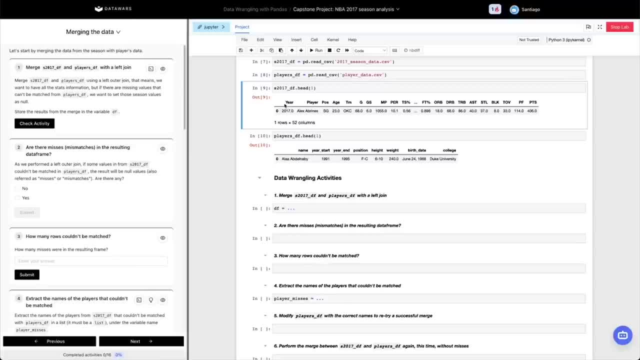 might remember, there are different types of merge to do. we can do an inner, we can do a left or right outer, we can do a full outer. In this case, by performing a left outer join, we're going to be able to contain, to like to keep all the information from these data frame 2017 and bring only the 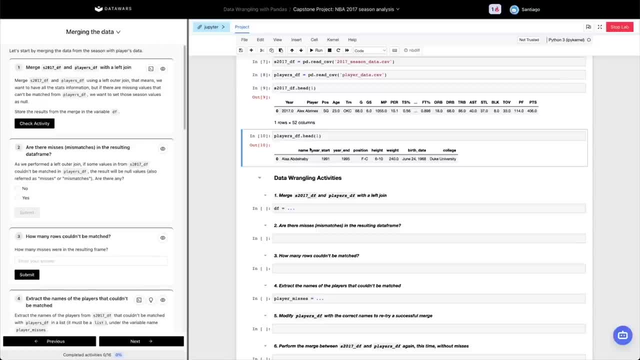 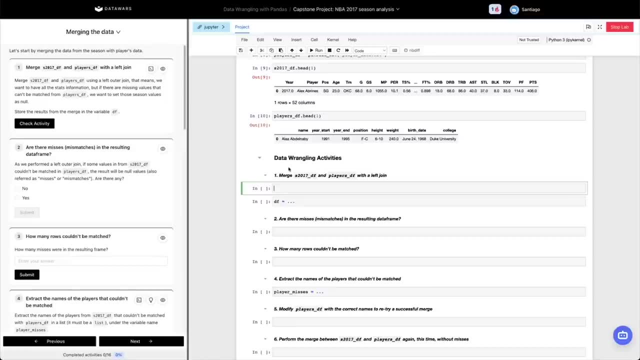 matches from the players DF data frame. So let's go ahead and do that Again, this is your, your opportunity to pause the video To do a merge. what we're going to do is we're going to start with season 2017 DF and we're going to merge, merge with merge- players DF. We have to first, I'm going 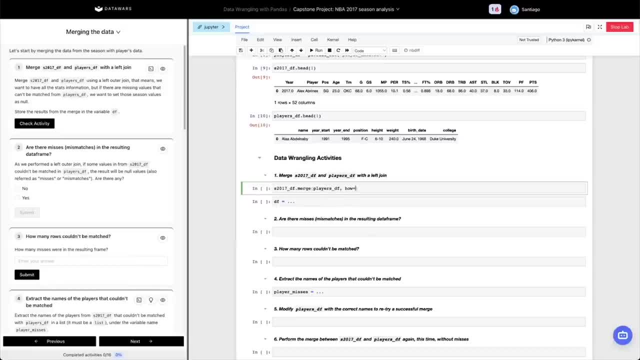 to players- DF. we're going to do a how left, Because that's basically what it's asked. And again, the reasoning is that we want to keep all the information in the same thing from 2017- DF, And we're going to pass the columns to merge. So, on the 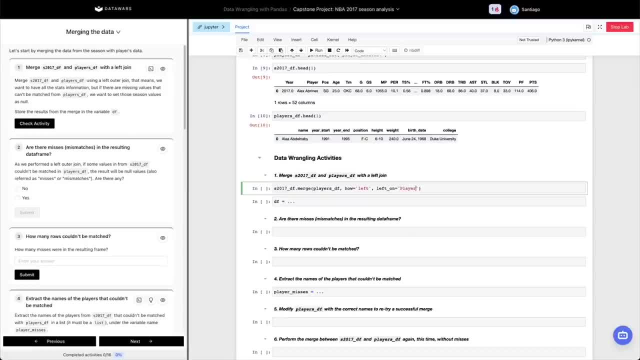 left side, we're going to pass the player And on the right on, we're going to pass the name. it's the same information but it's two different columns. If you remember, we have the on on based attributes To refer to individual columns and we also have the indices, if potentially you're merging per. 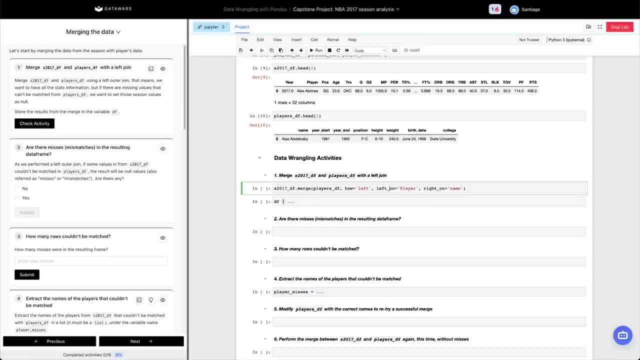 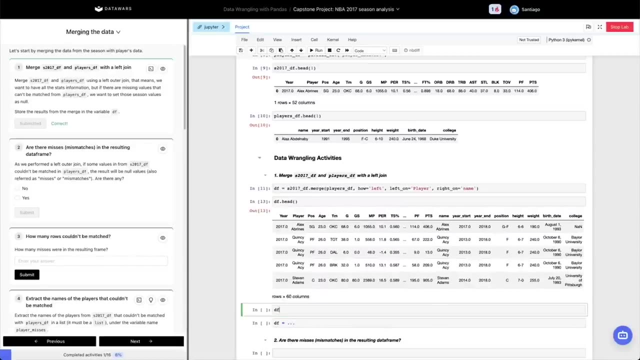 index. in this case we're just using the regular columns And we're going to assign all these two data frame And let's check the activity to see if it passes. We can take a look at the DF. this is going to be a long data frame. I can actually show you something like DF dot head and we can do just. 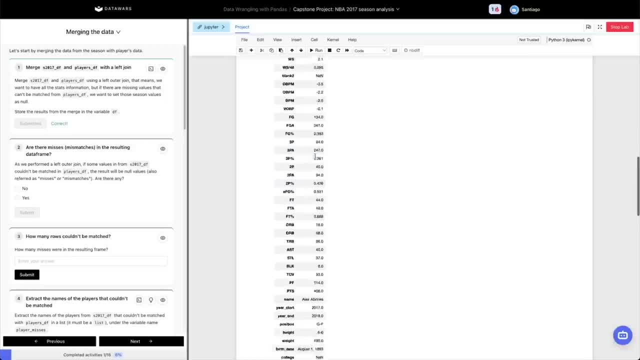 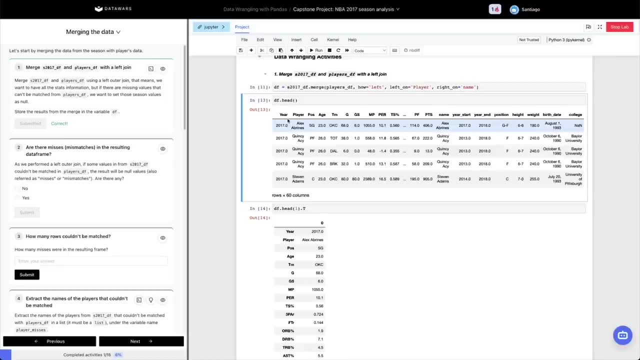 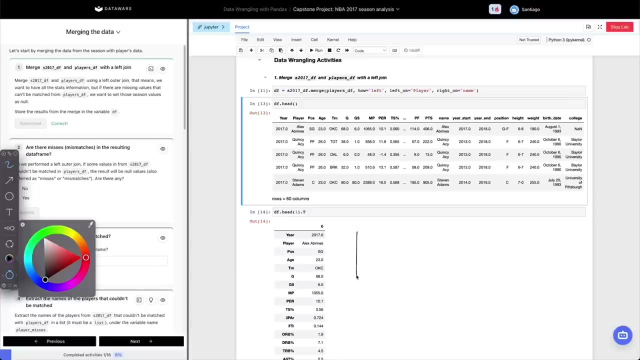 the first row under transpose So we can see all the information right here. So we had. let me potentially do a little bit of a drawing, if I'm allowed. here we're going to select red. Basically, what we did is we didn't. 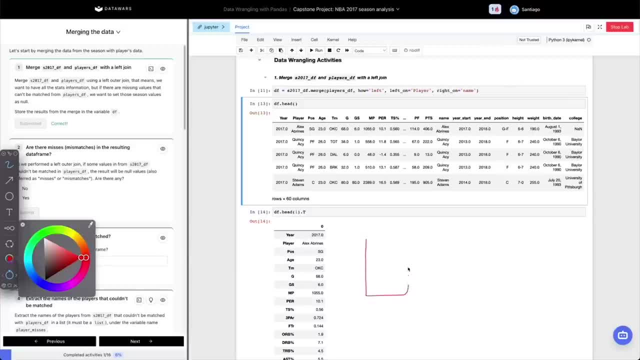 select red. there we go. So basically we have all the seasons that we're going to make like a long data frame. I'm going to use blue to the players merge. players merge right there. The resulting merge. we can use another color. 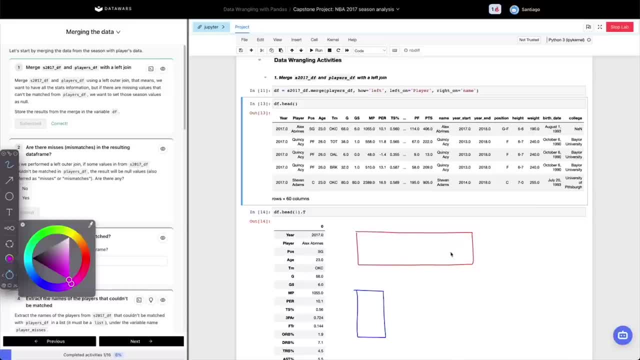 let's say here, purple. The resulting merge is gonna basically, as it's a left outer, join and this is left. what we're doing is we're bringing this data frame to the side here and basically make it match with whatever information we have in between. 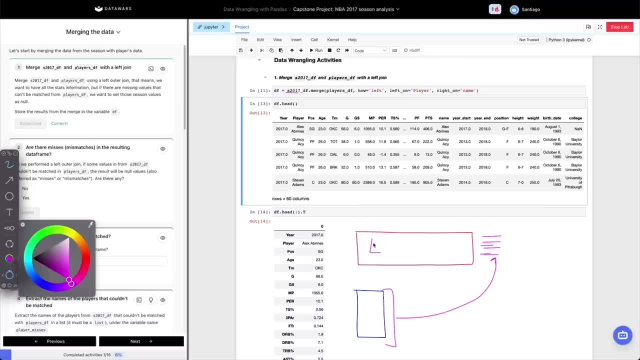 So if in the season 17, there were two players that were repeated, we could have potentially duplicated that data, And that's perfectly fine, because if we have the same player here two times because of any reason, because a player played in two different seasons- 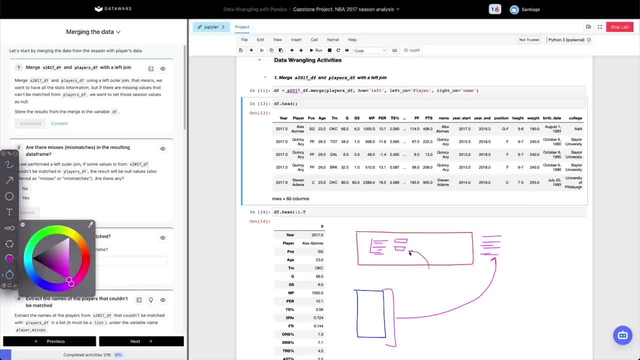 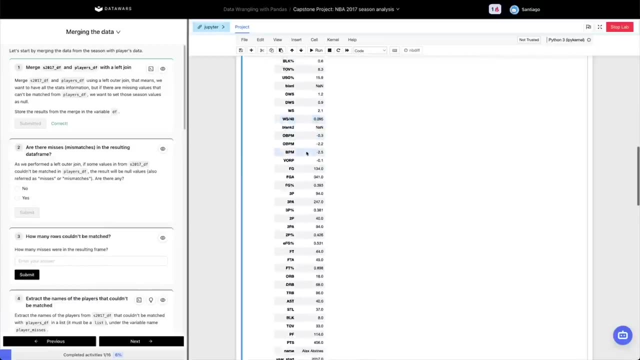 two different teams in the same season, we actually wanna duplicate the right hand information in both of them Because, again, what we're doing is we're completing with the personal information of the player. So, said that, let's take a look at the whole data that, where we have 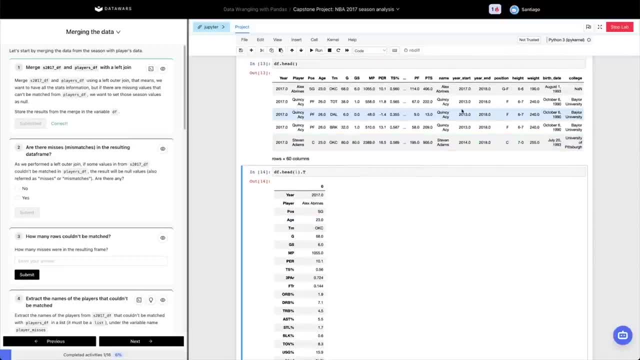 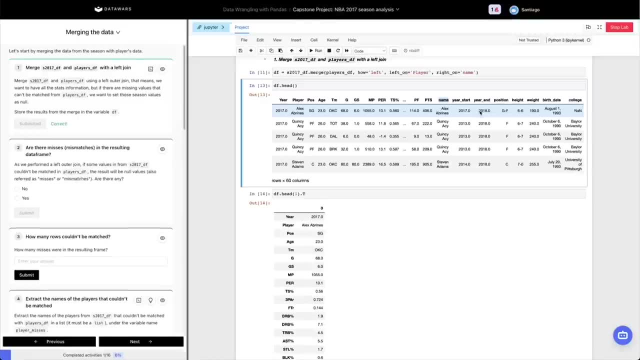 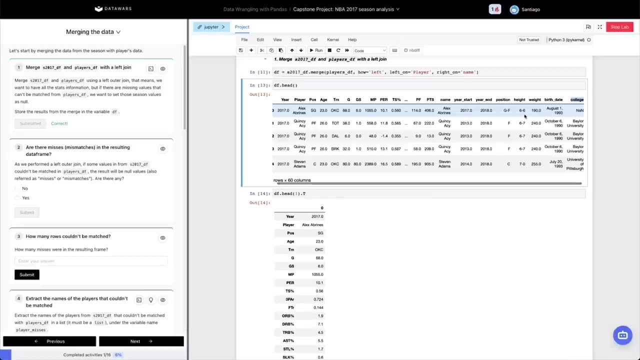 it's a large data frame, but what's gonna give us the key if the merge was successful? the important piece is the name, because sometimes you're gonna find that some columns are gonna be nullable- like, for example, college is nullable- but this doesn't indicate that the merge wasn't successful. 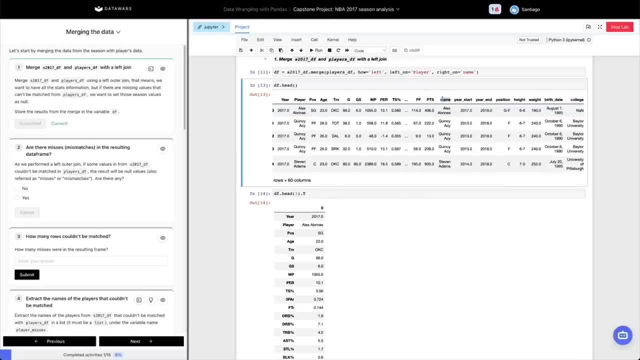 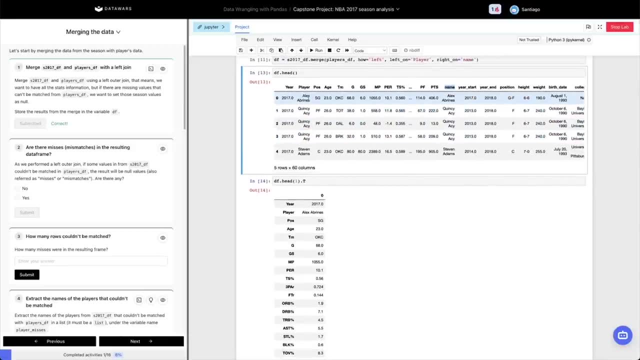 This indicates that just college was null, but the name column is not nullable. So that means that if we find a value, a row in the df variable that is null in name, that means that the merge was not successful. So are there any misses in that data frame? 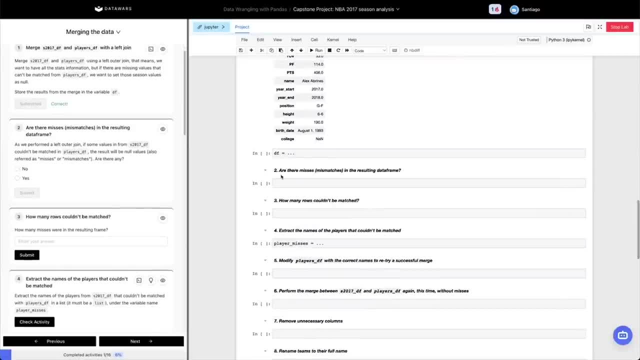 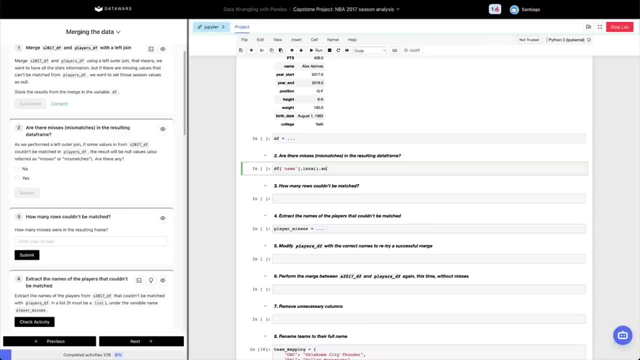 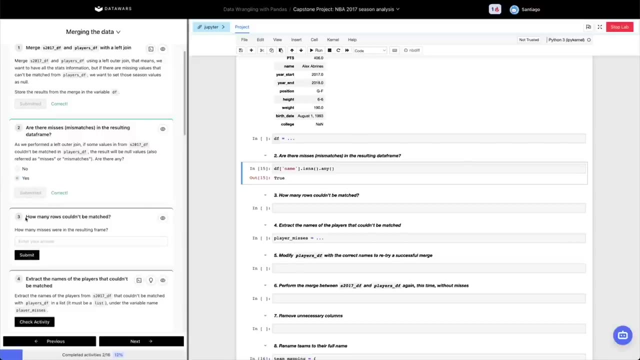 And this is the second activity. We can quickly take a look at that by doing df, add nameisna, and here we can do, for example, any, any. This is true. We can actually answer that real quick. and the next one is going to ask us how many. well, we can do a sum right there. we can. 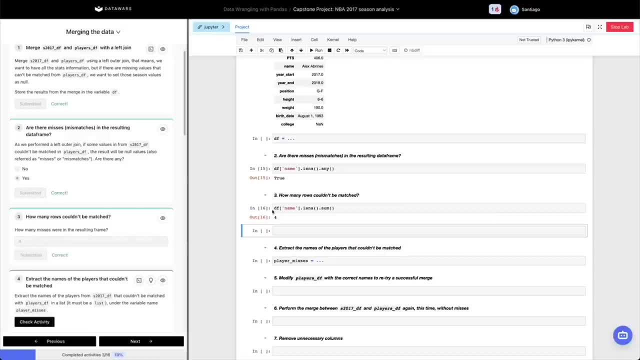 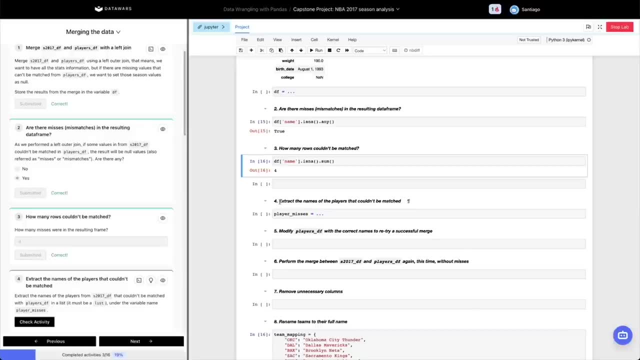 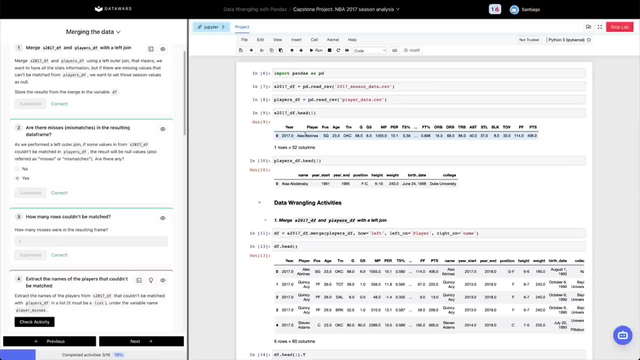 find there are four missing- uh, four missing players basically we couldn't match. so there are four people and i think now it's going to be a little bit more clear once we visualize- and there are four, four rows in the seasons data frame that we couldn't match for a valid player. 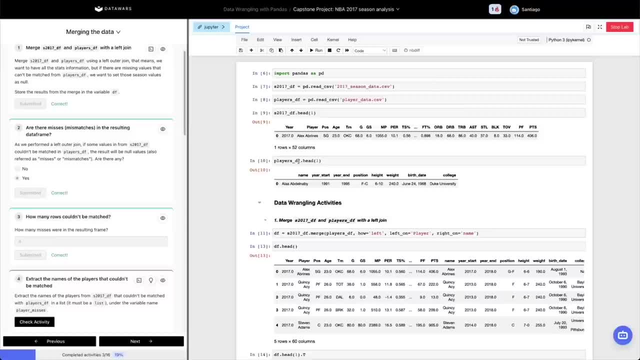 which is strange. right, because we know that this players df data frame contains information for all the players in the nba. so how is it possible we couldn't match four players? let's actually take a look at those people. and that's um the fourth activity that we have right here, that. 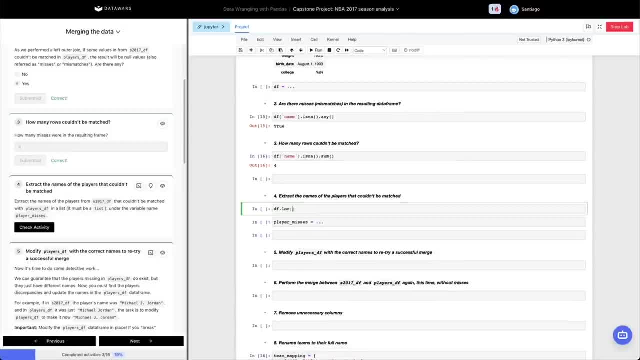 is extracting names. before we do so, i just want to show you who are these missing players. so let's take a look at the values in df that are that have a none or a null value in name. and those are these four players. right here we're. 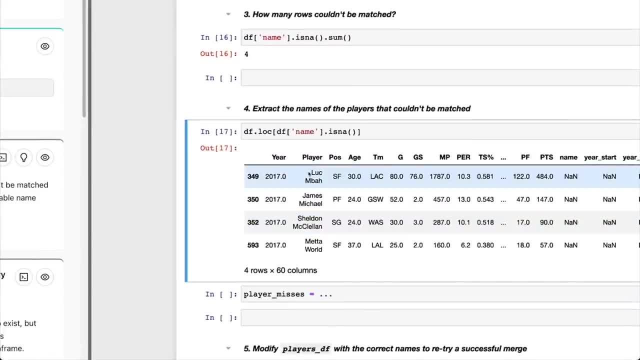 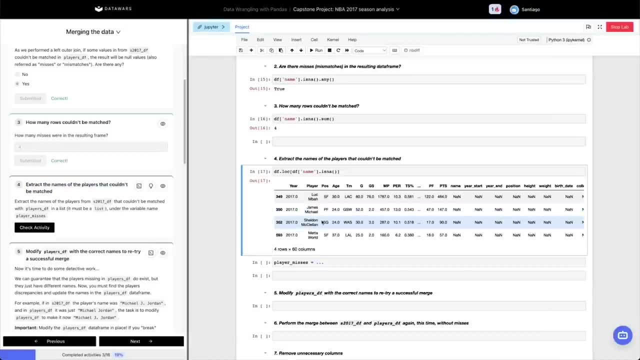 going to take a look in a second at these players and see why we had that mismatch. so this activity is asking us to basically find those four people. it's asking us to put them in a list. so what i'm going to do is just going to do that, and i'm going to plus here the player and we're going to do. 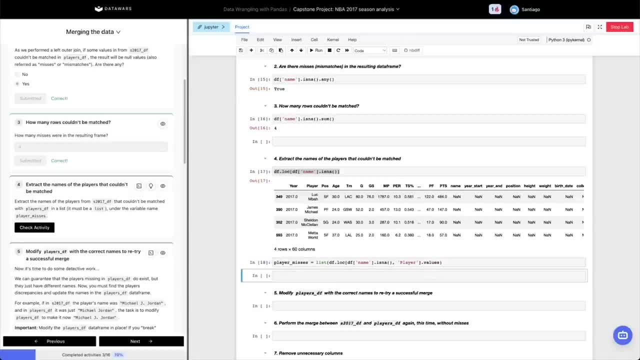 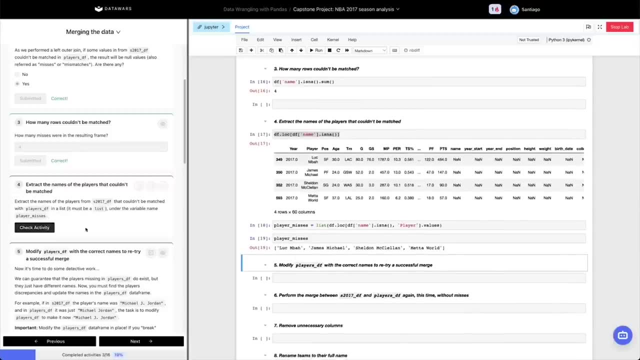 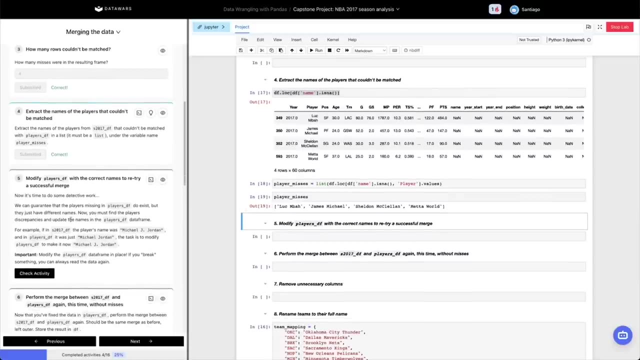 that and finally, i'm going to make here a list now. player misses contains the list of players that are missing. we're going to check the activity and it passed correctly. so this is a very interesting activity and this is the one that i think is the most representative. 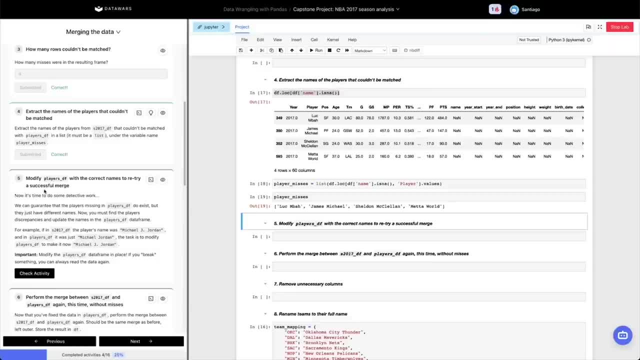 of the data cleaning process in general for any data scientist, data data analyst, data engineer- which is actually fixing these missing issues right, and there are sometimes different strategies. sometimes you can just delete the missing rows, because i mean, if you have millions of rows and there are a few that are null, you can just delete them. sometimes you can replace it with: 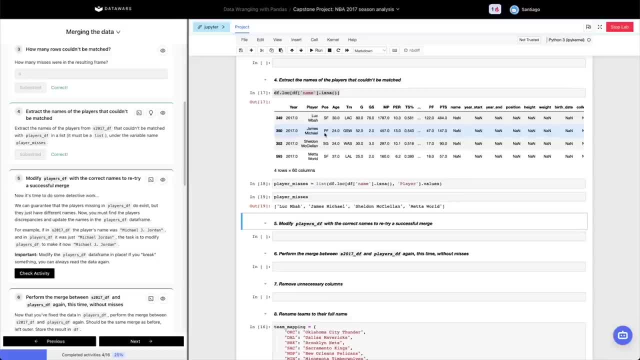 something else. sometimes you have to actually fix them. you have to realize, like, what happened and just fix it. and the way we're going to do is just doing some detective work and- and this is just perfectly normal- in the whole data engineering, data science, data analysis process, which is just 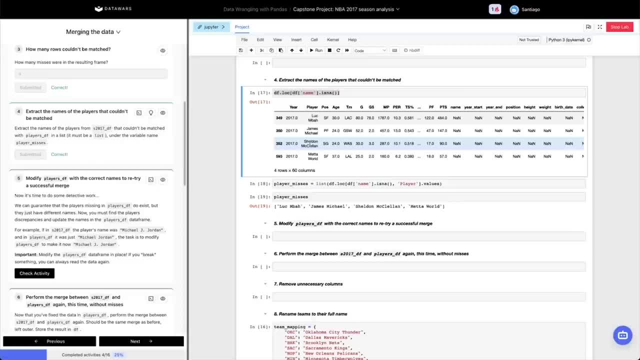 taking a look at your data and trying to understand with domain knowledge and this is a very important point- with the main knowledge, trying to understand what went wrong. and domain knowledge is very important because i can, i can and we will actually perform this, this cleaning we're going to fix. 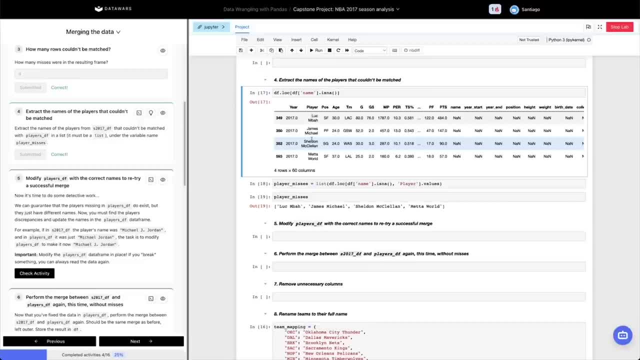 these values, but we need to understand a little bit of what happened with the basketball season. the same thing is going to happen with the basketball season and we're going to fix this. the same thing happens, for example- and i think i have already put this example in another project. 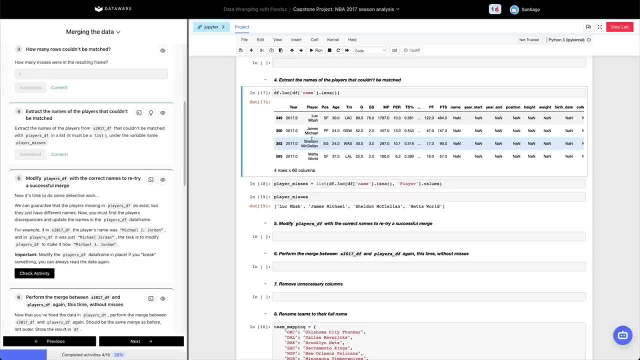 if i'm working, for example, in a biology lab or in a physics lab, in a nuclear physics lab, as a data scientist, there are going to be a ton of data cleaning tasks that i will just not be able to perform, not because i don't know the techniques, because i'm very good with pandas, but because i 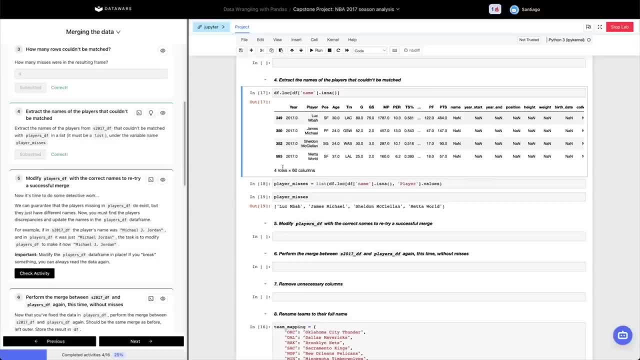 need to understand the domain that i'm working on in order to be able to perform some operations. understand my data right. so, for example, if you're working on a data science project and you're, you have no idea about basketball and you fee and you see a value for points that is a hundred. 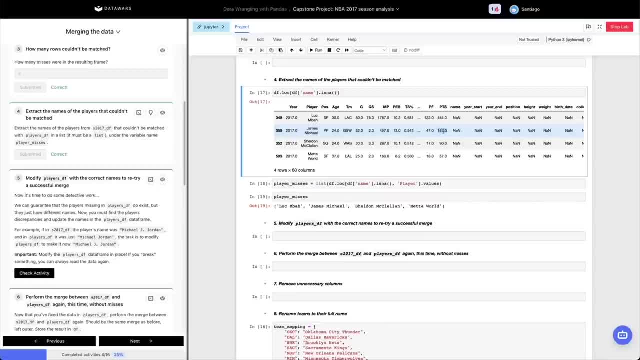 thousand. maybe that value is good for you, but of course it's pretty hard to make a hundred thousand points in a season in the nba. so by knowing the knowledge you have, you have just immediately placed the value in a in a given range, that of possibilities. so your data cleaning. 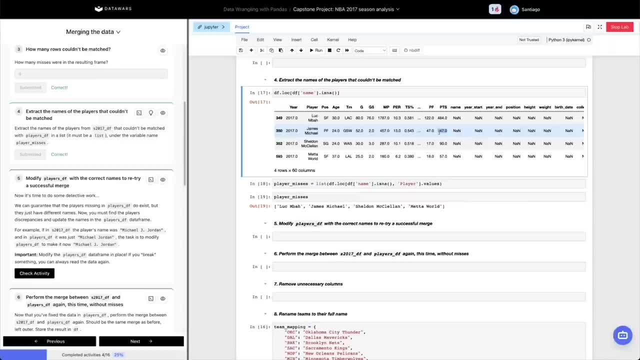 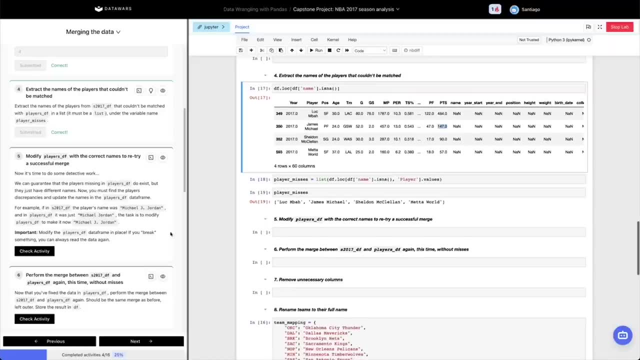 it's a lot more, it's it's easier and it's more precise because you knew the knowledge. so the same thing is going to happen here and actually, let's take a look at the activity and it tells us that with confidence, and i already know what the activity says with confidence. it says that 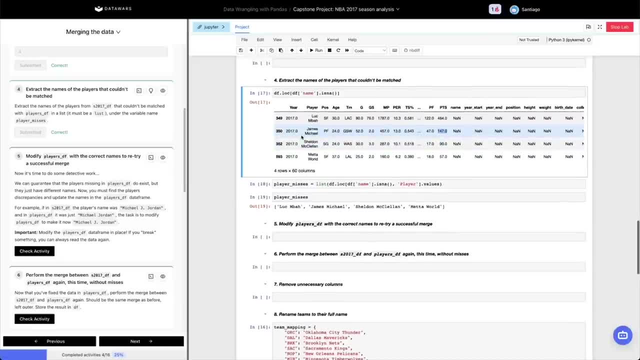 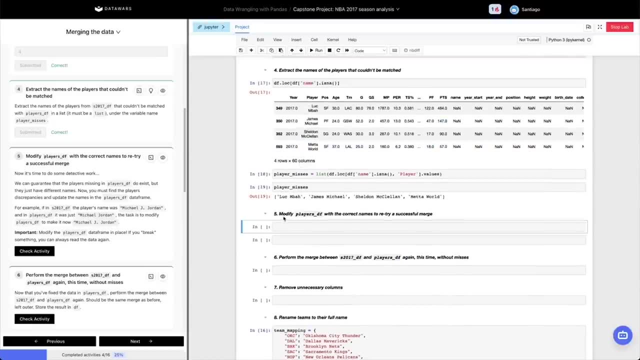 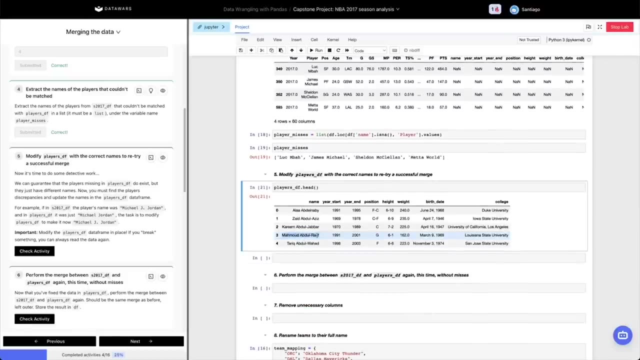 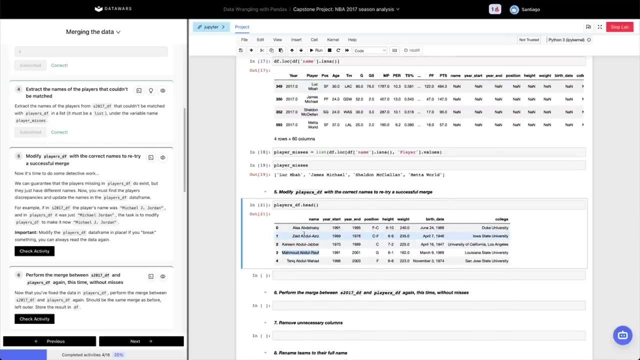 the players are actually in players df, so there is something wrong with players df the the right hand um data frame. so we're gonna players df dot head. so there are some. there is something wrong with the names here that somehow didn't match what we had in player in the stats of the 2017 season and the objective is to modify players. 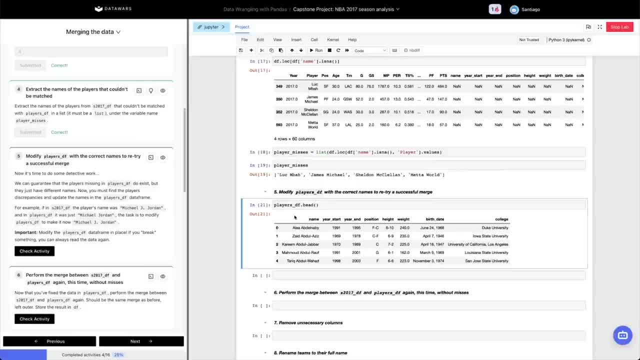 df, so they match whatever we had in the um in the 17, 20, 20, 17 season. that's, that's correct. so let's first identify where these players are in the 2017 season. are not in the players df. so basically, we can make a quick. 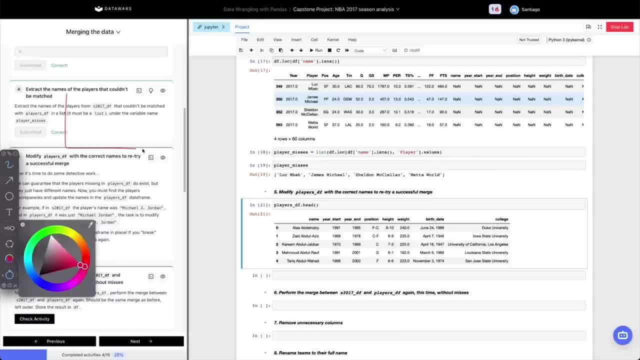 drawing here and potentially so we have in 2017. we have um this, this guy look uh and bah, which is not potentially in the players df. so in the players df um, the activity tells us for sure that it's there. we have to trust that for now. 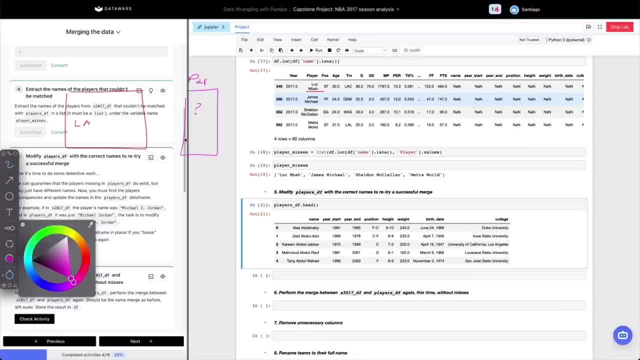 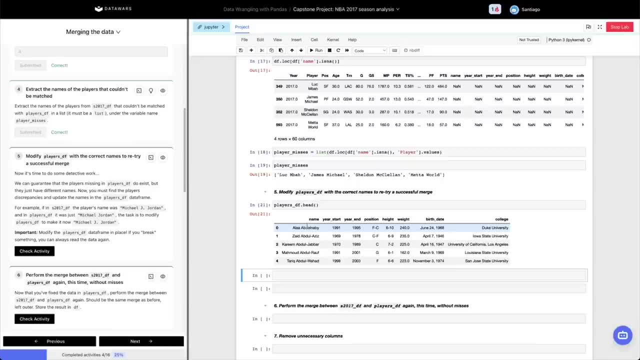 but these players, like, what name does he have? basically, we have to find these much to do, so one thing that i can do is just- and this is again a very detective work- um, there are multiple ways to basically find this, but i could do something like: let's keep it simple, maybe this: 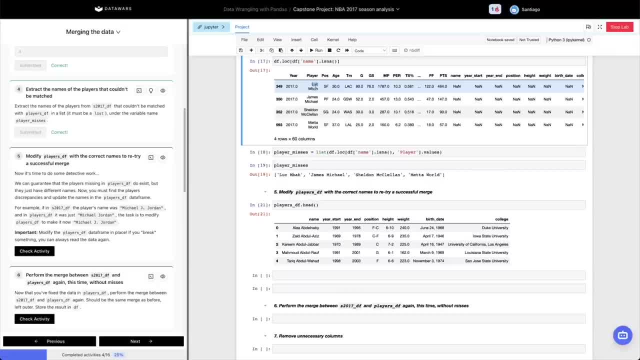 player has a middle name and that is part of the whole players df. but in the season that players wasn't listed with that name, So we can just go ahead and do something like playersDFlog And here I can do playersDF at name that contains the same last name. So is there any player? 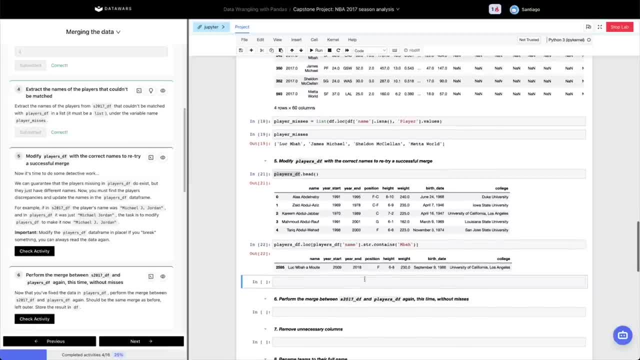 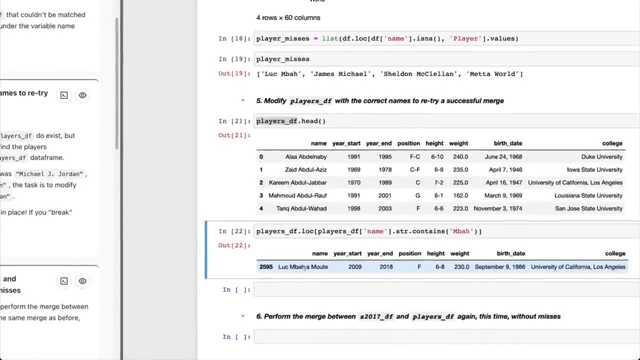 in playersDF that contains this last name And we can find the given player. What happened in this case- and we can just take a look at what happened- is that this player either added a new surname or always had the same surname, but in the 2017 season he was not listed with this. 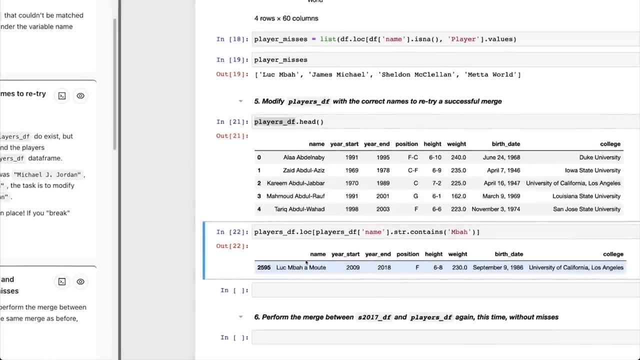 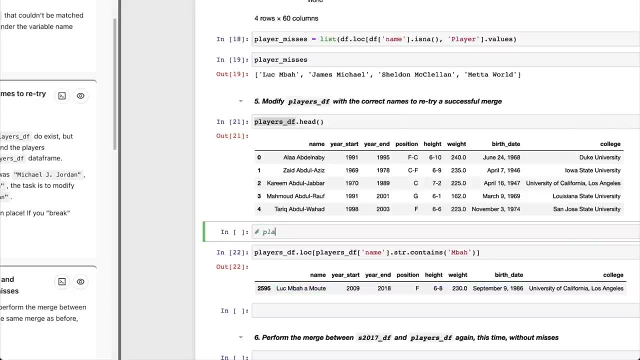 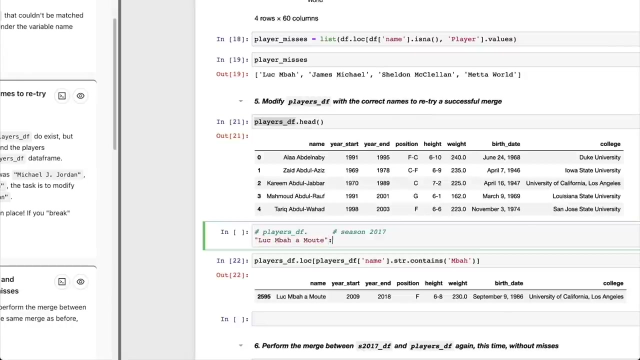 surname. So we are seeing the first incompatibility. let's say So. we can say that in playersDF- and we're going to do season 2017, this player should be named. should be named, we're going to do that. should be named. 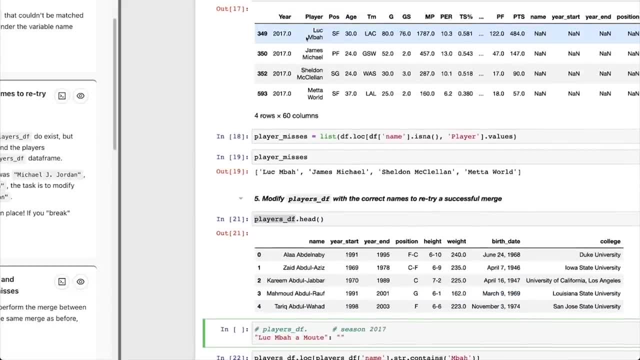 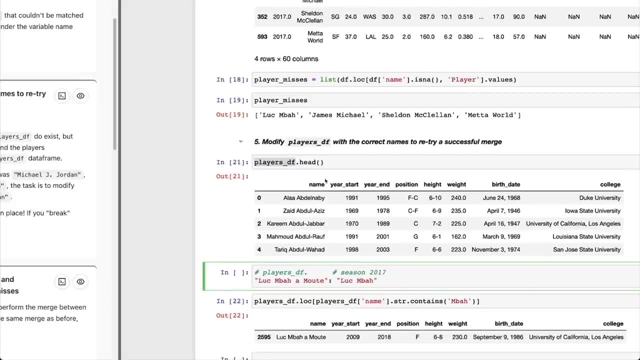 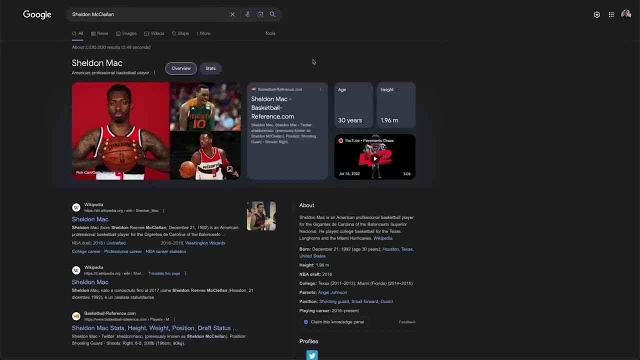 the name in 2017.. So we want that player to be that name And we can keep working, you know, with this detective work. Maybe you know what happened, for example, with: maybe you don't know this, but Muhammad Ali was born. 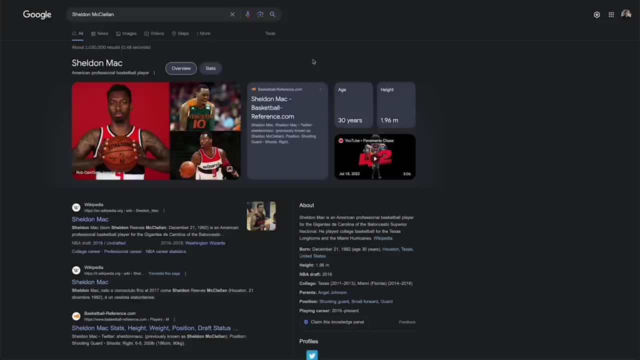 Ashish Clay, and then he switched religion, or I don't know how to say this, but basically he converted to Islam and he changed his name to Muhammad Ali. So the same thing can happen to anybody. We can change our names, and that's what happened here as well. So this person- 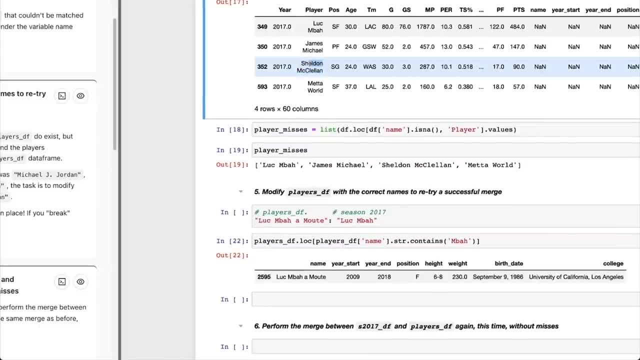 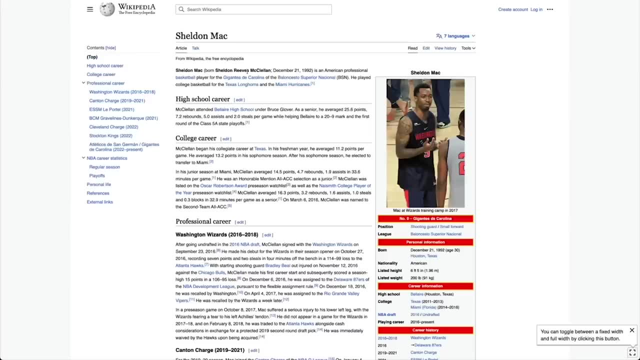 potentially goes by a surname. So, for example, Sheldon McLellan, which seems to be the original name- I can just go to Wikipedia- born Sheldon McLellan. Here he is right. So the guy either changed his name or just made it shorter. We don't. 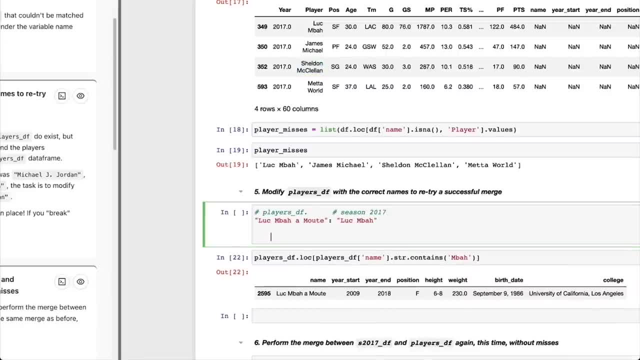 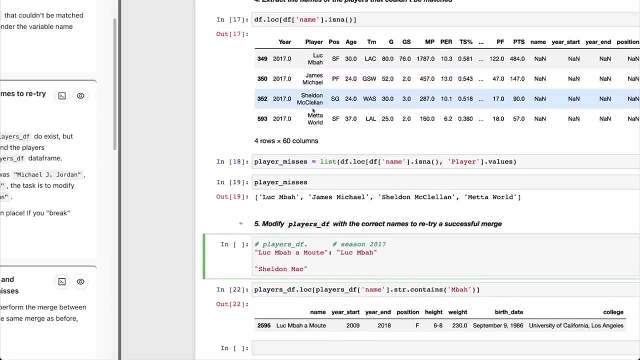 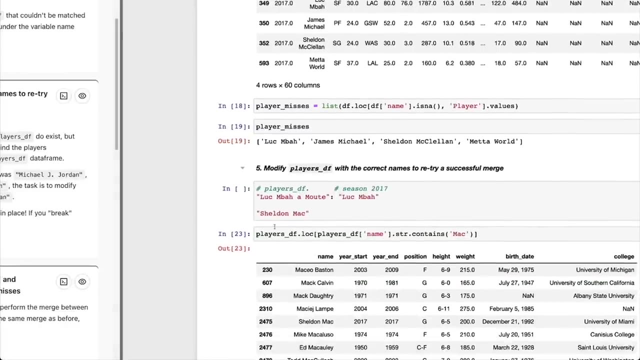 know, To be honest, we don't care. We have just found another player with a different name, So we're going to do that. So we know that in the let's actually do Mac here- No, Sheldon Mac, Where is? 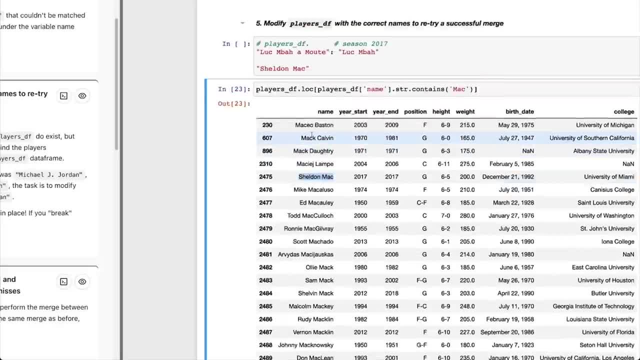 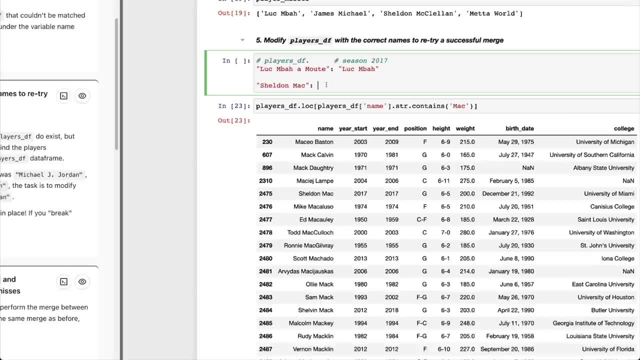 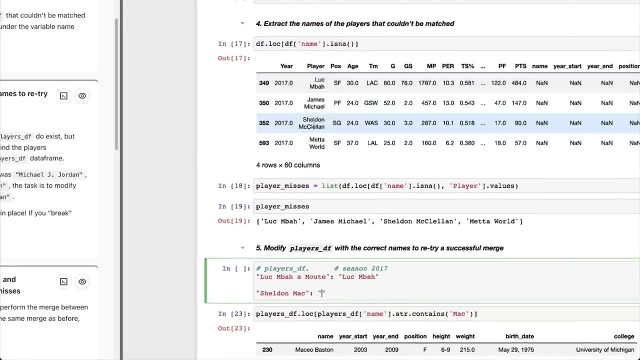 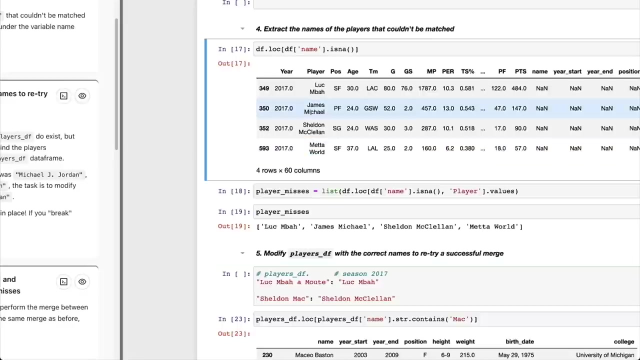 Sheldon Mac right here. So in playersdf we have Sheldon Mac and we want that player in the 2017 season. It's like, well, rewind it. It's like what was the name right in 2017? And that's the name. Who else? James, Michael- Let's take a look at Michael here. 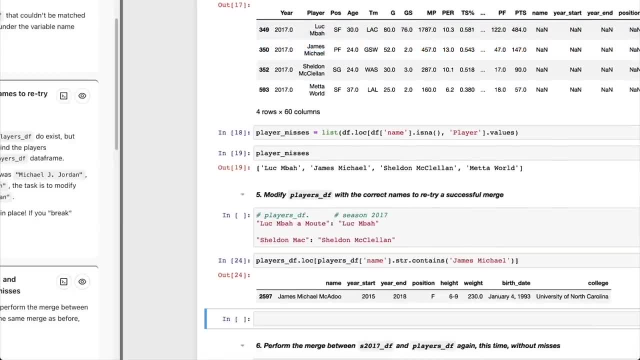 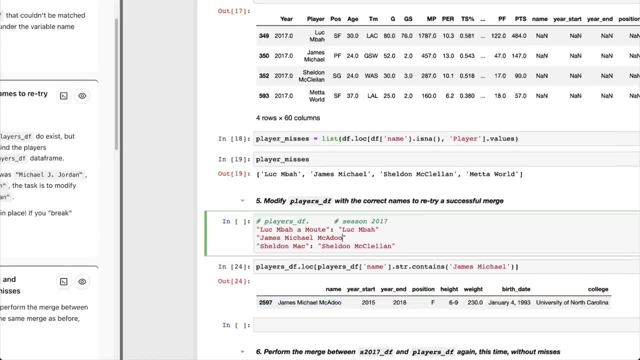 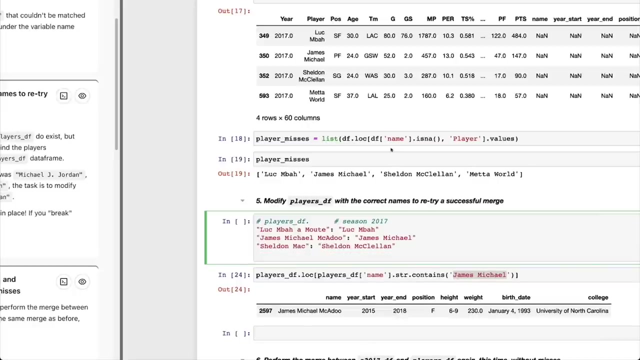 James Michael. Let's see if there is any changes. There is a new last name, So again in playersdf, this person is James Michael McAdoo and we want this person to be renamed. We are- it's like we are- rewinding the names to 2017.. And in at the end we have Meta World And 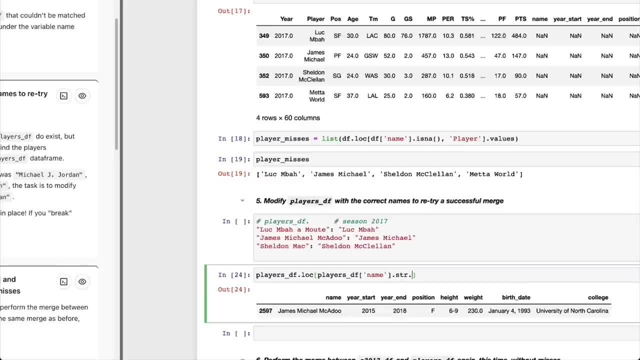 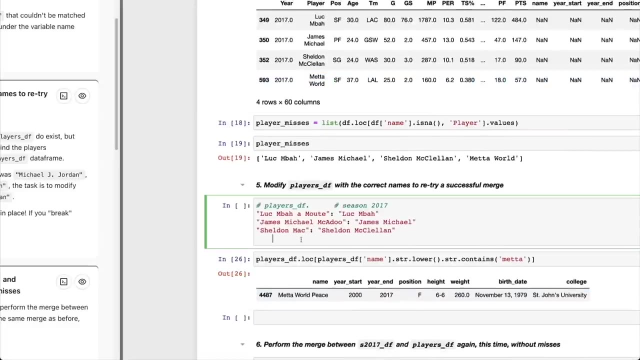 here I'm going to do another trick. Take a look at this. I'm going to first lower the names and then I'm going to do Meta Meta with a double T. There you go, And it seems like Meta World was the name in 2017, but now it's something different. So we're going. 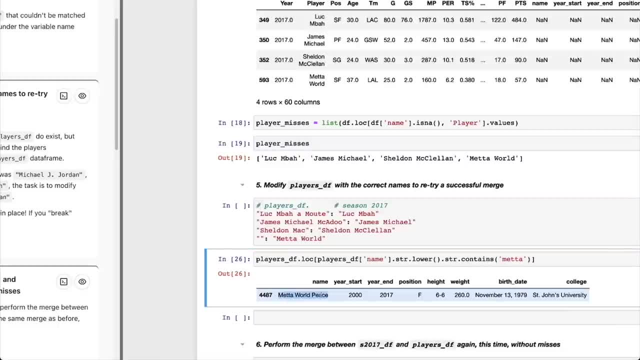 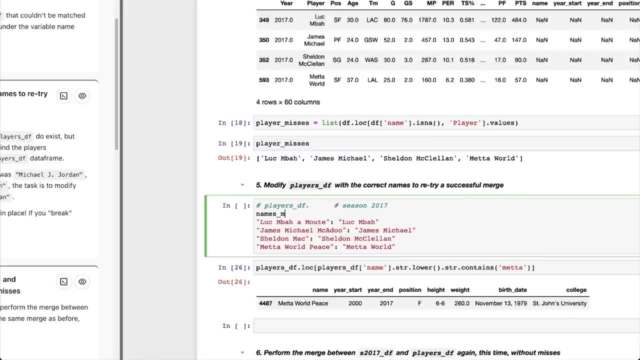 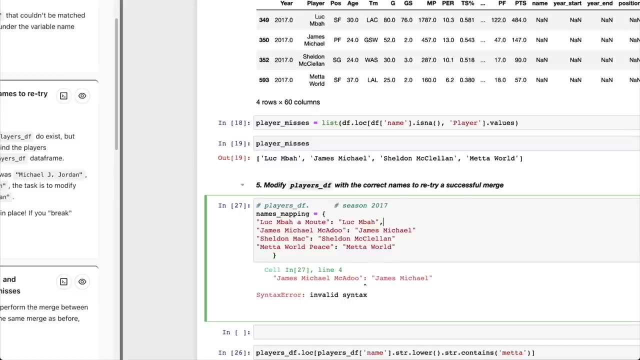 to rewind again, if you allow me the expression, to the old name in 2017.. We can store this in names mapping- There you go, There you go- So we can keep the names as a reminder. And, of course, I'm missing the. 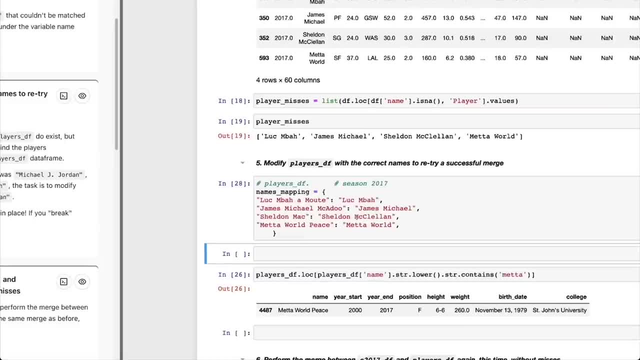 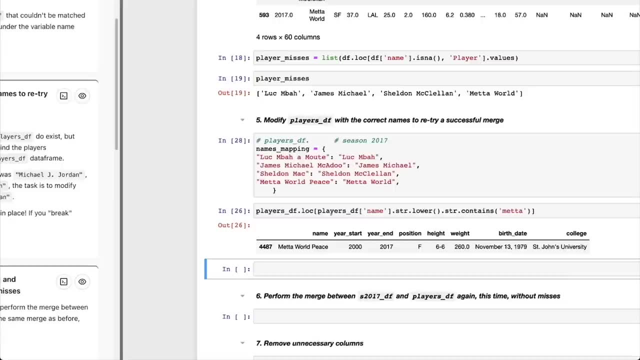 comments as usual, As we were doing. So how are we going to do this thing? Well, the way to do it is just: we're going to find a player. In this case, we're going to find a player with the same name. So, in this case, let's do it with the I don't know. first one, First: 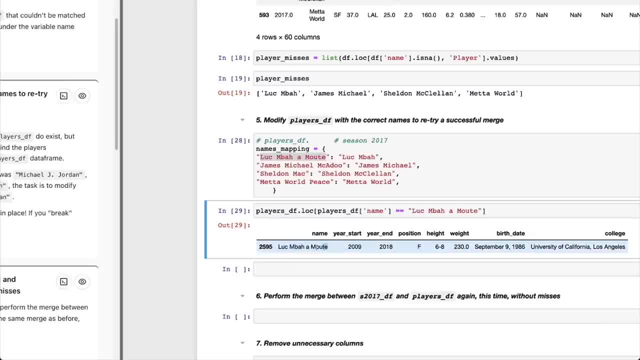 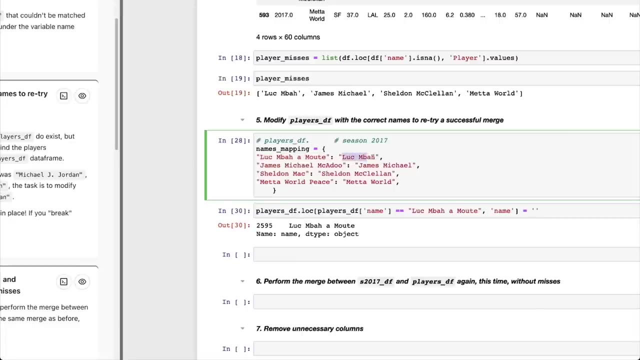 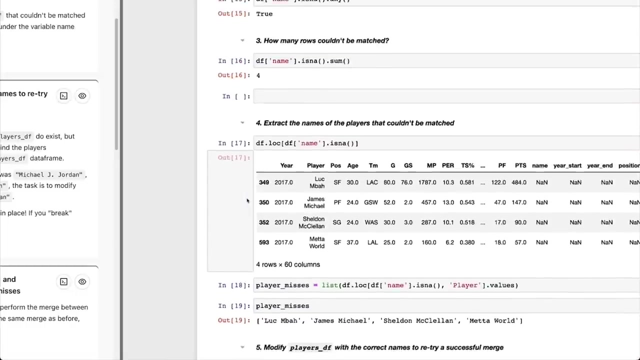 name And then player CF with the full name. We want to rewind that player back to the name in 2017.. And we want to take just name, right Name, And we want to assign that to the name in 2017.. So we can change that. There you go. If we do the merge, let's go ahead really. 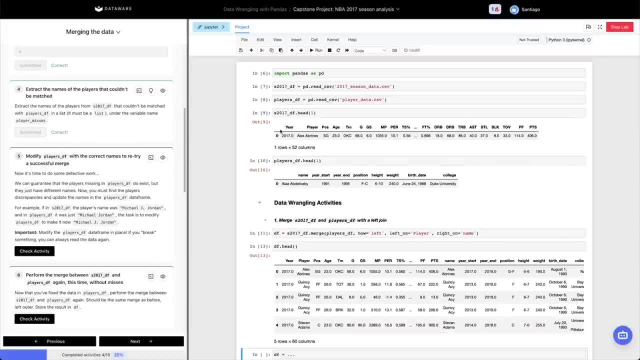 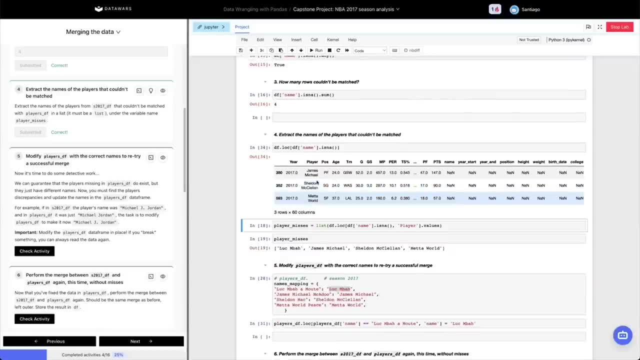 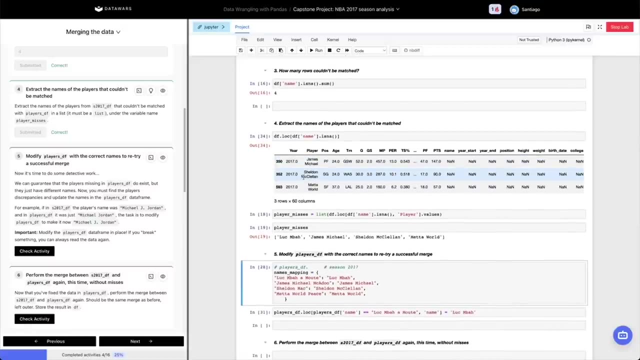 quickly- I'm going to zoom out. Let's do the merge once again really quickly And let's find the players don't match which, as you can see, it's just three, because we fixed the first one. So this works. What we can do now is we have four, but we can just 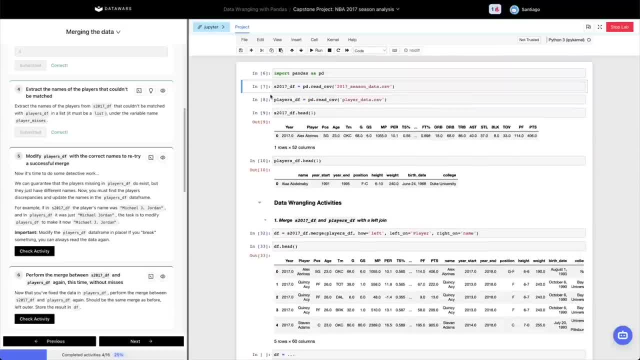 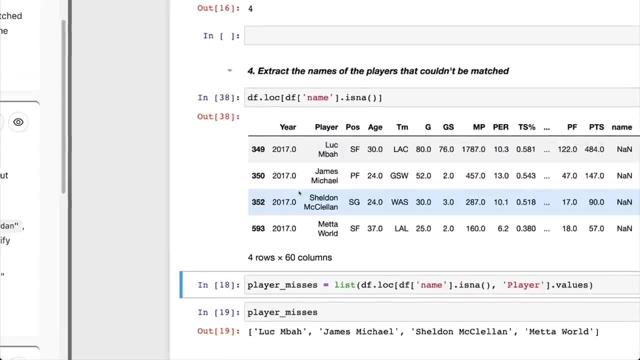 automate quote, unquote this process. Let me reread players, because I have modified players. Let's do the merge again. Let's go back to the state where we have these four players missing, including Luke Mba, And now we're going to do this same process, but we're going. 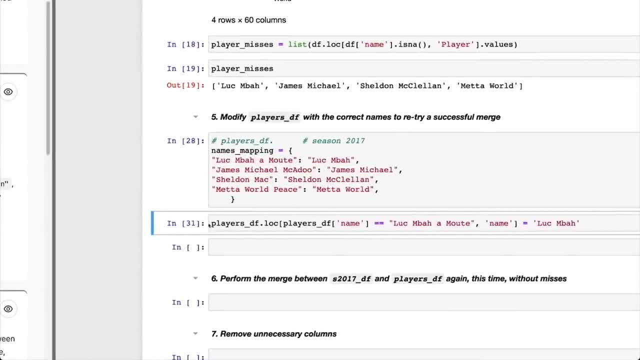 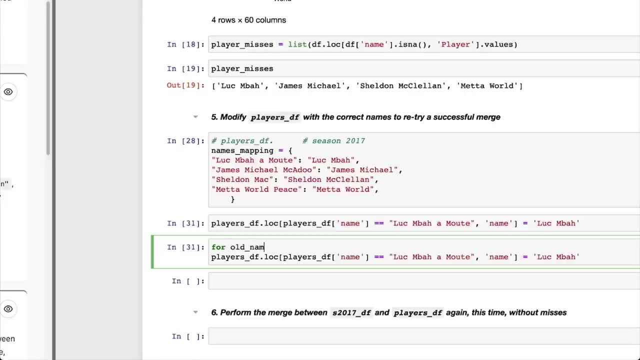 to automate it. We're going to use for loop, so we don't have to type it one by one, And the way to do that is going to do for old name or it's actually like new name, let's say, and name 2017.. So it's the new name and the name they had in 2017.. In names mapping, 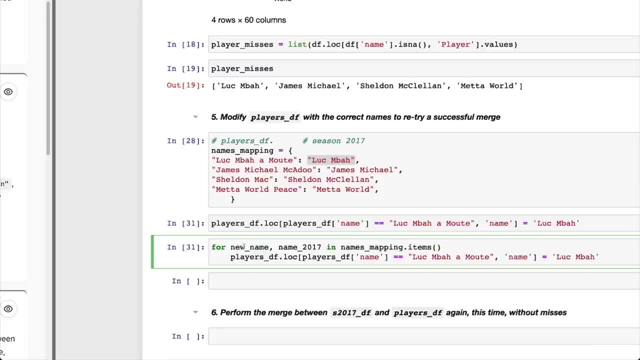 dot items. we're going to find the person. We're going to find the person with the new name And we're going to replace it with the name 2017, Bali, And of course, I'm missing now a colon. And there you go. We can now try. we can check the activity to see if we 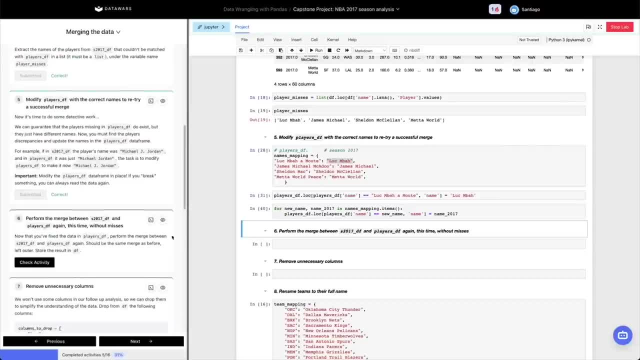 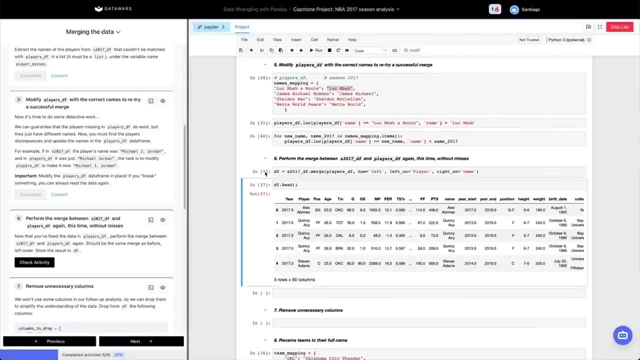 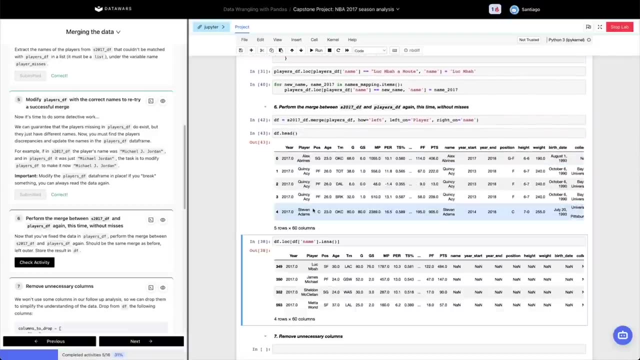 did everything correctly. It seems like it works. We can now perform the same merge again and see how it goes. Just let's take a look. So I copy these cells: same merge And we're done, And we we know what the activity is going to check, but we can borrow this cell. 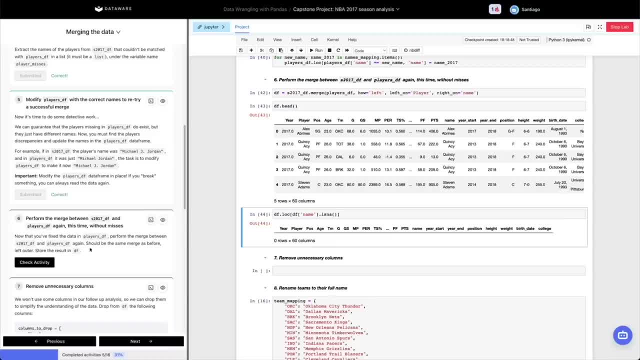 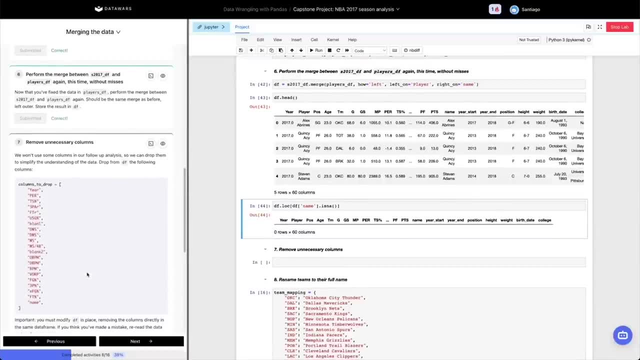 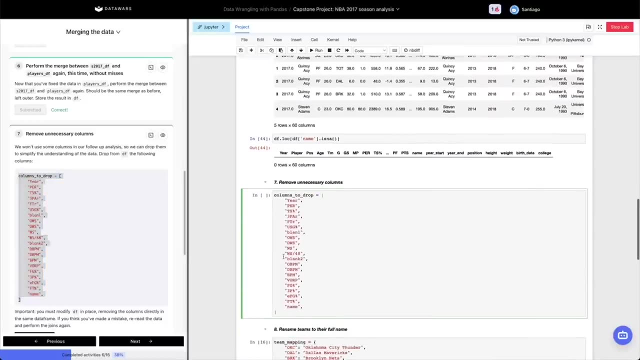 and try it again and see if we had any misses. No misses, So this will potentially. there you go. It worked as expected. Okay, remove unnecessary columns. is just again data wrangling very boring, just you know. we have to get rid of a few columns, as I show you The first. 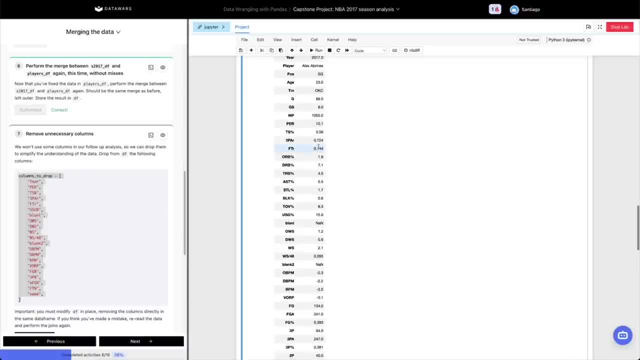 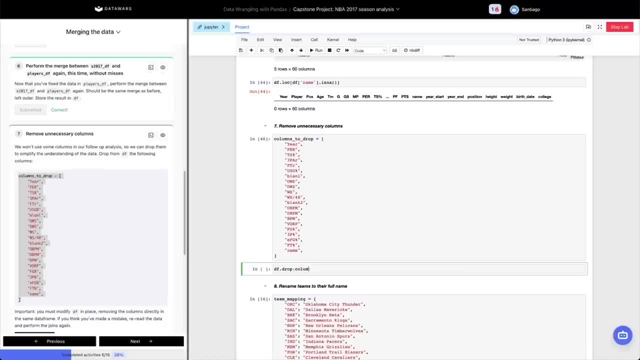 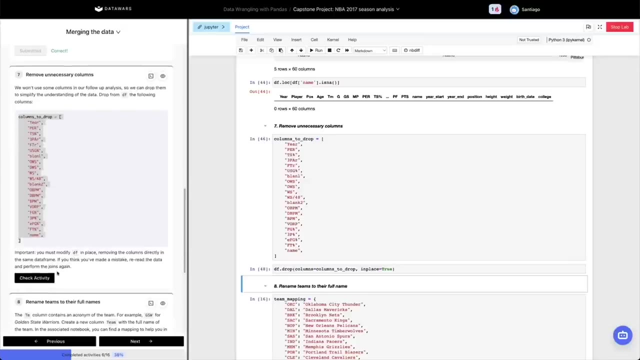 row is: there are a ton of columns we're not going to be using, So what we can do is just drop these columns. how to drop the f dot drop is the method columns. columns to drop in place equals true, because we want to modify data frame. Now we're going to check the activity. 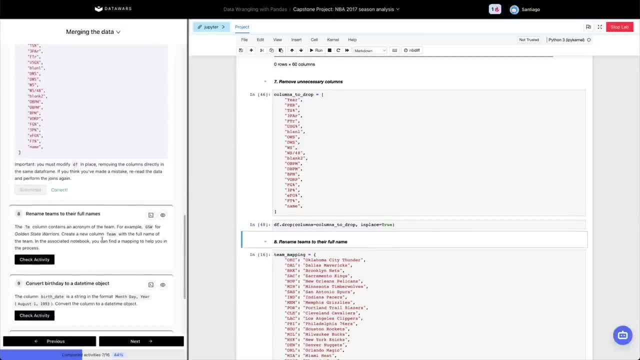 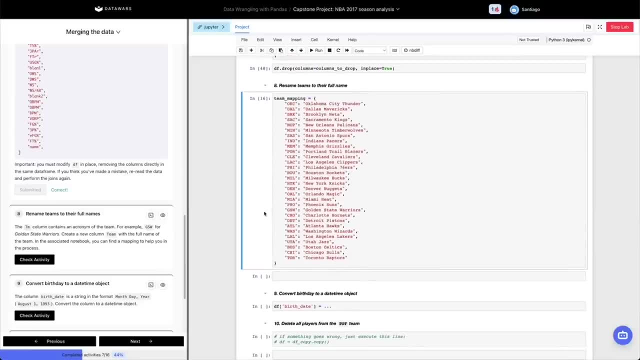 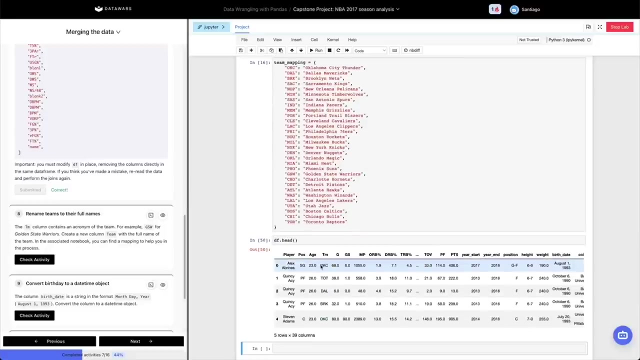 And it works. Rename teams to their four names. This is a very interesting one because it has a very simple solution, But it's usually not expected. I see some some very crazy solutions for this sort of activities that involve renaming. Basically, we have the team of the player is a three letter acronym we want to resort back to. 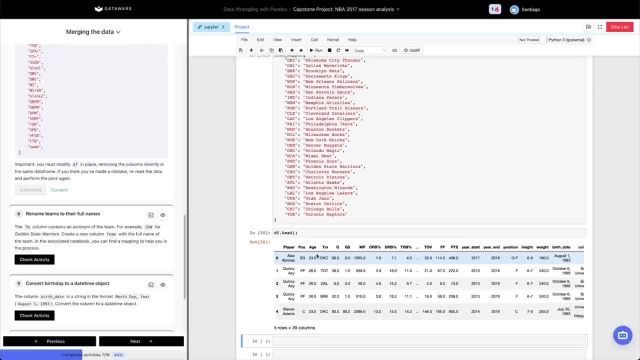 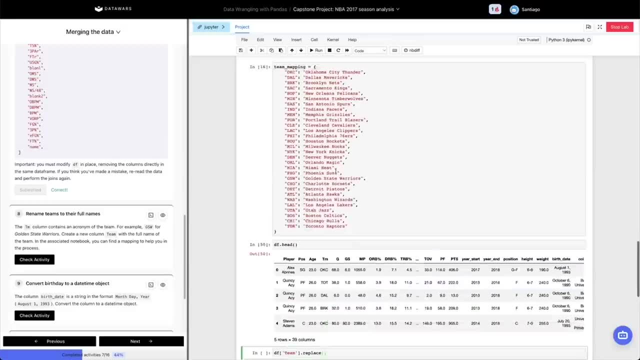 the full name of the team To do so. what we can do is the replace methods. we can do df at team, dot replace, and we can use this mapping that was given for the name And we're gonna add there. Now let's do something like a: j: The name of this is the name of the player. 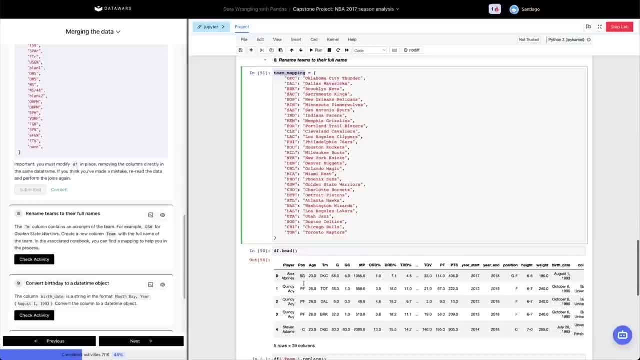 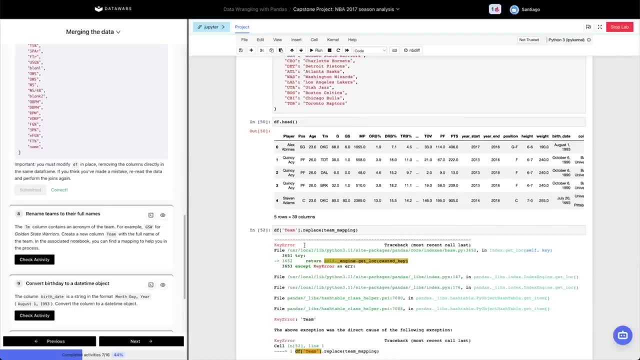 And then we're gonna call the player by name or the same name as the name of the player for us team mapping there. and you can, I will just execute this thing and it didn't work because it's actually team that I go TM. so we're replacing one by 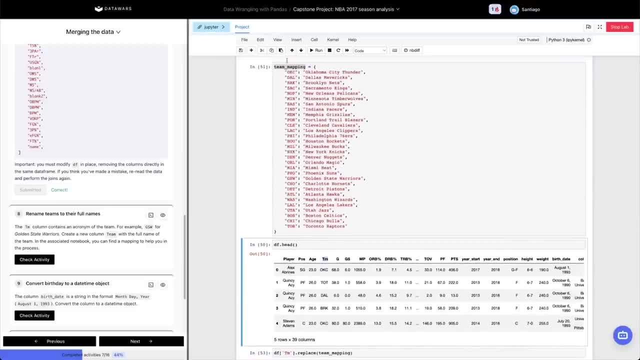 one these acronyms whenever you have- okay, see, it's gonna find here. okay, see, it's gonna replace with Oklahoma City Thunder- we're gonna find, for example, D al. it's gonna look for Dallas. where is it? I don't know where it is. basically, where is that? let that last second one. so basically it's gonna it's, it's just a. 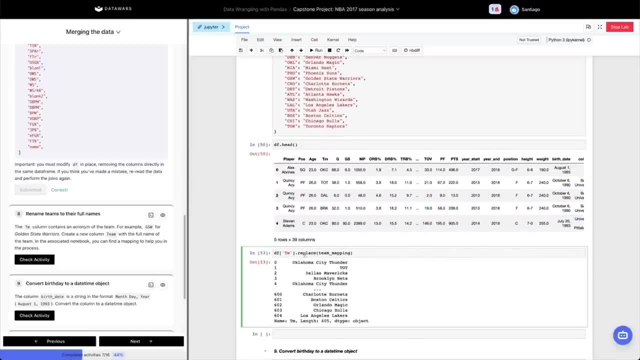 mapping and it replaces one by one, and we can sort this result right in the column team. that's gonna be it. so we're gonna do a DM, the effort team, which is the full name. it's gonna be this column with a replace mapping performed. and now 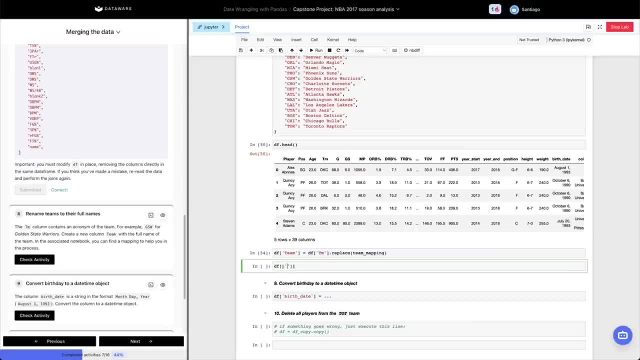 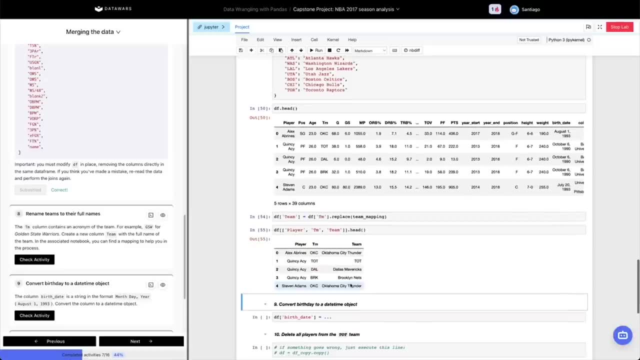 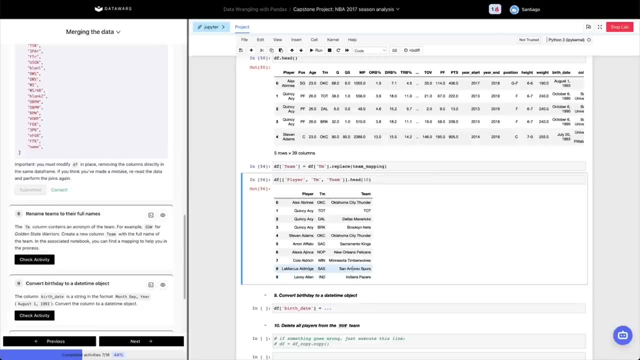 we can do the F. let's do the F at player TM and team. let's get the first 10 rows and we're gonna find 10 rows and I find a few things. so IND, Indiana Pacers, SAS, San Antonio Spurs, MIN, Minnesota Timberwolves. so this looks okay and see. 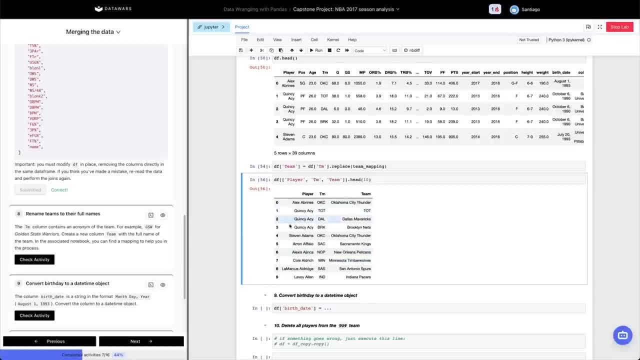 what happens here with this TOT in a second, but for now this is good and let's check that out and see what happens here with this TOT in a second. but for now this is good and let's check the activity to see if we did the correct thing. and there you go, it's working. 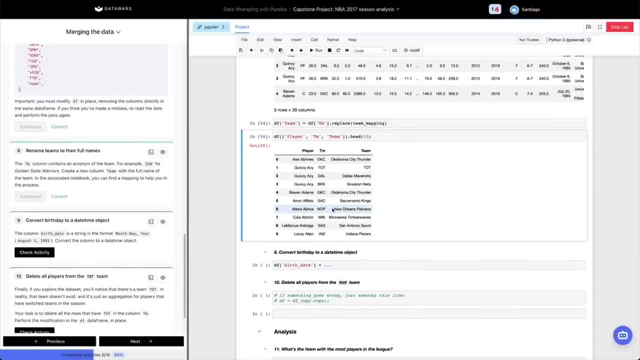 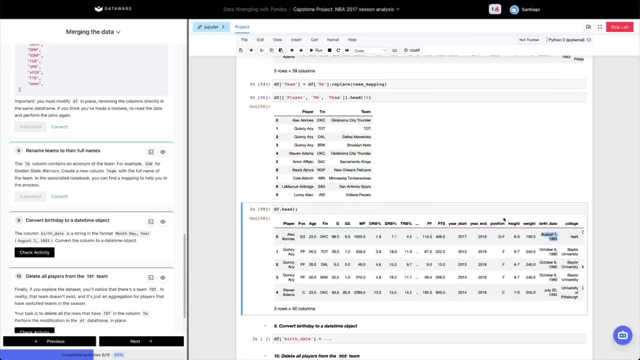 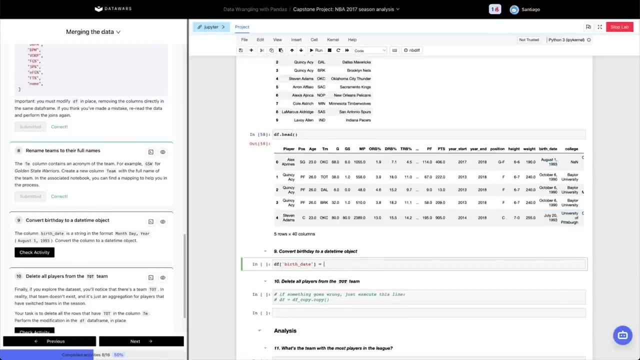 convert birthday to a daytime object. so this is another interesting one. the birthday of the player is a string. when they convert that to a day, a to it to a timestamp or daytime, it's very simple in pandas book. we're going to do is PD to daytime and we're gonna pass directly. 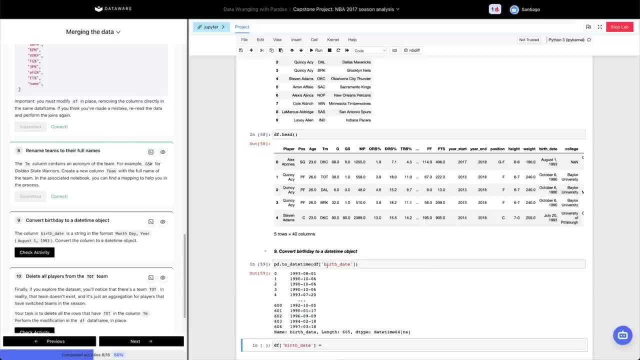 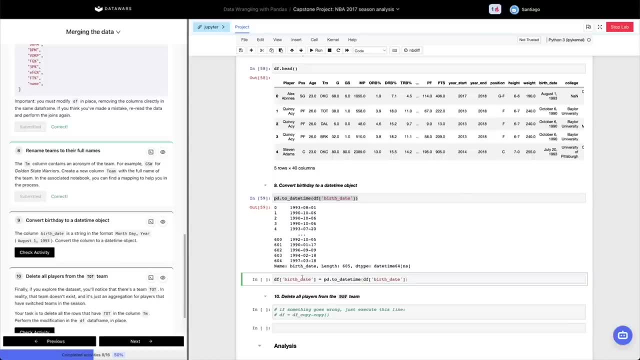 you birthdate column, that's. but of course this is an immutable operation. that's just returning a new series. what we want to do is just step over whatever value we had before, and of course this is a change we cannot undo so easily. so in this case we are safe to just- oh like, step over the. 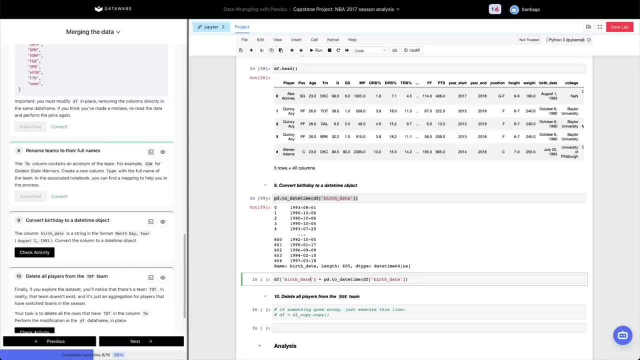 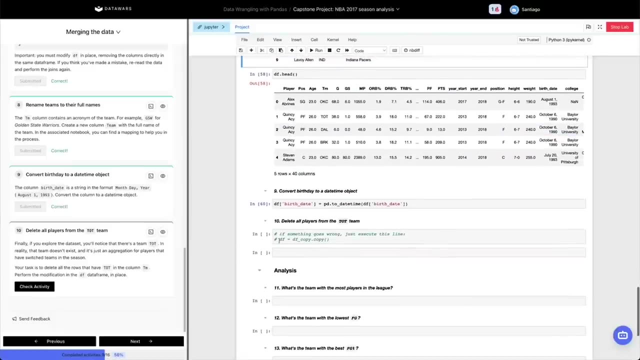 previous values. if not, you can just create a new column. you know, in this case we're safe. we can just convert the column back to daytime, we can check the activity and that worked as well. so, going back again to the previous values that i show you we had- let me borrow this thing here: 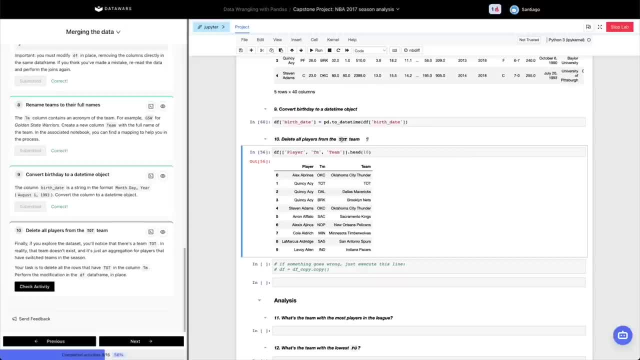 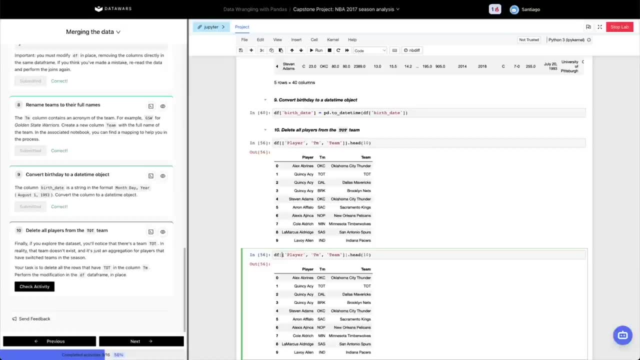 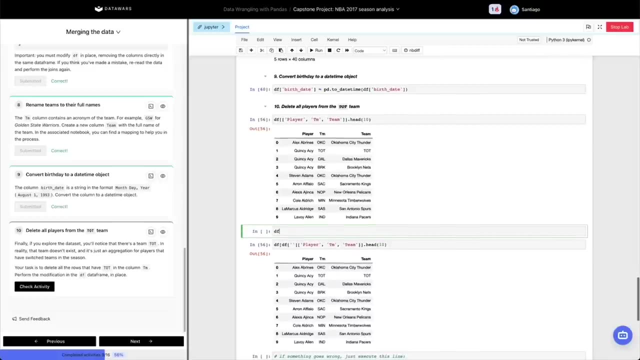 delete all players from the tot team. the tot is for the players and that's actually. let's do something. um. df at at. let's, let's, let's, let's, Let's. look for duplicate players. dflog, df at playerduplicated. Yes, and we're going to find we're going to duplicate it. 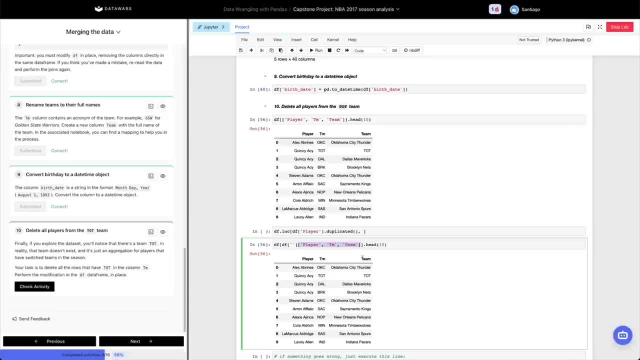 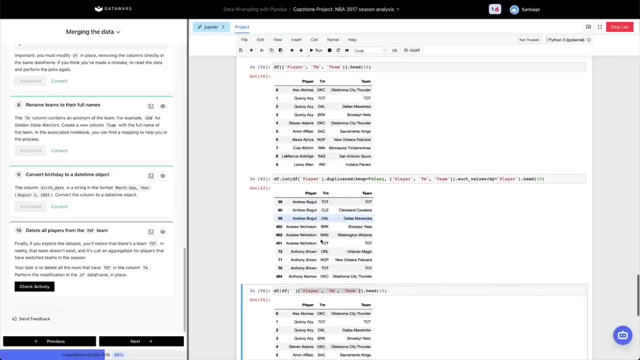 I want to now here. only these columns keep false. Yes, sort values. This is a long operation, but don't worry, it's pretty simple. Sort values by playertet. There you go. long operation, Some players in a given season can switch teams right. 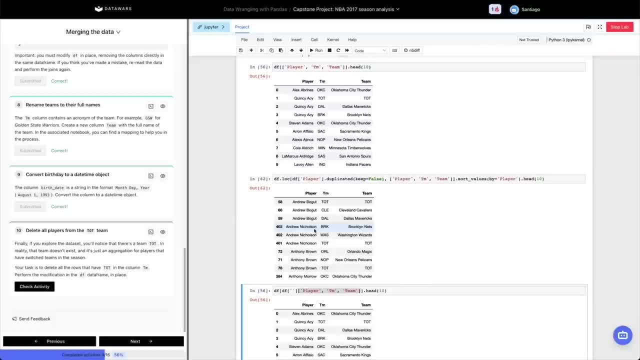 Just right in between there is a transfer window and they can switch teams, So you have the first, the same players. sorry, like this guy right here that play for both Cleveland And Dallas right in the same season. He was transferred in the middle of the season. 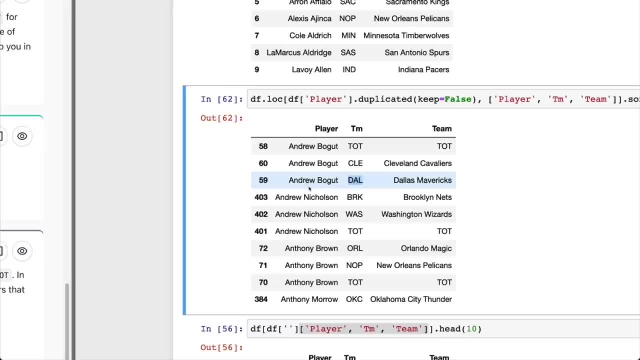 So this data that we have and we have to understand again, the data that we have includes kind of an aggregation column, which is the TOT column for totals. So totals of this person within the whole season is so many field goals. 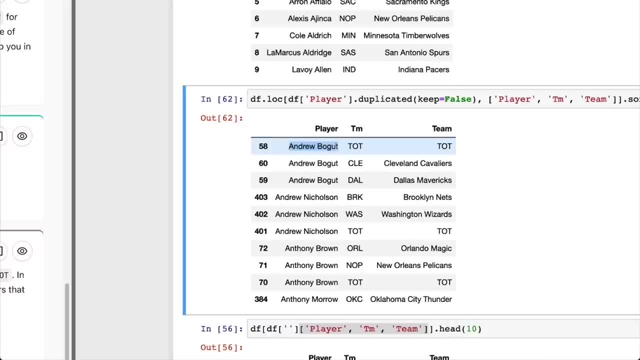 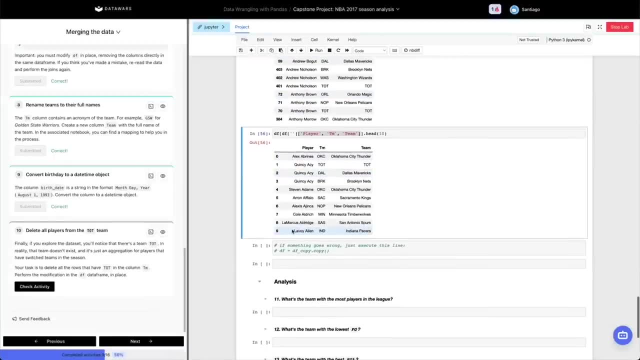 so many three-pointers, so many free throws, et cetera. Just a total, an aggregation of the season for this particular player. We need to get rid of that. so I'm going to do that. Oh, actually, we can use the same. no, we can't use the same condition. 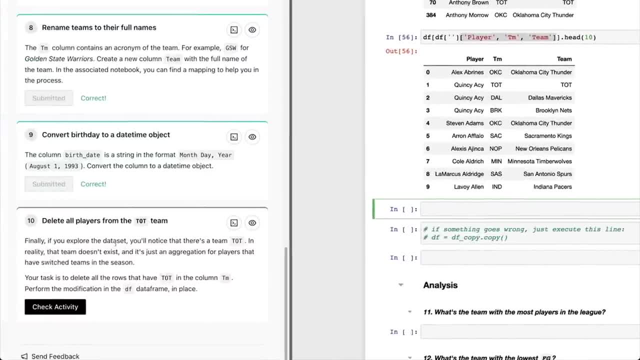 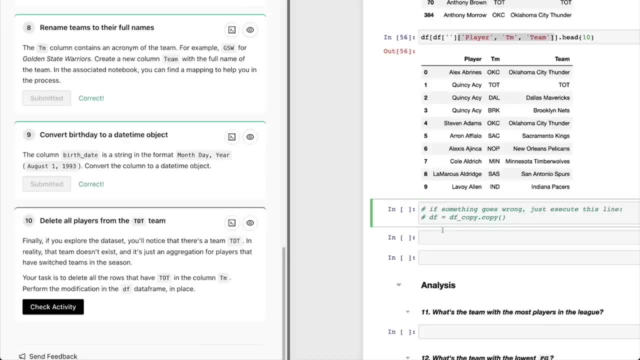 How are we going to get rid of these values? First, let's keep a copy, because I mean we're going to be breaking things, So we need to keep a copy. We're going to do a dfcopy, dfcopy. 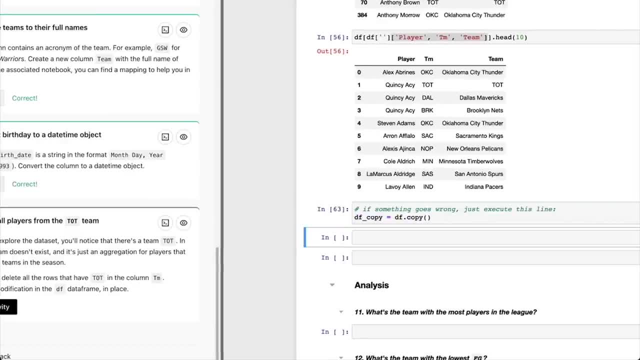 This is a very common technique. We're going to do a dfcopy. This is a very common technique. when you're modifying something, As usual, I encourage you not to modify things, but if you are certain you want to get rid of something, 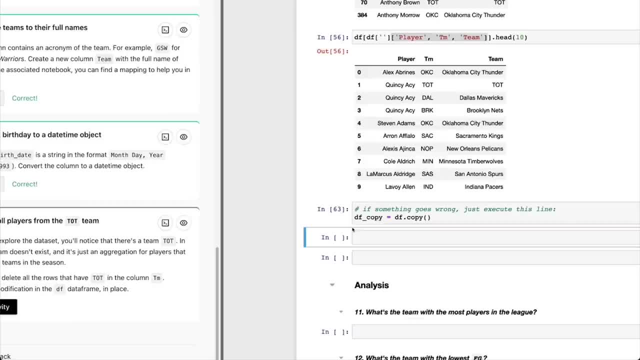 you can. while you're doing the process of understanding and analysis and all that, you can create a quick copy of your data if it's not large enough to fill the whole memory, of course, because you're literally copying values. So if your data frame takes one gigabyte of memory, 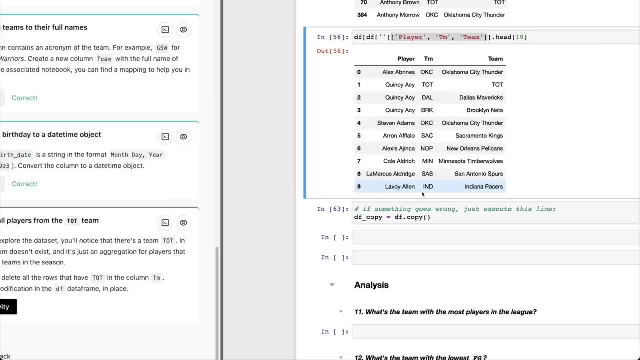 once you duplicate it. now you have. you have two gigabytes of memory allocated, So as long as that's possible, you can keep a copy, And I usually do like copy one, two, three, four, five and that's pretty much the data wrangling process. 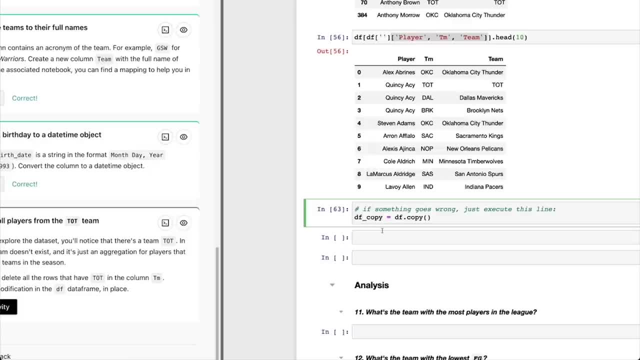 Until you figure things out and you're sure, then you can remove all the copies and, of course, automate the work. But for now we keep a copy If anything goes wrong. let me comment this thing out so we don't accidentally execute it. 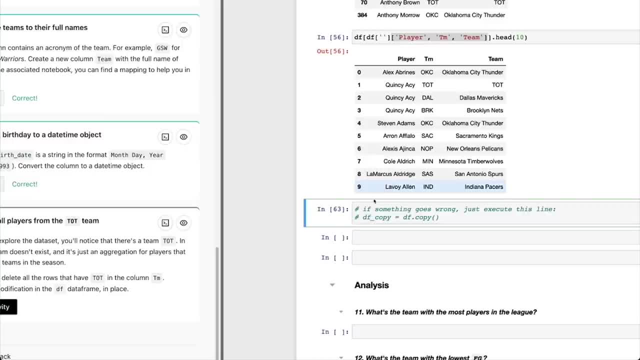 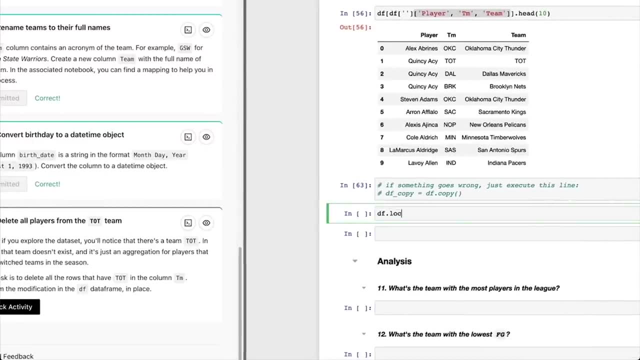 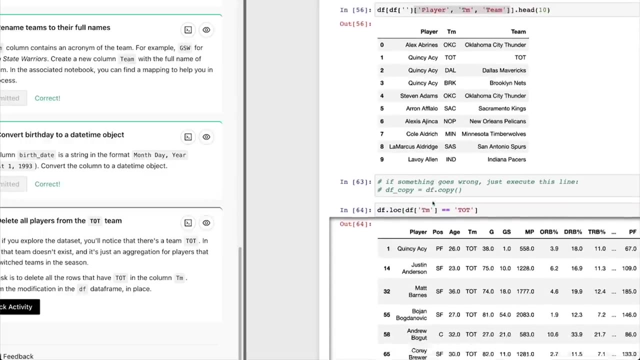 We have a copy in dfcopy. We have a copy in dfcopy. Go back to the activity. We have to get rid of the players that have a TOT team. So dflock, dfteam is equals TOT. All these players, we have to get rid of them. 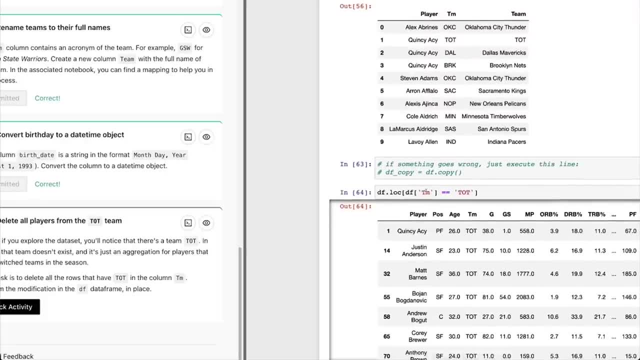 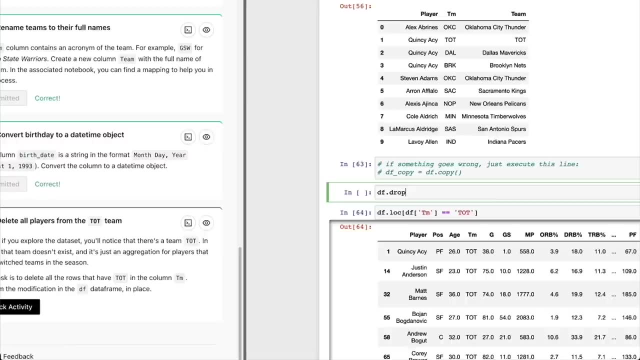 How can we get rid of them? There are multiple ways. The easiest is probably also with drop. Maybe not the easiest, because the easiest could be to just do something like df equals df equals all the players that don't have a TOT. 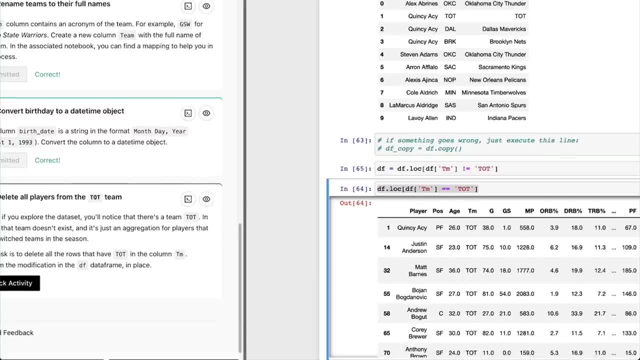 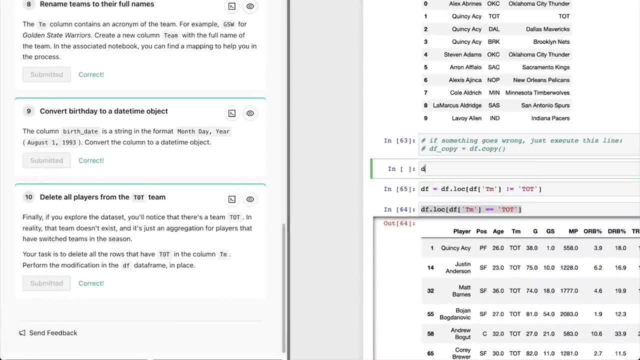 And actually let's try it out, And this should work for both, except I'm doing something wrong. It worked, But let's bring back the old data frame dfcopy copy. There it goes, so we have it as it was before. I'm going to delete the cell so I don't accidentally execute it. And there is another way, which is basically we can find all these rows right, So all the rows we want to get rid of, and we can get the indices. 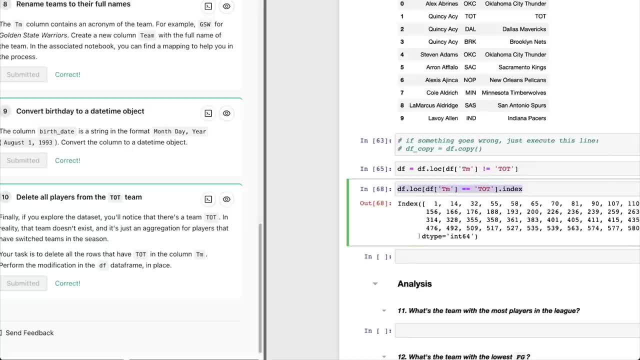 So the index of the rows we want to get rid of, And finally, we can use the drop method. So we want to get rid of these values and we can do in place, true, And let's see if that works as well. 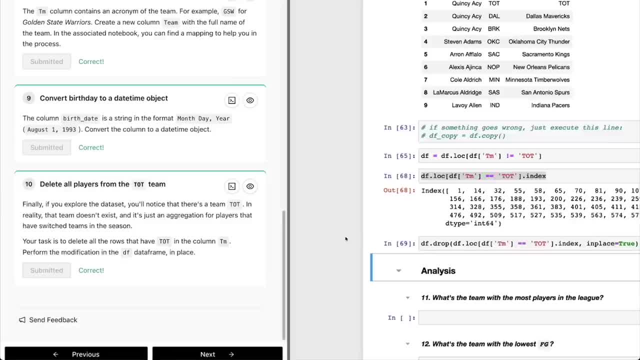 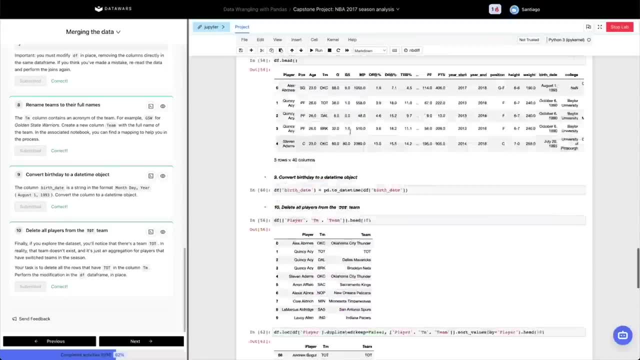 Well, I have to reset all the activities, but trust me, that's also going to work. It did serve some purpose. There is no way to catch the red axis, so we don't want to do it. All right, we have pretty much the whole process done. 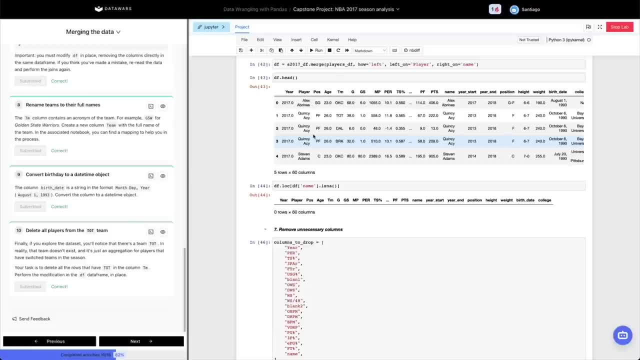 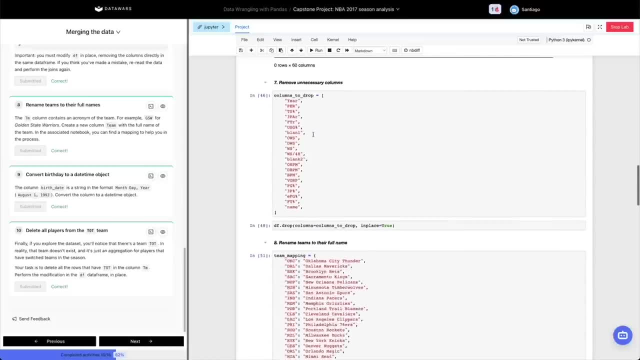 We merged the data frame. We found that there were a few mismatches where the names of the players changed, So we rolled them back to 2017, doing some investigation work, some detective work. We brought back to 2017, merged the data. 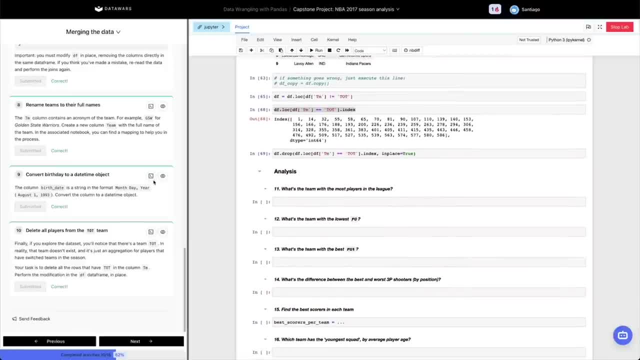 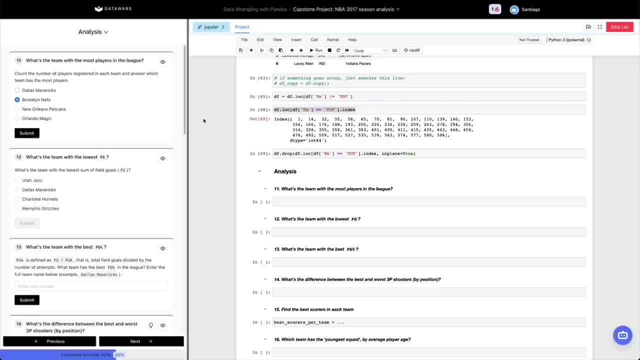 a little bit more cleaning, removing tot and all that, and now we're going to actually start with the analysis. so this is going to be very interesting. so, um, what's the team with the most players in the league? so we have again. so we have um information about all these players. they work. all these um players in the 2017 season and, of course, we know that some players switch teams, right. so how many, uh, what team had the most players within a season? either? if they went back and forth, they changed a lot- want to answer how many. which was the team with the most players? 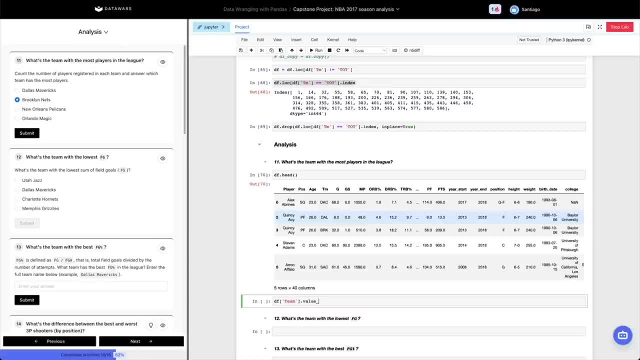 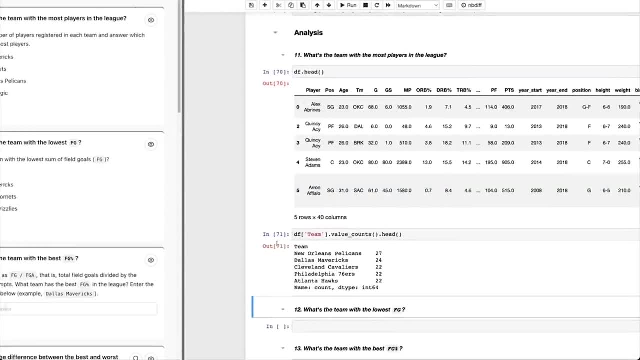 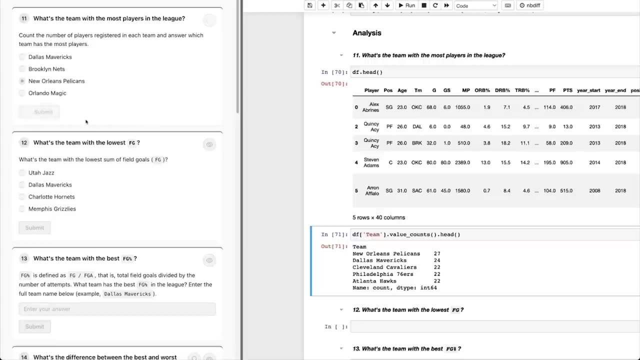 in a given season. that's pretty simple because we can just do a value, counts, counts and that's to head, and it's gonna tell us that the new orleans pelicans was the team with the most players to 27 in general register players and that's correct. 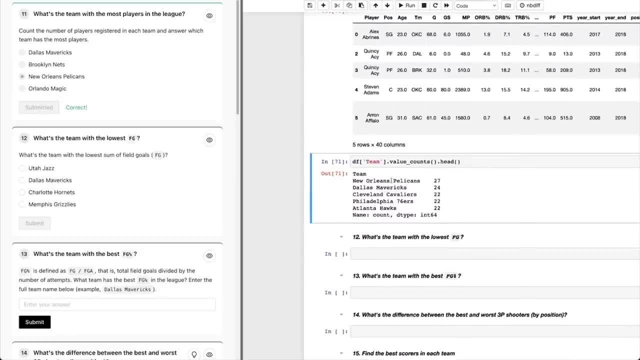 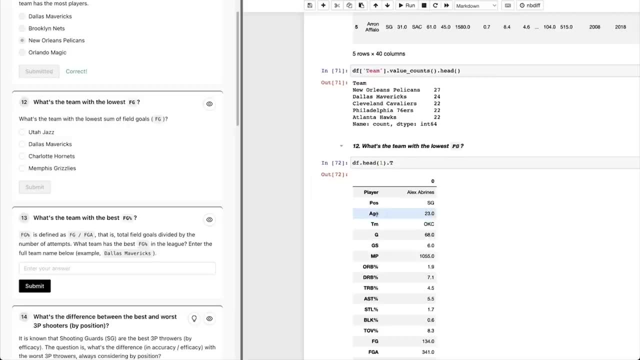 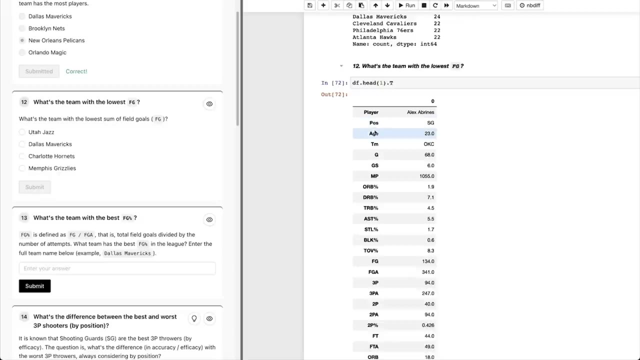 so what's the team with the lowest field goals? um, let's take a look at the data again so you understand what we're trying to do here. for each player, for each row, so each row is a player in the 2017 season. we have merged that with our personal information, which we don't need in this activity. 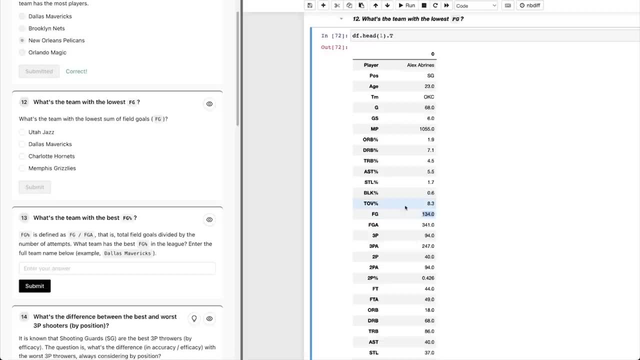 but basically we have field goals that the players scored in that given season. so we want to aggregate all the field goals of a given team, of all their players, and find the one with the lowest value for that to do. so we're gonna. we're gonna, group by team, team. 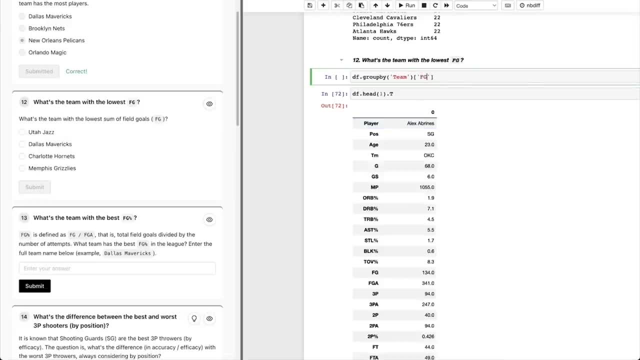 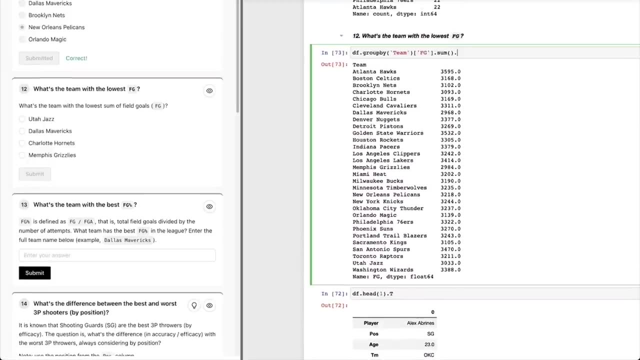 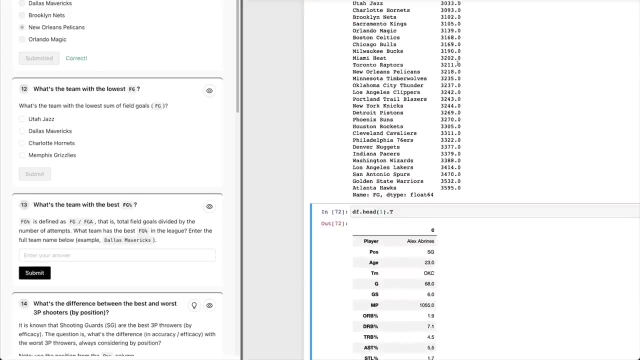 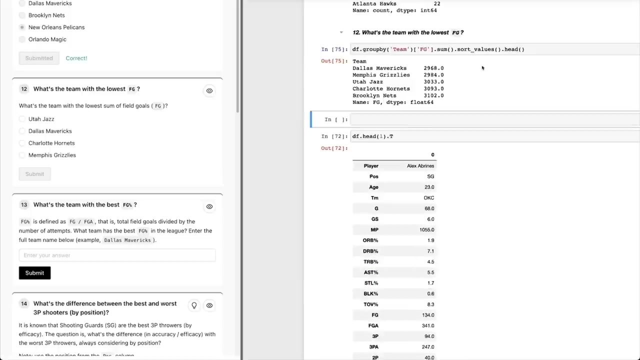 and we're gonna find the field goal column and we're gonna sum that column. of course this is a mess. so basically we're gonna do sort values by sort values by nothing, because just a series and it's gonna be ascending. we can actually do a head method here. i wanna dots so it doesn't switch. 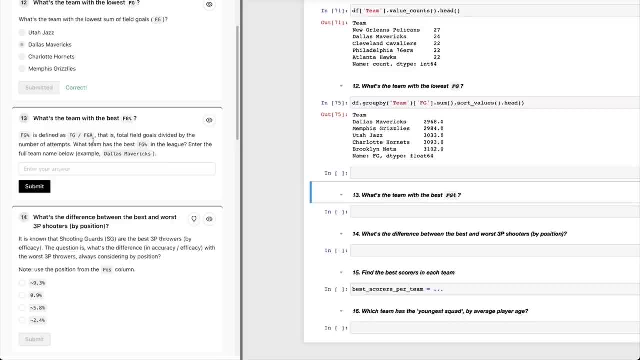 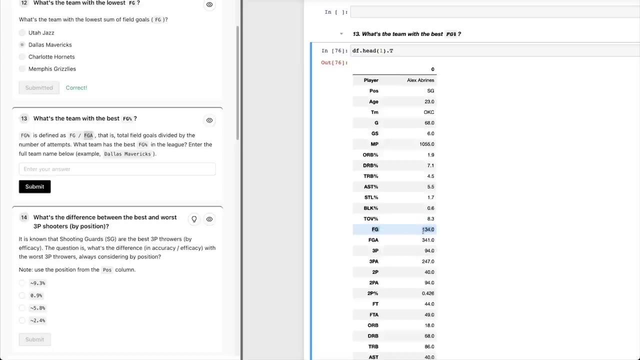 percentage, and this is a very interesting one, because field goal percentage is defined as field goals divided by field goals attempt. that is data we actually have here, so we're gonna put in a we have. let me show you again the values. so we have. we have field goals 134 over 341 attempts. so 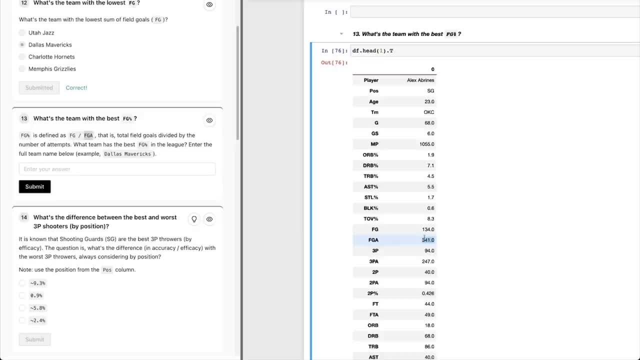 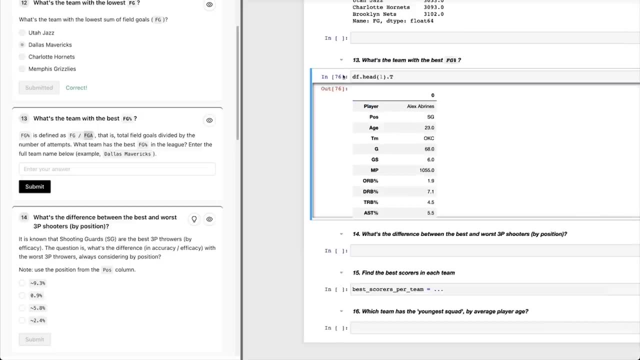 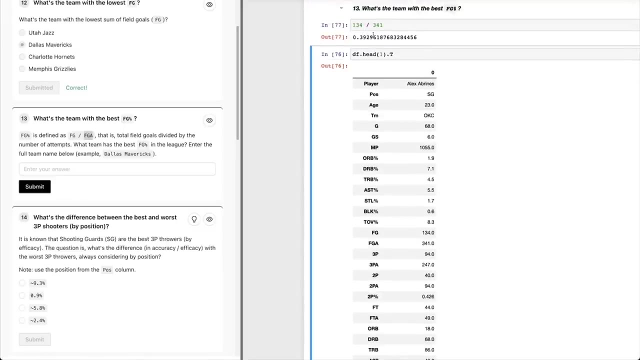 it's a little bit less than 50 percent, right you? you tried 341 times to score and you only made 134. so you made, you made 134 divided by 341. your accuracy to put it away was 0.39 or 39 percent. so that's the column that we want to compute, that's. 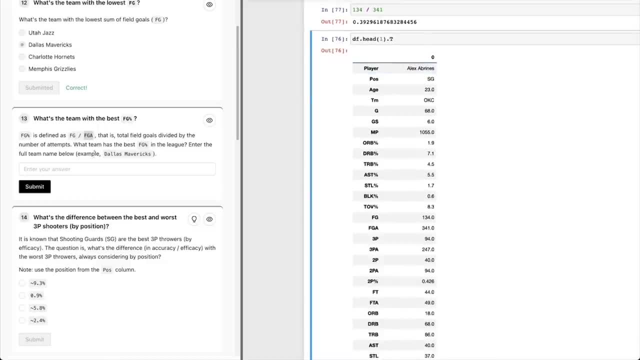 the value we want. i can, we want to compute, but we want to compute this by team. so we have to aggregate all the field goals and all the field goal attempts from a team and then find that given percentage. so we can start by doing pretty much the same thing we did before. it's going to be df. 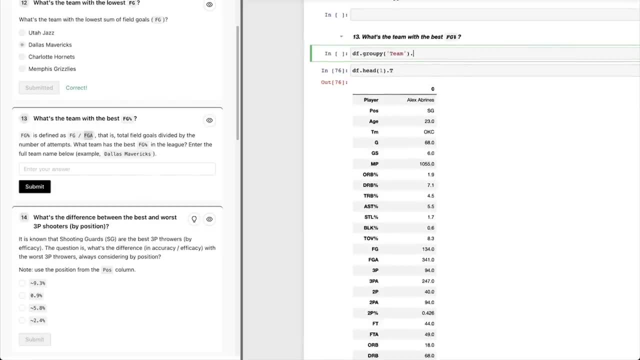 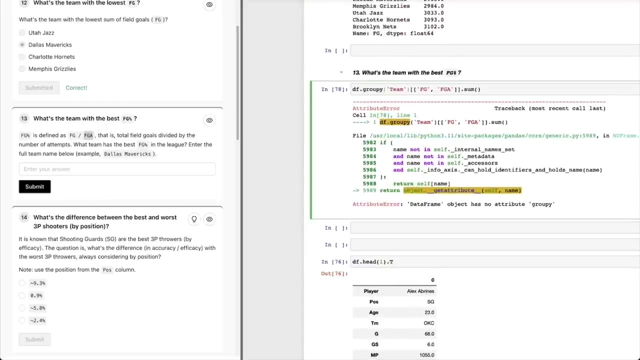 bro, group by team. and here we're going to compute two values. we're going to compute field goals and field goal attempts, and we're going to do some of these two and this method doesn't exist because i mistyped, mistyped it. group by there we go. we gotta find this thing. so we can, we can. 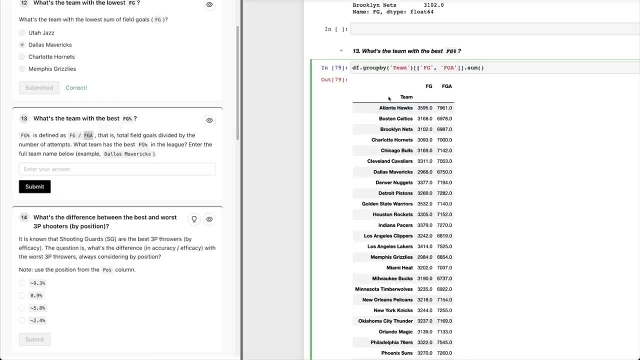 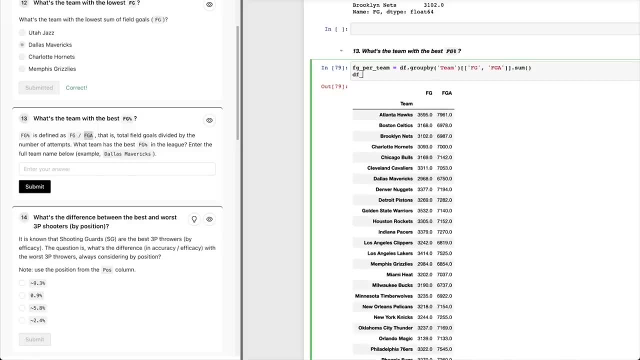 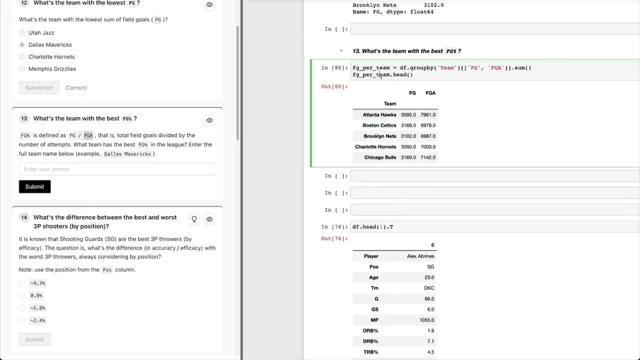 store this, this data frame, in a partial variable saying: uh, field goals per team and field goal, field goal per team. we're going to pre-visualize it and now we can compute a new column which is going to be: uh, it's going to be field goal percentage, which is equals to field. 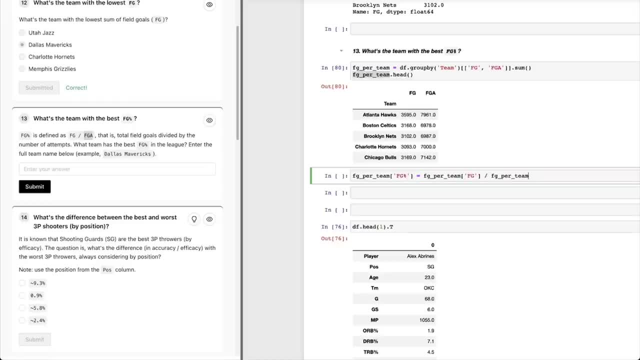 goal per team of fg, divided fga. and now what we can do is sort values by uh, field goal percentage, percentage head- and we're gonna find that's with the best. so we need to do ascending, ascending Falls, so the best field goal percentage is Golden State. Warriors. let's try the activity first. let's find 2017 season NBA. who was the champion play of Western champions finals champions, Golden State Warriors. so it's not it's it's not a triviality that the the player with the team with the best, with the best percentage, won the championship. anyway, let's take a. 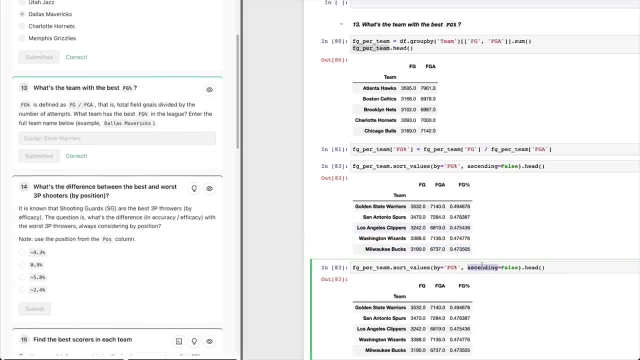 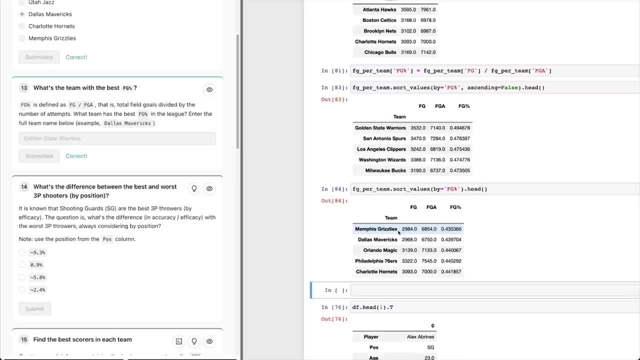 look at the one with the worst. or you know the the lowest, which it's not us, but just for the. so let's take a look at the one with the worst. or you know the the lowest, which it's not us, but just for the sake of of curiosity, we can find that Memphis Grizzlies the last Mavericks. 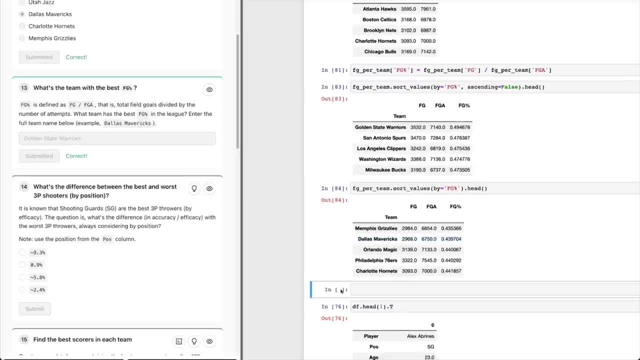 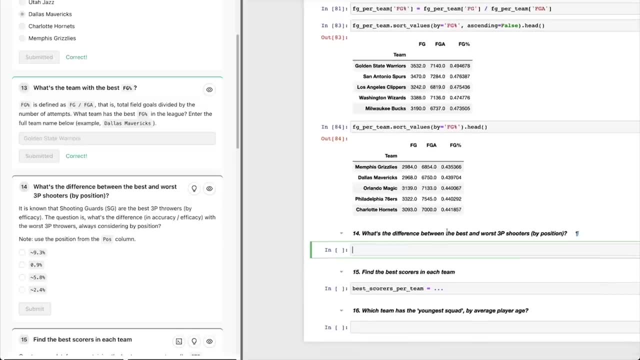 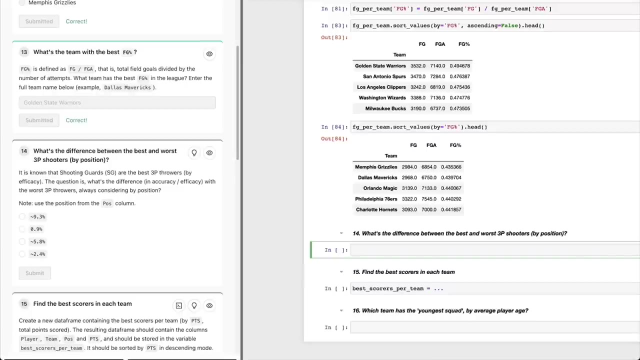 those were the teams with the least accuracy, to put it in a way. okay, so what's the difference between the best and worst 3p shooters by position? it is known that shooting guards are the best 3p throwers- three-pointer throwers- by efficacy or accuracy. the question is: what's the difference between the best and worst 3p shooters by position? it is known that shooting guards are the best three-pointer throwers by efficacy or accuracy. the question 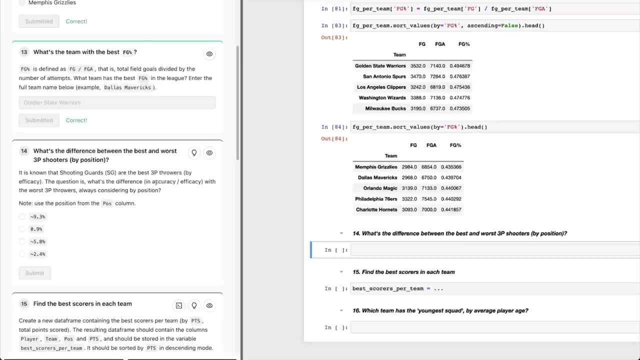 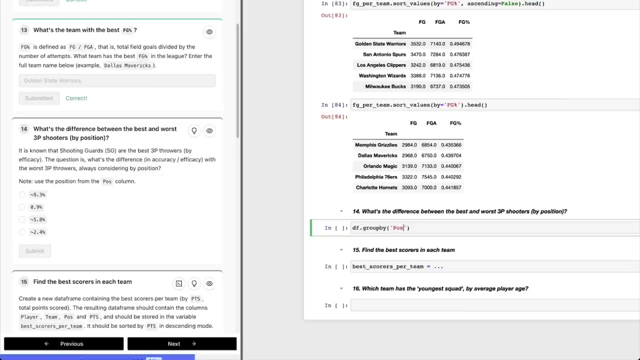 is what's the difference in accuracy with the worst 3p throwers? always considering by position. you note, use the position from POS column. so we're gonna group by position now and we're gonna compute both three pointers and three pointers attempts. I'm gonna sum all this and this is pretty much the same thing. 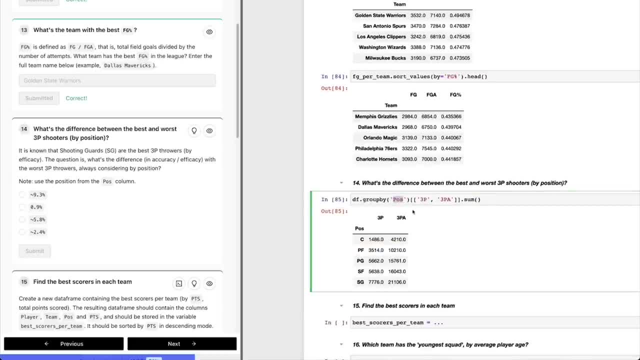 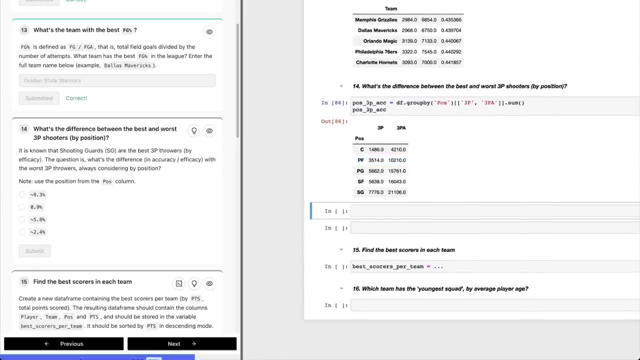 we did with the previous one, but in this case we're doing it by position. let's store that in a variable. so we're gonna say: position three pointer accuracy. we're gonna store that and now we can create the new column. we know it's three pointer. 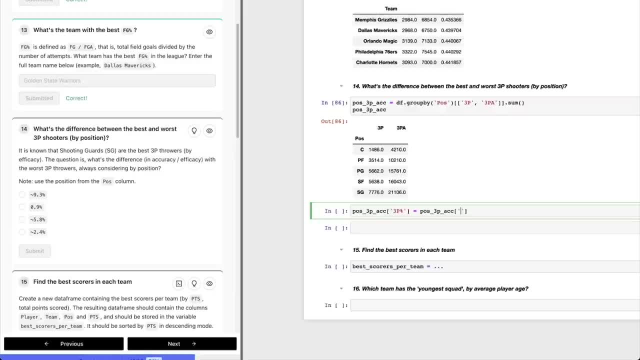 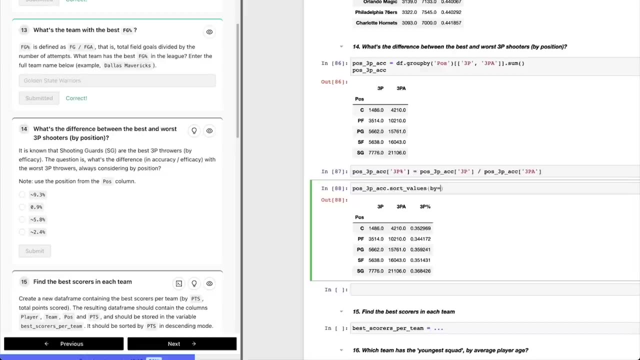 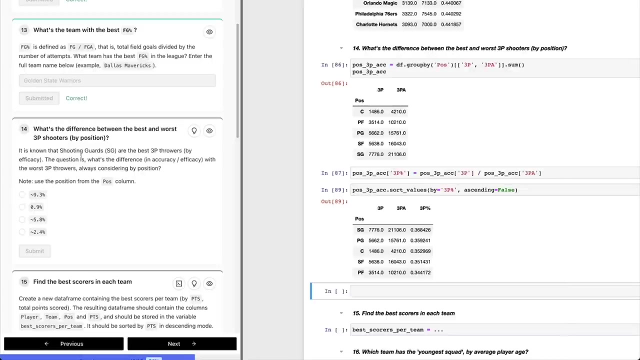 percentage. let's call it. it's gonna be three pointer divided by three PA and the attempts, and now we can do position three P accuracy. now let's sort values by three P percentage ascending folds. the best position: shooting guards: as expected, again, this is just two main knowledge in basketball shooting guards. 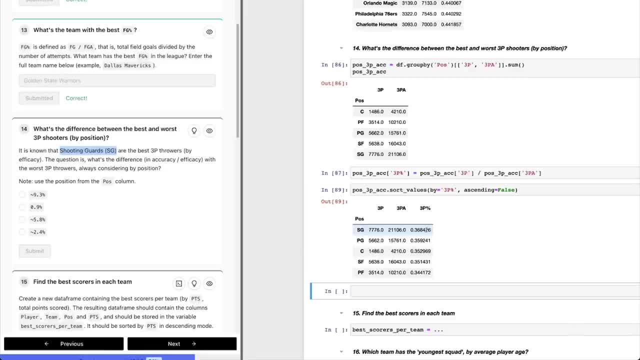 are usually the ones shooting better. I could have with a better accuracy, but it's telling dots that what we actually need to find is: what's the difference in accuracy between shooting guards and the worst position, the worst position. the data frame which we found was the pf, power forward. 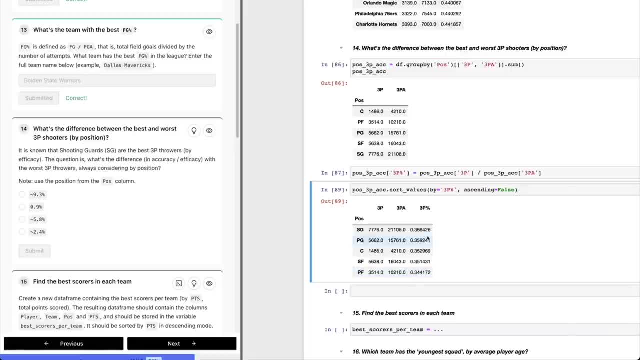 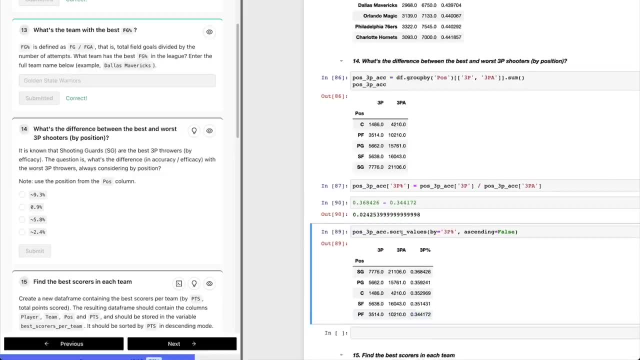 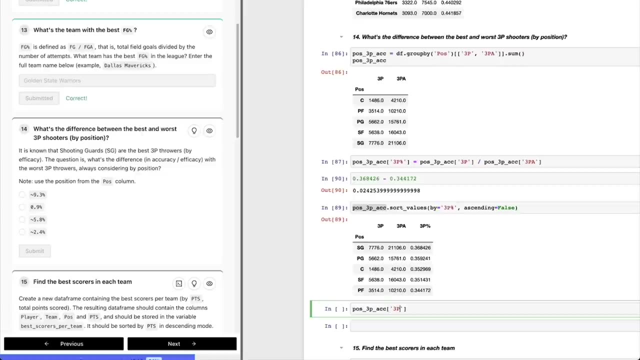 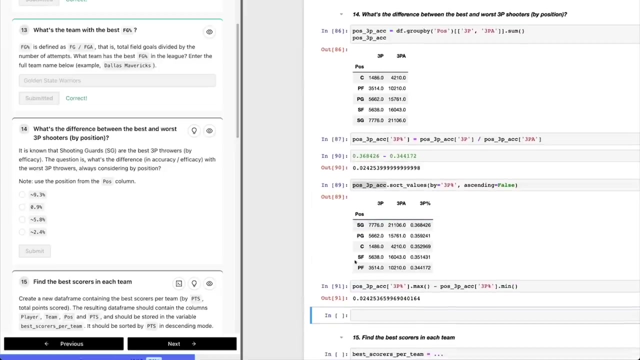 position right. so what's the difference in accuracy? well, we could do something like this: minus dots, it's going to give us the percentage. or we can do something like: um dots, uh, 3p, percentage dot max minus the one in min, and now we have pretty much the same value without hard coding. 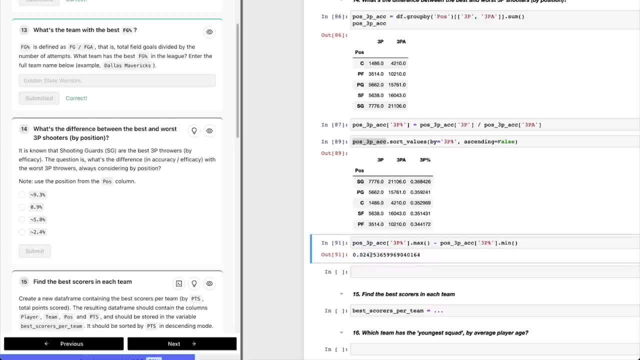 the difference is 0.024, so in percentage terms that's going to be 2.4 percent. that's basically this value, right here, a tiny difference, right, it's like from the first best position to the worst position and it's not a huge difference. but of course, with so many attempts it actually adds up. 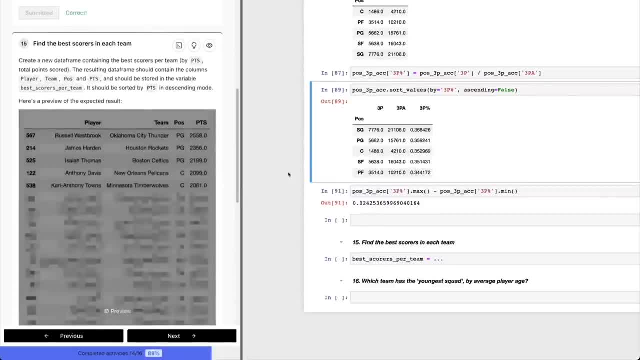 potentially in the league. all right, so this is a very interesting activity. i seriously encourage you to just pause here and try to resolve number 15 by yourself. it's a very interesting one. it might involve a ton of googling, uh, from you, because i mean it's a very interesting activity. 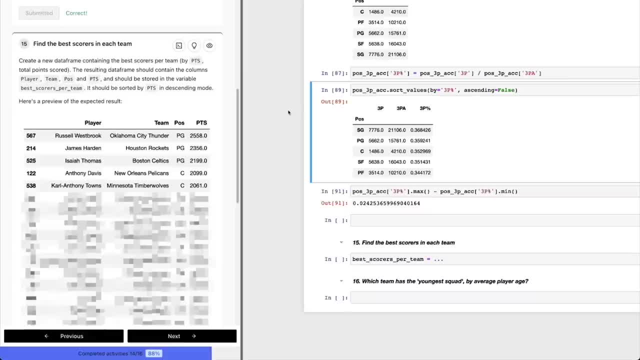 it's a very interesting activity and i wanna say this is the most interesting thing that i've ever seen, not trivial. so just you know this is your use your chance to go ahead and pause the activity. try to solve it. pause the video, sorry. try to solve it by. 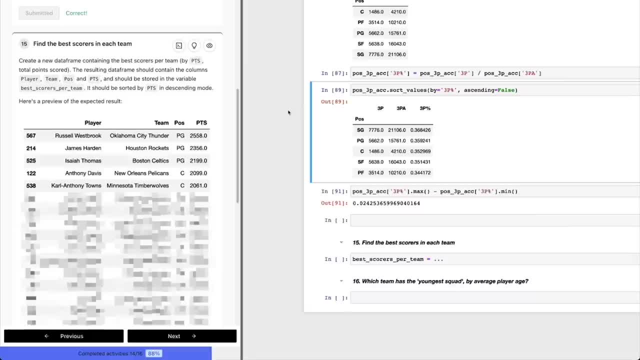 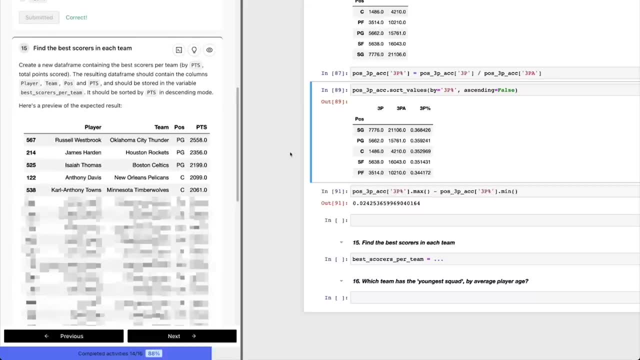 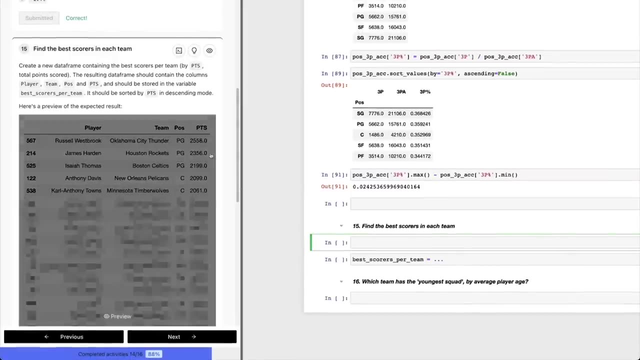 yourself. I'll give you one second. now we're gonna resume and I'm gonna solve it live right here, so you can see how I approached the problem. all right, let's take a stab at it. the activity is asking us to find the best score per team, right? so we want to basically generate this table. that it's the name. 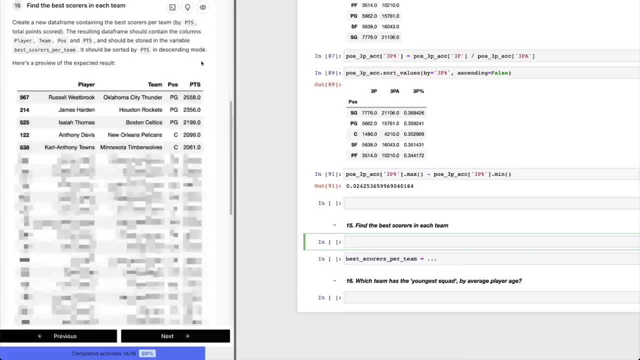 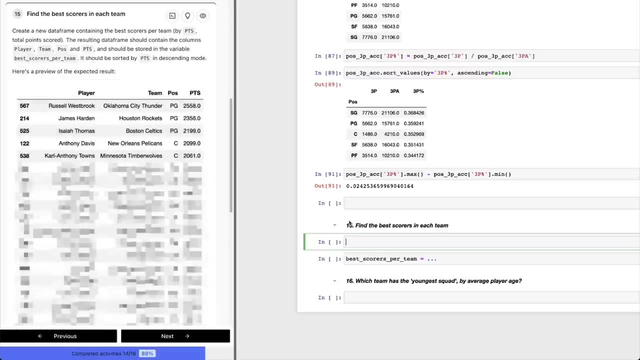 of the player, the team position on the total points- right so or not, best quarters in terms of you know just amount of score points in their team. so basically, we're gonna do something like, for example, the F dot log at the F right. so we're gonna do something like, for example, the F dot log at the F. 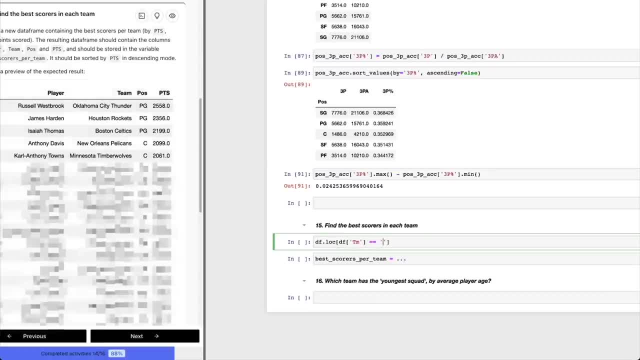 right. so we're gonna do something like, for example, the F dot log at the F team is Oklahoma and we're gonna get get points dot max. so basically the max score points in Oklahoma is this amount. and now we're gonna find where I find the player by saying these and: 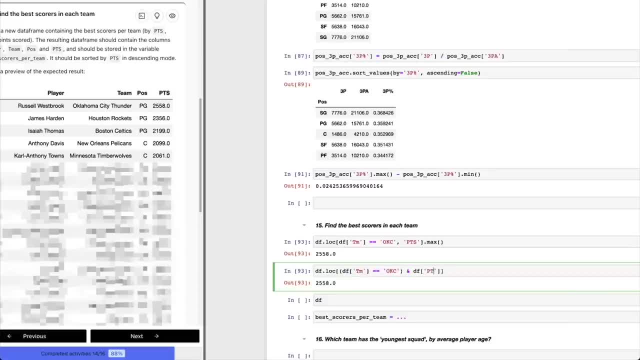 now we're gonna find where I find the player by saying these. and now we're gonna find where I find the player by saying these: and there at PTS equals that value a number and we there at PTS equals that value a number and we there at PTS equals that value a number, and we found that that was Russell Westbrook. 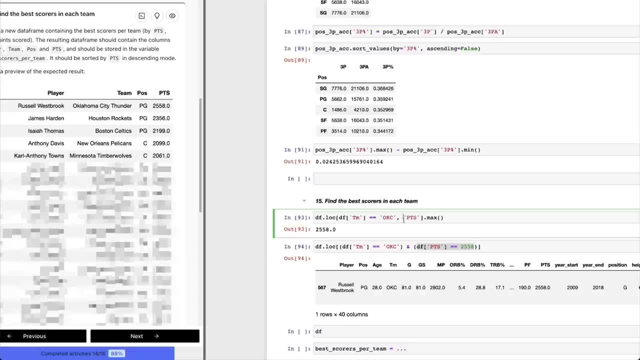 found that that was Russell Westbrook. found that that was Russell Westbrook. we can pretty much put everything in just. we can pretty much put everything in just. we can pretty much put everything in just a one-liner. so we're gonna do I'm gonna a one-liner. so we're gonna do, I'm gonna. 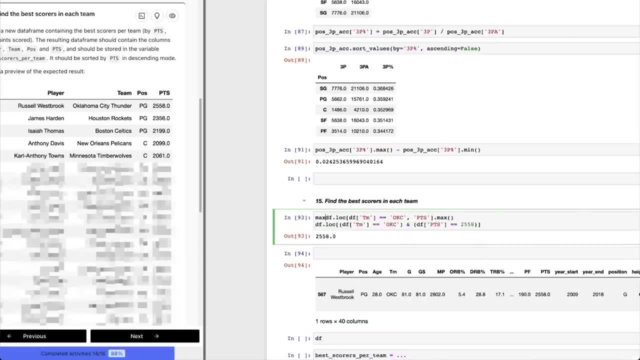 a one-liner. so we're gonna do: I'm gonna copy this thing here and I first find, copy this thing here, and I first find, copy this thing here and I first find the max points in team. max point in teams: the max points in team. max point in teams. 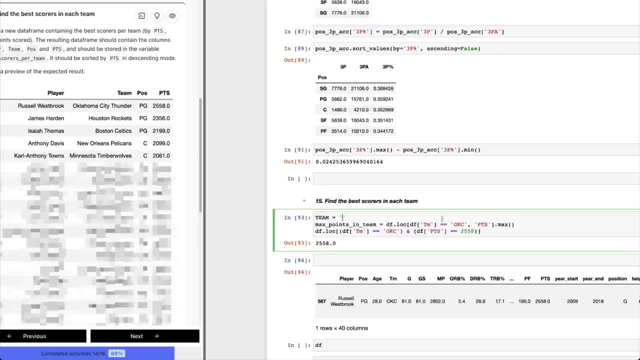 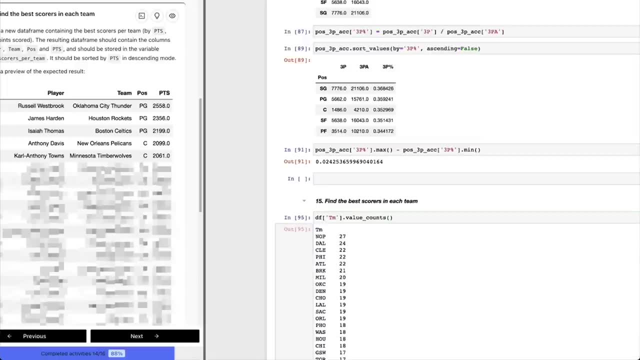 the max points in team. max point in teams. the max points in teams. the max points in teams. I'm gonna team is gonna be the f at TM dots. I don't I'm gonna. team is gonna be the f at TM dots. I don't I'm gonna. team is gonna be the f at TM dots. I don't remember the right Cleveland. 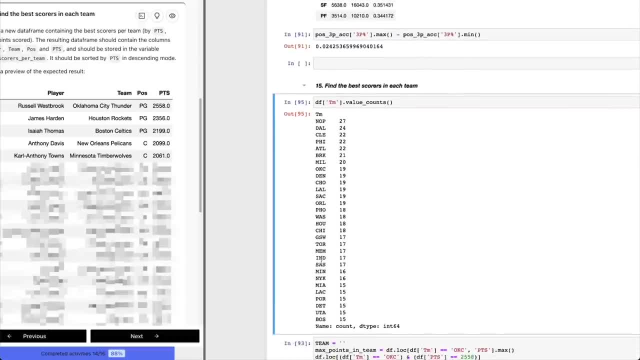 remember the right Cleveland. remember the right Cleveland. which one don't we were gonna do Boston. which one don't we were gonna do Boston? which one don't we were gonna do Boston? how is Boston's probably BOS, BOS, is it? how is Boston's probably BOS, BOS, is it? 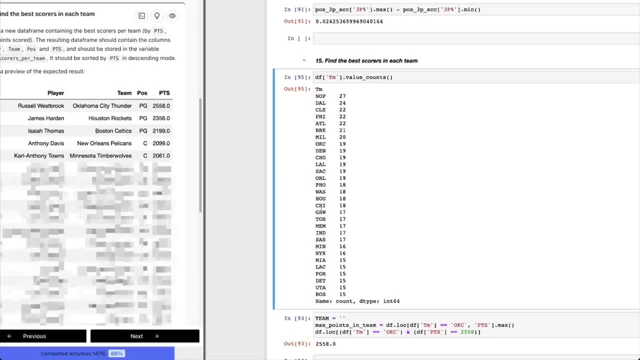 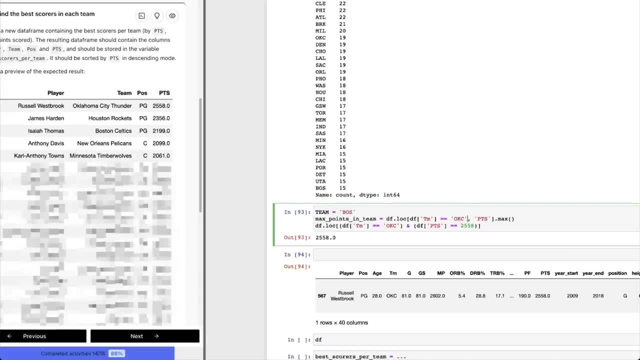 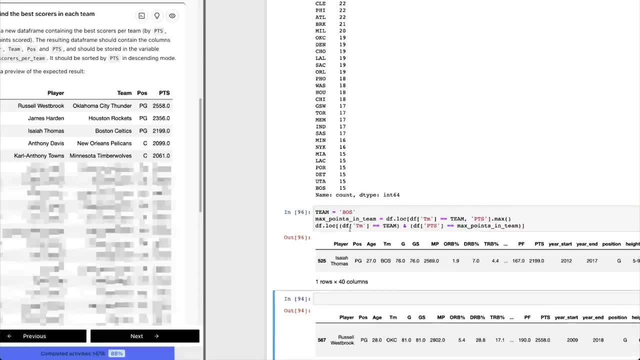 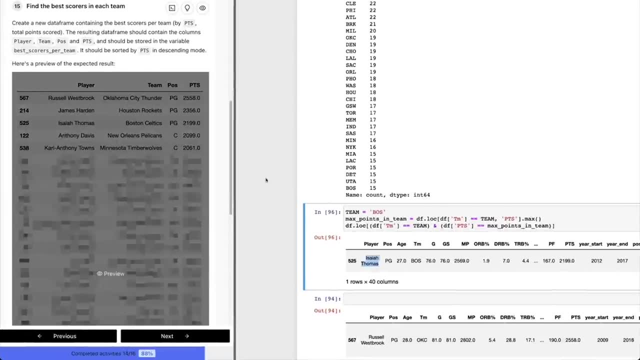 find that the team is team and this is find that the team is team and this is max points, it's corporate team and say max points, it's corporate team. and say max points, it's corporate team and say yeah is the best score of Boston. so I 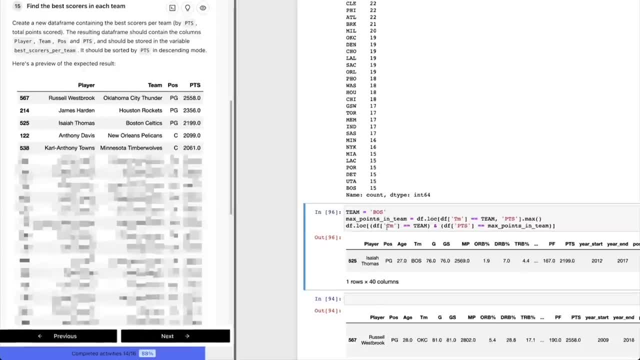 yeah is the best score of Boston. so I, yeah is the best score of Boston. so I want you to understand the problem. this want you to understand the problem. this want you to understand the problem. this is not the solution we're gonna use, is not the solution we're gonna use. 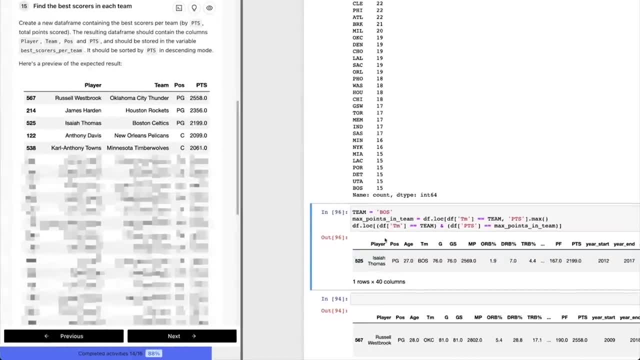 is not the solution we're gonna use, because I mean it involves a ton of. because I mean it involves a ton of, because I mean it involves a ton of manual work, manual work, manual work per team. we could potentially just eat per team. we could potentially just eat. 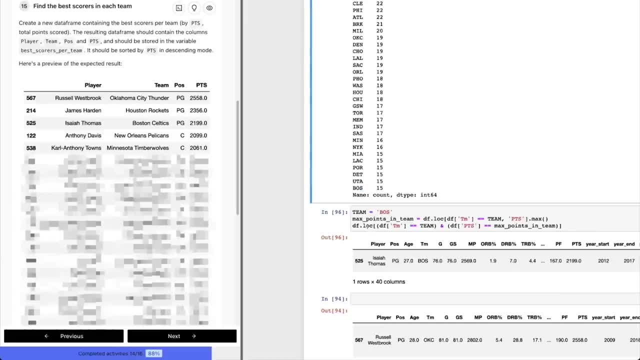 per team. we could potentially just eat: right, you know, get all the teams. but we- right, you know, get all the teams. but we- right, you know, get all the teams. but we can actually show that to use we can do, can actually show that to use we can do. 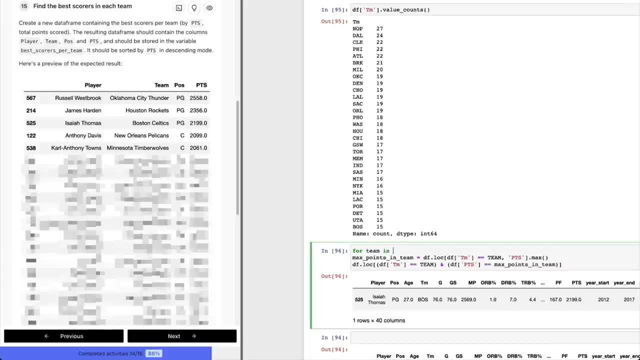 can actually show that to use. we can do something like for team in here dots. something like for team in here dots. something like for team in here dots- unique, unique. we're gonna do that. so unique, unique. we're gonna do that. so unique, unique, we're gonna do that. so we're gonna replace here team we're. 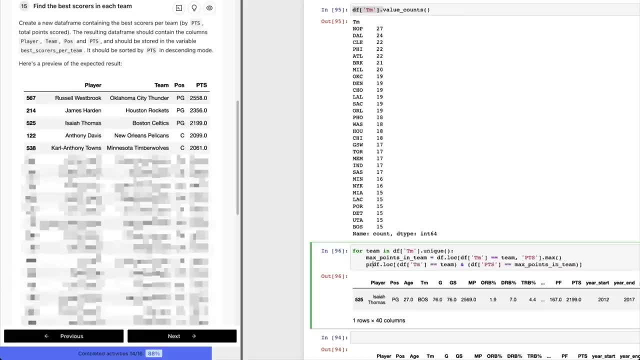 we're gonna replace here team. we're, we're gonna replace here team. we're gonna place here team and print. gonna place here team and print, gonna place here team and print: mmm, we're gonna get here, mmm, we're gonna get here here, mmm, we're gonna get here here two things. we're gonna get player. I'm. 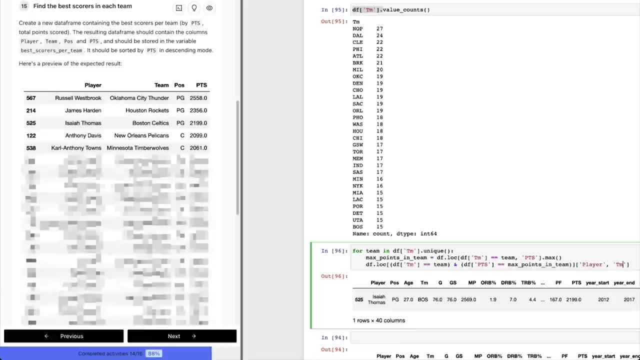 two things: we're gonna get player. I'm two things we're gonna get player. I'm gonna get team team there you go and gonna get team team there you go and gonna get team team there you go and gets the values. I'm gonna get player. gets the values. I'm gonna get player. 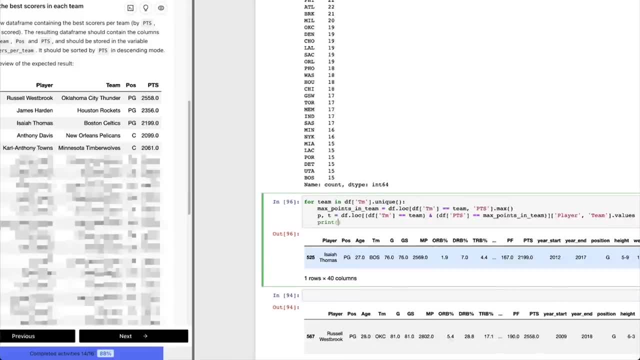 gets the values. I'm gonna get player team- sorry for my variable names. I'm team. sorry for my variable names. I'm team. sorry for my variable names. I'm gonna do prints. I actually can get gonna do prints. I actually can get gonna do prints. I actually can get points as well. PTS, PTS, my variable. 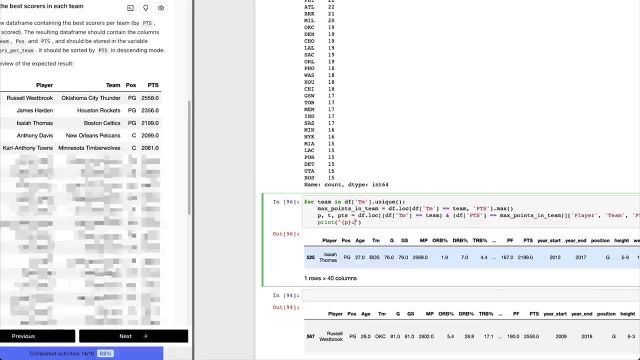 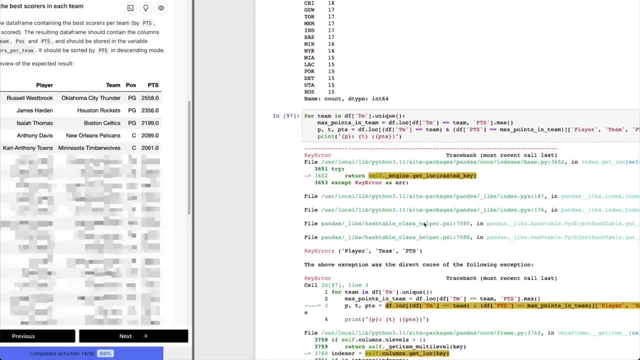 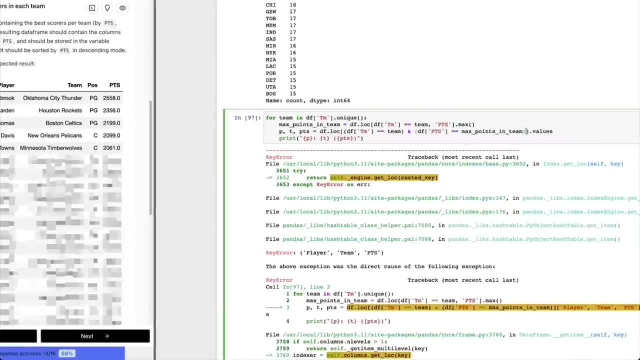 it. when I say P for team with PTS, I did it. when I say P for team with PTS, I did something wrong here. play your team the something wrong here. play your team the something wrong here. play your team the after block: not enough values to unpack. after block: not enough values to unpack. 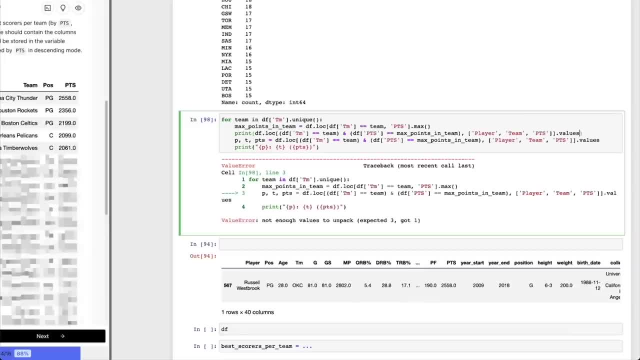 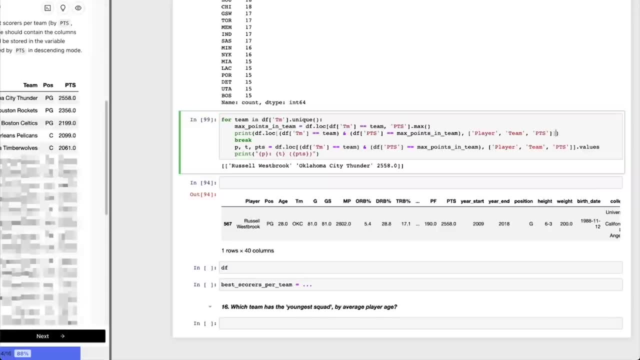 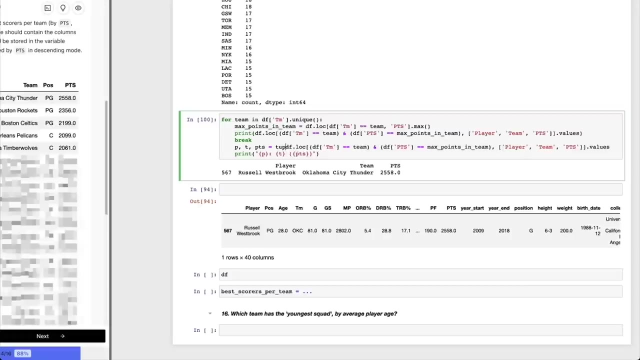 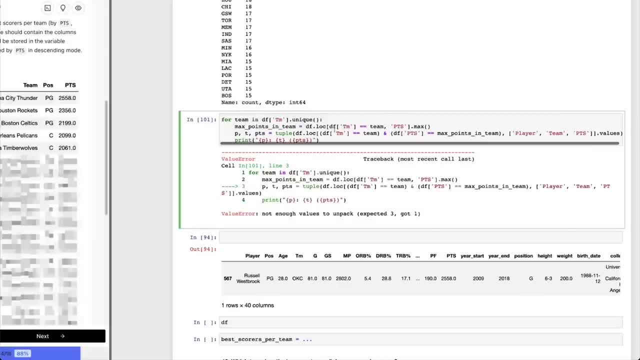 potentially what if I do this? okay, I'm doing something definitely wrong here, doing something definitely wrong here, doing something definitely wrong here which I can understand, but basically which I can understand, but basically which I can understand. but basically what I want to say is that we can. 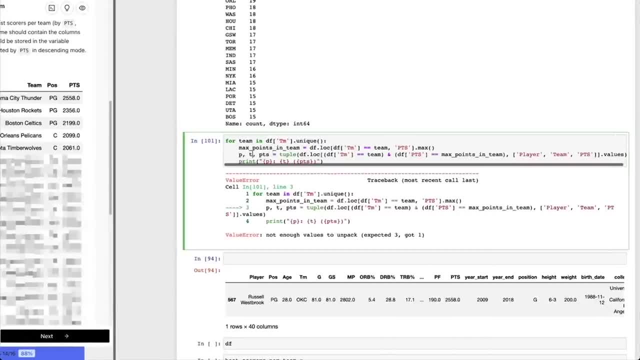 what I want to say is that we can. what I want to say is that we can potentially do these manually right. so potentially do these manually right. so potentially do these manually right. so, let's, let's just print this thing. let's, let's, let's just print this thing. let's. 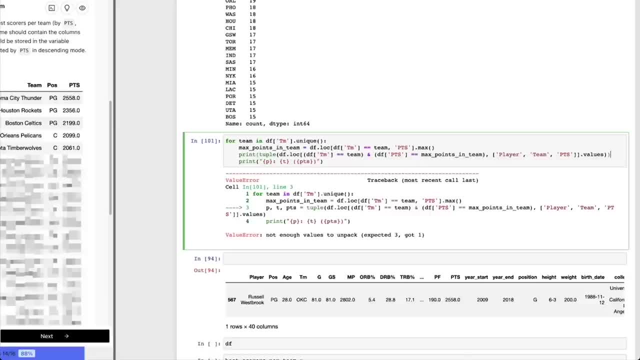 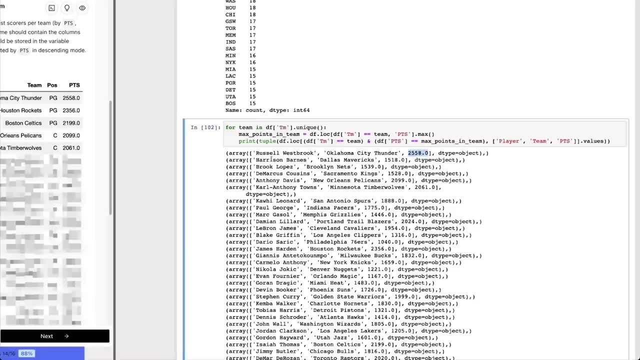 let's, let's just print this thing, let's print, print, print, print, print, print this thing, this thing, this thing, um so Russell Westbrook for Oklahoma, with um so Russell Westbrook for Oklahoma, with, um so Russell Westbrook for Oklahoma, with this amount of this amount of this amount of uh points. Harrison Burns for Dallas. 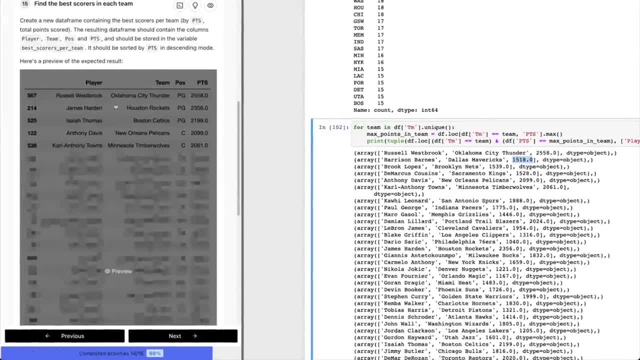 uh points Harrison Burns for Dallas. uh points, Harrison Burns for Dallas. Mavericks, with this amount of Mavericks, with this amount of Mavericks, with this amount of of points, um, let's see Houston of points. um, let's see Houston of points. um, let's see Houston again. it's like we can solve it. 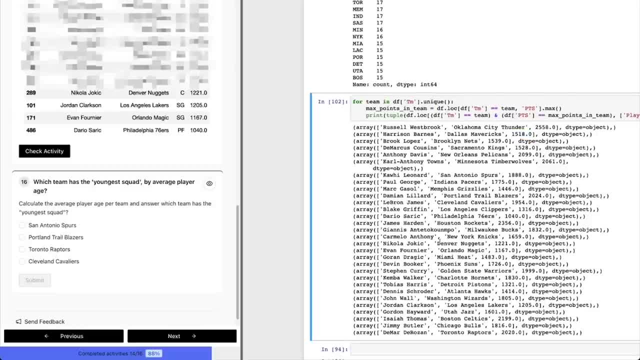 again, it's like we can solve it. again. it's like we can solve it manually. so Denver Nuggets, Denver Nuggets, manually. so Denver Nuggets, Denver Nuggets, manually. so Denver Nuggets, Denver Nuggets. Nicola Jokic, Nicola Jokic for name, Nicola Jokic, Nicola Jokic for name. 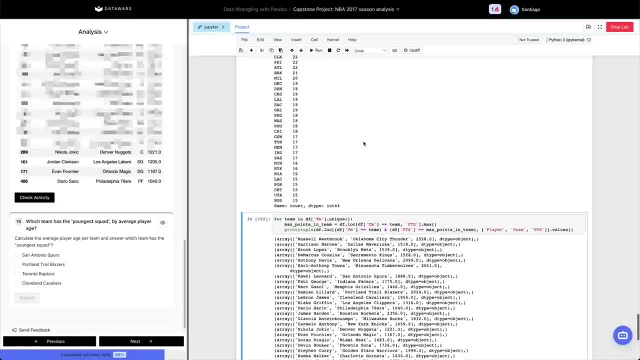 Nicola Jokic. Nicola Jokic for name number. we could potentially solve it number. we could potentially solve it number. we could potentially solve it manually. but the solution that I want to manually, but the solution that I want to manually, but the solution that I want to show you- and it took me some time- 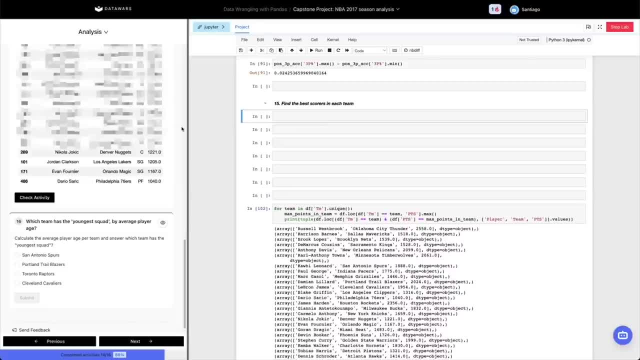 show you, and it took me some time. show you and it took me some time. solution I want to show you solution. I want to show you solution I want to show you. involves a, involves a, involves a group by operation. to put in a way, I'm group by operation. to put in a way I'm 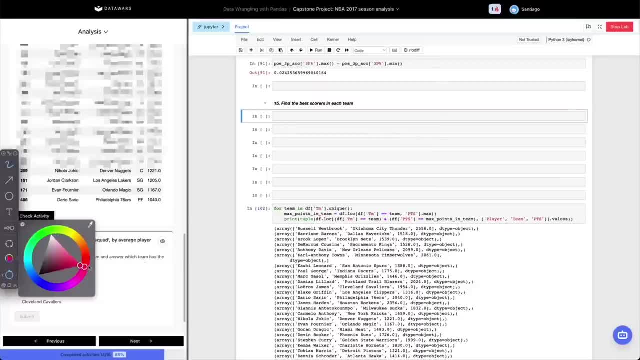 group by operation. to put in a way: I'm sorry because I'm drawing you lately. sorry because I'm drawing you lately, sorry because I'm drawing you lately. um, I'm going to show you a drawing. um, I'm going to show you a drawing. um, I'm going to show you a drawing signifying or trying to explain the. 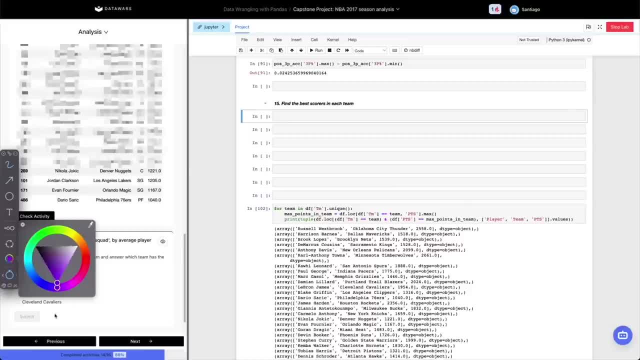 signifying, or trying to explain the signifying, or trying to explain the solution that I'm going to use, so solution that I'm going to use, so solution that I'm going to use. so, basically, we have a our full data frame. basically, we have a our full data frame. 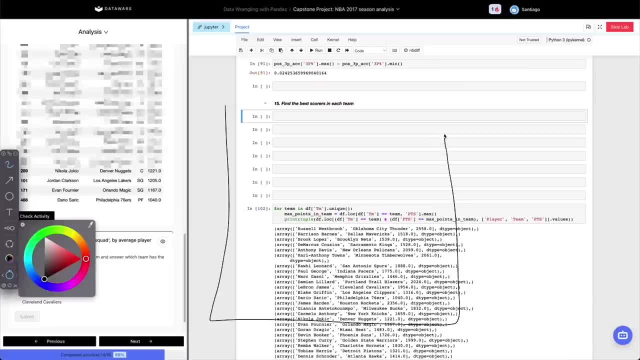 basically, we have a our full data frame. so we're going to use black so data. so we're going to use black so data. so we're going to use black so data frame, frame, frame. there you go, there is actually a way. there you go, there is actually a way. 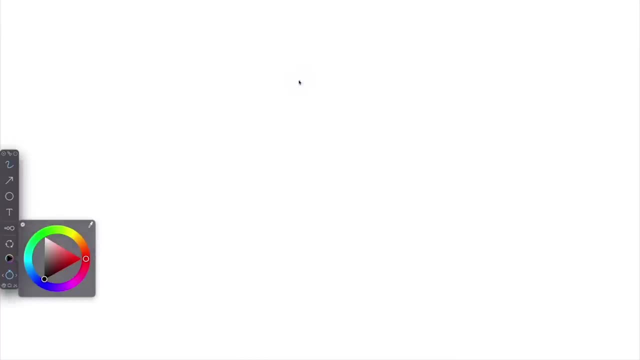 there you go. there is actually a way that I can make this, that I can make this, that I can make this thing a whiteboard there you go. thing a whiteboard there you go. thing a whiteboard there you go. so we're going to do this is our data. 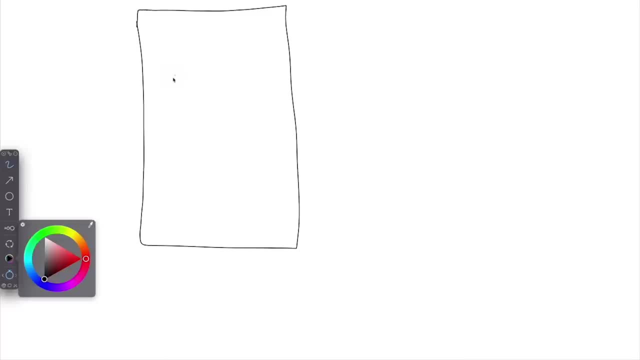 so we're going to do this. is our data, so we're going to do this. is our data frame, frame frame, and our data frame contains information and our data frame contains information and our data frame contains information about different players and let's say about different players, and let's say: 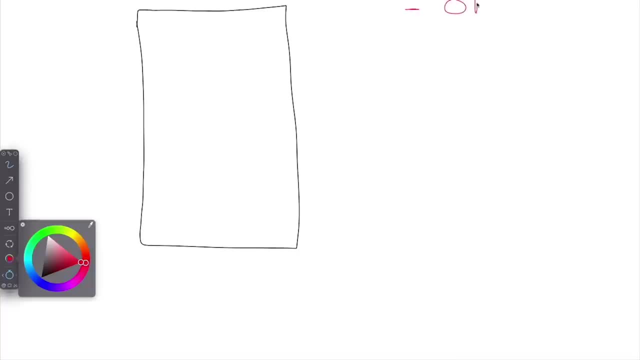 about different players and let's say that we have red for Oklahoma, that we have red for Oklahoma, that we have red for Oklahoma, we have or no. let's actually do red for we have or no. let's actually do red for we have or no. let's actually do red for Chicago. 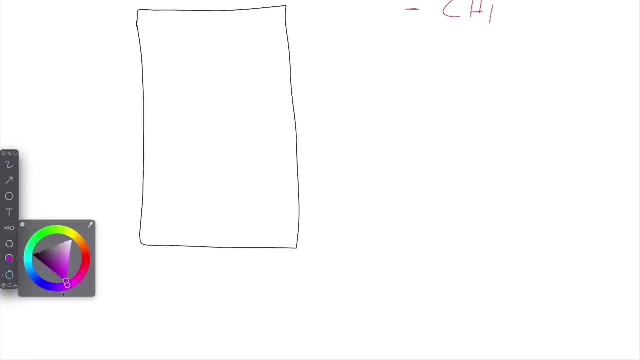 Chicago, Chicago, of course, of course, of course, we're going to use: uh, we're going to, we're going to use: uh, we're going to, we're going to use, uh, we're going to use um, use, um, use um. blue for Oklahoma, blue for Oklahoma, blue for Oklahoma. and we're going to use green. 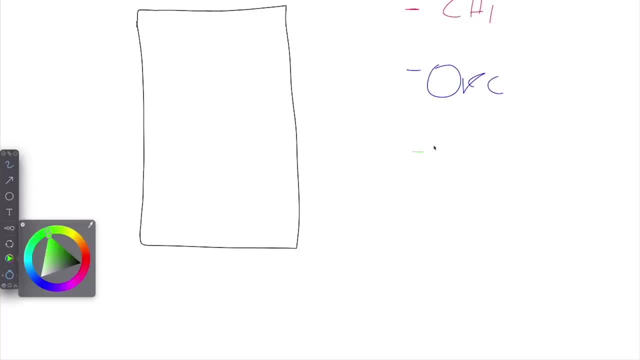 and we're going to use green, and we're going to use green, green, green, green, for, for, for, uh Boston, uh Boston, uh Boston. I need a darker grain grain for Boston. um, and the way it's gonna work, um, and the way it's gonna work, um, and the way it's gonna work is we're gonna have these. 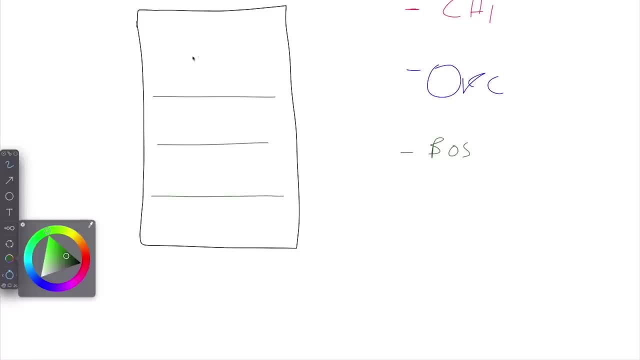 is we're gonna have these, is we're gonna have these. players are just intertwined in the whole. players are just intertwined in the whole. players are just intertwined in the whole data frame right, so data frame right, so data frame right. so, uh, there you go and let's say: 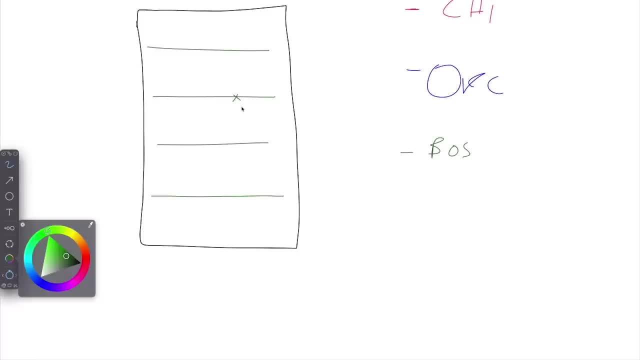 uh, there you go. and let's say: uh, there you go. and let's say that, right here, this is the best shooter, that, right here, this is the best shooter, that, right here, this is the best shooter or the best shooter in the given team or the best shooter in the given team. 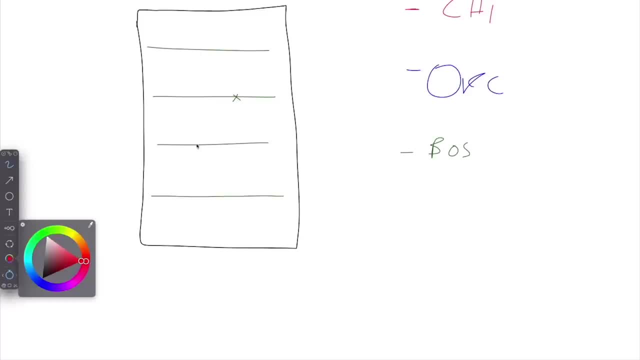 or the best shooter in the given team. we're gonna have the same thing for. we're gonna have the same thing for. we're gonna have the same thing for. for Chicago. we're gonna have this player for Chicago. we're gonna have this player for Chicago. we're gonna have this player and that player and that player and that. 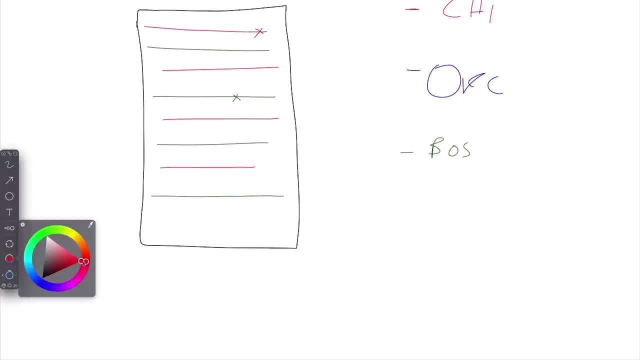 and that player and that player, and that and that player, and that player and that player, and it's gonna be the best player and it's gonna be the best player and it's gonna be the best scoring that in in the in the team and scoring that in in the in the team, and 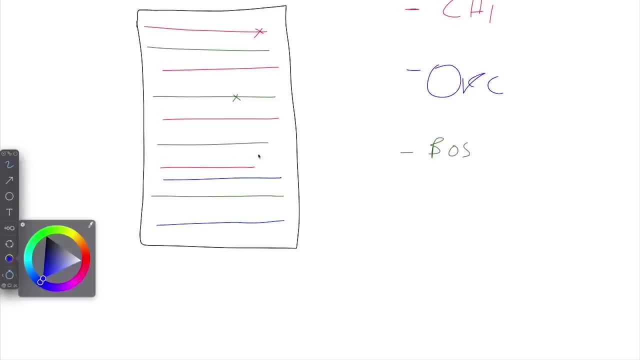 scoring that in in the in the team, and then we're gonna have this player from then, we're gonna have this player from then we're gonna have this player from Oklahoma and this player, this player and Oklahoma and this player, this player and Oklahoma and this player, this player and that player from Oklahoma. this is gonna. 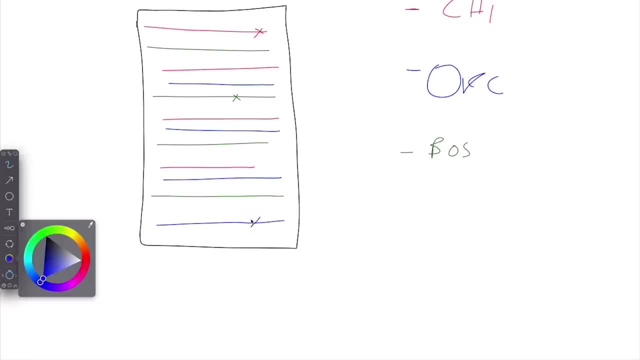 that player from Oklahoma. this is gonna that player from Oklahoma, this is gonna be the best. let's actually put it be the best. let's actually put it be the best. let's actually put it. put that player here, that's gonna be the. put that player here, that's gonna be the. 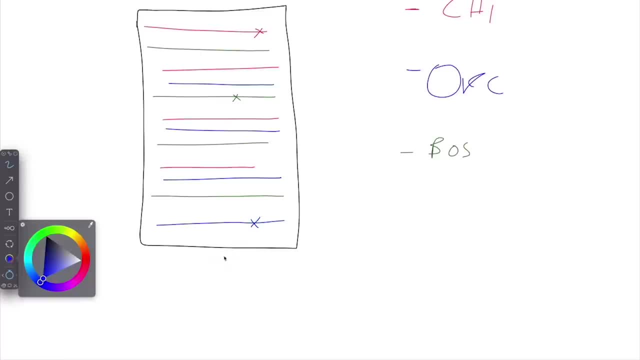 put that player here, that's gonna be the best from each team. so that's basically best from each team. so that's basically best from each team. so that's basically what we did in the previous solution. we, what we did in the previous solution, we, what we did in the previous solution, we filter. we said the previous solution, the. 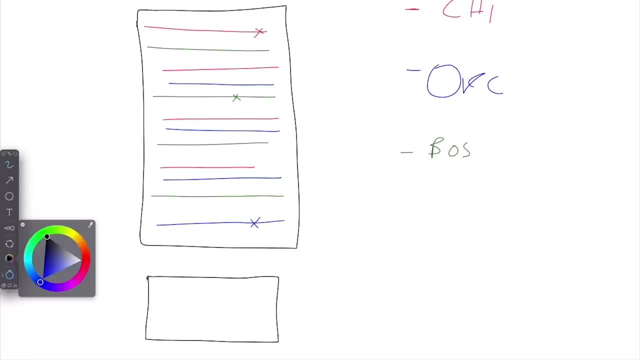 filter. we said the previous solution, the filter. we said the previous solution, the manual one. we've created an intermediate manual one. we've created an intermediate manual one. we've created an intermediate data frame that only contain data frame. that only contain data frame. that only contain players from a given team: Oklahoma. in. 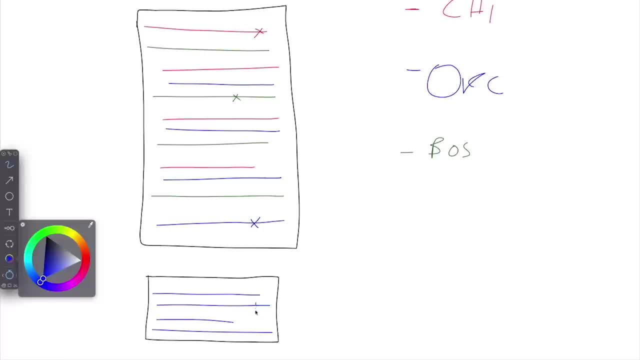 players from a given team Oklahoma in players from a given team Oklahoma. in this case, we then found the best quarter. this case, we then found the best quarter. this case, we then found the best quarter. was this value or actually this value? was this value or actually this value? 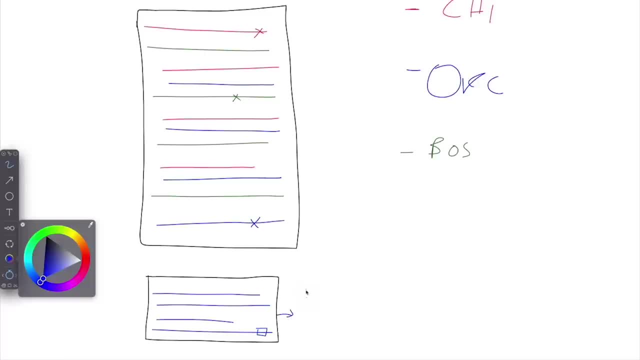 was this value, or actually this value, right here, and we made a second right here, and we made a second right here and we made a second filtering in which we said: find the filtering, in which we said: find the filtering in which we said: find the player player. 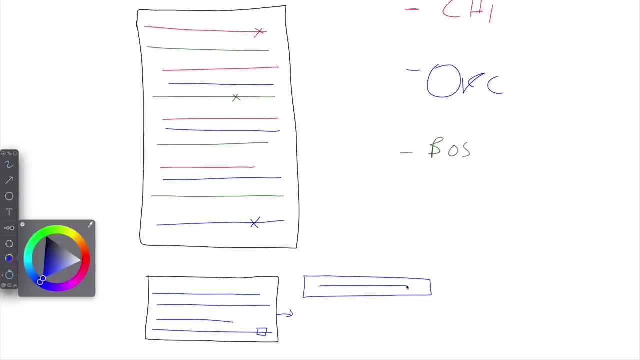 player in that team with that amount of points in that team, with that amount of points in that team, with that amount of points. so now we have a single player. so now we have a single player. so now we have a single player we wanna. this is, of course, a different. 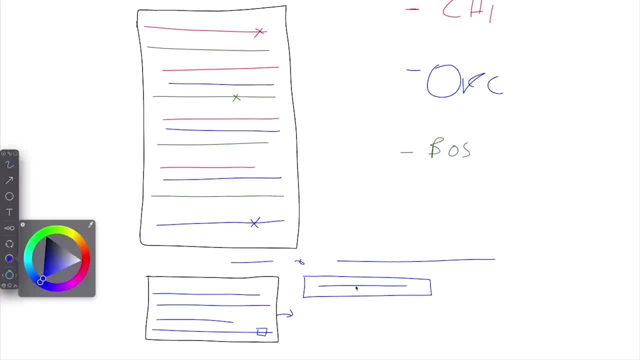 we wanna this is, of course a different. we wanna this is, of course, a different solution. what we want to do now or let's solution. what we want to do now or let's solution. what we want to do now or let's separate it, separate it, separate it. what i do now is using a group, by sort. 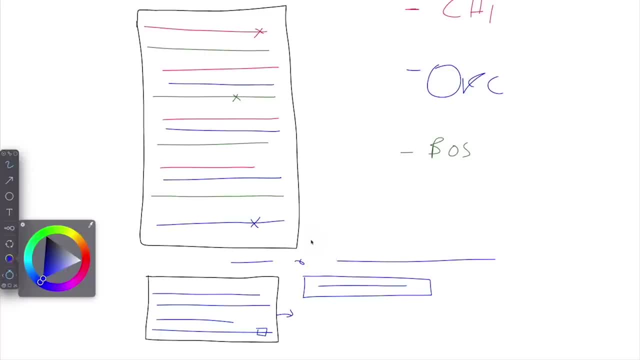 what i do now is using a group by sort. what i do now is using a group by sort of way: operation of way, operation of way. operation. we want the we want pandas to focus on. we want the we want pandas to focus on. we want the we want pandas to focus on different groups of players. so for 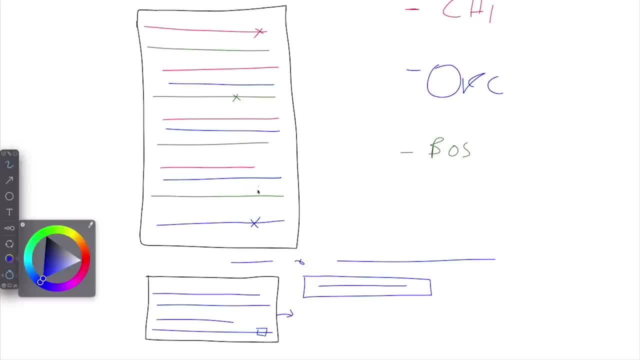 different groups of players, so for different groups of players. so, for example, all the blue players, all the example. all the blue players, all the example. all the blue players, all the green players, all the red players and green players, all the red players and green players, all the red players, and perform an operation in a group button. 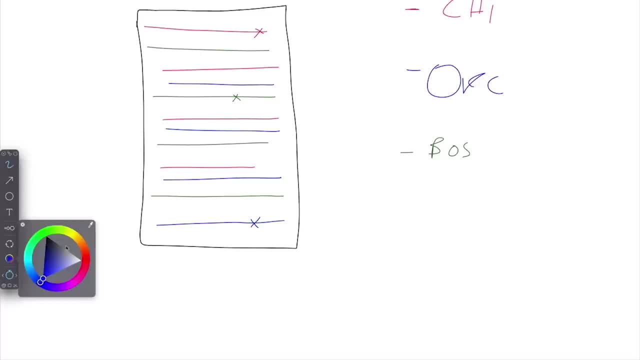 perform an operation in a group button, perform an operation in a group button, group by fashion, group by fashion, group by fashion, but, but, but we want it to the result expanding. we want it to the result expanding. we want it to the result expanding back to the whole group. so we want it. 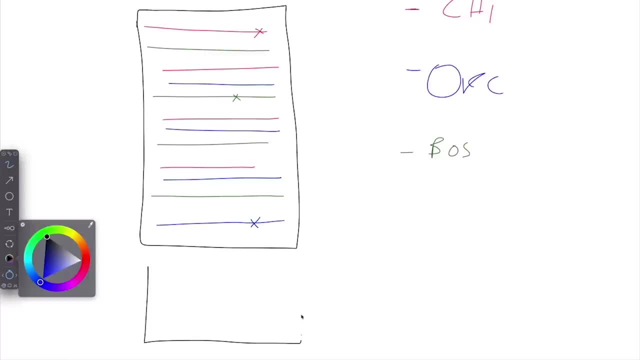 back to the whole group. so we want it back to the whole group. so we want it to just do that's pretty similar. we're to just do that's pretty similar. we're to just do that's pretty similar. we're gonna gonna, gonna, focus on the blue players from oklahoma. 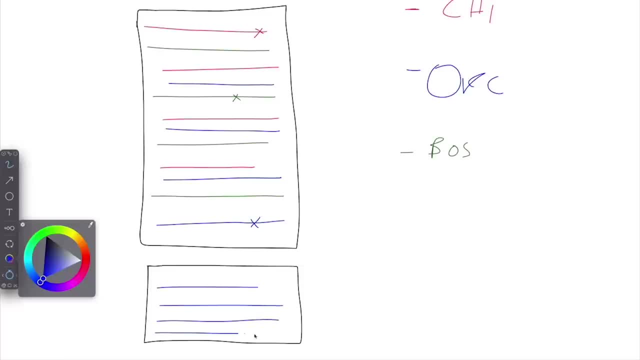 focus on the blue players from oklahoma. focus on the blue players from oklahoma. we're gonna do, we're gonna do, we're gonna do. create the group by operation: the. the. create the group by operation: the. the create the group by operation: the. the split piece. 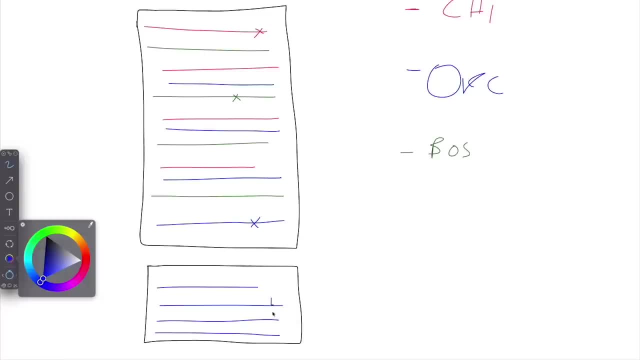 split piece, split piece. find something. in this case, we're going find something. in this case, we're going find something. in this case, we're going to find the maximum in points. so it's to find the maximum in points. so it's to find the maximum in points. so it's going to be, for example, these maximum. 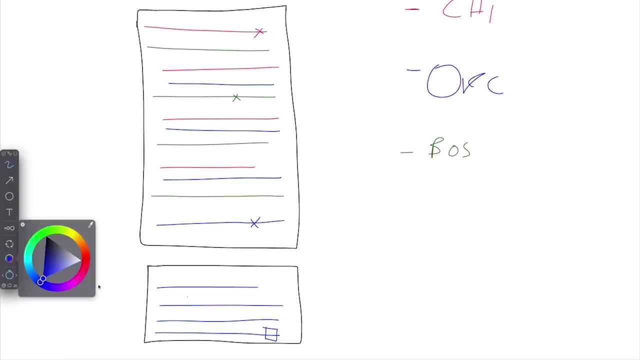 going to be, for example, these maximum. going to be, for example, these maximum points, but instead of what we did before, points. but instead of what we did before, points, but instead of what we did before, which is all manual, we wanted to go back, which is all manual. we wanted to go back. 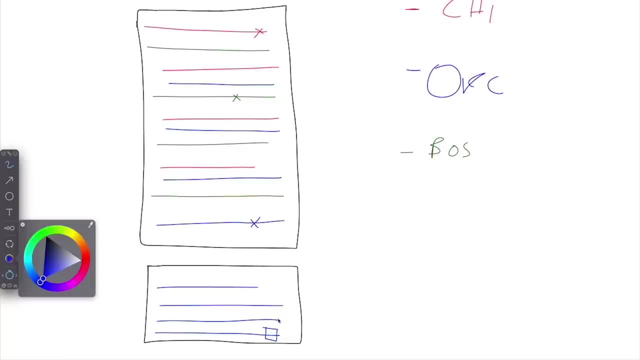 which is all manual. we wanted to go back and replicate this value. we're going to and replicate this value. we're going to and replicate this value. we're going to call this value v. call this value v. call this value v. this value v very important. we wanted to. 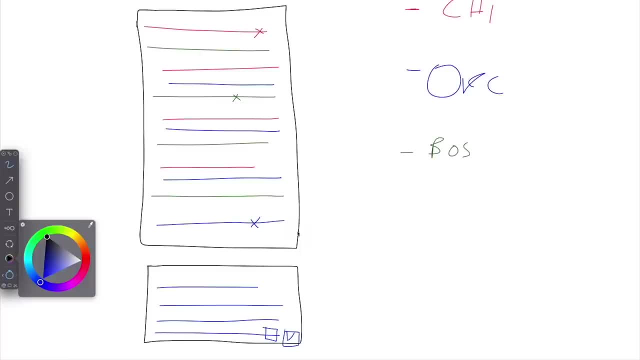 this value v very important. we wanted to this value v very important. we wanted to replicate it back to all the members of replicate it back to all the members of replicate it back to all the members of the group. so we want this value to be the group. so we want this value to be. 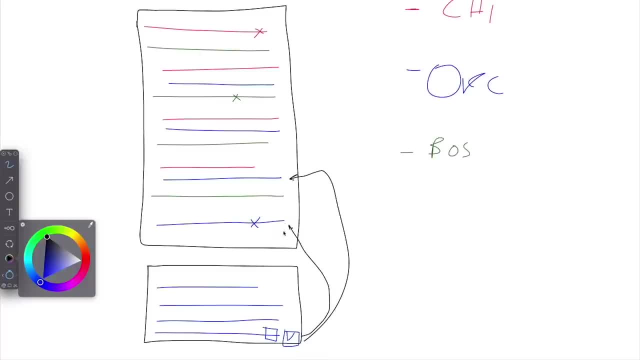 the group. so we want this value to be applied here and here, etc. so we want it applied here and here, etc. so we want it applied here and here, etc. so we want it. we want it to be it's going to be v. we want it to be it's going to be v. 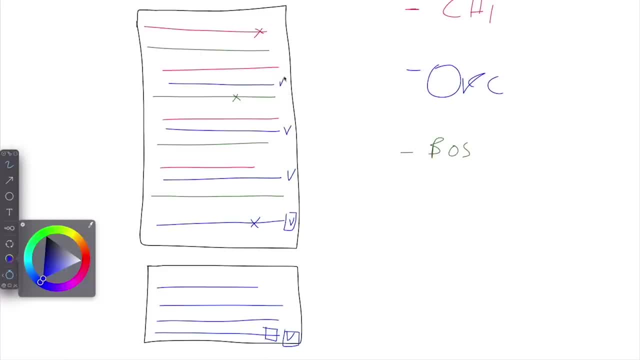 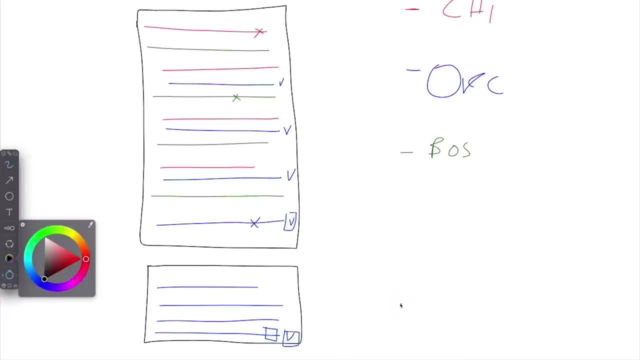 group that we have so for chicago now. group that we have so for chicago now. we're going to do another data frame. we're going to do another data frame. we're going to do another data frame. splock, splock, splock. we're going to do another data frame. 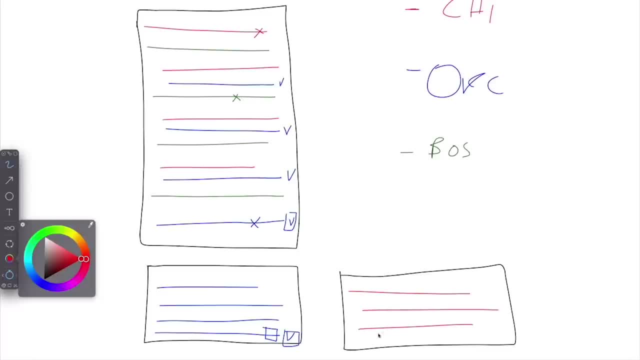 we're going to do another data frame. we're going to do another data frame and we're going to do player player and we're going to do player player and we're going to do player player, player, player. that's all going to be done. player, player. that's all going to be done. 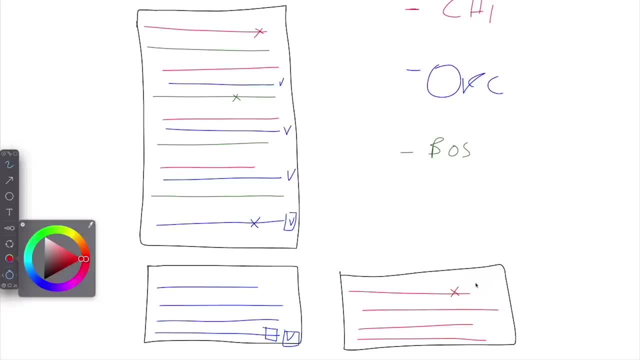 player, player. that's all going to be done automatically by pandas, automatically by pandas, automatically by pandas. find the given value we want in this. find the given value we want in this. find the given value we want in this case is v case is v case is v again, and just replicate that value, v. 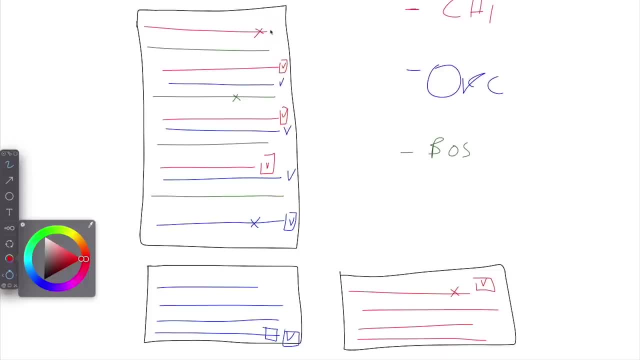 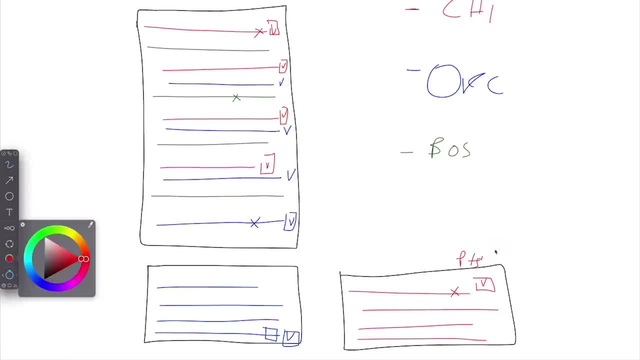 is the maximum, is the maximum of pts, so the column pts when i compute of pts, so the column pts when i compute of pts, so the column pts when i compute the underscore, the underscore, the underscore. so i don't know 900 points. so i don't know 900 points. 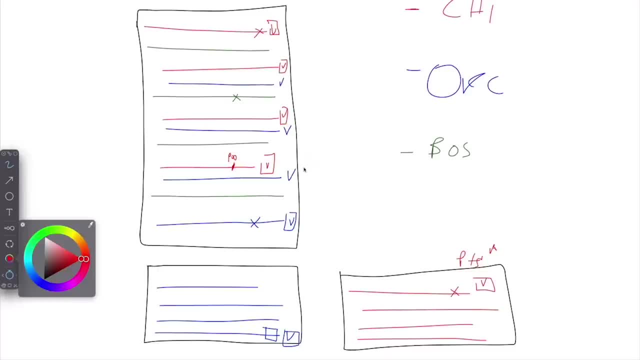 so i don't know, 900 points, or 300 points, whatever and next to it, or 300 points, whatever and next to it, or 300 points, whatever and next to it. there's going to be a new value. that's. there's going to be a new value. that's. 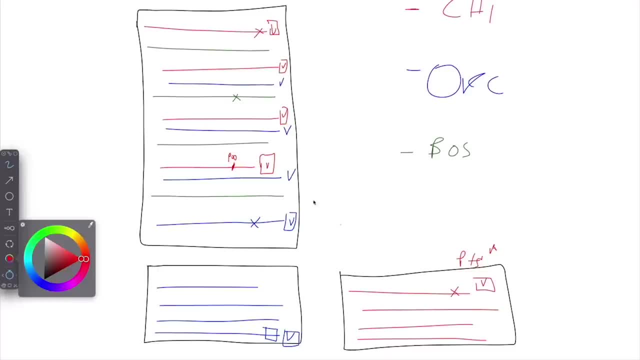 there's going to be a new value. that's going to be the top. going to be the top, going to be the top of that group, given the group by of that group, given the group by of that group, given the group by operation. here's going to say: 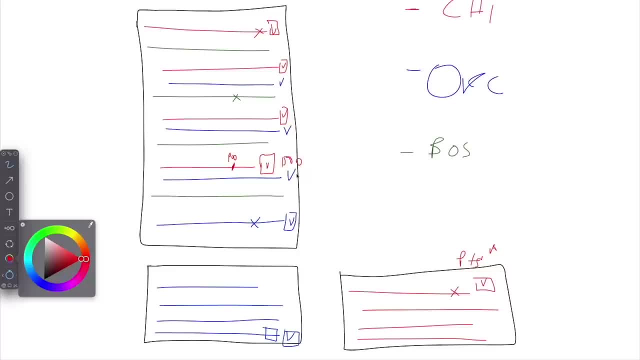 operation here's going to say: operation here's going to say: i don't know a ton of points, i don't know a ton of points, i don't know a ton of points. 1500, right, so we want um each player. 1500, right, so we want um each player. 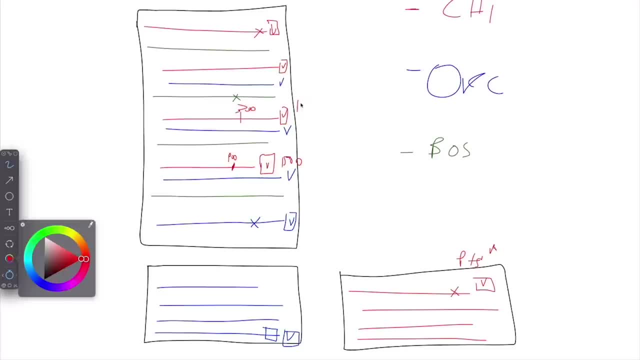 1500. right, so we want um each player. this is going to be. this is going to be. this is going to be 300, and next to it is going to be 1500. 300 and next to it is going to be 1500. 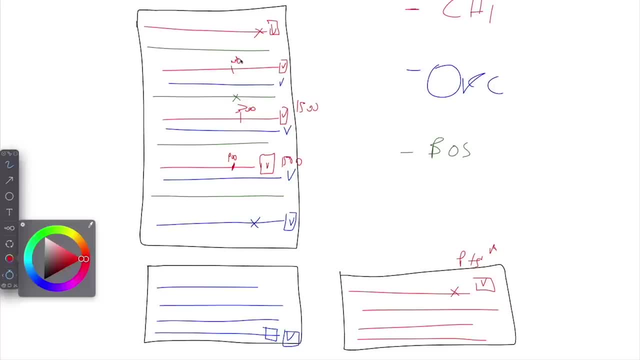 300, and next to it is going to be 1500, and this is going to be 30 point player and this is going to be 30 point player, and this is going to be 30 point player. didn't even play. didn't even play. 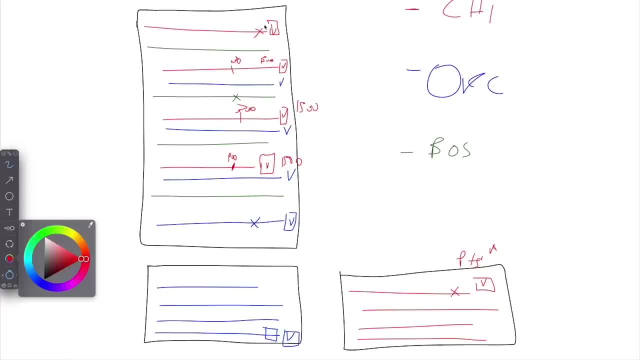 didn't even play, and this is going to be 1500 right, and this is going to be 1500 right, and this is going to be 1500 right, and of course this one is going to be, and of course this one is going to be. 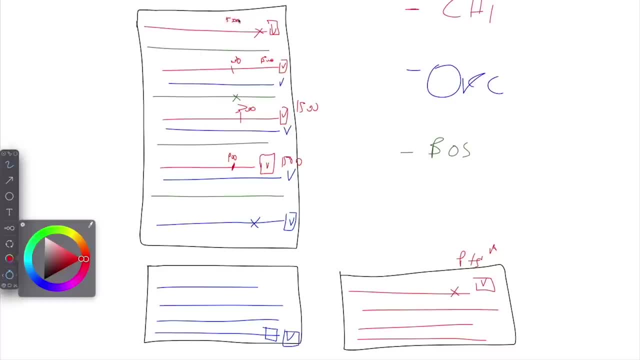 and of course this one is going to be 1500 in the, in the, 1500 in the in the, 1500 in the, in the points, and 1500 in the points and 1500 in the values. then what we're going to do is: 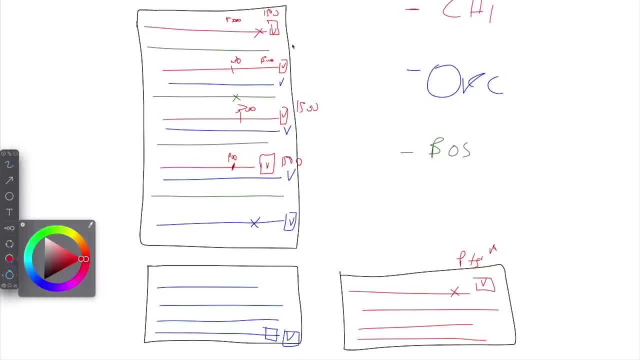 values, then what we're going to do is values, then what we're going to do is we're going to just, we're going to just we're going to just find the top player, or the player with find the top player, or the player with find the top player or the player with the top points. 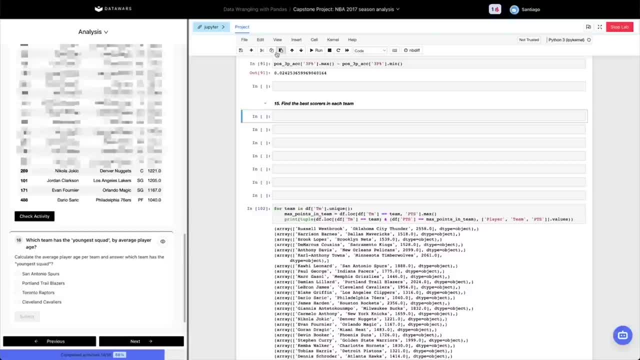 the top points, the top points per per team. all right, let's get rid of per per team. all right, let's get rid of per per team. all right, let's get rid of that, that, that, and finally resolve the task which is. and finally resolve the task which is. 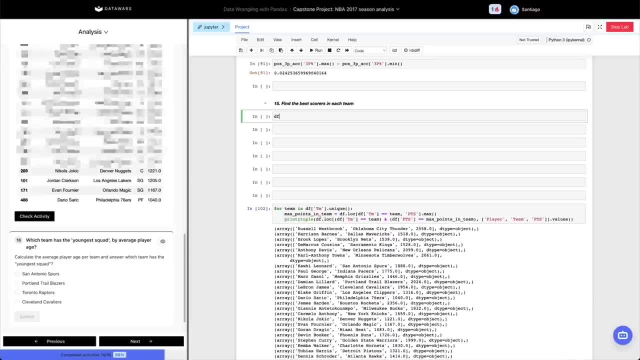 and finally resolve the task, which is relatively simple, relatively simple, relatively simple. i mean there was a huge explanation, but i mean there was a huge explanation, but i mean there was a huge explanation, but trust me, it's simple the way we're. trust me, it's simple the way we're. 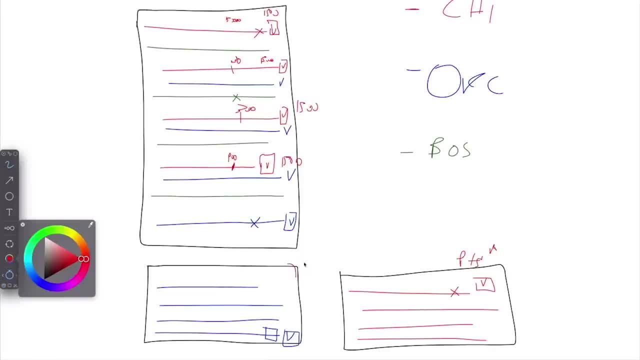 trust me, it's simple the way we're doing it. it's like we want to group by doing it. it's like we want to group by doing it. it's like we want to group by team. we want to perform this operation. team, we want to perform this operation. 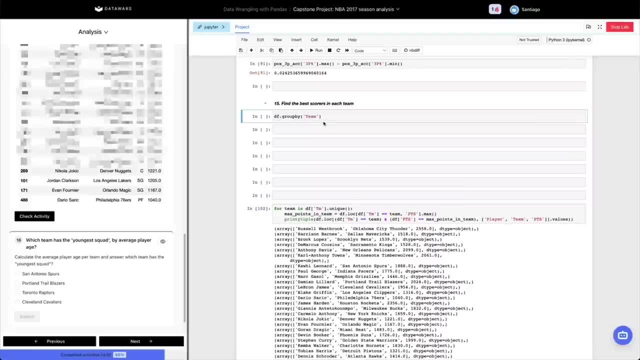 team. we want to perform this operation here and this operation here for each here and this operation here for each here and this operation here for each team. we're going to group by team team. we're going to group by team team. we're going to group by team. but we're going to get a pts, the column. 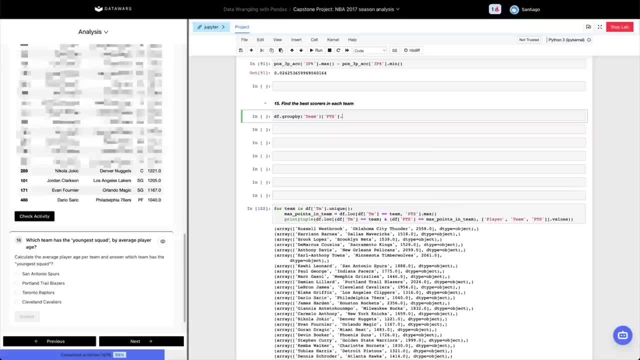 but we're going to get a pts the column, but we're going to get a pts the column. we want to compute, we want to compute, we want to compute. but here we're going to apply the, but here we're going to apply the. but here we're going to apply the operation transform. 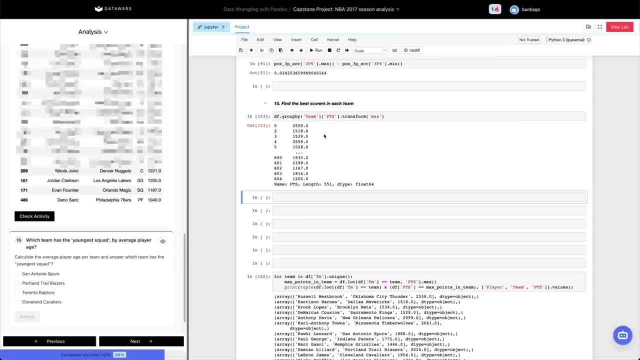 and pass the value max, and pass the value max, and pass the value max, and that's going to give us a value, and, and that's going to give us a value, and, and that's going to give us a value. and that's basically what i told you before. 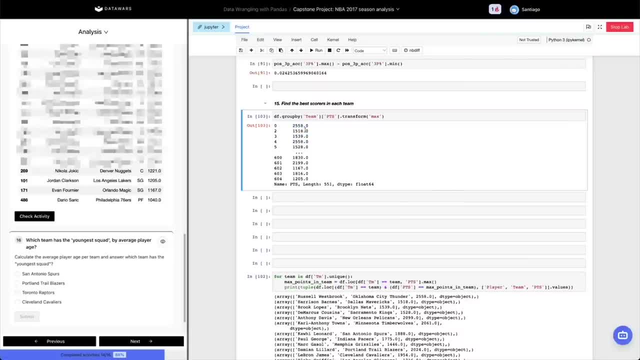 that's basically what i told you before. that's basically what i told you before. for each team, for each group, for each. for each team, for each group, for each, for each team, for each group, for each individual. so it found individual. so it found individual. so it found it found it first broke. 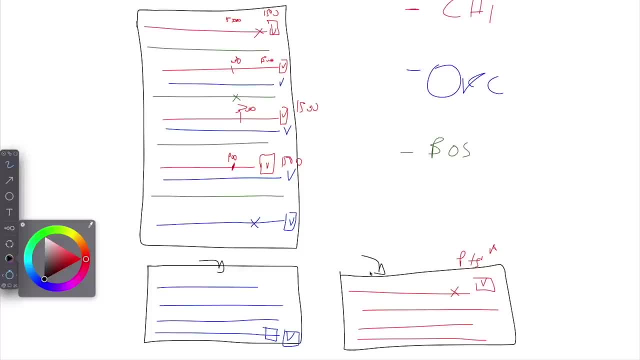 it found it first broke. it found it first broke the players into different groups, based the players into different groups, based the players into different groups based on their team, on their team, on their team. it's uh found the value we were looking. it's uh found the value we were looking. 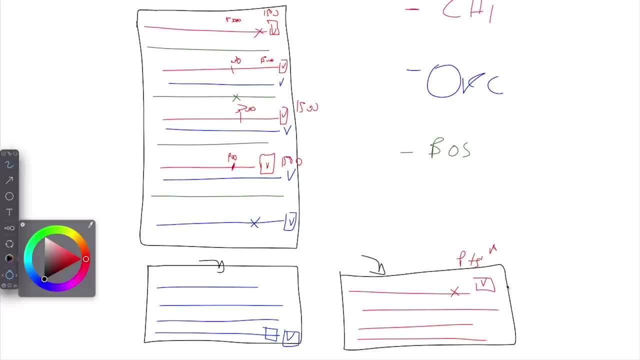 it's uh found the value we were looking for. pts max. for pts max. for pts max, it's it's it's uh assigned the value to each one. it's uh assigned the value to each one. it's uh assigned the value to each one. it's found the value. put the value next to. 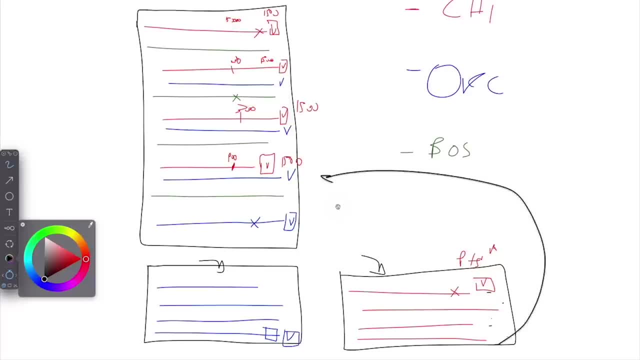 found the value. put the value next to found the value. put the value next to each one of this and reassemble the same, each one of this, and reassemble the same, each one of this, and reassemble the same data frame, data frame, data frame. and now we're going to have this: 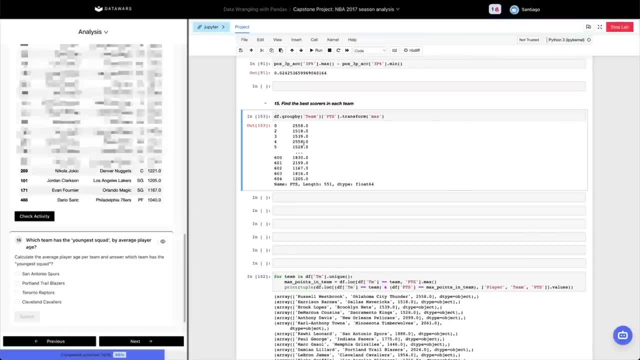 and now we're going to have this, and now we're going to have this: value once again. so value once again, so value once again. so let's, let's, let's hide that, and we're going to do dn at hide that, and we're going to do dn at. 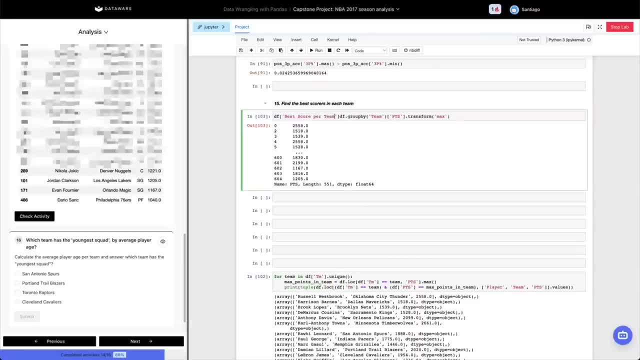 hide that and we're going to do dn at best. best. best score score: score per team, per team, per team. it's going to be that thing we're going. it's going to be that thing we're going. it's going to be that thing we're going to assign it. we can call it. this is our v. 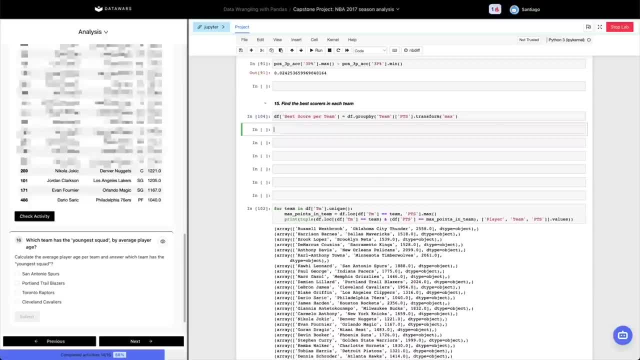 to assign it. we can call it: this is our v to assign it. we can call it: this is our v value. of course i want to use a better value. of course i want to use a better value. of course i want to use a better firewall name. 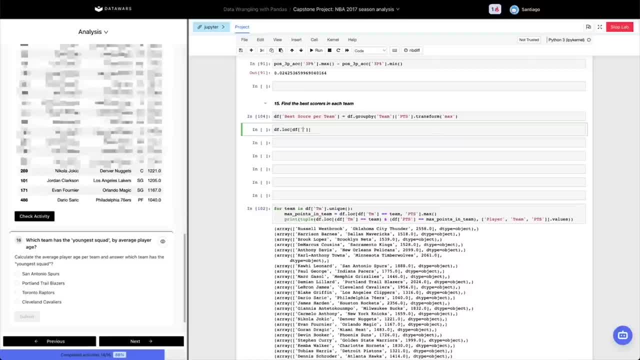 firewall name, firewall name. and now we're going to look at let's, and now we're going to look at let's, and now we're going to look at let's say df, at say df, at say df at team is, team is team, is uh, oklahoma city thunder. 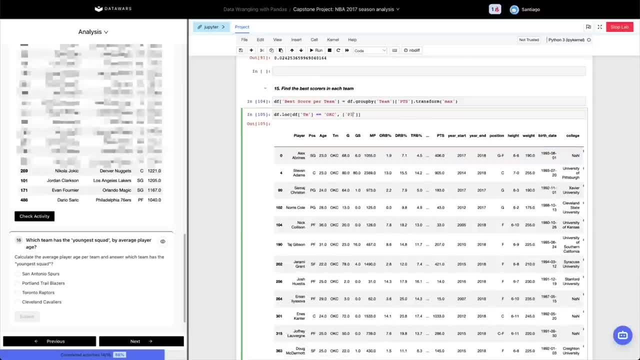 uh oklahoma city, thunder uh, oklahoma city, thunder oklahoma city. and we're going to find oklahoma city and we're going to find oklahoma city, thunder, oklahoma city, thunder, only uh player and we're going to only uh player and we're going to. 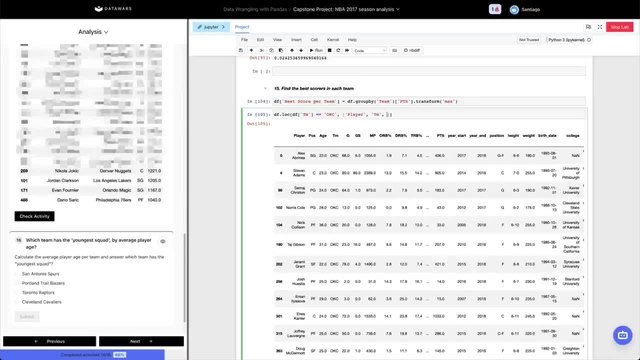 only uh player and we're going to find um, um um team. if you want to repeat it on pts team. if you want to repeat it on pts team. if you want to repeat it on pts values: values, values by by, by pts, pts- pts ascending, ascending, ascending falls. 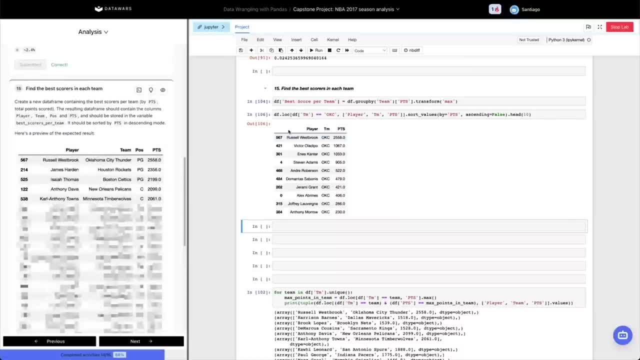 falls, falls. first rows, first rows, first rows, and here and here and here, you're gonna have that four. oh, of course you're gonna have that four. oh, of course you're gonna have that four. oh, of course i'm i'm forgetting the most important. i'm i'm forgetting the most important. 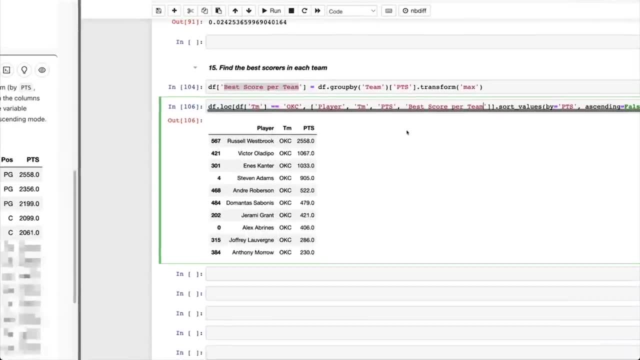 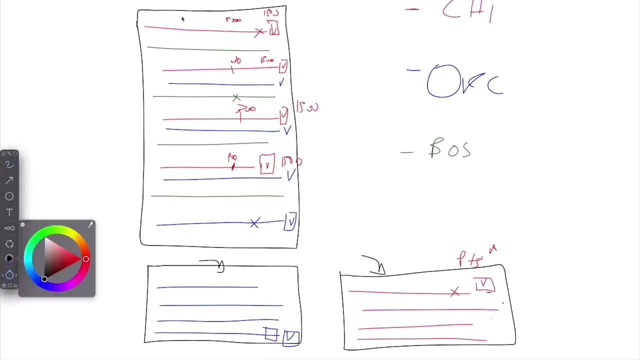 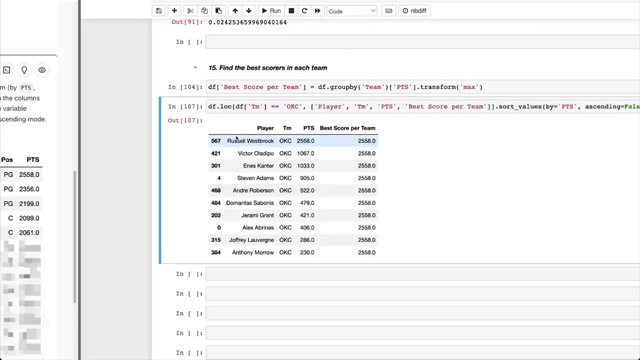 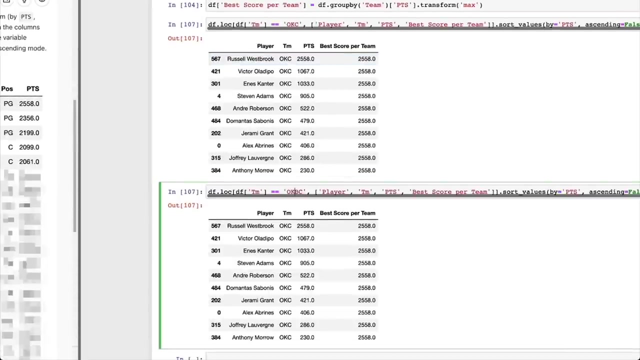 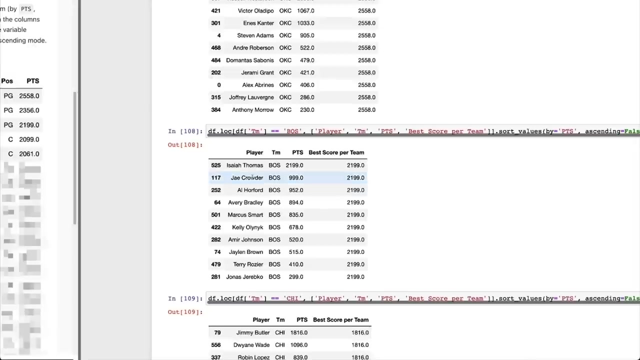 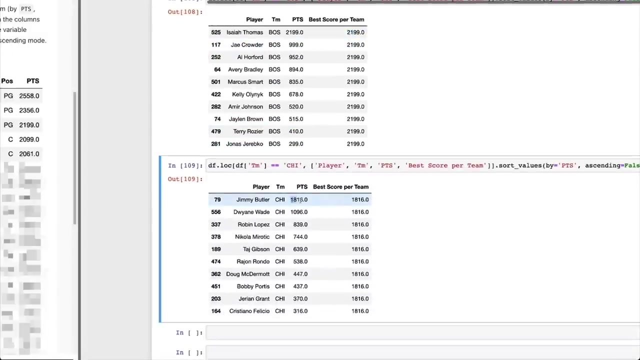 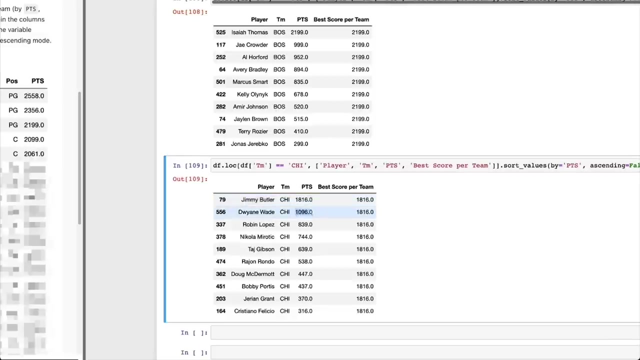 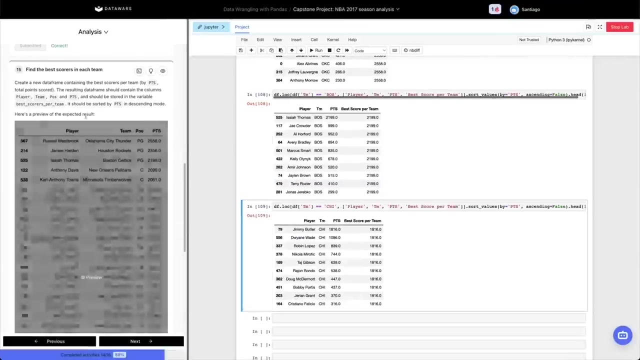 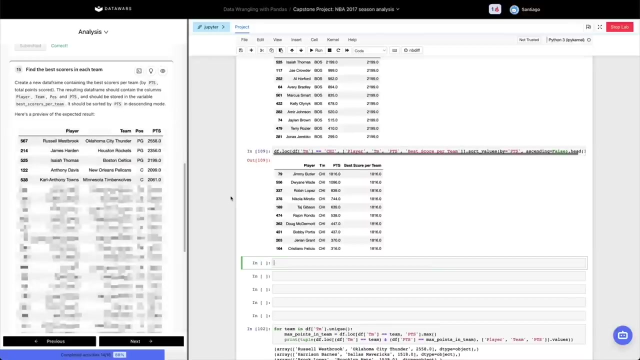 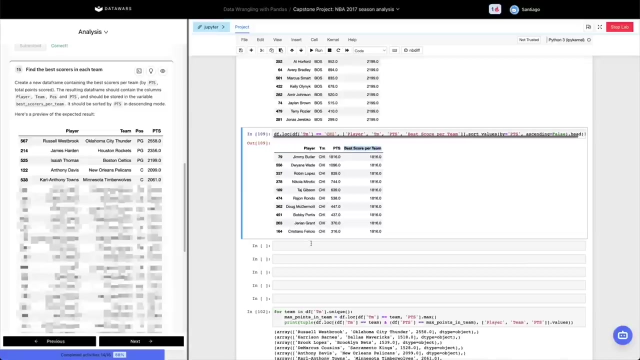 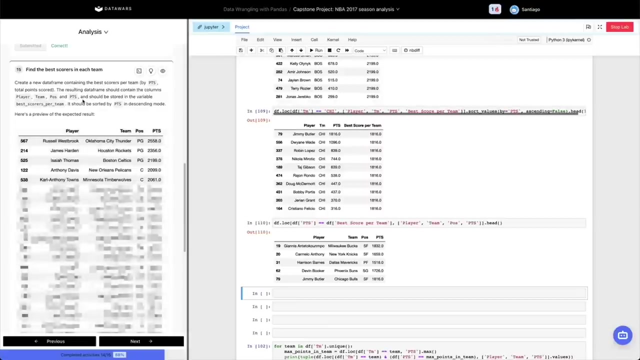 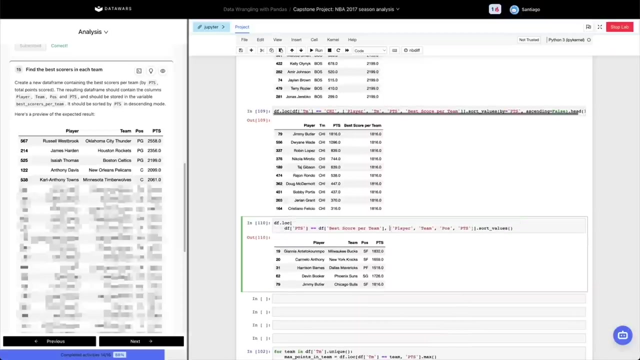 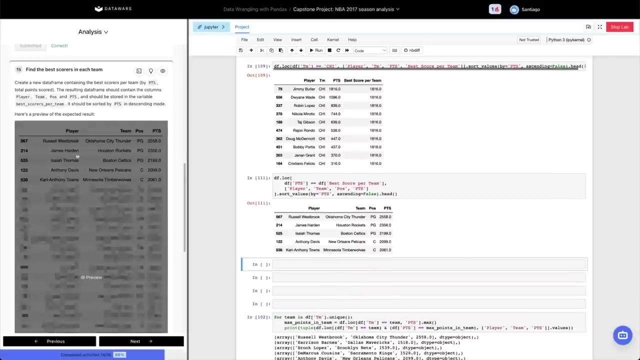 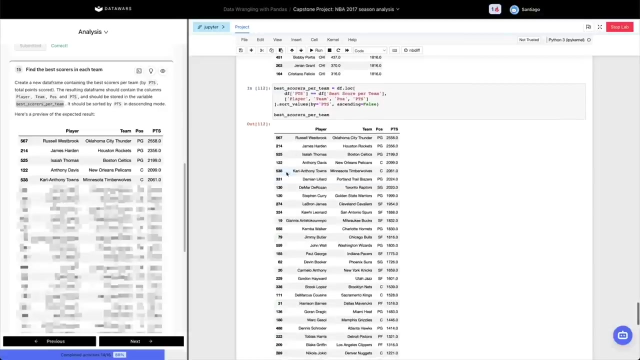 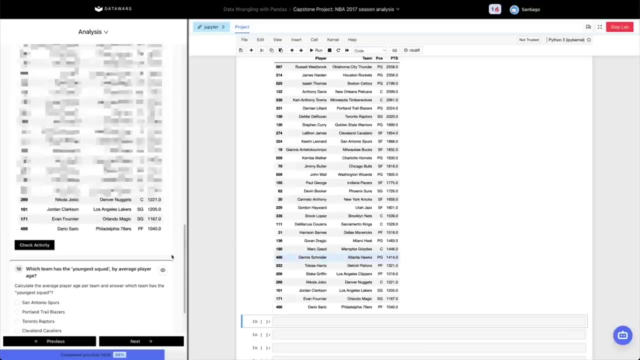 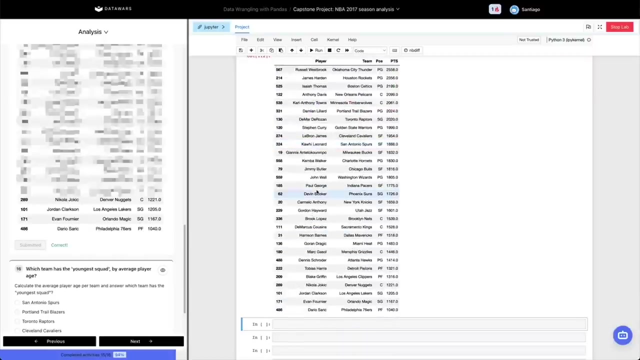 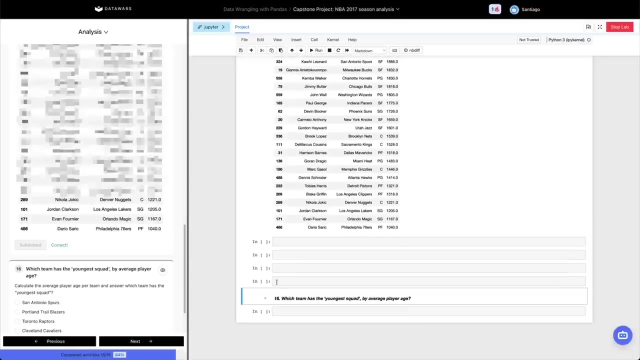 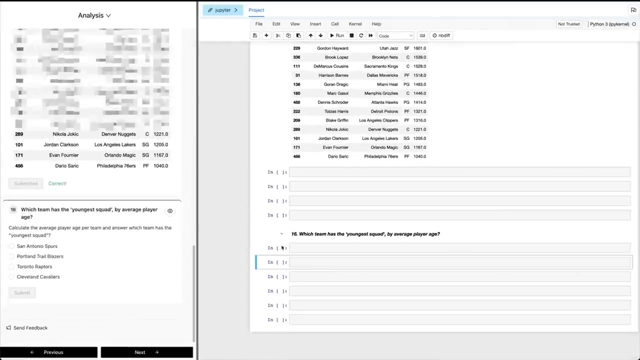 i'm i'm forgetting the most important column. we computed column, we computed column, we computed there, there, there, even, even, even, even it, it, it, the first one, the first one, the first one is going to well, let me show you first. is going to well, let me show you first. 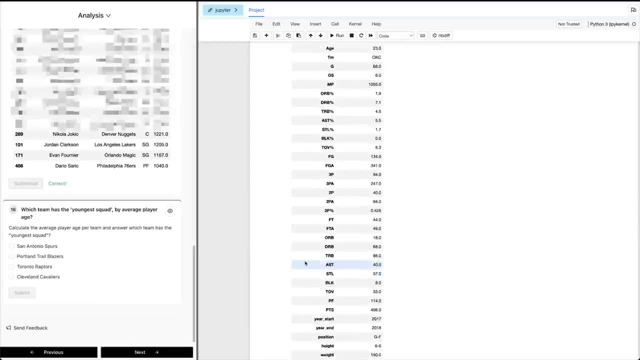 is going to. well, let me show you first how we we actually, how we we actually, how we we actually computed birth date as a daytime before, computed birth date as a daytime before, computed birth date as a daytime before. so this is from the players df. so this is from the players df. 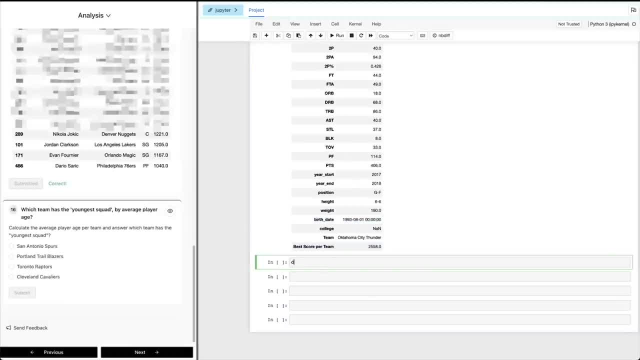 so this is from the players df: we turn into a birthday. this is we turn into a birthday. this is we turn into a birthday. this is very easily solved by doing um. i'm very easily solved by doing um. i'm very easily solved by doing um. i'm just giving you the answers right away. 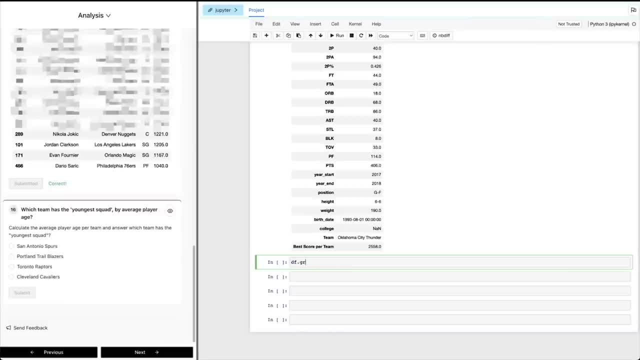 just giving you the answers right away. just giving you the answers right away: um df, um df, um df. dots. uh group by dots. uh group by dots. uh group by group by birth. uh team team group by birth. uh team team group by birth. uh team team at birthday. 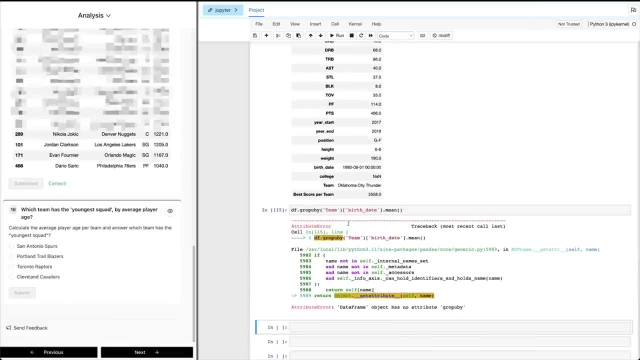 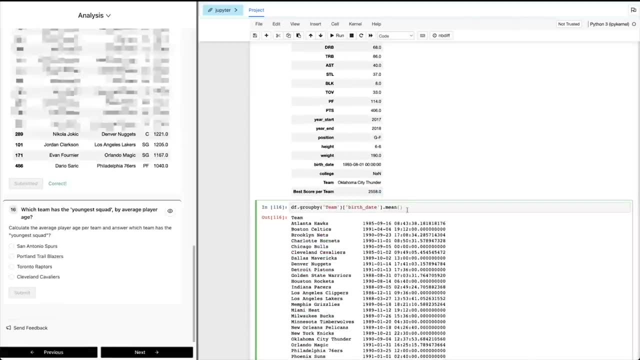 dot mean, dot mean, dot mean. and of course i made another typo here, and of course i made another typo here, and of course i made another typo here. group by, group by, group by, and let's just sort the values and let's just sort the values, and let's just sort the values um. 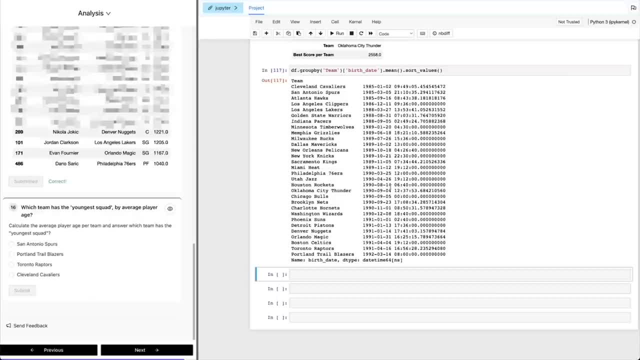 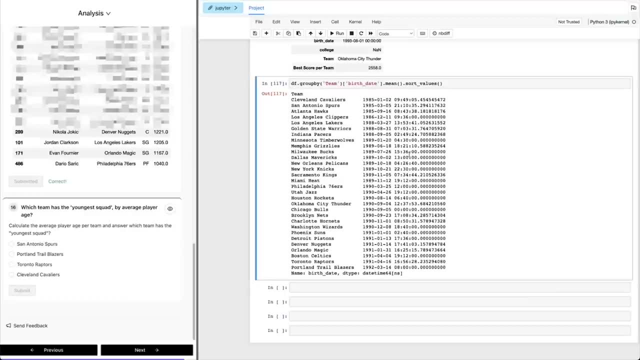 um, um, there, you, there, you, there you go, go um, and the interesting piece here: um, and the interesting piece here: um, and the interesting piece here. i don't know if you are noticing this. i don't know if you are noticing this. i don't know if you are noticing this right away, is that? 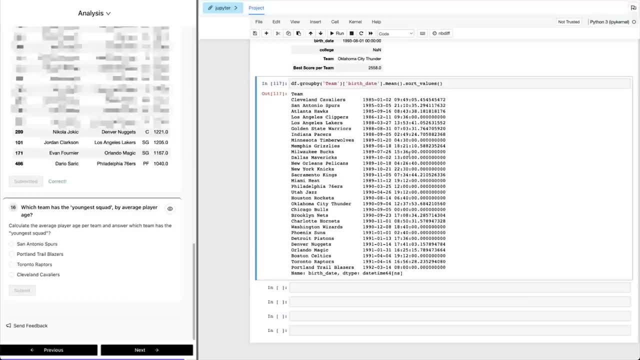 right away. is that right away? is that this operation that seems like a very this operation that seems like a very this operation that seems like a very mathematical operation of computing, the mathematical operation of computing. the mathematical operation of computing the average or the mean. average or the mean. 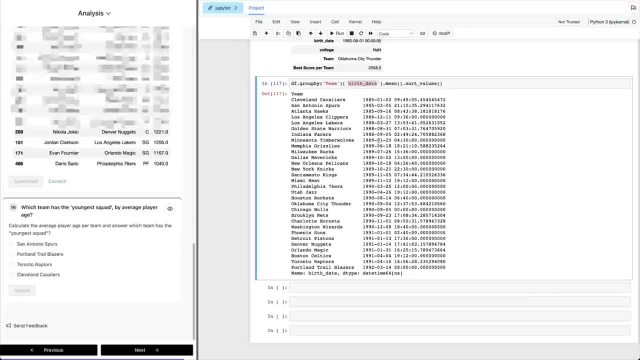 average or the mean, was actually applied to a daytime object. was actually applied to a daytime object. was actually applied to a daytime object. right? so that is right. so that is right. so that is that is pretty interesting, because day that is pretty interesting, because day that is pretty interesting, because day times. 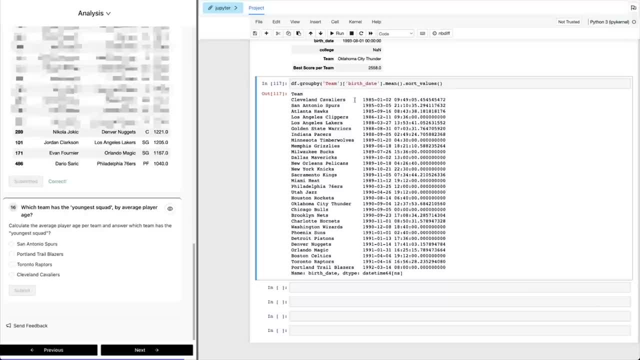 times times um are not numbers per se, they're just um are not numbers per se, they're just um are not numbers per se, they're just points in time, points in time, points in time. but basically what pandas is doing is. but basically what pandas is doing is. 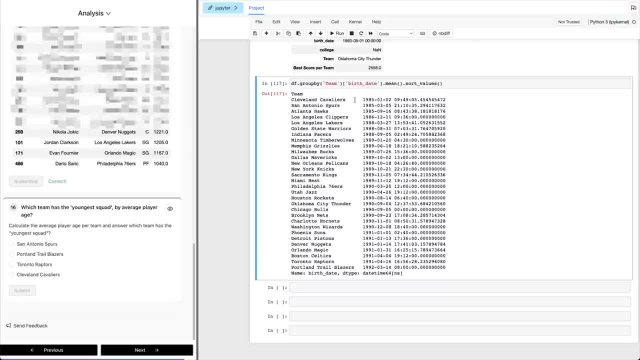 but basically what pandas is doing is finding, finding, finding that birthday it kind of in a timeline, that birthday it kind of in a timeline, that birthday it kind of in a timeline. i'm finally computing, i'm finally computing, i'm finally computing the, the mean, the, the mean. 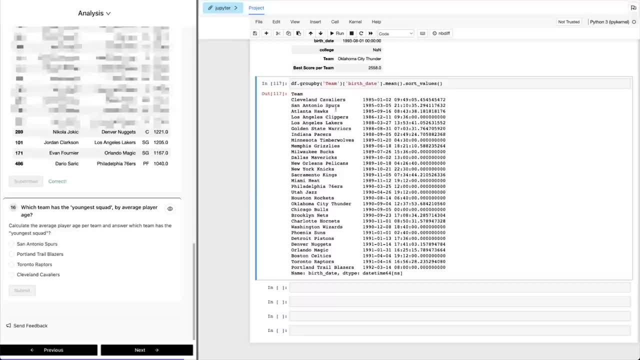 the, the mean, which is the youngest? which is the youngest, which is the youngest team? well, it's based. it's basically the team. well it's based. it's basically the team. well it's based. it's basically the team, team, team that has the greatest, that has the greatest. 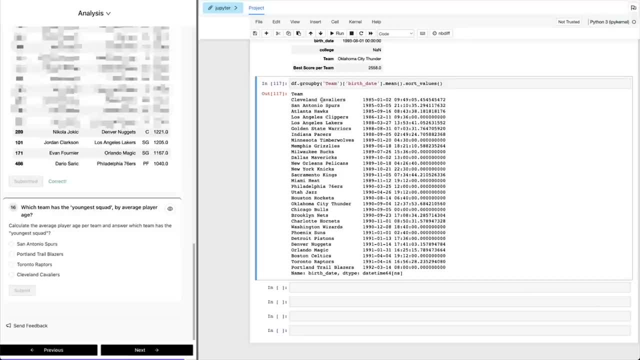 that has the greatest to put in a way, to put in a way, to put in a way the, the, the latest, the the latest, the the latest. birth date: right so 19, 22. birth date: right so 19, 22. birth date: right so 19, 22. oh, 3, 14 is the. 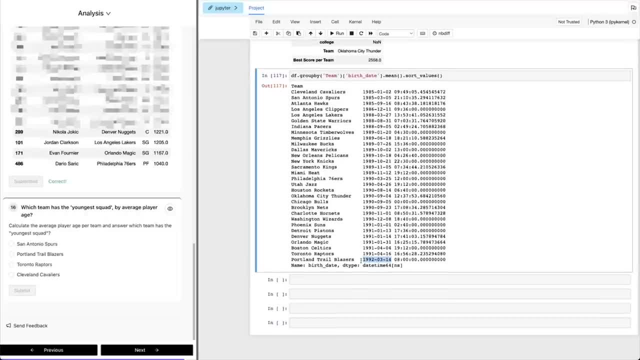 oh 3 14 is the oh 3, 14 is the? um latest date birth date, um latest date birth date. um latest date birth date mean um um birth date right. so if, if we do birth date right, so if, if we do birth date right, so if if we do something like 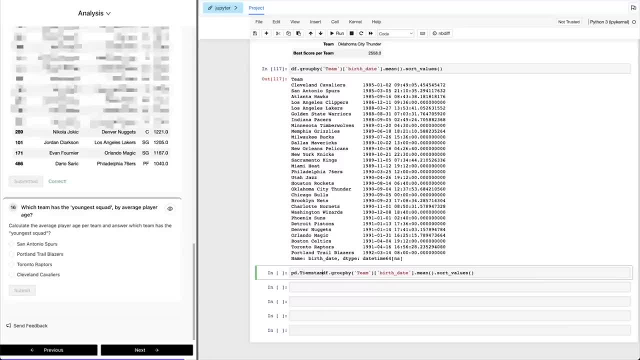 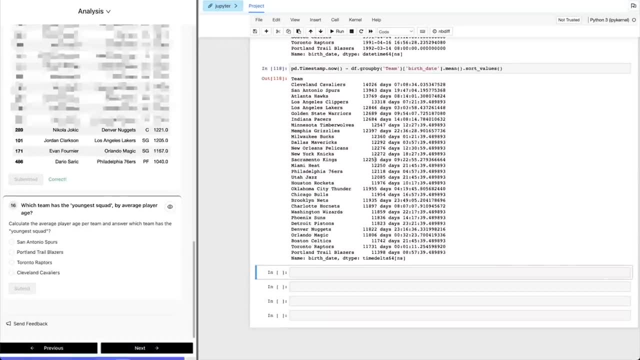 something like. something like like: let's, let's put this in in, like, let's, let's put this in in, like let's, let's put this in in timestamp dot now. timestamp dot now. timestamp dot- now, let's put this in. let's put this in. let's put this in in days, right. so basically, or: 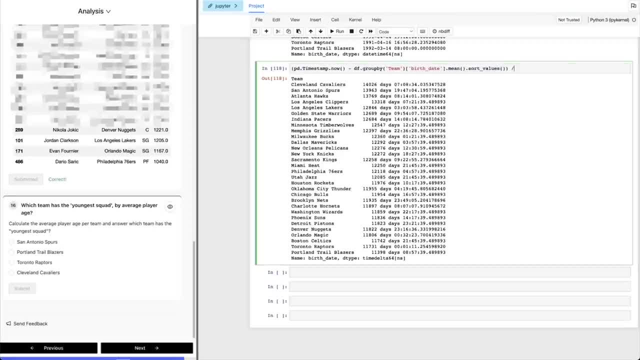 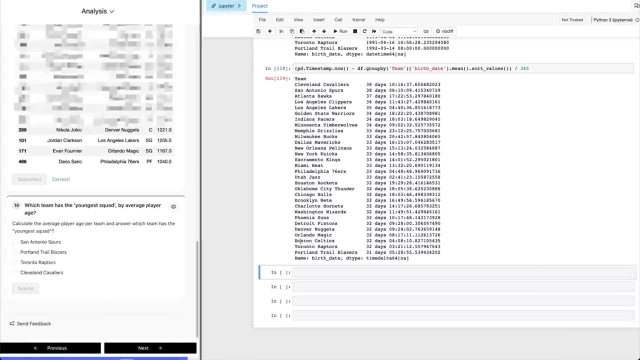 in days: right so, basically. or in days- right so basically, or actually. let's put this in years actually. let's put this in years actually. let's put this in years uh days. there you go, so the average uh days. there you go, so the average uh days. there you go, so the average age, and, of course, this is 2017. we can. 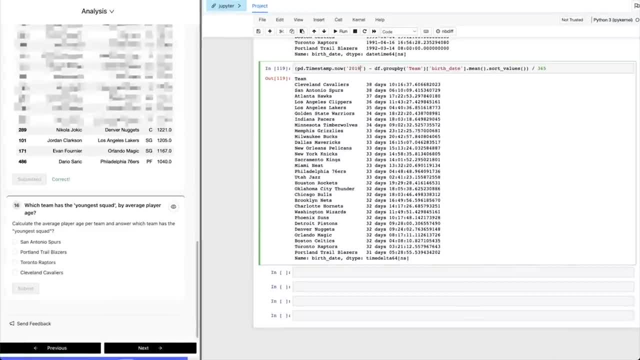 age and of course this is 2017. we can age and of course this is 2017. we can actually do that. we can say actually do that. we can say actually do that. we can say this to 2018 0101, this to 2018 0101. 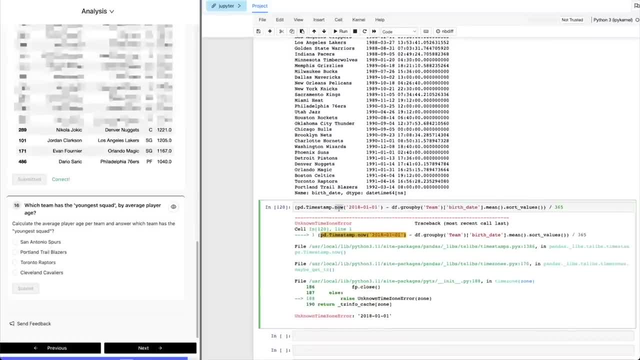 this to 2018. 0101 is the same thing. this doesn't change is the same thing. this doesn't change is the same thing. this doesn't change anything, anything, anything, uh timestamp there, uh timestamp there, uh timestamp there. so the, the, the team portland. so the the the team portland, so the the the team portland for the trail trailblazers. portland for the trail trailblazers. portland for the trail trailblazers portland has the youngest squad by average. has the youngest squad by average. has the youngest squad by average. right, because basically the average age. 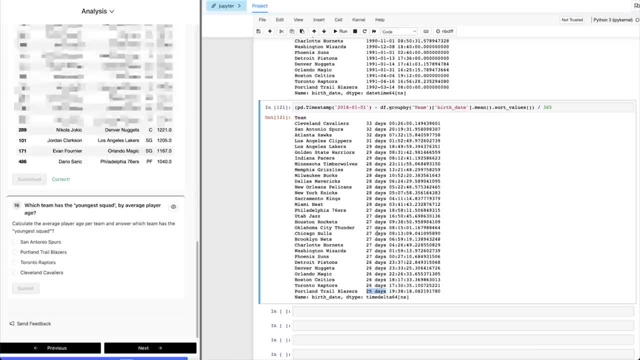 right because basically the average age, right because basically the average age was 25, was 25, was 25 years, not days because we're we're years, not days because we're we're years, not days, because we're we're dividing by 365.. dividing by 365.. dividing by 365.. so 25 years. so 25 years. so 25 years was the average. was the average, was the average age of the portland trailblazers and age of the portland trailblazers and age of the portland trailblazers. and two concepts here i want to separate in. 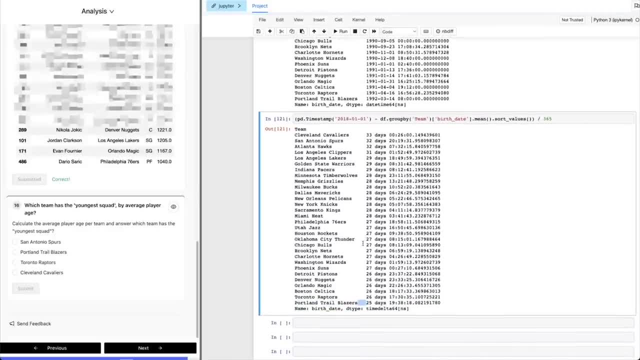 two concepts here. i want to separate in two concepts here. i want to separate in the first one and sorry the second one. the first one and sorry the second one. the first one and sorry the second one that i mentioned. that i mentioned. that i mentioned was that we are here finding the 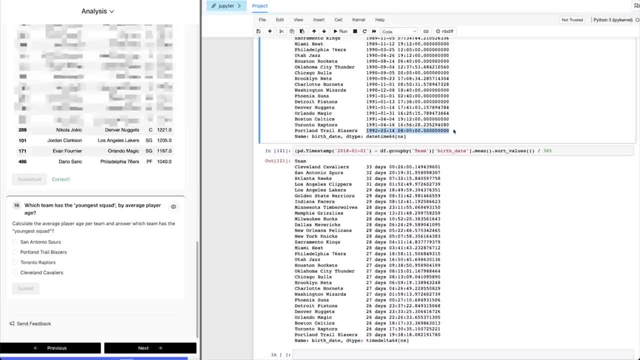 was that we are here finding the was that we are here finding the youngest team. that's basically the youngest team. that's basically the youngest team. that's basically the greatest, greatest, greatest. date right. if i was born in, i was born. date right: if i was born in, i was born. 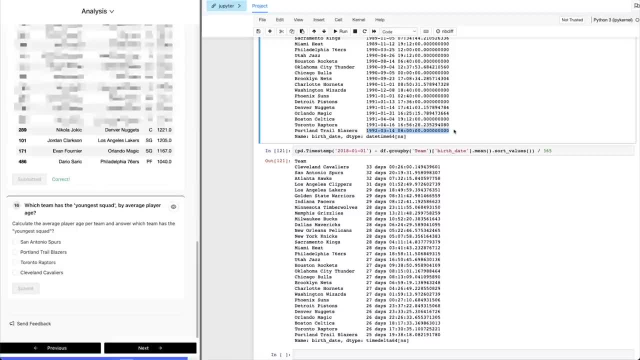 date: right if i was born in. i was born in in in 1987. my brother was born in 1992, 1987. my brother was born in 1992, 1987. my brother was born in 1992. he has a newer. he has a newer. 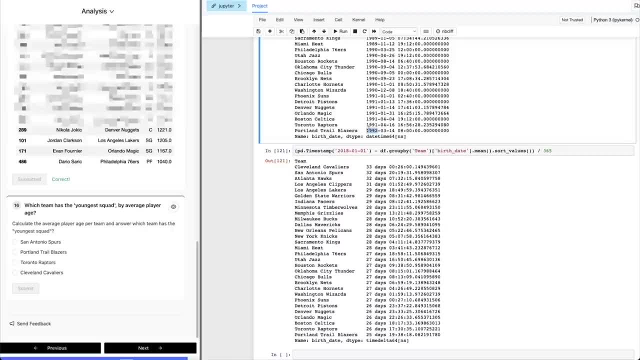 he has a newer birth date right- most more recent birth date right most more recent birth date right most more recent. but that makes him younger, right i? but that makes him younger, right i. but that makes him younger, right i. have a an older, have a an older. 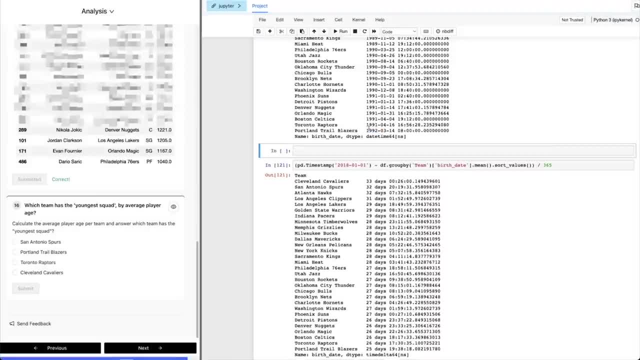 have a an older date date: a lower value right 1987 date date: a lower value right 1987 date date a lower value right 1987 is lower than 1992, but that makes that is lower than 1992, but that makes that. 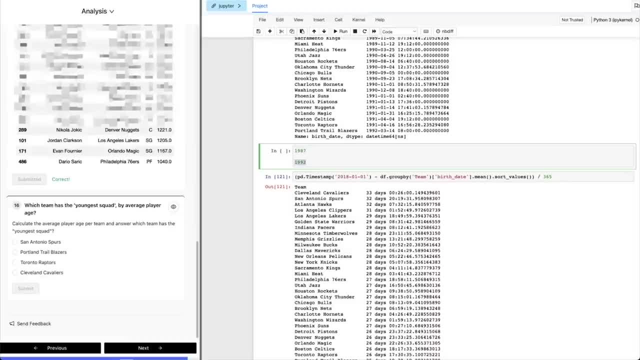 is lower than 1992. but that makes that makes me, makes me, makes me older. that makes him younger, right, that's older. that makes him younger, right, that's older. that makes him younger, right, that's. that's the second thing that i mentioned. that's the second thing that i mentioned. 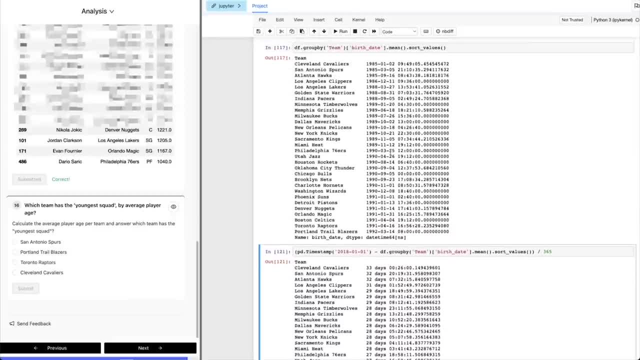 that's the second thing that i mentioned very quickly, very quickly, very quickly. the first thing which is the most, the first thing which is the most, the first thing which is the most important one, important one, important one, is that let's get rid of. that is that. 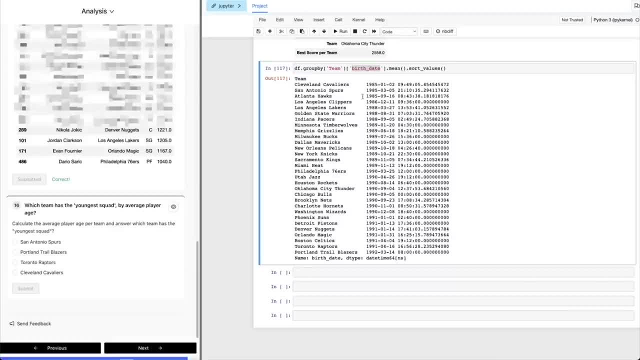 is that let's get rid of. that is that is that let's get rid of. that is that the birth date column is a. the birth date column is a. the birth date column is a daytime and we correctly daytime and we correctly daytime and we correctly had a mean competed for that will be. 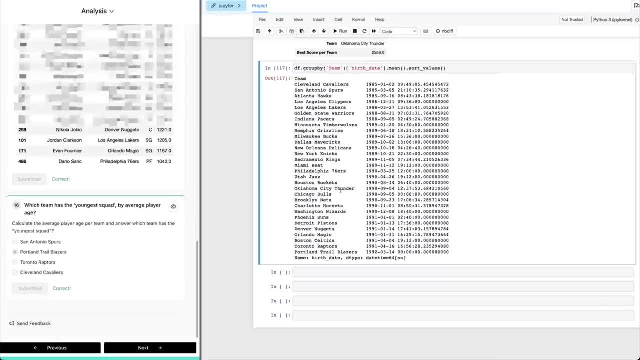 had a mean competed for, that will be. had a mean competed for. that will be the alternative. and actually, let's try the alternative, and actually let's try the alternative and actually let's try the activity, the activity, the activity that works. what is the the alternative that works? what is the the alternative? 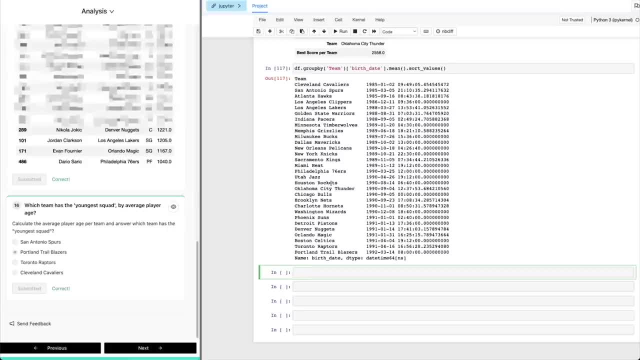 that works. what is the? the alternative- and i think we have that listed in the, and i think we have that listed in the, and i think we have that listed in the solution solution. solution is: let's say this didn't exist, well, we is. let's say this didn't exist, well, we. 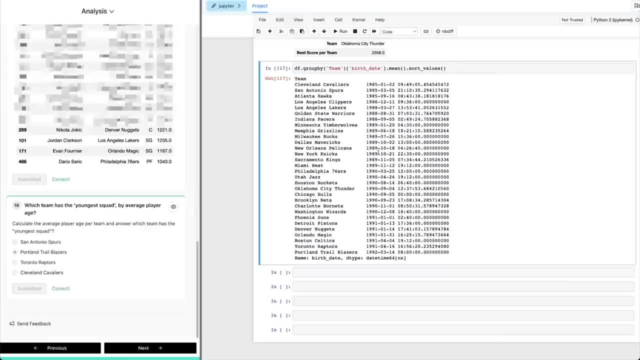 is, let's say, this didn't exist. well, we basically need to transform the, basically need to transform the basically need to transform the. let's say dates, um, we can say let's say dates, um, we can say let's say dates, um, we can say age in days. we have to transform this. 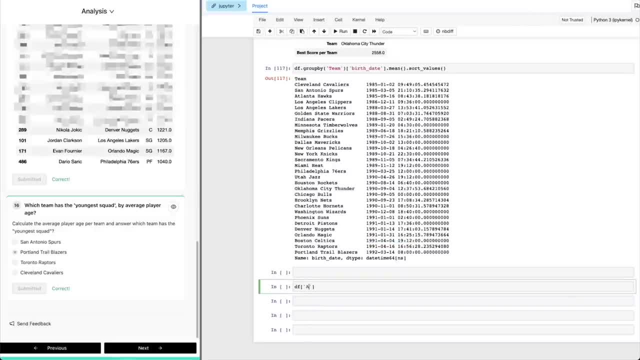 age in days. we have to transform this age in days. we have to transform this thing from a date to a number so we can thing from a date to a number, so we can thing from a date to a number, so we can say: say, say the f at age in days and we can say: 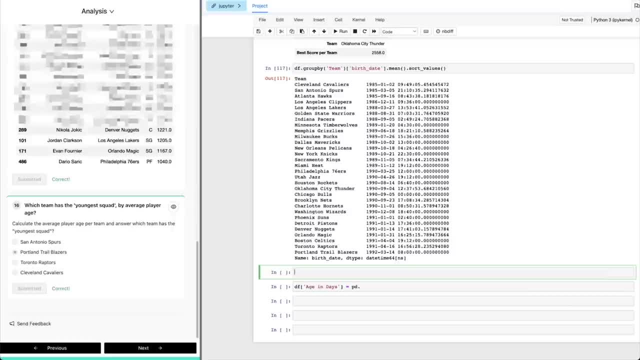 the f at age in days and we can say the f at age in days and we can say pd. let's actually let me actually show you pd. let's actually let me actually show you pd. let's actually let me actually show you the, the result. first the f at um. 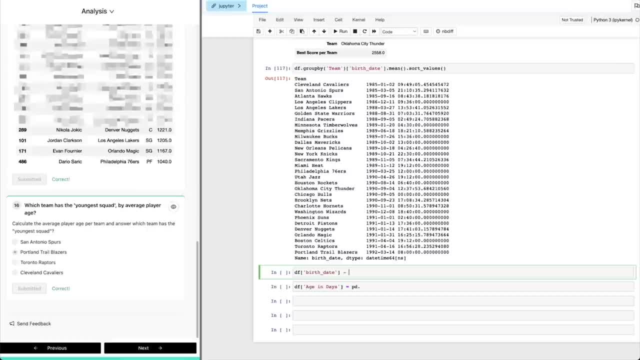 the the result first the f at um. the the result first the f at um. birth date, birth date: birth date um minus, or actually the other way: pd dot um minus, or actually the other way pd dot um minus or actually the other way: pd dot timestamp. we said: 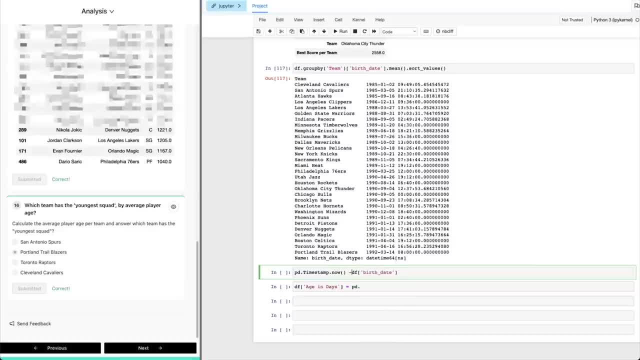 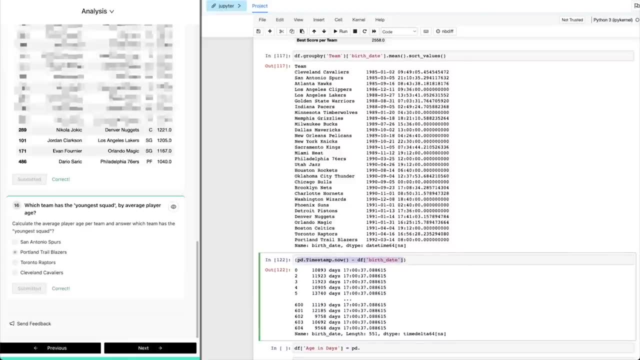 timestamp. we said timestamp, we said um, um, um, dot now, dot now, dot now, minus that, minus that, minus that, that gives you a time delta. that gives you a time delta. that gives you a time delta. that's the the name of the value pandas. that's the the name of the value pandas. 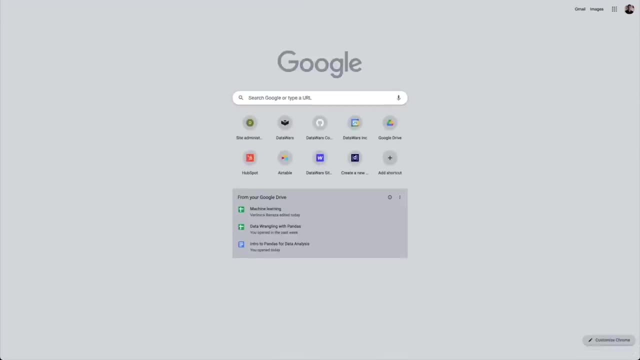 that's the the name of the value pandas. time delta. i'm gonna. time delta. i'm gonna time delta, i'm gonna. i'm googling it real quick. i'm googling it real quick. i'm googling it real quick and we can find a time delta. it's just. 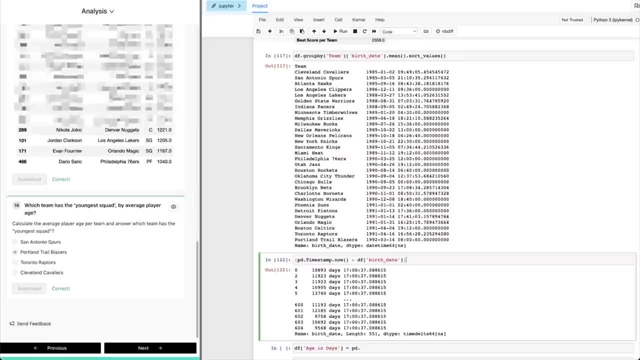 and we can find a time delta. it's just, and we can find a time delta. it's just a relative duration of time, a relative duration of time, a relative duration of time, um, and that is the time delta and we. um, and that is the time delta and we. 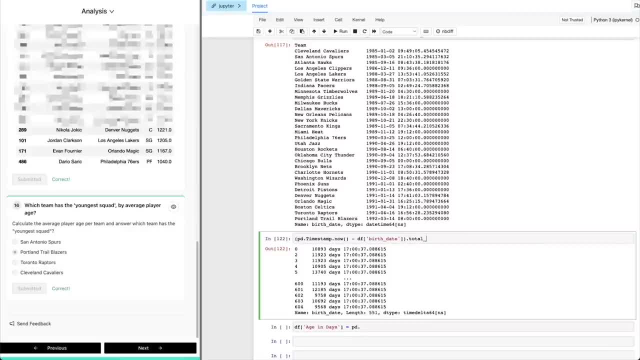 um, and that is the time, delta. and we can get, for example, to be very precise. we can get, for example, to be very precise. we can get, for example, to be very precise. we can get total, can get total, can get total seconds, seconds, seconds, right, um, right, um. 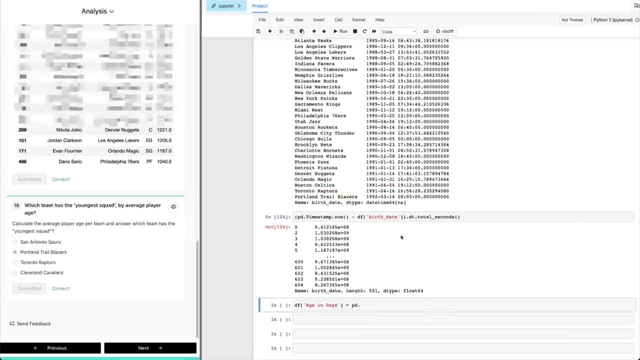 right, um. total seconds. dt. total seconds. dt. total seconds. dt. total seconds, total seconds, total seconds. or we can get something like days, or we can get something like days, or we can get something like days, and here what i'm doing is a dt and here what i'm doing is a dt. 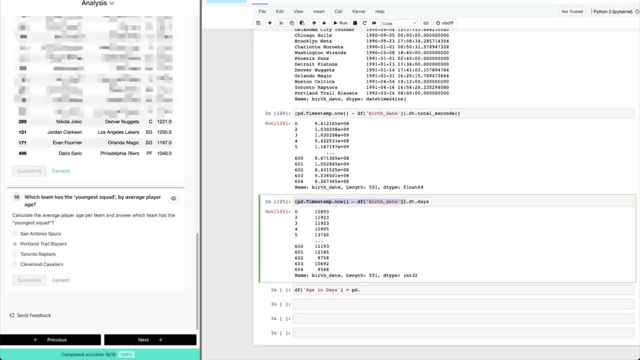 and here what i'm doing is a dt daytime accessor, so daytime accessor, so daytime accessor. so if a, if a, if a pandas series, pandas series, pandas series- a column in a data frame is of time, if a a column in a data frame is of time, if a 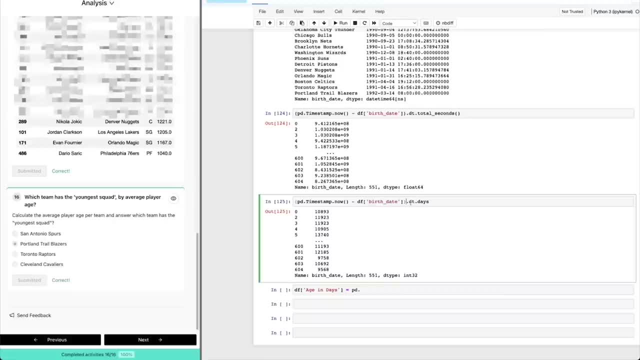 a column in a data frame is of time if a is a daytime or a time, delta is a daytime or a time. delta is a daytime or a time delta. it has a special accessor dot dt. it has a special accessor dot dt. it has a special accessor dot dt that lets you perform some daytime. 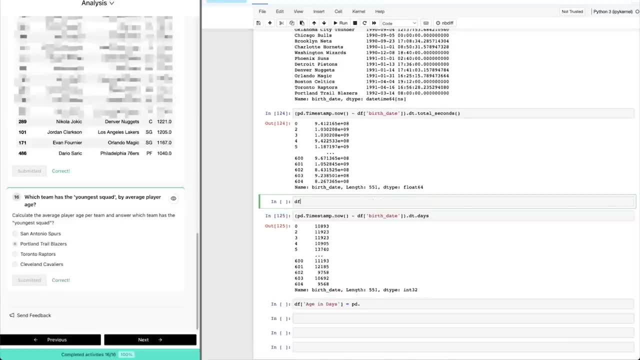 that lets you perform some daytime. that lets you perform some daytime calculation on it, similar as with uh for calculation on it. similar as with uh for calculation on it. similar as with uh, for example: df. example. df. example. df. team dot str. we have the str accessor. team dot str. we have the str accessor. 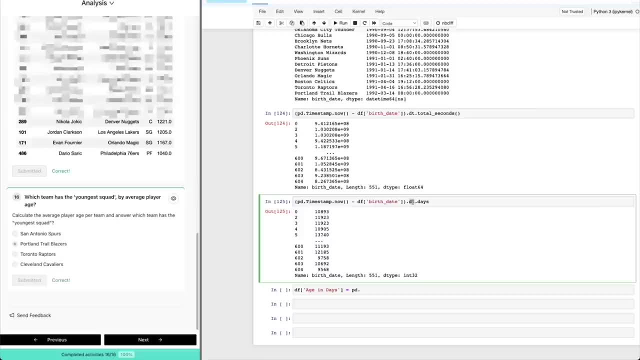 team dot str. we have the str accessor for for for string columns. we have the dt accessor string columns. we have the dt accessor string columns. we have the dt accessor for daytime and time delta columns, or for daytime and time delta columns, or for daytime and time delta columns or series. 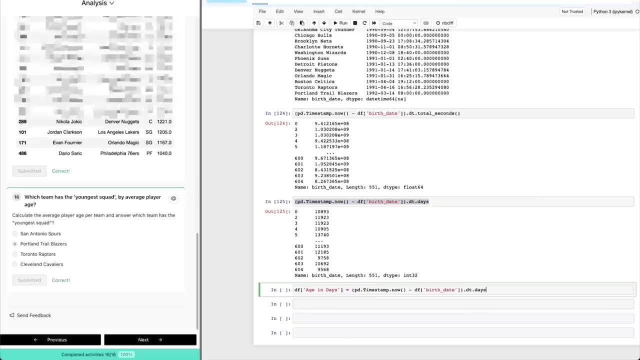 series, series. so anyway we can say um this thing. so anyway we can say um this thing. so anyway we can say um this thing age in, age in, age in. we probably will not say it, so we say we. we probably will not say it, so we say we. 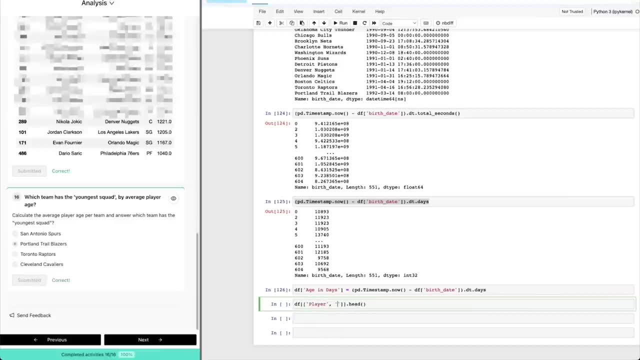 we probably will not say it. so we say we say say say player, we say um player, we say um player, we say um birth dates, birth dates, birth dates. and we are going to say age in days and we are going to say age in days and we are going to say age in days: birth. 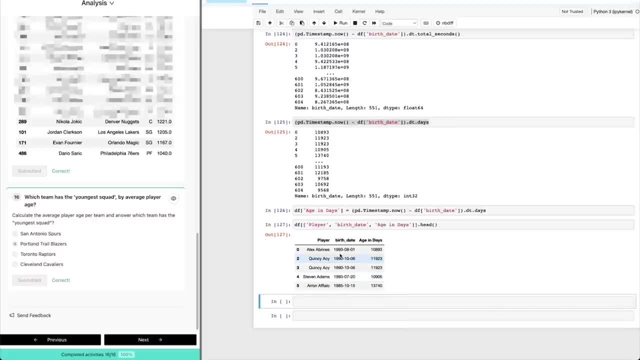 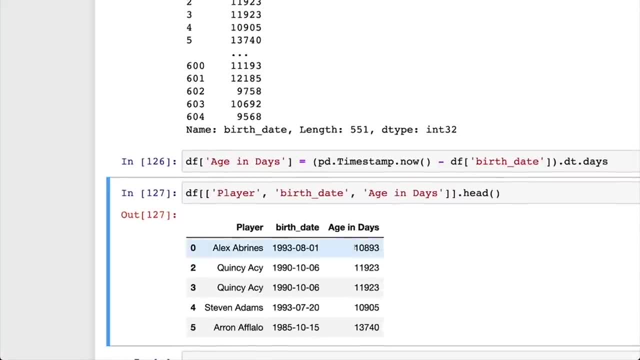 0801, so august 1st is 0801, so august 1st is 10 899, 10 899, 10 899, 893 days old, 893 days old, 893 days old. so now we have transformed the daytime. so now we have transformed the daytime. 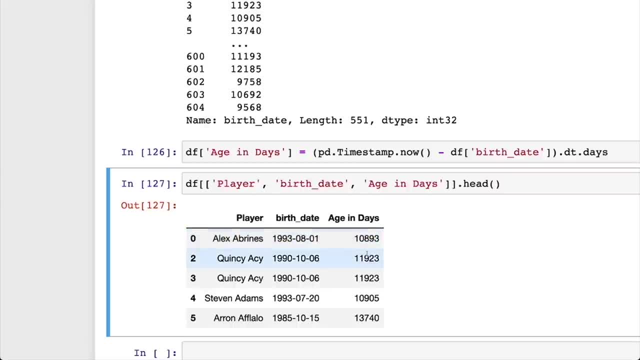 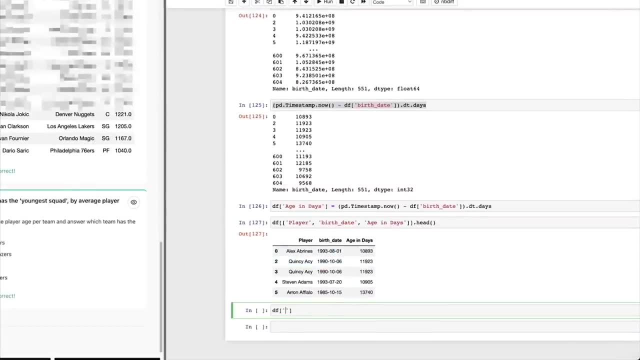 so now we have transformed the daytime back into a back, into a back into a numeric column, and we can now compute numeric column. and we can now compute numeric column and we can now compute the um, the um, the um, the average age. so we can say the average age. so we can say: 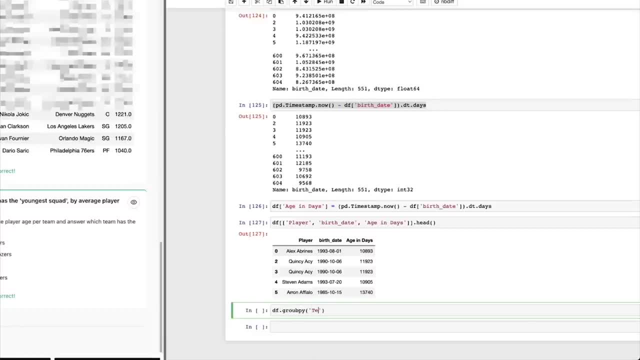 the average age. so we can say group by group by group, by same same, same, same, same thing, thing, thing, team, team, team. at age in days at age, in days at age in days: uh dot min, uh, dot min, uh dot min, sort values, sort values, sort values. and i did something wrong, as usual, 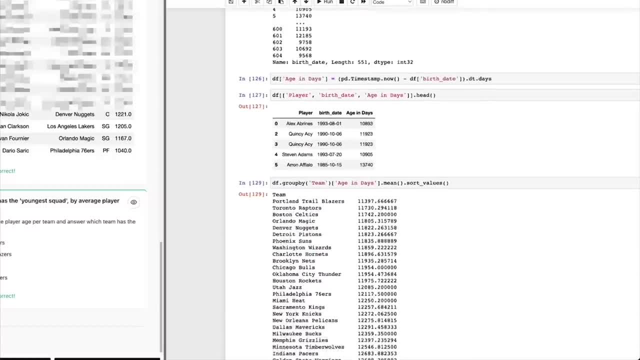 and i did something wrong as usual. and i did something wrong as usual group. i don't know why i have so many group. i don't know why i have so many group. i don't know why i have so many issues with this group by the name. 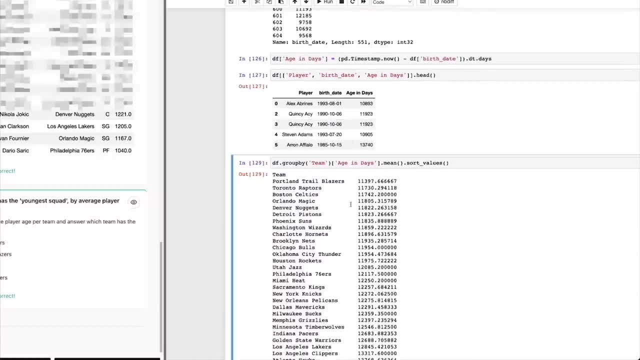 issues with this group by the name, issues with this group by the name, and now what you can see is that we, and now what you can see is that we, and now what you can see is that we actually have to think, actually have to think, actually have to think. the result in an opposite direction. now 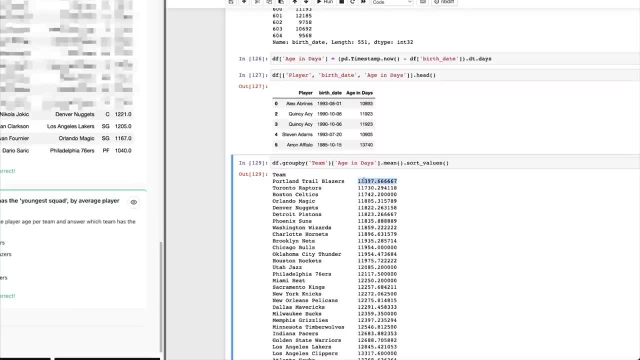 the result in an opposite direction. now the result in an opposite direction. now the lowest value, the lowest value, the lowest value is the youngest one. of course the is the youngest one. of course the is the youngest one. of course the previous one was the previous one was the. 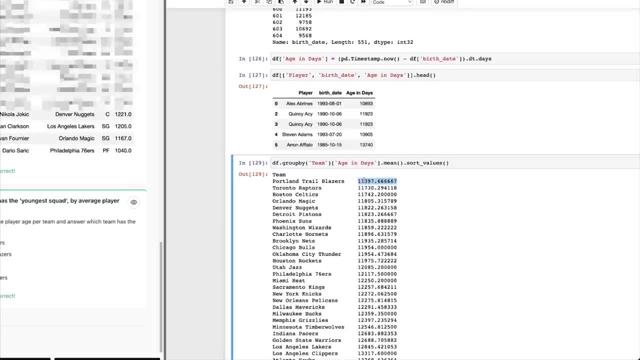 previous one was the. the, the date, the most recent date. the, the date the most recent date. the, the date, the most recent date, gave us the youngest um team, gave us the youngest um team, gave us the youngest um team, now the team with the lowest age in. now the team with the lowest age in now. the team with the lowest age in days is, of course, the youngest team. days is, of course, the youngest team. days is, of course, the youngest team. that's basically what we're finding. that's basically what we're finding. 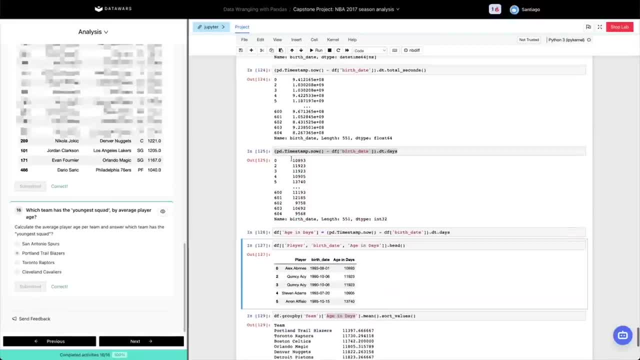 that's basically what we're finding right here, and we have let me clear this right here, and we have let me clear this right here and we have let me clear this whole thing, whole thing, whole thing. so we can compare uh, birth date and these aging days. we 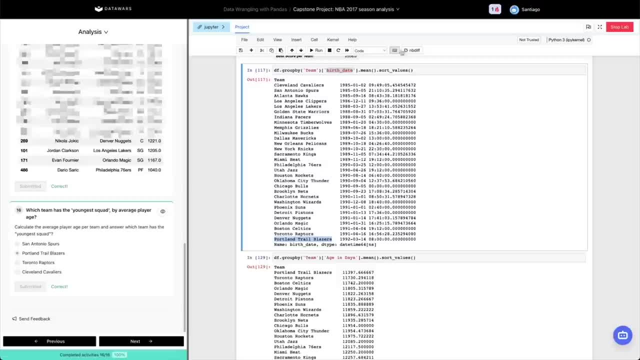 uh birth date and these aging days. we uh birth date and these aging days. we have the same, have the same, have the same results. ideally portland, let me actually results. ideally portland, let me actually results. ideally portland, let me actually sorted, sorted, sorted sword um ascending. 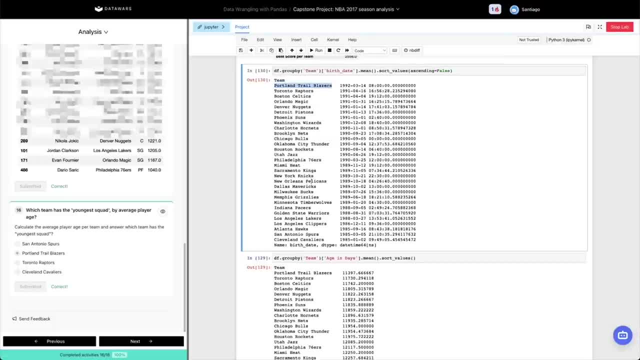 sword um ascending sword um ascending falls. so we compare the values and we falls. so we compare the values and we falls. so we compare the values and we have portland, portland, toronto, toronto, have portland, portland, toronto, toronto, have portland, portland, toronto, toronto, boston, boston, orlando, orlando. so it's. 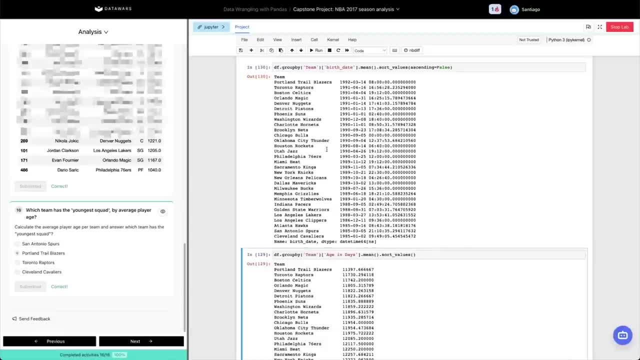 boston, boston, orlando, orlando. so it's boston, boston, orlando, orlando. so it's the same, the same, the same value for both. i think the interesting value for both. i think the interesting value for both. i think the interesting takeaway here is how pandas implements. 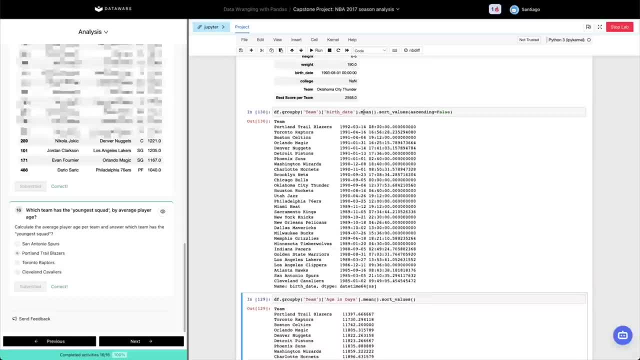 takeaway here is how pandas implements. takeaway here is how pandas implements all these useful daytime, all these useful daytime, all these useful daytime, modifications, modifiers, methods and modifications, modifiers, methods and modifications, modifiers, methods and even these operations. i think that's the even these operations. i think that's the. 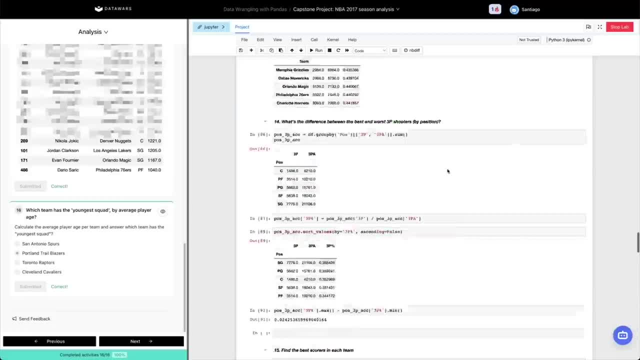 even these operations. i think that's the most interesting piece so far, most interesting piece so far, most interesting piece so far. so again, wrapping it up, this project, so again wrapping it up this project. so again wrapping it up this project. extremely interesting because we did, extremely interesting because we did. 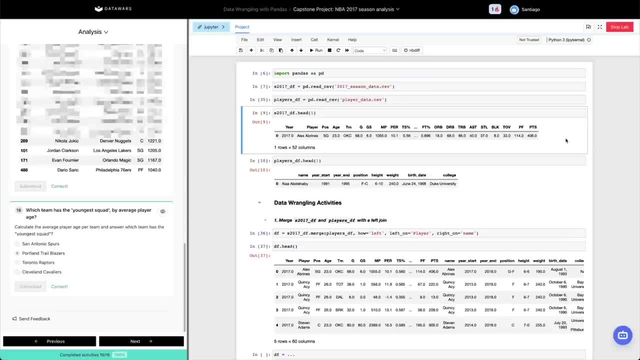 extremely interesting because we did pretty much the full cycle. we pretty much the full cycle, we pretty much the full cycle. we got the data, we merged it. we identified: got the data, we merged it. we identified: got the data, we merged it. we identified invalid values using this detective. 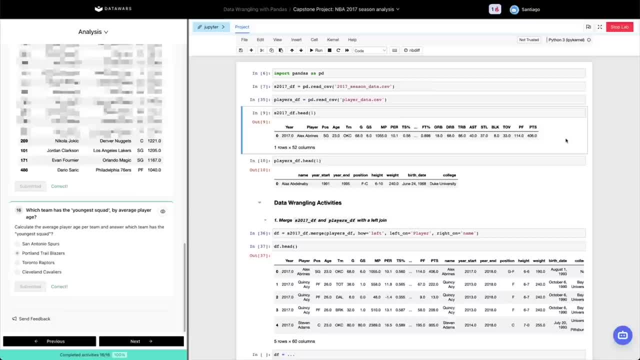 invalid values using this detective invalid values using this detective work. finding what happened work. finding what happened work. finding what happened. rewinding time. we did some googling. rewinding time, we did some googling. rewinding time. we did some googling. we finally did some cleaning transform. 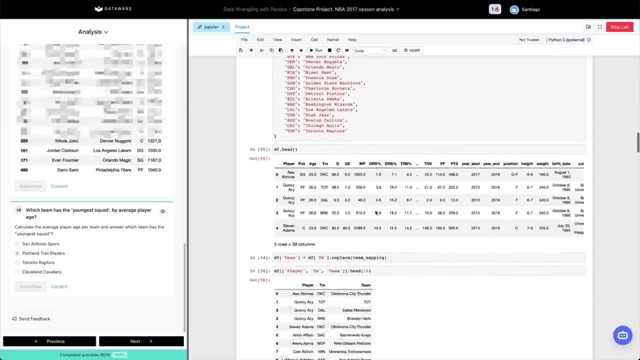 we finally did some cleaning, transform. we finally did some cleaning, transform data types like birth date, data types like birth date, data types like birth date. then we did um all these, then we did um all these, then we did um all these. you know munging of the data. there you go. 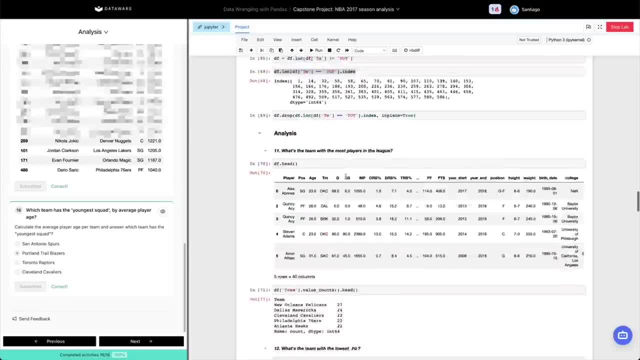 you know munging of the data, there you go. you know munging of the data, there you go. deleting, deleting, deleting. these totals understanding data. we were these totals understanding data, we were these totals understanding data. we were working with and finally we did all working with and finally we did all. 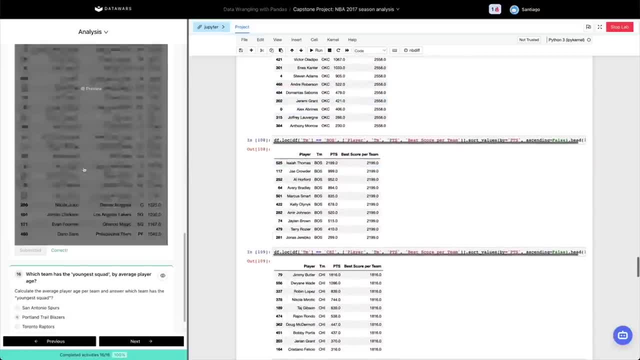 working with and finally, we did all these analysis, these analysis, these analysis. my favorite activity is by far the number. my favorite activity is by far the number. my favorite activity is by far the number. 15 one with the transform method. 15 one with the transform method. 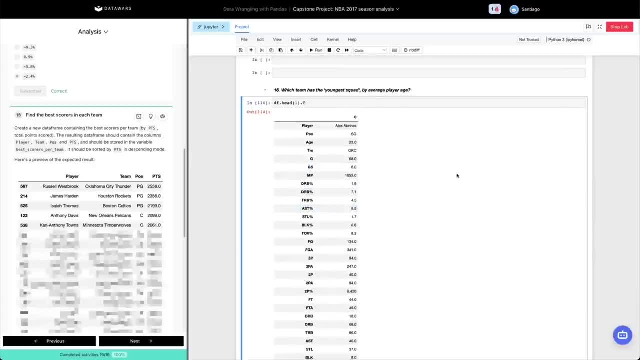 15, one with the transform method, extremely useful method. so, if you want extremely useful method, so if you want extremely useful method, so if you want to replay it, to replay it, to replay it. just you know, try to solve it by yourself. just you know, try to solve it by yourself. 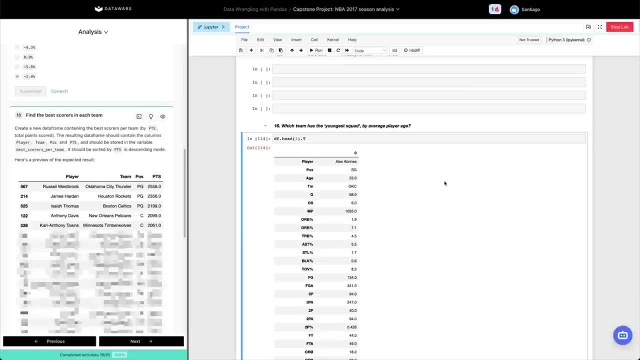 just, you know, try to solve it by yourself. and i think i think this project and i think i think this project and i think i think this project represents very well the whole process, represents very well, the whole process represents very well the whole process of data science, data, rumbling data. 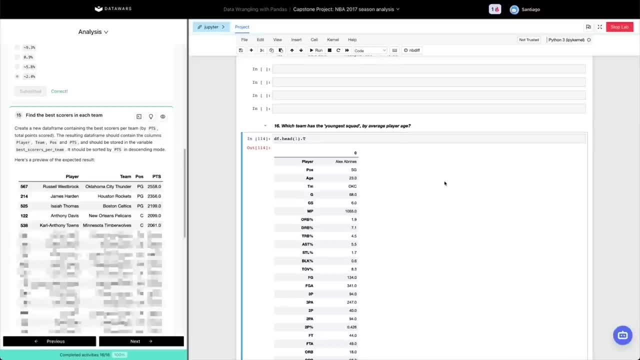 of data science: data rumbling. data of data science. data rumbling, data. munging data engineering. munging data engineering. munging data engineering. everything you're gonna find in a in a. everything you're gonna find in a in a. everything you're gonna find in a in a regular project dealing with data. regular project dealing with data. 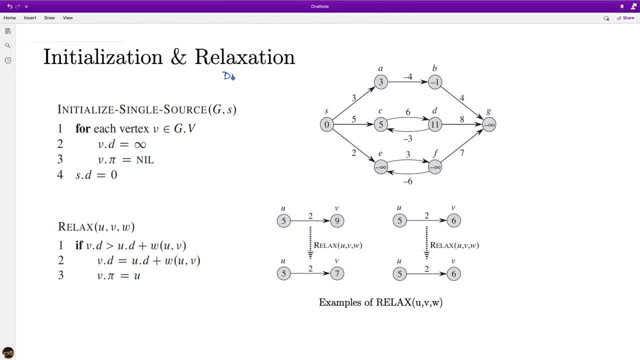 Two common operations for running the Dijkstra's algorithm and the Bellman-Ford algorithm are the initialized single source and the relaxed operation. So let's see what these two operations do Say. we have a graph like this, a directed graph, and we are interested in finding the shortest path from this vertex S to all other vertices. 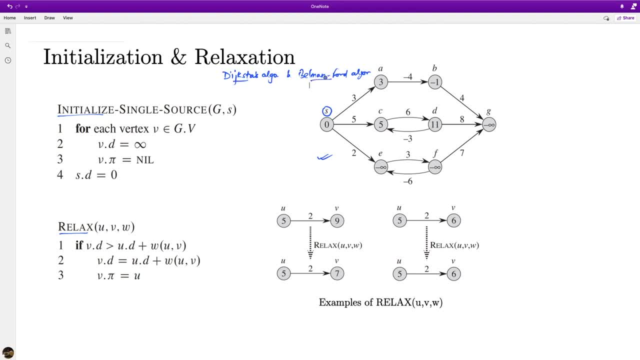 So, before we run either Dijkstra's algorithm or Bellman-Ford algorithm, we first assume that every node in this graph has two attributes. The first attribute is D and the second attribute is pi. What this attribute D is, it's an estimate of the shortest path. 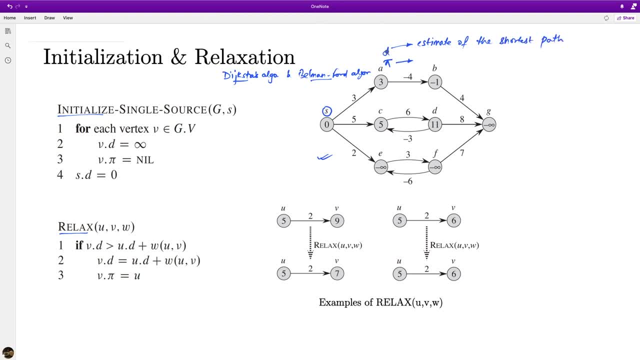 And this attribute, pi, is the parent node or predecessor attribute. Now, before running either of these two algorithms, we first want to assume that the shortest path estimate for each of these vertices. so I maintain D and pi for each vertex. D and pi for each vertex. and we assume that or we set.